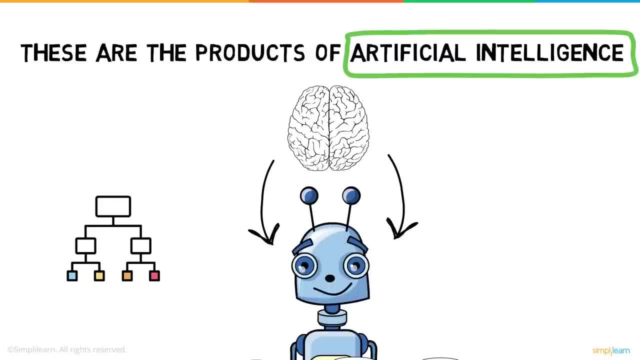 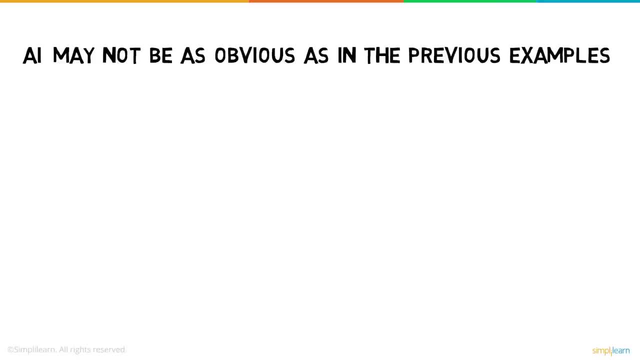 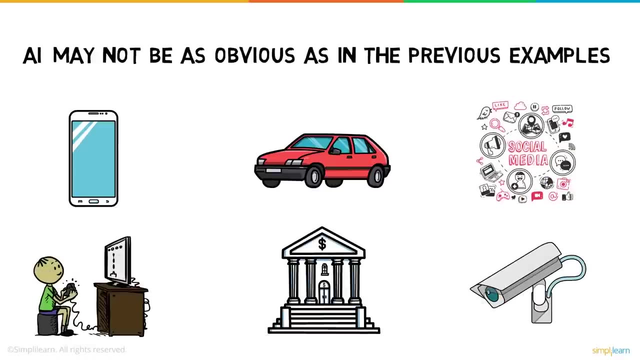 This intelligence is built using complex algorithms and mathematical functions, But AI may not be as obvious as in the previous examples. In fact, AI is used in smartphones, cars, social media feeds, video games, banking surveillance and many other aspects of our daily. 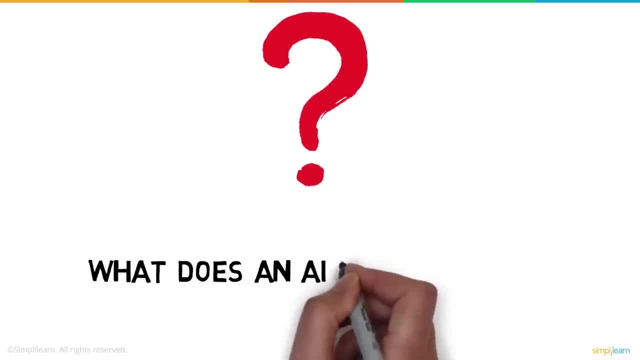 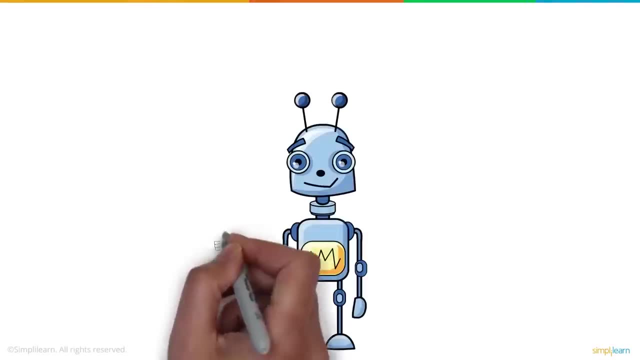 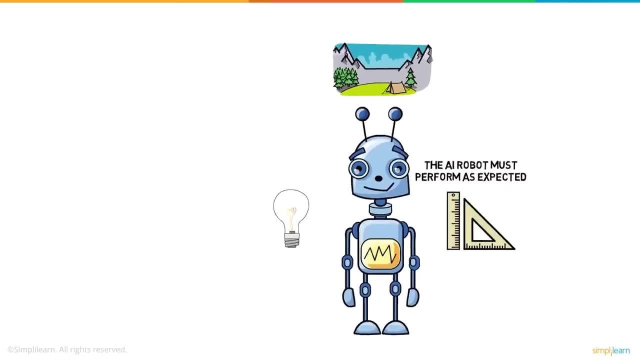 life. The real question is: what does an AI do at its core? Here is a robot we built in our lab, which is now dropped onto a field. In spite of a variation in lighting, landscape and dimensions of the field, the AI robot must perform as expected: This ability to react appropriately to a new situation. 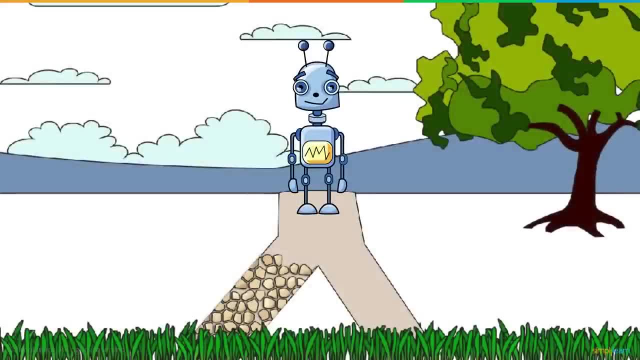 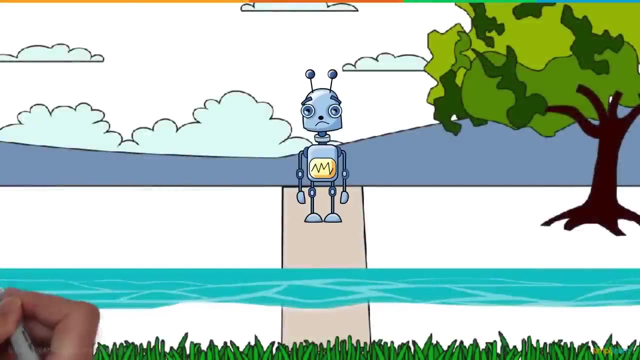 is called generalized learning. The robot is now at a crossroad, one that is paved and the other rocky. The robot must determine which path to take based on the circumstances. This portrays the robot's reasoning ability. After a short stroll, the robot 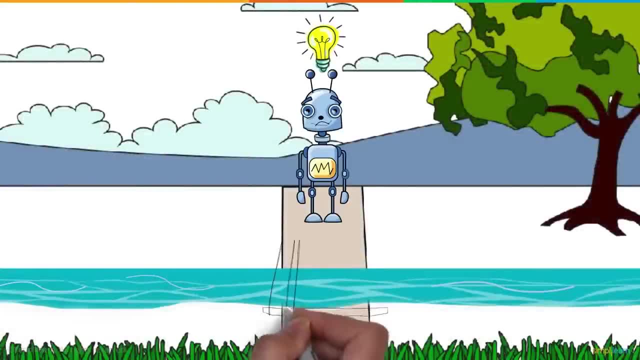 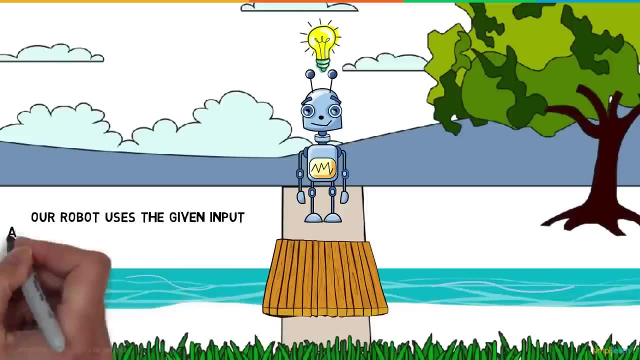 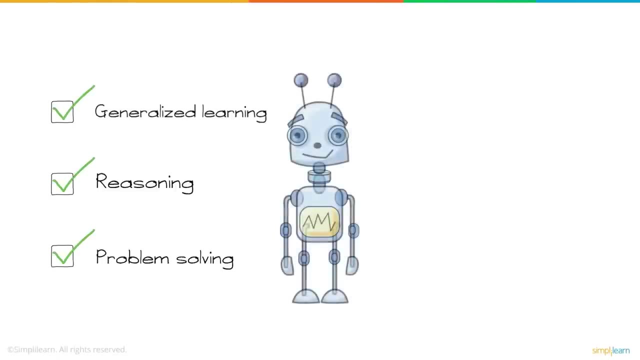 encounters a stream that it cannot swim across. Using the plank given as an input, the robot is able to cross this stream. So our robot uses the given input and finds the solution for a problem. This is problem solving. These 3 capabilities make the robot. 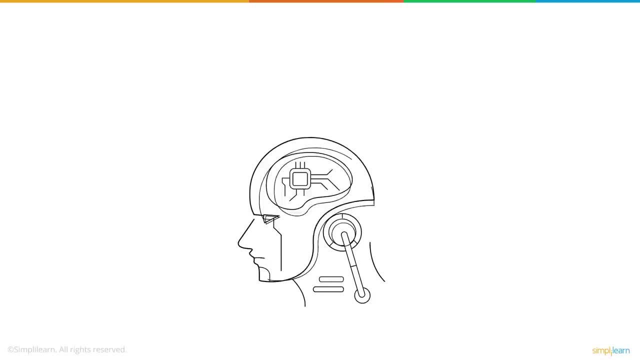 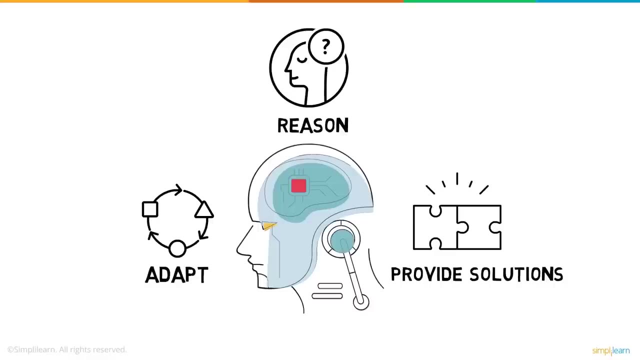 artificially intelligent. In short, AI provides machines with the capability to adapt, reason and provide solutions. Well, now we know where the AI goes. Let's día down immediately so that we may go to the base point. we know what AI is. let's have a look at the two broad categories an AI is classified into. 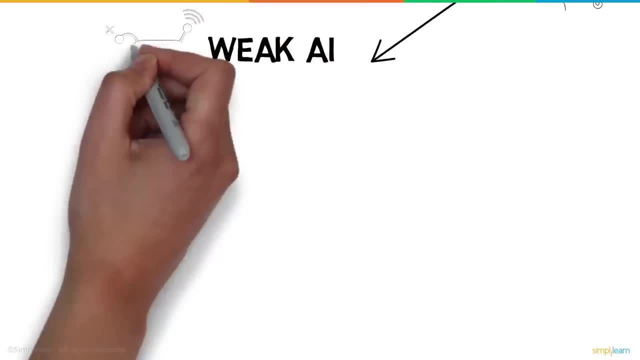 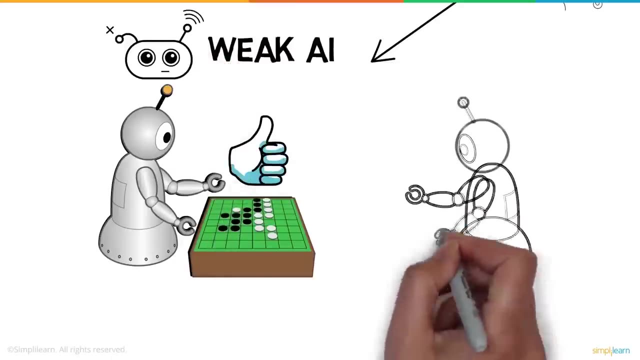 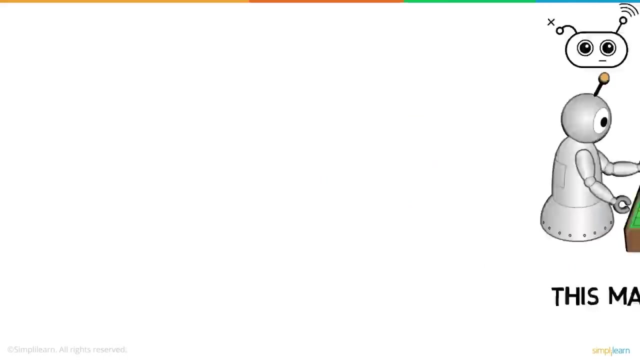 Weak AI, also called narrow AI, focuses solely on one task. For example, AlphaGo is a maestro of the game Go, but you can't expect it to be even remotely good at chess. This makes AlphaGo a weak AI. You might say Alexa is definitely not a weak AI, since it can perform multiple tasks. 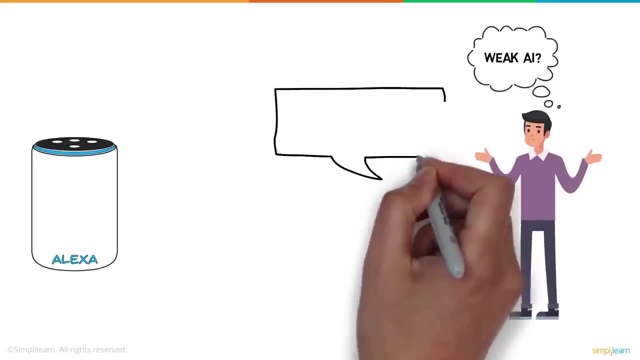 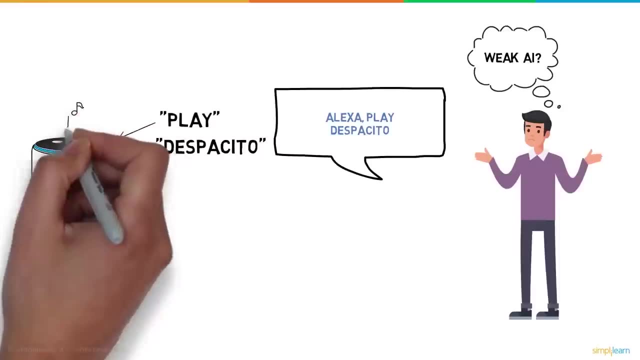 Well, that's not really true. When you ask Alexa to play Despacito, it picks up the keywords Play and Despacito and runs a program it is trained to. Alexa cannot respond to a question it isn't trained to answer. For instance, try asking Alexa the status of traffic from work to home. 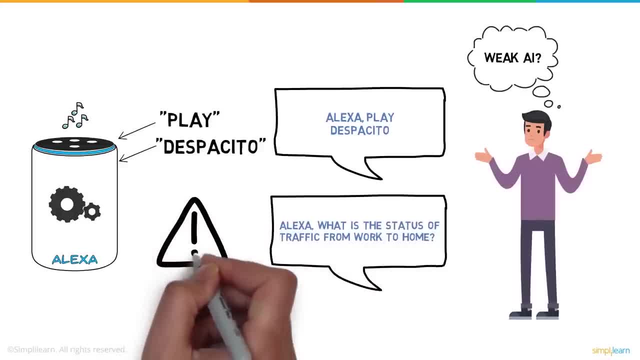 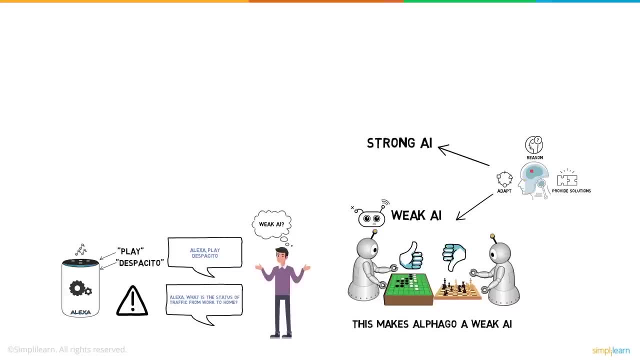 Alexa cannot provide you this information, as she is not trained to. And that brings us to our second category of AI: Strong AI. Now, this is much like the robots that only exist in fiction as of now. Ultron from Avengers is an ideal example of a strong AI. 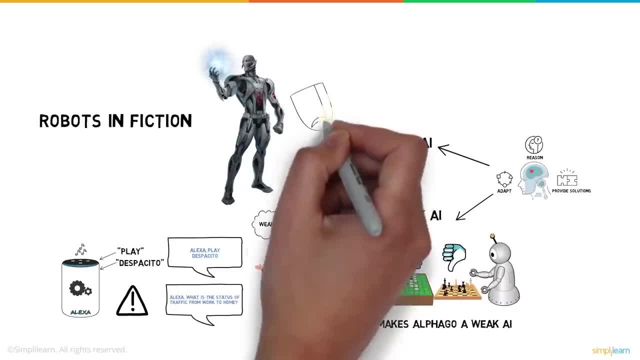 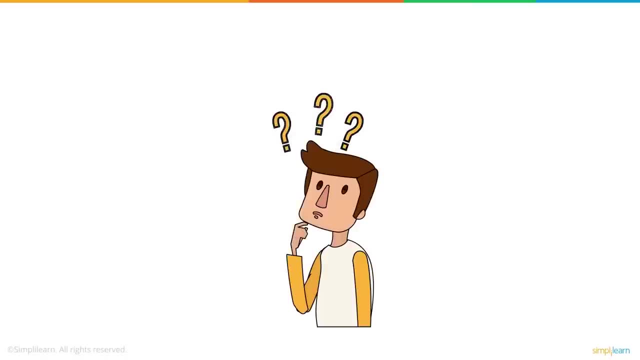 That's because it's self-aware and eventually even develops emotions. This makes the AI's response unpredictable. You must be wondering well, how is Artificial Intelligence different from machine learning and deep learning? We saw what AI is – machine learning, machine learning, artificial intelligence and deep learning. And now let's go see what AI is. 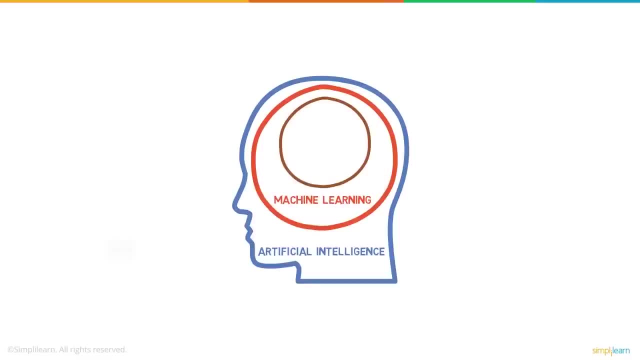 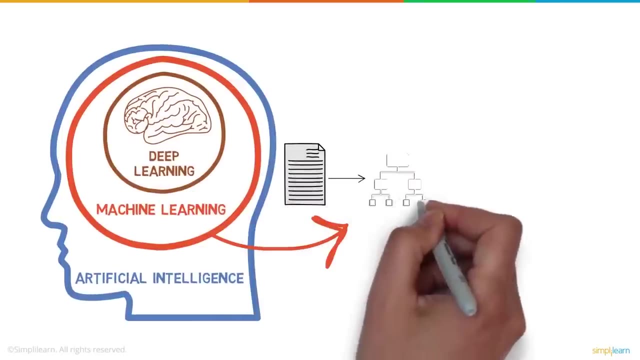 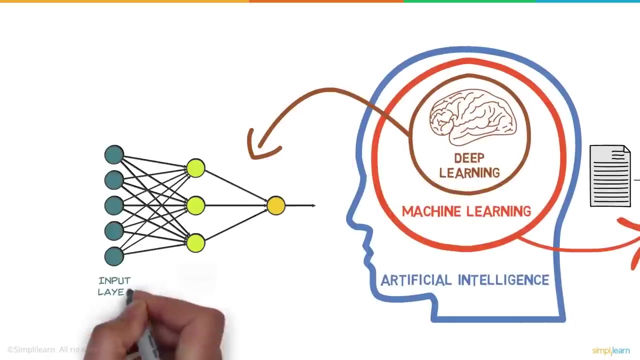 Machine learning is a technique to achieve AI, and deep learning, in turn, is a subset of machine learning. Machine learning provides a machine with the capability to learn from data and experience through algorithms. Deep learning does this learning through ways inspired by the human brain. 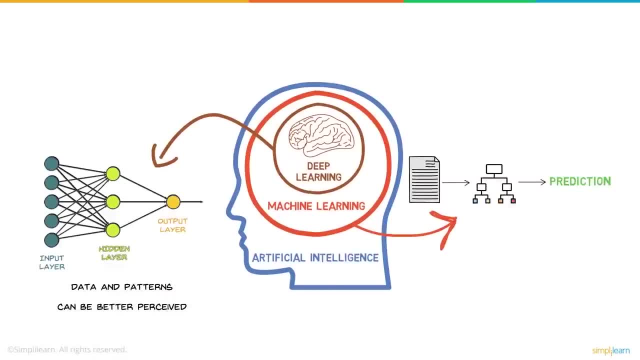 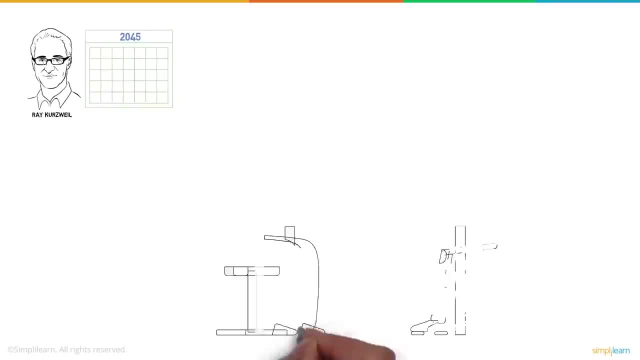 This means through deep learning, data and patterns can be better perceived. Ray Kurzweil, a well-known futurist, predicts that by the year 2045, we would have robots as smart as humans. This called the point of singularity. 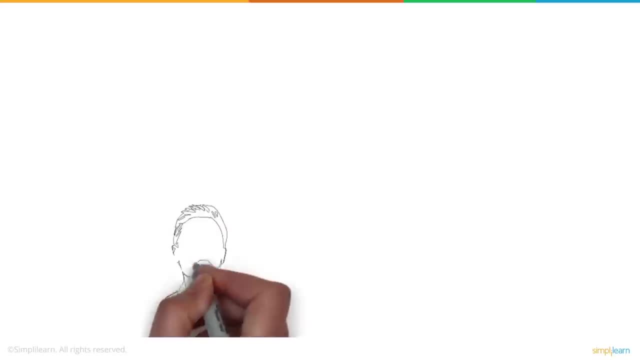 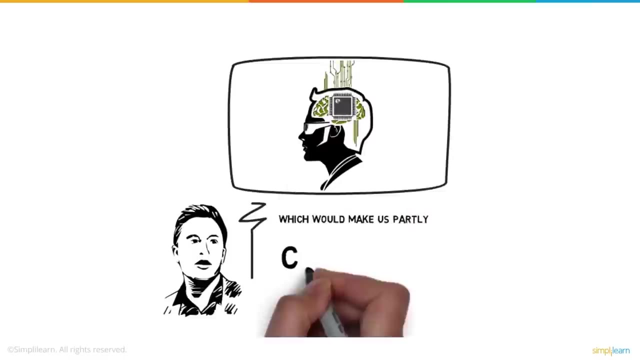 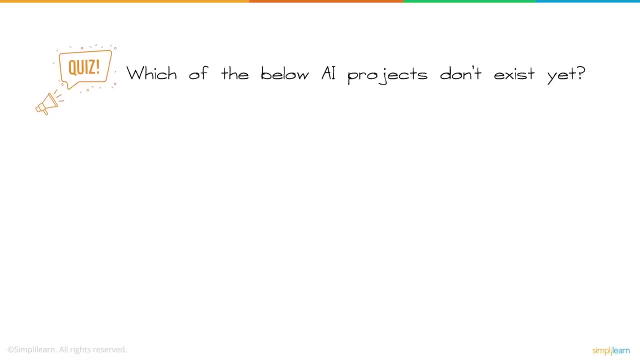 Well, that's not all. In fact, Elon Musks predicts that the human mind and body will be enhanced by AI implants, which would make us partly cyborgs. So here's a question for you: Which of the below AI projects don't exist yet? 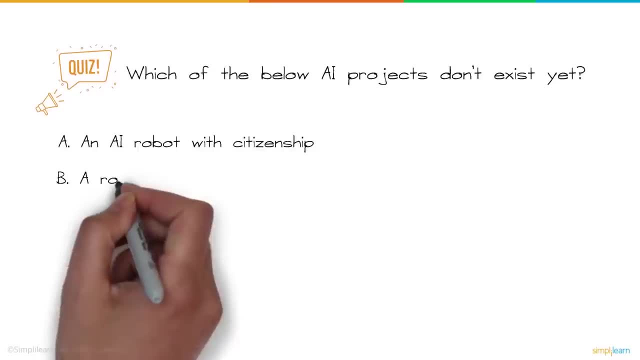 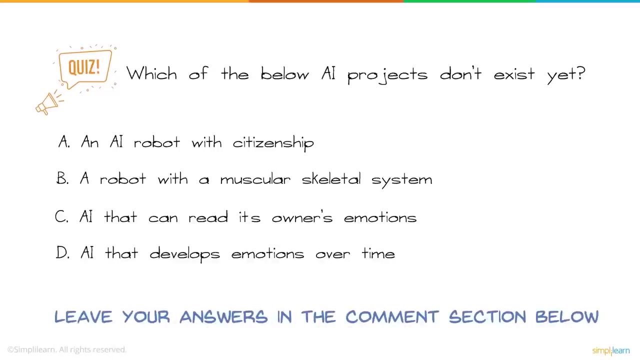 AI robot with citizenship. A robot with a muscular skeletal system. C A AI that can read its owner's emotions. D- AI that develops emotions over time. Give it a thought and leave your answers in the comment section below. Since the human brain is still a mystery, it's no surprise that AI, too, has a lot of. 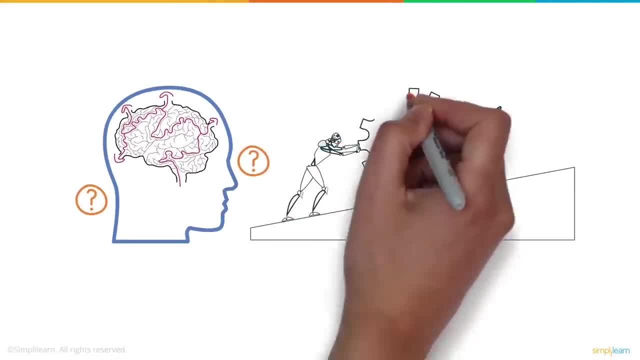 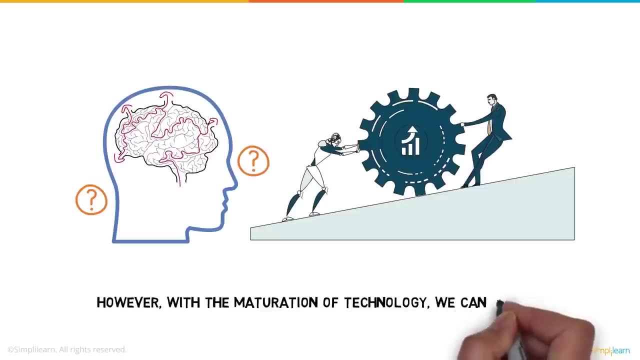 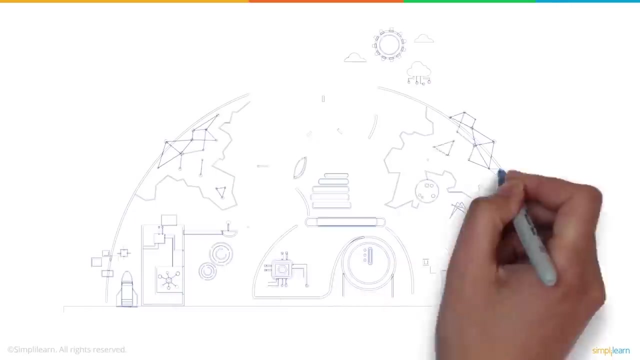 unventured domains. For now, AI is built to work with humans and make our tasks easier. However, with the maturation of technology, we can only wait and watch what the future of AI holds for us. Well, that is artificial intelligence for you. in short, 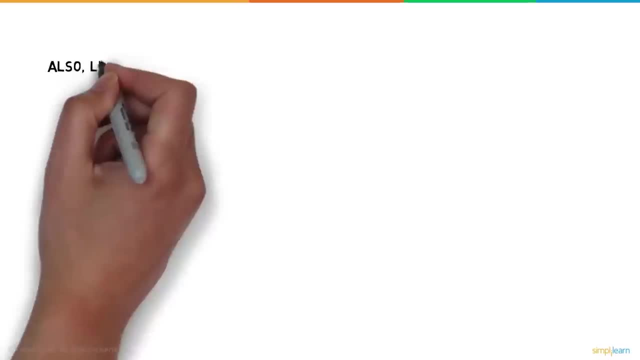 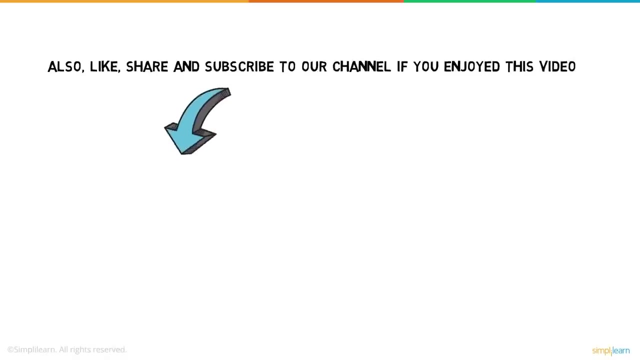 Do not forget to leave your answer to the quiz in the comment section below. Also, like, share and subscribe to our channel. if you enjoyed this video, Stay tuned and keep learning. Then we will draw a comparison between machine learning, deep learning and artificial intelligence. 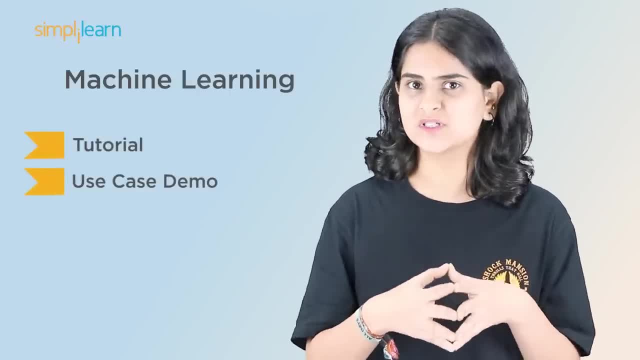 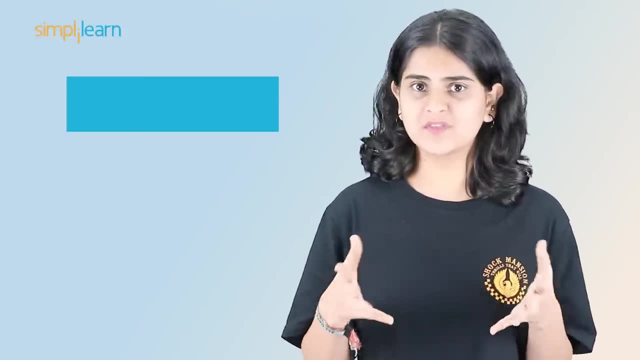 We will also learn about machine learning with a tutorial and a use case demo. After that, we will see the top 10 applications of machine learning. We will also understand the basics of deep learning- deep learning with python and a deep learning tutorial. 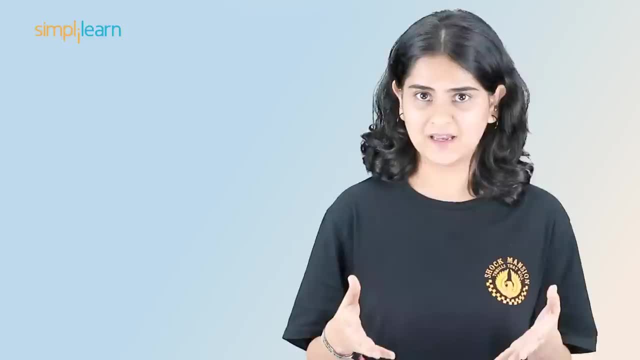 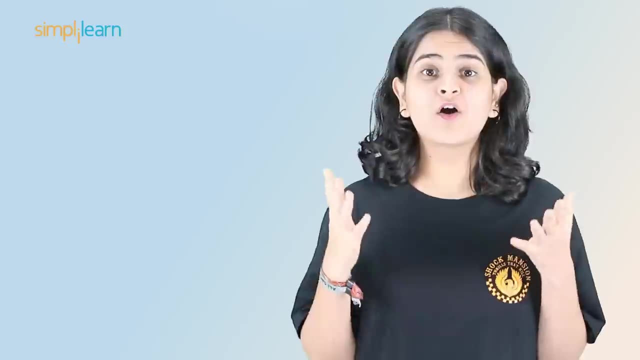 We will look at some important deep learning applications. At the end, we will explain to you how to become an AI engineer and look at a few important questions that will help you crack an AI interview. Alright, I hope that has got you excited. 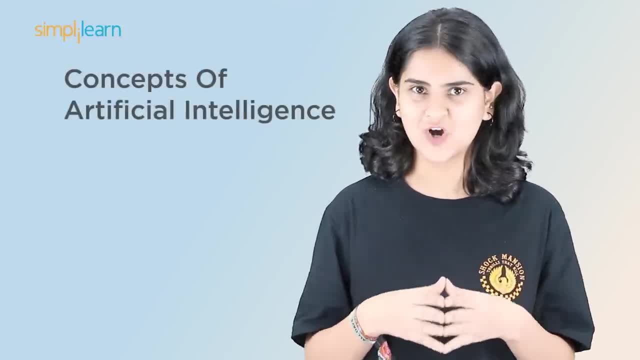 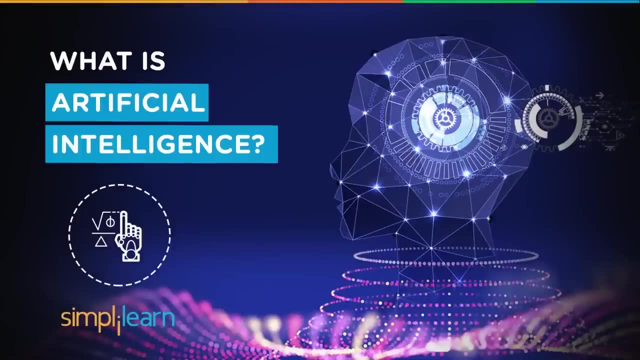 We now have Richard, Mohan and Rahul, who will explain the various concepts of artificial intelligence. What is artificial intelligence? Hello, my name is Richard Kirshner And today we are going to go over what is artificial intelligence. One example of today's artificial intelligence is a smart home. 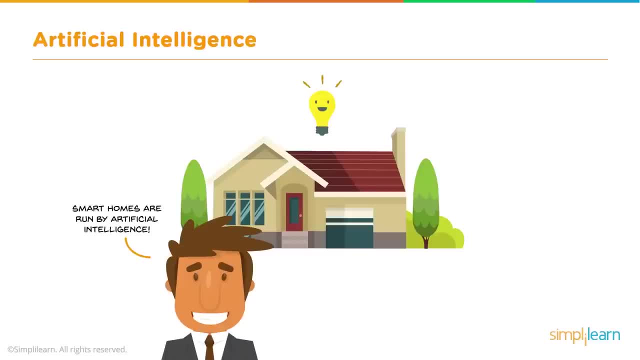 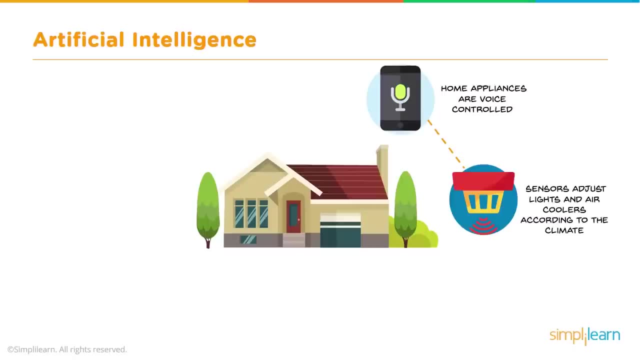 So welcome to my smart home. Smart homes are run by artificial intelligence. Let's have a look at some of the key features of a smart house. Home appliances are voice controlled. Sensors adjust lights and air coolers according to the climate. Security systems can detect movement outside and warn the residents. 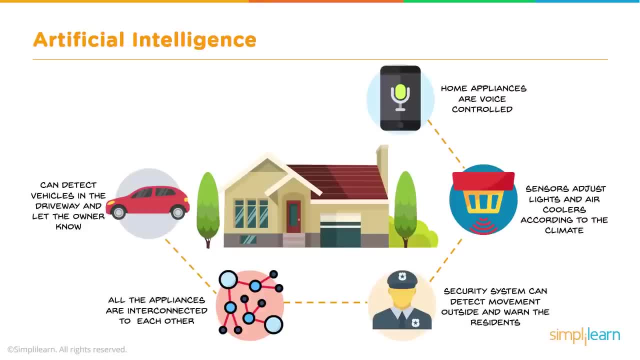 All the appliances are interconnected to each other And can detect vehicles in the driveway And let the owner know. Home appliances can be controlled remotely through the phone. Now, this is just one example in today's world. So what's in it for you today? 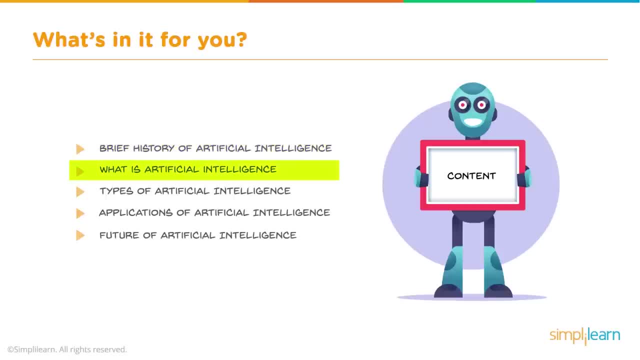 Today we are going to cover a brief history of artificial intelligence. What is artificial intelligence, Types of artificial intelligence, Applications of artificial intelligence And just a quick glimpse of the future of artificial intelligence. Let us start with a brief history of artificial intelligence. 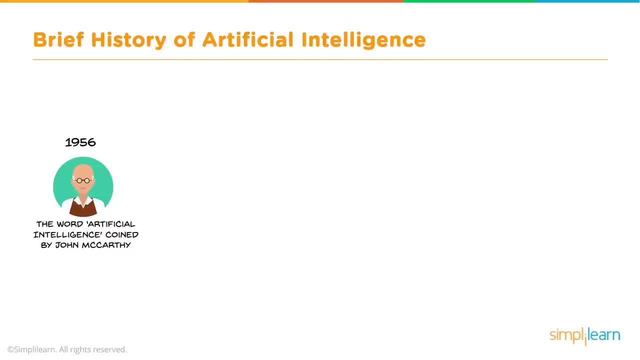 Let's start with John McCarthy. He was the first one to Coin the word artificial intelligence And in 1956 had the first artificial intelligence conference. Let's jump forward to 1969 with Shakey. Shakey was the first general purpose mobile robot built. 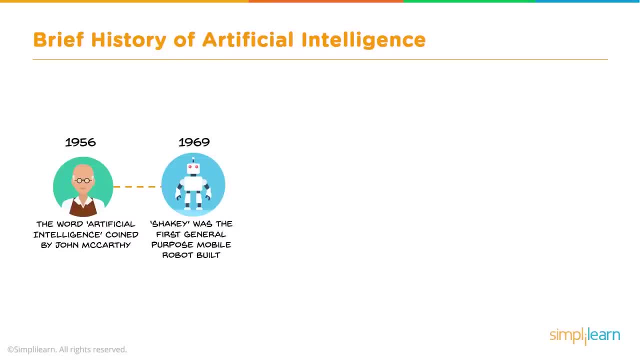 And although by today's standard he was very simple, He did mark a milestone in that we were now processing data differently. He was now able to do things with a purpose versus just a list of instructions. Albeit, the list included things like turning on and off lights. 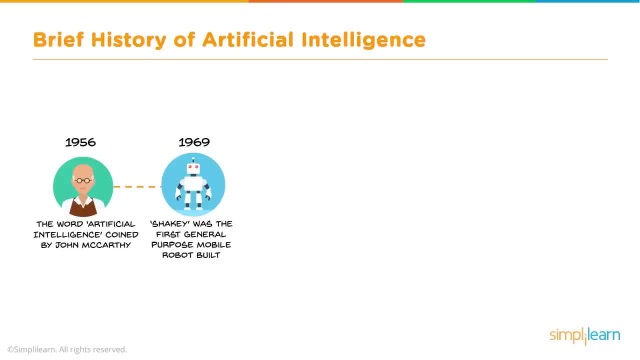 And Pushing boxes around the room. We're going to move forward to 1997.. In 1997, the supercomputer Deep Blue was designed, which defeated the world's chess champion in a game. This is the first time when we're actually seeing the computer using logic to beat a human doing some kind of logical, in this case a game. 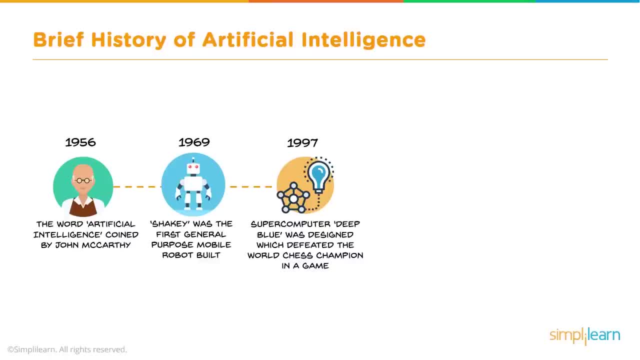 So it's a huge milestone by IBM to create this large computer that was able to do that in a timely fashion. Let's jump up to 2002, when we have our first commercially successful robotic vacuum Cleaner. Nowadays you can go down to the target and buy one, but back in 2002, that was the first model that was put out. and finally, 2005 to 2018. today, in the last more than a decade, we have a speech recognition, RPA, dancing robots, smart homes and many more to come. 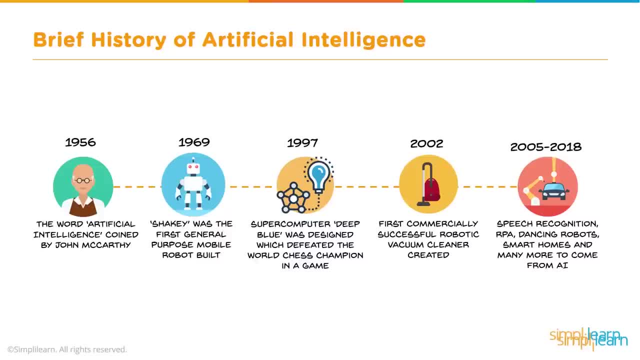 What I want you to notice about this brief history of artificial intelligence is the compression of time. in 1956 it was just an idea, and more than 10 years later we have our shaky the first one who's able to solve these problems. So 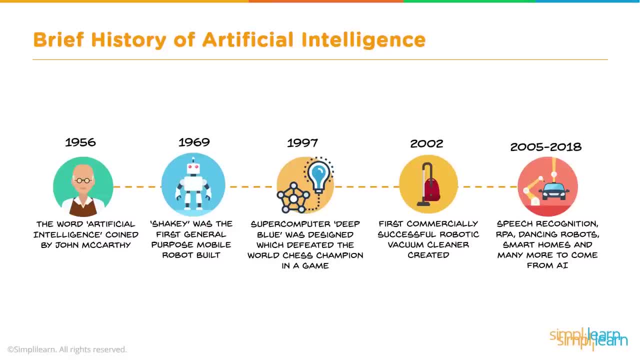 Let's flip light switches and then we go all the way to 97, where we have deep blue and there's a lot of little steps between 69 and 97, but it's actually able to take on a human in chess and beat them regularly. 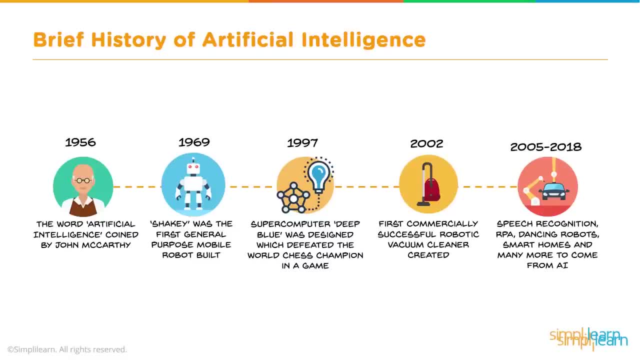 Now they did have a lot of ties, so don't think that it won every game. and then we go: only four years later we have our first commercially successful robotic vacuum cleaner. And as we go from 2005 to 2018, we go from simple speech recognition to very complicated, able to really register with your Google voice. 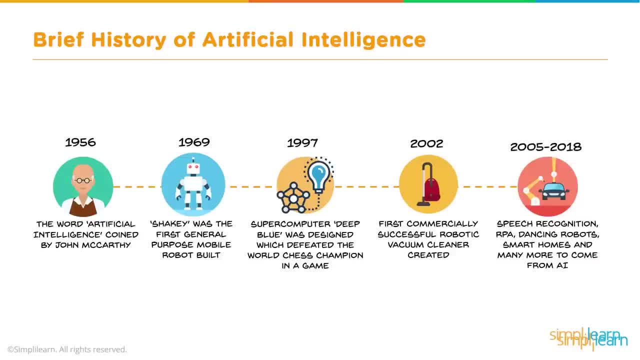 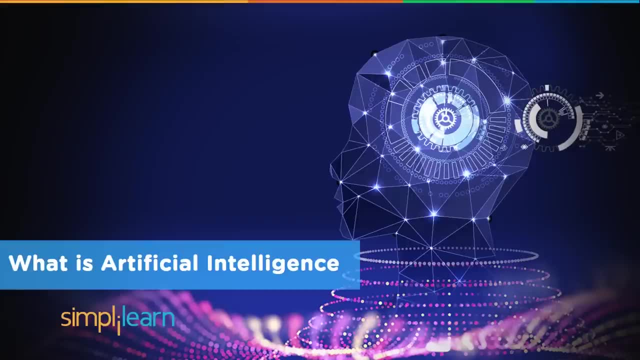 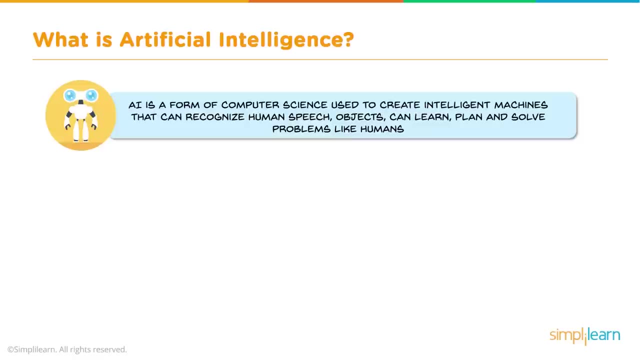 In Your Siri. we have our RPA, we have dancing robots, smart homes and many more things are just coming out almost monthly in the world of artificial intelligence. so what is artificial intelligence? AI is a form of computer science used to create intelligent machines that can recognize human speech, objects, can learn, plan and solve problems like humans, and I'd like you to focus just on that last one can solve problems like humans, as we saw earlier. 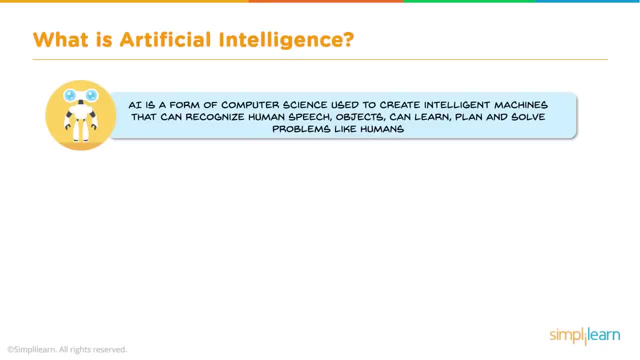 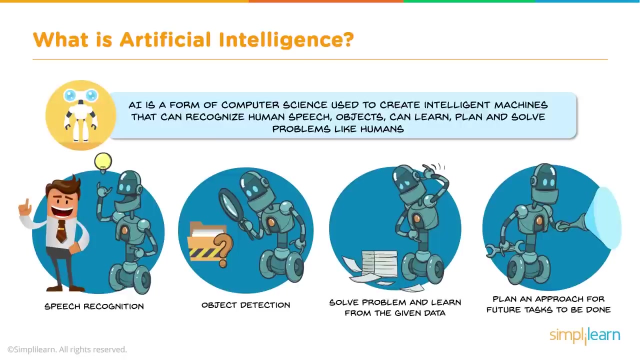 We compare the computer that can beat the chess champion- it's able- to the one before that, able to turn on and off lights in the house. so right now our concept of artificial intelligence is based primarily on our understanding of how it interacts with humans and how we can compare it to humans. so speech recognition, that's a big one today. object detection, solve problems and learn from the given data and plan an approach for future tasks to be done. these are all very human things that we do to plan and solve for the future. 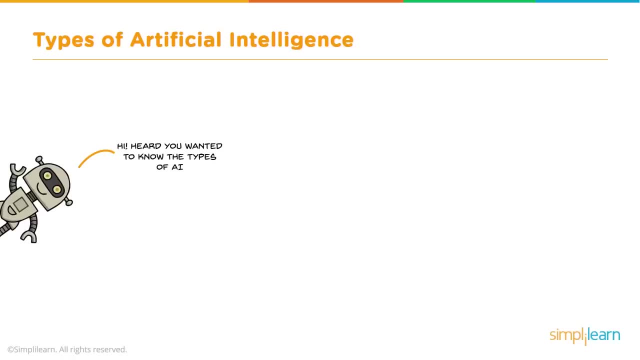 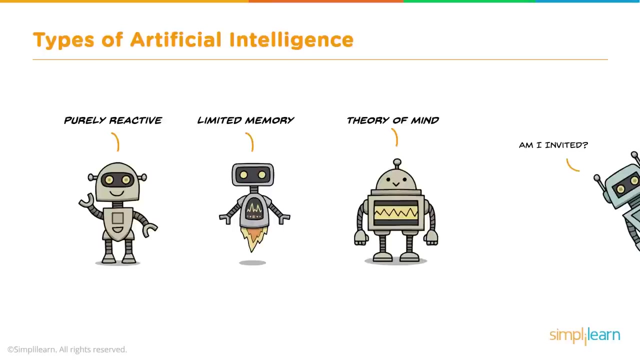 Types of artificial intelligence. Hi heard you want to know the types of AI. you can imagine a little robot taking us on a tour. the first type is purely reactive. the second type is limited memory. the third type, theory of mind, which is still in the process of being invented, and definitely the question of self awareness being the fourth, which is still not invented yet, or is it? let's look at these a little closer. here we have our purely reactive. he does not have any past memory. 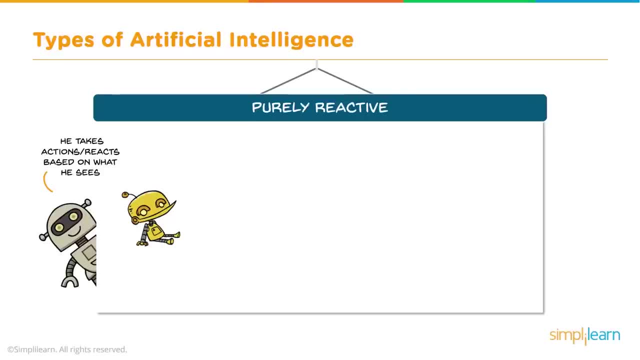 Or data to work with. he takes actions, reacts based on what he sees- okay, it's not that tough- observes every move- you see, we have a nice game of chess going on here- and wins. takes the best possible decision. purely reactive machines specialize in one field of work. 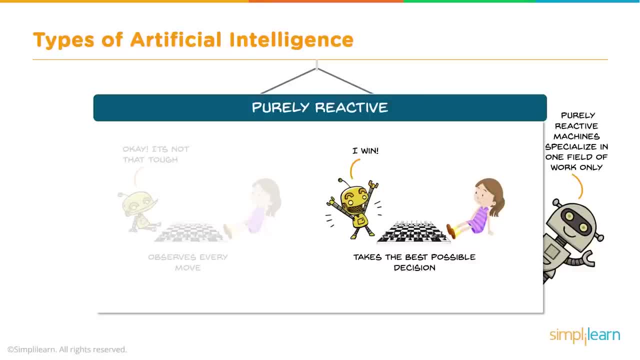 Only in this case we see a chess game where they figure out the best moves, calculating all the different moves- maybe it's calculating the next one in a row. in a linear regression models you can figure out the best marketing, But the very reaction If they don't have a lot of data, they just have what's in front of them to look at. 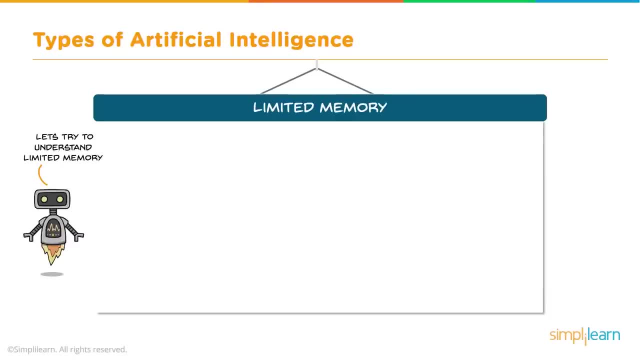 Next, let's look at limited memory. Let's try to understand the limited memory setup. These machines use previous data and keep adding it to their memory. Suggest me a good restaurant. So maybe we're looking to go out for dinner tonight and we're not sure what we want to eat. 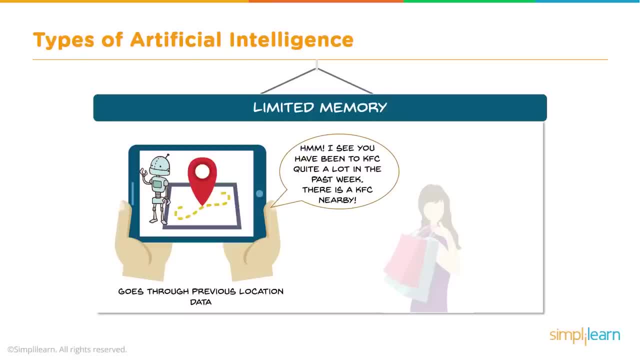 Hmm, I see you have been to KFC quite a lot in the past week. There is a KFC nearby, So it goes through the previous location data and where they ate prior and says, hmm, this is probably a good suggestion for you tonight. 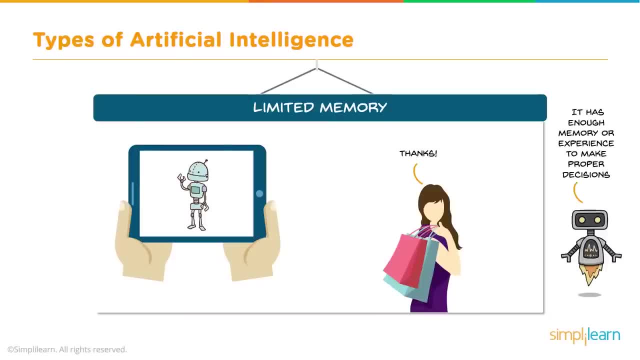 Thanks. It has enough memory or experience to make proper decisions, But the memory is very limited. This isn't trying to guess what a new location would be or anything like that. It just takes what it has in front of it and goes: okay, this is where you've been. 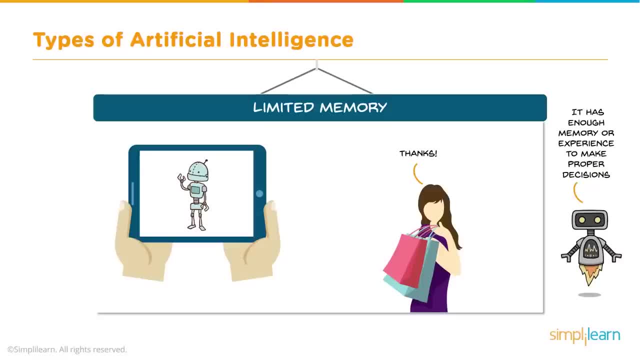 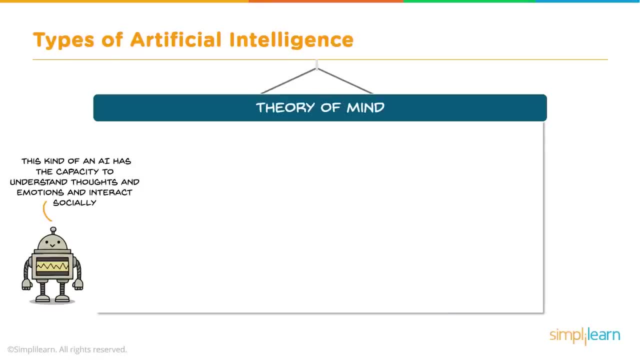 This is what you liked. You gave it two thumbs up, one thumb down, whatever, And then it goes from these suggestions. this is where I think you should go. Theory of mind. This kind of AI has the capacity to understand thoughts and emotions. 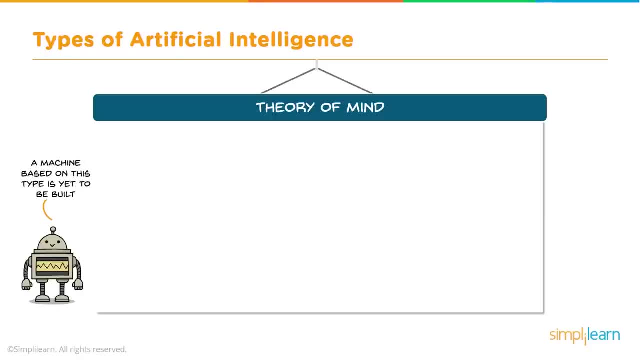 and interact socially. A machine based on this type is yet to be built. That human looks lonely. Hey human, you want to be my friend? Huh, Okay, Theory of mind is a thing of the future. Certainly, we see a lot of the industry poking a little bit at this. 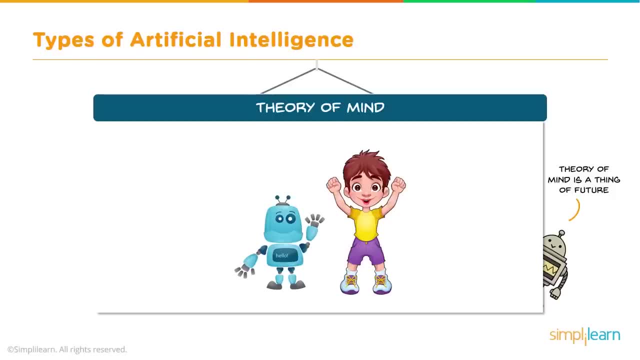 as it tries to guess how you feel about things, But most of that is still based on previous data, You know, yes, no two thumbs up, one thumb down. Theory of mind would take it one step further in understanding the emotions behind it. 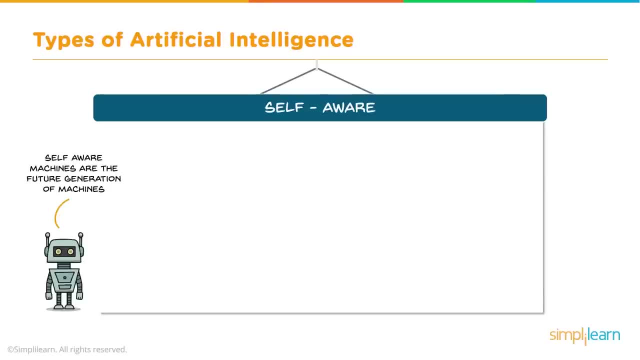 And finally, as we get deep into the sci-fi, futuristic, we have self-aware. Self-aware machines are future generation of machines. They will be super intelligent, sentient and conscious, Like the Terminator, the good guy in the thing, or Ultron, or Vision from Avengers. 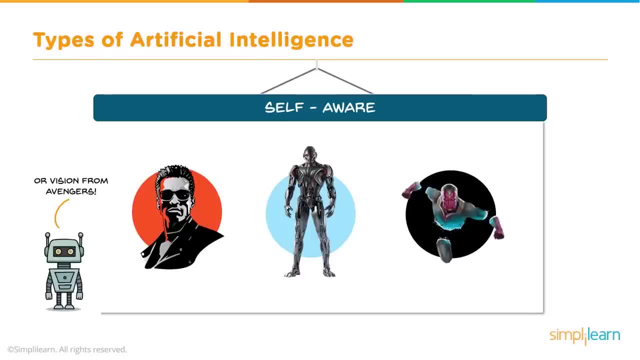 For right now these are mostly movie characters or cartoon characters, but we certainly are getting closer to seeing them in the real world. Hopefully they'll be of the type of the good guys and not the bad guys we see also in the artificial intelligence, sci-fi movies. 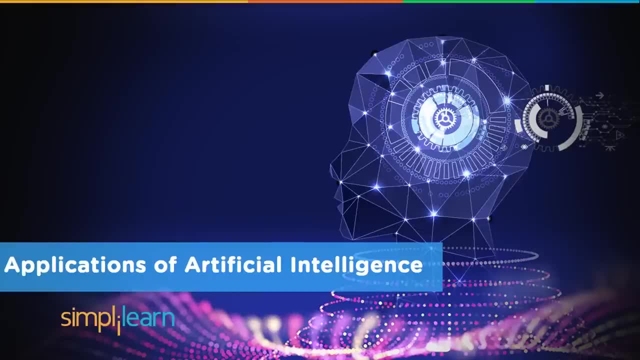 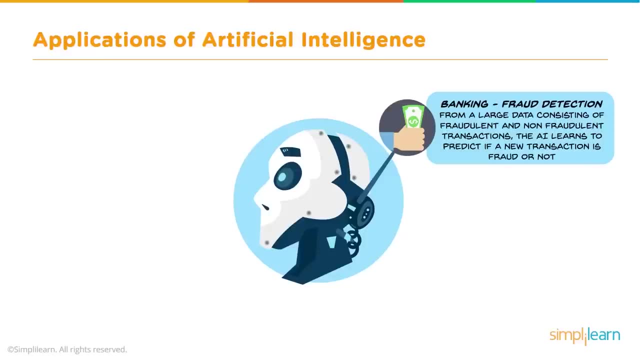 Applications of artificial intelligence. Let's take a look at some of today's commercial and business uses for the AI. We have banking fraud detection. From a large data consisting of fraudulent and non-fraudulent transactions, the AI learns to predict if a new transaction is fraud or not. 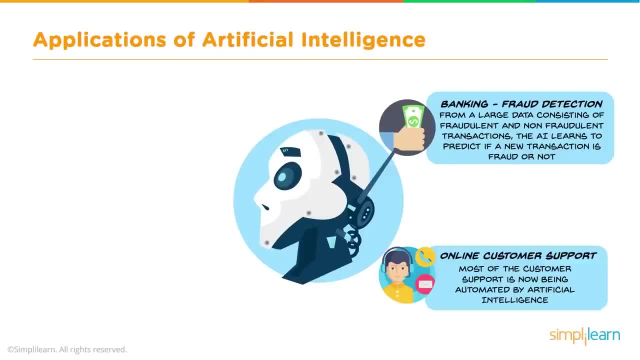 Online customer support. Most of the customer support is now being automated by artificial intelligence, Cyber security, Using machine learning algorithms and a lot of sample data. AI can be used to detect anomalies, adapt and respond to threats. Virtual assistants, Siri, Cortana, Alexa and Google now use voice recognition to follow the user's commands. 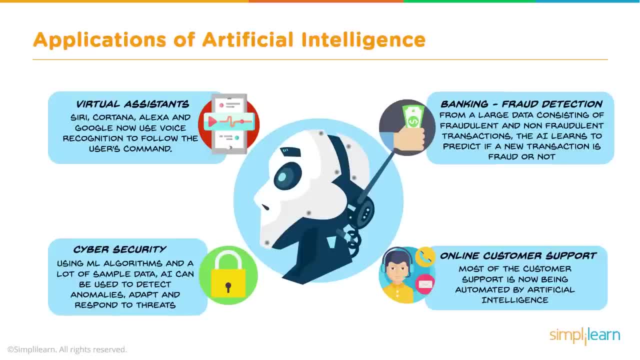 These are all wonderful examples of current AIs that are in the commercial and business world, and these ones in particular have matured over the last half a decade. For instance, very few large banks in today's world would not use banking for fraud detection. 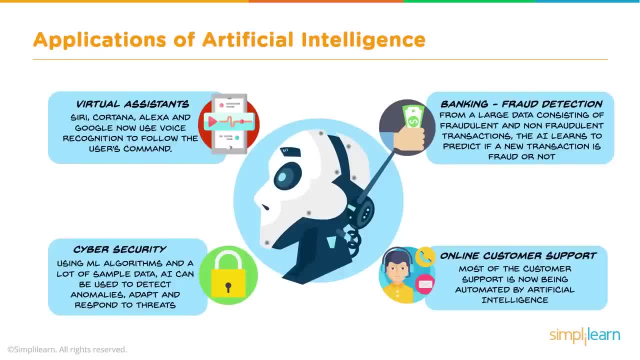 or for deciding whether it's a good person to give a loan to or not, based on their credit scores and where they're from and their income. Same thing with cybersecurity, Detecting anomalies Or online customer support. Could you imagine in, say, HP, who has over 70,000 help pages across 17 different languages? 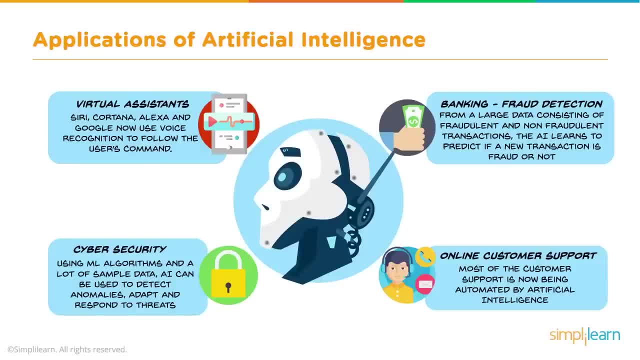 Now they have to figure out how to do online customer support to cover new problems that come up and track them so they can build new pages. If they had one person doing that, that would take them a year just to do what they need to have posted yesterday. 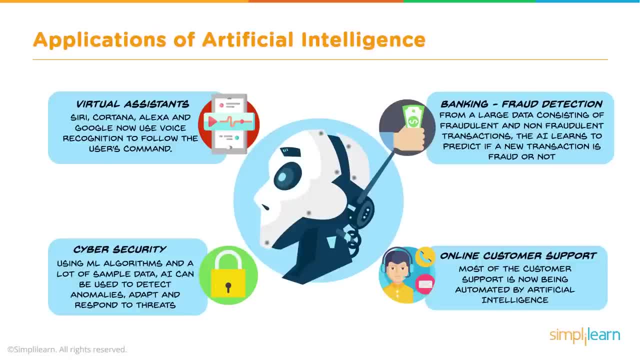 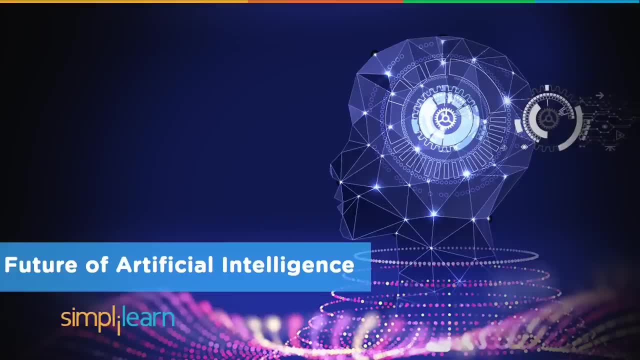 And, of course, our virtual assistants. I don't know about you, but I love mine. Kind of like having a private server Or having a private secretary without having a private secretary. Future of artificial intelligence: If we see where it's at now commercially and business-wise, then where is it going? 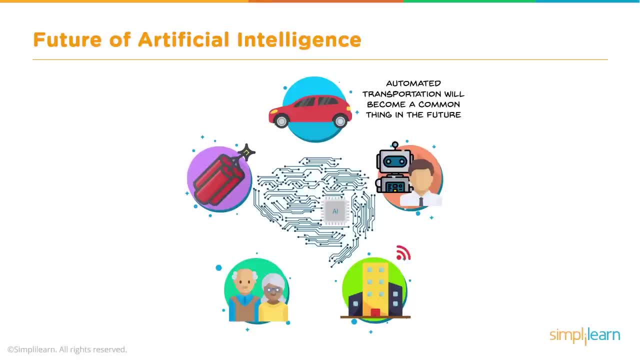 Of course, the imagination's a limit on this one, but you can already see the development in the world today for automated transportation. It'll become a common thing, maybe even early as 2020, when they have the final release from the leaders in the industry. 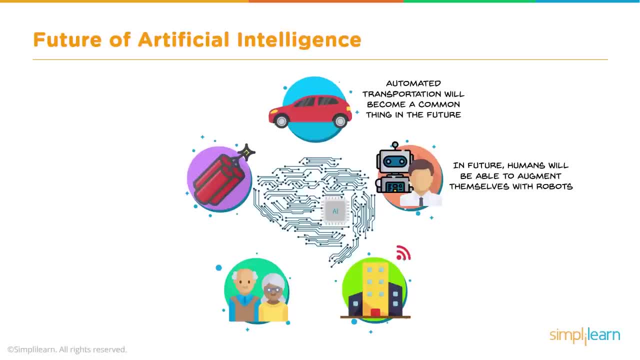 Humans will be able to augment themselves with robots. Certainly, the idea of having the robot bring me my coffee is lovely, But when I'm doing reports or something else on the computer, it does part of that work for me, so that I'm freed up to think about other things. 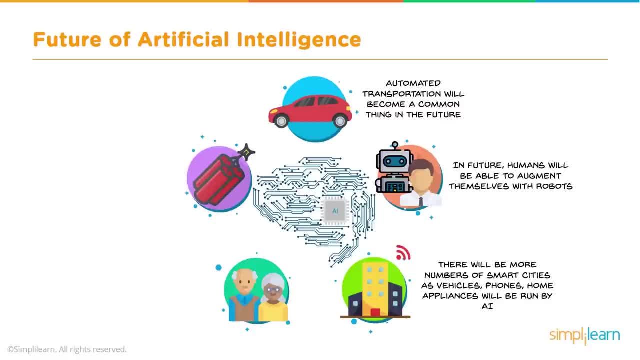 There'll be more numbers of smart cities, as vehicles, phones, home appliances will be run by AI. Home robots will help elderly people with the day-to-day work. Japan already has a very in-depth program where they've begun to integrate robots helping elderly. 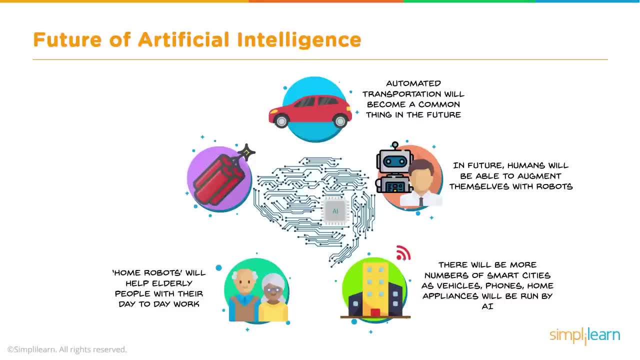 Even some of the simple things like getting that box of cereal off the top shelf or monitoring if they fall and need to contact the doctor or an emergency to show up. Robots will take over hazardous jobs like bomb defusing, welding, etc. For the future of artificial intelligence. 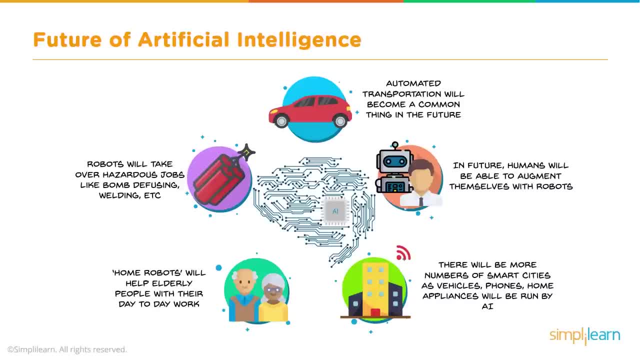 you can see here a number of robotic uses that are already in development. People are already working on these and trying to bring them to us in a commercial business fashion. Your own imagination can take this to the next level, or a simple Google search will show you some of the stuff that's out there now, in addition to these. 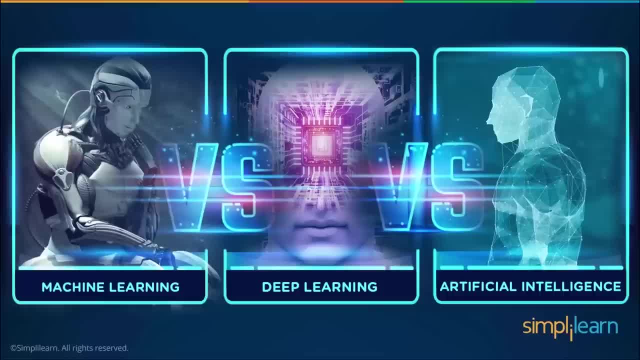 Versus deep learning versus artificial intelligence, Some of the most exciting technologies, Technologies evolving in today's world. Covering the basics of these three topics and how they connect and how they are different, let's just look at a few examples so we get an understanding of what's going on. 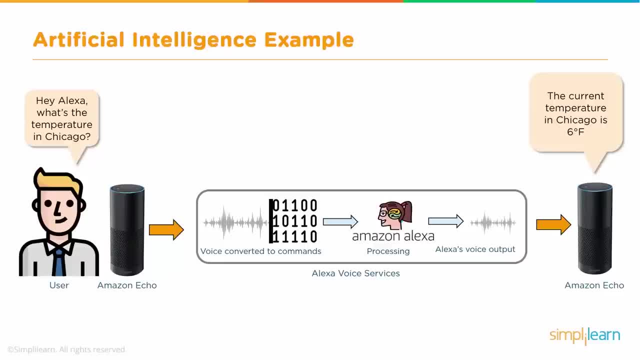 Here's an example of artificial intelligence in today's world: Amazon Echo. Amazon Echo is a wonderful tool. We can go in there and you can say: Hey, Alexa, what's the temperature in Chicago? And the Amazon Echo then translates that into zeros and ones and something the computer understands. 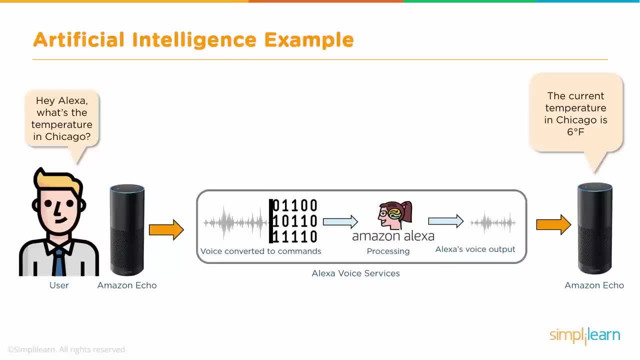 It comes in and processes that information to identify what you're asking and what you need and where to get that information, And then it comes back and says the current temperature in Chicago is six degrees Fahrenheit or whatever it is at the moment. So this is a wonderful example of artificial intelligence that we're using right now, today, and where that's at as far as a commercial deployment. 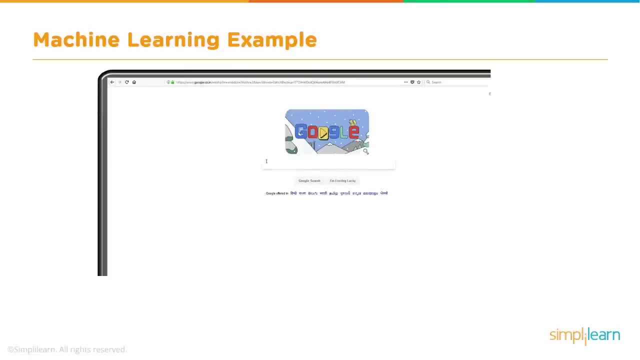 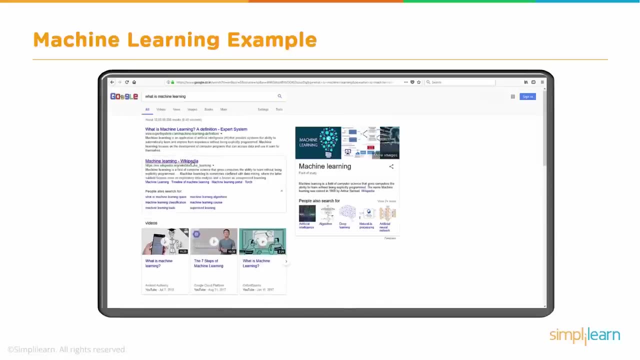 Machine learning. A machine learning example: out there is Google. You're on your Google search engine. It comes up. You spend a lot of time on the first link You come into and you read the page and Google looks at that and says: 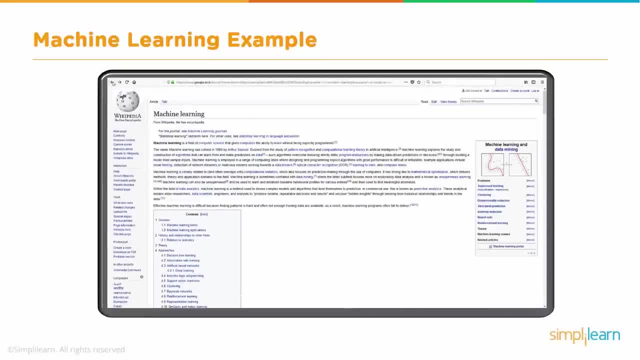 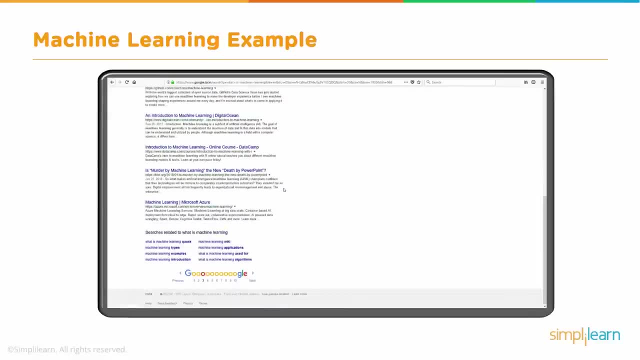 Okay, he spent five minutes on this. Let's give it a thumbs up. And then you go to the second page and the third page. You just kind of skip over them and glance at them for a couple seconds And Google says, Ah, I wasn't interested in those pages. 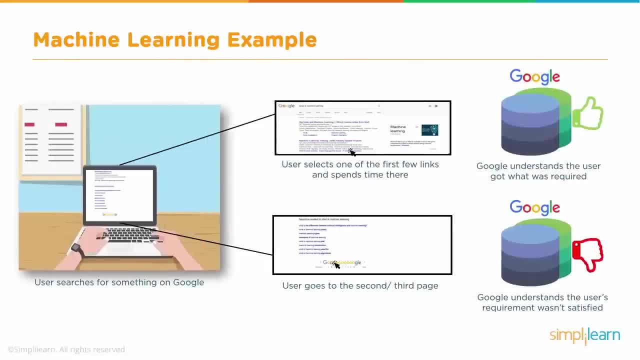 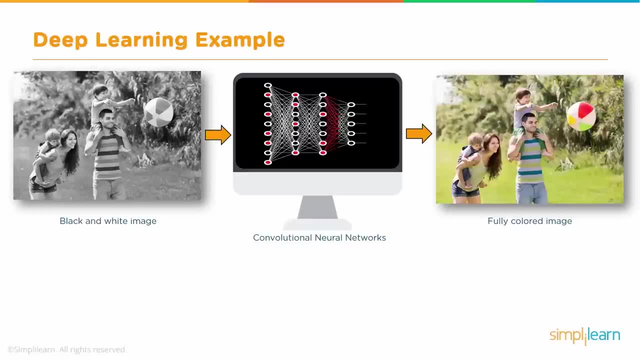 Let's give them a thumbs down. So this is a good example of machine learning, as it starts guessing what you like and what you don't like, So it gives you more information along what you're going to read and actually use, And then we have an example of deep learning. 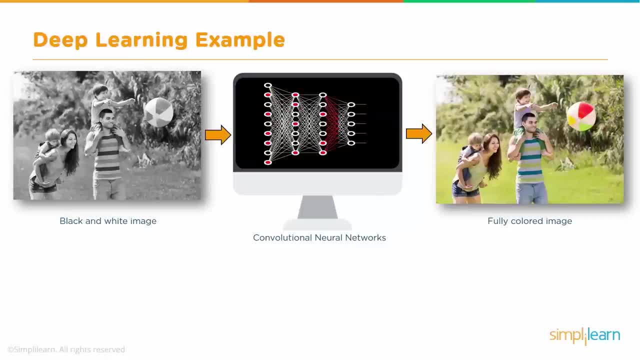 In this example we have a black and white image. It comes into, in this case, a neural network. Some people like to call it a magic box, because it's hard to follow all that's going on in there. There's all these different weights and connections and nodes. 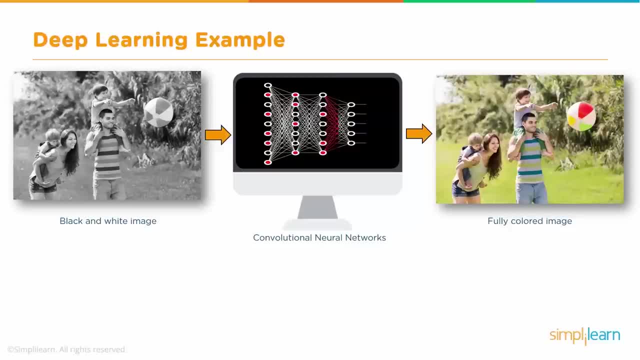 And then it comes out and colors the beach ball, the people, the background. What's going on in here is the black and white image, goes into this neural network And, before it's ever gone in, the neural network has looked at all these different pictures on the web or wherever it pulls the data from. 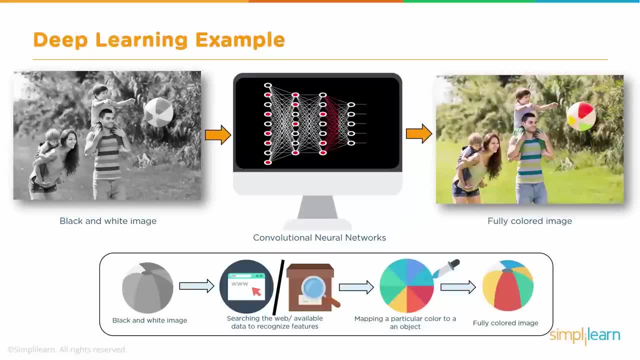 And it's already itemized them and kind of separated them, that we have some that look like beach balls, We have some that look like people And it programs that, so that when the black and white image comes in, it goes, Okay, that piece right there resembles this and all these other photos. 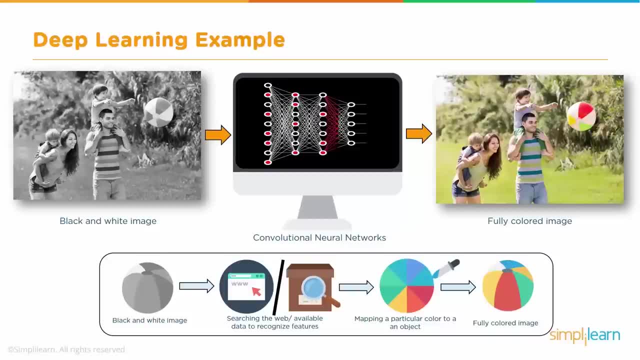 And the neural network is able to identify that and then color the beach ball with the colors that you see on there. So this is really wonderful, because they did a wonderful job. coloring this picture- And that's the full setup- is where the deep learning example comes in. 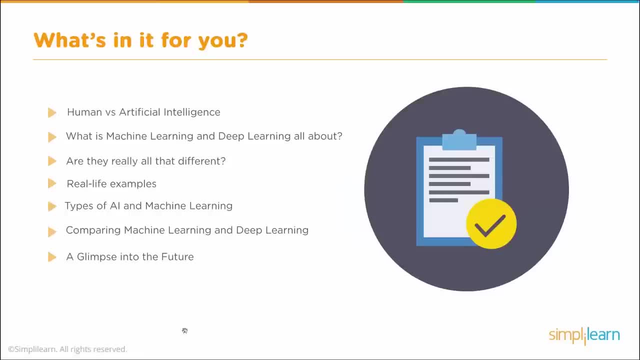 And they usually center around neural networks. So we looked at a few examples. What's in it for you? First, we're going to talk about human versus artificial intelligence. This is very important because this is our marker: We, as humans, are amazing. 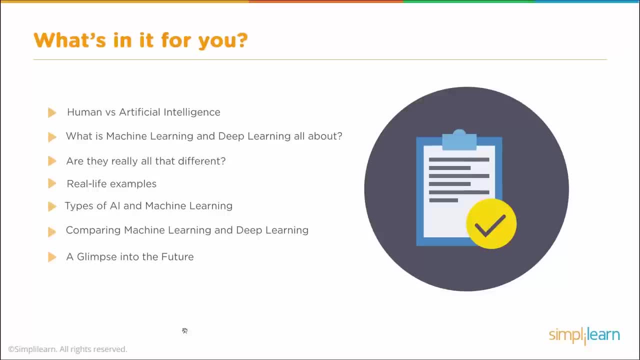 And so we want to understand how artificial intelligence compares and what it does, that it can accelerate above humans, and how it can integrate with the human. What is machine learning and deep learning all about? Are they really all that different? We'll have a few more examples in here. 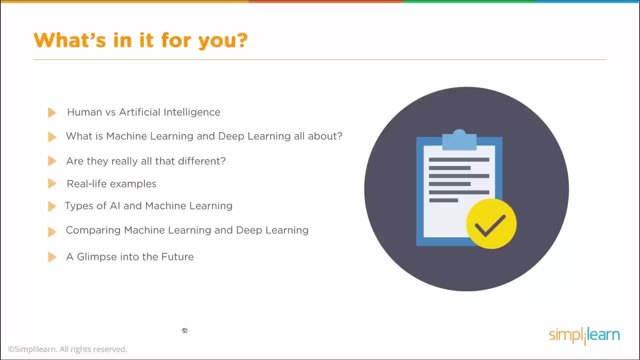 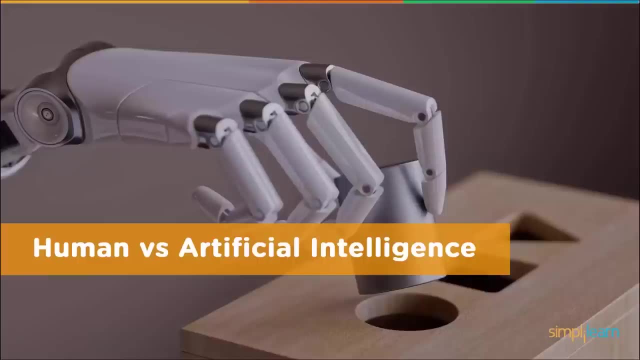 And then we'll talk a little bit about types of AI and machine learning and comparing machine learning and deep learning And finally, a glimpse into the future: Human versus artificial intelligence. Humans are amazing. Let's just face it. We're amazing creatures. 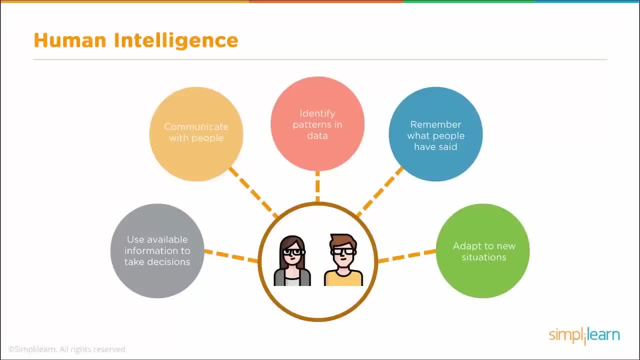 We're all over the planet. We're exploring every nook and cranny. We've gone to the moon, We've gone into outer space. We're just amazing creatures. We're able to use the available information to make decisions, to communicate with other people. 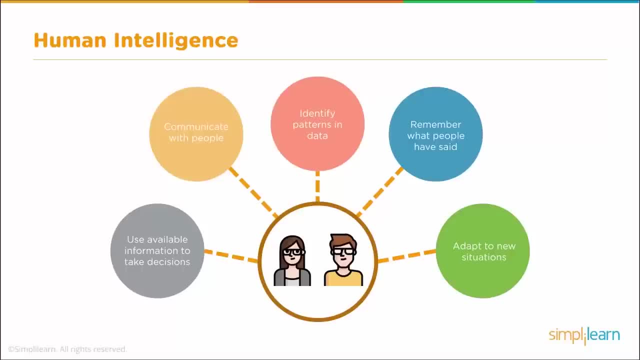 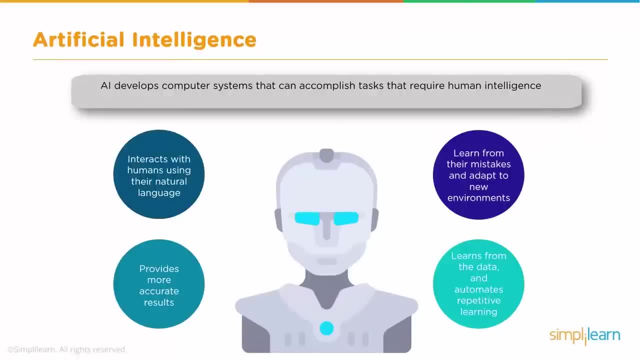 identify patterns in data. remember what people have said: adapt to new situations. So let's take a look at this So you can get a picture. You're a human being, so you know what it's like to be human. Let's take a look at artificial intelligence versus the human. 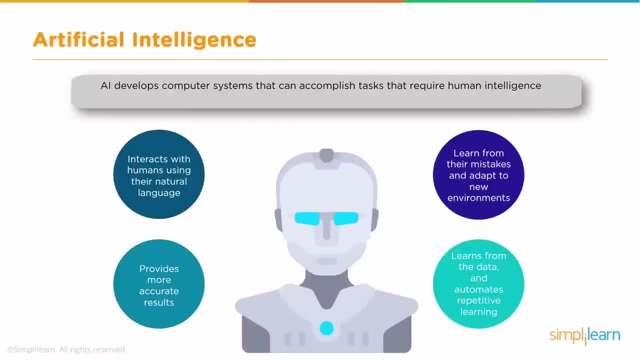 Artificial intelligence develops computer systems that can accomplish tasks that require human intelligence. So when we're looking at this, one of the things that computers can do is they can provide more accurate results. This is very important. Recently, I did a project on cancer where it's identifying markers. 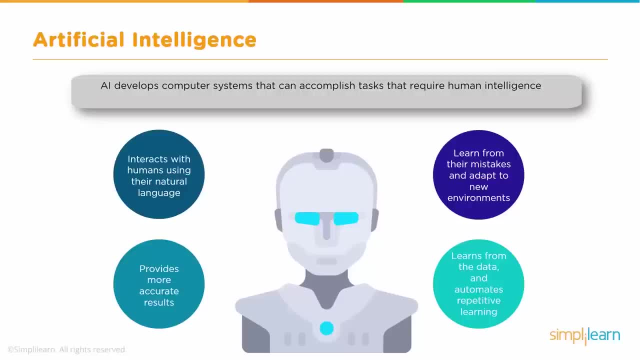 And, as a human being, you look at that and you might be looking at all the different images and the data that comes off of them and say: I like this person, So I want to give them a very good outlook. And the next person you might not like, so you want to give them a bad outlook. 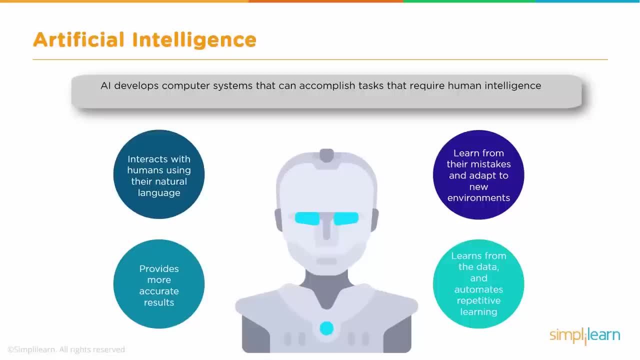 Well, with artificial intelligence, you're going to get a consistent prediction of what's going to come out. It interacts with humans using their natural language. We've seen that as probably the biggest development feature right now. that's in the commercial market that everybody gets to use, as we saw with the example of Alexa. 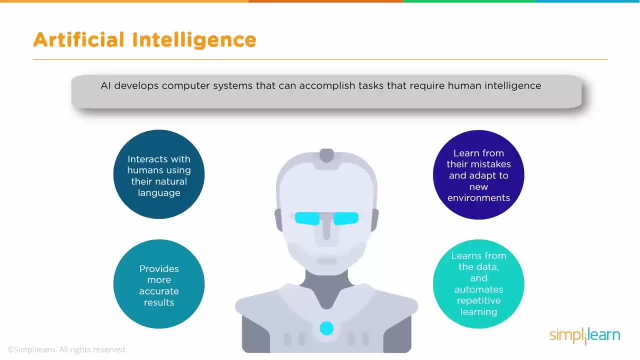 They learn from their mistakes and adapt to new environments. So we see this slowly coming in more and more, And they learn from the data and automate repetitive learning. And repetitive learning has a lot to do with the neural networks. You have to program thousands upon thousands of pictures in there and it's all automated. 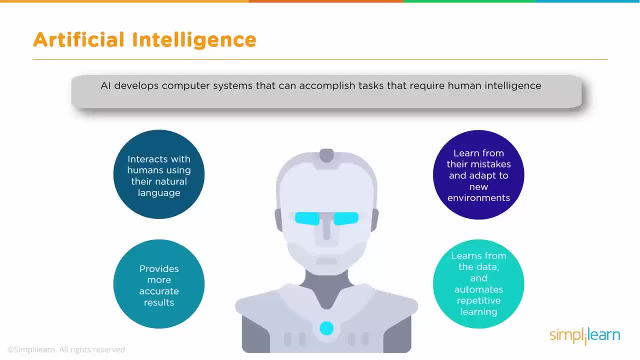 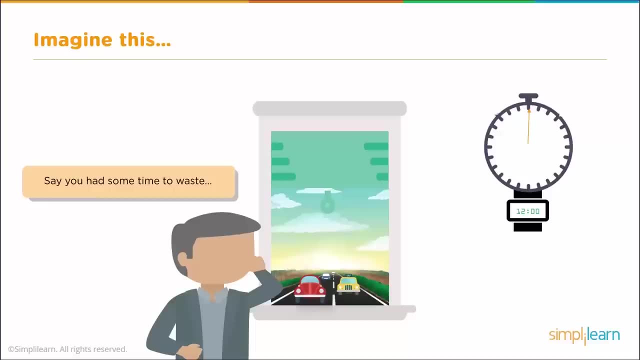 So, as today's computers evolve, it's very quick and easy and affordable to do this. What is machine learning and deep learning all about? Imagine this: Say you had some time to waste- Not that any of us really have a lot of time anymore to just waste in today's world. 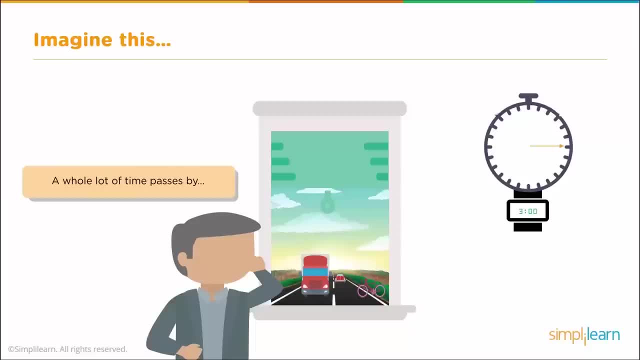 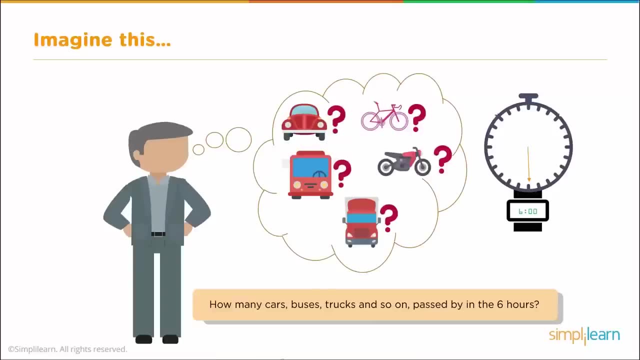 And you're sitting by the road And a whole lot of time passes by. Here's a few hours And suddenly you wonder how many cars, buses, trucks and so on passed by in the six hours. Now, chances are you're not going to sit by the road for six hours and count buses, cars and trucks, unless you're working for the city and you're trying to do city planning. 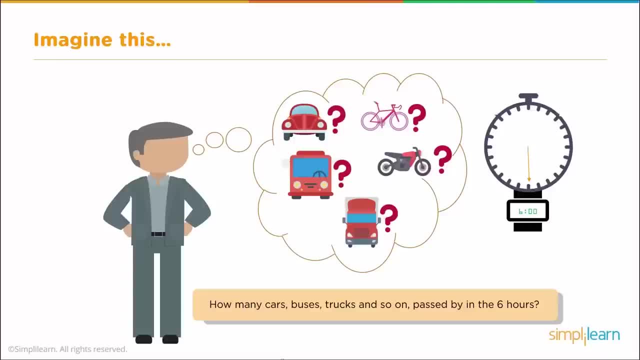 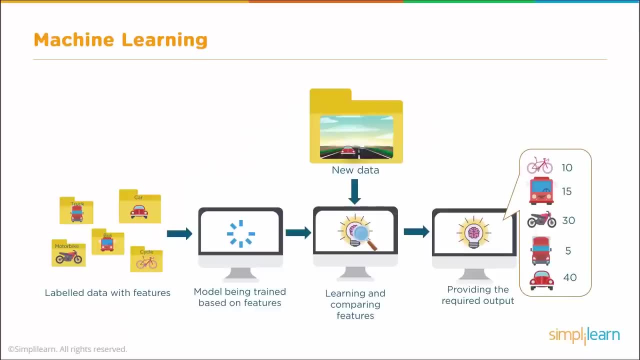 And you want to know: hey, do we need to add a new truck route? Maybe we need a bicycle lane, because we have a lot of bicyclists here, That kind of thing. So maybe city planning would be great for this. Machine learning. 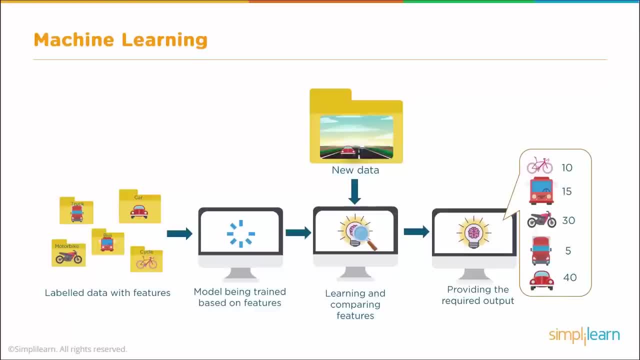 The way machine learning works is we have labeled data with features. Okay, So you have a truck or a car, a motorcycle, a bus or a bicycle And each one of those are labeled. It comes in And, based on those labels and comparing those features, it gives you an answer. 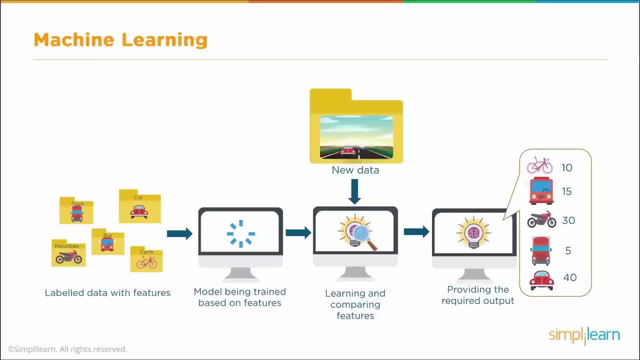 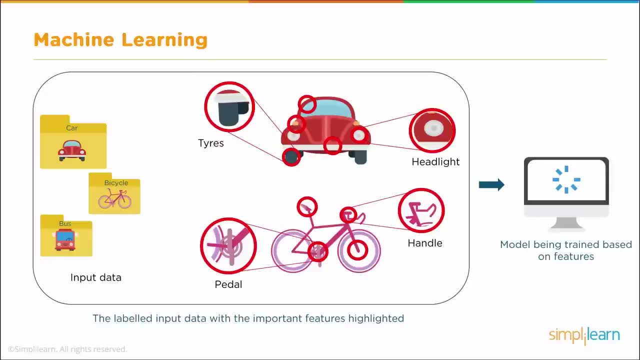 It's a bicycle, It's a truck, It's a motorcycle. Let's look a little bit more in depth on this. In the model here, it actually the features we're looking at would be like the tires, So a person sits there and figures out what a tire looks like. 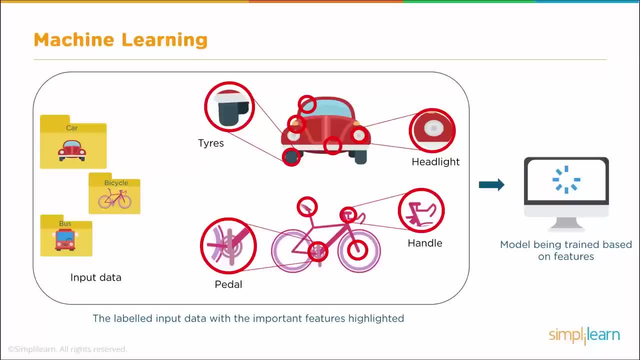 It takes a lot of work If you try to figure the difference between a car tire, a bicycle tire, a motorcycle tire. So in the machine learning field this could take a long time if you're going to do each individual aspect of a car and try to get a result on there. 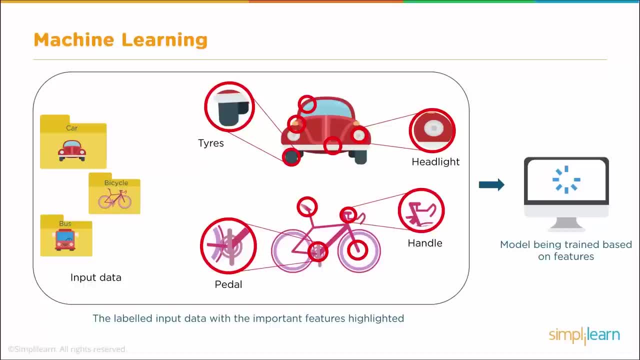 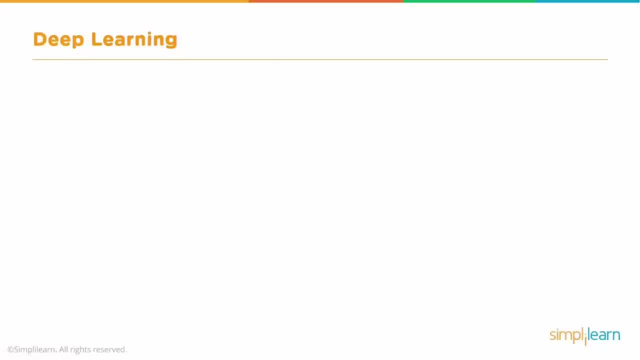 And that's what they did do. This is still used on smaller amounts of data, where you figure out what those features are and then you label them- Deep learning. So with deep learning, one of our solutions is to take a very large unlabeled data set and we put that into a training model using artificial neural networks. 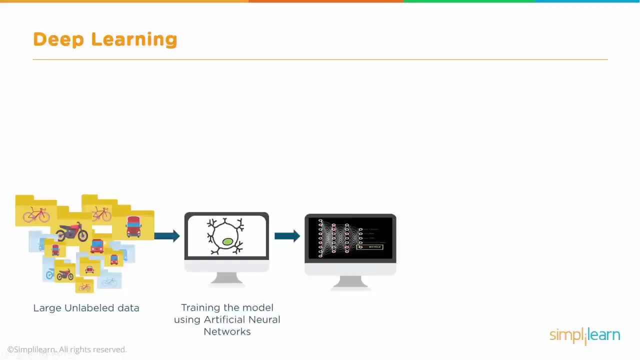 And then that goes into the neural network itself. when we create a neural network And you'll see, the arrows are actually kind of backward, which actually is a nice point, because when we train the neural network we put the bicycle in and then it comes back and says, if it's a truck? it comes back and says, well, you need to change that to bicycle. 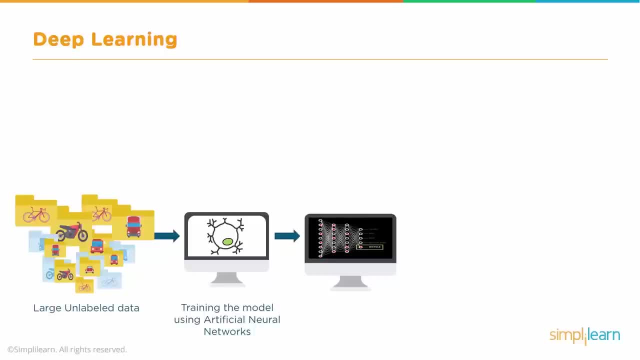 And then it changes all those weights going backward. They call it back propagation And let it know it's a bicycle and that's how it learns. Once you've trained the neural network, you then put the new data in and they call this testing the model. 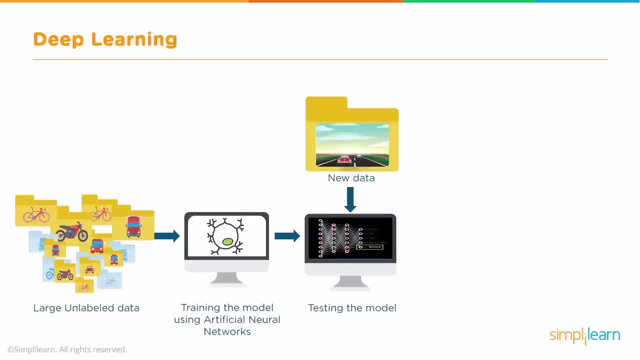 So you need to have some data you've kept off to the side where you know the answer to, And you take that and you provide the required output and you say, okay, is this neural network working correctly? Did it identify a bike as a bike, a truck as a truck, a motorcycle as a motorcycle? 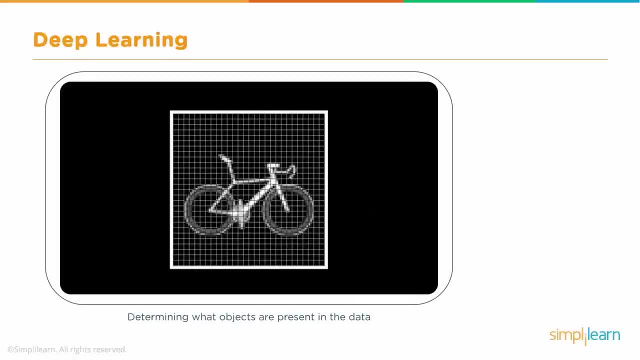 Let's just take a little closer look at that, Determining what objects are present in the data. So how does deep learning do this? And here we have the image of the bike. It's 28 by 28 pixels. That's a lot of information there. 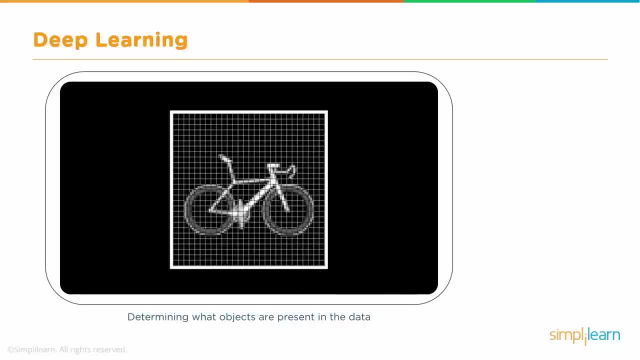 Could you imagine trying to guess that this is a bicycle image by looking at each one of those pixels and trying to figure out what's around it? And we actually do that as human beings? It's pretty amazing. We know what a bicycle is and even though it comes in as all this information, 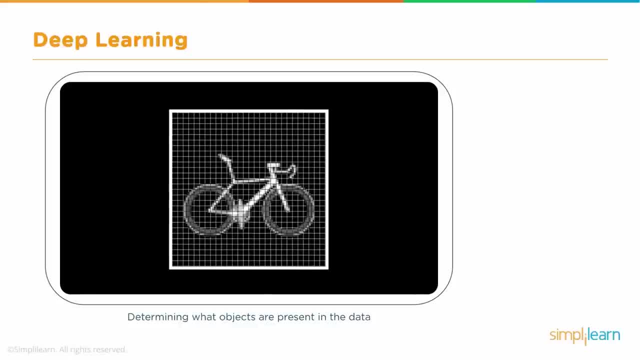 And what this looks like is. the image comes in, It converts it into a bunch of things, A bunch of different nodes- In this case, there's a lot more than what they show here- And it goes through these different layers and outcomes and says, okay, this is a bicycle. 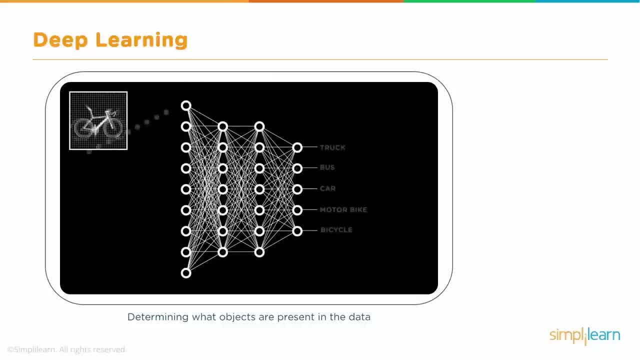 A lot of times they call this the magic black box. Why? Because as we watch it, go across here all these weights and all the math behind this, And it's not. it's a little complicated on the math side. You really don't need to know that when you're programming or doing working with the deep learning. 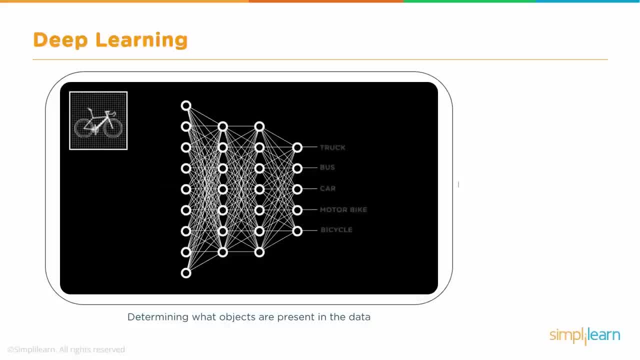 But it's like magic. You don't know, you really can't figure out what's going to come out by looking. what's in each one of those layers And each one of those dots and each one of those lines are firing and what's going in between them. 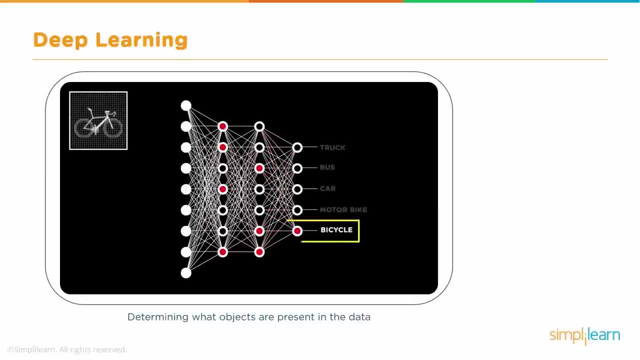 So we like to call it the magic box. So that's where deep learning comes in. And in the end it comes up and you have this whole neural network. It comes up and it says, okay, we fire all these different pixels and we connect all these different dots. 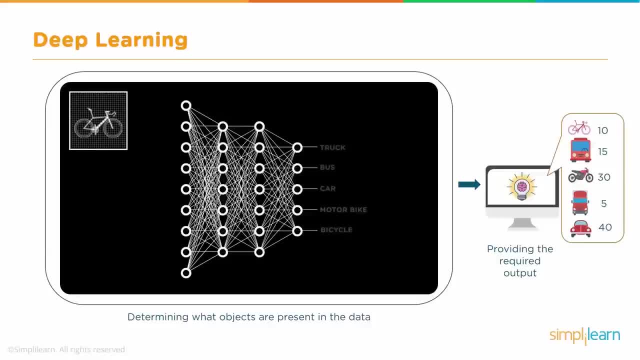 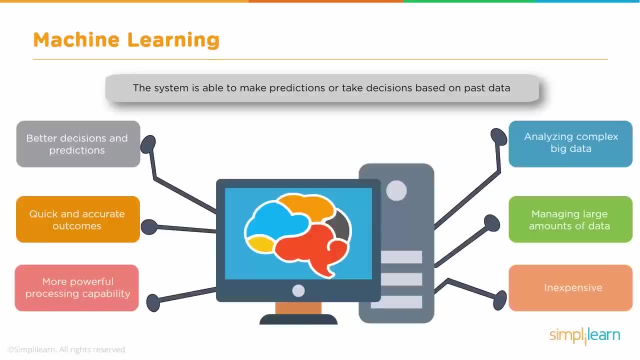 And gives them different weights and it says, okay, this is a bicycle And that's how we determine what the object is present in the data. with deep learning- Machine learning- We're going to take a step into machine learning here And you'll see how these fit together in a minute. 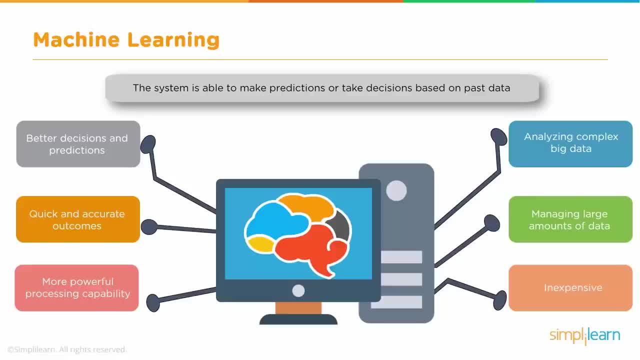 The system is able to make predictions or take decisions based on past data. That's very important for machine learning is that we're looking at stuff and, based on what's been there before, we're creating a decision on there. We're creating something out of there. 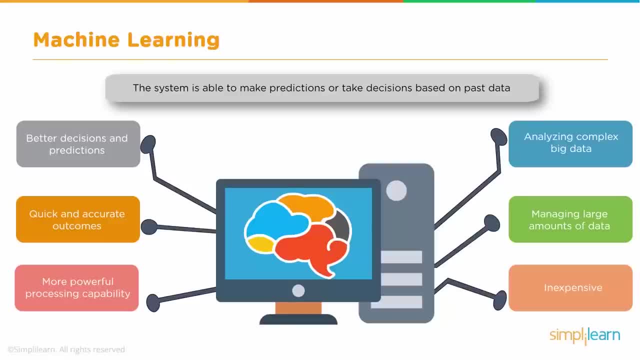 We're coloring a beach ball. We're telling you what the weather is in Chicago. What's nice about machine learning is a very powerful processing capability. It's quick and accurate outcomes, So you get results right away. You don't have to have the system. 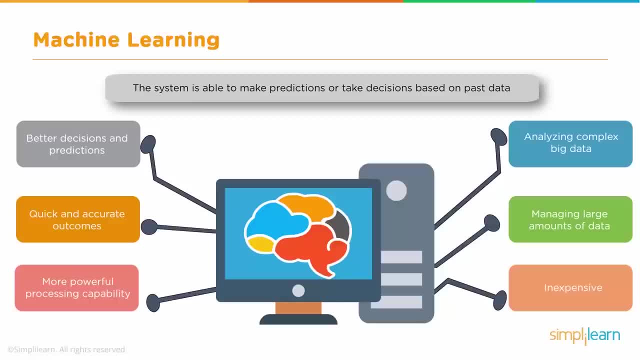 The results are very fast And the decisions and predictions are better. They're more accurate. They're consistent. You can analyze very large amounts of data. Some of these data things that they're analyzing now are petabytes and terabytes of data. 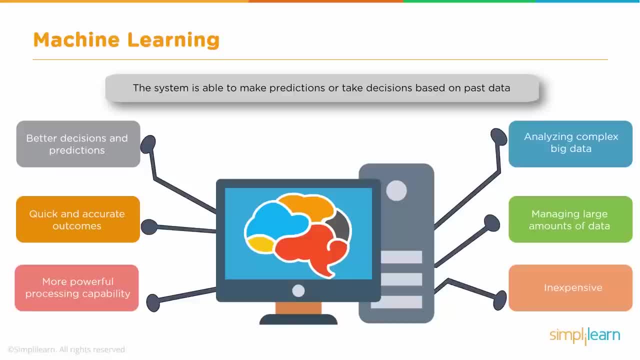 It would take hundreds of people, hundreds of years, to go through some of this data and do the same thing that the machine learning can do in a very short period of time, And it's inexpensive compared to hiring hundreds of people, So it becomes a very affordable way to move into the future is to apply the machine learning. 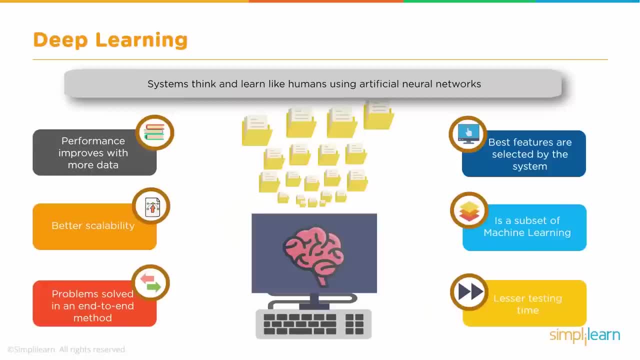 to whatever businesses you're working on, And deep learning Systems think and learn like humans using artificial neural networks. Again, it's like a magic box. Performance improves with more data, So the more data that deep learning gets, the more it gives you better results. 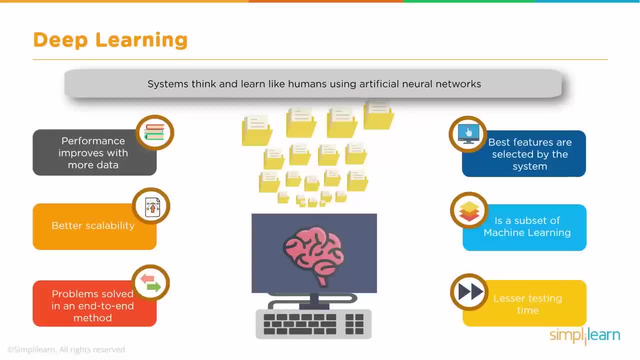 It's scalability, So you can scale it up, You can scale it down, You can increase what you're looking at. We're limited by the amount of computer processing power as to how big that can get, But that envelope continually gets pushed every day on what it can do. 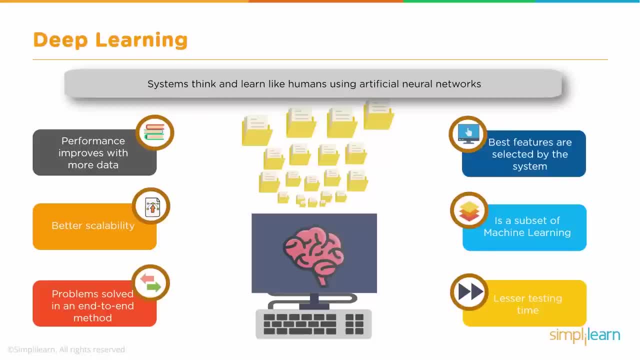 Problem solved in an end-to-end method. So instead of having to break it apart, and you have the first piece coming in and you identify tires and the second piece is labeling handlebars and then you bring that together that if it has handlebars and tires it's a bicycle. 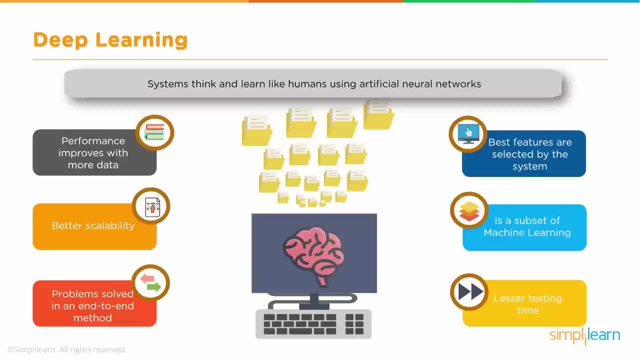 And if it has something that looks like a large square, it's a truck. The neural networks does this all in one network. You don't really know what's going on in all those weights and all those little bubbles, But it does it pretty much in one package. 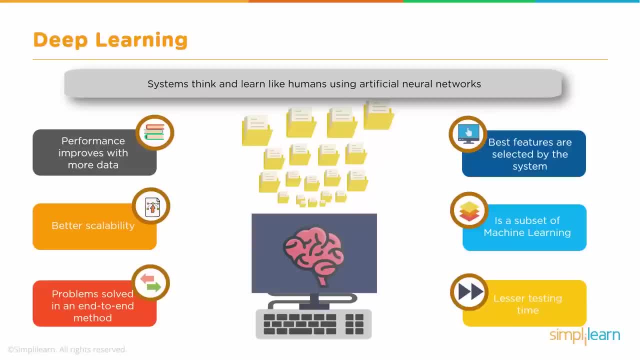 That's why the neural network systems are so big nowadays and coming into their own Best features are selected by the system, And this is important. They kind of put it on a bullet on the side here. It's a subset of machine learning. 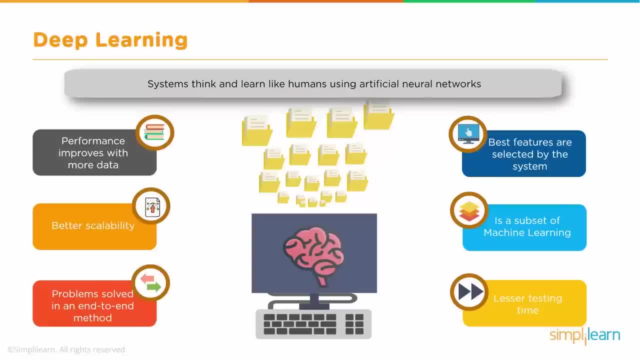 This is important When we talk about deep learning. it is a form of machine learning. There's lots of other forms of machine learning- data analysis- But this is the newest and biggest thing: that they apply to a lot of different packages and they use all the other machine learning tools available to work with it. 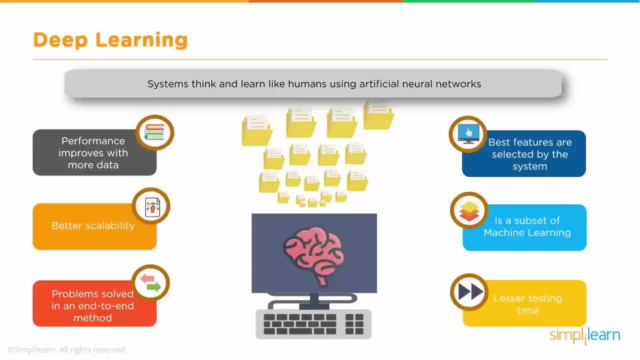 And it's very fast to test. You put in your information, You then have your group of tests And then you held some aside and you see how does it do. It's very quick to test it and see what's going on with your deep learning and your neural network. 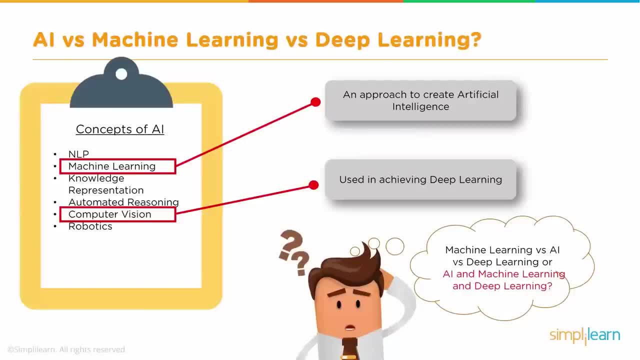 Are they really all that different? Hmm, AI versus machine learning versus deep learning: Concepts of AI. So we have concepts of AI, You'll see, natural language processing, machine learning, an approach to create artificial intelligence. So it's one of the subsets of artificial intelligence. 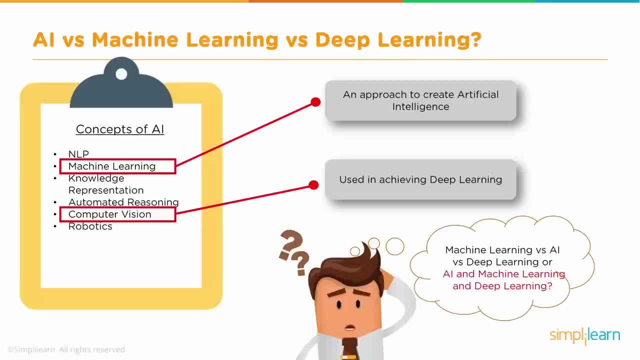 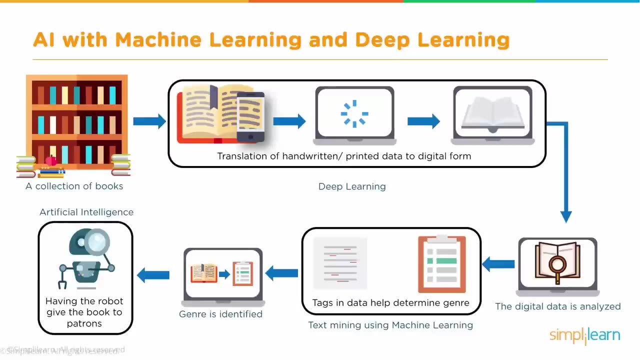 Knowledge representation, automated reasoning, computer vision, robotics, Machine learning versus AI versus deep learning or AI and machine learning and deep learning. So we look at this: We have AI with machine learning and deep learning, And so we're going to put them all together. 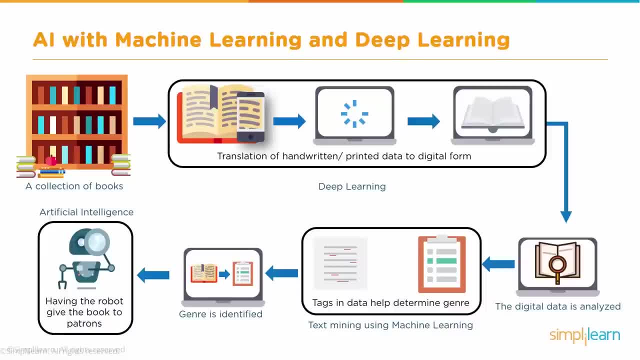 We find out that AI is the big picture. We have a collection of books. It goes through some deep learning. The digital data is analyzed. Text mining comes through. The particular book you're looking for- maybe it's a genre of books- is identified. 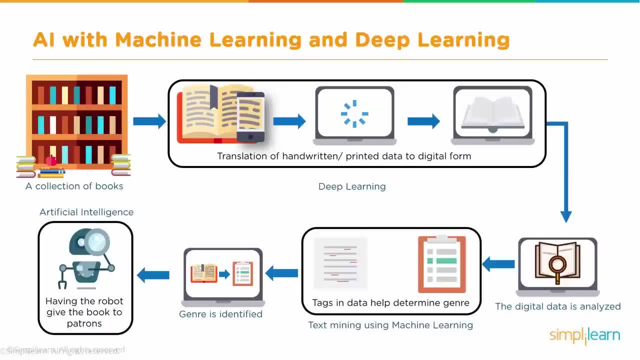 And in this case we have a robot that goes and gives a book to the patron. I have yet to be at a library that has a robot: bring me a book, But that will be cool when it happens. So we look at some of the pieces here. 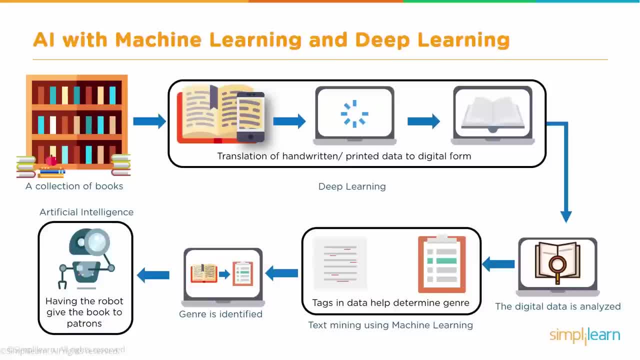 This information goes into as far as this example- the translation of the handwritten printed data to digital form. That's pretty hard to do. That's pretty hard to go in there and translate hundreds and hundreds of books and understand what they're trying to say if you've never read them. 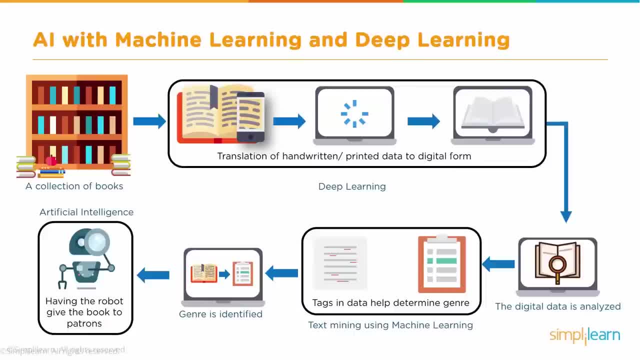 So in this case we use the deep learning, because you can already use examples where they've already classified a lot of books, And then they can compare those texts and say, oh okay, this is a book on automotive repair, This is a book on robotic building. 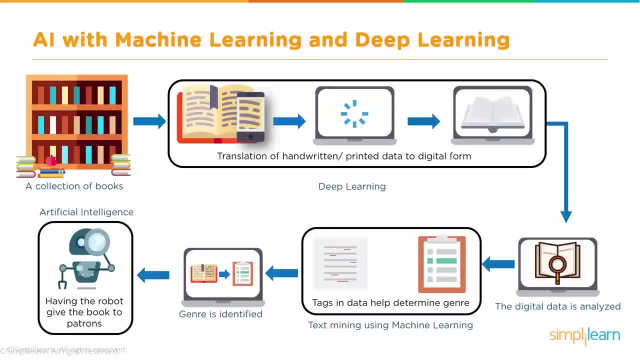 The digital data is analyzed, Then we have more text mining using machine learning. So maybe we'd use a different program to do a basic classify what you're looking for and say: oh, you're looking for auto repair and computers, So you're looking for automated cars. 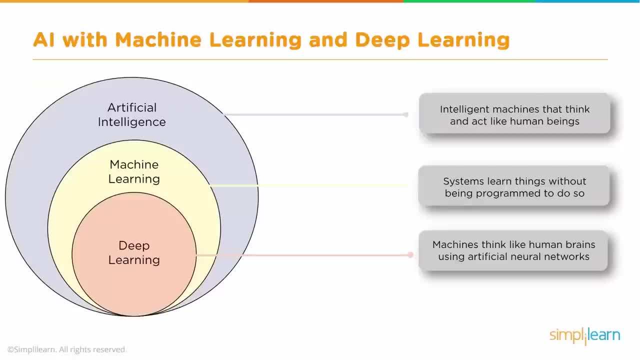 Once it's identified, then of course it brings you the book. So here's a nice summation of what we were just talking about: AI with machine learning and deep learning. Deep learning is a subset of machine learning, which is a subset of artificial intelligence. 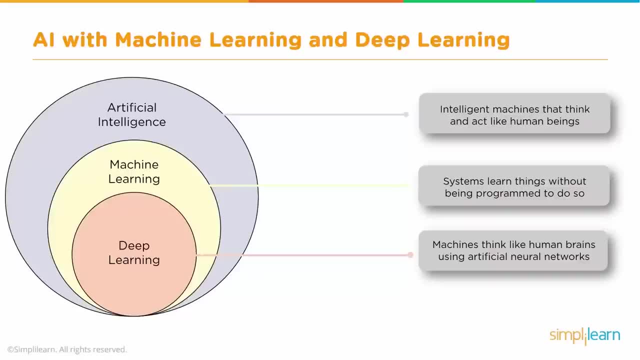 So you can look at artificial intelligence as the big picture. How does this compare to the human experience in either doing the same thing as a human we do or does it better than us? And machine learning, which has a lot of tools, is something that learns from data. 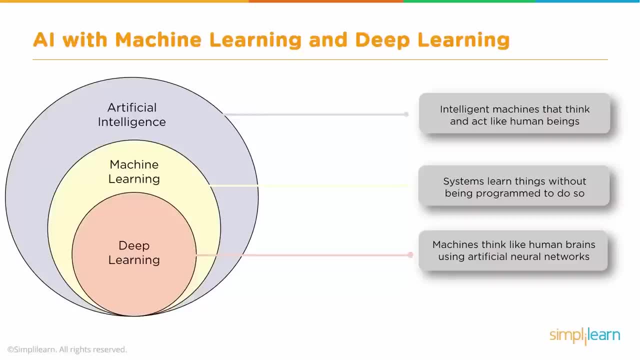 Past experiences, It's programmed, It comes in there and it says, hey, we already had these five things happen. The sixth one should be about the same. And then there's a lot of tools in machine learning, But deep learning, then, is a very specific tool in machine learning. 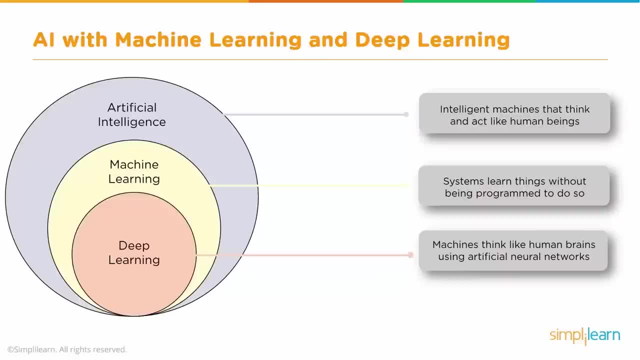 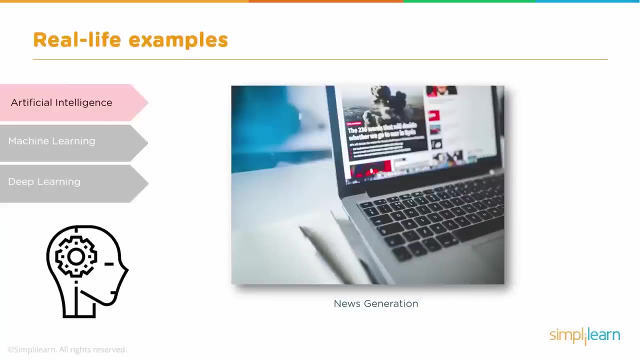 It's the artificial neural network which handles large amounts of data and is able to take huge pools of experiences, pictures and ideas and bring them together. Real life examples: Artificial intelligence- News generation, Very common nowadays, as it goes through there and finds the news articles or generates the news based upon the news feeds or the back end coming in. 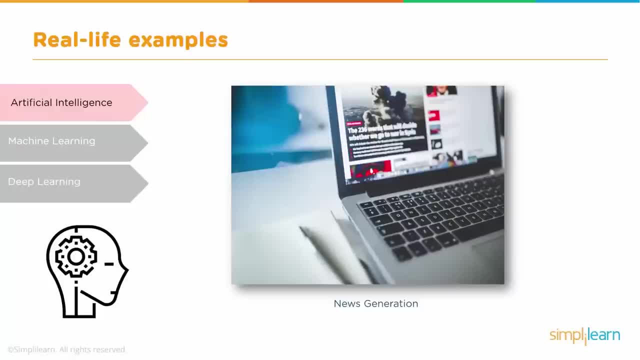 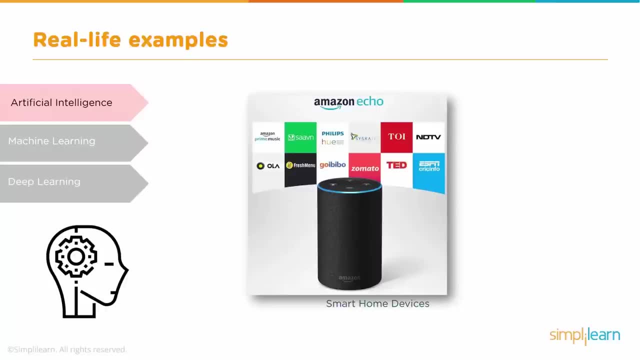 It says: okay, let's give you the actual news based on this. There's all the different things: Amazon Echo, They have a number of different Prime Music on there. Of course, there's also the Google Command And there's also Cortana. 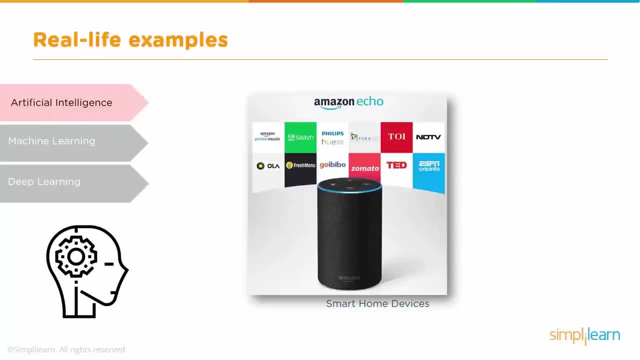 There's tons of smart home devices now where we can ask it questions. We don't have to turn the TV on or play music for us. That's all artificial intelligence From front to back. you're having a human experience with these computers and these objects that are connected to the processing. 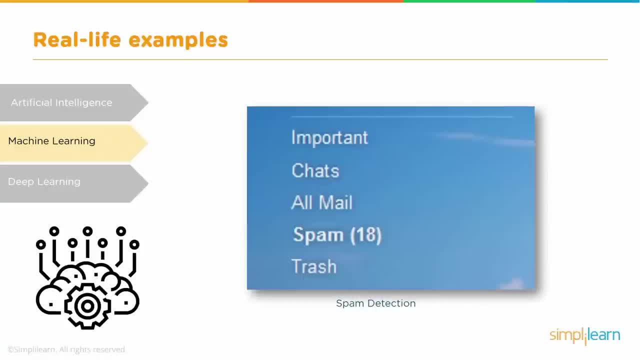 Machine learning, Spam detection- Very common Machine learning doesn't really have the human interaction part. So this is the part where it goes and says, okay, that's a spam, That's not a spam, And it puts it in your spam folder. 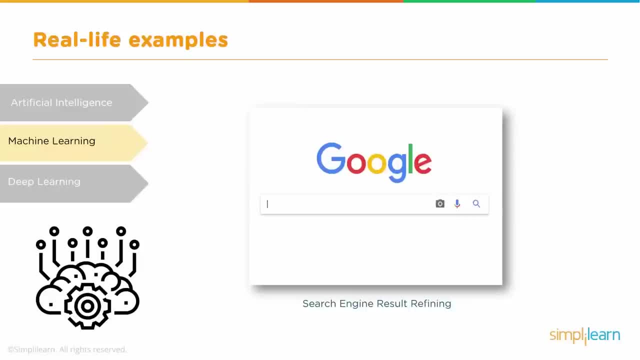 Search engine result refining. Another example of machine learning. Whereas it looks at your different results and it is able to categorize them, as far as this had the most hits, This is the least viewed. This has five stars, You know. however, they want to weight it. 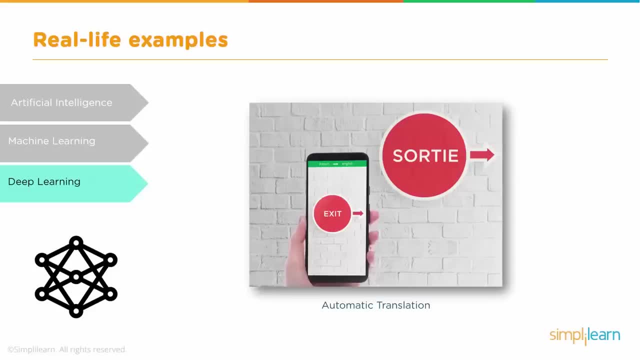 All good examples of machine learning. And then the deep learning. Deep learning- another example is, as you have like an exit sign. In this case it's translating it into French: Sortie. I hope I said that right. The neural network has been programmed with all these different words and images. 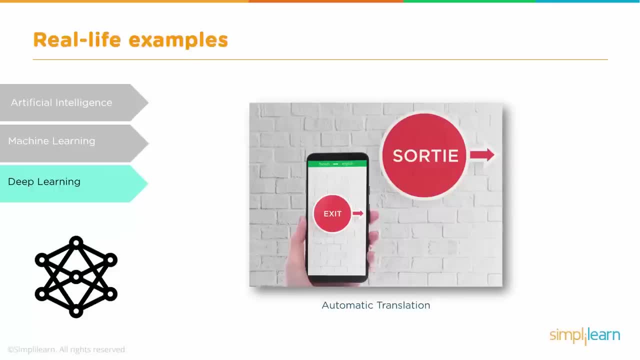 And so it's able to look at the exit in the middle And it goes: okay, we want to know what that is in French, And it's able to push that out in French and learn how to do that. And then we have chat bots. 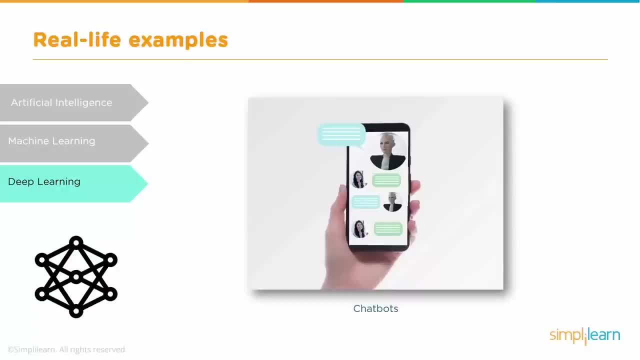 I remember when Microsoft first had their little paper clip Boy- that was like a long time ago. They came up and you would type in there and chat with it. These are growing. You know, it's nice to just be able to ask a question and it comes up and gives you the answer. 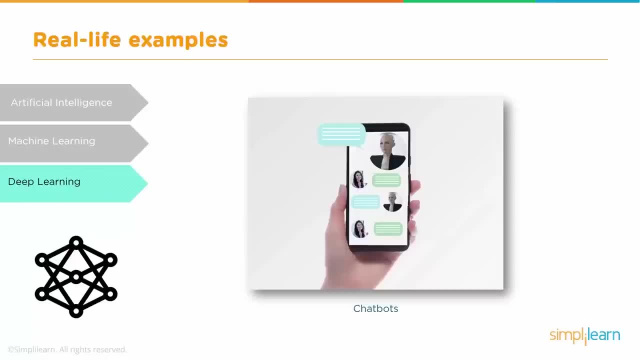 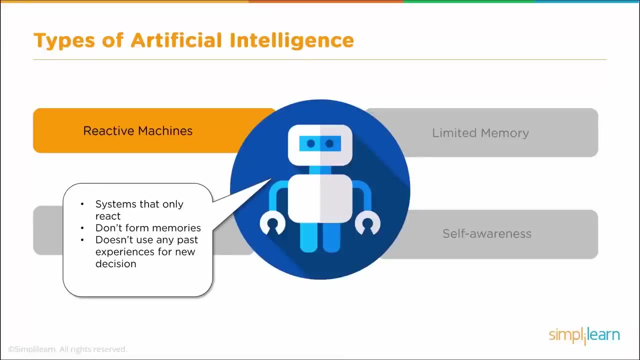 And instead of it being where you're just doing a search on certain words, it's now able to start linking those words together and form a sentence in that chat box. Types of AI and machine learning. Types of artificial intelligence. This and the next few slides are really important. 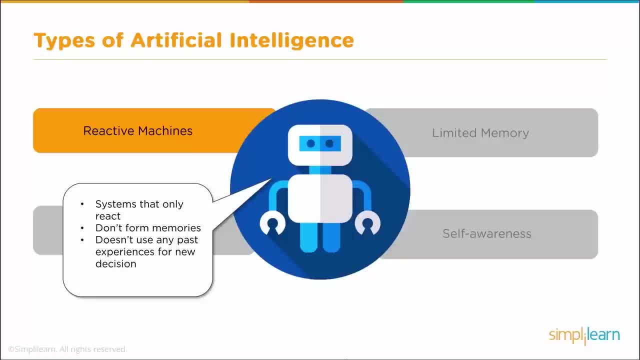 So one of the types of artificial intelligence is reactive machines, Systems that only react. They don't form memories, They don't have past experiences. They have something that happens to them and they react to it. My washing machine is one of those. 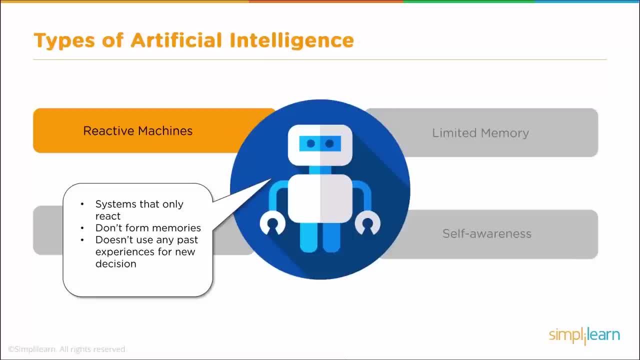 If I put a ton of clothes in it and they get all clumped on one side, it automatically adds a weight to reciter it. So my washing machine is actually a reactive machine. working with whatever the load is, It keeps it nice and so when it spins it doesn't go thumping against the side. 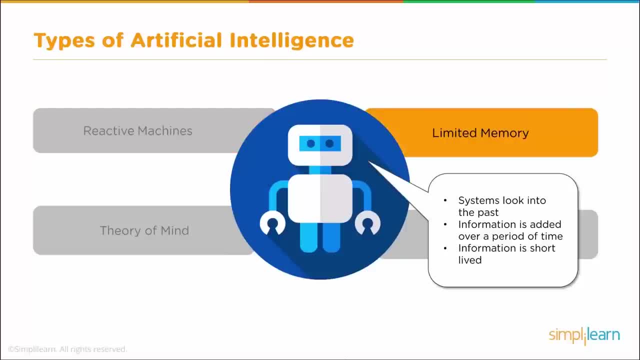 Limited memory. Artificial intelligence systems look into the past. Information is added over a period of time and information is short lived. When we're talking about this and you look at like a neural network that's been programmed to identify cars, it doesn't remember all those pictures. 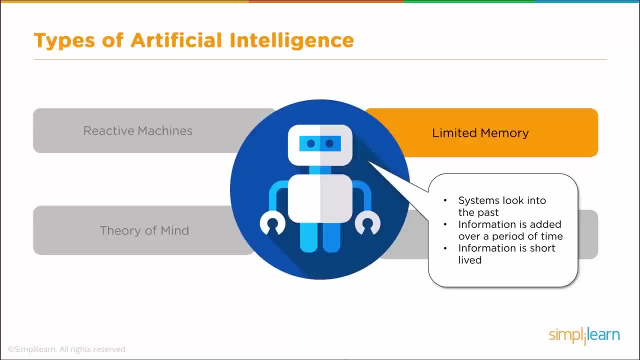 It has no memory as far as the hundreds of pictures you process through it. All it has is: this is the pattern I used to identify cars as the final output for that neural network we looked at. So when they talk about limited memory, this is what they're talking about. 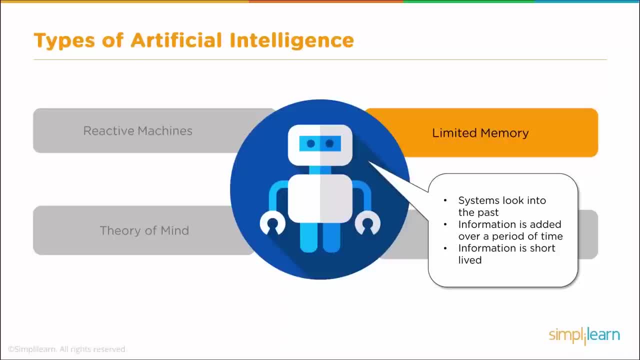 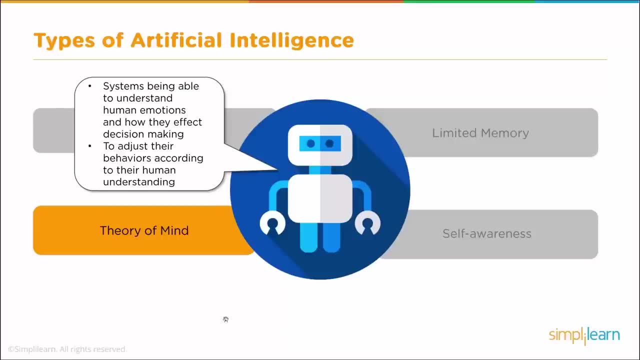 They're talking about. I've created this based on all these things, but I'm not going to remember any one specifically Theory of mind Systems being able to understand human emotions and how they affect decision making, to adjust their behaviors according to their human understanding. 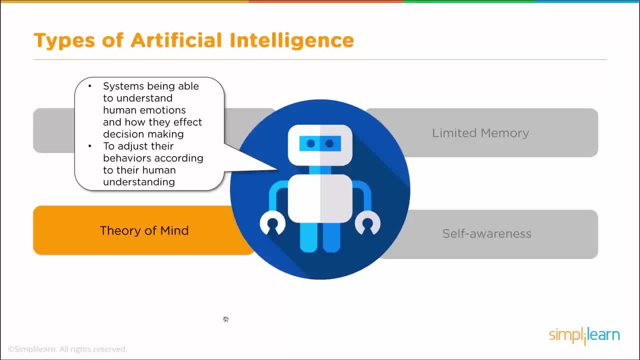 This is important because this is our page mark. This is how we know whether it is an artificial intelligence or not. Is it interacting with humans in a way that we can understand? Without that interaction, it's just an object. So when we talk about theory of mind, 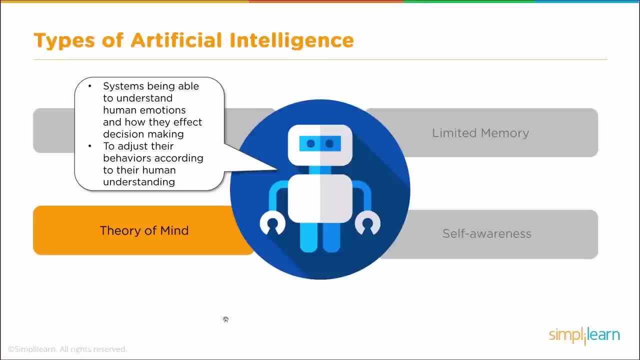 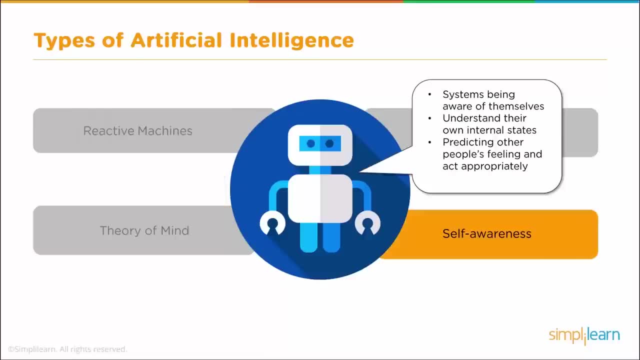 we really understand how it interfaces that whole. if you're in web development, user experience would be the term I would put in there. So the theory of mind would be user experience. How is the whole UI connected together? And one of the final things, as we get into artificial intelligence, 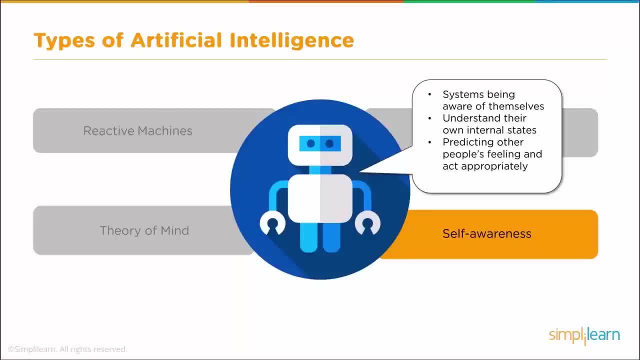 is systems being aware of themselves, understanding their internal states and predicting other people's feelings and act appropriately. So as artificial intelligence continues to progress, we see ones that are trying to understand well what makes people happy. How would they increase our happiness? 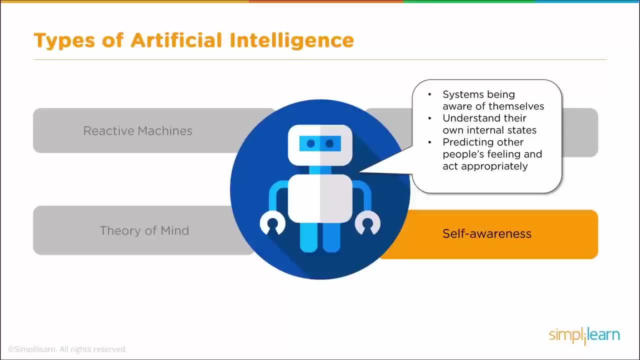 How would they keep themselves from breaking down? if something's broken inside, They have that self-awareness to be able to fix it And, just based on all that information, predicting which action would work the best. What would help people If I know that you're having a cup of coffee? 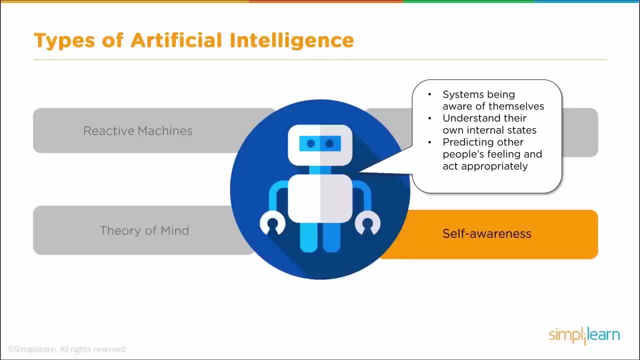 first thing in the morning is what makes you happy. as a robot, I might make you a cup of coffee every morning at the same time to help your life and help you grow. That would be the self-awareness as being able to know all those different things. 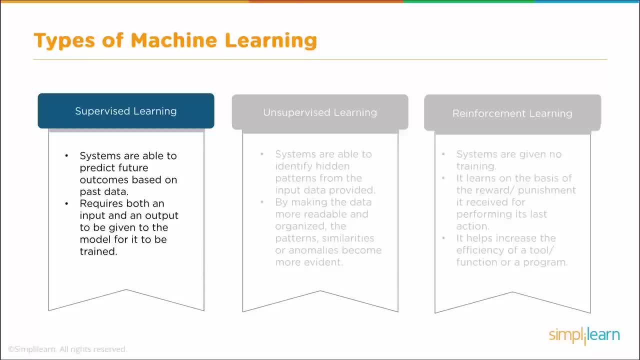 Types of machine learning and, like I said on the last slide, this is very important If you decide to go in and get certified in machine learning or know more about it. these are the three primary types of machine learning. The first one is supervised learning. 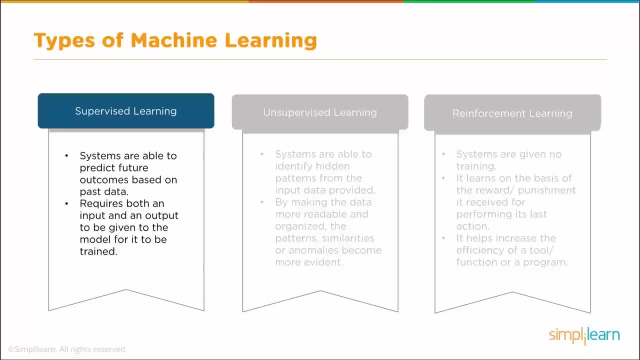 Systems are able to predict future outcome based on past data. It requires both an input and an output to be given to the model for it to be trained. So in this case we're looking at anything where you have a hundred images of a bicycle and those hundred images, you know, are bicycle. 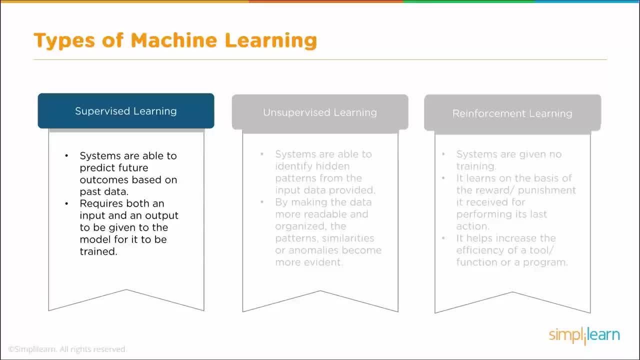 So they're pre-set. Someone already looked at all hundred images and said: these are pictures of bicycles, And so the computer learns from those, and then it's given another picture, and maybe the next picture is a bicycle, and it says: oh, that resembles all these other bicycles. 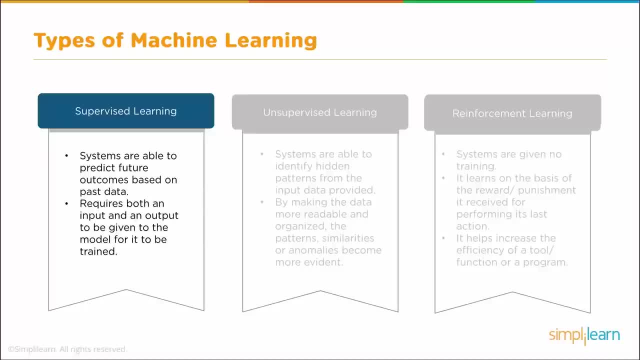 so it's a bicycle And the next one's a car and it says it's not a bicycle. That would be supervised learning and we had to train it. We had to supervise it. Unsupervised learning Systems are able to identify hidden patterns. 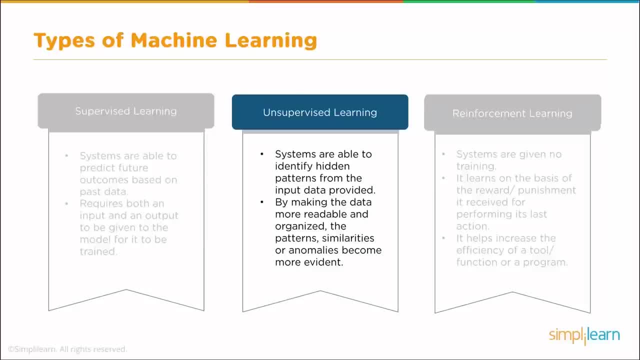 from the input data provided. by making the data more readable and organized, The patterns, similarities or anomalies become more evident. You'll heard the term cluster. How do you cluster things together? Some of these things go together. some of these don't. 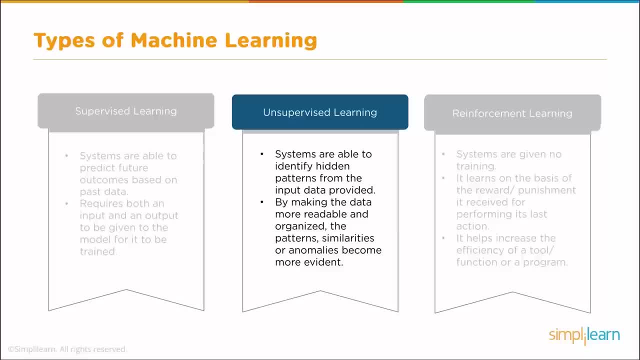 This is unsupervised, where you can look at an image and start pulling the different pieces of the image out because they aren't the same. The human, all the parts of the human, are not the same because there's a fuzzy tree behind them, because it's slightly out of focus. 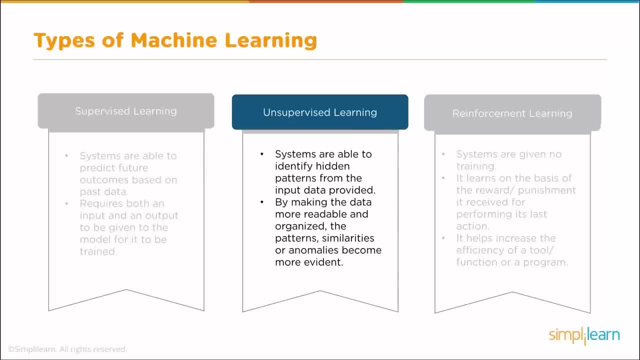 which is not the same as the beach ball. It's unsupervised, because we never told it what a beach ball was, We never told it what the human was and we never told it that those were trees. All we told it was: hey, separate this picture. 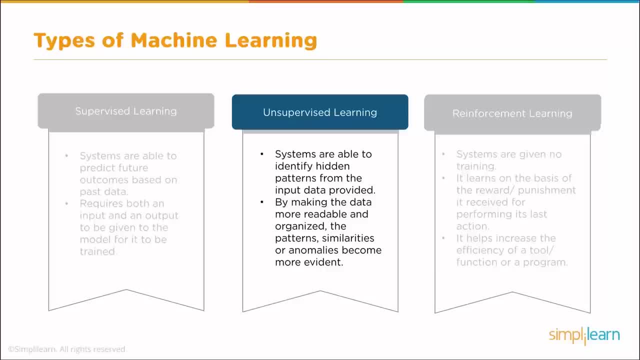 by things that don't match and things that do match and come together. And finally there's reinforcement. learning Systems are given no training. It learns on the basis of the reward punishment it received for performing its last action. It helps increase the efficiency of a function or a program. 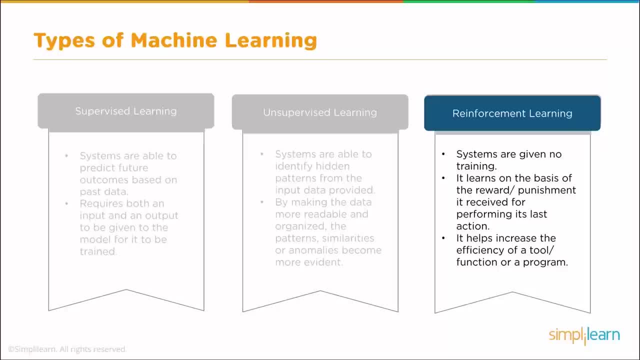 Reinforced learning or reinforcement learning is kind of you, give it a yes or no. Yes, you gave me the right response, No, you didn't. And then it looks at that and says, oh okay, so based on this data coming in, what I gave you was a wrong response. 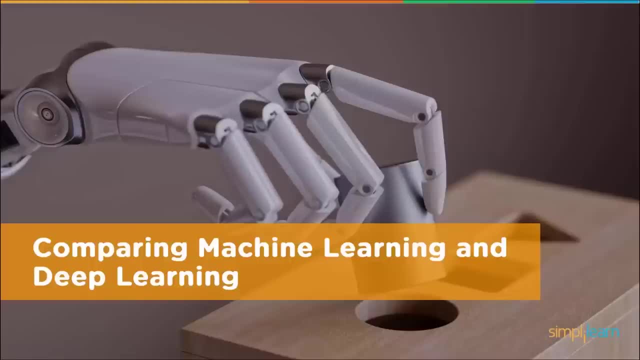 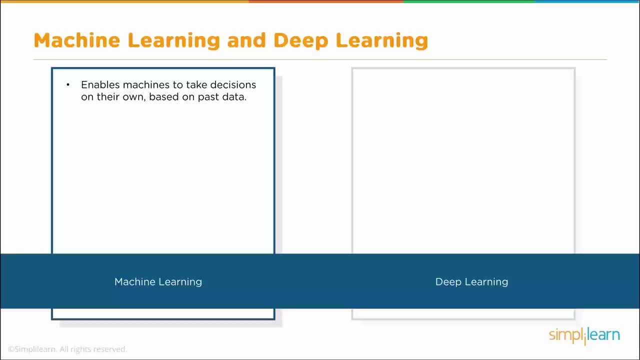 so next time I'll give you a different one, Comparing machine learning and deep learning. So remember that deep learning is a subcategory of machine learning, So it's one of the many tools, And so we're grouping a ton of machine learning tools all together. 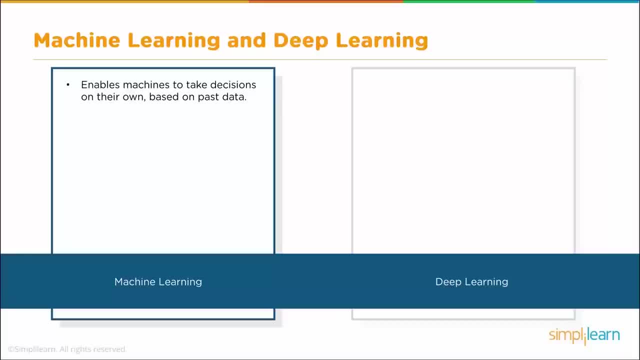 There's regression, k-means, clustering. there's all kinds of cool tools out there you can use in machine learning. Enables machines to take decisions, to make decisions on their own based on past data. Enables machines to make decisions with the help of artificial neural networks. 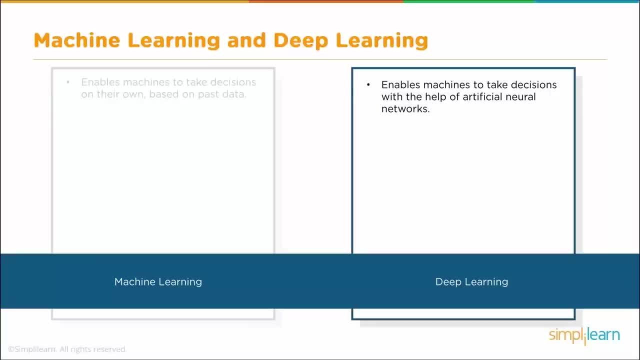 So it's doing the same thing, but we're using an artificial neural network, as opposed to one of the more traditional machine learning tools- Needs only a small amount of training data. This is very important. When you're talking about machine learning, they're usually not talking about huge amounts of data. 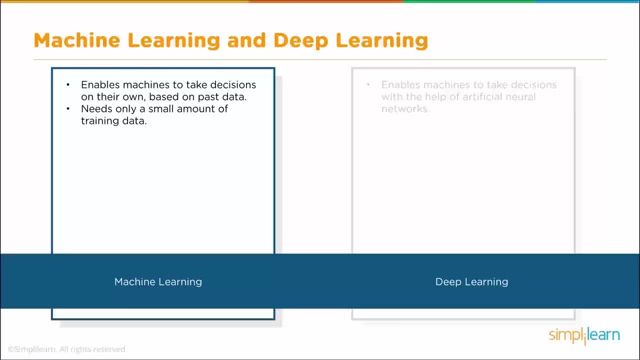 We're talking about maybe your spreadsheet from your business and your totals for the end of the year. When you're talking about neural networks, you usually need a large amount of data to train the data, So there's a lot of training involved If you have under 500 points of data. 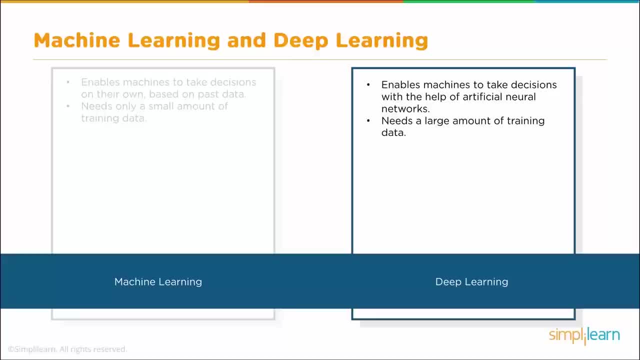 that's probably not going to go into machine learning, Or maybe you have, like in the case of one of the things, 500 points of data and 30 different fields. It starts getting really confusing there in artificial intelligence or machine learning and the deep learning aspect really shines. 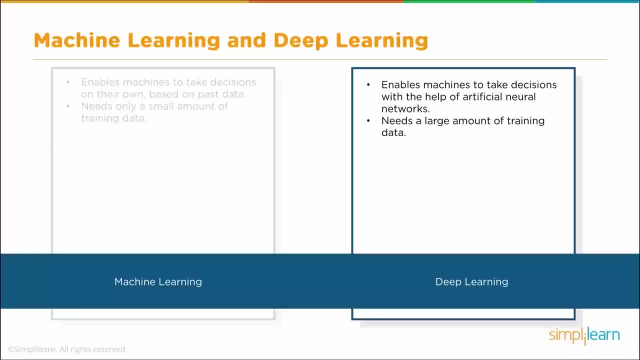 when you get to that larger data that's really complex. Works well on low-end systems. So a lot of the machine learning tools out there you can run on your laptop with no problem and do the calculations there, Where, with the machine learning, it usually needs a higher-end system to work. 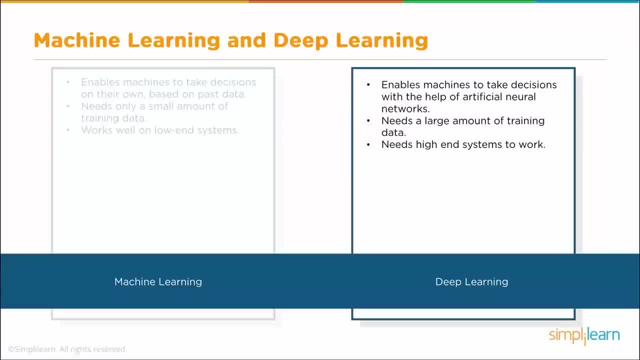 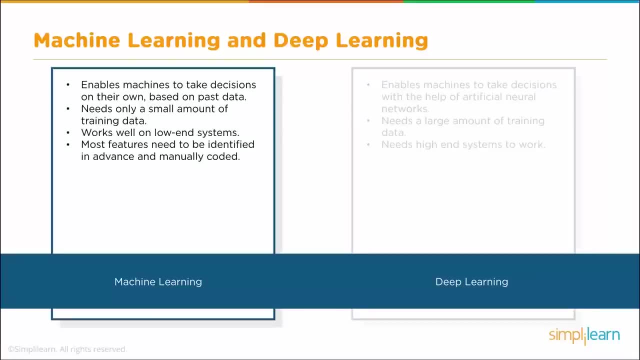 It takes a lot more processing power to build those neural networks and to train them. It goes through a lot of data. We're talking about the general machine learning tools. Most features need to be identified and advanced and manually coded, So there's a lot of human work on here. 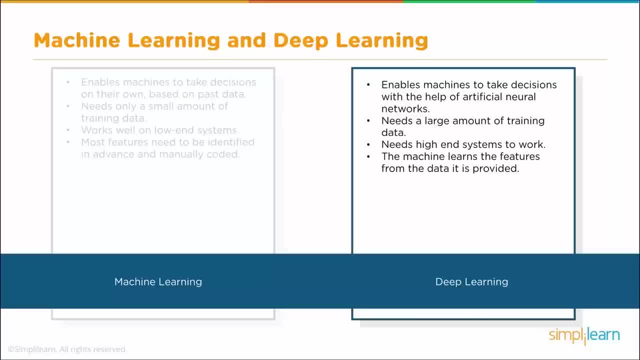 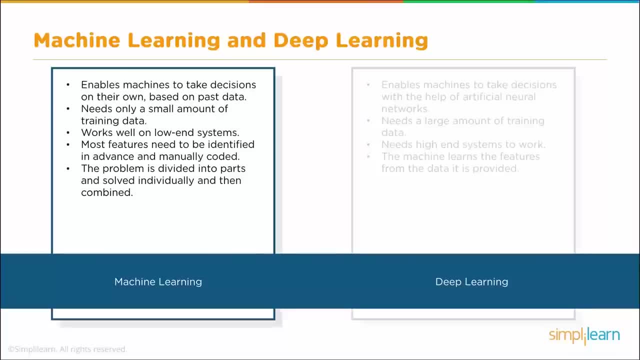 The machine learns the features from the data it is provided. So again, it's like a magic box. You don't have to know what a tire is, It figures it out for you. The problem is divided into parts and solved individually, and then combined. 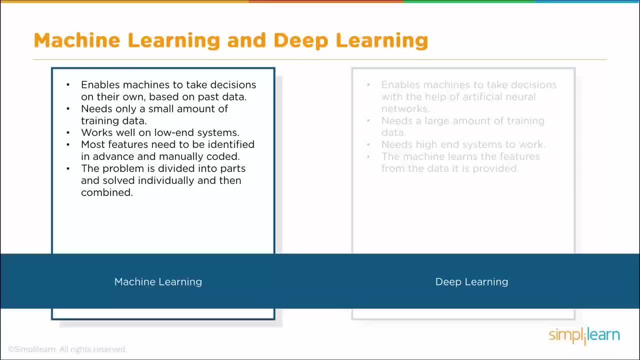 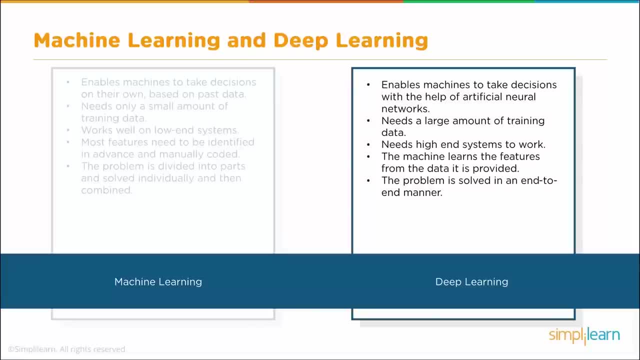 So in machine learning you usually have all these different tools and use different tools for different parts, And the problem is solved in an end-to-end manner. So you only have one neural network or two neural networks bringing the data in and putting it out. 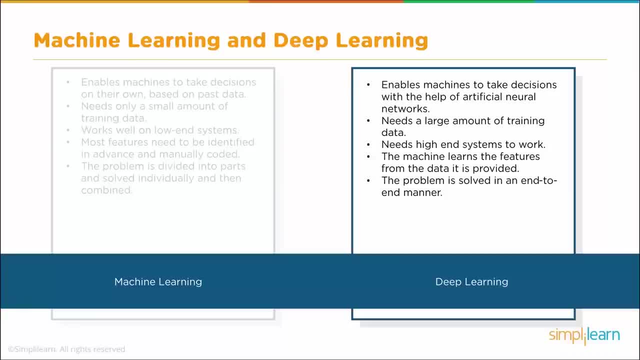 It's not going through a lot of different processes to get there. And remember you can put machine learning and deep learning together So you don't always have just the deep learning solving the problem. You might have it solving one piece of the puzzle. 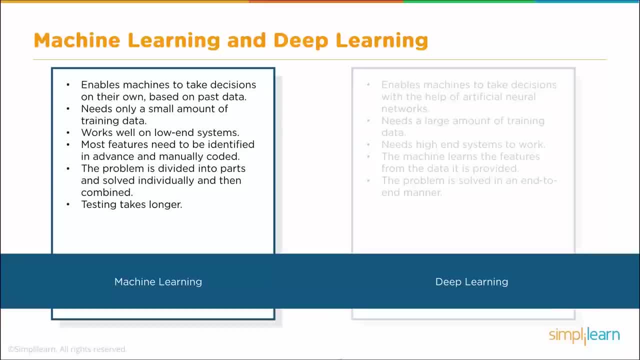 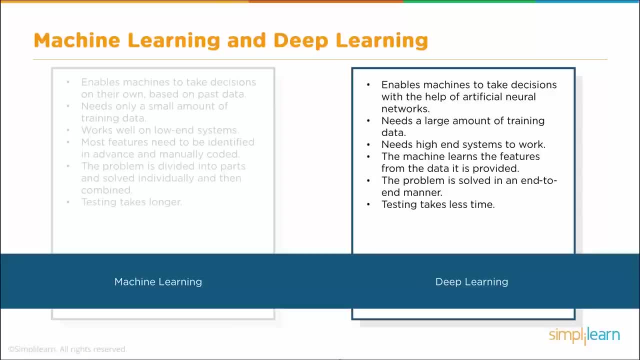 With regular machine learning and most machine learning tools out there, they take longer to test and understand how they work, And with the deep learning it's pretty quick. Once you build that neural network, you test it and you know. So we're dealing with very crisp rules. 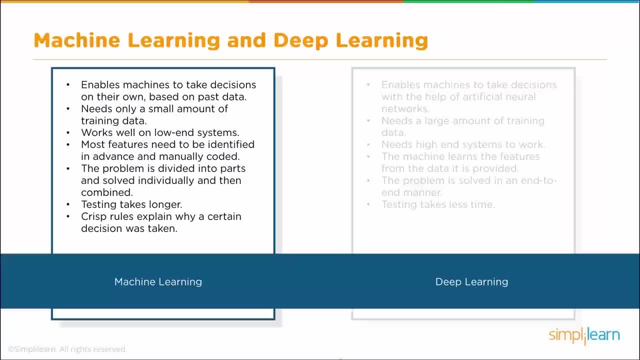 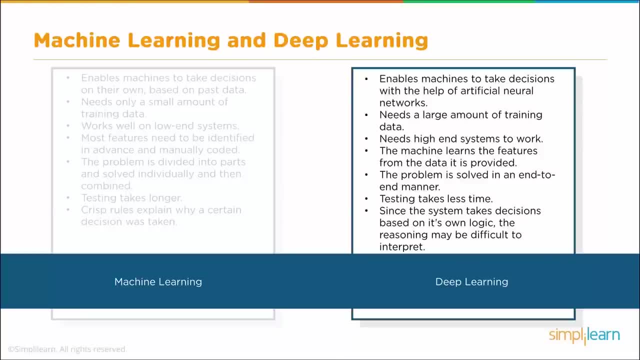 very clear sources. You have to really explain how the decision was made when you use most machine learning tools. But when you use the deep learning tool inside the machine learning tools, the system takes care of it based on its own logic and reasoning, And again it's like a magic black box. 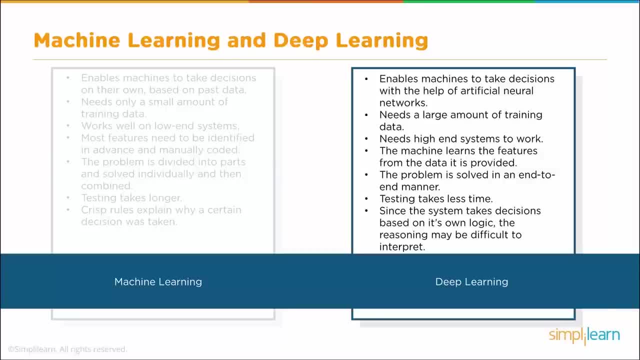 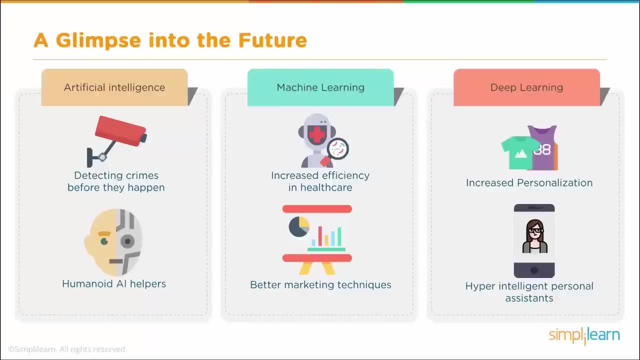 You really don't know how it came up with the answer. You just know it came up with the right answer, A glimpse into the future. So a quick glimpse into the future: Artificial intelligence. Be using it to detecting crimes before they happen. 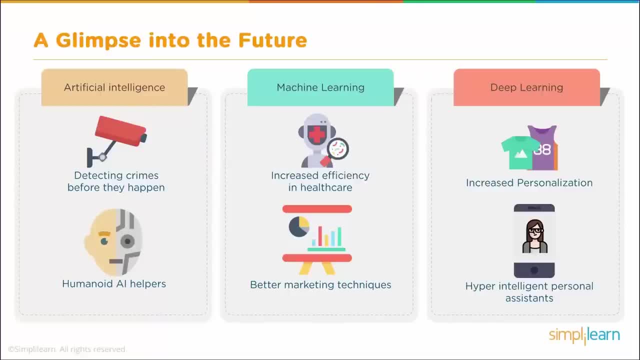 AI helpers, which we already have a lot of, There'll be more and more. Maybe it'll actually be androids. That'd be cool to have an android that comes and gets stuff out of my fridge for me. Machine learning: Increasing efficiency in healthcare. 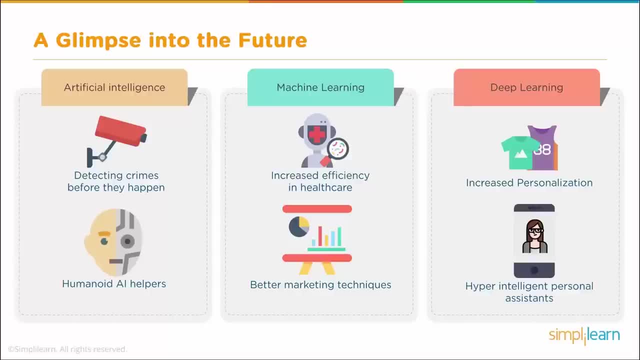 That's really big. in all the forms of machine learning, Better marketing techniques, Any of these things. if we get into the sciences it's just off the scale. Machine learning and artificial intelligence go everywhere. And then the subcategory deep learning. 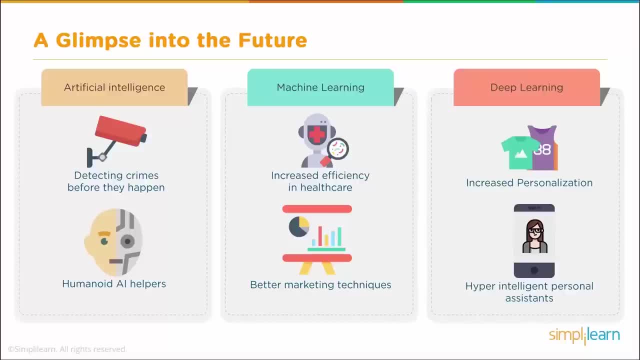 Increased personalization. So what's really nice about the deep learning is we can start now catering to you. That'll be one of the things we see more and more of, And we'll have more of a hyper intelligent personal assistant. I'm excited about that. 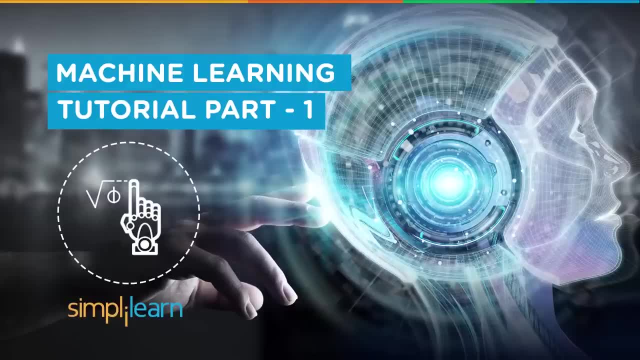 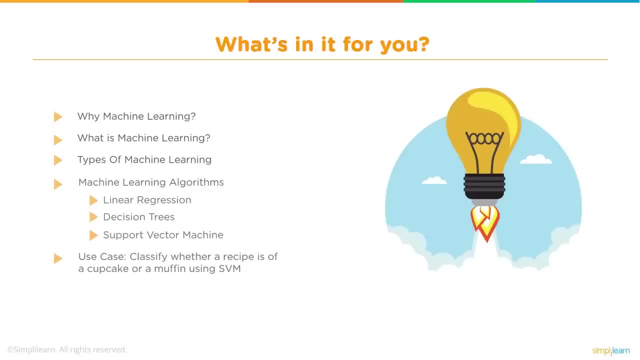 Hello and welcome to Machine Learning Tutorial Part 1.. This is part 1 of a machine learning series put on by Simply Learn. What's in it for you today? Well, we'll start off with a brief explanation of why machine learning and what is machine learning. 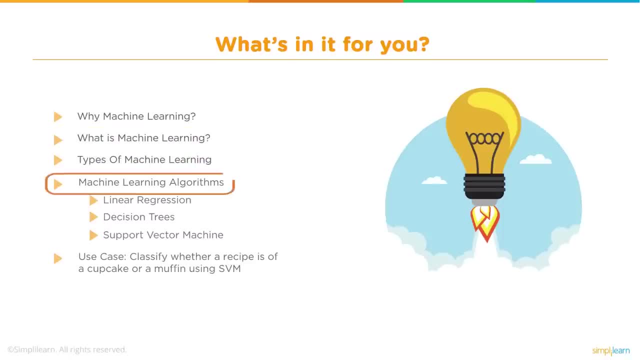 And then we'll get into a few of the types of machine learning: Machine learning algorithms, linear regression, decision trees, support vector machine and finally we'll do a use case where we're going to classify whether a recipe is of a cupcake or a muffin. 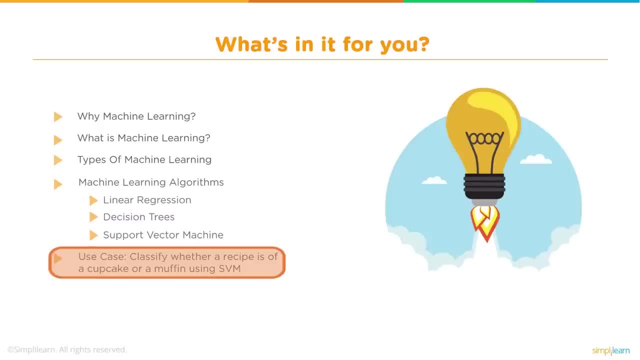 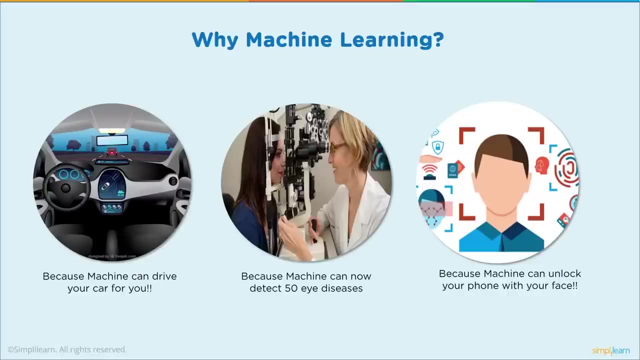 using the SVM or the support vector machine Sounds like a delicious way to explore machine learning. So why machine learning? Why do we even care about having these computers come up and be able to do all these new things for us? Well, because machines. 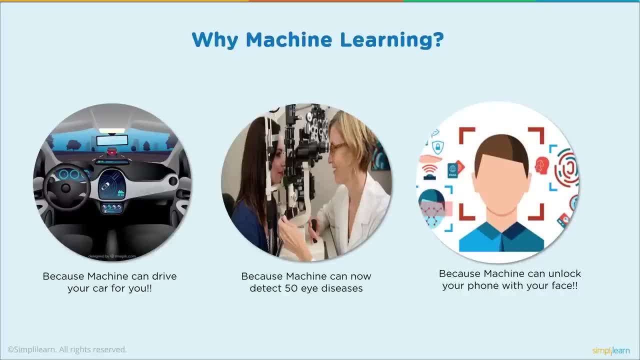 can now drive your car for you. It's still very in the infant stage, but it's just exploding, as we see with Google's Waymo. and then Uber had their program, which unfortunately crashed. They know that this is huge. This is going to be the huge industry. 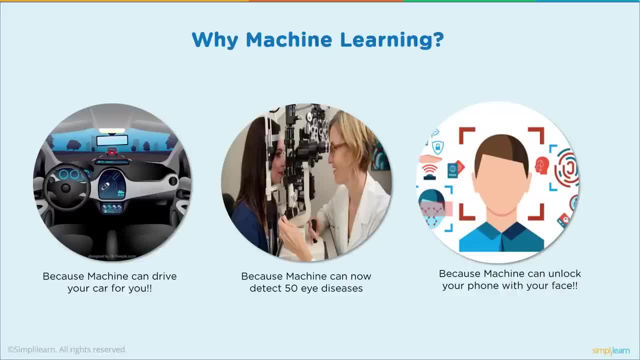 to change our whole transportation infrastructure. Machine learning has now used to detect over 50 eye diseases. Do you know how amazing that is to have a computer that double checks for the doctor for things they might miss? That's just huge in the health industry. 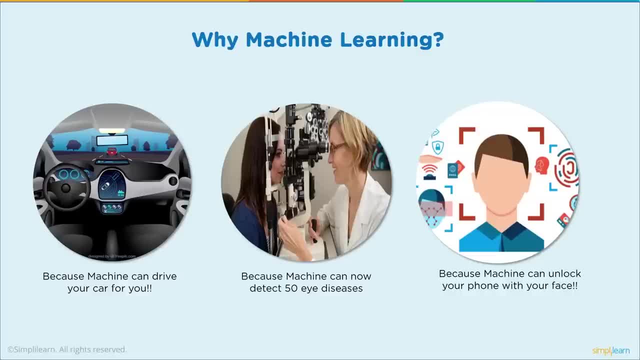 Pretty soon. they actually do already have that in some areas where- maybe not for eyes but for other diseases- where they're using the camera on your phone to help pre-diagnose the doctor, And because the machine can now unlock your phone with your face. 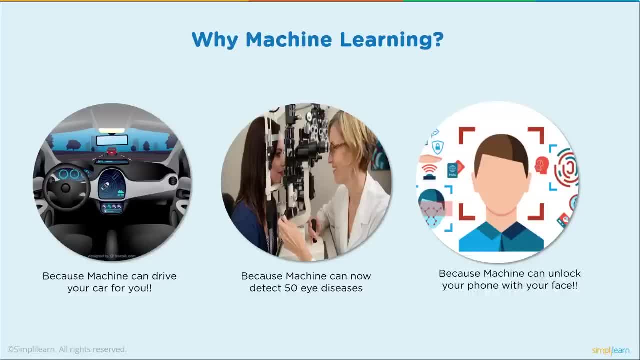 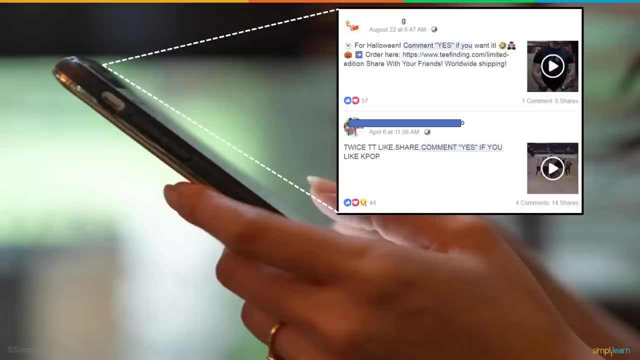 I mean that's just cool Having it be able to identify your face or your voice and be able to turn stuff on and off for you, depending on where you're at and what you need. Talk about an ultimate automation with our world we live in. 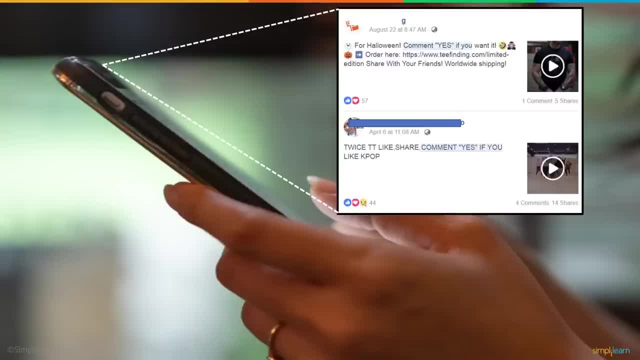 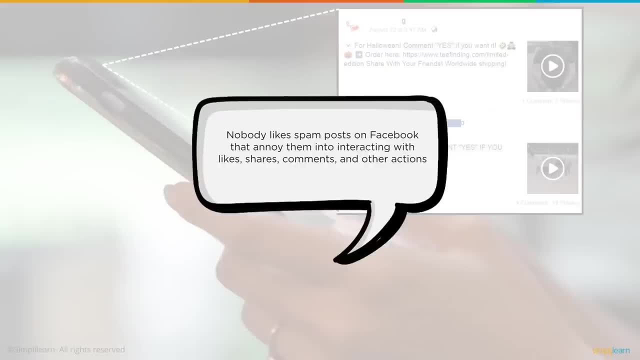 And as we dig in deeper, we have a nice example of Facebook. As you can see here, they have the Facebook post with Halloween Comment. yes, if you want it, Order here. Nobody likes spam posts on Facebook unless you're interacting with likes, shares. 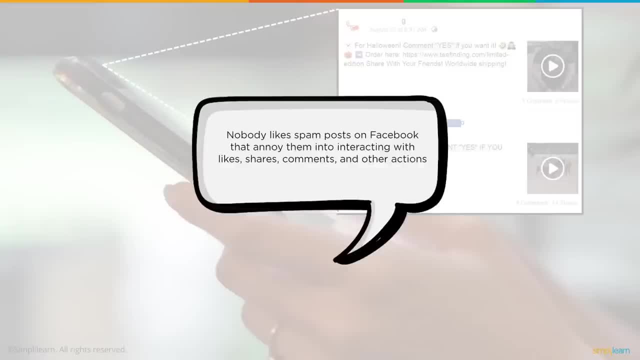 comments and other actions. I remember the original ones were all: if you don't click on here, you will have bad luck or some kind of fear factor. Well, this is a huge thing in social media when people are getting spammed, And so this tactic. 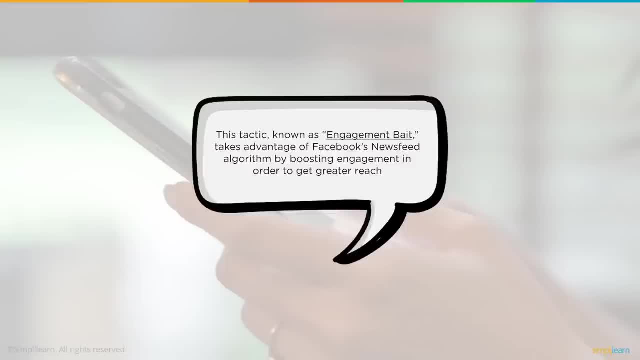 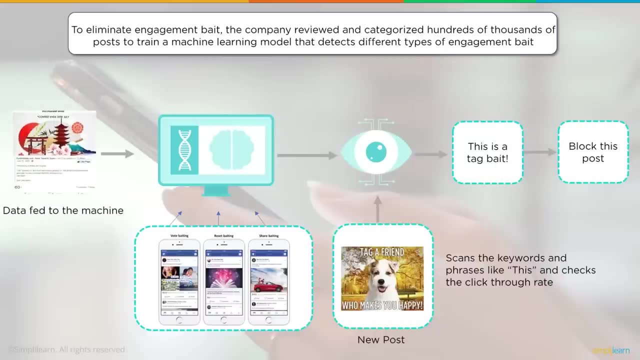 known as engagement bait, takes advantage of Facebook's newsfeed algorithm by choosing engagement in order to get the greater reach. To eliminate engagement bait, the company reviewed and categorized hundreds of thousands of posts to train a machine learning model that detects different types of engagement bait. 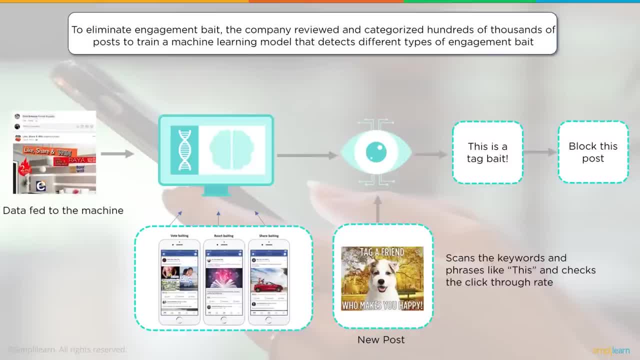 So in this case we have, we're using Facebook, but this is, of course, across all the different social media. They have different tools, they're building And the Facebook scroll GIF will be replaced, Kind of like a virus coming in there. It notices that there's a certain setup. 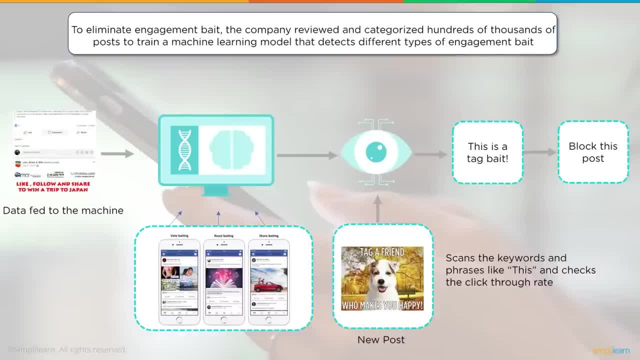 with Facebook and it's able to replace it, And they have like: vote baiting, react baiting, share baiting. They have all these different. these are kind of general titles, But there certainly are a lot of ways of baiting you to go in there and click on something. 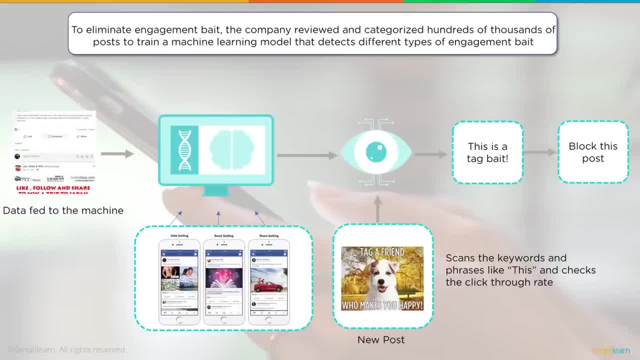 So they fed all this. This data was fed into the machine, And then they have the new post. The new post comes up that takes over part of the Facebook setup, And that's what you're looking at. You're looking at this new post. that's replaced. 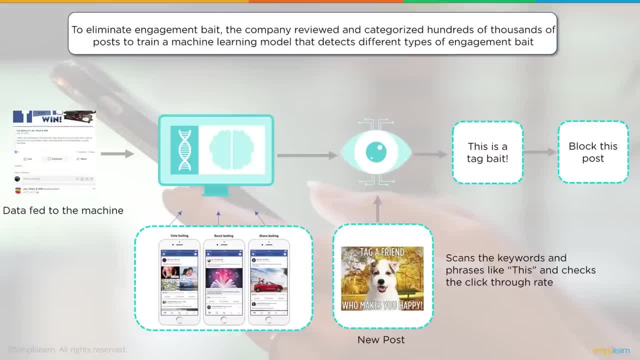 like a virus, has replaced that. So what Facebook did to eliminate this is they start scanning for keywords and phrases like this And checks the click through rate, So it starts looking for people who are clicking through it without even looking at it Or clicking through it, and it's not something. 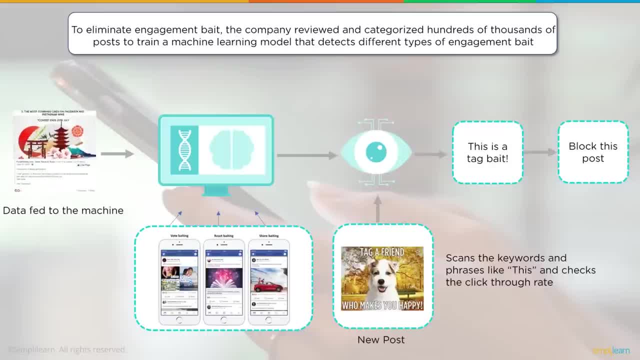 that you're looking at. It is now able to identify the spam coming in, And this makes your life easier, So you're not getting spammed. It's not like walking through an airport and in a lot of countries you have like hundreds of people trying to sell you timeshare. 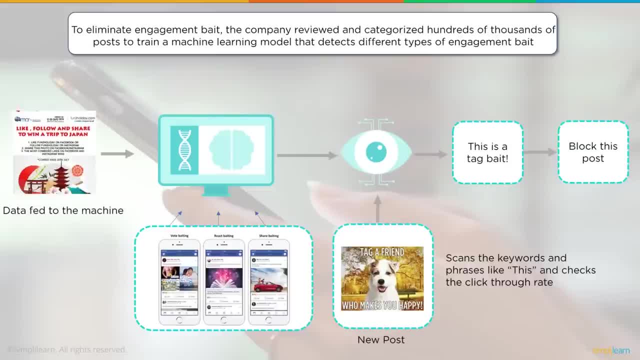 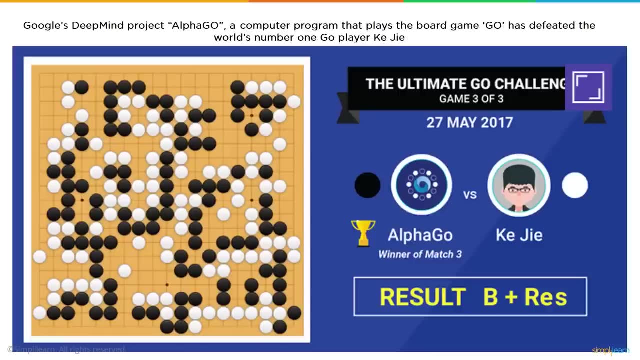 Come join us, Sign up for this. It eliminates that annoyance. So now you can just enjoy your Facebook and your cat pictures, Or maybe it's your family pictures- Mine is family. Certainly people like their cat pictures too. A program that plays a board game: Go. 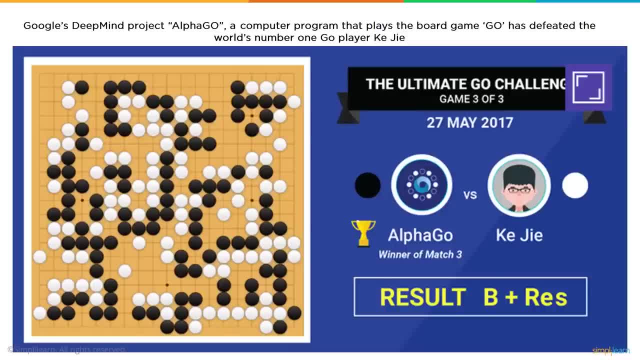 has defeated the world's number one Go player- And I hope I say his name right- Key G. The ultimate Go challenge game of three of three was on May 27, 2017.. So that was just last year that this happened. 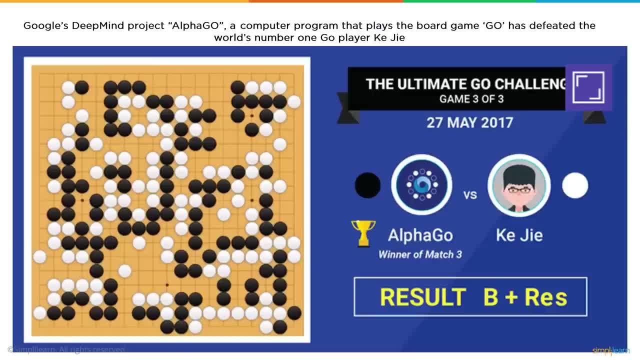 And what makes this so important is that Go is just a game, So it's not like you're driving a car or something in our real world, But they are using games to learn how to get the machine learning program to learn. They want it to learn. 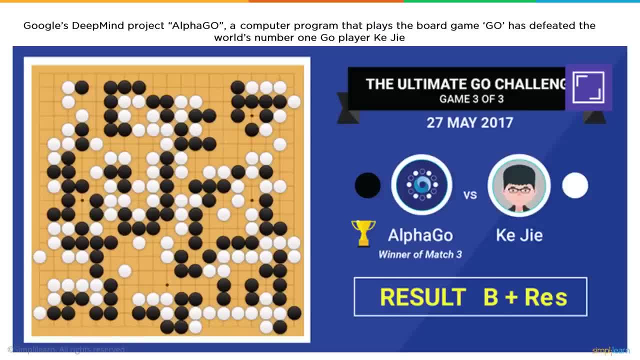 how to learn, And that is a huge step. A lot of this is still in its infant stage as far as development, As we saw what happened with the- as I referred to earlier- the Uber cars. They lost their whole division because they jumped ahead too fast. 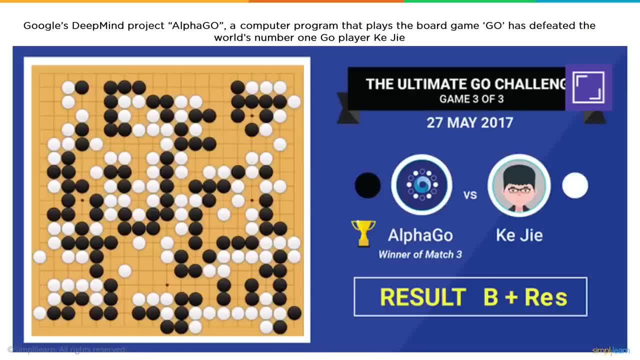 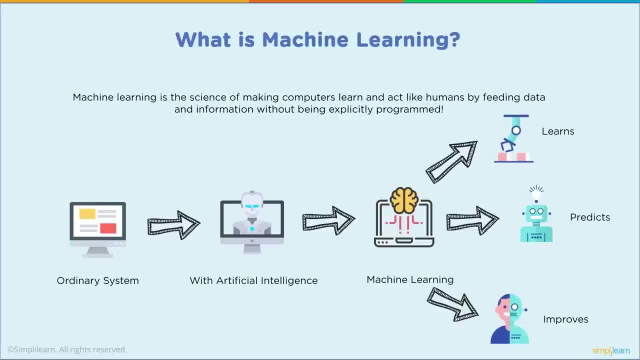 So it's still an infant stage, But boy is this like the beginning of just an amazing world that is automated in ways we can't even imagine what tomorrow is going to look like. We've looked at a lot of examples of machine learning. What is machine learning? 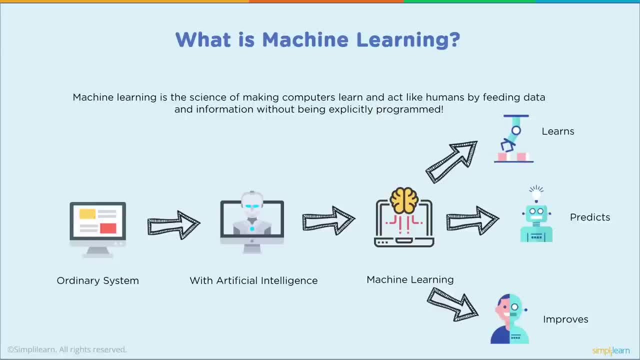 Machine learning is the science of making computers learn and act like humans by feeding data and information without being explicitly programmed. We see, here we have a nice little diagram where we have our ordinary system, Your computer. nowadays you can even run a lot of this stuff. 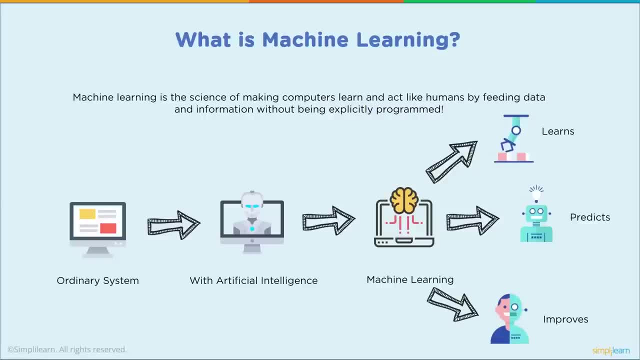 on a cell phone, because cell phones advance so much. And then, with artificial intelligence and machine learning, it now takes the data and it learns from what happened before, And then it predicts what's going to come next. And then really the biggest part right now: 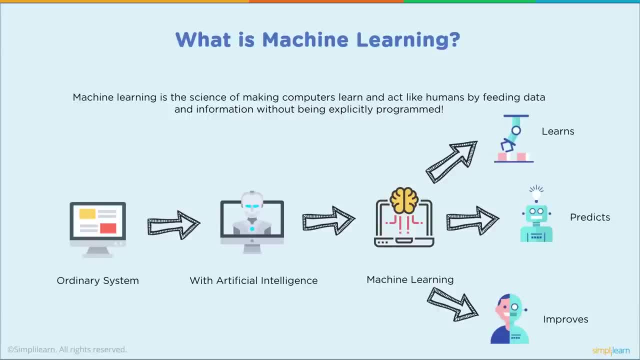 in machine learning that's going on, is it improves on that? How do we find a new solution? So we go from descriptive, where it's learning about stuff and understanding how it fits together, to predicting what it's going to do, to postscripting, coming up with a new solution. 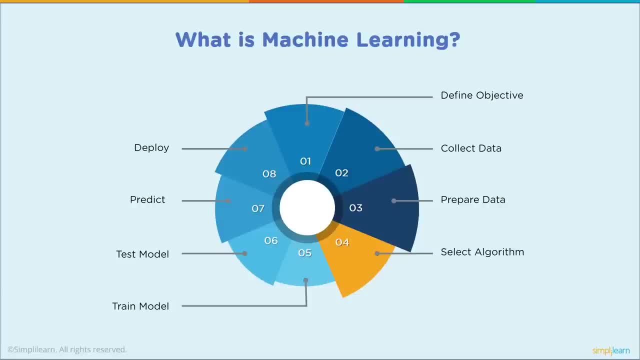 And when we're working on machine learning, there's a number of different diagrams that people have posted for what steps to go through. A lot of it might be very domain specific. So if you're working on bio-identification versus language, versus medical or physics, 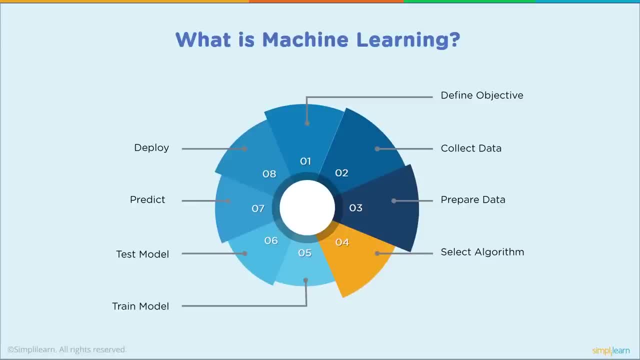 some of these are switched around a little bit or new things are put in that are very specific to the domain. This is kind of a very general diagram. First, you want to define your objective. Very important to know what it is you're wanting to predict. 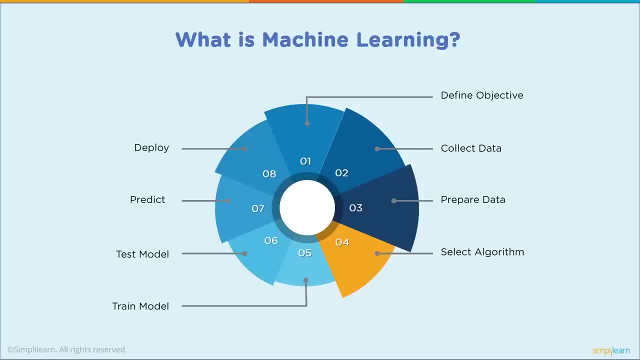 Then you're going to be collecting the data. So once you've defined an objective, you need to collect the data that matches. You spend a lot of time in data science, collecting data and the next step, preparing the data. There's the old saying. 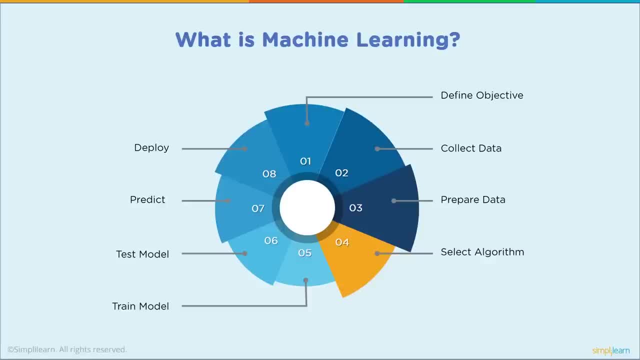 bad data in, bad answer out, Or bad data out, And then, once you've gone through and we've cleaned all this stuff coming in, then you're going to select the algorithm. Which algorithm are you going to use? You're going to train that algorithm. 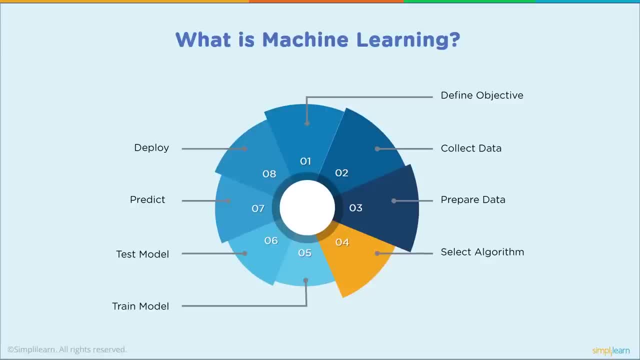 In this case, I think we're going to be working with SVM, the support vector machine. Then you have to test the model. Does this model work? Is this a valid model for what we're doing? And then, once you've tested it, you want to run your prediction. 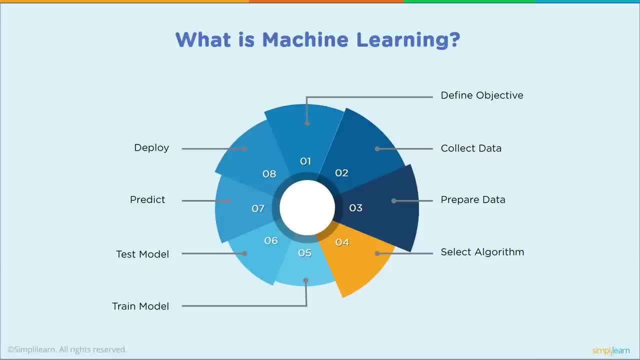 You want to run your choice or whatever output it's going to come up with And then, once everything is set and you've done lots of testing, then you want to go ahead and deploy the model. And remember I said domain specific, This is very general. as far as the scope, 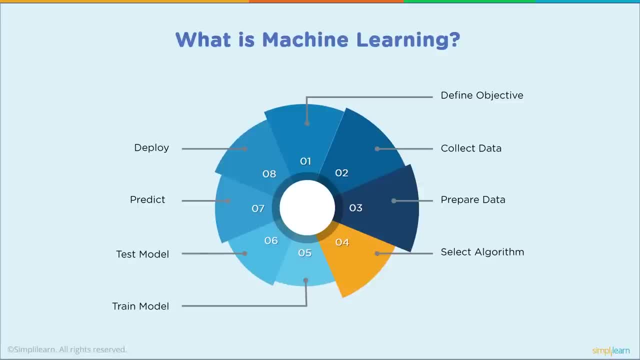 of doing something. A lot of models you get halfway through and you realize that your data is missing something And you have to go collect new data because you've run a test in here, someplace along the line and you're saying, hey, I'm not really getting the answers I need. 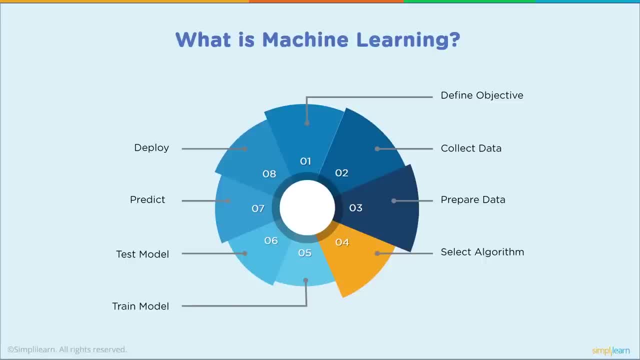 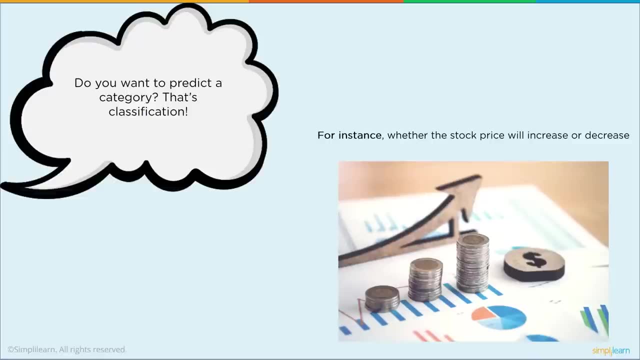 So there's a lot of things that are domain specific and it's a very good model to start with, And we do have some basic divisions of what machine learning does. that's important to know. For instance, do you want to predict a category? Well, if you're categorizing things, 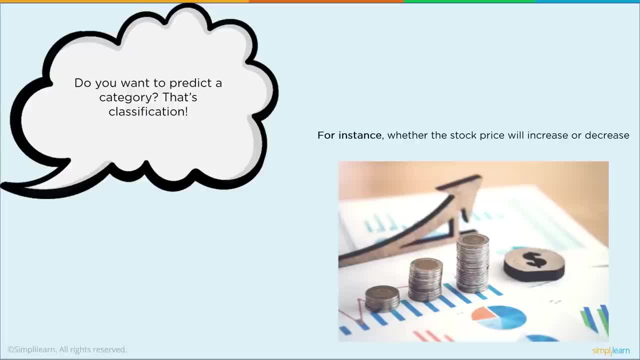 that's classification, For instance, whether the stock price will increase or decrease. So, in other words, I'm looking for a yes- no answer: Is it going up or is it going down? And in that case we'd actually say: is it going up, True? 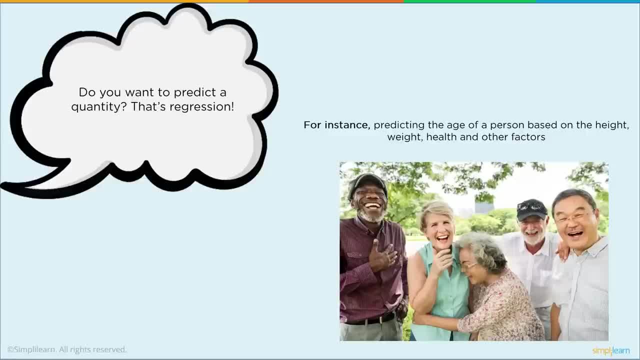 If it's not going up, it's false meaning, it's going down. And then there's quantity, That's regression. So, remember, we just did classification, now we're looking at regression. These are the two major divisions in what data is doing, For instance, predicting the age of a person. 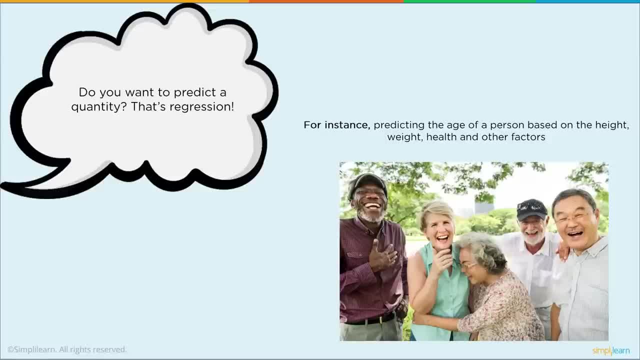 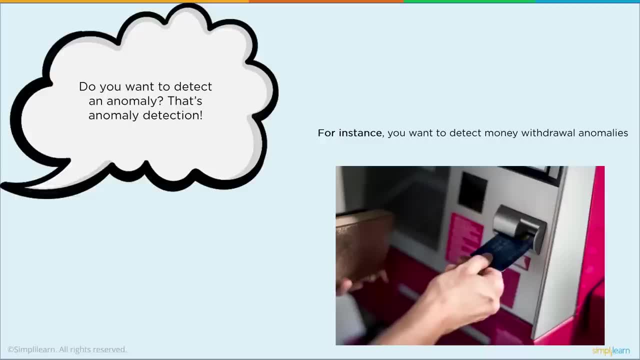 based on the height, weight, health and other factors. So based on these different factors, you might guess how old a person is. And then there are a lot of domain specific things Like: do you want to detect an anomaly? That's anomaly detection. 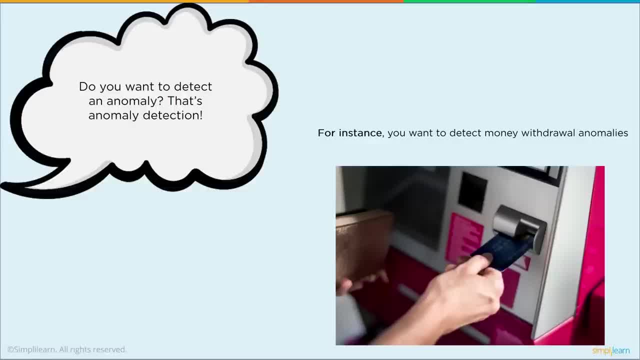 This is actually very popular right now. There are a lot of organizations making a withdrawal that might not be their own account. We've actually brought this up because this is really big right now. If you're predicting the stock, whether to buy stock or not. 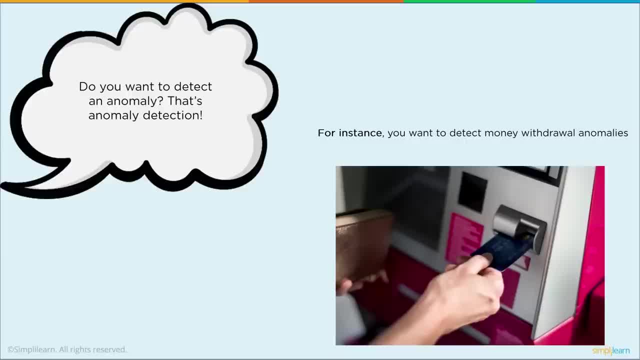 you want to be able to know if what's going on in the stock market is an anomaly. It's a different prediction model. because something else is going on, you've got to pull out new information in there. Or is this just the norm? I'm going to get my normal return. 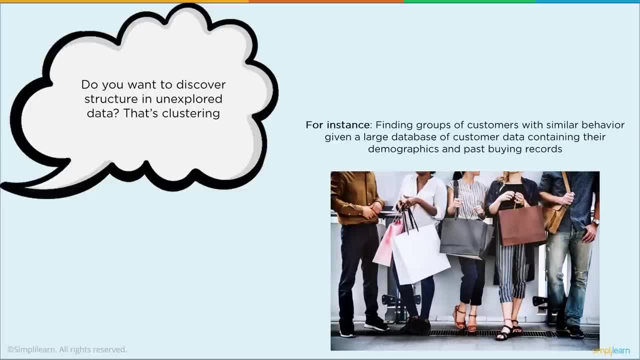 on my money invested. The next question that comes up, which is on what we call untrained data, is: do you want to discover structure in unexplored data, And that's called clustering, For instance, finding groups of customers with similar behavior, given a large database of customer data? 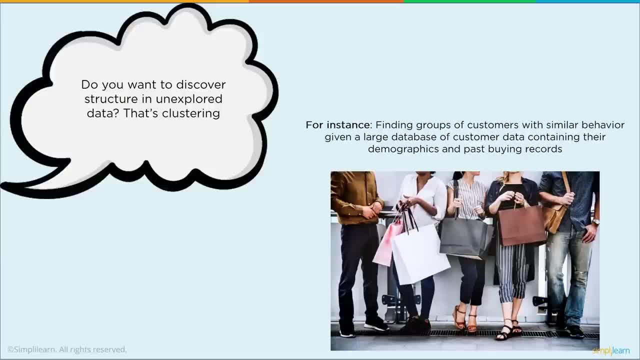 containing their demographics and past buying records, And in this case, we might notice that anybody who's wearing a certain set of shoes goes shopping at certain stores or whatever it is They're going to make certain purchases, And that helps us to market or group people together. 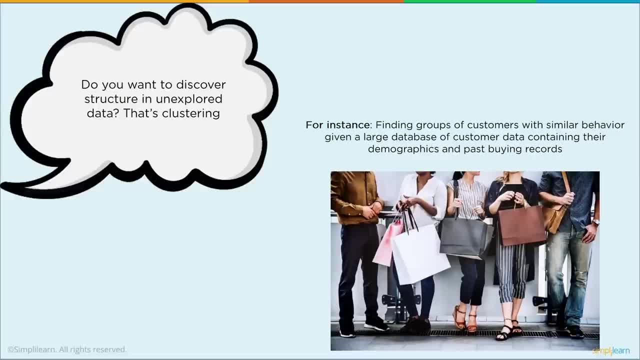 so that we can now explore that group and find out what it is we want to market to them. if you're in the marketing world- And that might also work in just about any arena- You might want to group people together, whether they're based on their different areas. 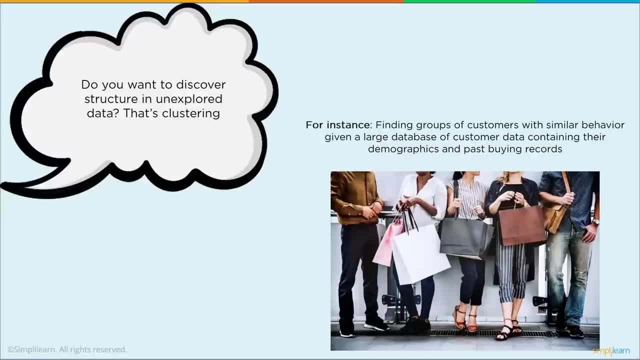 and investments and financial background, whether you're going to give them a loan or not. before you even start looking at whether they're a valid customer for the bank, You might want to look at all these different areas and group them together, based on unknown data. 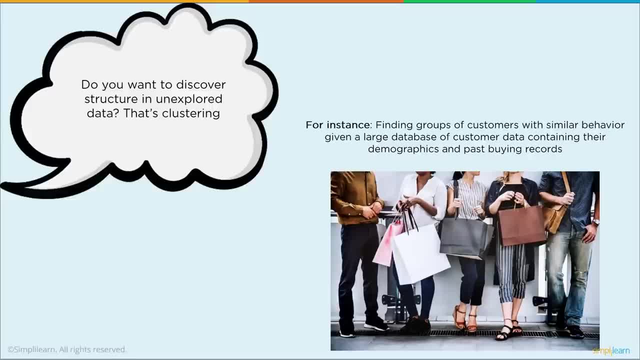 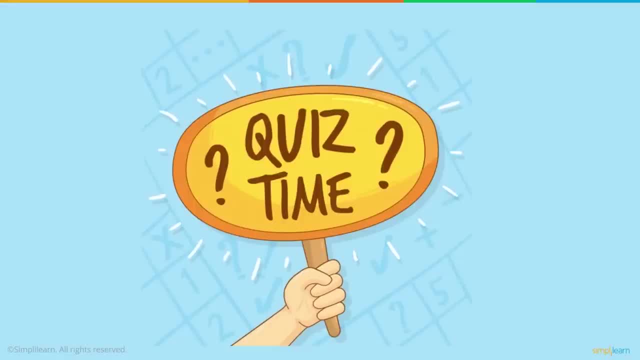 You don't know what the data's going to tell you, but you want to cluster people together. that come together. Let's take a quick detour for quiz time. Oh, my favorite. So we're going to have a couple questions here under quiz time. 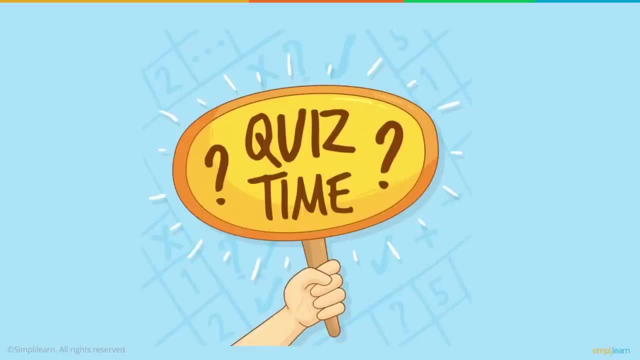 and we'll be posting the answers in the part two of this tutorial. So let's go ahead and take a look at these quiz time questions and hopefully you'll get them all right and it'll get you thinking about how to process data and what's going on. 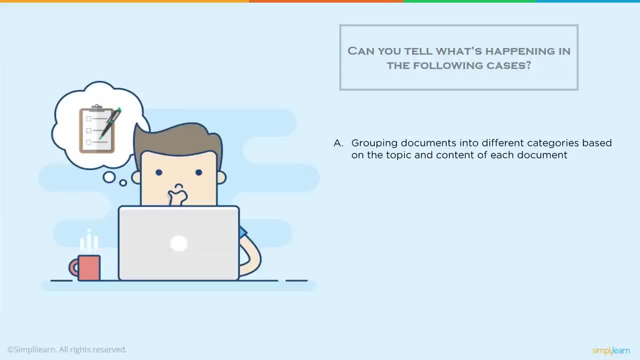 Can you tell what's happening in the following cases? Of course, you're sitting there with your cup of coffee and you have your checkbox and your pen trying to figure out what's your next step in your data science analysis. So the first one is grouping documents. 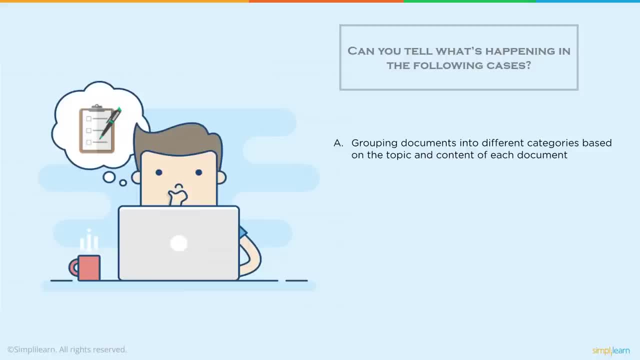 into different categories based on the topic and content of each document- Very big these days. You know you have legal documents, you have. maybe it's a sports group document, maybe you're analyzing newspaper postings, But certainly having that automated is a huge thing in today's world. 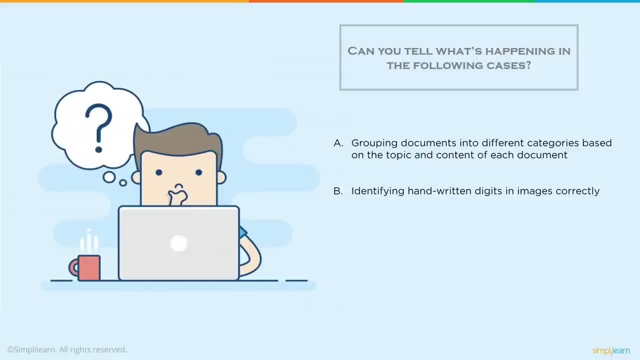 B- Identifying handouts or handwritten digits in images correctly. So we want to know whether they're writing in A or capital, A, B, C. What are they writing out in their handwriting? C- Behavior of a website indicating that the site 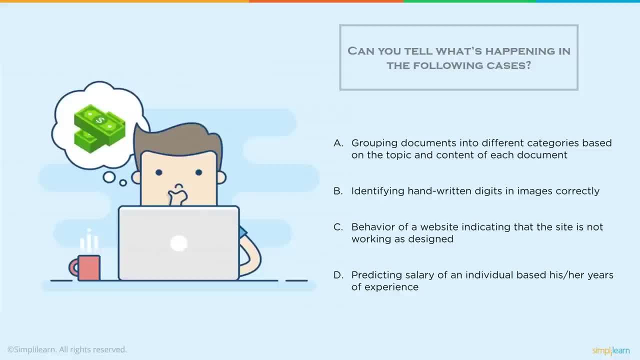 is not working as designed. D Predicting salary of an individual based on his or her years of experience, HR hiring set up there. So stay tuned for part two. We'll go ahead and answer these questions when we get to the part two of this tutorial. 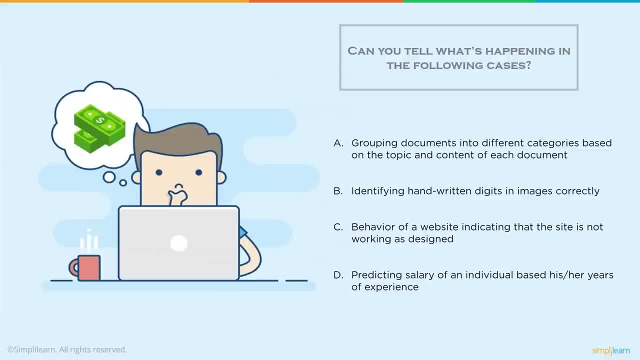 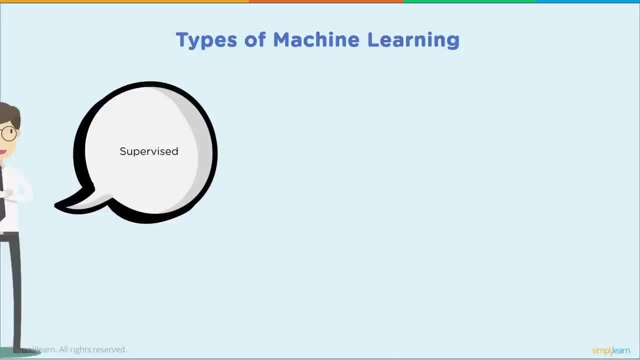 Or you can just simply write at the bottom and send a note to Simply Learn, and they'll follow up with you on it. Back to our regular content Now. these last few bring us into the next topic, which is another way of dividing our types of machine learning. 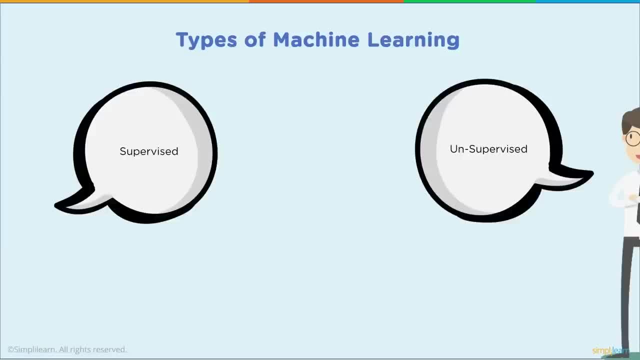 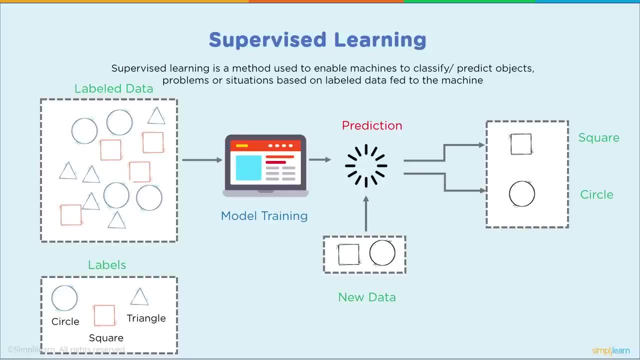 And that is with supervised, unsupervised and reinforcement learning. Supervised learning is a method used to enable machines to classify, predict objects, problems or situations based on labeled data fed to the machine. And in here you see, we have a jumble of data with circles, triangles. 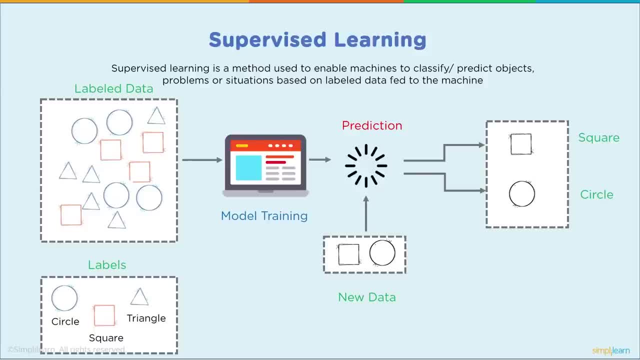 and squares and then we label them. We have what's a circle, what's a triangle, what's a square, and we have our model training and it trains it, so we know the answer. Very important when you're doing supervised learning. 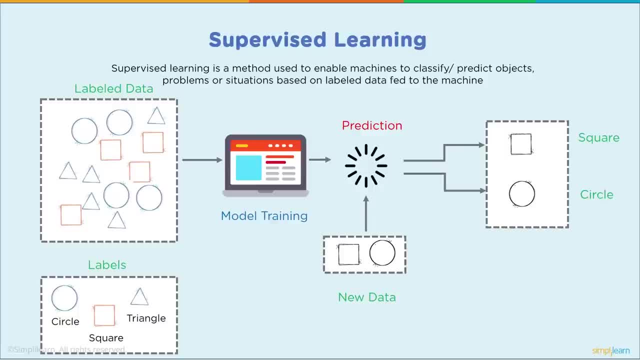 you already know the answer to a lot of your information coming in. So you have a huge group of data coming in and then you have new data coming in. So we've trained our model. the model now knows the difference between a circle, a square, a triangle. 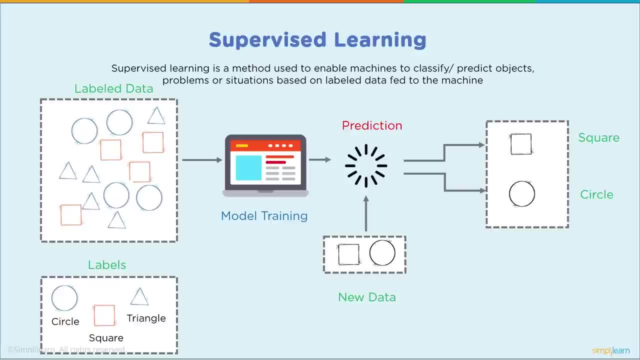 and now that we've trained it, in this case a square and a circle goes in and it predicts that the top one's a square and the next one's a circle, And you can see that this is being able to predict whether someone's going to default on a loan. 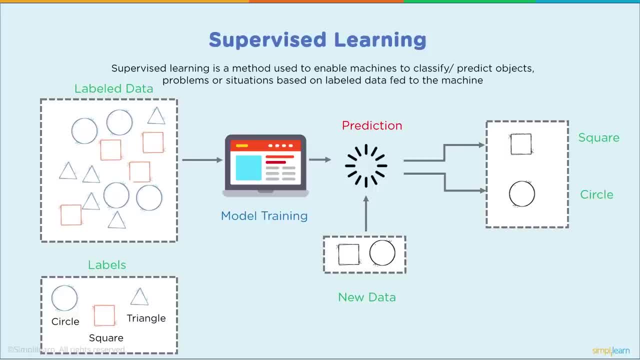 because I was talking about banks earlier- Supervised learning on stock market. whether you're going to make money or not, that's always important And if you are looking to make a fortune on the stock market, keep in mind it is very difficult to get all the data. 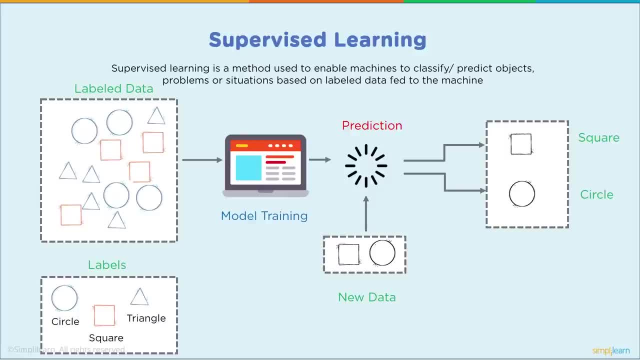 correct on the stock market. It fluctuates in ways really hard to predict, So it's quite a lot of work on a roller coaster ride. if you're running machine learning on the stock market, You start realizing you really have to dig for new data. 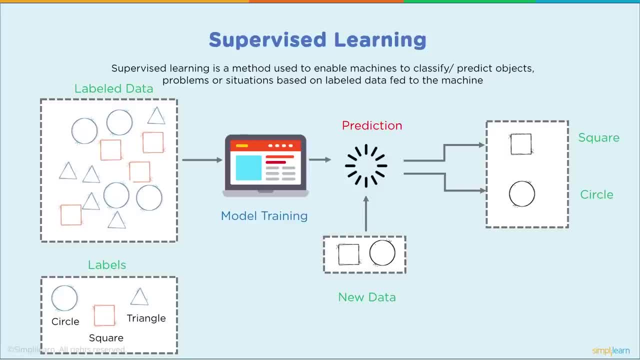 So we have supervised learning, and if you have supervised, we should need unsupervised learning. In unsupervised learning, machine learning model finds the hidden pattern in an unlabeled data. So in this case, instead of telling it what the circle is and what a triangle is, 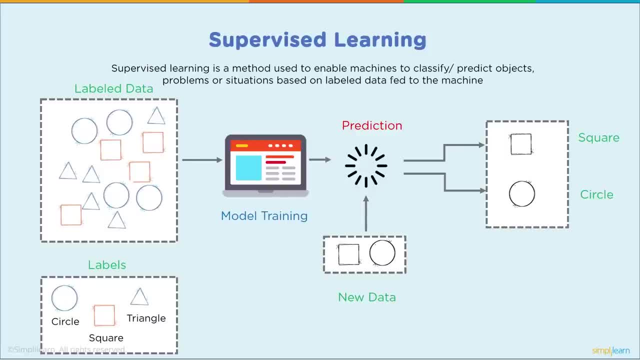 and what a square is. it goes in there and looks at them and says, for whatever reason it groups them together. Maybe it'll group it by the number of corners. It's that a number of them all have three corners. a number of them all have four corners. 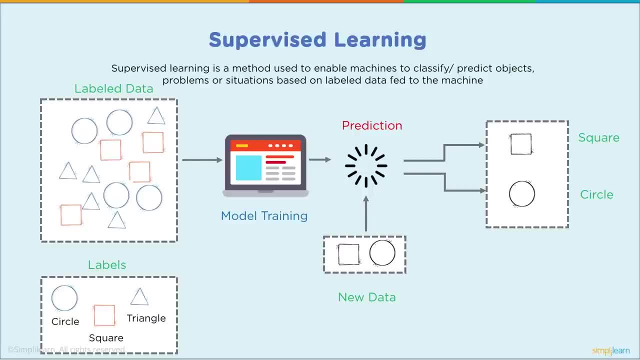 and a number of them all have no corners And it's able to filter those through and group them together. We talked about that earlier, with looking at a group of people who are out shopping. We want to group them together to find out what they have in common. 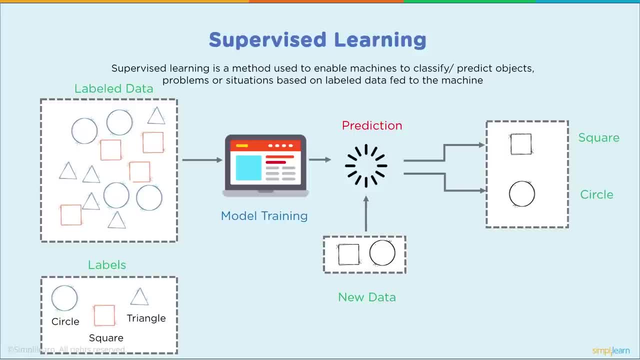 And, of course, once you understand what people have in common, maybe you have one of them who's a customer at your store, or you have five of them who are a customer at your store and they have a lot in common with five others who are not customers at your store. 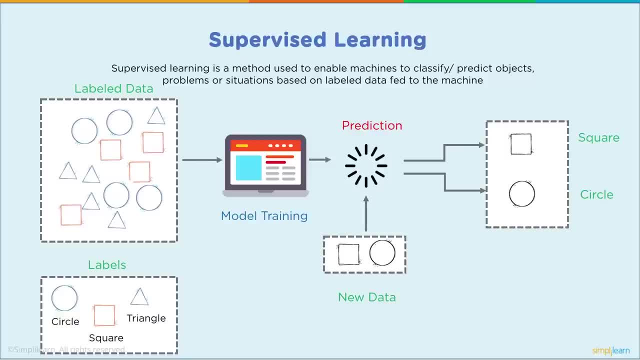 They aren't customers at your store, yet They fit the demographics of who's going to shop there, and you'd like them to shop at your store and not the one next door. Of course, this is a simplified version. You can see very easily the difference between: 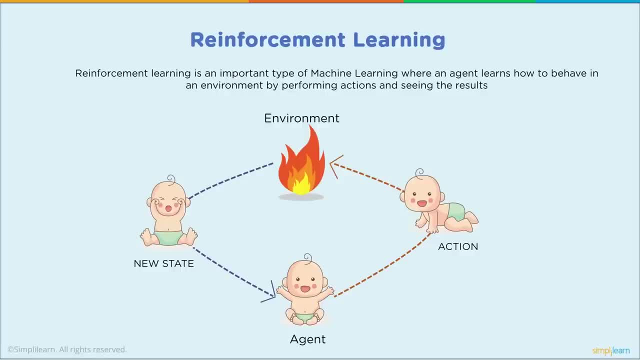 a triangle and a circle, which might not be so easy in marketing Reinforcement learning. Reinforcement learning is an important type of machine learning where an agent learns how to behave in an environment by performing actions and seeing the result. We have here, in this case, a baby. 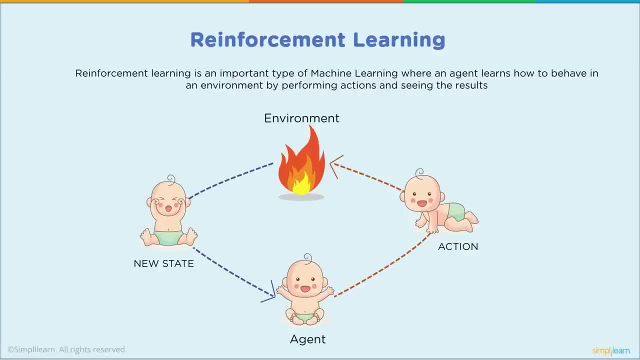 It's actually great that they used an infant for this slide because the reinforcement learning is very much in its infant stages. But it's also probably the biggest machine learning demand out there right now. or in the future It's going to be coming up over the next few years. 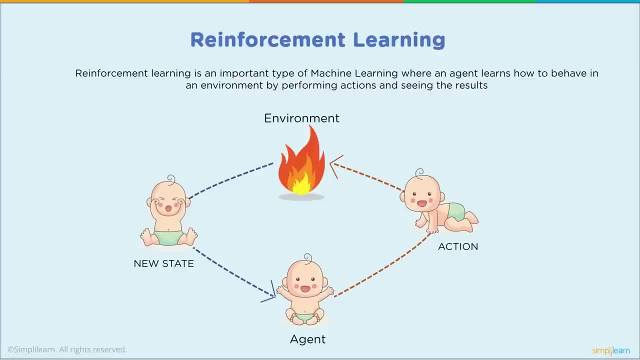 is reinforcement learning and how to make that work for us, And you can see here where we have our action In the action. in this one it goes into the fire. Hopefully the baby didn't. It was just a little candle, not a giant fire pit. 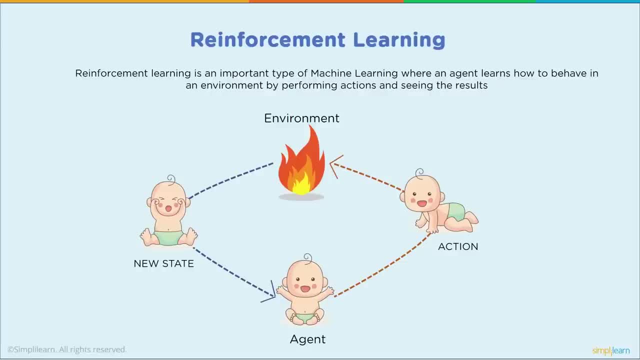 like it looks like here. When the baby comes out and the new state is, the baby is sad and crying because he got burned on the fire, And then maybe they take another action and the baby is called the agent because it's the one taking the actions. 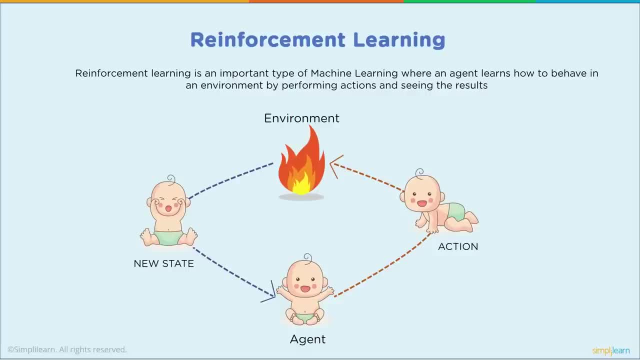 And in this case, they didn't go into the fire. They went a different direction and now the baby is happy and laughing and playing. Reinforcement learning is very easy to understand because that's how, as humans, that's one of the ways we learn. 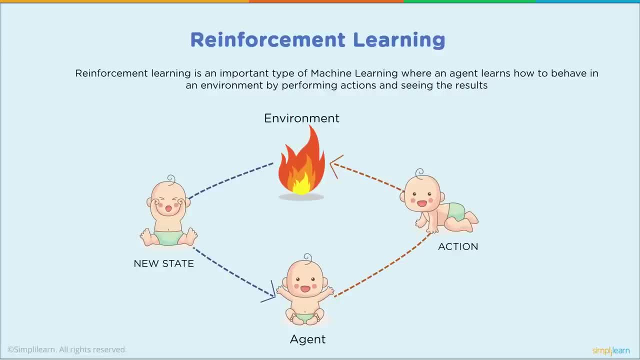 We learn. whether it is you know, you burn yourself on the stove. don't do that anymore. Don't touch the stove. In the big picture, being able to have a machine learning program or an AI be able to do this, is huge. 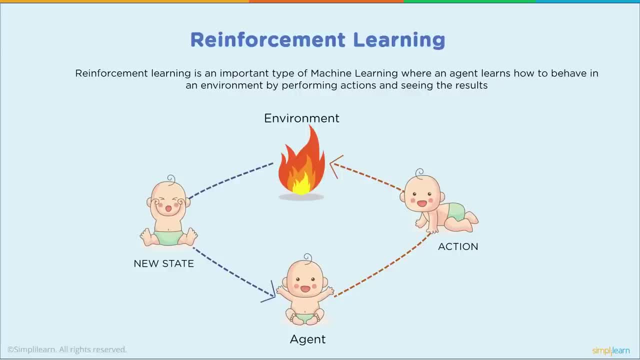 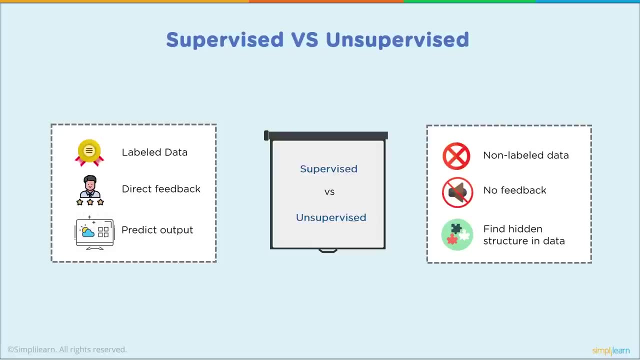 because now we're starting to learn how to learn, We're starting to jump in the world of computer and machine learning And we're going to go back and just kind of go back over supervised versus unsupervised learning. Understanding this is huge because this is going to come up in any project. 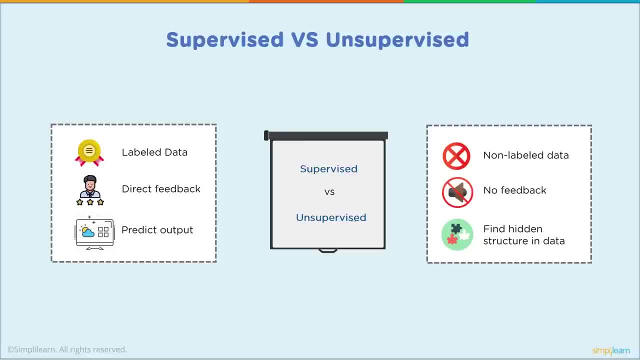 you're working on. We have in supervised learning, we have labeled data, We have direct feedback. So someone's already gone in there and said, yes, that's a triangle, No, that's not a triangle. And then you predict an outcome. 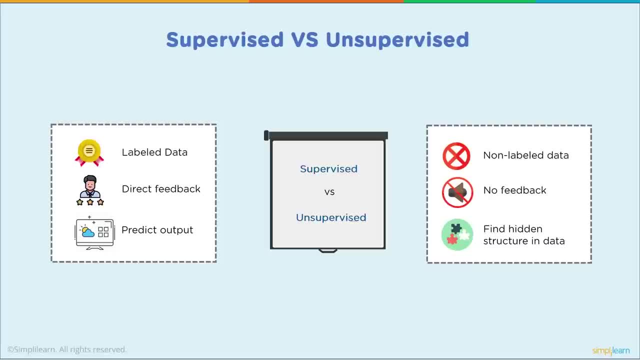 So you have a nice prediction. This new set of data is coming in from unsupervised training. It's not labeled, So we really don't know what it is. There's no feedback, So we're not telling it whether it's right or wrong. 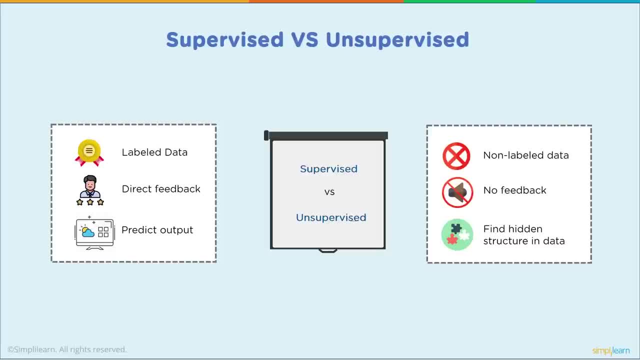 We're not telling it whether it's a triangle or a square. We're not telling it to go left or right. All we do is we're finding hidden structure in the data, Grouping the data together to find out what connects to each other. 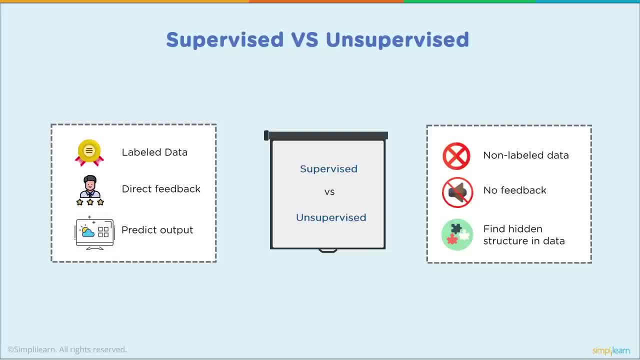 And then you can use these together. So imagine you have an image and you're not sure what you're looking for. So you go in and you have the unstructured data, Find all these things that are connected together, And then somebody looks at those. 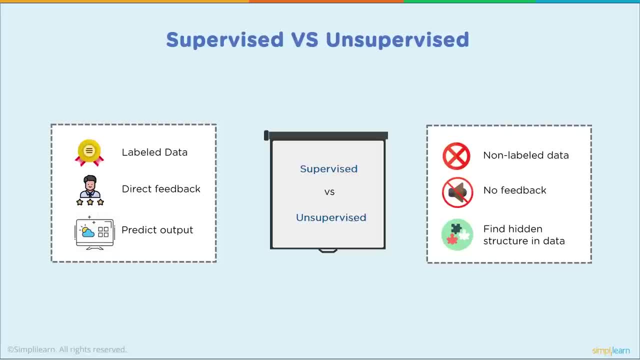 and labels them. Now you can take that labeled data and program something to predict what's in the picture, So you can see how they go back and forth and you can start connecting all these different tools together to make a bigger picture. There are many interesting machine learning algorithms. 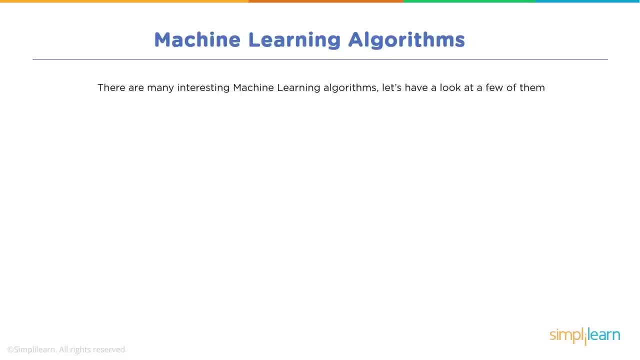 Let's have a look at a few of them. Hopefully, this will give you a little flavor of what's out there, And these are some of the most important ones that are currently being used. So let's take a look at this tree and the support vector machine. 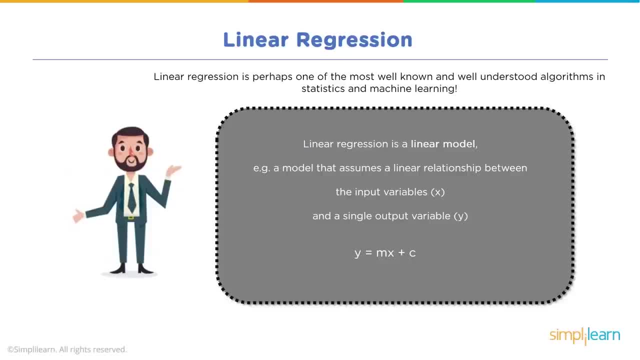 Let's start with a closer look at linear regression. Linear regression is perhaps one of the most well known and well understood algorithms in statistics and machine learning. Linear regression is a linear model, For example, a model that assumes a linear relationship between the input variables x. 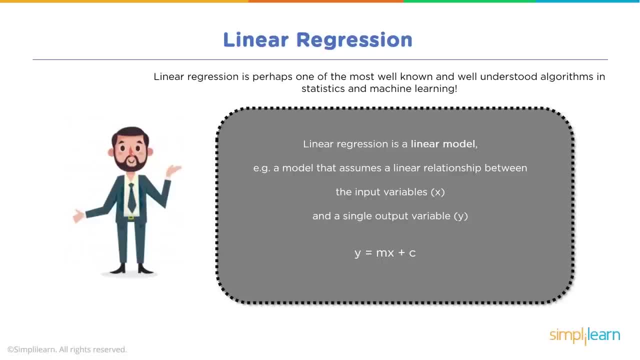 and the single output variable y, And you'll see this if you remember from your algebra classes: y equals mx plus c. Imagine we are predicting distance traveled at speed x. Our linear regression model representation for this problem would be: y equals m times x plus c. 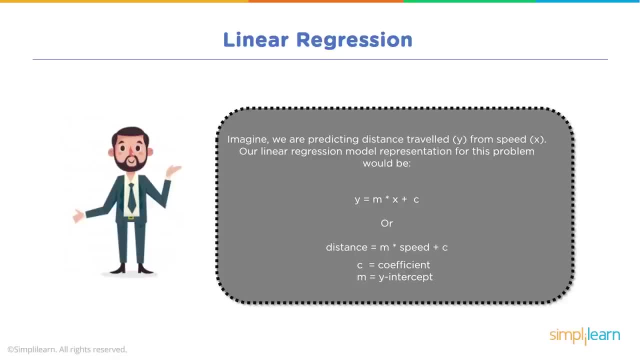 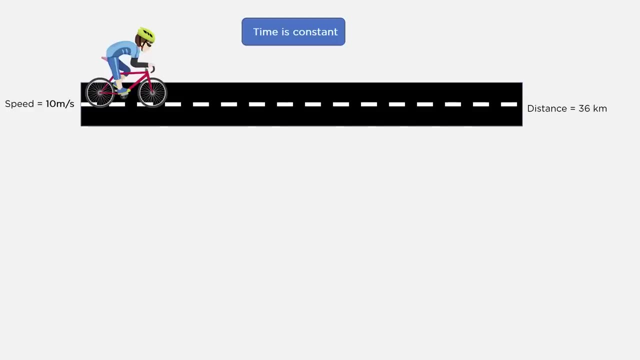 or distance, equals m times speed plus c, Where m is the coefficient and c is the y-intercept. And we're going to look at two different variations of this. First, we're going to start with time as constant And you can see we have a bicyclist. 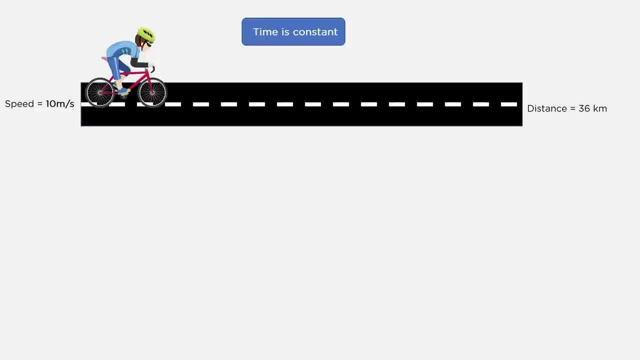 He's got his safety gear on, thank goodness, Speed equals 10 meters per second, And so, over a certain amount of time, his distance equals 36 kilometers per second. So we're going to start with 30 meters per second. We have a second bicyclist. 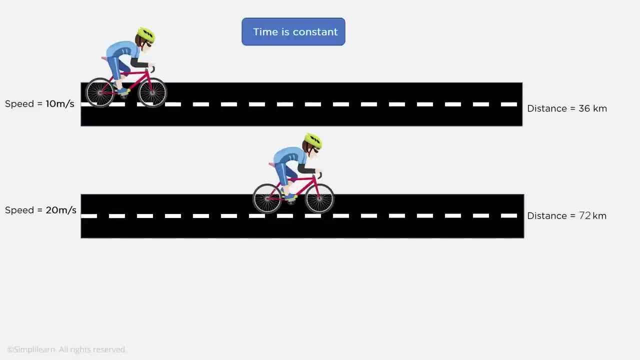 who's going twice the speed, or 20 meters per second. And you can guess: if he's going twice the speed and time is a constant, then he's going to go twice the distance And that's easily to compute: 36 times 2,, you get 72 kilometers. 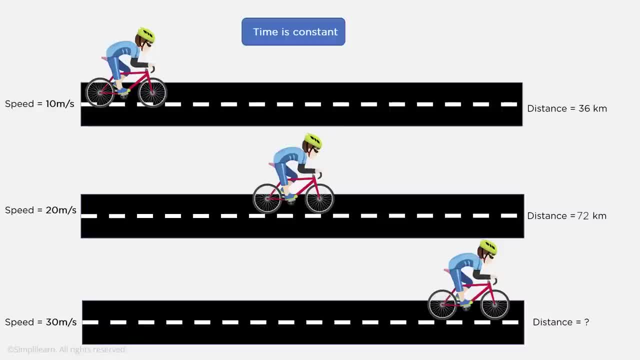 And so if you had the question of how fast would somebody who's going three times that speed, or 30 meters per second, is, you can easily compute the distance In our head. we can do that without needing a computer, But we want to do this for more complicated data. 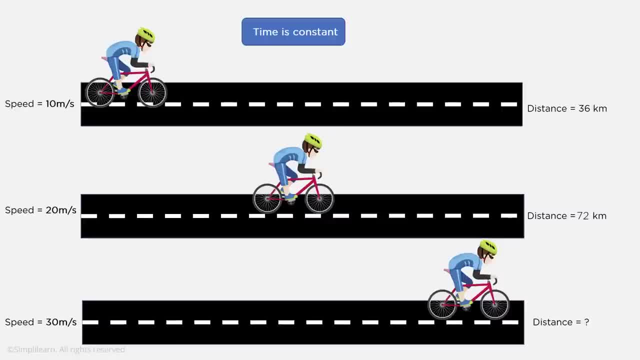 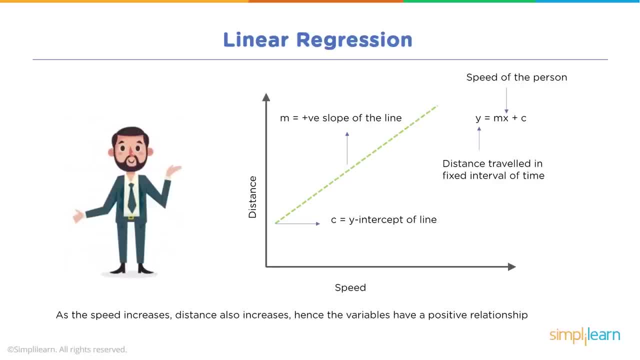 So it's kind of nice to compare the two, But let's just take a look at that and what that looks like in a graph. So in a linear regression model we have our distance to the speed And we have our m equals the ve slope of the line. 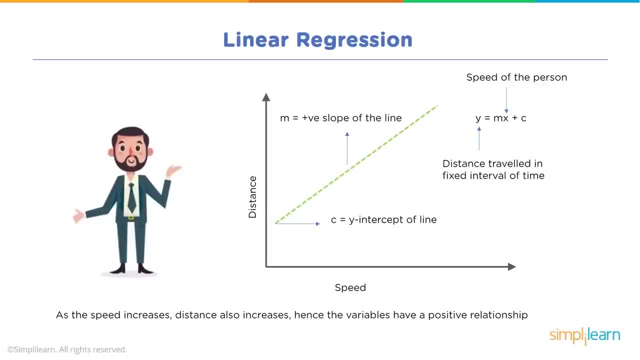 And we'll notice that the line has a plus slope, And as the speed increases, distance also increases. Hence the variables have a positive relationship. And so your speed of the person, which equals y, equals mx plus c: distance traveled in a fixed interval of time. 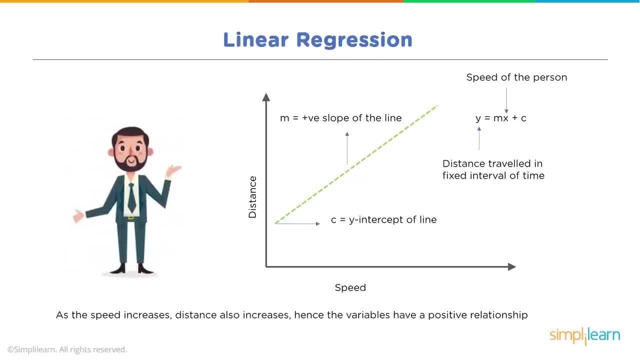 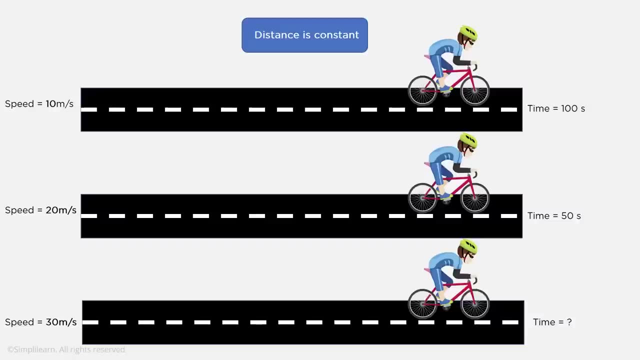 And we could very easily compute either following the line or just knowing it's 3 times 10 meters per second, that this is roughly 102 kilometers distance that this third bicyclist has traveled. One of the key definitions on here is positive relationship. 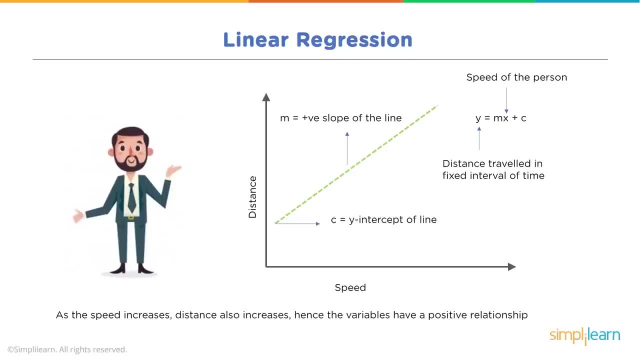 So the slope of the line is positive. As distance increases, so does speed increase. Let's take a look at our second example, where we put distance as a constant, So we have speed equals 10 meters per second. They have a certain distance to go. 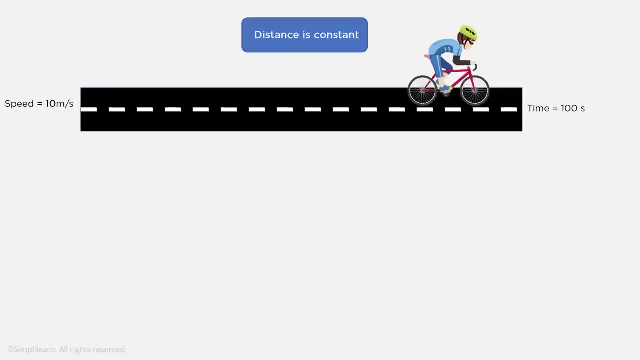 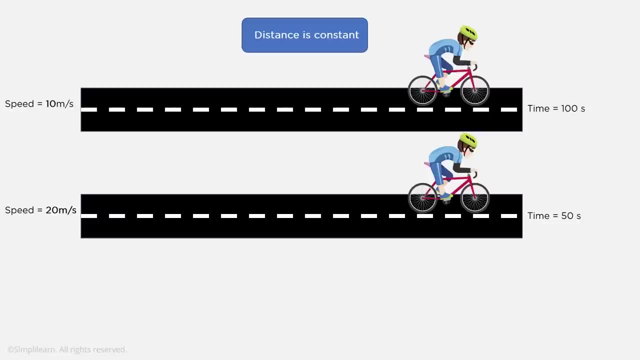 And it takes them 100 seconds to travel that distance. And we have our second example where we have a second bicyclist who's still doing 20 meters per second. Since he's going twice the speed, we can guess that he'll cover the distance. 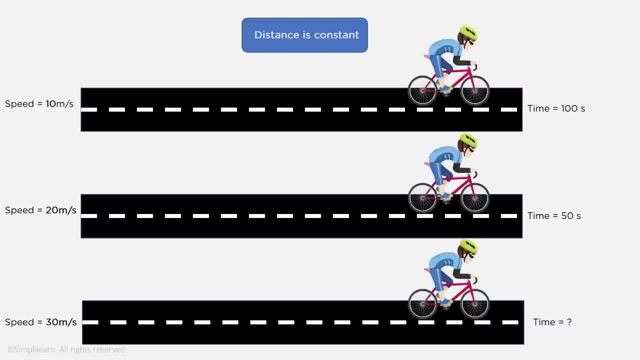 in about half the time, 50 seconds. And of course you could probably guess on the third one: 100 divided by 30, since he's going 3 times the speed, you could easily guess that this is 33.333 seconds time. 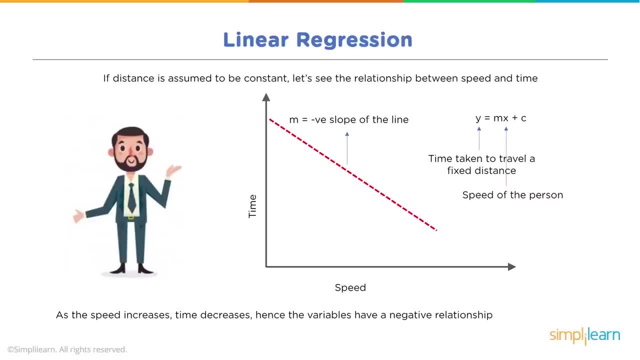 We put that into a linear regression model or a graph. If the distance is assumed to be constant, let's see the relationship between speed and time. And as time goes up the distance goes down. So now your m equals a minus v-e slope of the line. 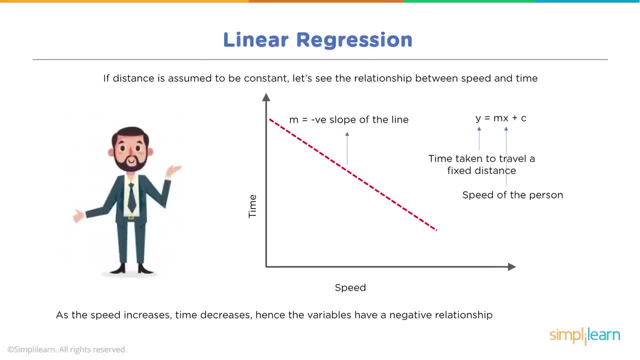 As the speed increases, time decreases, Hence the variable has a negative relationship. Again, there's our definition: Positive relationship and negative relationship depended on the slope of the line. And with a simple formula like this and even a significant amount of data, 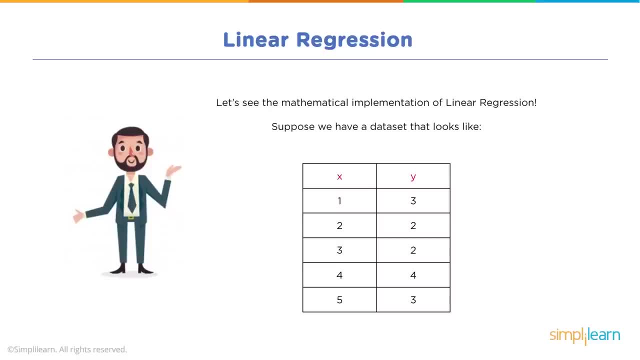 let's see what the mathematical implementation of linear regression And we'll take this data. So suppose we have this data set where we have xy, x equals 1,, 2,, 3,, 4, 5, standard series and the y value is 3,, 2,, 2,, 4, 3.. 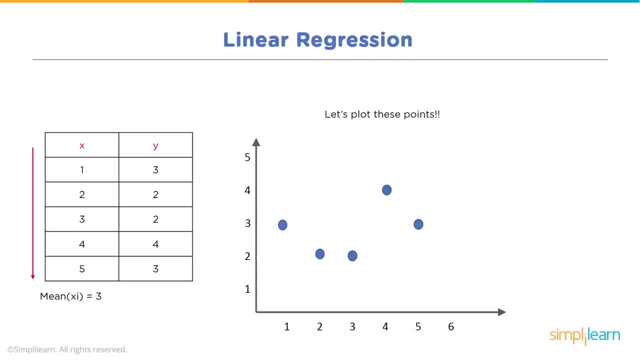 When we take that and we go ahead and plot these points on a graph, you can see there's kind of a nice scattering and you could probably eyeball a line through the middle of it. But we're going to calculate that exact line for linear regression. 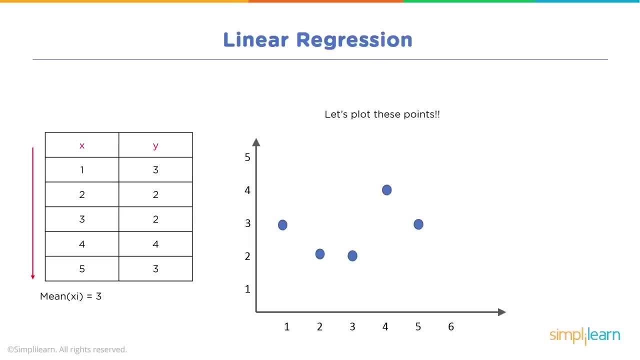 And the first thing we do is we come up here and we have the mean of xy, And remember, mean is basically the average. So we added 5 plus 4 plus 3 plus 2 plus 1 divided by 5. And that simply comes out as 3.. 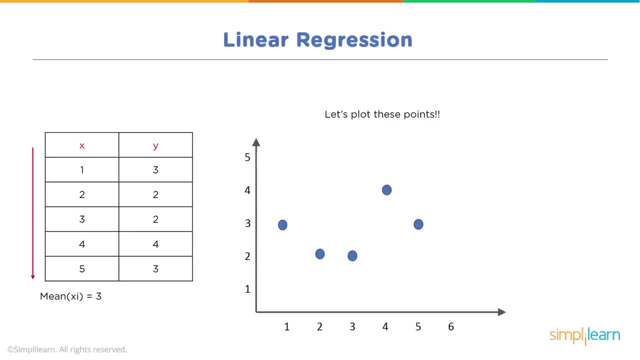 And then we'll do the same for y. We'll go ahead and add up all those numbers and divide by 5.. And we end up with the mean value of y of i equals 2.8.. Where the xy references, it's an average. 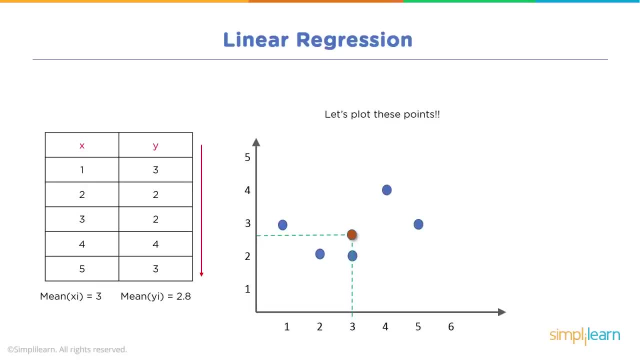 or means value, and the yi also equals a means value of y And when we plot that you'll see that we can put in the y equals 2.8 and the x equals 3. in there on our graph We kind of gave it a little different color. 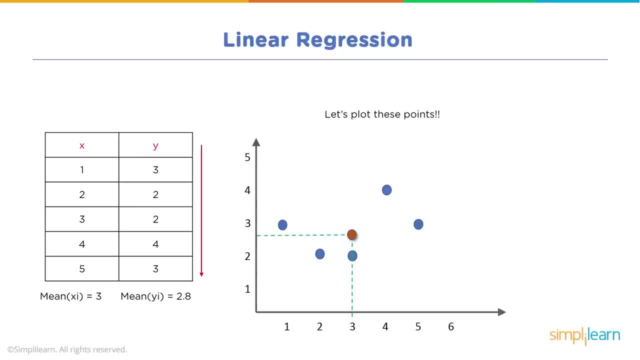 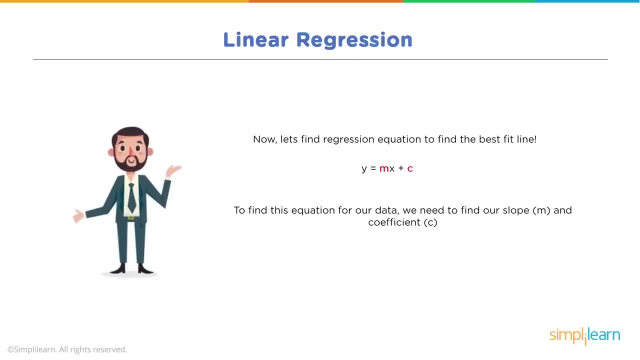 so you could sort it out with the dashed lines on it. And it's important to note that when we do the linear regression, the linear regression model should go through that dot. Now let's find our regression equation to find the best fit line. 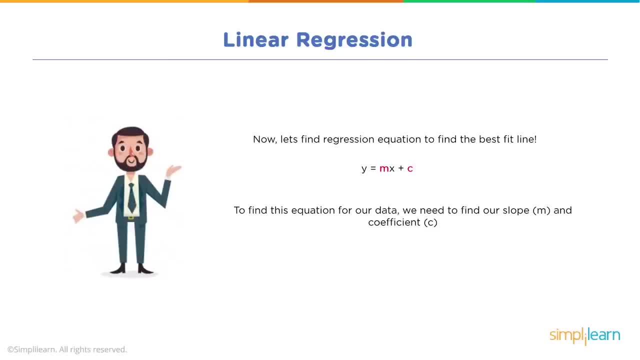 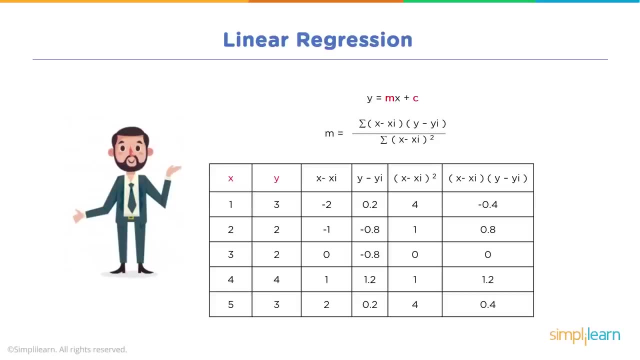 Remember, we go ahead and take our y equals mx plus c, So we're looking for m and c. So to find this equation for our data, we need to find our slope of m and our coefficient of c And we have y equals mx plus c. 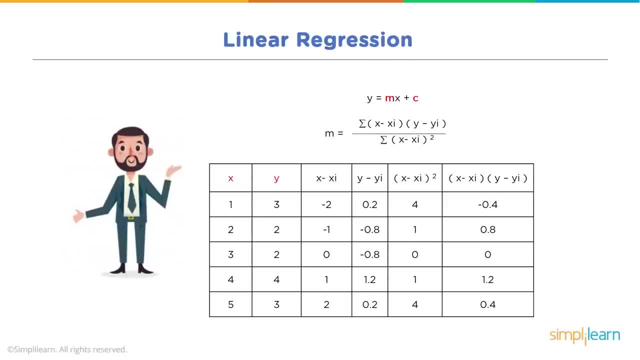 Where m equals the sum of x minus x average times y minus y. So that's the y average, or y means and x means over. the sum of x minus x means squared. That's how we get the slope of the value of the line. 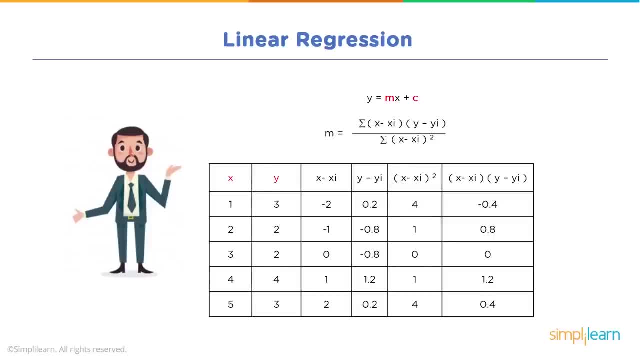 And we can easily do that by creating some columns. here We have x, y. Computers are really good about iterating through data, And so we can easily compute this and fill in a graph of data, And in our graph you can easily see: 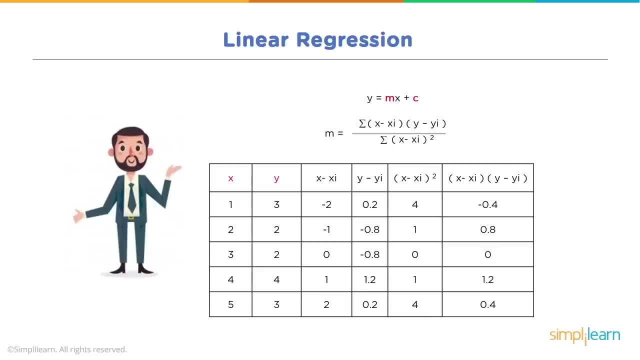 that if we have our x value of 1, and if you remember, the xi or the means value is 3, 1 minus 3 equals a negative 2. And 2 minus 3 equals a negative 1.. So on and so forth. 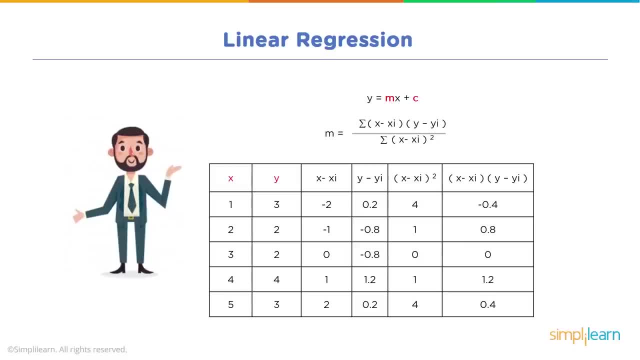 And we can easily fill in the column of x minus xi, y minus yi, and then from those we can compute x minus xi squared and x minus xi times y minus yi, And you can guess it that the next step is to go ahead and sum the different columns. 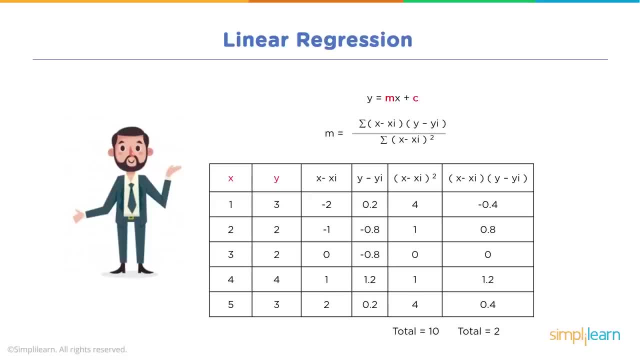 for the answers we need. So we get a total of 10 for our x minus xi squared and a total of 2 for x minus xi times y minus yi. And we plug those in, We get 2 tenths, which equals 0.2.. 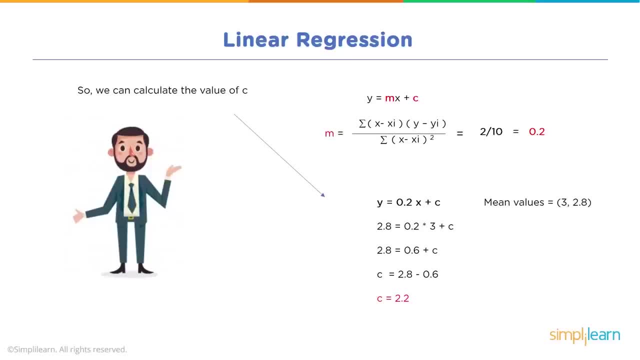 So now we know the slope of our line equals 0.2.. So we can calculate the value of c. That'd be. the next step is we need to know where it crosses the y-axis And if you remember, I mentioned earlier that the linear regression line. 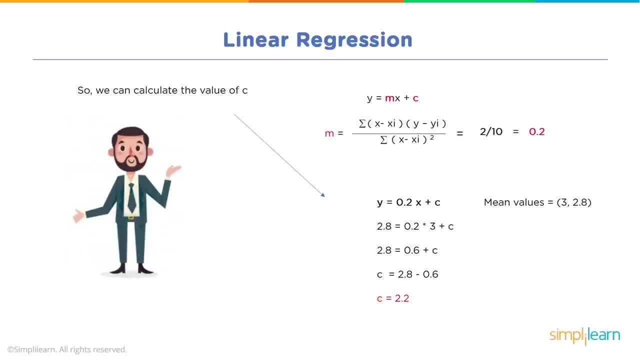 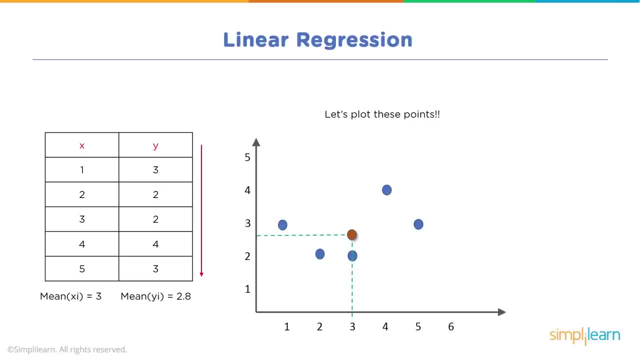 has to pass through the means value, the one that we showed earlier. We can just flip back up there to that graph And you can see right here there's our means value, which is 3, x equals 3, and y equals 2.8.. 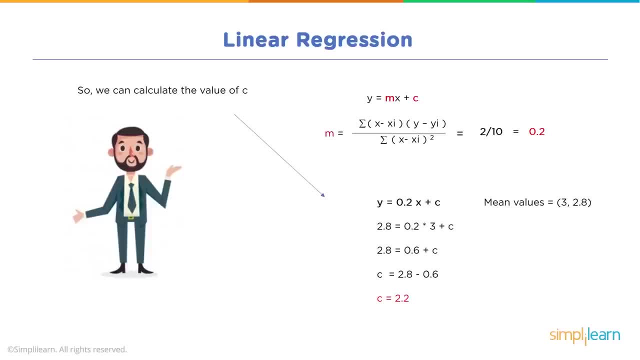 And since we know that value, we can simply plug that into our formula: y equals 0.2 x plus c. So we plug that in and we get 2.8 equals 0.2 times 3 plus c, And you can just solve for c. 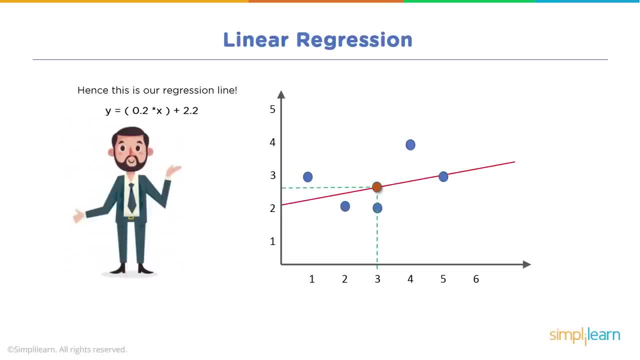 So now we know that our coefficient equals 2.2.. And once we have all that, we can go ahead and plot our regression line: y equals 0.2 times x plus 2.2.. And then from this equation we can compute new values. 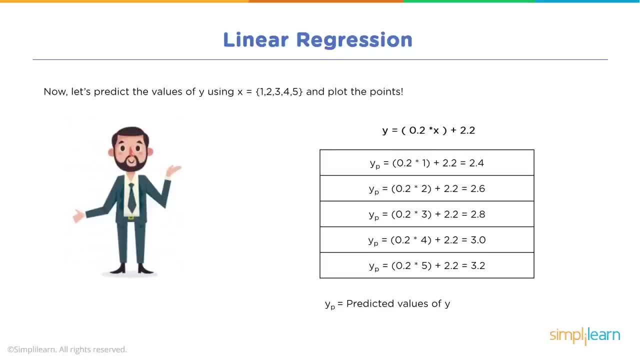 So let's predict the values of y using x equals 1,, 2,, 3,, 4, 5- and plot the points. Remember the 1,, 2,, 3,, 4, 5 was our original x values. 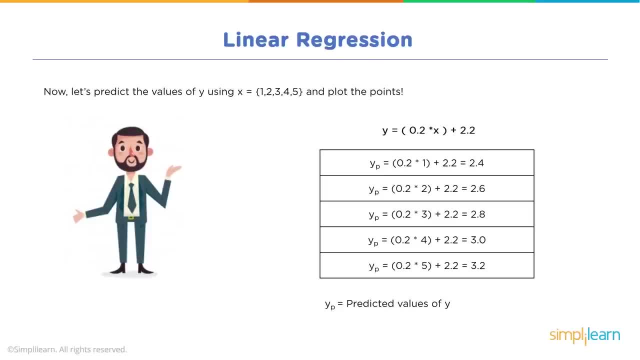 So now we're going to see what y thinks they are, not what they actually are, And when we plug those in we get y designated with y of p. You can see that x equals 1 equals 2.4,. x equals 2 equals 2.6,. 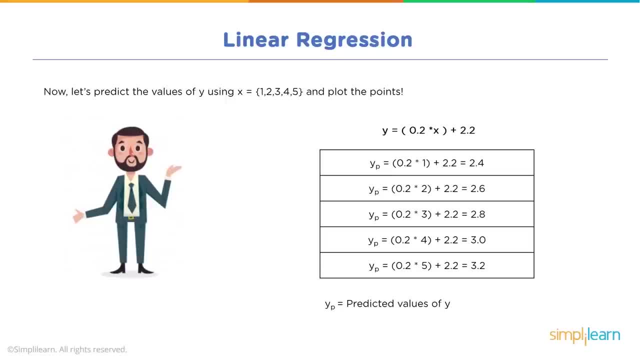 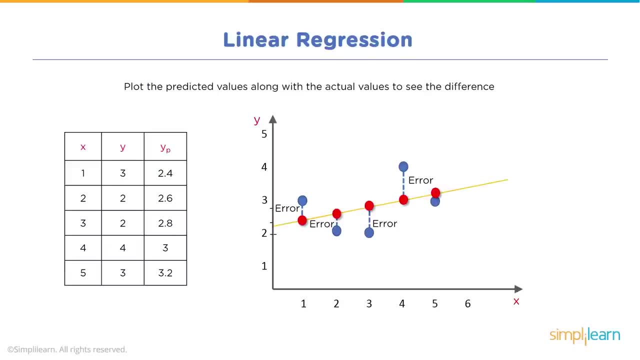 and so on and so on. So we have our y predicted values of what we think it's going to be. when we plug those numbers in And when we plot the predicted values along with the actual values, we can see the difference, And this is one of the things that's very important. 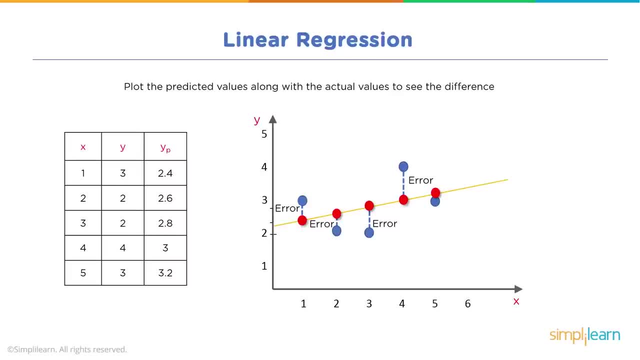 with linear regression in any of these models is to understand the error, And so we can calculate the error on all of our different values. And you can see over here we plotted x and y and y predict And we draw in a little line. 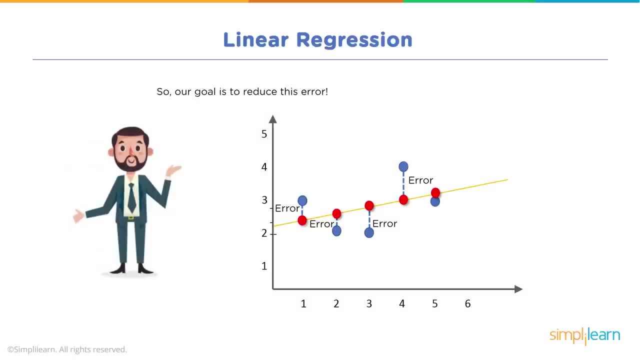 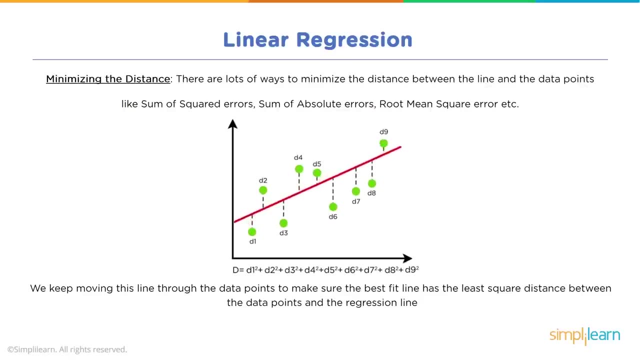 so you can sort of see what the error looks like there between the different points. So our goal is to reduce this error By reducing the distance. there are lots of ways to minimize the distance between the line and the data points like sum of squared errors. 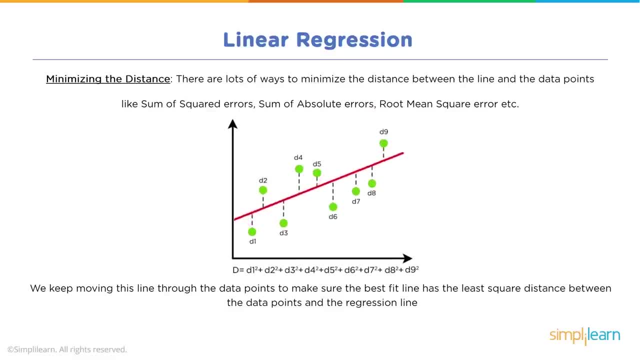 sum of absolute errors, root mean square error, etc. We keep moving this line through the data points to make sure the best fit line has the least squared distance between the data points and the regression line. So to recap with a very simple linear regression model. 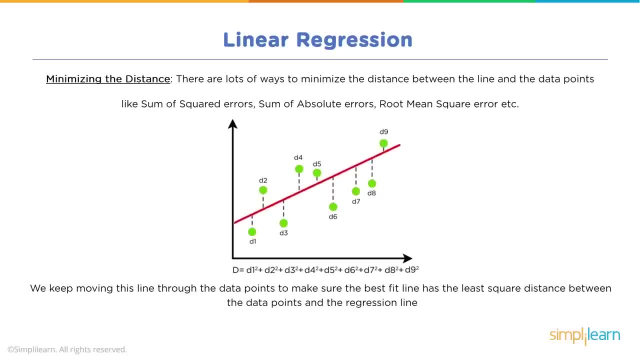 we first figure out the formula of our line through the middle and then we slowly adjust the line to make sure that we get the best result. Keep in mind: this is a very simple formula. The math gets. even though the math is very much the same, it gets much more complex. 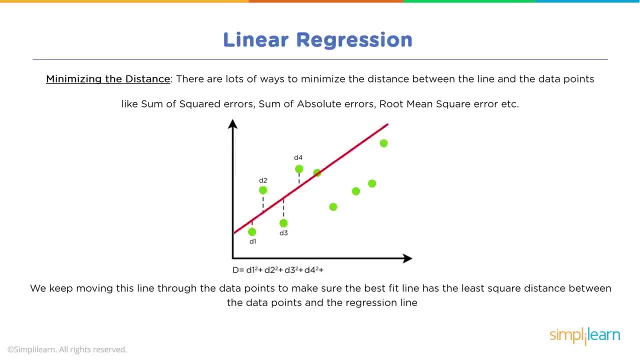 as we add in different dimensions. So this is only two dimensions. y equals mx plus c, but you can take that out to x, z, ijq, all the different features in there, and they can plot a linear regression model on all of those using the different formulas. 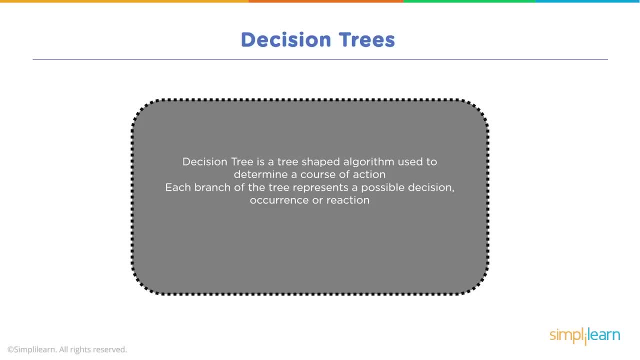 to minimize the error. Let's go ahead and take a look at decision trees, a very different way to solve problems. in the linear regression model, It is a tree-shaped algorithm used to determine a course of action. Each branch of a tree represents a possible decision occurrence or reaction. 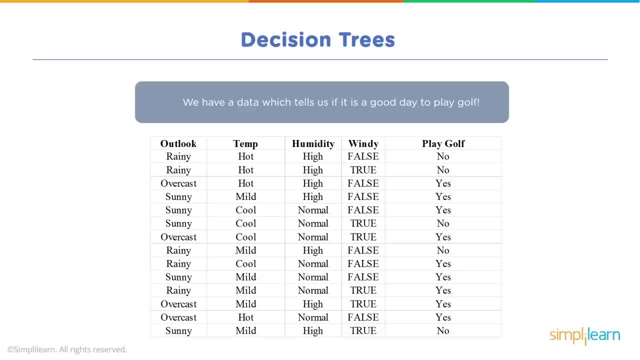 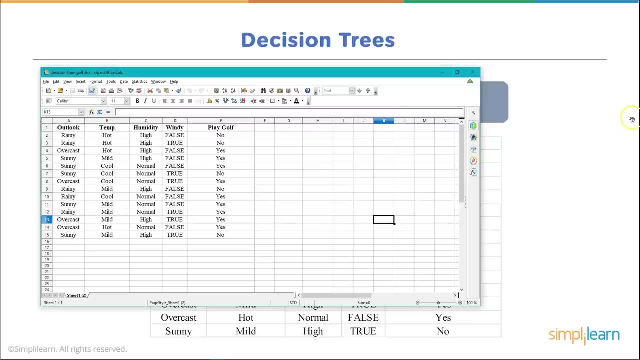 We have data which tells us if it is a good day to play golf, And if we were to open this data up in a general spreadsheet, you can see. we have the outlook, whether it's rainy, overcast, sunny temperature, hot, mild, cool. 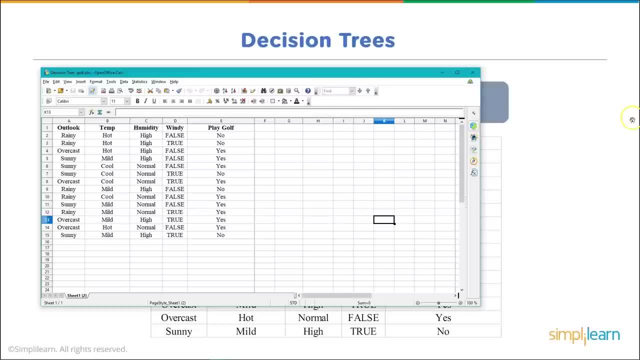 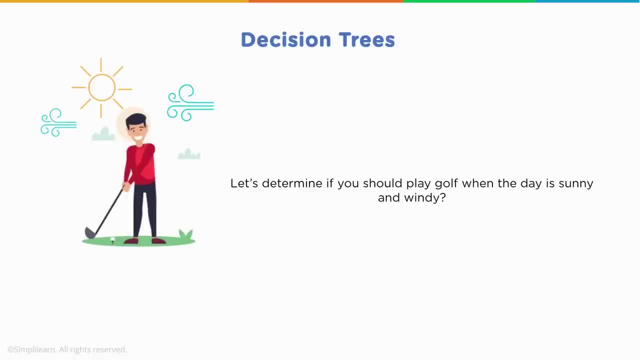 humidity, windy, and did I like to play golf that day, yes or no? So we're taking a census and certainly I wouldn't want a computer telling me when I should go play golf or not. But you can imagine if you got up the night before. 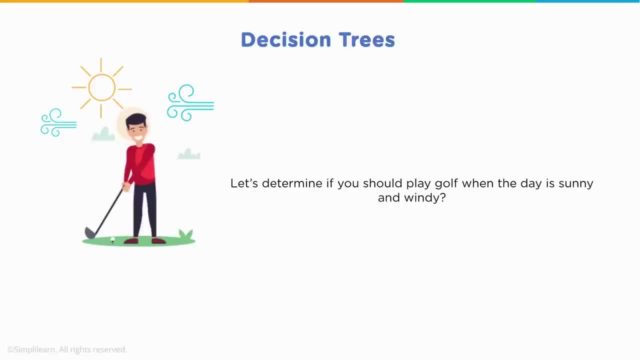 you're trying to plan your day and it comes up and says: tomorrow would be a good day for golf for you in the morning and not a good day in the afternoon, or something like that. This becomes very beneficial and we see this in a lot of applications coming out now. 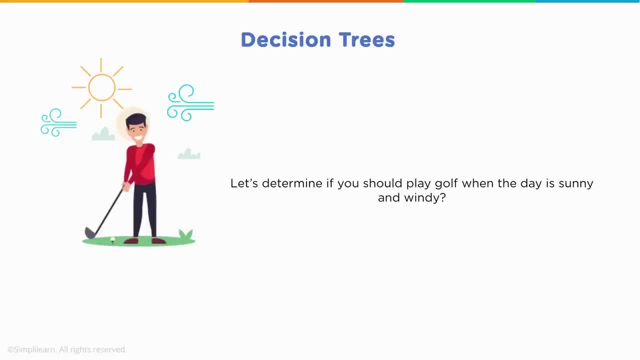 where it gives you suggestions and lets you know what would fit the match for you for the next day, or the next purchase, or the next, whatever next meal out, In this case, is tomorrow a good day to play golf, based on the weather coming in? 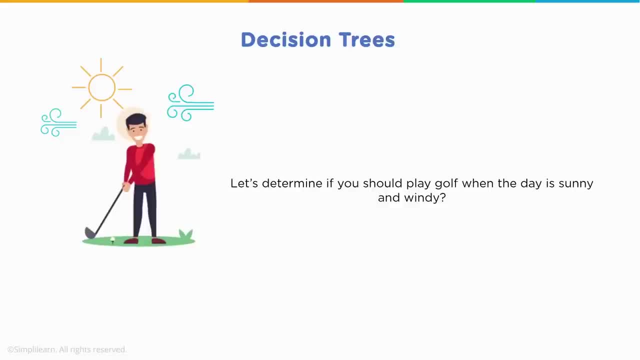 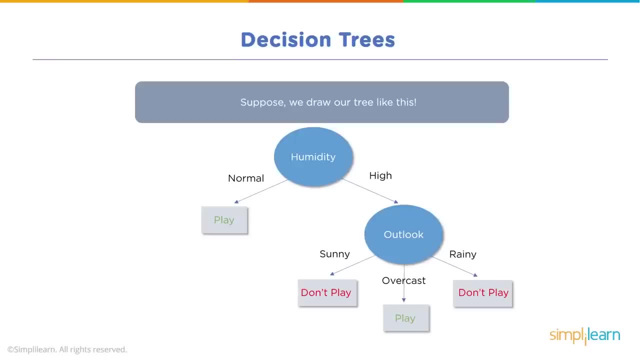 And so we come up and let's determine if you should play golf when the day is sunny and windy. So we found out the forecast tomorrow is going to be sunny and windy, And suppose we draw our tree like this, We're going to have our humidity. 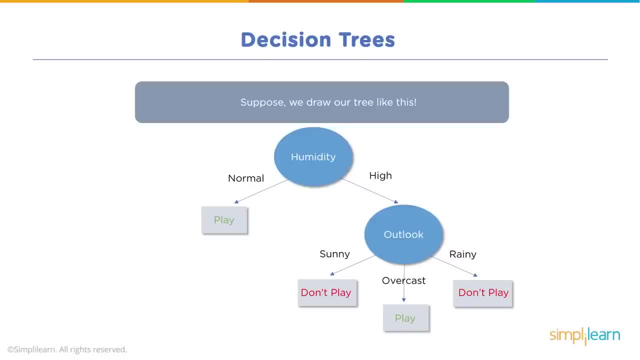 and then we have our normal, which is, if you have a normal humidity, you're going to go play golf, And if the humidity is really high, then we look at the outlook And if the outlook is sunny, overcast or rainy, 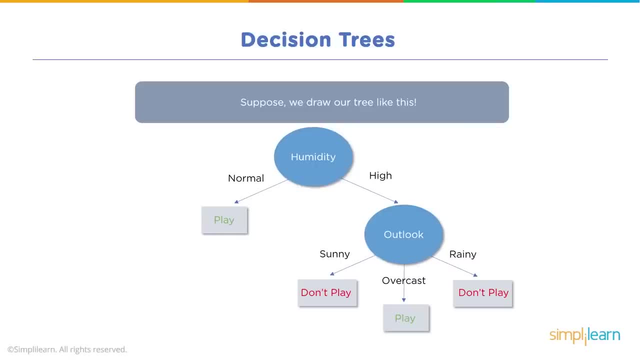 it's going to change what you choose to do. If you know that it's a very high humidity and it's sunny, you're probably not going to play golf because you're going to be out there miserable, fighting off the mosquitoes that are out. 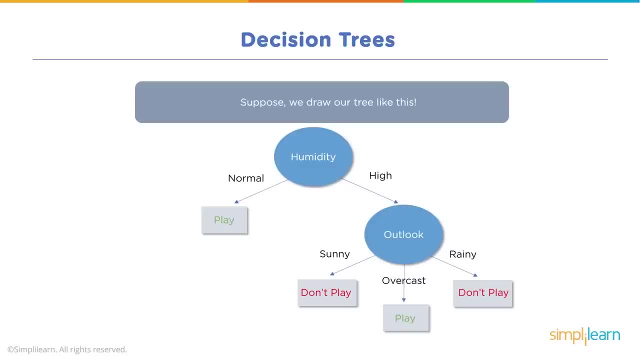 joining you to play golf with you, Maybe if it's rainy. you probably don't want to play in the rain, But if it's slightly overcast and you get just the right shadow, that's a good day to play golf and be outside out on the green. 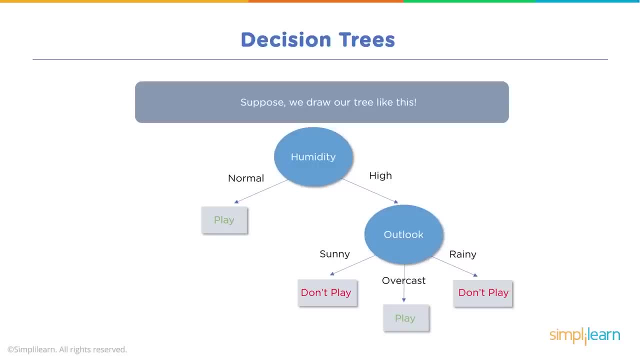 Now in this example, you can probably make your own tree pretty easily because it's a very simple set of data going in. But the question is: how do you know what to split? Where do you split your data? What if this is much more complicated data? 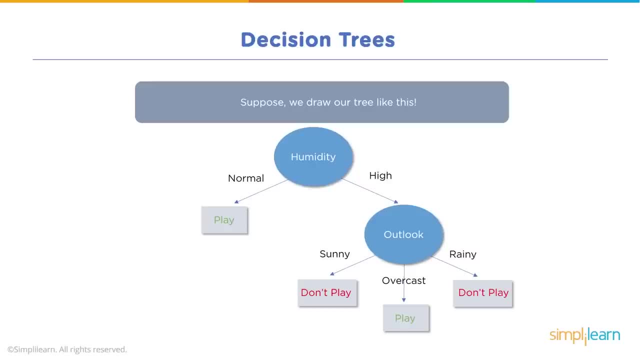 where it's not something that you would particularly understand. Like studying cancer, they take about 36 measurements of the cancerous cells and then each one of those measurements represents how bulbous it is, how extended it is, how sharp the edges are. 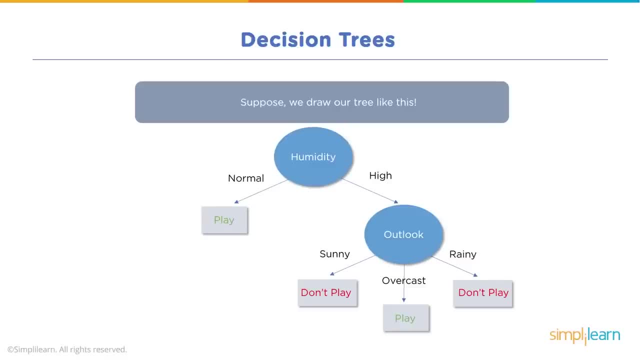 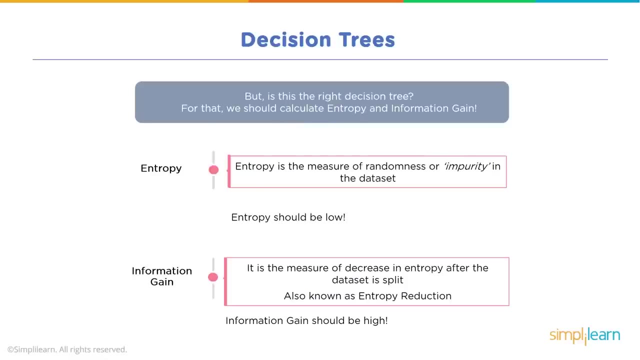 Something that, as a human, we would have no understanding of. So how do we decide how to split that data up, And is that the right decision tree? So that's the question that's going to come up: Is this the right decision tree? 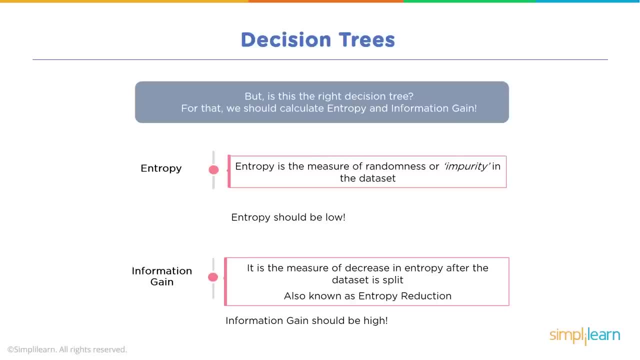 For that we should calculate entropy and information gain. Two important vocabulary words there are the entropy and the information gain. Entropy: Entropy is a measure of randomness or impurity in the data set. Entropy should be low, So we want the chaos to be as low as possible. 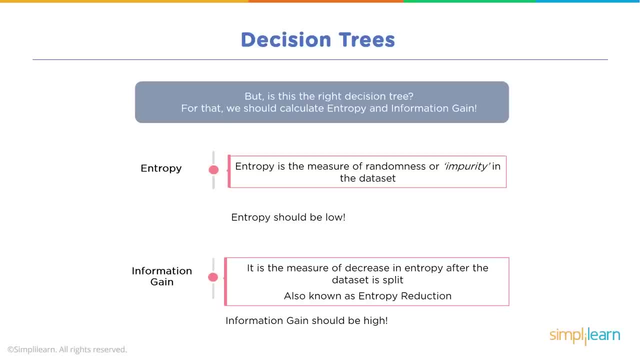 We don't want to look at it and be confused by the images or what's going on there. with mixed data And the information gain, it is a measure of decrease in entropy after the data set is split, also known as entropy reduction. Information gain should be high. 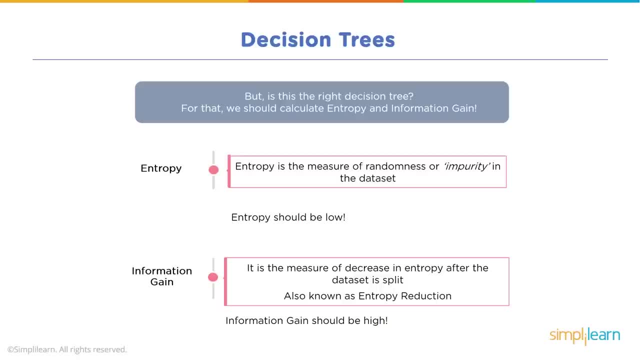 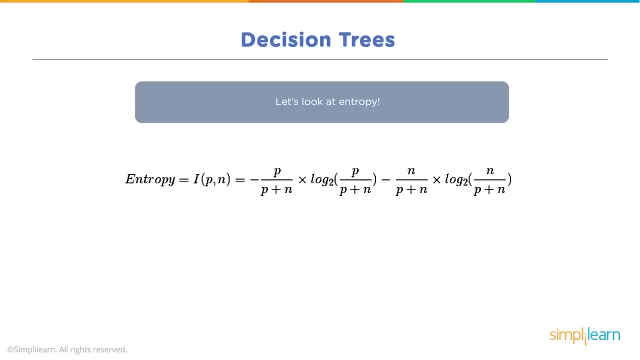 So we want our information that we get out of the split to be as high as possible. Let's take a look at entropy from the mathematical side. In this case, we're going to denote entropy as I of P and N, where P is the probability. 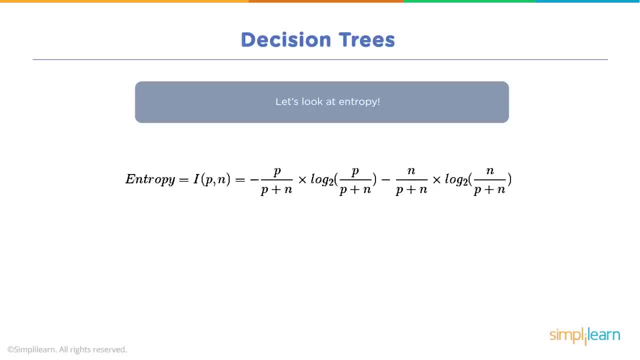 that you're going to play a game of golf and N is the probability where you're not going to play the game of golf. There's a few of them out there, depending on what you're working with, But it's important to note that this is. 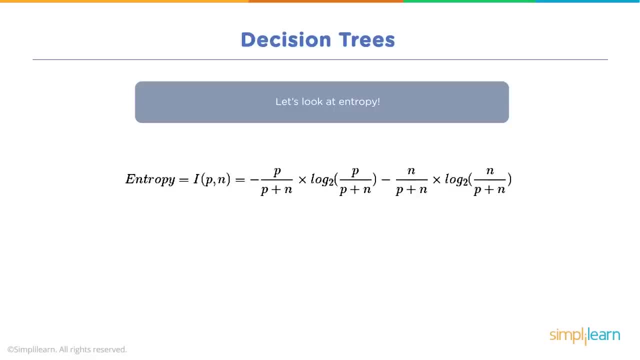 where this formula is coming from. so, when you see it, you're not lost when you're running your programming, unless you're building your own decision tree code in the back And we simply have a log squared of P over P plus N minus N over P plus N. 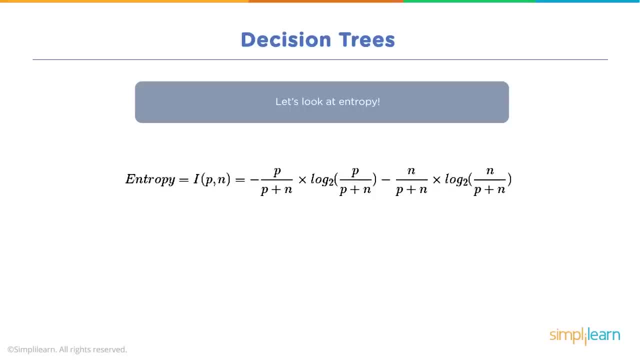 times the log squared of N, of P plus N. But let's break that down and see what it actually looks like when we're computing that from the computer script side. So we have entropy play golf. And when we look at this, if we go back to the data, 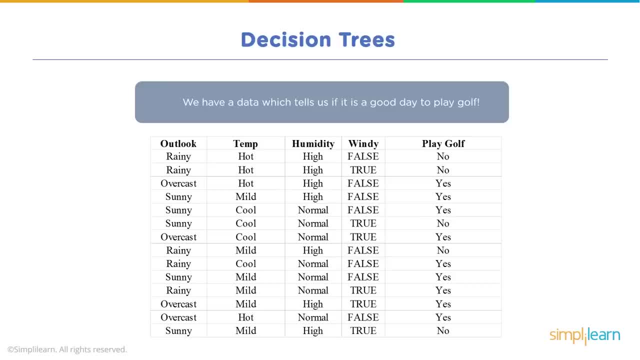 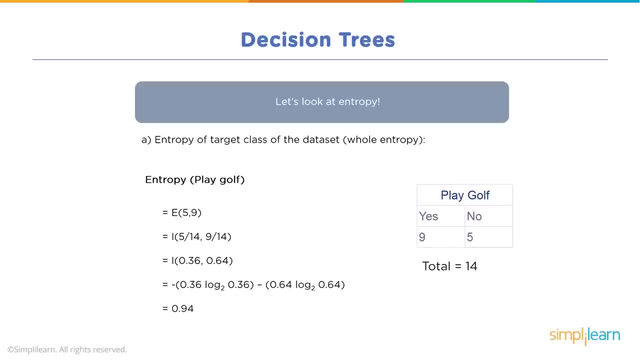 you can simply count how many yeses and no in our complete data set for playing golf days. In our complete set we find we have 5 days we did play golf and 9 days we did not play golf, And so our I equals. 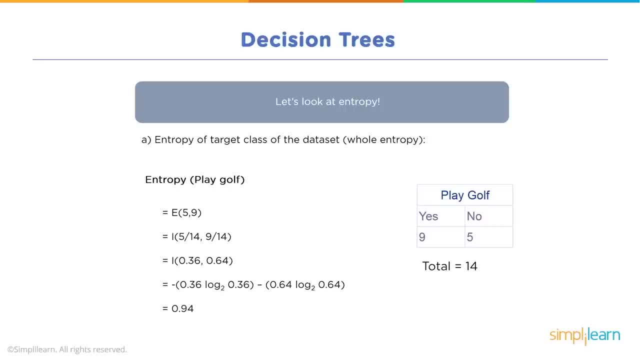 if you add those together, 9 plus 5 is 14.. And so our I equals 5 over 14 and 9 over 14.. That's our P and N values that we plug into that formula: 9 over 14 equals .36.. 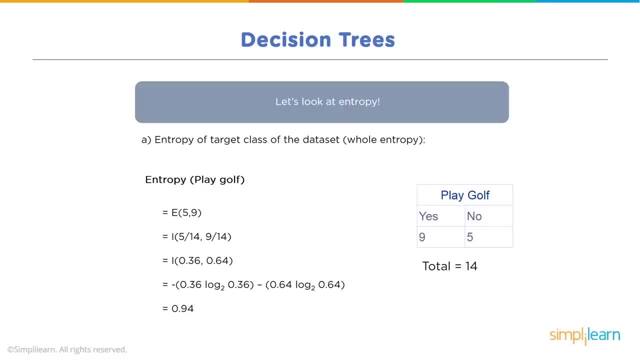 9 over 14 equals .64.. And when you do the whole equation you get the minus .36 log root squared of .36, minus .64 log squared root of .64.. And we get a set value. We get .94.. 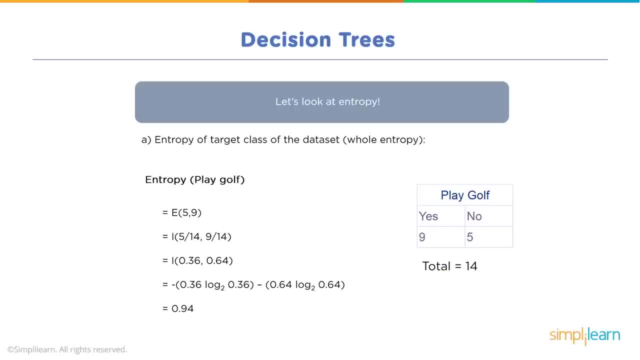 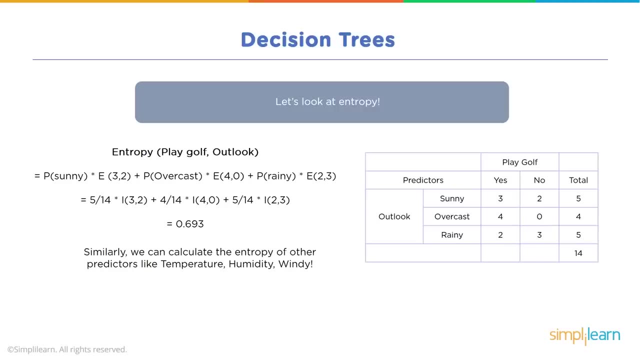 So we now have a full entropy value for the whole set of data that we're working with And we want to make that entropy go down. And just like we calculated the entropy out for the whole set, we can also calculate entropy for playing golf. 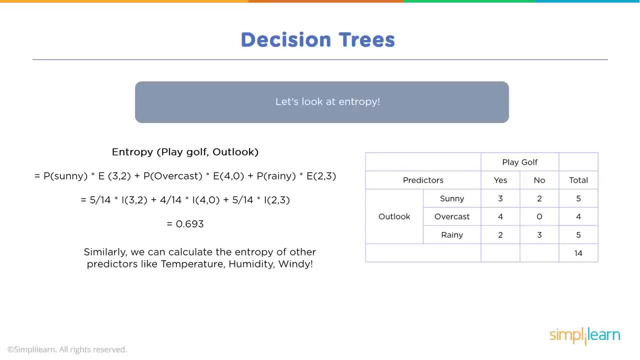 and the outlook. Is it going to be overcast or rainy or sunny? And so we look at the entropy. We have P of sunny times, E of 3 of 2. And that just comes out: how many sunny days yes and how many sunny days no. 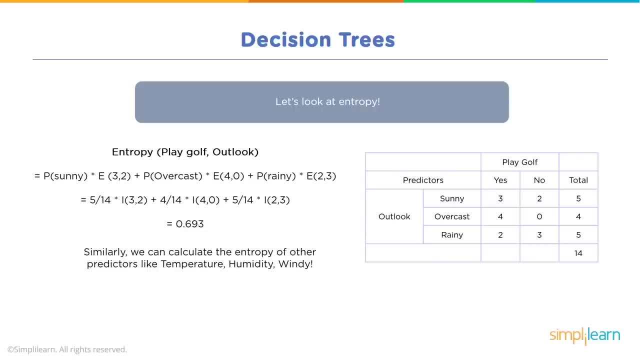 over the total, which is 5.. We'll divide that 5 out later on. Equals: P overcast equals 4 comma 0, plus rainy equals 2 comma 3.. And then, when you do the whole setup, we have 5 over 14. 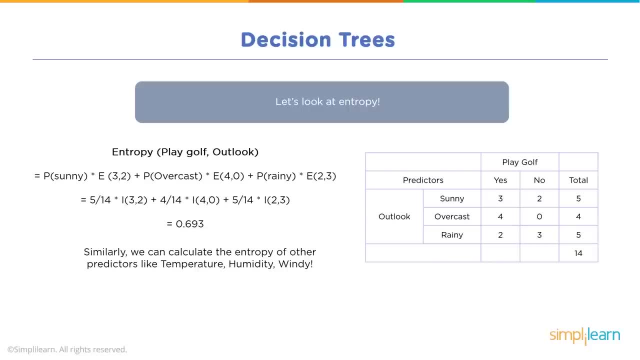 Remember I said there was a total of 5?: 5 over 14 times the I of 3 of 2, plus 4 over 14 times the 4 comma 0 and 5 over 14 times the I of 2 of 3.. 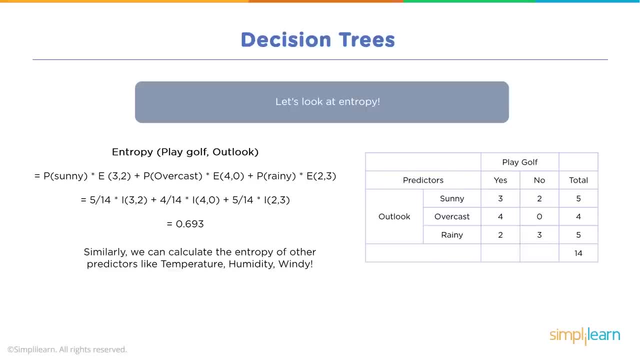 And so we can now compute the entropy of just the part that has to do with the forecast, And we get .693.. Similarly, we can calculate the entropy of other predictors like temperature, humidity and wind, And so we look at the gain outlook. 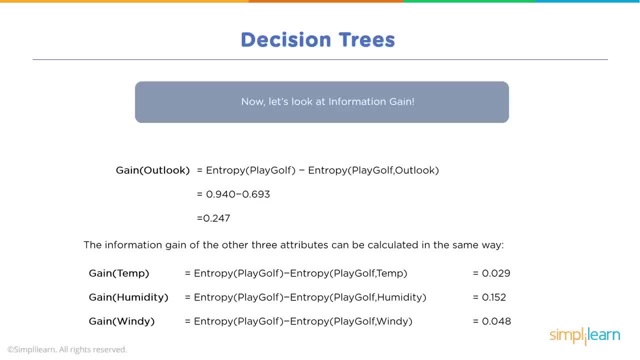 How much are we going to gain from this? Well, we can calculate the entropy of other predictors: entropy play golf minus entropy play golf outlook, And we can take the original .94 for the whole set minus the entropy of just the rainy day and temperature. 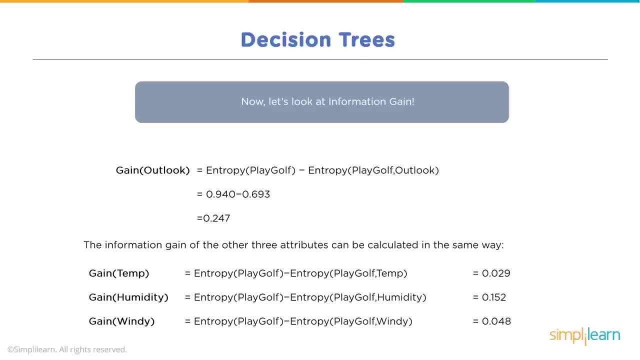 And we end up with a gain of .247.. So this is our information gain. Remember, we define entropy and we define information gain. The higher the information gain, the lower the entropy, the better. The information gain of the other three attributes can be calculated in the same way. 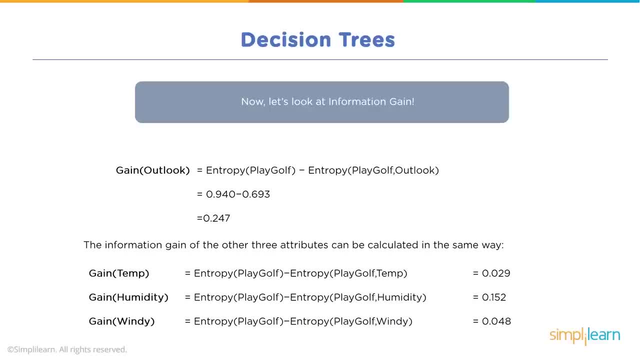 So we have our gain for temperature equals .029.. We have our gain for humidity equals .152.. And our gain for a windy day equals .048.. And if you do a quick comparison you'll see the .247 is the greatest gain of information. 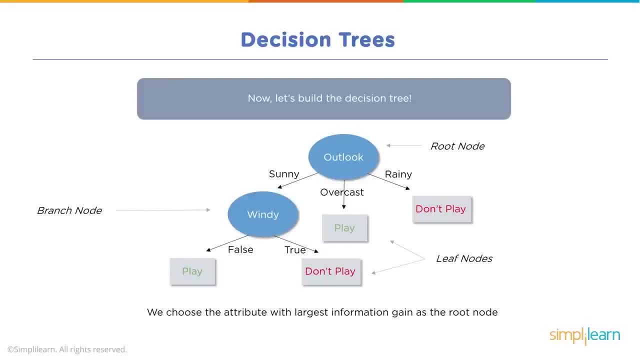 So that's the split we want. Now let's build the decision tree. So we have the outlook: Is it going to be sunny, overcast or rainy? That's our first split, because that gives us the most information gain And we can continue to go down the tree. 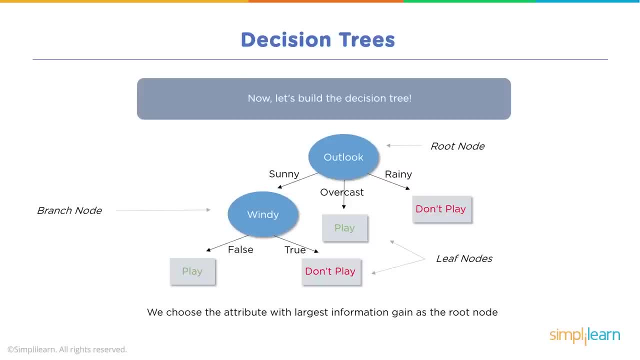 using the different information gains. We can continue down the nodes of the tree where we choose the attribute with the largest information gain as the root node and then continue to split each subnode with the largest information gain that we can compute, And although it's a little bit of a tongue twister, 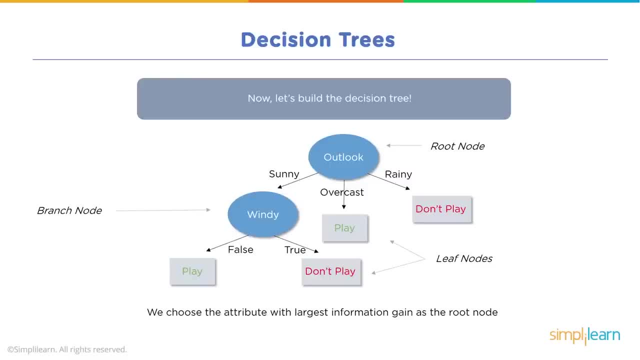 to say all that. you can see that it's a very easy to view visual model. We have our outlook, We split it three different directions. If the outlook is overcast, we're going to play, And then we can split those further down. 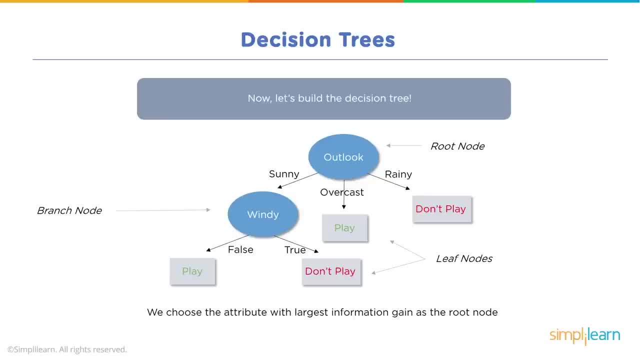 if we want. So the outlook is sunny, but then it's also windy. If it's windy, we're not going to play, If it's not windy, we'll play. So we can easily build a nice decision tree to guess what we would like to do tomorrow. 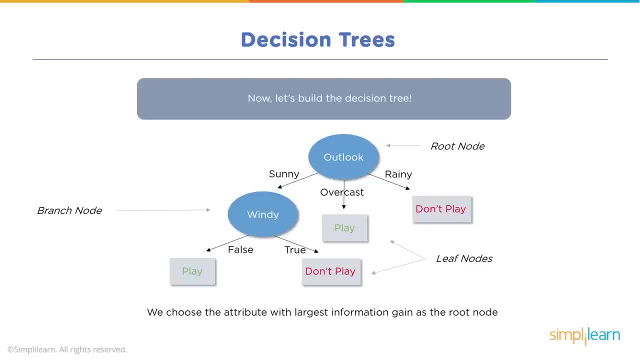 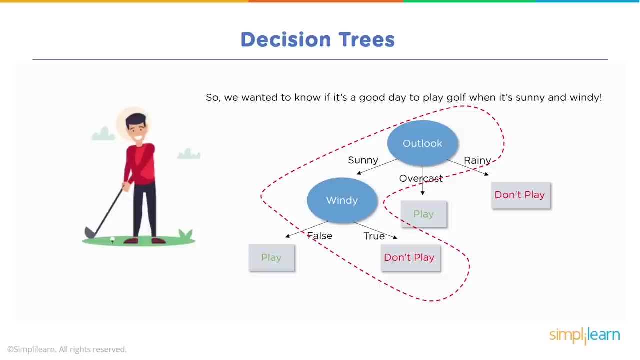 and give us a nice recommendation for the day. So we want to know if it's a good day to play golf when it's sunny and windy. Remember the original question that came out. Tomorrow's weather report is sunny and windy. You can see by going down the tree. 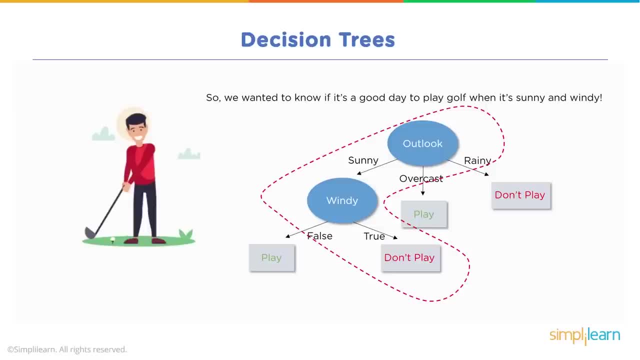 we go: outlook sunny, outlook windy. We're not going to play golf tomorrow. So our little smart watch pops up and says: I'm sorry, tomorrow's weather report is sunny. Tomorrow's not a good day for golf. It's going to be sunny and windy. 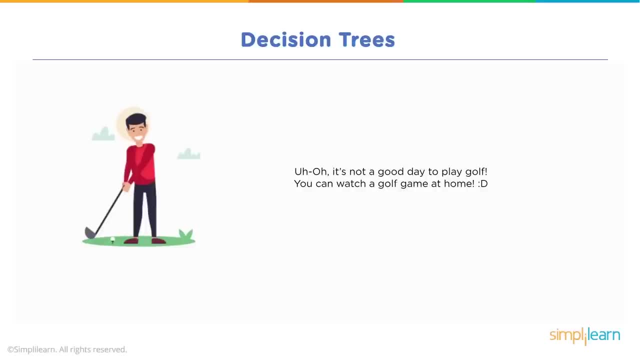 And if you're a huge golf fan, you might go. uh oh, it's not a good day to play golf. We can go in and watch a golf game at home, So we'll sit in front of the TV instead of being out playing golf in the wind. 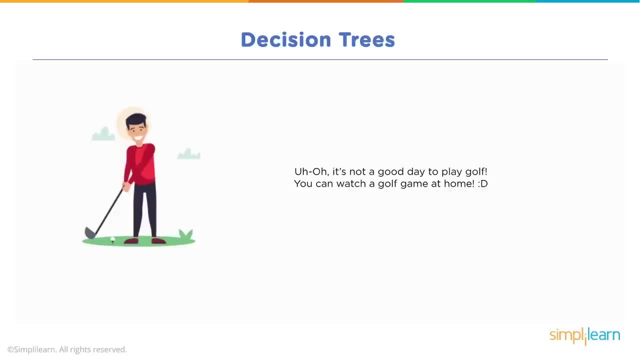 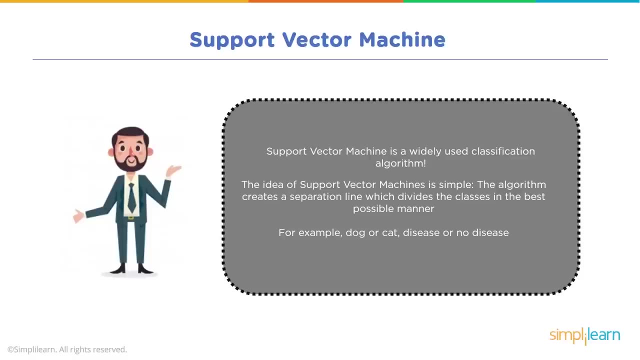 Now that we've looked at our decision tree, let's look at the third one of our algorithms. we're investigating Support Vector Machine. Support Vector Machine is a widely used classification algorithm. The idea of Support Vector Machine is simple: The algorithm creates a separation line. 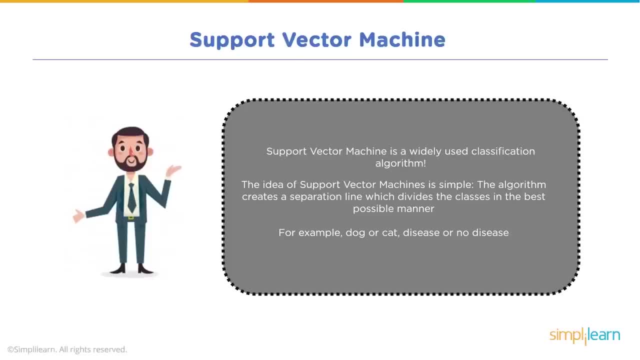 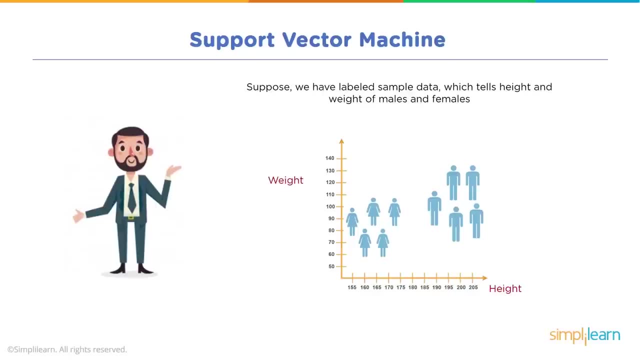 that divides the classes in the best possible manner, For example, dog or cat disease or no disease. Suppose we have a labeled sample data which tells height and weight of males and females. A new data point arrives and we want to know whether it's going to be a male or a female. 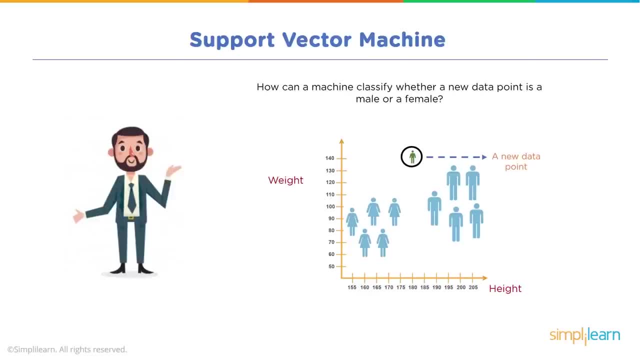 So we start by drawing a line, We draw decision lines, but if we consider decision line one then we will classify the individual as a male And if we consider decision line two then it will be a female. So you can see this person kind of lies. 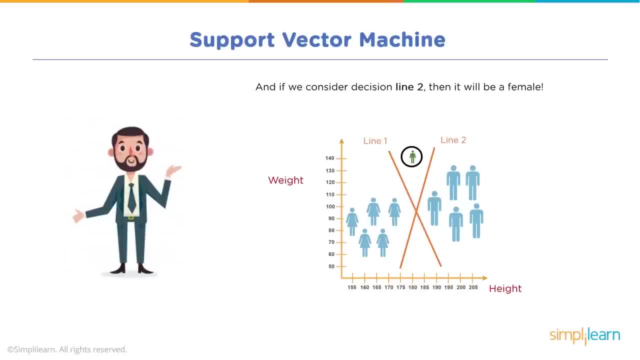 in the middle of the two groups, so it's a little confusing trying to figure out which line they should be under. We need to know which line divides the classes correctly, but how. The goal is to choose a hyperplane, and that is one of the key words they use. 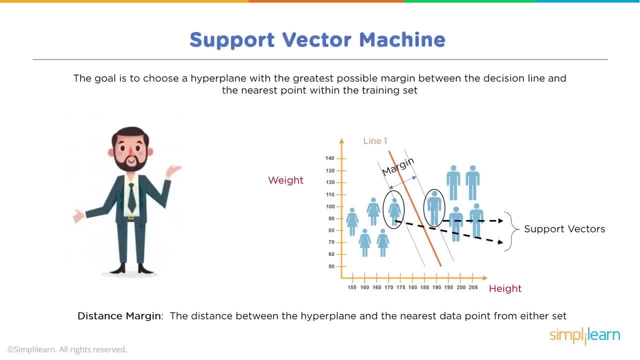 when we talk about Support Vector Machines, Choose a hyperplane with the greatest possible margin between the decision line and the nearest point within the training set. So you can see, here we have our support vector, we have the two nearest points to it. 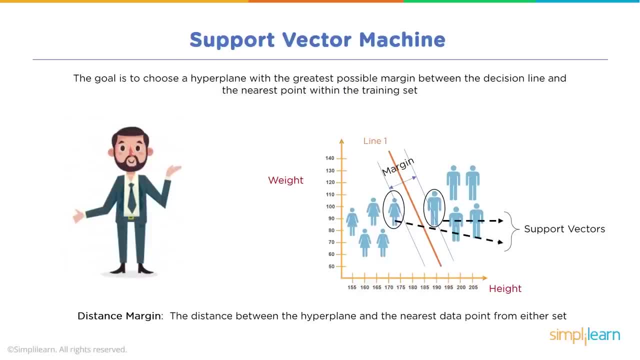 and we draw a line between those two points. The distance margin is the distance between the hyperplane and the nearest data point from either set. So we actually have a value and it should be equally distant between the two points that we're comparing it to. 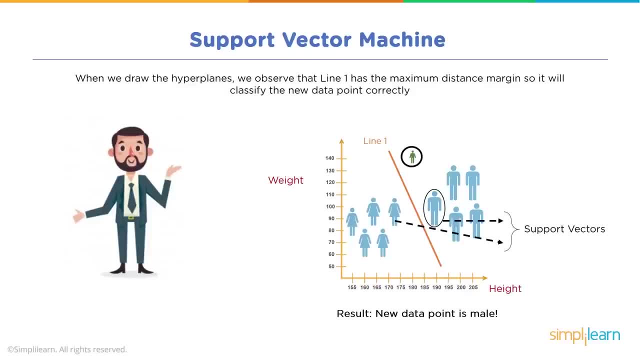 When we draw the hyperplanes, we observe that line one has a maximum distance. So we observe that line one has a maximum distance margin. so we'll classify the new data point correctly And our result on this one is going to be that the new data point is male. 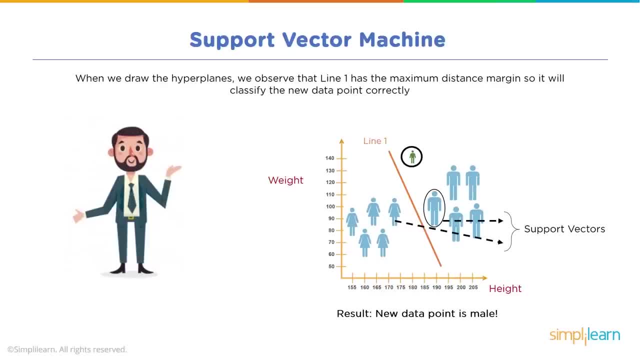 One of the reasons we call it a hyperplane versus a line is that a lot of times we're not looking at just weight and height. We might be looking at 36 different features or dimensions, And so when we cut it with a hyperplane, 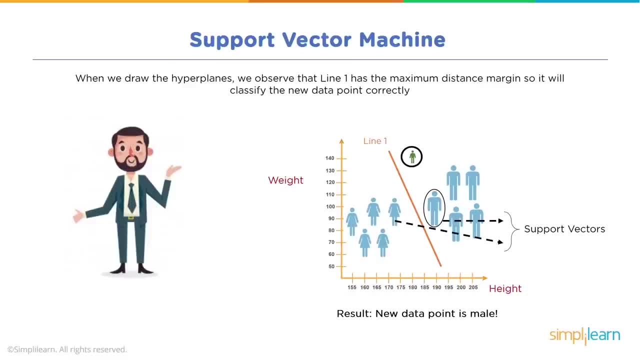 it's more of a three-dimensional cut in the data or multi-dimensional. It cuts the data a certain way And each plane continues to cut it down until we get the best fit or match. Let's understand this with the help of an example. 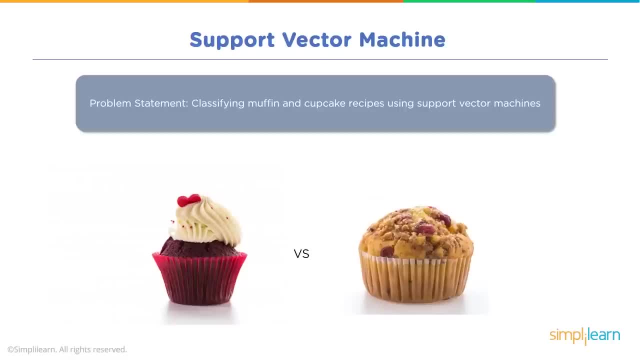 Problem statement. I always start with a problem statement when you're going to put some code together. Let's look at the different cupcake recipes using support vector machines. So the cupcake versus the muffin. Let's have a look at our data set. 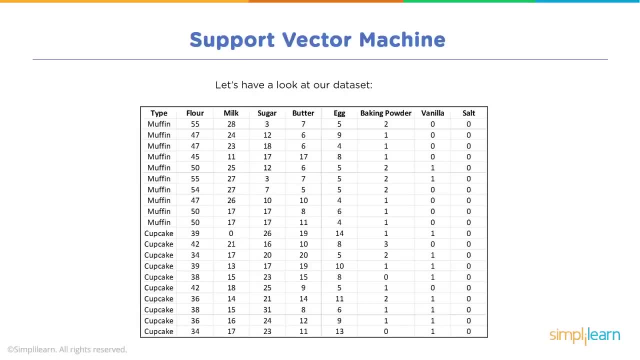 And we have the different recipes. here We have a muffin recipe that has so much flour- I'm not sure what measurement 55 is in, but it has 55, maybe it's ounces, But it has a certain amount of flour. 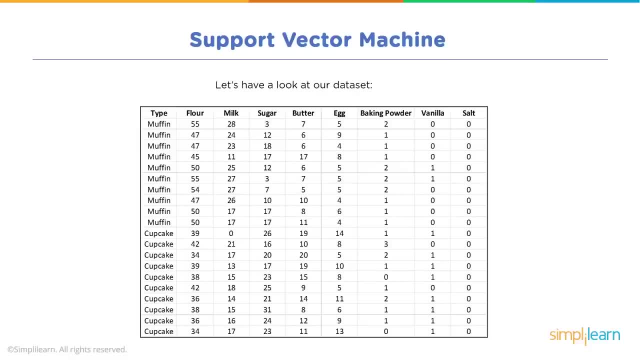 a certain amount of milk, sugar, butter, egg, baking powder, vanilla and salt, And so, based on these measurements, we want to guess whether we're making a muffin or a cupcake, And you can see in this one: 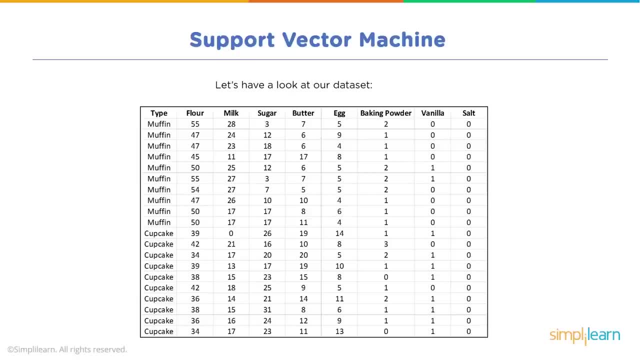 we don't have just two features. We don't just have height and weight, as we did before, between the male and female In here we have a number of features. In fact, in this we're looking at eight different features. to guess. 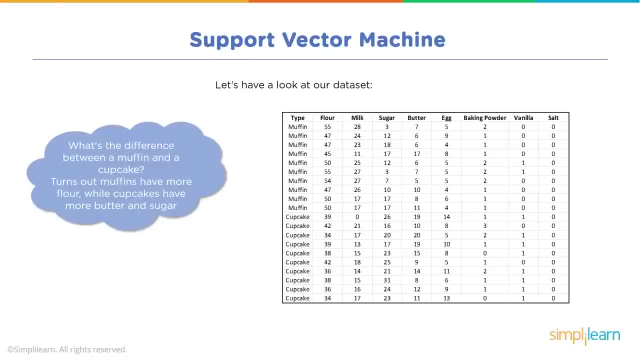 whether it's a muffin or a cupcake. What's the difference between a muffin and a cupcake? It turns out muffins have more flour, while cupcakes have more butter and sugar. So basically, the cupcake's a little bit more of a dessert, where the muffin's 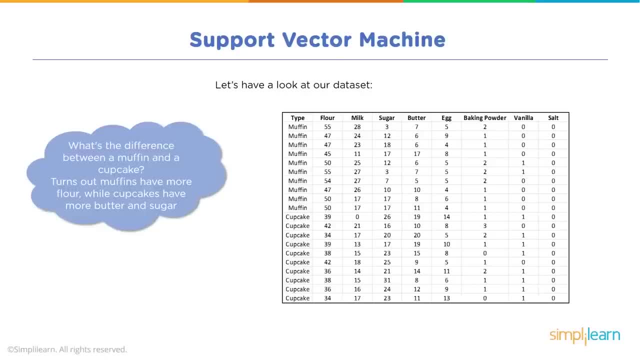 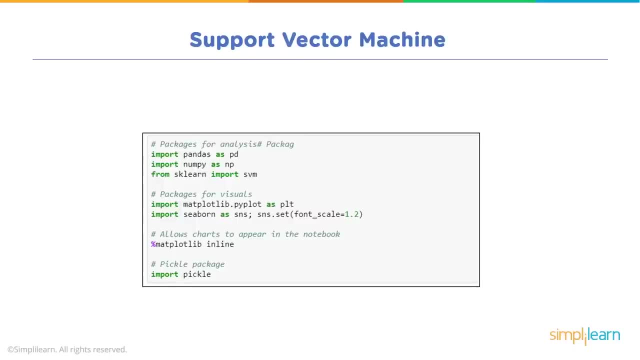 a little bit more of a dessert. How do we code that to go through recipes and figure out what the recipe is? And I really just want to say cupcakes versus muffins, Like some big professional wrestling thing, Before we start in our cupcakes versus muffins. 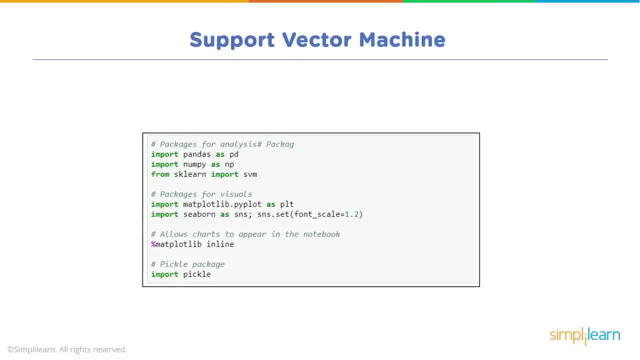 we are going to be working in Python. There's many versions of Python, many different editors. That is one of the strengths and weaknesses of Python is it just has so much stuff attached to it, and it's one of the more popular data science programming packages. 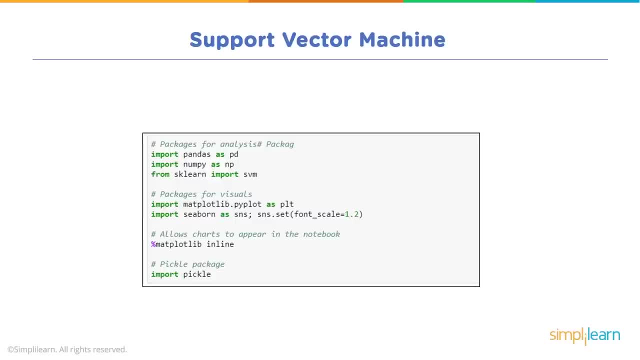 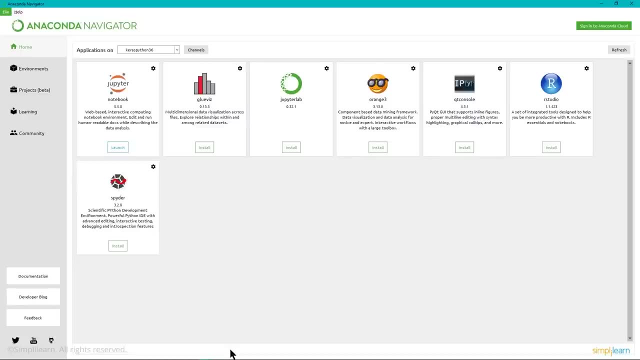 that you can use. In this case we're going to go ahead and use Anaconda in Jupyter Notebook. The Anaconda Navigator has all kinds of fun tools. Once you're into the Anaconda Navigator, you can change environments. I actually have a number of environments on here. 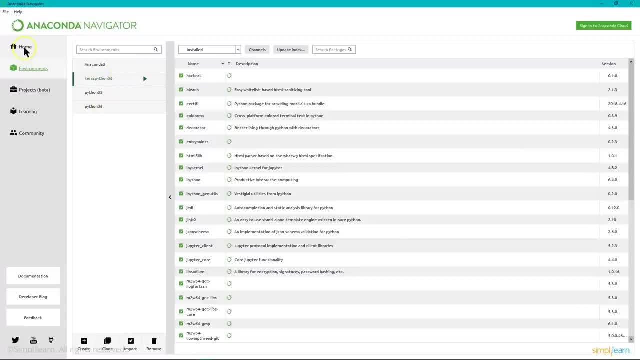 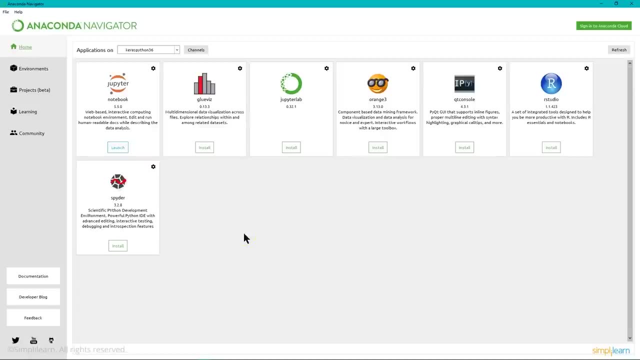 We'll be using Python 3.6 environment, So this is in Python version 3.6.. Although it doesn't matter too much which version you use, I usually try to stay with the 3.x because they're current, unless you have a project. 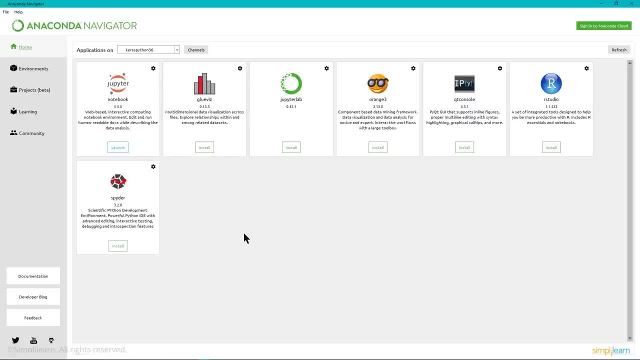 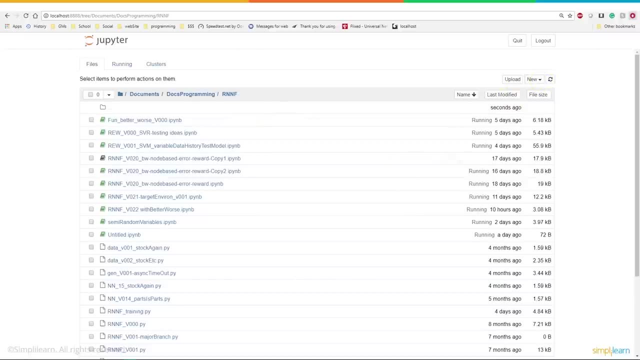 in version 2.x. 2.7,, I think, is usually what most people use in version 2.. Once we're in our Jupyter Notebook editor, I can go up and create a new file. We'll just jump in here. 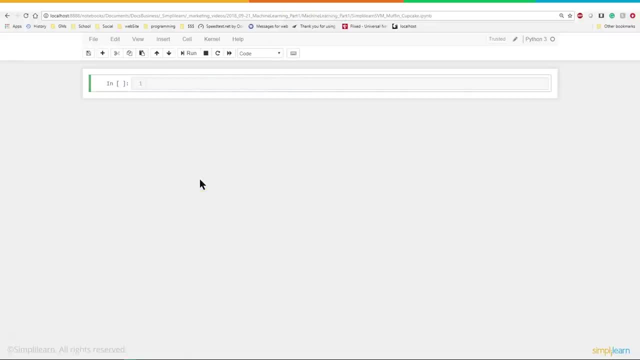 In this case we're doing SVM Muffin vs Cupcake. Let's start with our packages for data analysis. We almost always use a couple. there's a few very standard packages we use. We use import, oops, import, import. 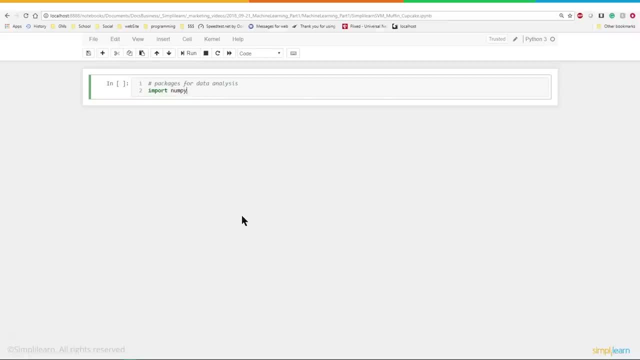 numpy, that's for number Python. They usually denote it as np. that's very common. That's very common. And then we're going to import pandas as pd, And numpy deals with number arrays. There's a lot of cool things you can do. 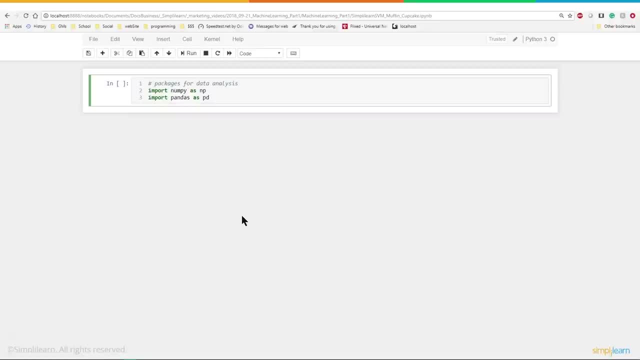 with the numpy setup. as far as multiplying all the values in an array, in a numpy array, data array, Pandas- I can't remember if we're using it actually, but I think we do. as an import, It makes a nice data frame. 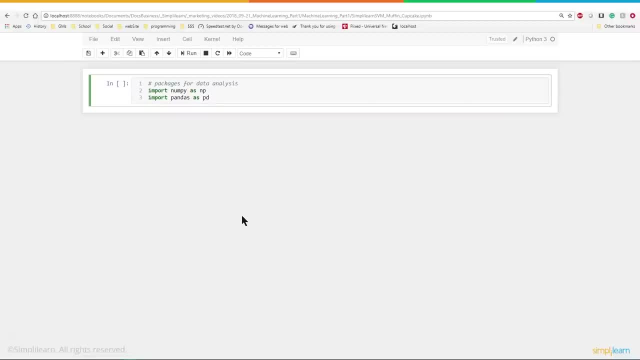 And the difference between a data frame and a numpy array is that a data frame is more like your Excel spreadsheet. You have columns, you have indexes, so you have different ways of referencing it, easily viewing it, and there's additional features. you can run on a data frame. 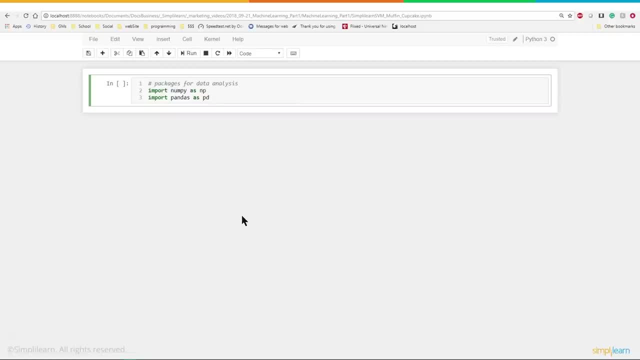 And pandas kind of sits on numpy, so you need them both in there. And then, finally, we're working with the support vector machine. So from sklearn we're going to use the sklearn learn model, import svm support vector machine. And then 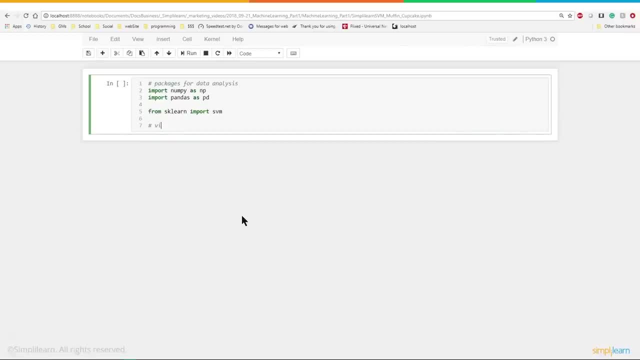 as a data scientist, you should always try to visualize your data. Some data obviously is too complicated or doesn't make any sense to the human, But if it's possible, it's good to take a second look at it so that you can actually see what you're doing. 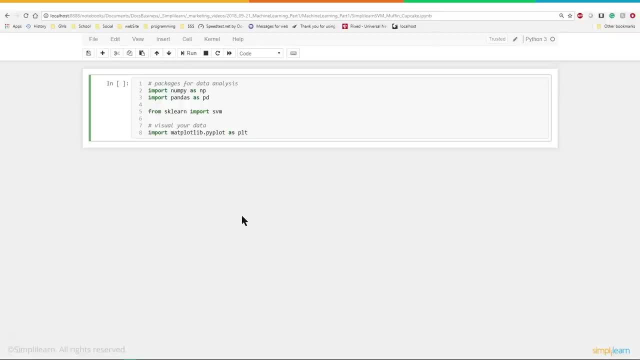 Now for that we're going to use two packages. We're going to import matplotlibrarypiplot as plt- Again very common- And then we're going to import seaborn as sns And we'll go ahead and set the font scale in the sns right in our import line. 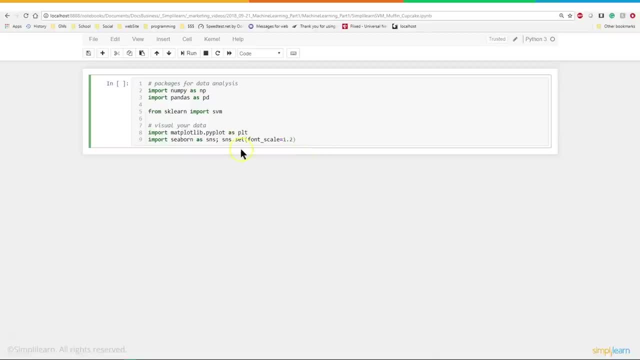 That's with this semicolon, followed by a line of data, We're going to set the sns. And these are great because the seaborn sits on top of matplotlibrary just like pandas sits on numpy. So it adds a lot more features and uses and control. 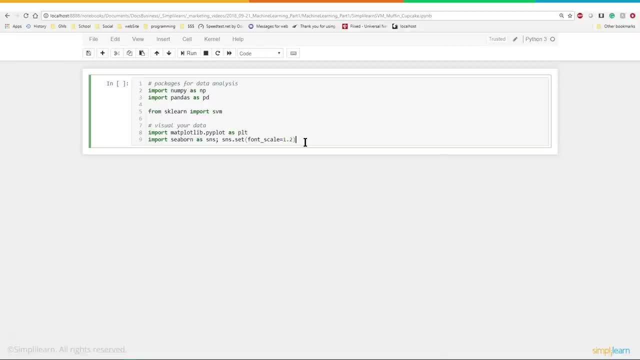 We're obviously not going to get into matplotlibrary and seaborn. That would be its own tutorial. We're really just focusing on the svm, the support vector machine from sklearn. And since we're in Jupyter Notebook, we have to add a special line in here. 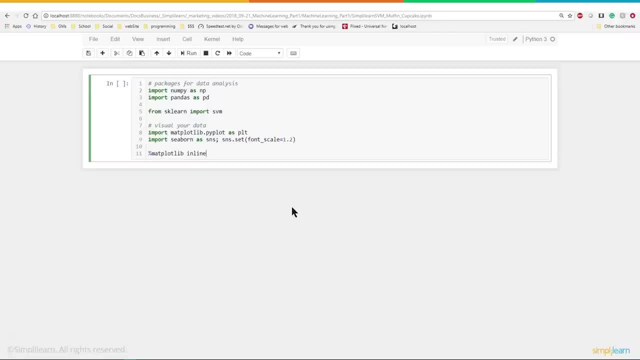 for our matplotlibrary And that's your percentage sign or amber sign, matplotlibrary in line. Now, if you're doing this in just a straight code project, a lot of times I use notepad++ and I'll run it from there. You don't have to have that line in there. 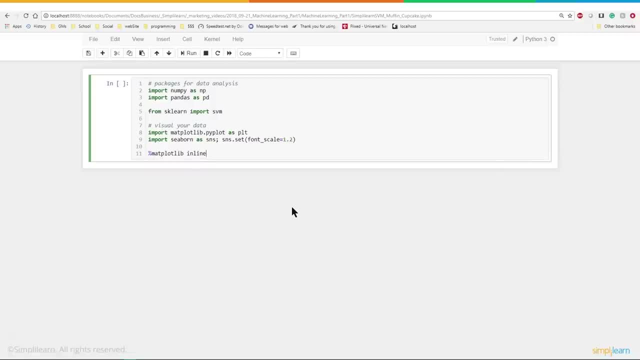 because it'll just pop up as its own window on your computer, depending on how your computer's set up. Because we're running this in the Jupyter Notebook as a browser setup, this tells it to display all of our graphics right below on the page. 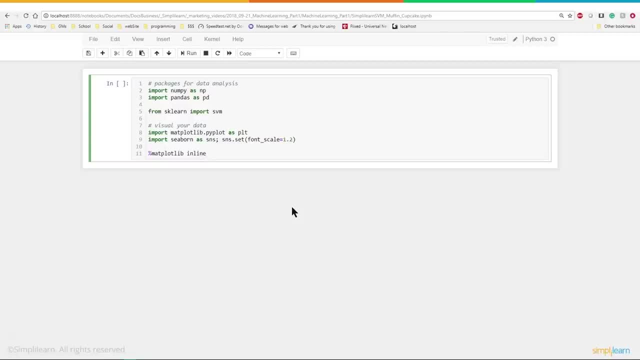 So that's what that line is for. Remember, the first time I ran this I didn't know that I had to go look that up years ago. It was quite a headache. So matplotlibrary inline is- just because we're running this on the web- setup. 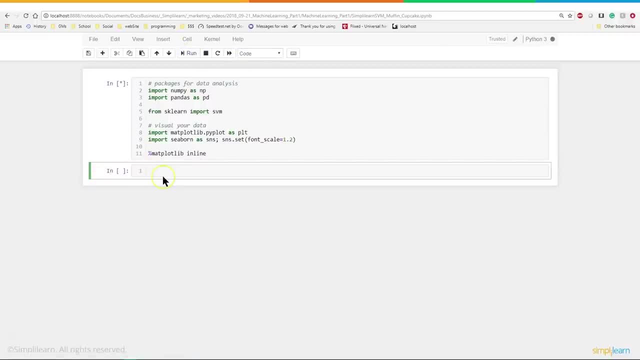 And we can go ahead and run this. make sure all our modules are in. They're all imported, which is great. If you don't have them import, use the PIP or however you do it. There's a lot of other install packages. 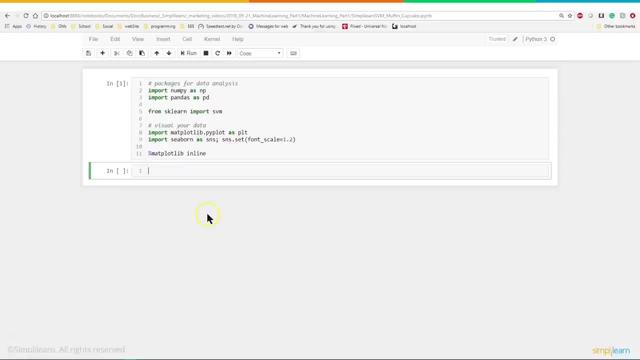 out there, although pip is the most common, And you have to make sure these are all installed on your Python setup. The next step, of course, is we've got to look at the data. You can't run a model for predicting data. 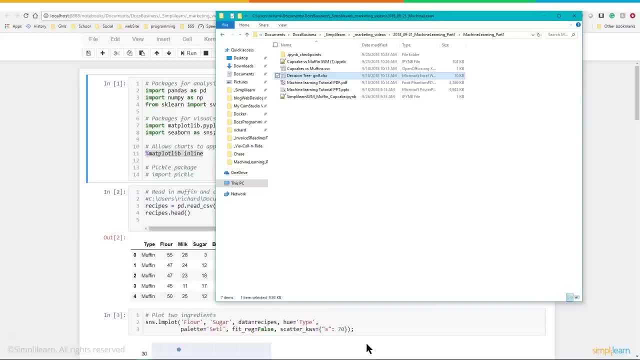 if you don't have actual data. So to do that, let me go ahead and open this up and take a look. And we have our cupcakes versus muffins And it's a CSV file, or csv, meaning that it's comma-separated variable. 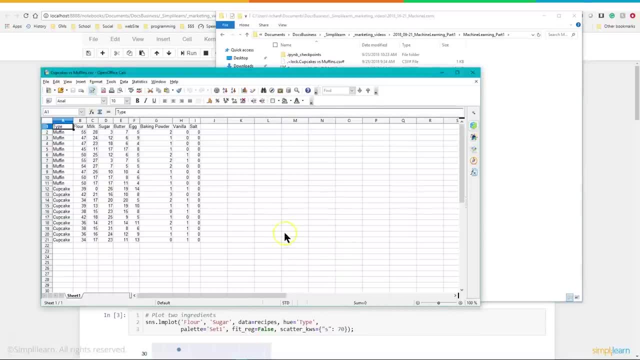 And it's going to open it up in a nice spreadsheet for me And you can see. up here we have the type We have: muffin muffin, muffin cupcake, cupcake cupcake, And then it's broken up into flour, milk, sugar. 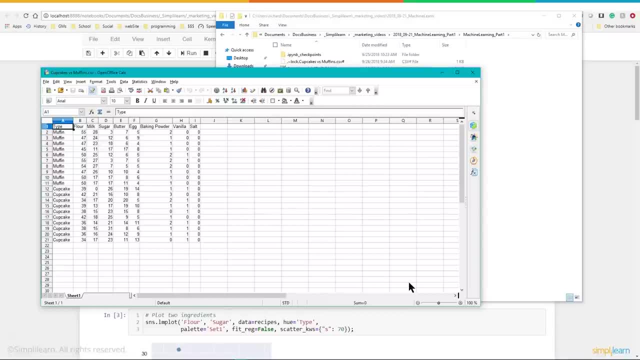 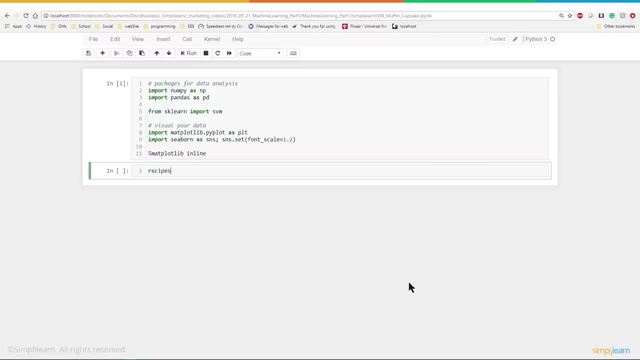 butter, egg, baking powder, vanilla and salt. So what we can do is we can go ahead and look at this data also in our Python. Let us create a variable recipes equals. we're going to use our pandas module, readcsv. 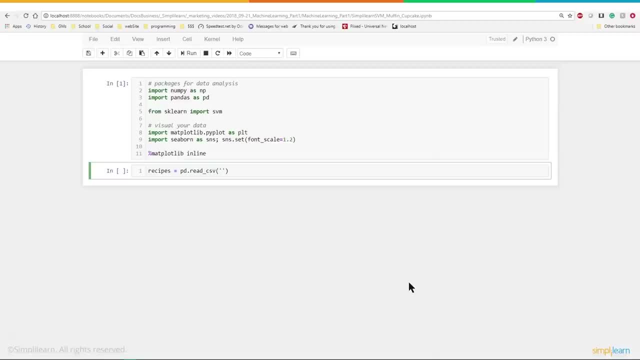 Remember it was a comma-separated variable And the file name happened to be cupcakes versus muffins. Oops, I got double brackets there. Do it this way. There we go: Cupcakes versus muffins. Because the program I loaded or the place I saved this particular. 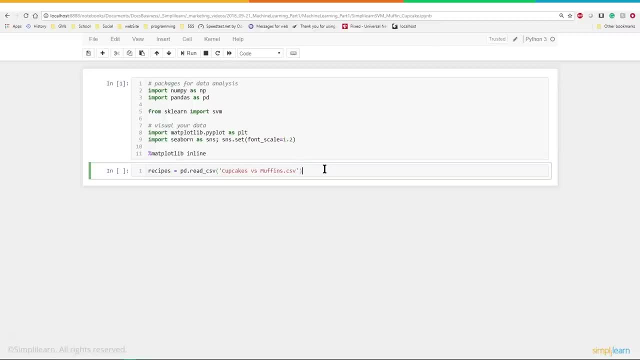 Python program is in the same folder. we can get by with just the file name, But remember, if you're storing it in a different location, you have to also put down the full path on there. And then, because we're in pandas, we're going to go ahead and 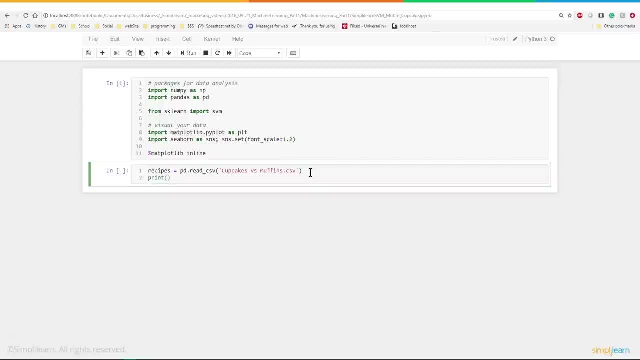 you can actually inline. you can do this, but let me do the full print. You can just type in recipeshead in the Jupyter Notebook, But if you're running in code in a different script, you'd need to go ahead and type out the whole print recipeshead. 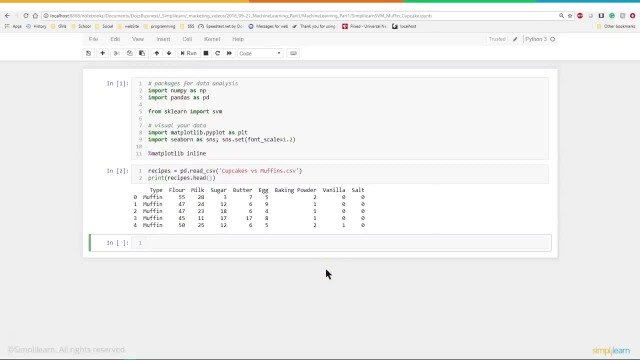 And pandas knows that's going to do the first five lines of data. If we flip back on over to the spreadsheet where we opened up our CSV file, you can see where it starts, on line two. This one calls it zero, And then two, three, four, five, six. 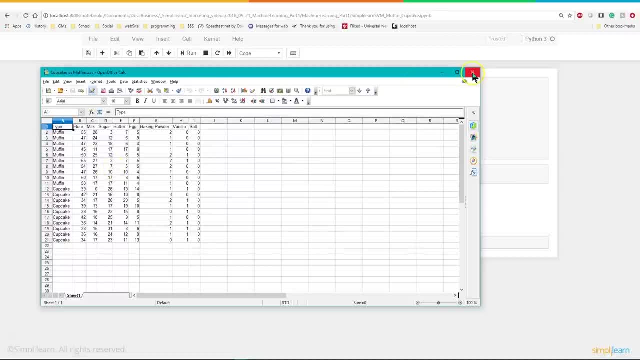 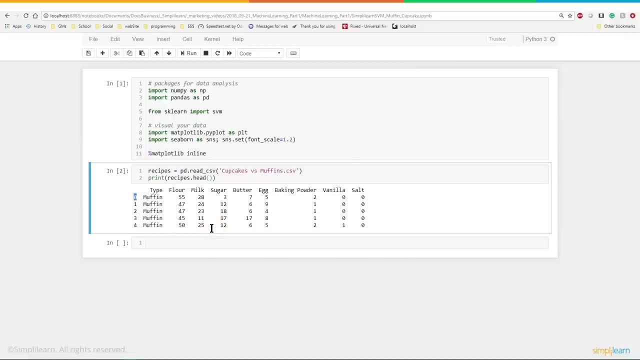 is going to match. Go ahead and close that out, because we don't need that anymore. And it always starts at zero. It automatically indexes it, since we didn't tell it to use an index in here. So that's the index number for the left-hand side. 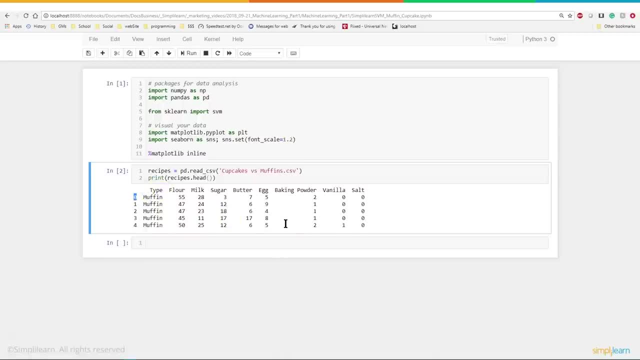 And it automatically took the top row as labels. So pandas, using it to read a CSV is just really slick and fast. One of the reasons we love our pandas, Not just because they're cute and cuddly teddy bears. And let's go ahead and plot. 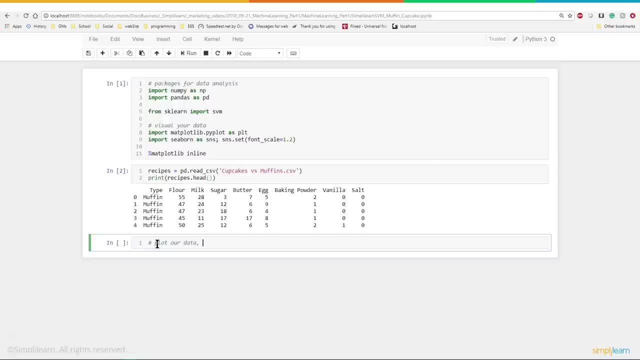 our data And I'm not going to plot all of it. I'm just going to plot the sugar and flour. Now, obviously, you can see where they get really complicated if we have tons of different features, And so you'll break them up and maybe look at just two of them. 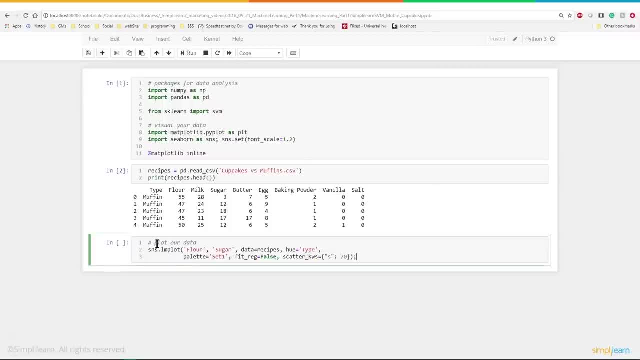 at a time to see how they connect And to plot them. we're going to go ahead and use Seaborn, So that's our SNS And the command for that is snslmplot, And then the two different variables. I'm going to plot is flour. 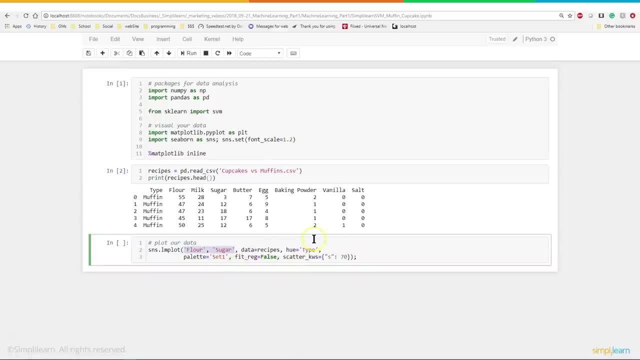 and sugar Data equals recipes, The hue equals type, And this is a lot of fun because it knows that this is pandas coming in. So this is one of the powerful things about pandas mixed with Seaborn And doing graphing. And then we're going to use a palette set one. 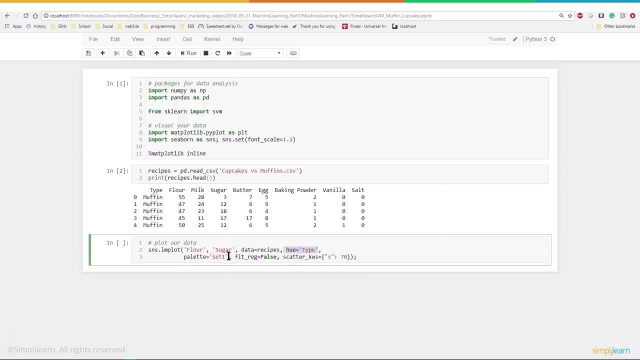 There's a lot of different sets in there. You can go look them up. for Seaborn We'll do a fit. regular equals false. So we're not really trying to fit anything And it's a scatter KWS. A lot of these settings you can look up in Seaborn. 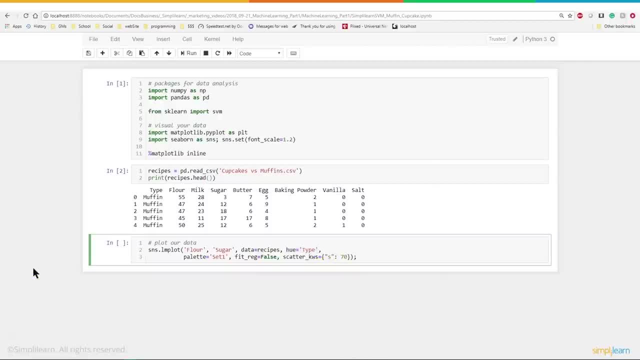 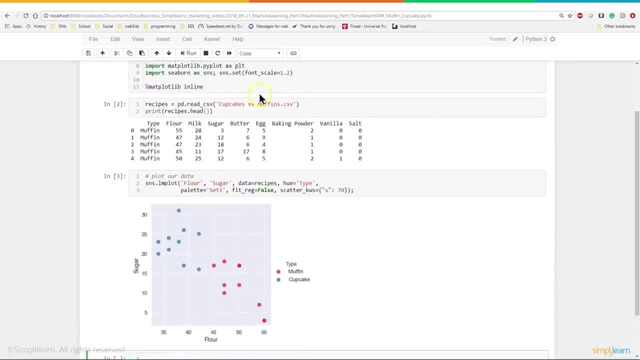 Half of these you could probably leave off when you run them. Somebody played with this and found out that these were the best settings for doing a Seaborn plot, And let's go ahead and run that. And because it does it in line, it just puts it. 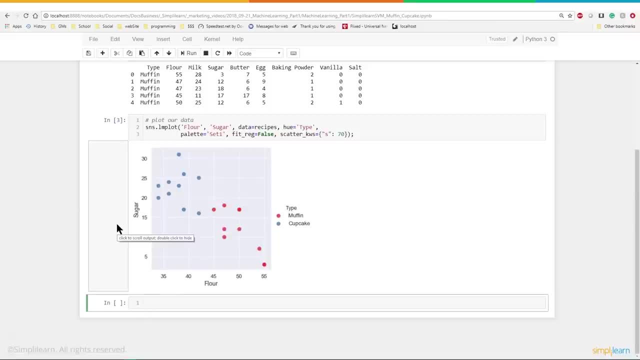 right on the page And you can see right here that, just based on sugar and flour alone, there's a definite split. And we use these models because you can actually look at it and say, hey, if I drew a line right between the middle of the blue dots and the red. 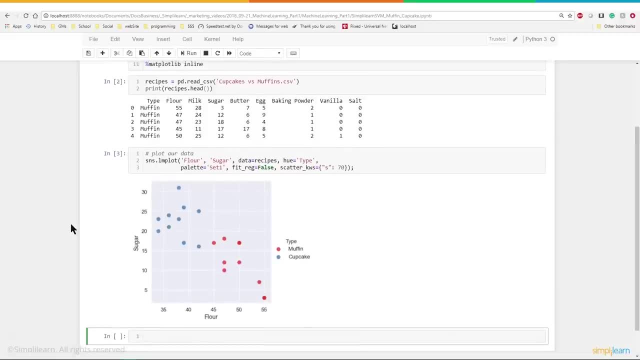 dots, we'd be able to do an SVM and a hyperplane right there in the middle. Then the next step is to format or pre- process our data, And we're going to break that up into two parts. We need a type label And remember. 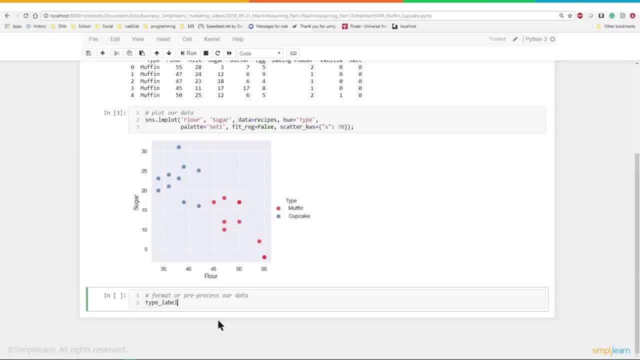 we're going to decide whether it's a muffin or a cupcake. Well, a computer doesn't know muffin or cupcake, It knows zero and one. So what we're going to do is we're going to create a type label And from this, 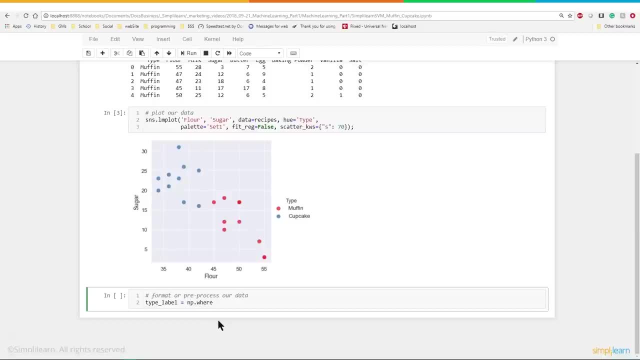 we'll create a numpy array and p where- and this is where we can do some logic- We take our recipes from our panda and wherever a type equals muffin, it's going to be zero, And then, if it doesn't equal muffin, which is cupcakes, it's going to be one. 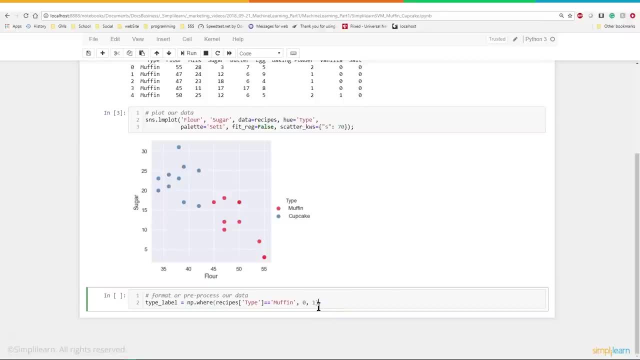 So we create our type label. This is the answer. So when we're doing our training model, remember we have to have a training data. this is what we're going to train it with. is that it's zero or one? It's a muffin or it's not. 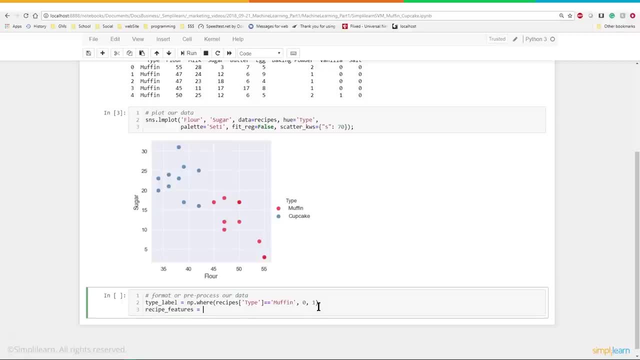 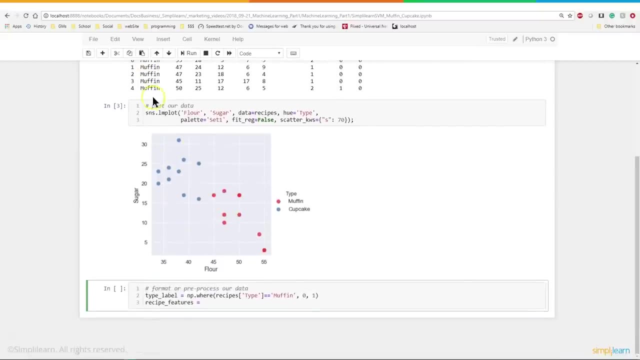 And then we're going to create our recipe features And if you remember correctly from right up here, the first column is type. So we really don't need the type column, because that's our muffin or cupcake And in pandas we can easily 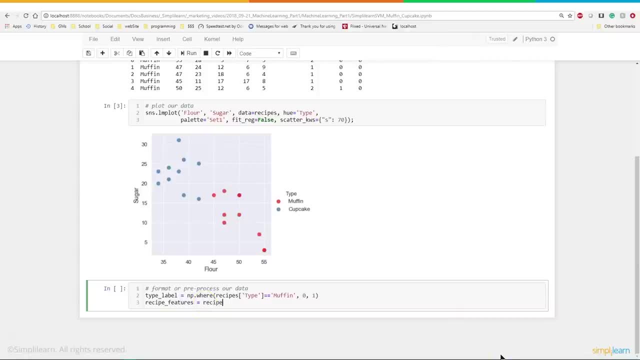 sort that out? We take our value recipes dot columns. That's a pandas function built into pandas Dot values, Converting them to values. So it's just the column titles going across the top, And we don't want the first one. 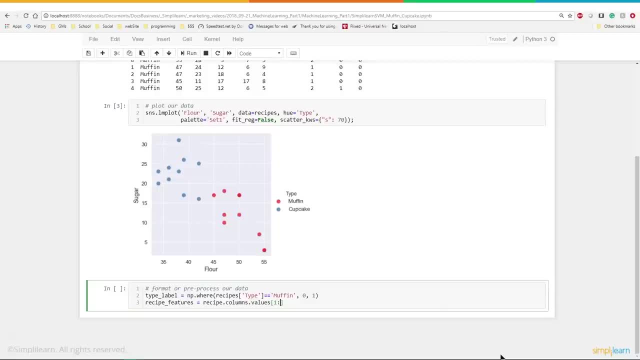 So what we do is, since it always starts at zero, we want one colon till the end, And then we want to go ahead and make this a list, And this converts it to a list of strings, And then we can go ahead and just take a. 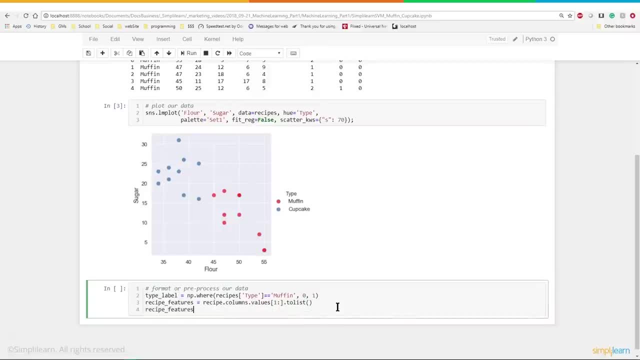 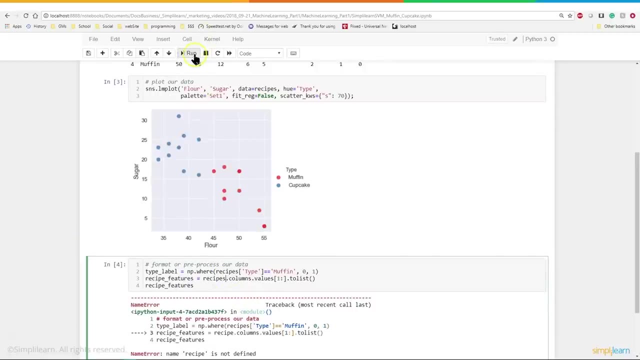 look and see what we're looking at for the features. Make sure it looks right, Go ahead and run that. And I forgot the S on recipes, So we'll go ahead and add the S in there and then run that And we can see we have flour. 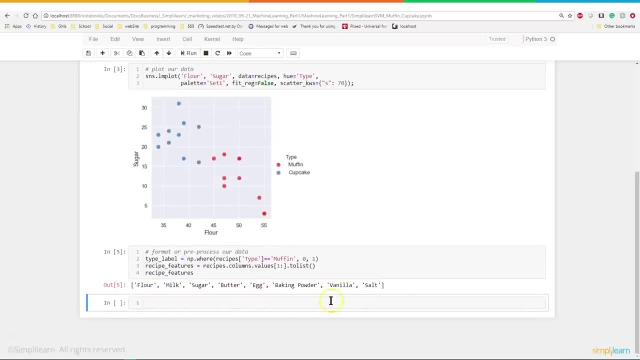 milk, sugar, butter, egg, baking powder, vanilla and salt, And that matches what we have up here, Right where we printed out everything but the type. So we have our features and we have our label. Now the recipe features is just. 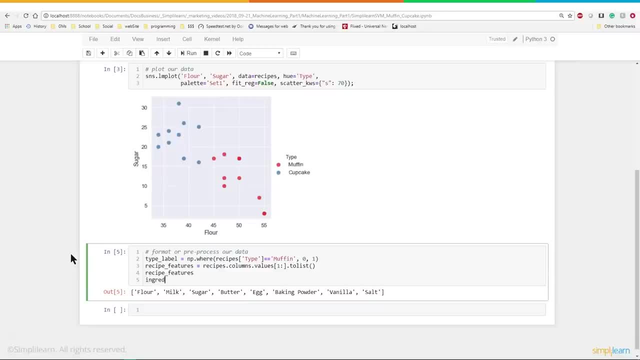 the titles of the columns And we actually need the ingredients. And at this point we have a couple options. One: we could run it over all the ingredients, And when you're doing this, usually you do, But for our example, we want to limit it. 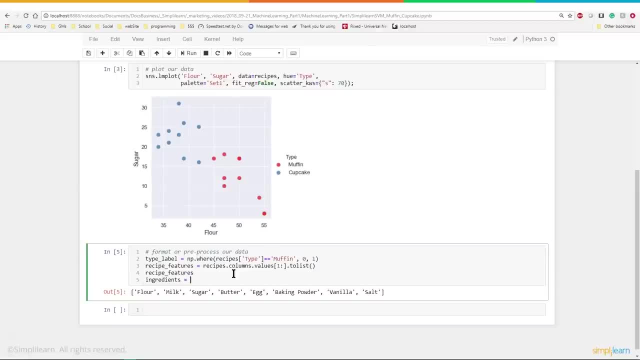 so you can easily see what's going on. Because if we did all the ingredients we have, you know that's what seven, eight different hyperplanes that would be built into it, And we only want to look at one so you can see what. 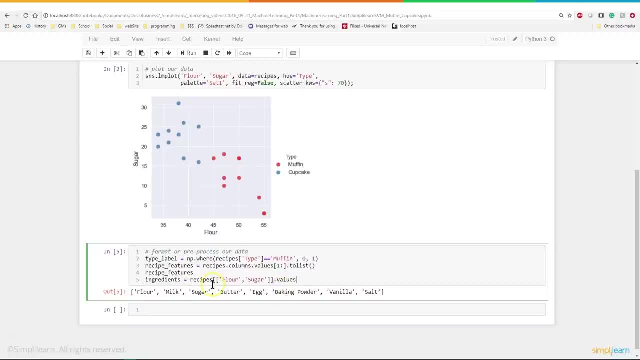 the SVM is doing, And so we'll take our recipe and we'll do just flour and sugar. Again, you can replace that with your recipe features and do all of them, But we're going to do just flour and sugar and we're going to convert that to values. 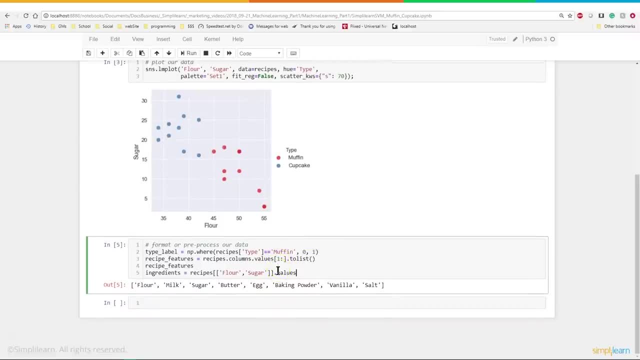 We don't need to make a list out of it because it's not string values. These are actual values on there And we can go ahead and just print ingredients And you can see what that looks like. And so we have just the amount of flour and sugar. 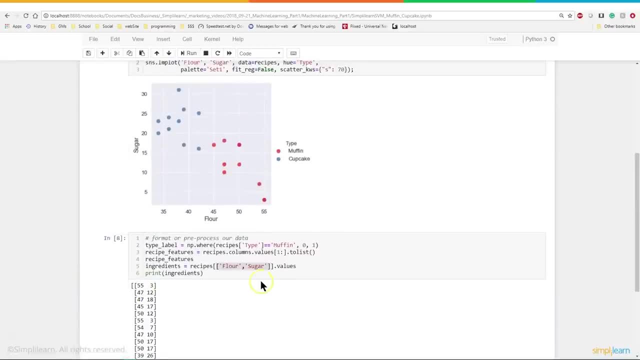 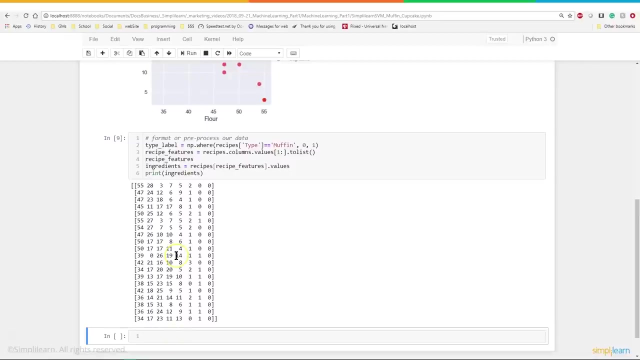 Just the two sets of plots And just for fun, let's go ahead and take this over here and take our recipe features, And so if we decided to use all the recipe features, you'll see that it makes a nice column of different data. 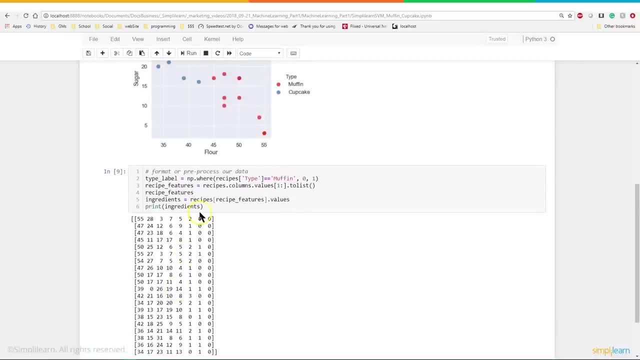 So it just strips out all the labels and everything and we just have just the values. But because we want to be able to view this easily in a plot later on, we'll go ahead and take that and just do flour and sugar And we'll run that. 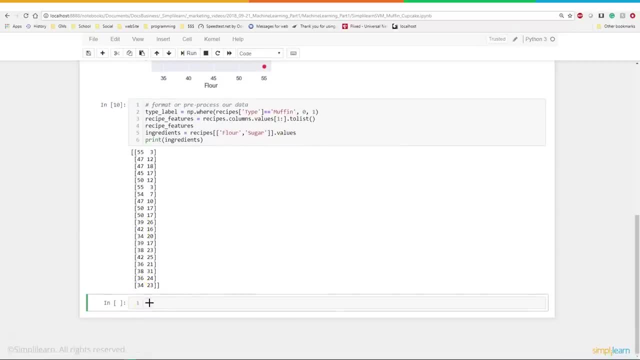 and you'll see it's just the two columns. So the next step is to go ahead and fit our model. We'll go ahead and just call it model And it's a SVM. We're using a package called SVC In this case. 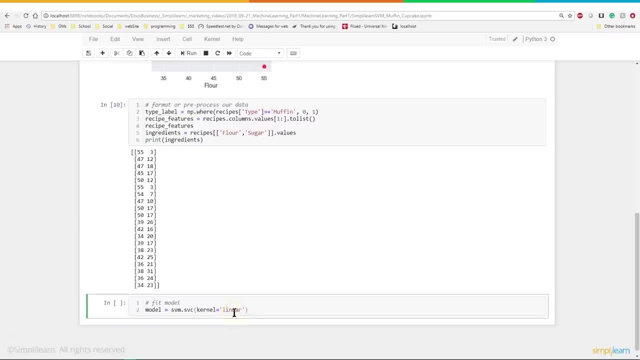 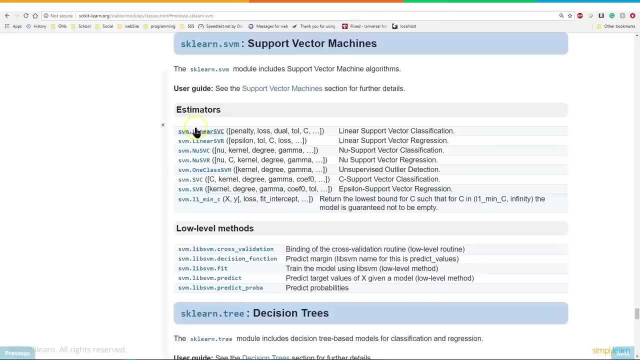 we're going to go ahead and set the kernel equals linear, So it's using a specific setup on there, And if we go to the reference on their website for the SVM, you'll see that there's about there's eight of them here. Three of them are 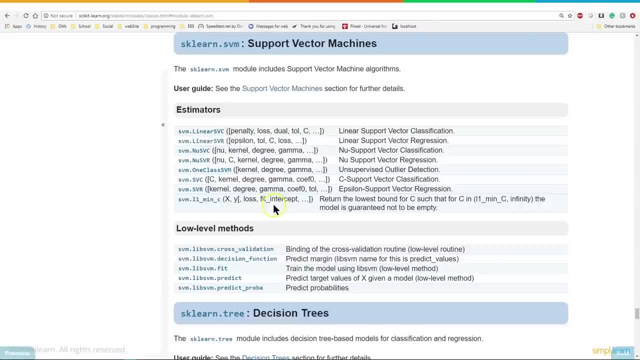 for regression, Three are for classification. The SVC support vector classification is probably one of the most commonly used, And then there's also one for detecting outliers And another one that has to do with something a little bit more specific on the model. 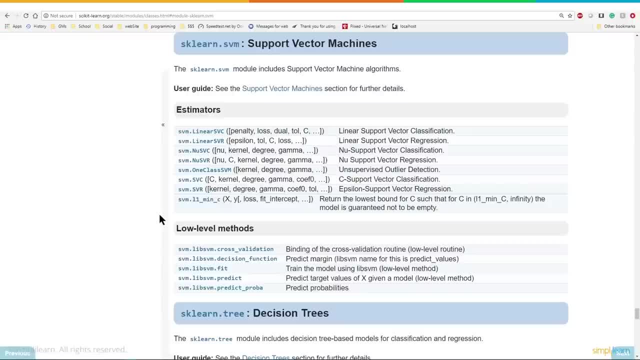 But SVC and SVR are the two most commonly used, standing for support vector classifier and support vector regression. Remember, regression is an actual value, A float value or whatever you're trying to work on, And SVC is a classifier, So it's a yes. 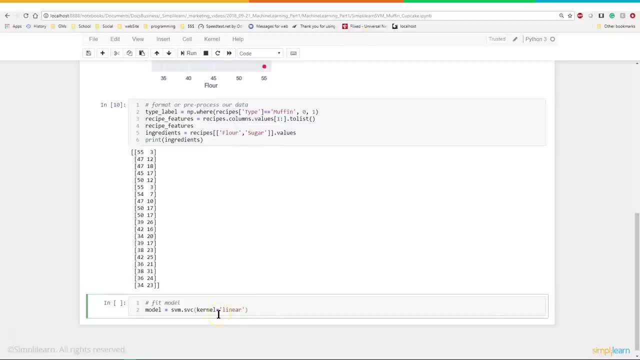 no, true, false. But for this we want to know: zero, one muffin cupcake. So we go ahead and create our model And once we have our model created, we're going to do modelfit, And this is very common, especially in the sklearn. 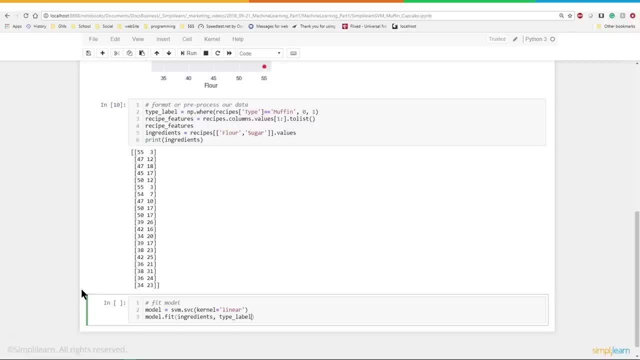 All their models are followed with the fit command, And what we put into the fit, what we're training with it is we're putting in the ingredients, which in this case, we limited to just flour and sugar, And the type label. Is it a model? 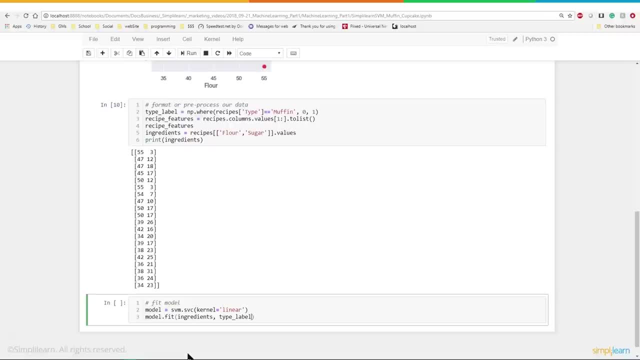 muffin or cupcake. Now, in more complicated data science series you'd want to split into. we won't get into that today. we split it into training data and test data, And they even do something where they split it into thirds. where a third? 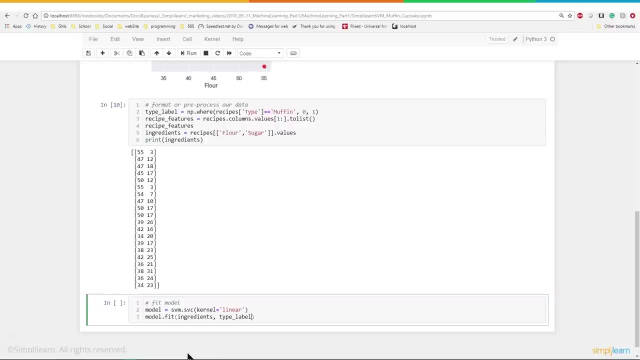 is used for, where you switch between which one's training and test. There's all kinds of things that go into that. It gets very complicated when you get to the higher end- Not overly complicated. Just an extra step, which we're not going to do today because this is a very 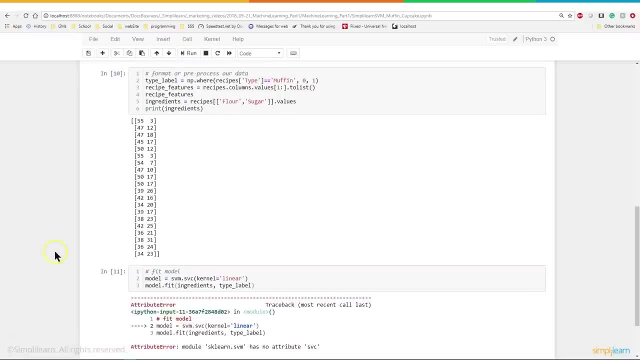 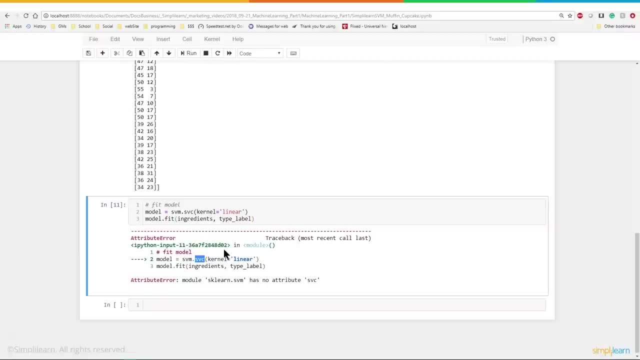 simple set of data And let's go ahead and run this And now we have our model fit And I got an error here, so let me fix that real quick. It's capital SVC, it turns out. I did it lower case. 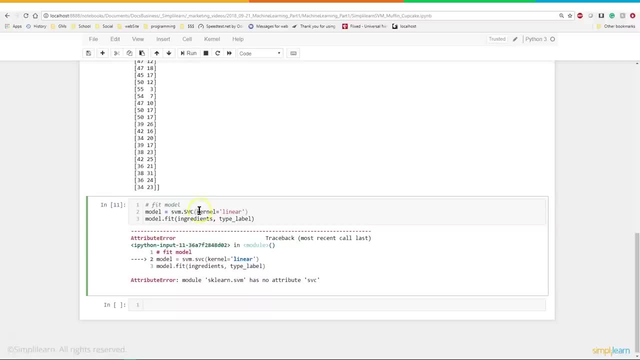 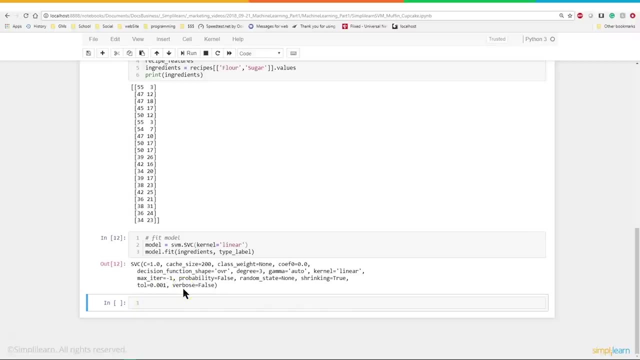 Support vector classifier. There we go. Let's go ahead and run that And you'll see it comes up with all this information that it prints out automatically. These are the defaults of the model. You notice that we changed the kernel to linear. 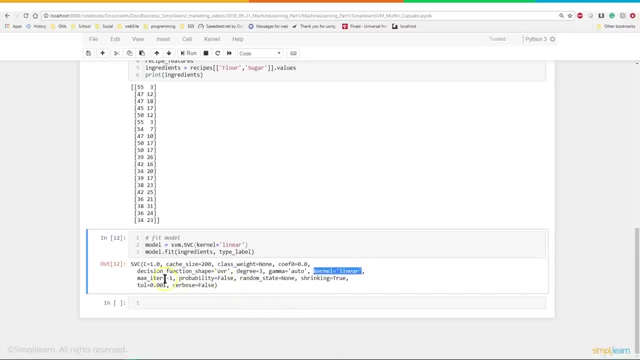 And there's our kernel linear on the printout And there's other different settings you can mess with. We're going to just leave that alone right now for this. We don't really need to mess with any of those. So next we're going to dig a little bit into 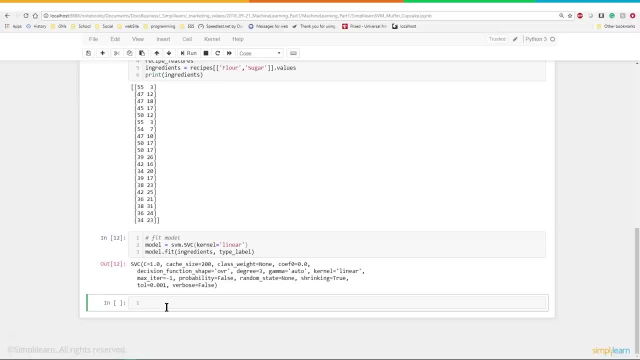 our newly trained model And we're going to do this so we can show you on a graph And let's go ahead and get the separating. We're going to use a W for our variable on here. We're going to do modelcoefficient. 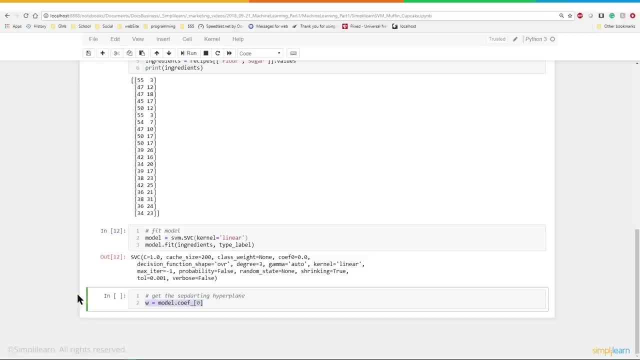 underscore zero. So what the heck is that? Again, we're digging into the model, So we've already got a prediction and a train. This is the math behind it that we're looking at right now, And so the W is going to represent. 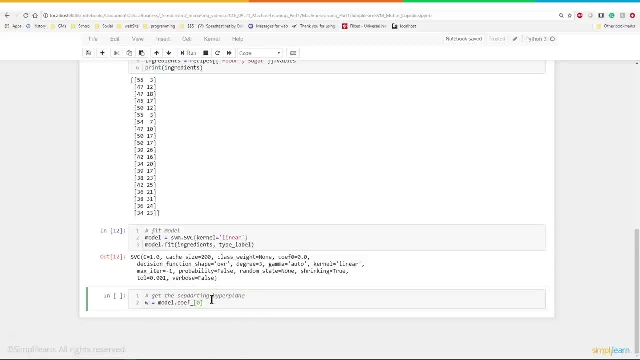 two different coefficients And if you remember we had y equals mx plus c, So these coefficients are connected to that. but in two-dimensional It's a plane. We don't want to spend too much time on this because you can get lost. 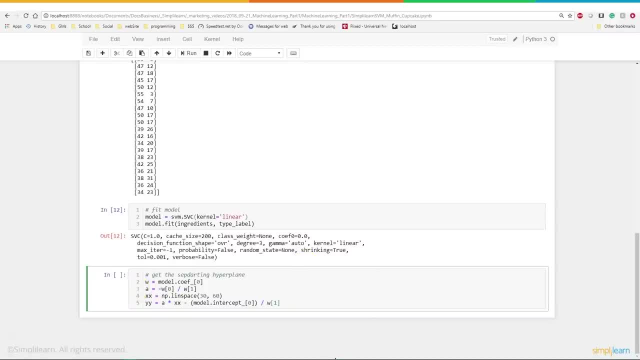 in the confusion of the math. So if you're a math whiz, this is great. You can go through here and you'll see that we have a equals minus W of zero over W of one. Remember there's two different values there. 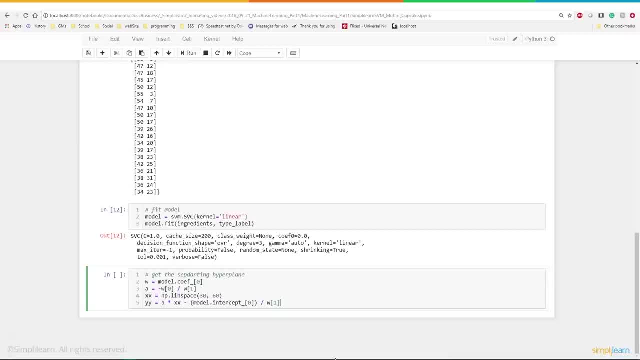 And that's basically the slope that we're generating. And then we're going to build an xx. What is xx? We're going to set it up to a numpy array. There's our numpylinespace, So we're creating a line of values between: 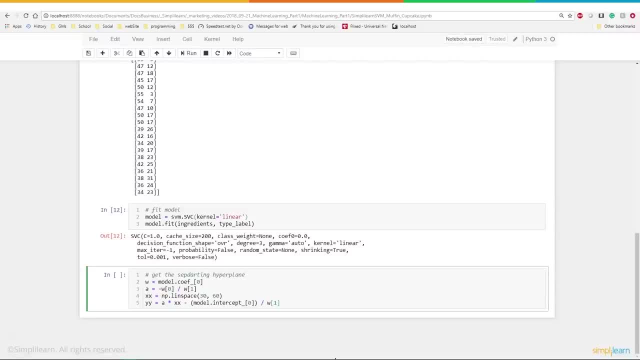 30 and 60. So it just creates a set of numbers for x And then, if you remember correctly, we have our formula: y equals the slope times x plus the intercept. Well, to make this work, we can do this as yy. 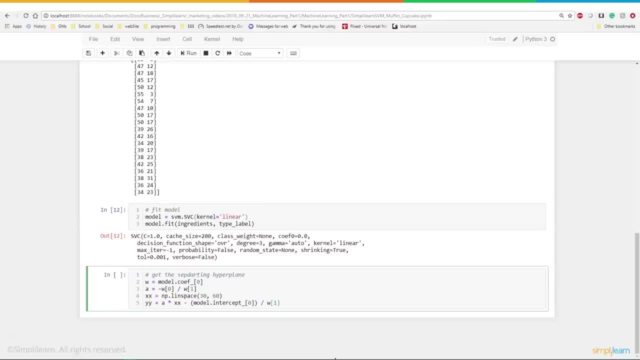 equals the slope times each value in that array. And that's the neat thing about numpy. So when I do a times xx, which is a whole numpy array of values, it multiplies a across all of them And then it takes those same values. 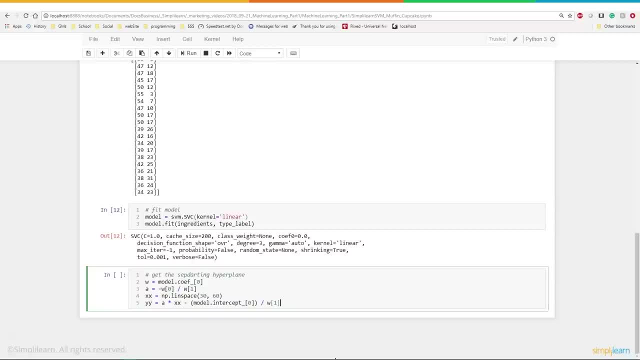 and we subtract the model intercept. That's your. Remember we had mx plus c, So that would be the c from the formula y equals mx plus c, And that's where all these numbers come from. A little bit confusing because it's digging out. 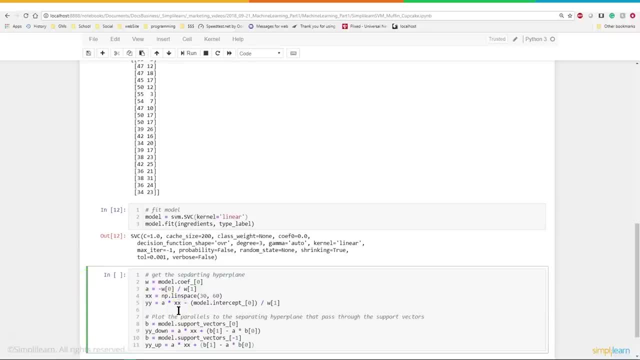 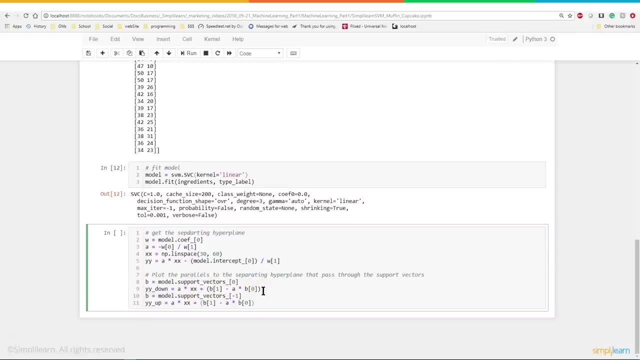 of these different arrays, And then what we want to do is we're going to take this and we're going to go ahead and plot it. So plot the parallels to separating hyperplane that pass through the support vectors, And so we're going to create 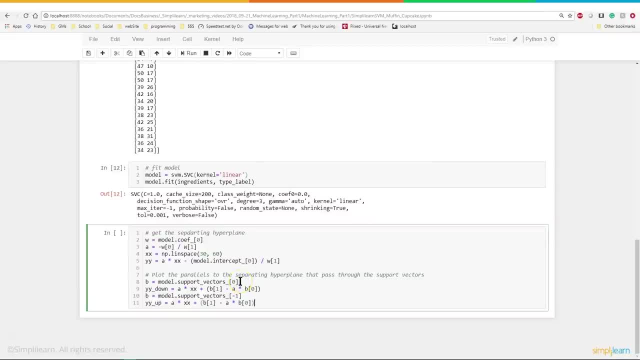 b equals a model support vectors. Pulling our support vectors out there, Here's our yy, which we now know is a set of data And we have We're going to create. yy down equals a times xx plus b1 minus a times b0. 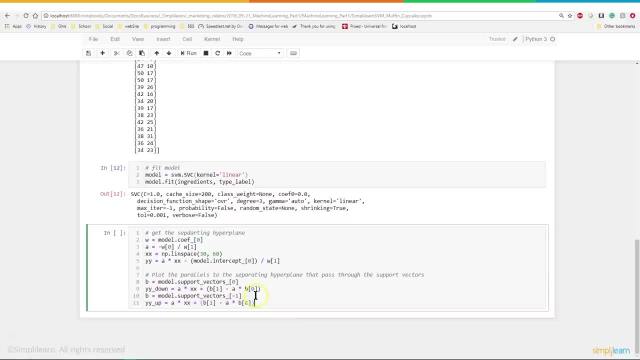 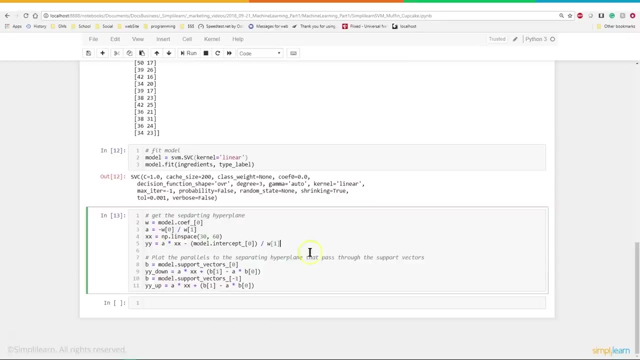 And then model support vector b is going to be. Set that to a new value and yy up equals a times xx plus b1 minus a times b0. And we can go ahead and just run this to load these variables up. If you wanted to understand. 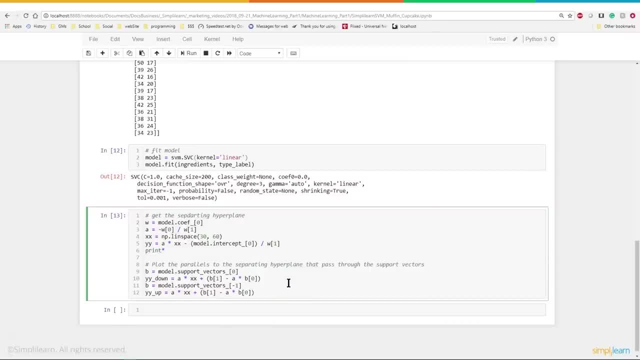 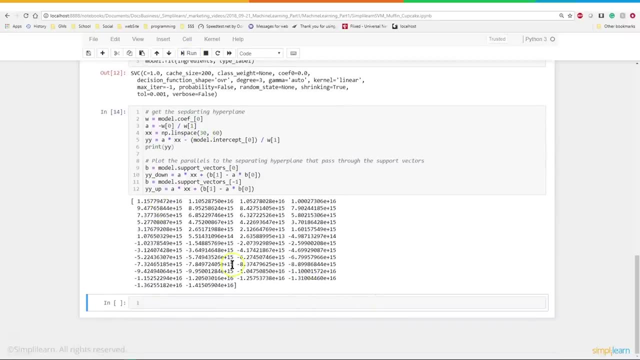 a little bit more of what's going on. you can see if we print yy, we just run that. you can see it's an array. This is a line It's going to have, in this case between 30 and 60.. 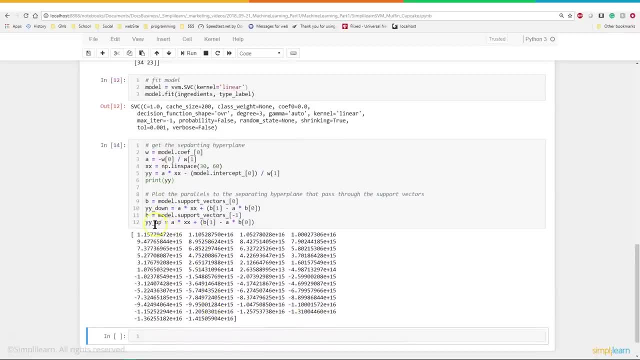 So it's going to be 30 variables in here And the same thing with yy up, yy down, And we'll plot those in just a minute on a graph so you can see what those look like. I'll just go ahead and delete that out of here. 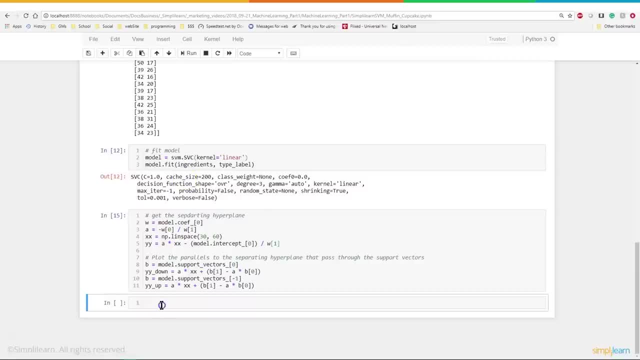 And run that so it loads up the variables. Nice, clean slate. I'm just going to copy this from before. Remember this: our sns, our seaborn plot, lm plot: flowers, sugar. And I'll just go ahead and run that real quick so you can see. 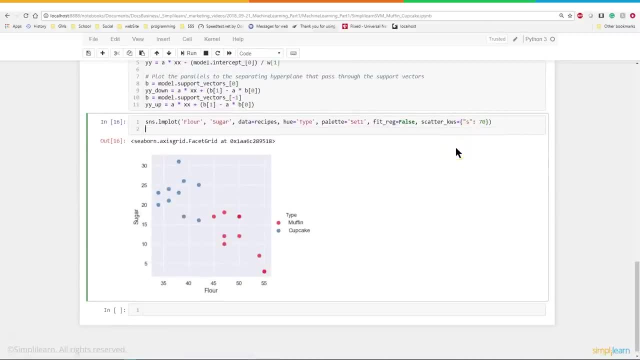 what that looks like. Let's run that on there. And then one of the neat things is, because seaborn sits on top of pyplot, we can do the pyplot for the line going through And that is simply pltplot And that's our xx. 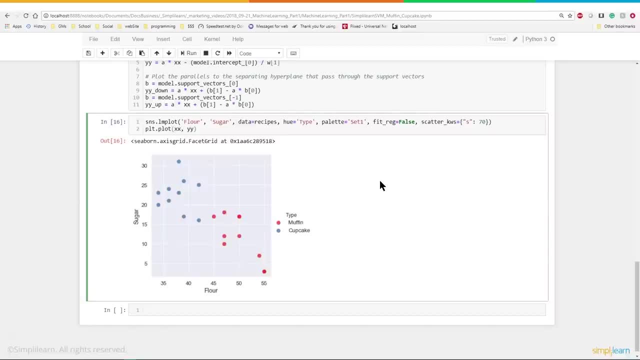 and yy, our two corresponding values, xy. And then somebody played with this to figure out that the line width equals 2 and the color black would look nice. So let's go ahead and run this whole thing with the pyplot on there And you can see when we do this. 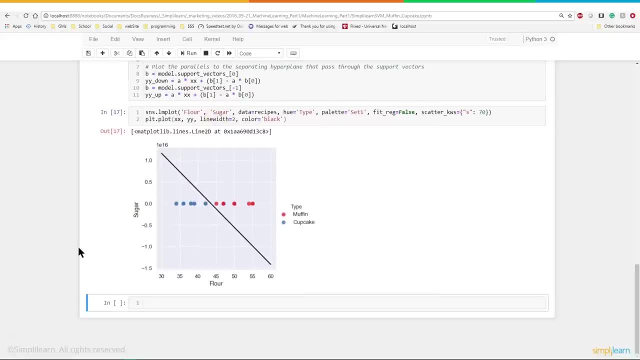 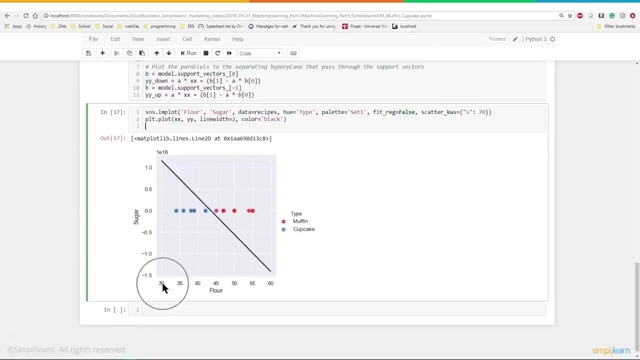 it's just doing flour and sugar on here, Corresponding line between the sugar and the flour and the muffin versus cupcake, And then we generated the support vectors, the yy down and yy out. So let's take a look and see what that looks like. 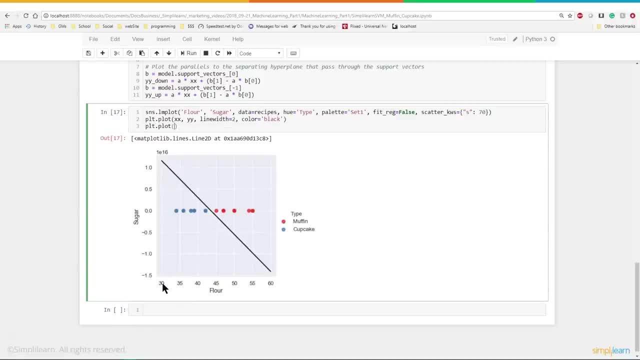 So we'll do our plplot, And again, this is all against xx, our x value. But this time we have yy down And let's do something a little fun with this. We can put in a k dash dash. That just tells it. 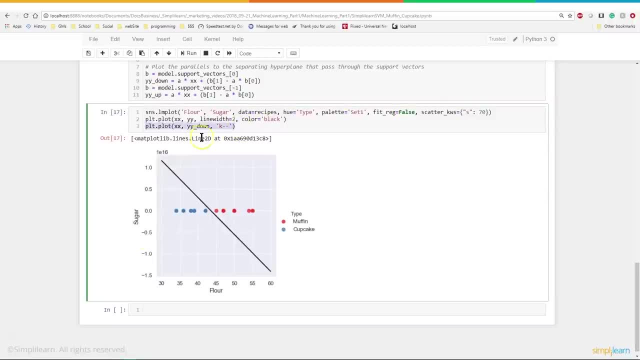 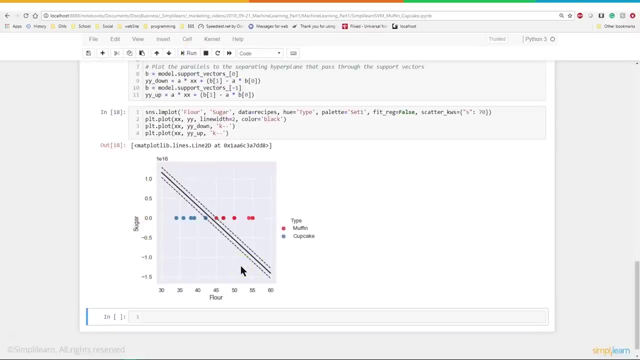 to make it a dotted line, And if we're going to do the down one, we also want to do the up one. So here's our yy up, And when we run that, it adds both sets of line, And so here's our support. 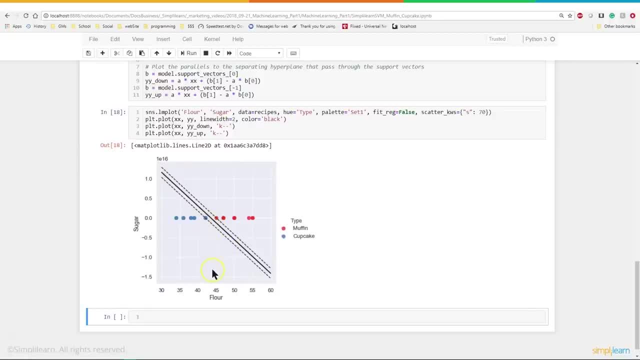 And this is what you expect. You expect these two lines to go through the nearest data point. So the dash lines go through the nearest muffin and the nearest cupcake when it's plotting it, And then your SVM goes right down the middle. 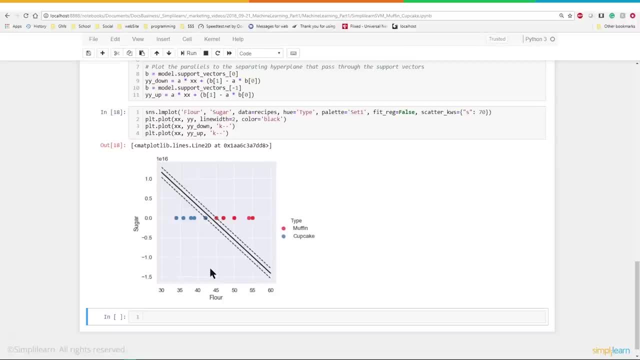 So it gives it a nice split in our data And you can see how easy it is to see, based just on sugar and flour, which one's a muffin or a cupcake. Let's go ahead and create a function to predict muffin or cupcake. 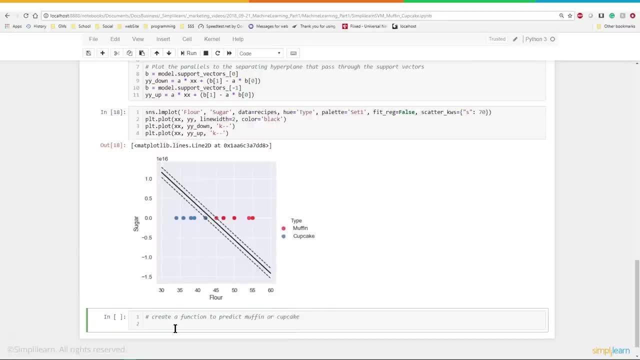 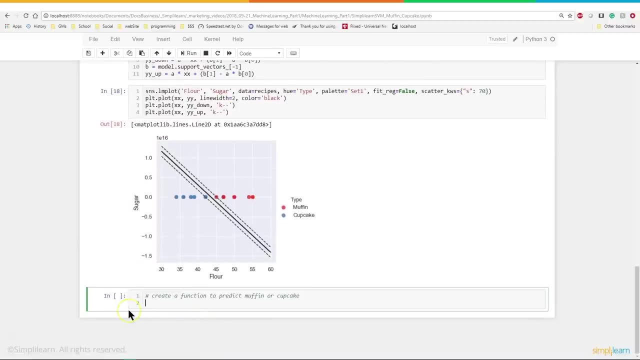 Muffin or cupcake. I've got my recipes. I pulled off the internet and I want to see the difference between a muffin or a cupcake, And so we need a function to push that through And create a function with def. 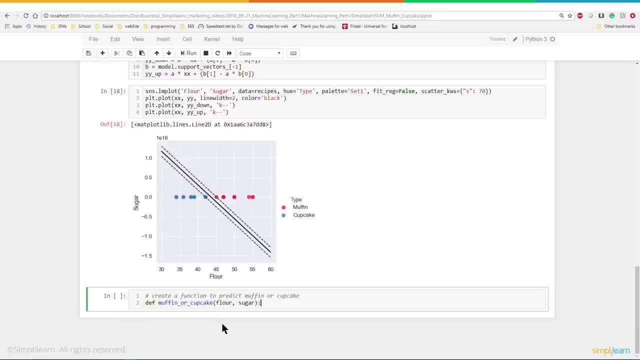 And let's call it muffin or cupcake. And remember we're just doing flour and sugar today, We're not doing all the ingredients, And that actually is a pretty good split. You really don't need all the ingredients to know the difference between flour and sugar. 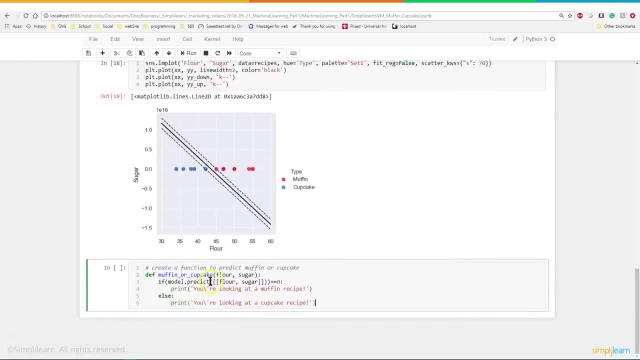 And let's go ahead and do an if-else statement. So if model predict is of flour and sugar equals zero, So we take our model and we run a predict. It's very common in sklearn where you have a dot predict, You put the data in. 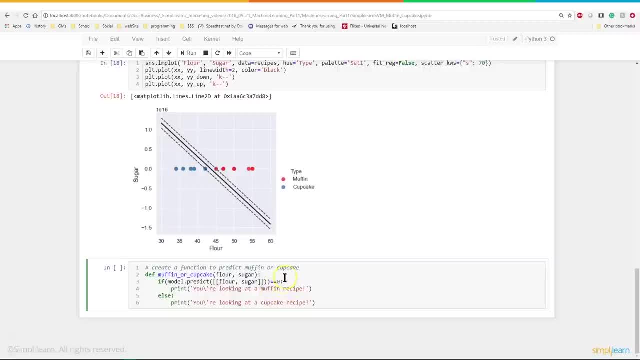 and it's going to return a value. In this case, if it equals zero, then you're looking at a muffin recipe. Else, if it's not zero, that means it's one, then you're looking at a cupcake recipe. 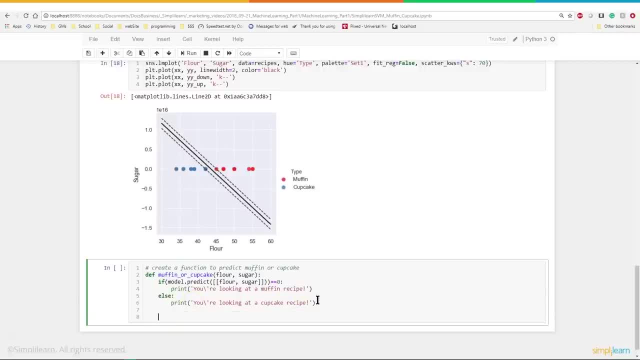 That's pretty straightforward for a function, or def for definition. D-E-F is how you do that in Python, And of course, if you're going to create a function, you should run something in it, And so let's run a cupcake. 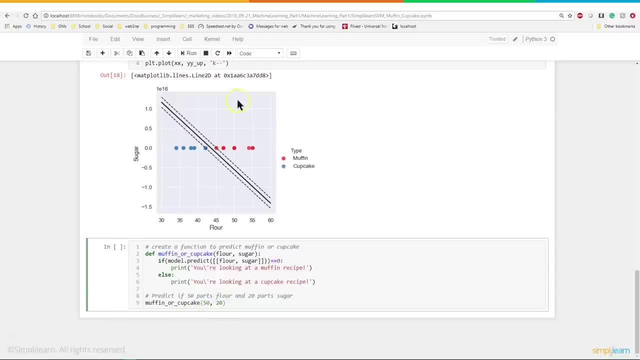 and we're going to send it. values 50 and 20.. A muffin or a cupcake? I don't know what it is. And let's run this and just see what it gives us And it says: oh, it's a muffin. 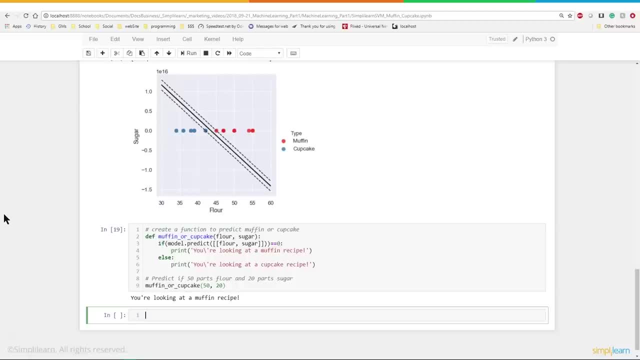 You're looking at a muffin recipe, So it very easily predicts whether we're looking at a muffin or a cupcake recipe. Let's plot this on the graph so we can see what that actually looks like, And I'm just going to copy it. 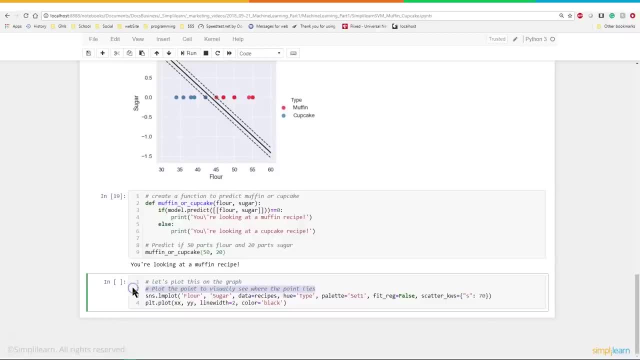 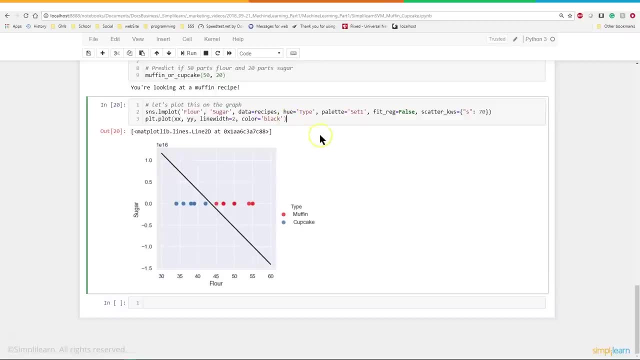 and paste it from below, where we're plotting all the points in there. So this is nothing different than what we did before. If I run it, you'll see it has all the points and the lines on there. What we want to do is we want to add another point. 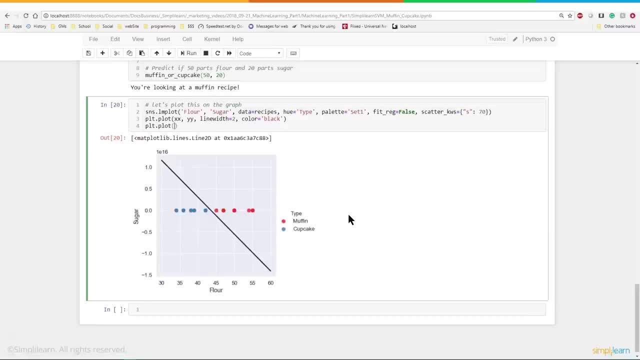 And we'll do pltplot And if I remember correctly we did for our test, we did 50 and 20.. And then we're going to, and then somebody went in here and decided we'll do a YO for yellow, or it's kind of an orangeish yellow color. 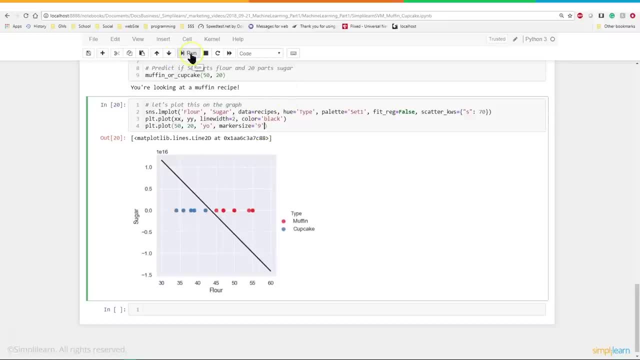 that's going to come up, Marker size 9.. Those are settings you can play with. Somebody else played with them to come up with the right setup. so it looks good And you can see there it is graphed clearly- a muffin. 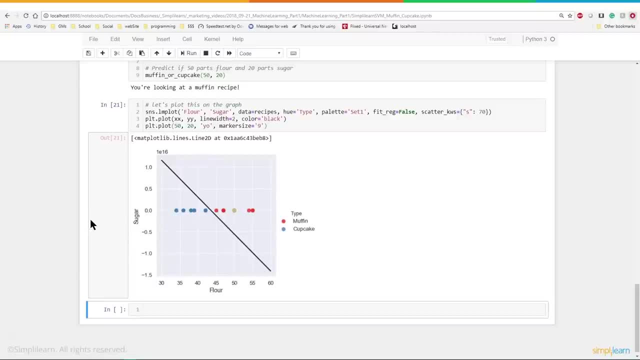 In this case, in cupcakes versus muffins, the muffin has won, And if you'd like to do your own muffin cupcake contender series, you certainly can send a note down below and the team at Simply Learn will send you over the data they use. 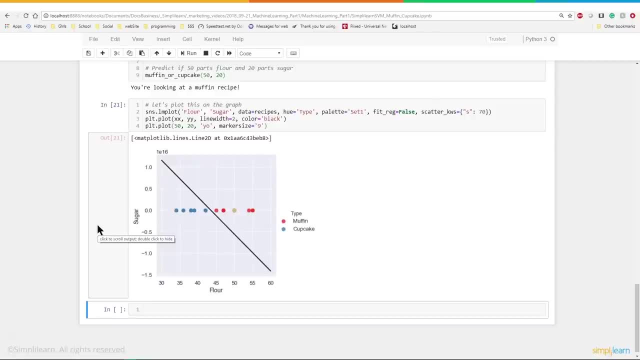 for the muffin and cupcake, And that's true of any of the data. We didn't actually run a plot on it. earlier We had men versus women. You can also request that information to run it on your data setup so you can test that out. 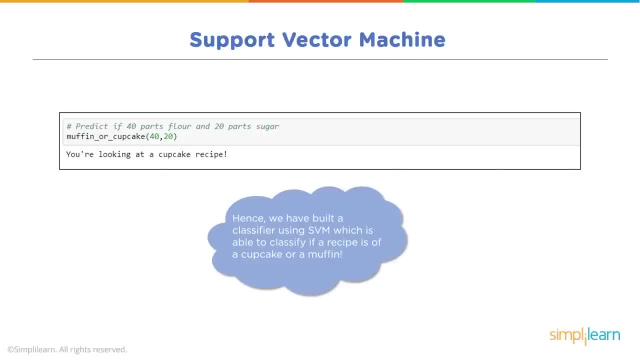 So to go back over our setup, we went ahead. for our support vector machine code, We did a predict: 40 parts flour, 20 parts sugar. It was different than the one we did, whether it's a muffin or a cupcake. 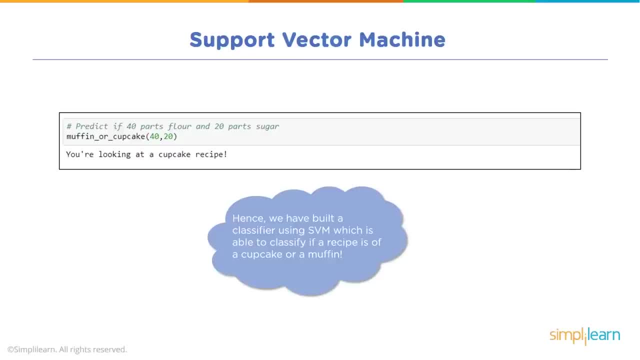 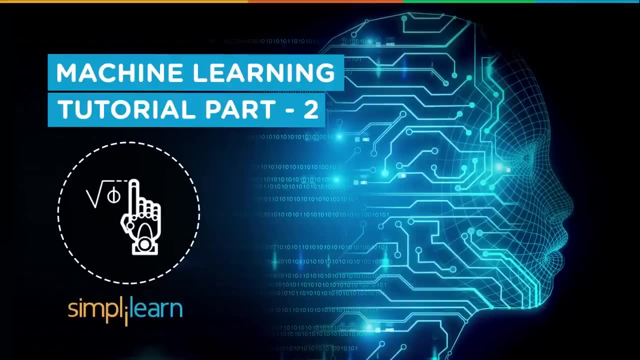 Hence we have built a classifier using SVM, which is able to classify if a recipe is of a cupcake or a muffin Which wraps up our cupcake versus muffin. Welcome to Machine Learning Tutorial Part 2.. My name is Richard Kirshner. 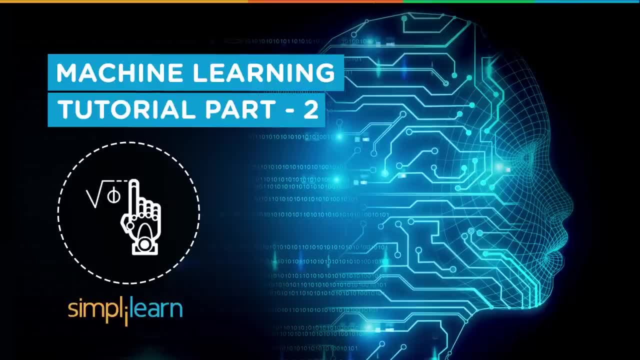 with the Simply Learn team That is, wwwsimplylearncom. Get certified, Get ahead. Today in our second tutorial, we're going to cover K-Means and linear regression, along with going over the quiz questions we had during our first tutorial. 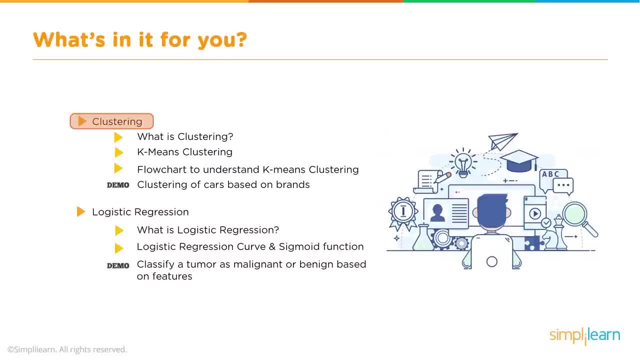 What's in it for you? We're going to cover clustering. What is clustering? K-Means clustering, which is one of the most common used clustering tools out there, Including a flow chart to understand K-Means clustering and how it functions. 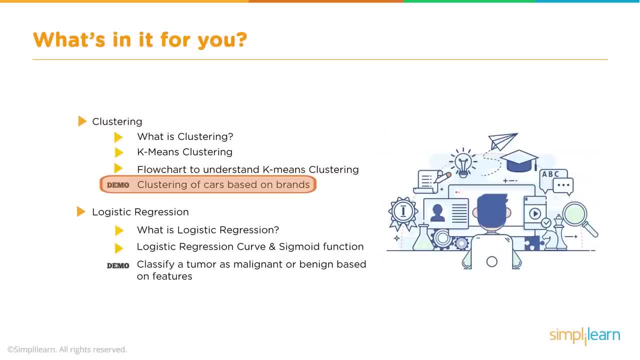 And then we'll do an actual Python live demo on clustering of cars based on brands. Then we're going to cover logistic regression. What is logistic regression? Logistic regression is the regression curve in sigmoid function. And then we'll do another Python code demo. 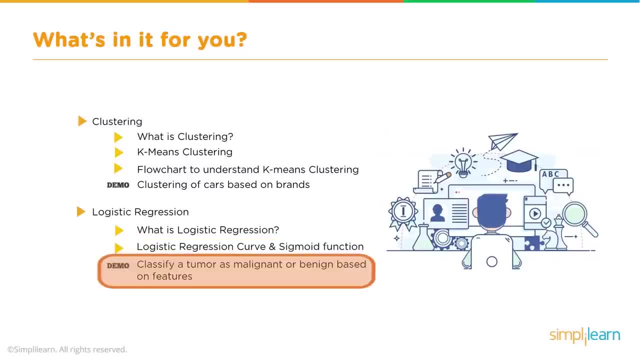 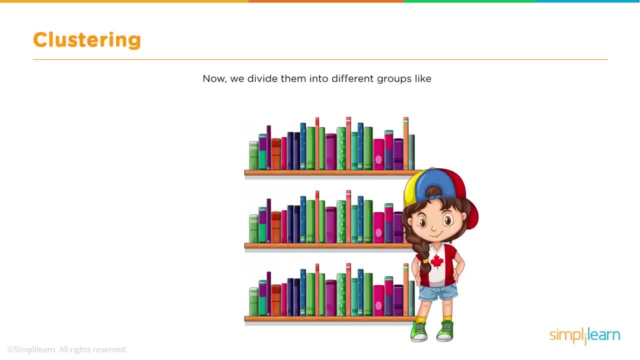 to classify a tumor as malignant or benign based on features. And let's start with clustering. Suppose we have a pile of books of different genres. Now we divide them into different groups, like fiction, horror, education And, as we can see from this young lady, 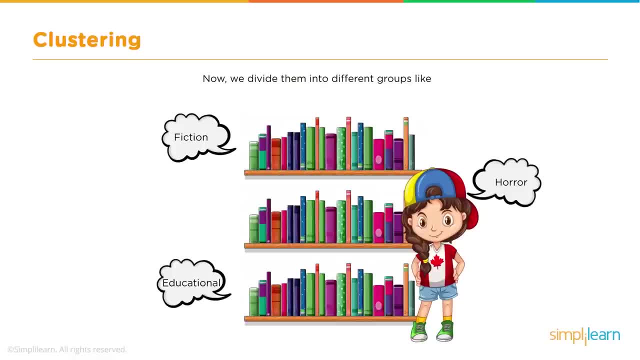 she definitely is into heavy horror. You can just tell by those eyes and the maple Canadian leaf on her shirt. But we have fiction, horror and education And we want to go ahead and divide them and divide our books up. Well, organizing objects into groups. 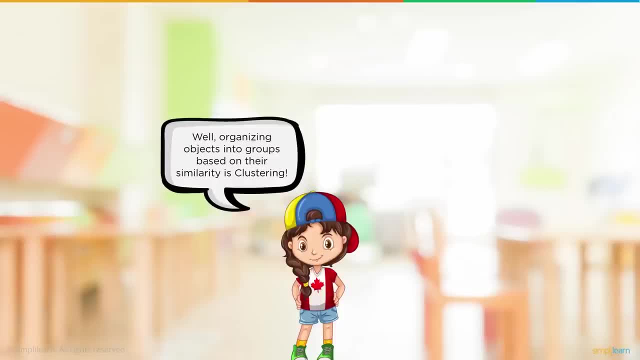 based on similarity is clustering, And in this case, as we're looking at the books, we're talking about clustering things with known categories, But you can also use it to explore data, So you might not know the categories. you just know that you need to divide it up. 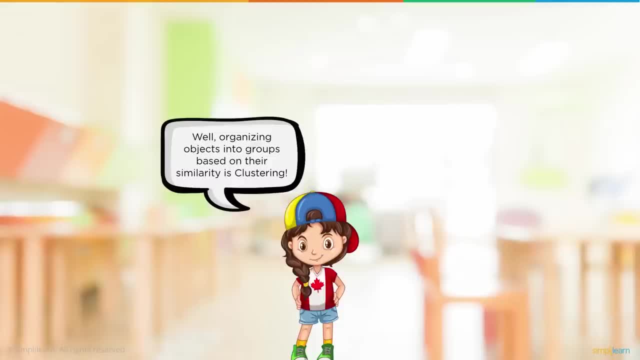 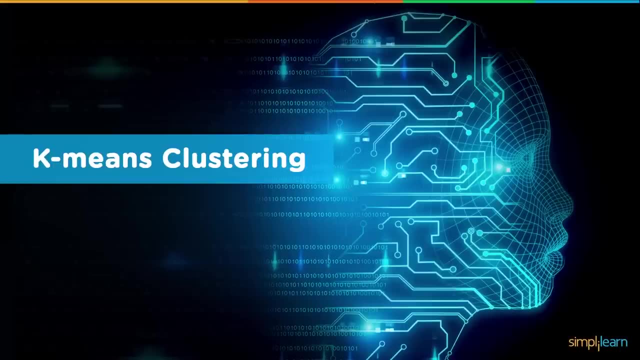 in some way to conquer the data and to organize it better. But in this case we're going to be looking at clustering in specific categories And let's just take a deeper look at that. We're going to use K-Means clustering. 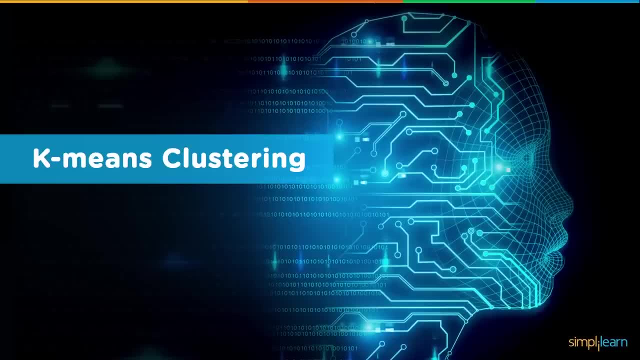 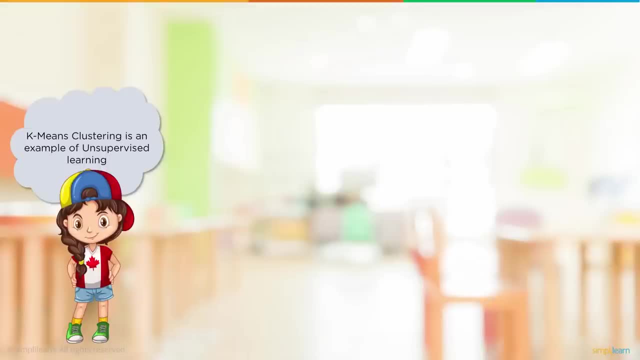 K-Means clustering is probably the most commonly used clustering tool in the machine learning library. K-Means clustering is an example of unsupervised learning. If you remember from our previous thing, it is used when you have unlabeled data. 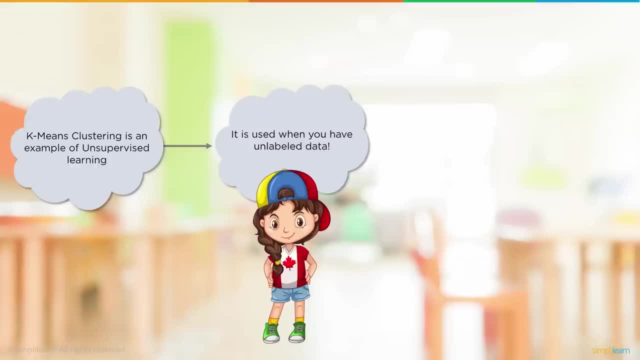 So we don't know the answer yet. We have a bunch of data that we want to cluster into different groups, Define clusters in the data based on feature similarity, So we've introduced a couple terms here. We've already talked about unsupervised learning. 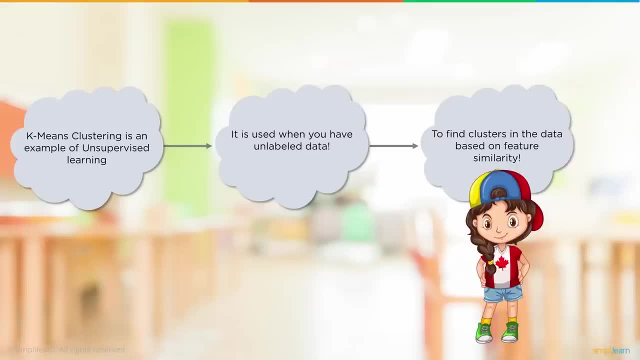 and unlabeled data. We don't know the answer yet. We're just going to group stuff together and see if we can find an unanswer of how things connect. We've also introduced feature similarity, Features being different features of the data. Now, with books, we can easily see fiction. 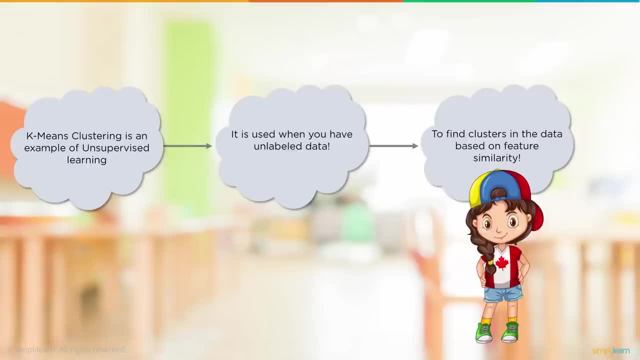 and horror and history books, But a lot of times, with data, some of that information isn't so easy to see right when we first look at it, And so K-Means is one of those tools where we can start finding things that connect that match with each other. 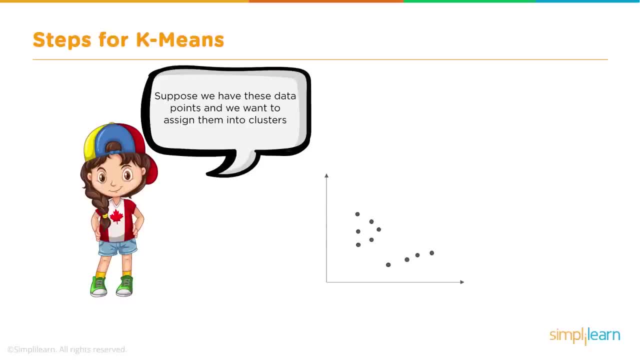 Suppose we have these data points that go into a cluster. Now when I look at these data points I would probably group them into two clusters. just by looking at them I'd say two of these groups of data kind of come together. But in K-Means we pick K clusters. 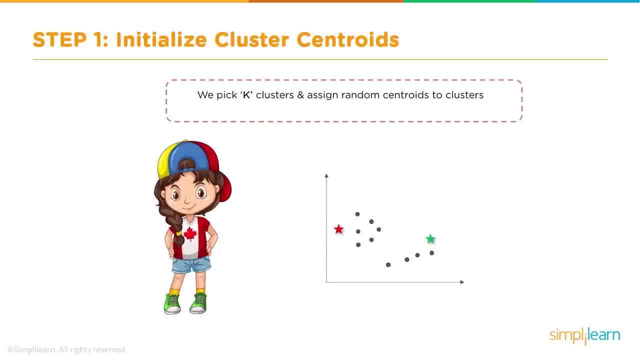 and assign random centroids to clusters Where the K clusters represents two different clusters. We pick K clusters and assign random centroids to the clusters. Then we compute distance from objects to the centroids. Now we form new clusters based on the number of centroids, So we figure out what the best distance. 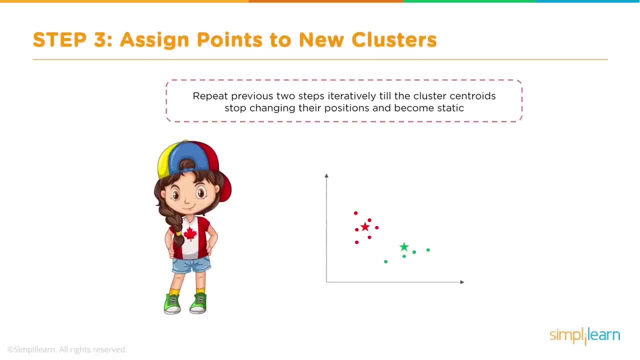 is for the centroid. then we move the centroid and recalculate those distances. Repeat previous two steps iteratively till the cluster centroid. stop changing their positions and become static. Repeat previous two steps iteratively till the cluster centroid. stop changing and the positions become static. 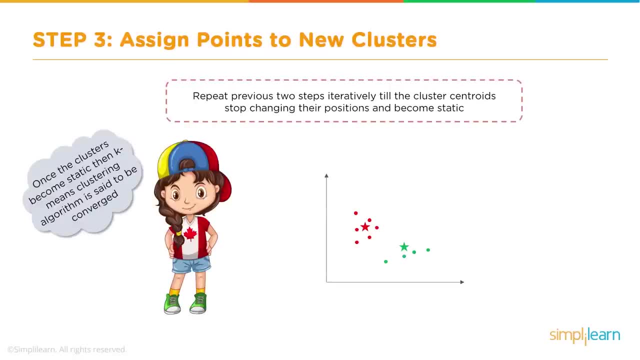 Once the clusters become static, then K-Means clustering algorithm is said to be converged, And there's another term we see throughout machine learning is converged. It's a term we're using to figure out the answer has come to a solution or it's converged on an answer. 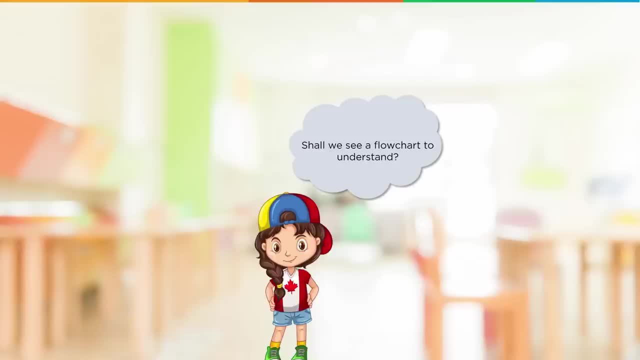 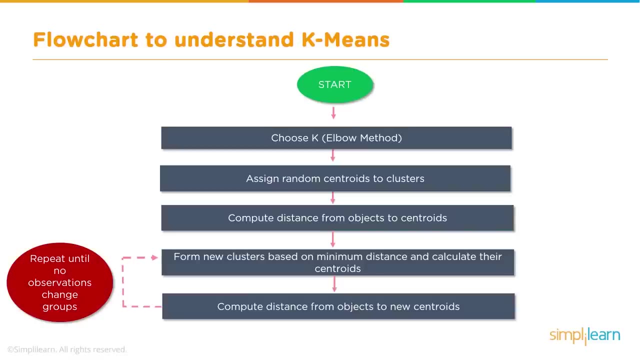 Shall we see the flow chart to understand, Make a little bit more sense by putting it into a nice easy step-by-step. So we start, we choose K. We'll look at the ELBO method in just a moment. We assign random centroids to clusters. 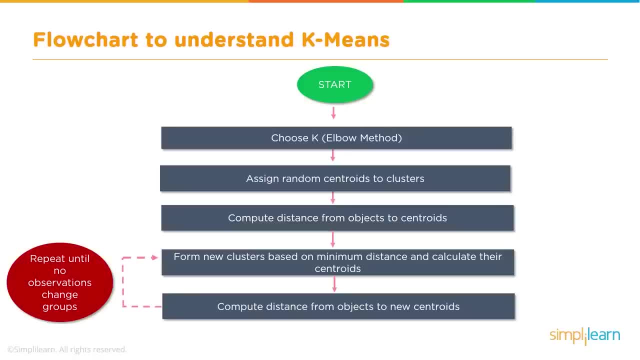 And sometimes you pick the centroids because you might look at the data in a graph and say, oh, these are probably the central points. Then we compute the distance from the objects to the centroids, We take that and we form new clusters based on minimum distance. 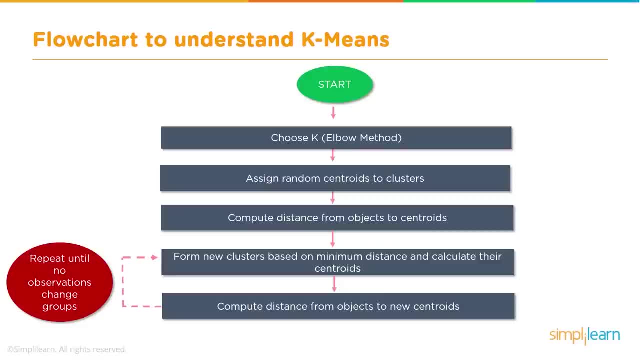 and calculate their centroids. Then we compute the distance from objects to the new centroids And then we go back and repeat those last two steps. We calculate the distances, So as we're doing it, it brings into the new centroid And then we move the centroid around. 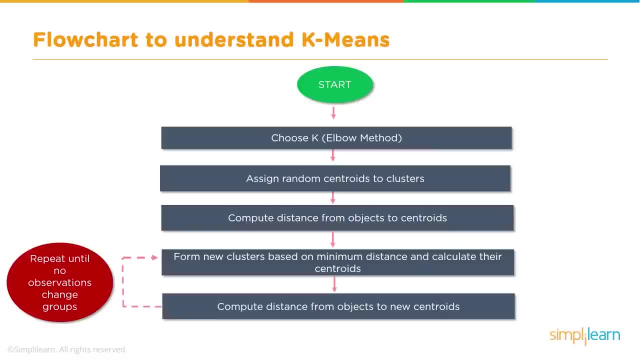 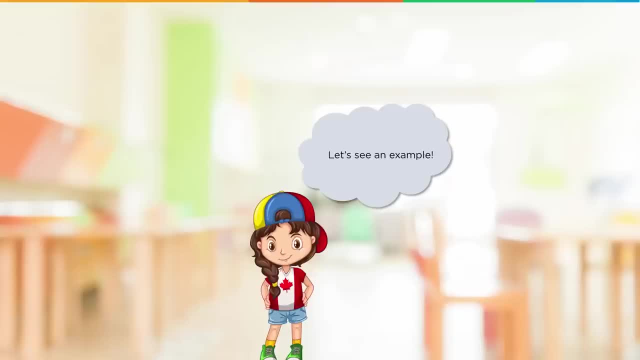 and we figure out what the best, which objects are closest to each centroid. So the objects can switch from one centroid to the other as the centroid are moved around And we continue that until it is converged. Here's an example of this. Suppose we have this data set. 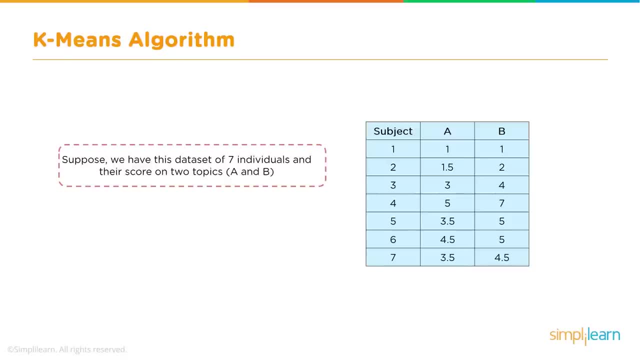 of seven individuals and their score on two topics, A and B. So here's our subject, in this case referring to the person taking the test, And then we have subject A, where we see what they've scored on their first subject, And we have subject B. 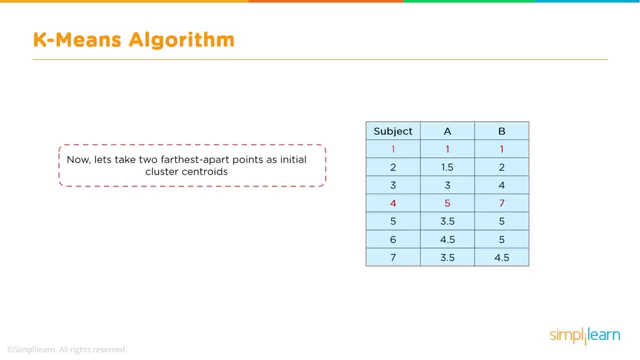 and we can see what they score. on the second subject Now let's take two farthest apart points as initial cluster centroids. Let's take the furthest one apart so they move together. Either one works okay, depending on what kind of data you're working on. 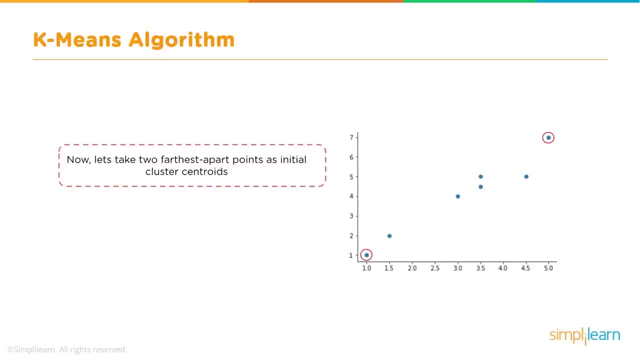 and what you know about it. So we took the two furthest points, one and one, and five and seven, And now let's take the two farthest apart points as initial cluster centroids. Each point is then assigned to the closest cluster with respect to the distance from the centroids. 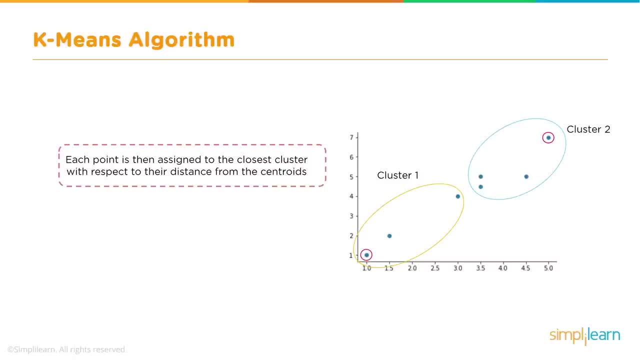 So we take each one of these points in there and we measure that distance And you can see that if we measure each of those distances we can get an equilibrium theorem for a triangle in this case, because you know the x and the y and you can figure out the diagonal line from that. 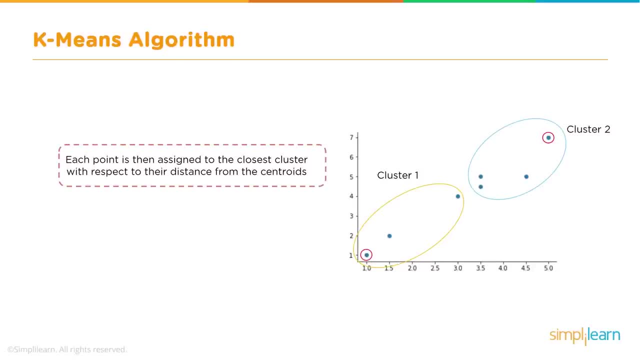 Or you can just take a ruler and put it on your monitor. That'd be kind of silly, but it would work. if you're just eyeballing it, You can see how they naturally come together in certain areas. Now we again calculate the centroids. 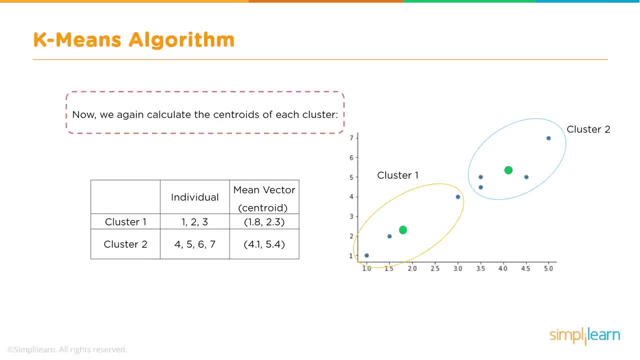 of each cluster, So cluster one and then cluster two, and we look at each individual dot. There's one, two, three. We're in one cluster, One point eight, comma two point three. So remember it was that one and one. Well, the very center of the data we're looking at. 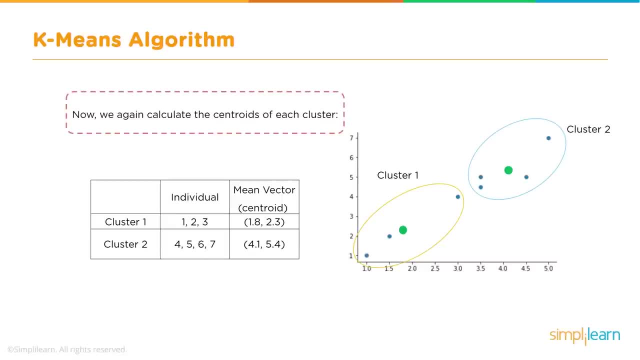 would put it at the one point roughly two, two, But one point eight and two point three And the second one, if we wanted to make the overall mean vector the average vector of all the different distances to that centroid we come up with. 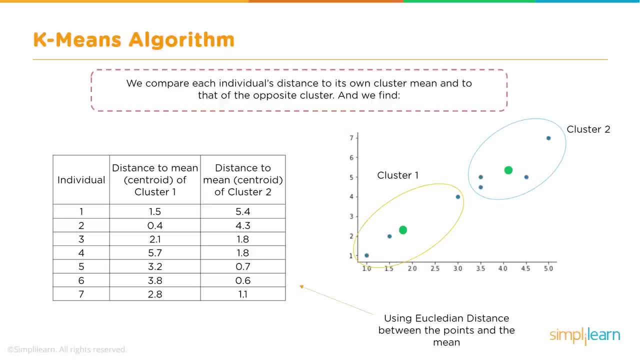 four comma one and five four. So we've now moved the centroids. We compare each individual's distance to its own cluster mean and to that of the opposite cluster And we find build a nice chart on here as we move the centroid around. 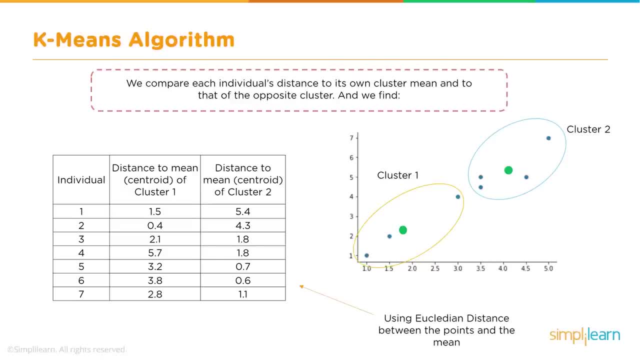 we now have a new, different kind of clustering of groups And using Euclidean distance between the points and the mean, we get the same formula. You see new formulas coming up. So we have our individual dots: distance to the mean centroid of the cluster. 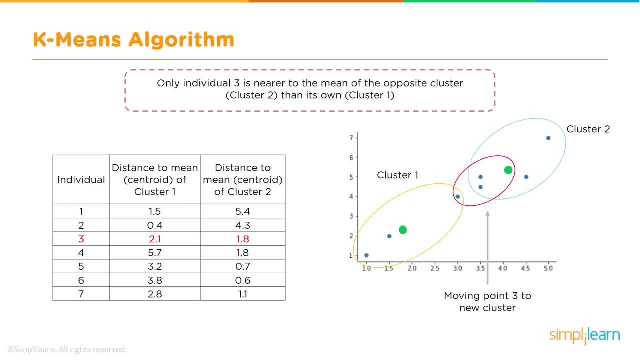 and distance to the mean centroid of the cluster. Only individual three is nearer to the mean of the opposite cluster, cluster two, than its own cluster one, And you can see here in the diagram where we've kind of circled that one in the middle. 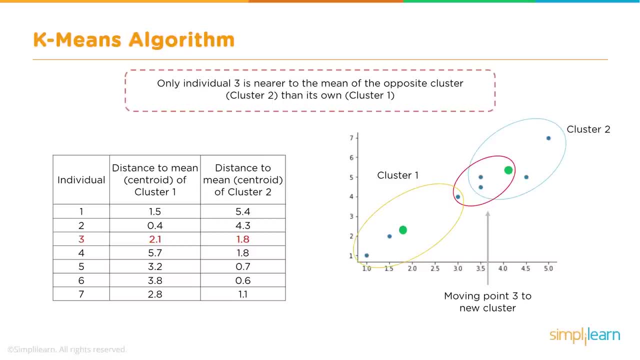 So when we've moved the centroid over, one of the points shifted to the other cluster because it's closer to that group of individuals. Thus, individual three is relocated to cluster two, resulting in a new partition, And we regenerate all those numbers. 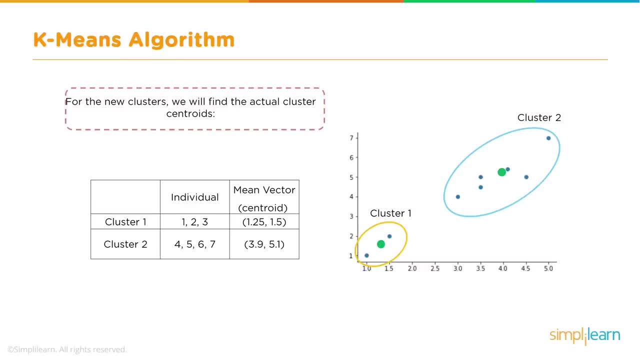 of how close they are to the different clusters. For the new clusters we will find the actual cluster centroids. So now we move the centroids over And you can see that we've now formed two very distinct clusters on here. On comparing the distance of each individual's 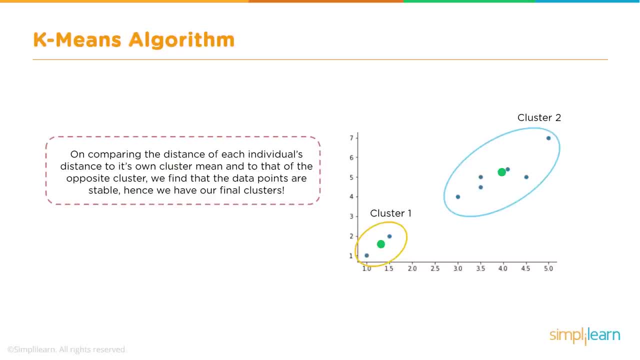 distance to its own cluster mean and to that of the opposite cluster, we find that the data points are stable. Hence we have our final clusters. Now, if you remember, I brought up a concept earlier on the k-means algorithm: Choosing the right value of k. 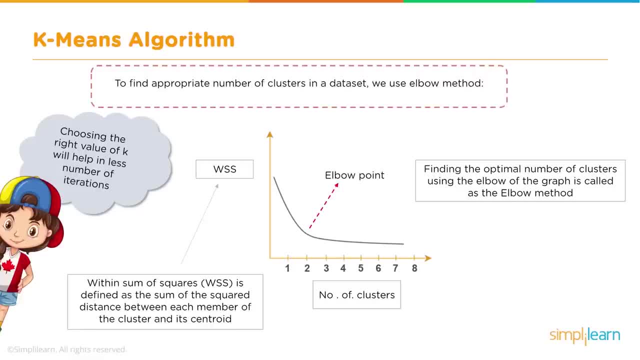 will help in less number of iterations And to find the appropriate number of clusters in a data set. we use the ELBO method And, within sum of squares, WSS is defined as the sum of the squared distance between each member of the cluster in its centroid. 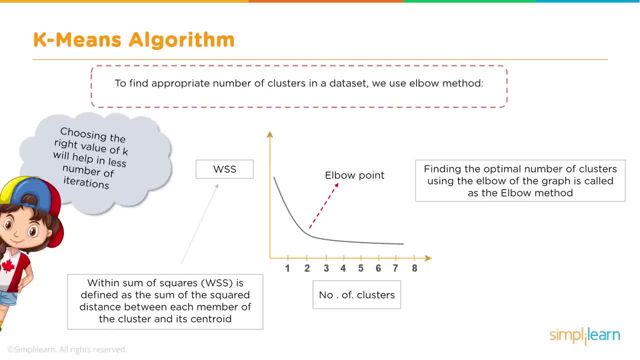 And so you see, what we've done here is we have the number of clusters and, as you do, the same k-means algorithm over the different clusters and you calculate what that centroid looks like and you find the optimal. you can actually find the optimal number of clusters using the ELBO. 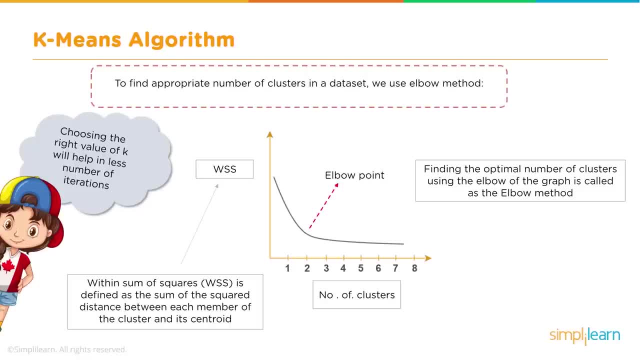 the graph is called as the ELBO method And on this we guessed at two just by looking at the data. But as you can see the slope, you actually just look for right there where the ELBO is in the slope and you have a clear answer. 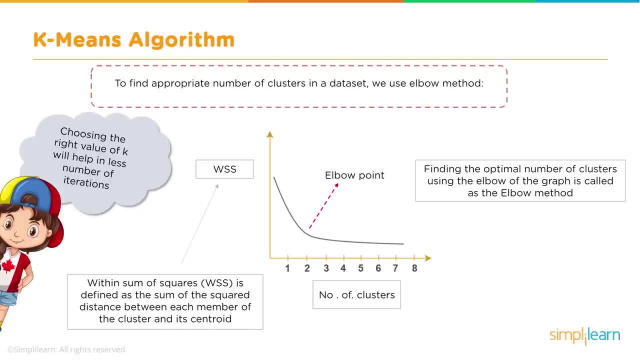 that we want two different to start with. k-means equals two, Three, four, five, until they find the value which fits on the ELBO joint. Sometimes you can just look at the data and if you're really good with that specific domain. 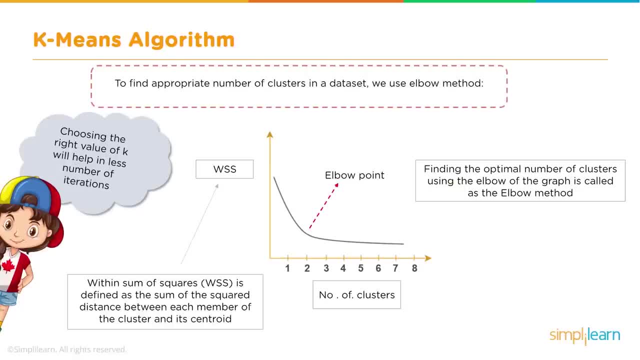 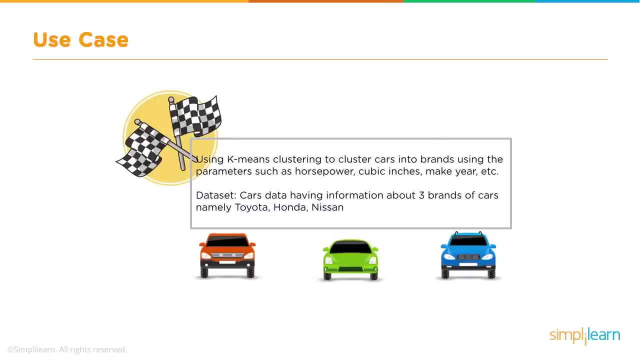 remember domain. I mentioned that last time. you'll know where to pick those numbers and where to start guessing at what that k-value is. So let's take this and we're going to use a use case using k-means clustering to cluster cars into brands. 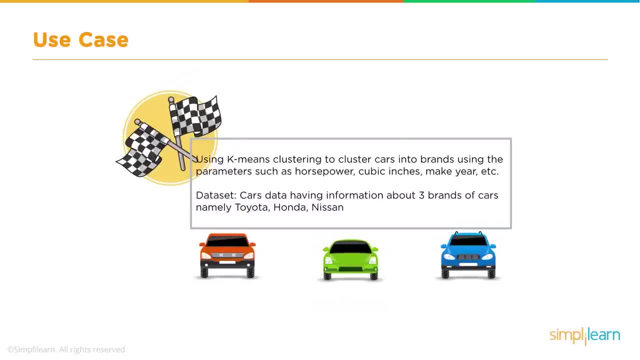 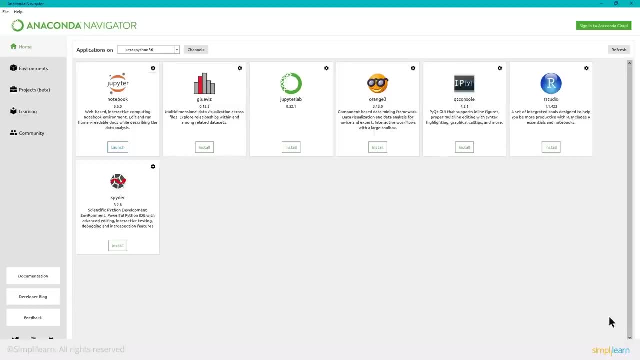 using parameters such as horsepower, and we're going to use the dataset cars data, having information about three brands of cars: Toyota, Honda and Nissan. We'll go back to my favorite tool, the Anaconda Navigator with the Jupyter Notebook, And let's go ahead and flip over. 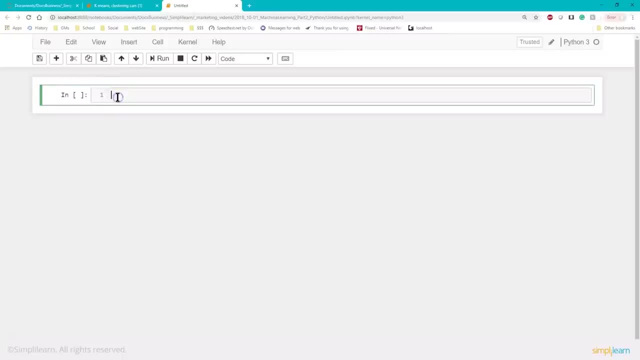 to our Jupyter Notebook And in our Jupyter Notebook I'm going to go ahead and just paste the basic code that we usually start a lot of these off with. We're not going to go too much into this code because we've already discussed NumPy. 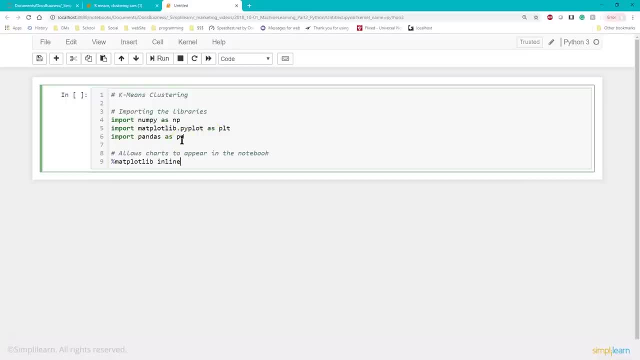 we've already discussed MatplotLibrary, Pandas being the number array, Pandas being the Pandas dataframe and Matplot for the graphing. And don't forget, since if you're using the Jupyter Notebook, you do need the MatplotLibrary inline, so that 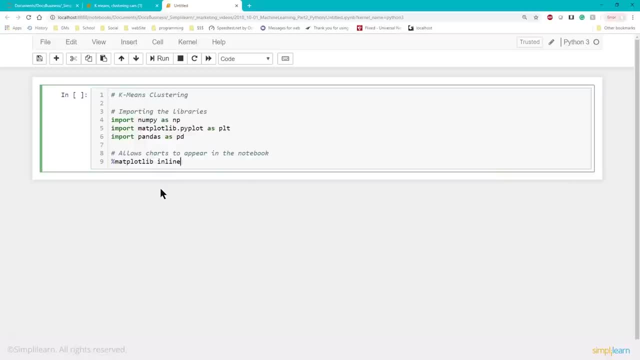 it plots everything on the screen. If you're using a different Python editor, then you probably don't need that, because it'll have a pop-up window on your computer And we'll go ahead and run this just to load our libraries and our setup into here. 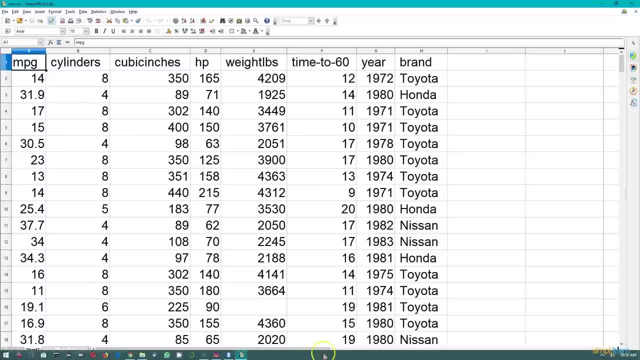 The next step is, of course, to look at our data, which I've already opened up in a spreadsheet, And you can see here we have the miles per gallon, cylinders, cubic inches, horsepower, weight, pounds, how heavy it is. time it takes. 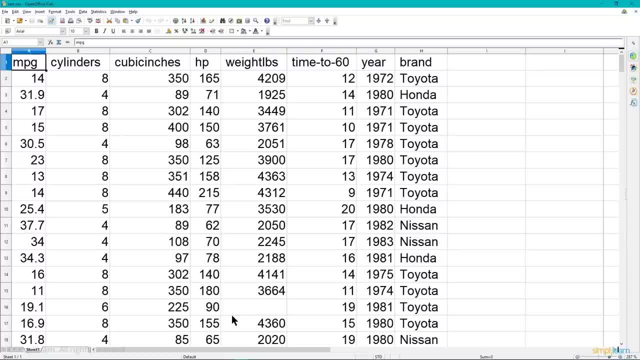 to get to 60. My card is probably on this one at about 80 or 90. What year it is? so this is. you can actually see this is kind of older cars. and then the brand Toyota, Honda, Nissan. 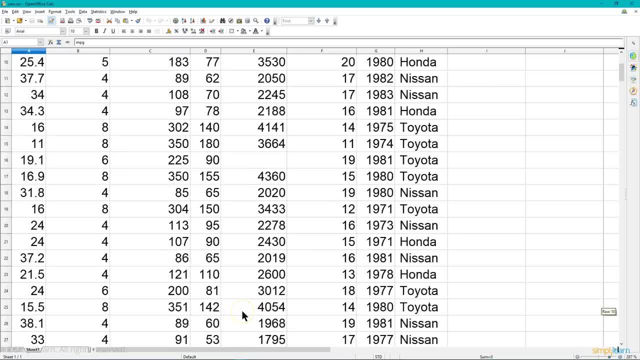 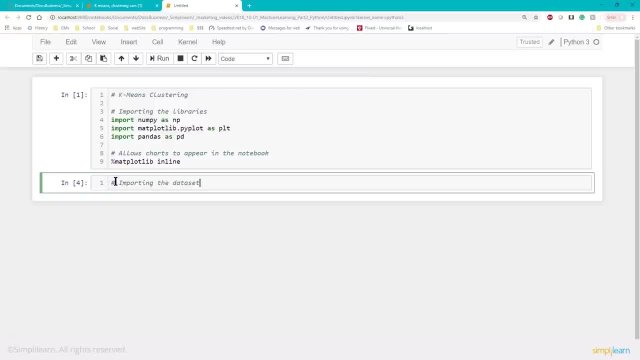 So the different cars are coming from all the way from 1971. if we scroll down to the 80s, We have, between the 70s and 80s, the number of cars that they've put out. And let's, when we come back here, 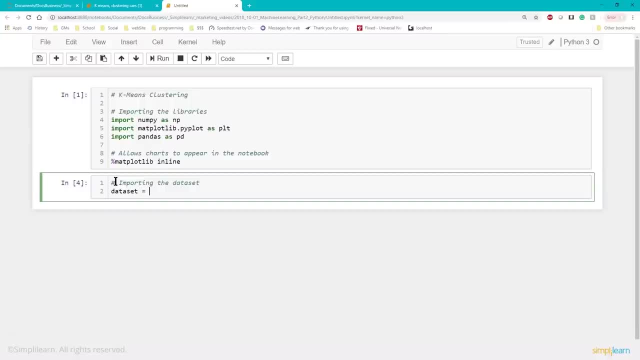 we're going to do importing the data, So we'll go ahead and do dataset equals And we'll use pandas to read this in. And it's from a CSV file. Remember, you can always post this in the comments and request the data files for these, Either in the comments. 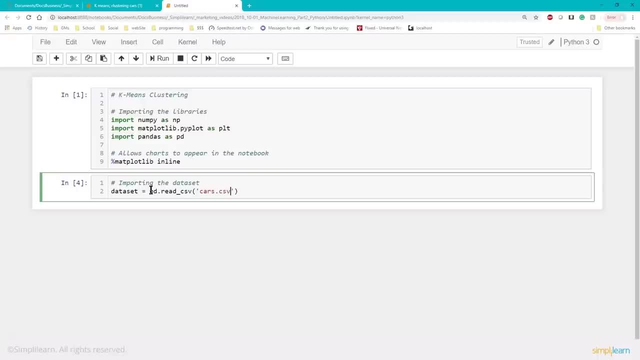 here on the YouTube video or go to simplylearncom and request that The car's CSV. I put it in the same folder as the code that I've stored. So my Python code is stored in the same folder, so I don't have to put the full path. 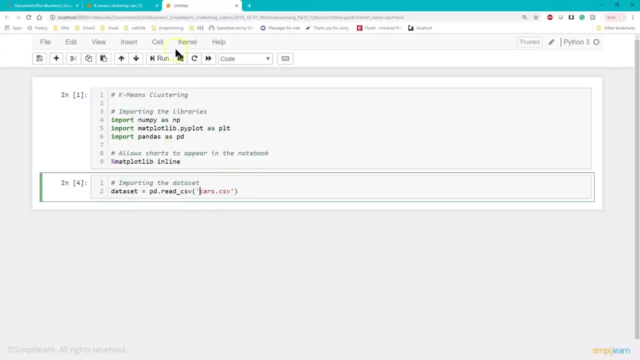 You can store them in different folders. You do have to change this and double check your name variables And we'll go ahead and run this. And we've chosen dataset arbitrarily because it's a dataset we're importing And we've now imported our car's CSV. 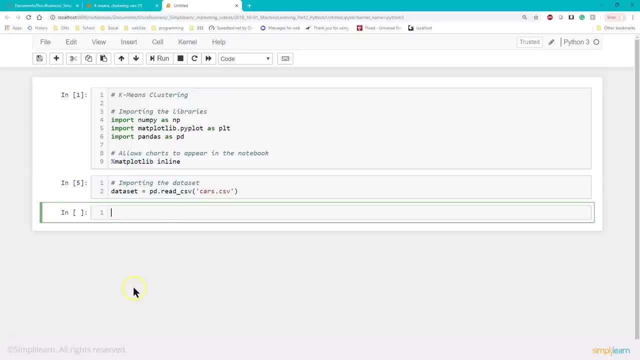 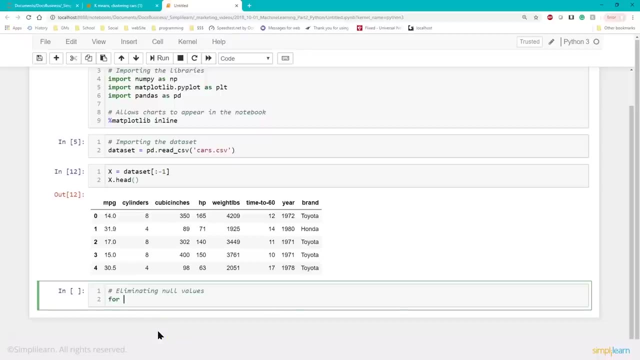 into the dataset. As you know, you have to prep the data, So we're going to create the xdata. This is the one that we're going to try to figure out what's going on with, And then there's a number of ways to do this. 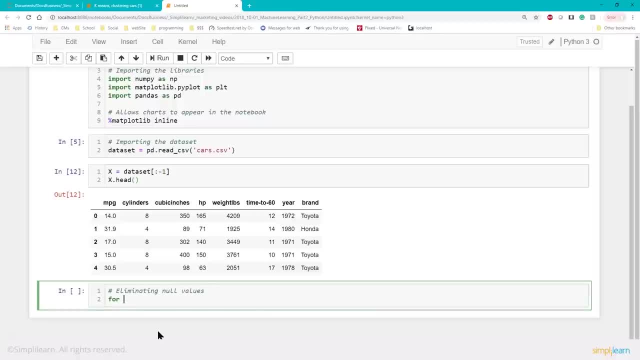 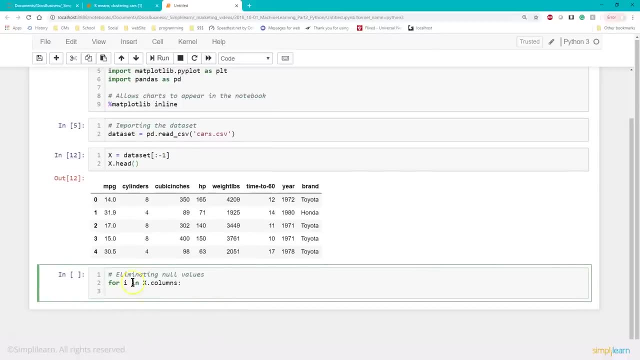 But we'll do it in a simple loop so you can actually see what's going on. So we're going to go through each of the columns And a lot of times it's important. I'll make lists of the columns and do this because I might remove. 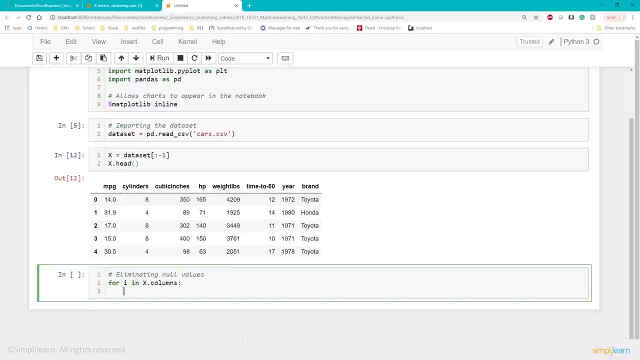 certain columns, Or there might be columns that I want to be processed differently. But for this we can go ahead and take x of i And we want to go fill na, And that's a pandas command. But the question is, what are we going? 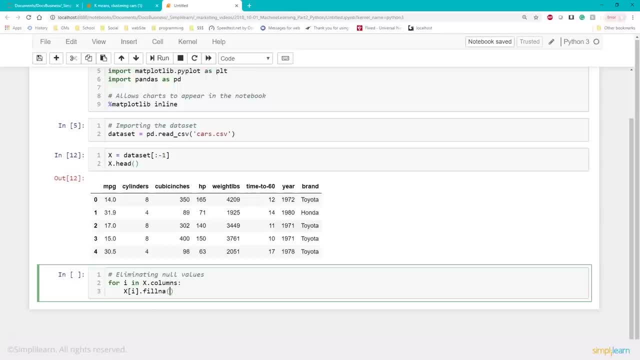 to fill the missing data with. We definitely don't want to just put in a number that doesn't actually have anything to actually mean something, And so one of the tricks you can do with this is we can take x of i And then, in addition to that, 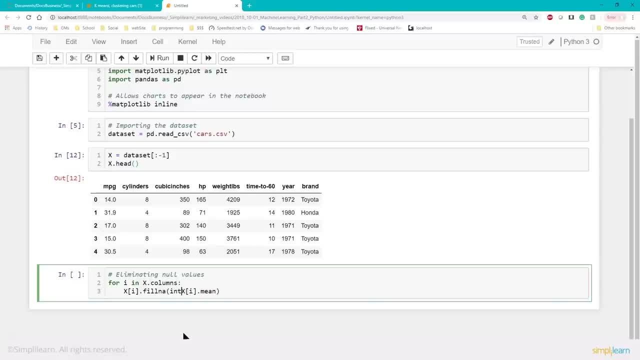 we want to go ahead and turn this into an integer, because a lot of these are integers, So we'll go ahead and keep it integers And we add the bracket here, And a lot of editors will do this. They'll think that you're closing one bracket. 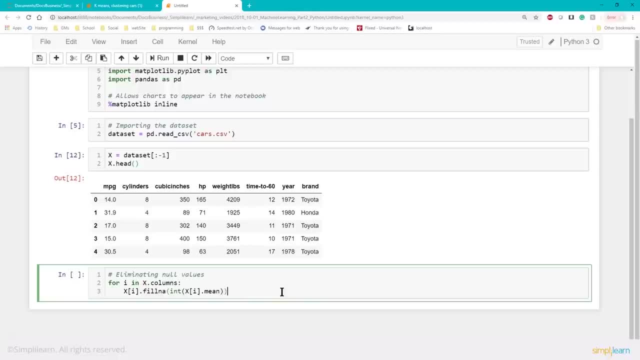 Make sure you get that second bracket in there. if it's a double bracket, That's always something that happens regularly. So once we have our integer of x of i, this is going to fill in any missing data, and I was so busy closing one set of brackets. 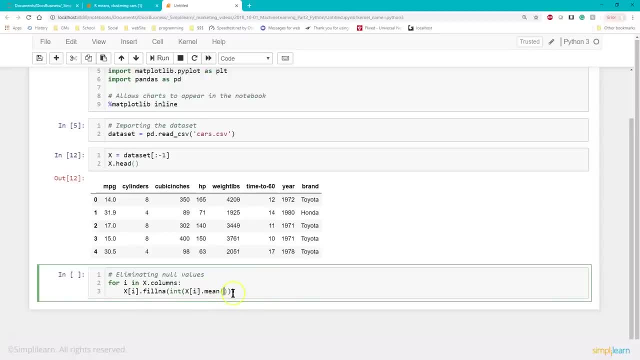 I forgot that the mean also has brackets in there for the pandas. So we can see here we're going to fill in all the data with the average value for that column. so if there's missing data it's in the average of the data it does have. 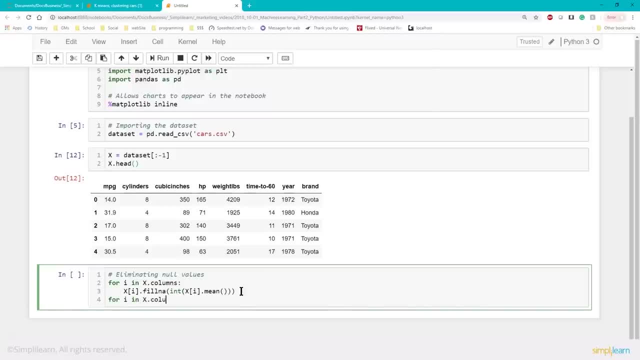 Then, once we've done that, we'll go ahead and loop through it again And just check and see to make sure everything is filled in correctly And we'll print. and then we take x is null And this returns a set of the null value. 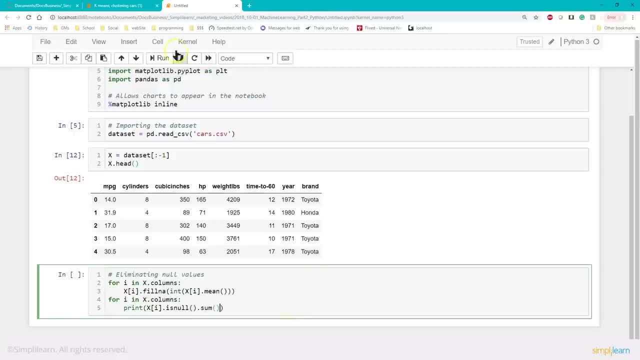 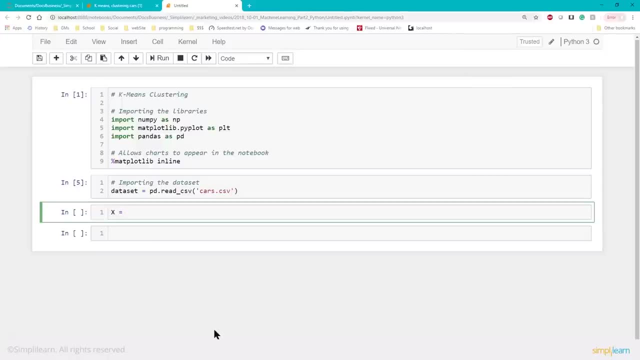 or how many lines are null, And we'll just sum that up to see what that looks like. And so when I run this and so with the x, what we want to do is we want to remove the last column because it had the models. 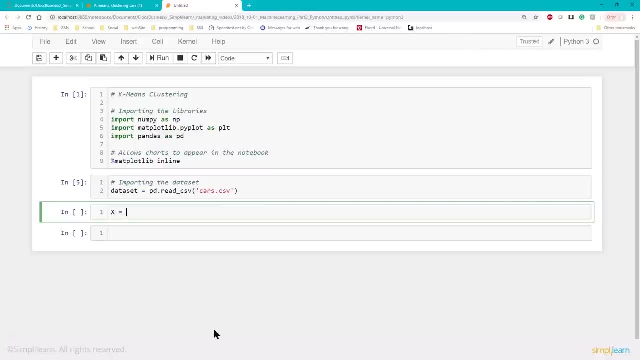 That's what we're trying to see: if we can cluster these things and figure out the models. There is so many different ways to sort the x out. For one, we could take the x and we could go dataset, our variable we're using. 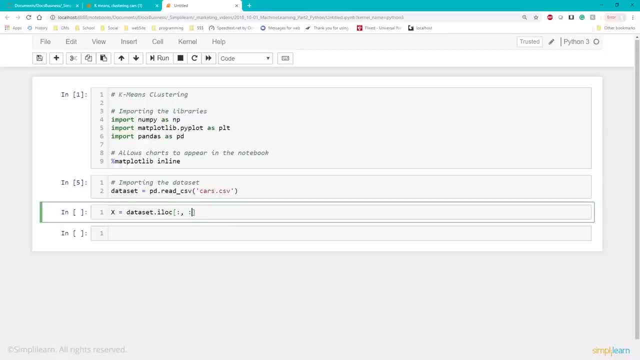 and use the i location all the rows and all but the last column of the dataset And at this time we could do values. We just convert it to values. So that's one way to do this, And if I just put this down here, 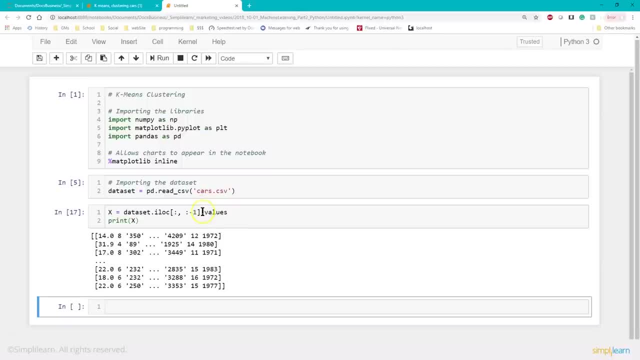 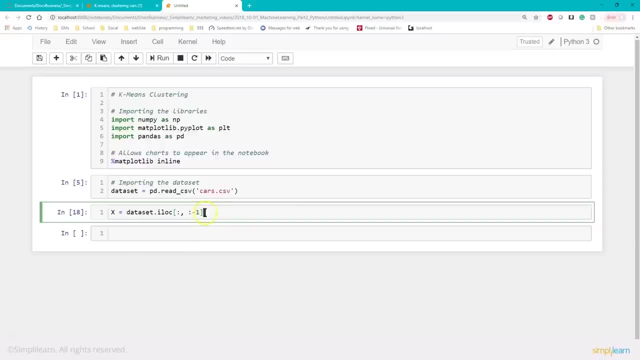 and print x and I run this. you can see it's just the values. We could also take out the values and it's not going to return anything because there's no values connected to it. What I like to do with this is, instead of doing the i location. 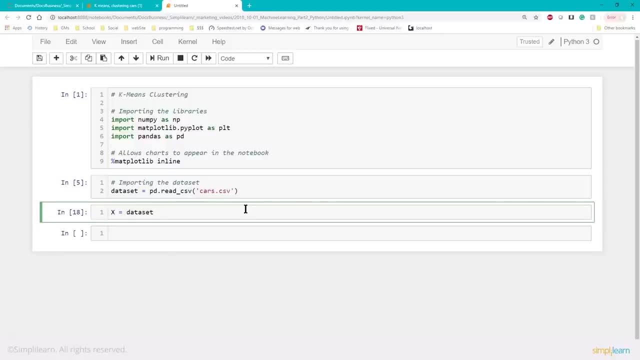 what I like to do is more common is to come in here and we have our dataset and we're going to do datasetcolumns and remember that lists all the columns. So if I come in here, let me just mark that as red and I print datasetcolumns. 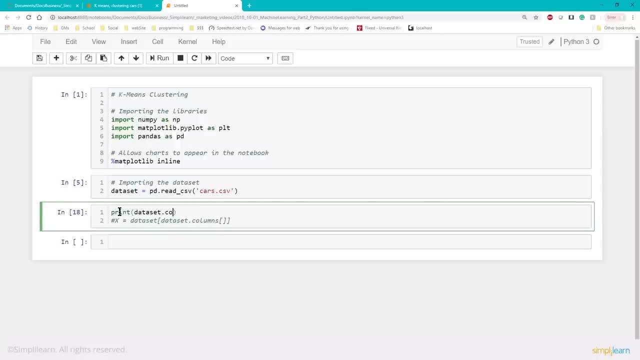 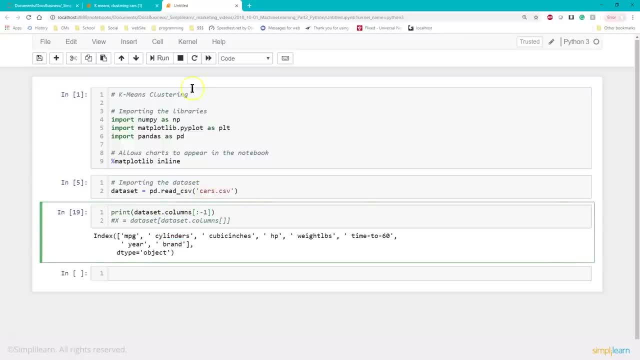 datasetcolumns of everything but the last one minus one. So now if I print this, you'll see the brand disappears. So I can actually just take datasetcolumns minus one and I'll put it right in here for the columns we're going to look at. 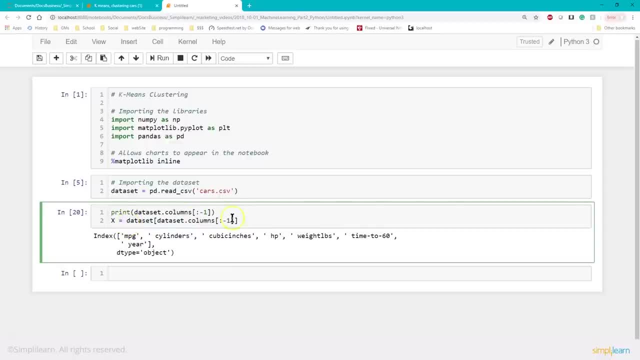 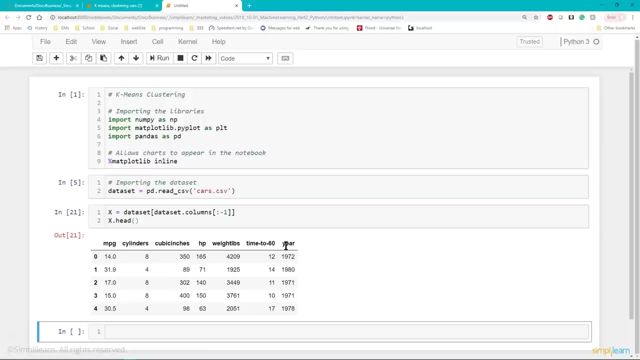 and let's unmark this, and unmark this, and unmark this, and now, if I do an xhead, I now have a new datasetcolumns data frame and you can see right here we have all the different columns except for the brand at the end of the year. 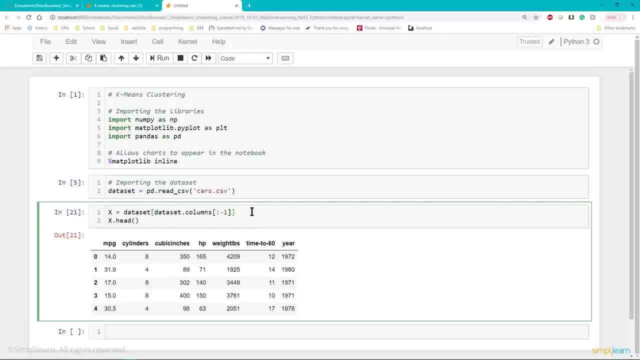 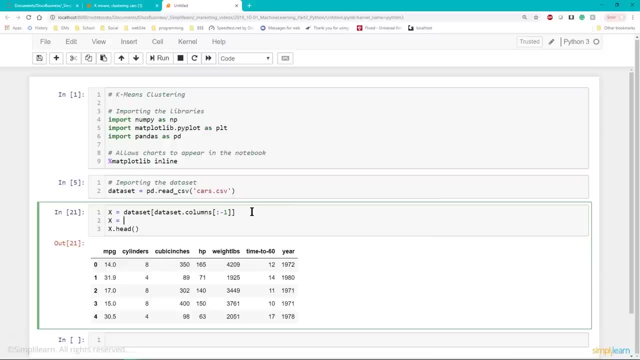 And it turns out when you start playing with the dataset, you're going to get an error later on and it'll say: cannot convert string to float value. and that's because for some reason, these things, the way they recorded them, must have been recorded as strings. 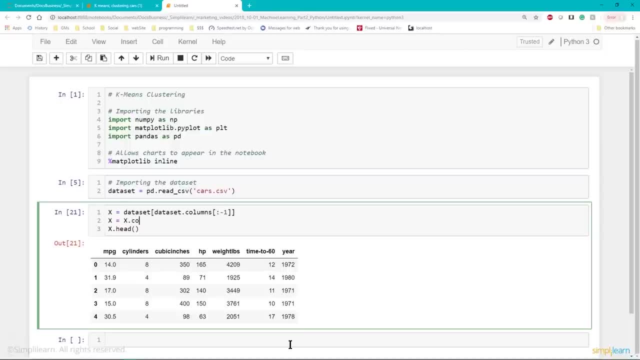 So we have a neat feature in here on pandas to convert and it is simply convert objects and for this we're going to do convert, convert underscore numeric. numeric equals true- and yes, I did have to go look that up, I don't have it memorized- the convert numeric. 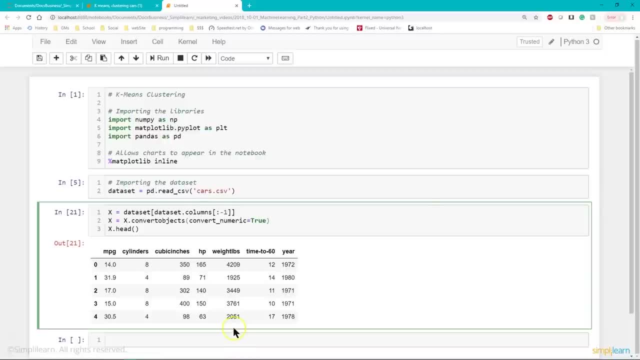 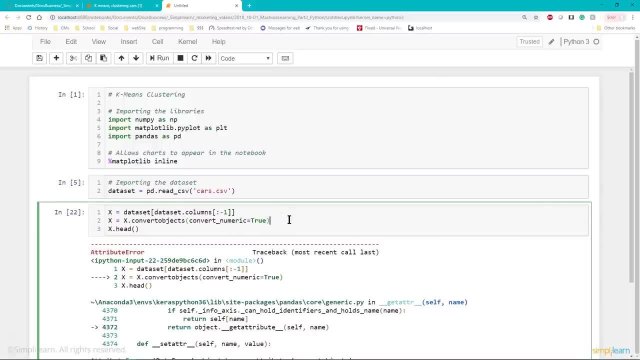 in there. If I'm working with a lot of these things, I remember them, but depending on where I'm at and what I'm doing, I usually have to look it up And we run that. oops, I must have missed something in here. let me double check my spelling. 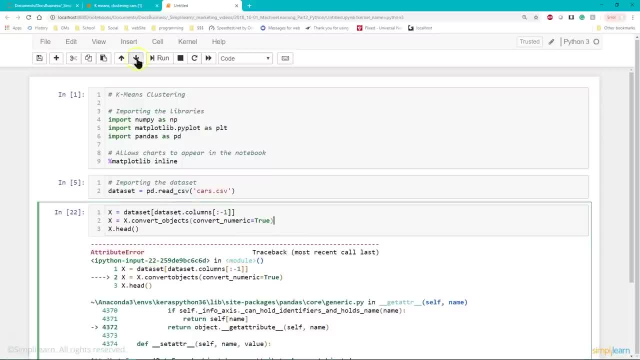 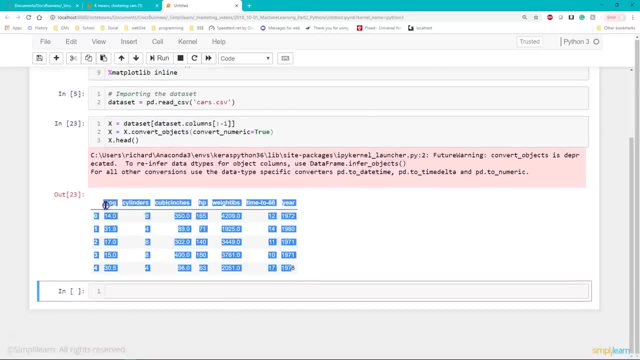 and when I double check my spelling, you'll see I missed the first underscore in the convert object. and when I run this, it now has everything converted into a numeric value, because that's what we're going to be working with, is numeric values down here And the next part. 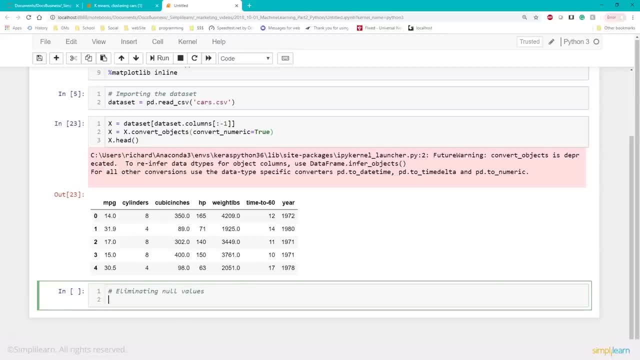 is that we need to go through the data and eliminate null values. Most people, when they're doing small amounts, working with small data pools, discover afterwards that they have a null value and they have to go back and do this. So be aware, whenever we're. 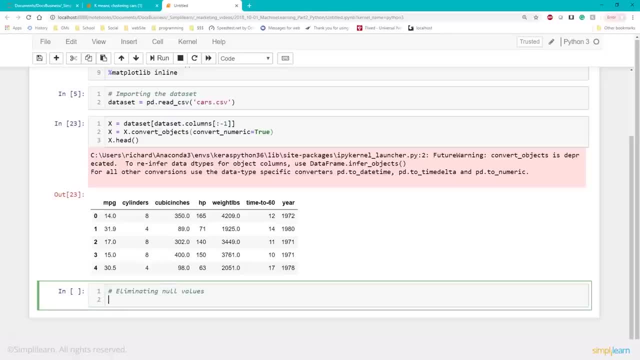 formatting this data. things are going to pop up and sometimes you go backwards to fix it, And that's fine. That's just part of exploring the data and understanding what you have, And I should have done this earlier. but let me go ahead and increase the size. 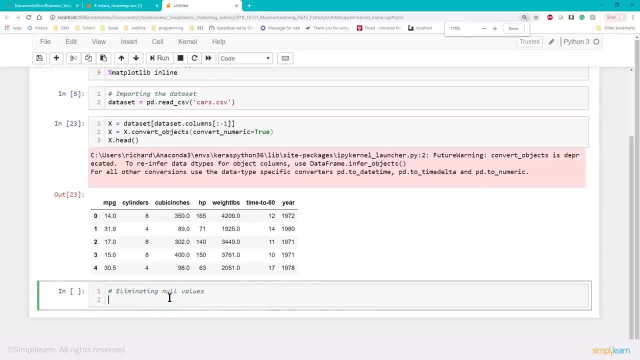 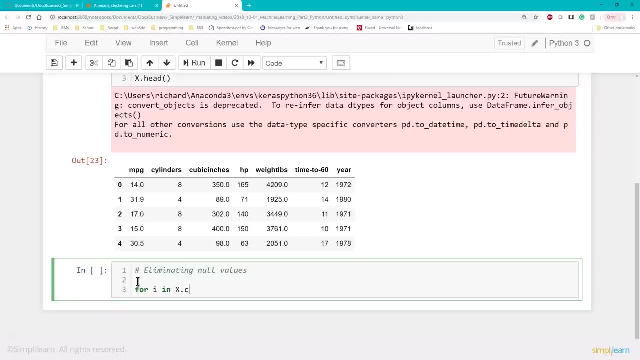 of my window one notch. There we go Easier to see. So we'll do for i in working with x dot columns, we'll page through all the columns and we want to take x of i and we're going to change that and we're going to alter it. 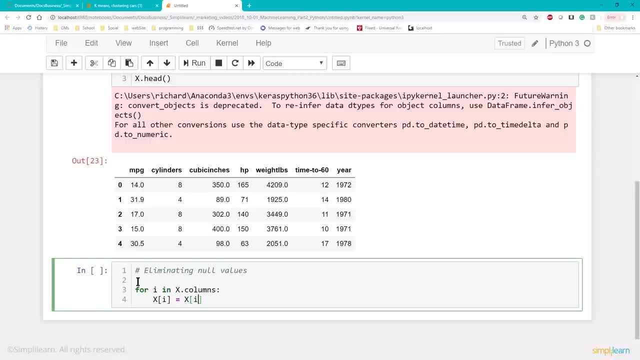 With this. we want to go ahead and fill in x of i. Pandas has the fill in a and that just fills in any non-existent missing data And we'll put my brackets up, and there's a lot of different ways to fill this data. 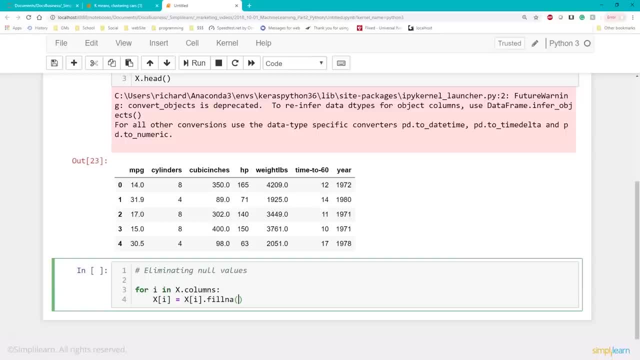 If you have a really large data set, some people just void out that data and then look at it later in a separate exploration of data. One of the tricks we can do is we can take our column and we can find the means, And the means is in. 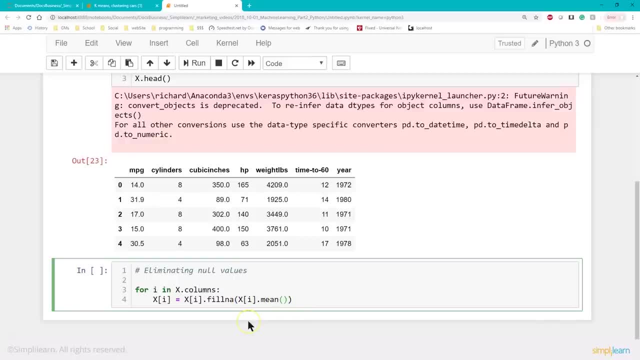 quotation marks. So we take the columns and we're going to fill in the non-existing one with the means. The problem is that returns a decimal float, So some of these aren't decimals. Certainly, you need to be a little careful doing this, but for this example we're just going to. 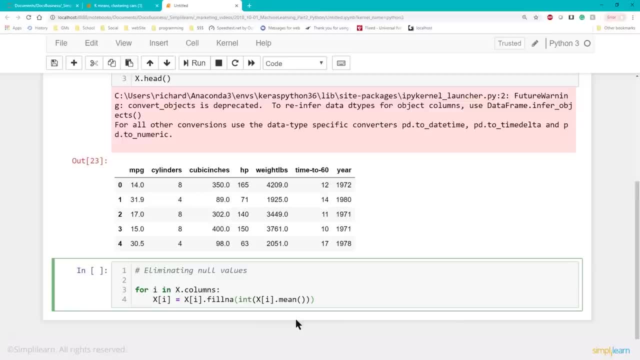 fill it in with the integer version of this. It keeps it on par with the other data. that isn't a decimal point. And then what we also want to do is we want to double check. A lot of times you do this first part first to double check, then you do the fill. 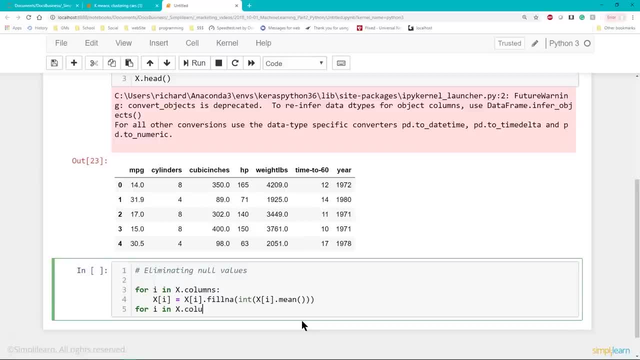 and then you do it again just to make sure you did it right. So we're going to go through and test for missing data And one of the ways you can do that is simply go in here and take our x of i column. so it's going to go through the x of i. 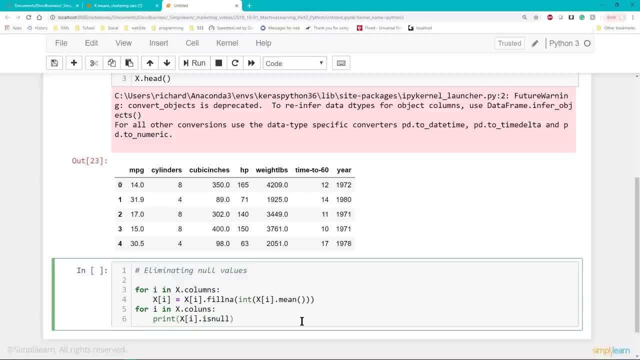 column that says is null, So it's going to return any place. there's a null value. it actually goes through all the rows of each column And then we want to go ahead and sum that. So we take that and we add the sum value, and these are all pandas. 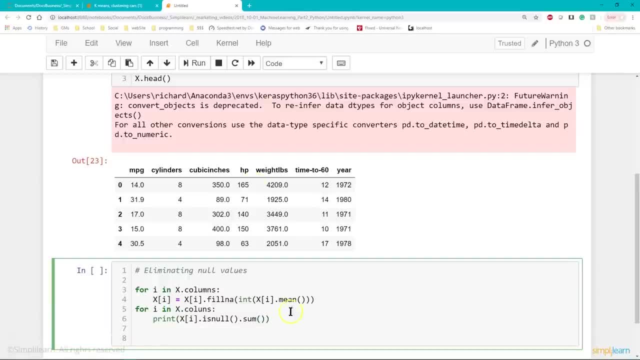 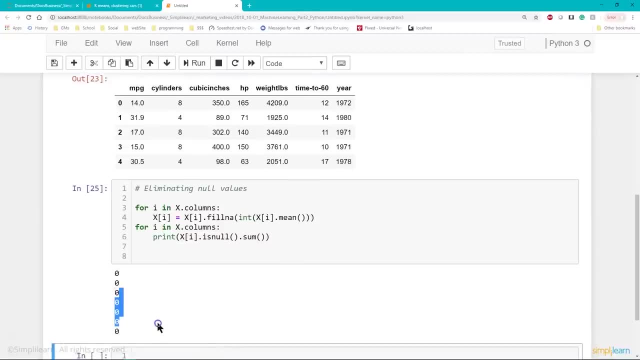 so is null is a panda command, and so is sum, And if we go through that and we go ahead and run it, and we go ahead and take and run that, you'll see that all the columns have zero null values. So we've now tested and double checked and our data is nice. 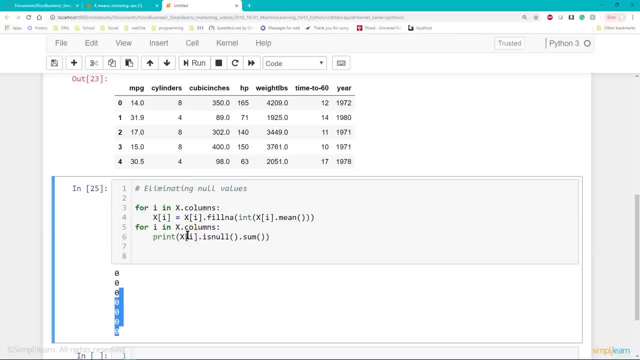 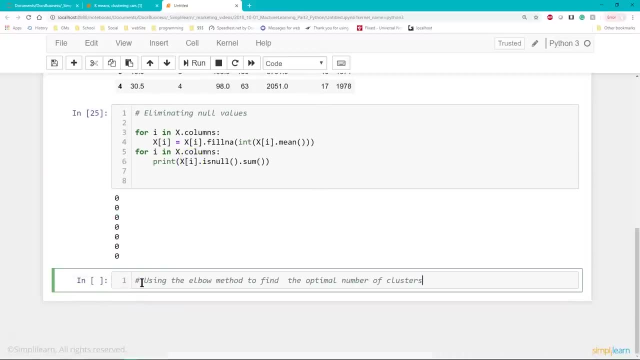 and clean. we have no null values. everything is now a number value. we turned it into numeric And we've removed the last column in our data, And at this point we're actually going to start using the ELBO method to find the optimal number of clusters. So we're now actually 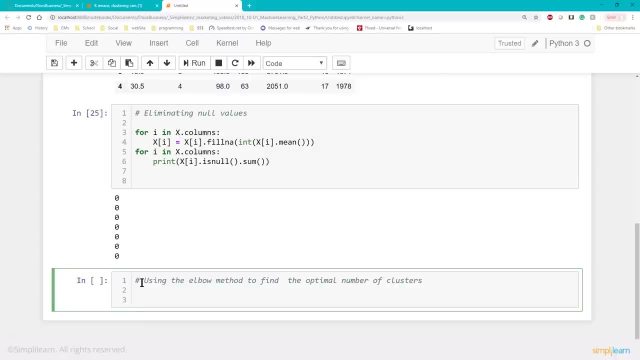 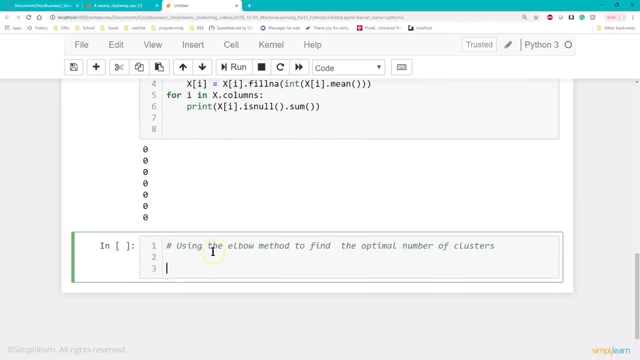 getting into the sklearn part. The k means clustering on here. I guess we'll go ahead and zoom it up one more knot so you can see what I'm typing in here. And then from sklearn going to our sklearn cluster, we're going to import. 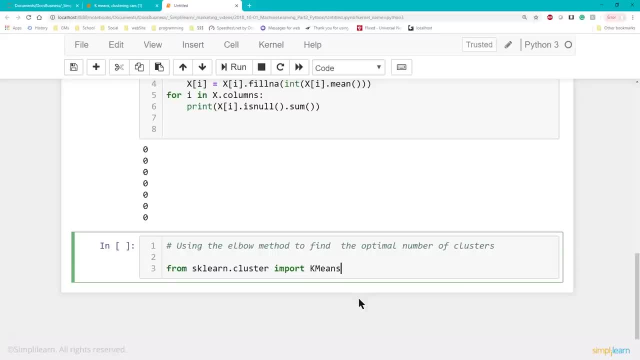 k means I always forget to capitalize the k and the m when I do this. So it's capital K, capital M. k means And we'll go ahead and create a ray. WCSS equals. let me get an empty ray, If you remember. 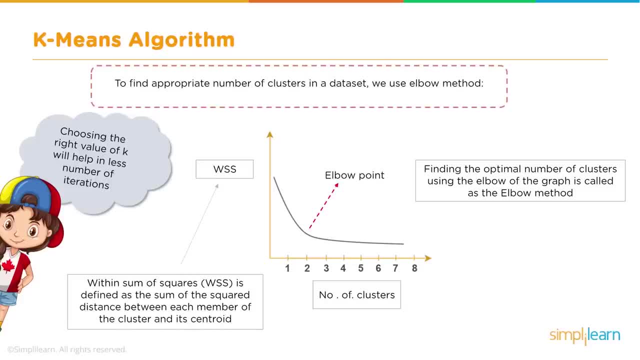 from the ELBO method, from our slide. within the sum of squares, WSS is defined as the sum of square distance between each member of the cluster in a centroid. So we're looking at that change in differences as far as a square distance And we're going to run this over a number 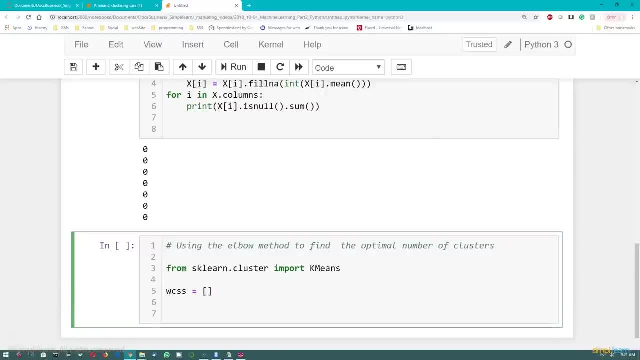 of k mean values. In fact, let's go for i in range. we'll do 11 of them, Range 0 of 11. And the first thing we're going to do is we're going to create the actual. we'll do it all. lower case. 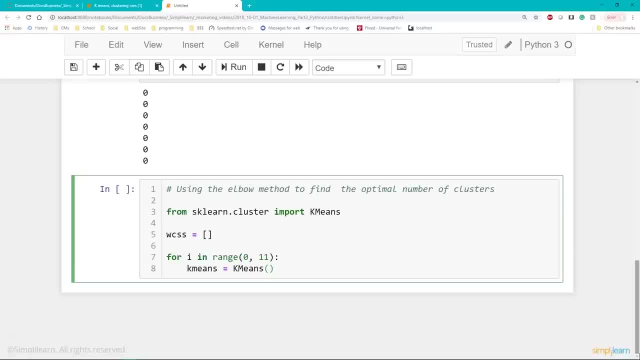 So we're going to create this object from the k means that we just imported And the variable that we want to put into this is in clusters And we're going to set that equals to i. That's the most important one, because we're looking. 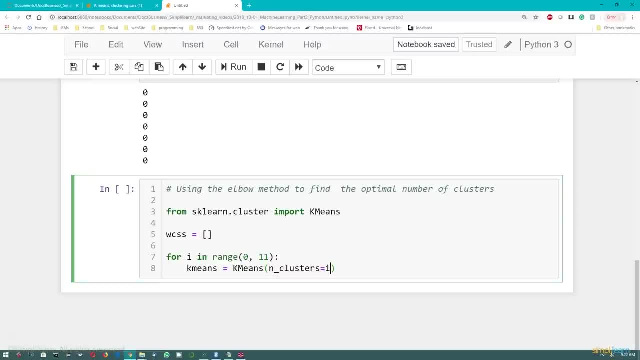 at how increasing the number of clusters changes our answer. There are a lot of settings to. the k means Our guys in the back did a great job, just kind of playing with some of them. The most common ones that you see in a lot of stuff is: 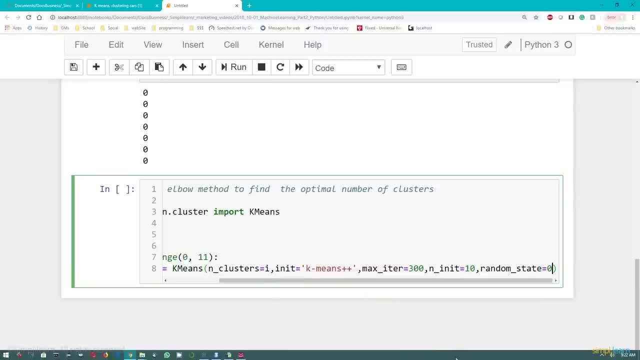 how you init your k means. So we have k means plus plus. This is just a tool to let the model itself be smart, how it picks its centroids to start with its initial centroids. We only want to iterate no more than 300 times. We have a max iteration we put. 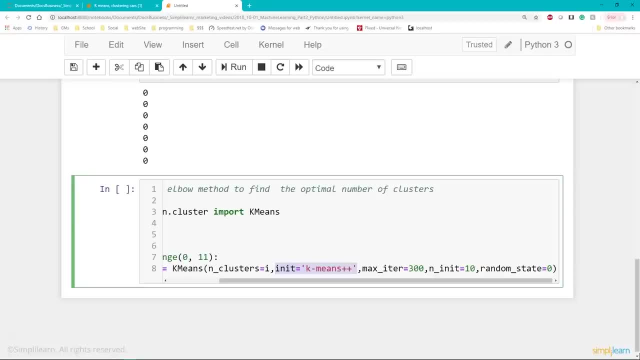 in there We have the int init. the random state equals 0.. You really don't need to worry too much about these when you're first learning this. As you start digging in deeper, you start finding that these are shortcuts that will speed up the process. 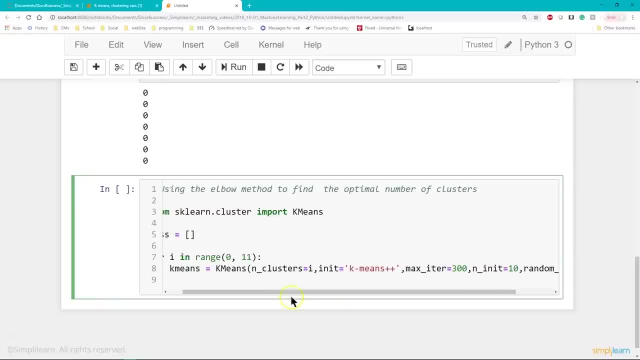 As far as the setup, But the big one that we're working with is the. in clusters equals i, So we're going to literally train our k means 11 times. We're going to do this process 11 times And if you're working, 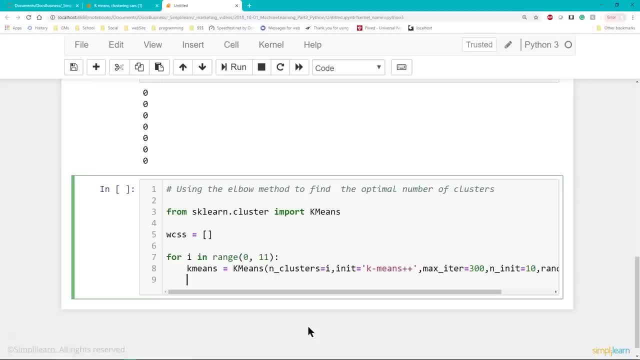 with big data, you know the first thing you do is you run a small sample of the data so you can test all your stuff on it. And you can already see the problem that if I'm going to iterate through a terabyte of data 11 times, 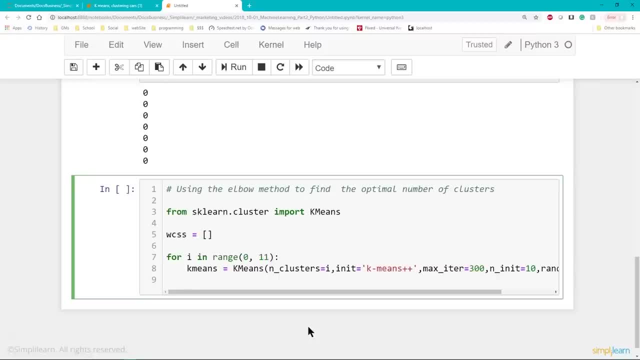 and then the k means itself is iterating through the data multiple times. that's a heck of a process, So you've got to be a little careful with this. A lot of times, though, you can find your ELBO using the ELBO method. find your optimal number on a sample of data. 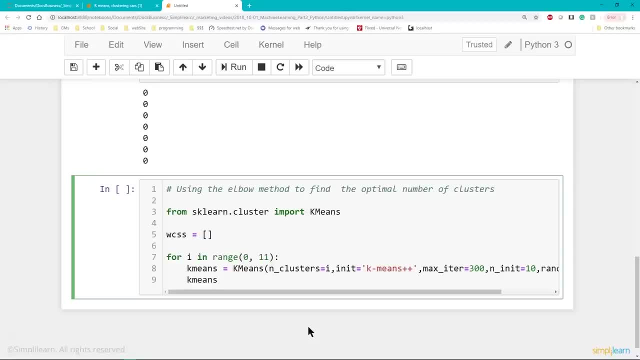 Especially if you're working with larger data sources. So we want to go ahead and take our k means and we're just going to fit it. If you're looking at any of the sklearn- very common- you fit your model If you remember correctly our variable. 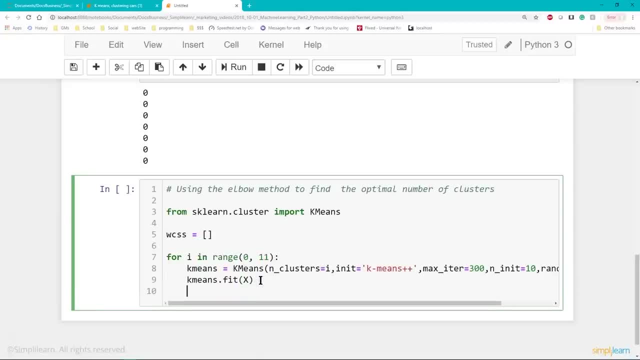 we're using is the capital X And once we fit this value we go back to the array we made. I'm just going to pin that value on the end And it's not the actual fit we're pinning in there. it's. 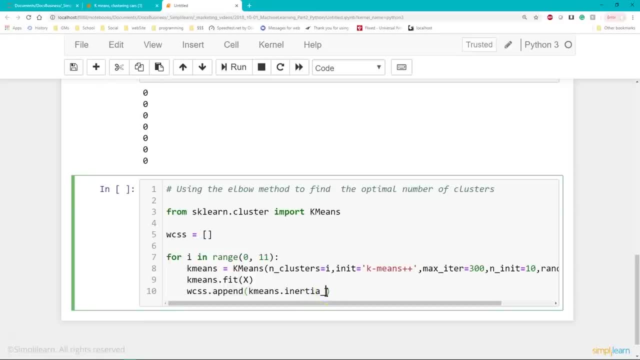 when it generates it. it generates. the value you're looking for is inertia, So kmeansinertia will pull that specific value out that we need And let's get a visual on this. We'll do our PLT plot and what we're plotting here 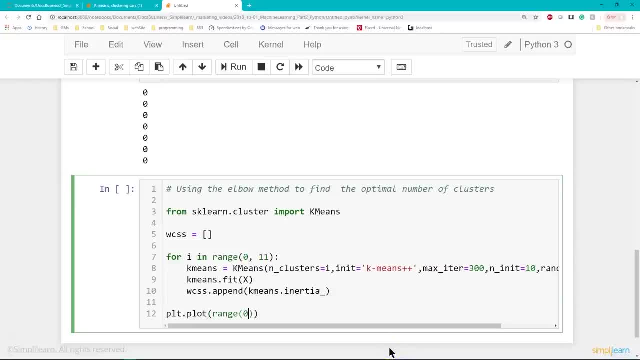 is first the X axis, which is range 0, 11.. So that will generate a nice little plot there, And the WCSS for our Y axis. It's always nice to give our plot a title, And let's see, we'll just give it the elbow. 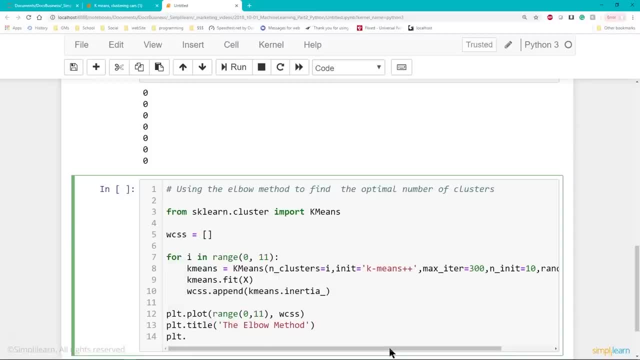 method for the title And let's get some labels. So let's go ahead and do PLT X label, And we'll do number of clusters for that, And PLT Y label, And for that we can do WCSS, since that's what we're. 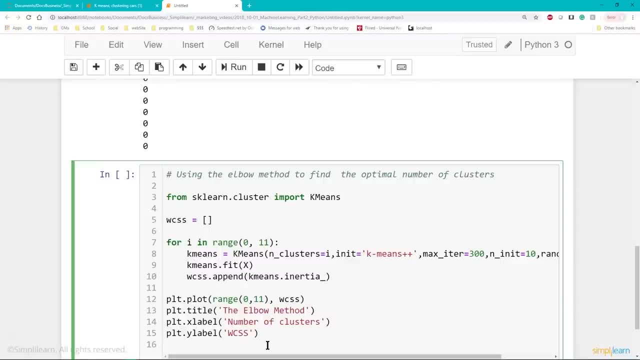 doing on the plot on there. And finally, we want to go ahead and display our graph, Which is simply PLT dot show. There we go And because we have it set to inline, it will appear inline. Hopefully I didn't make a type. 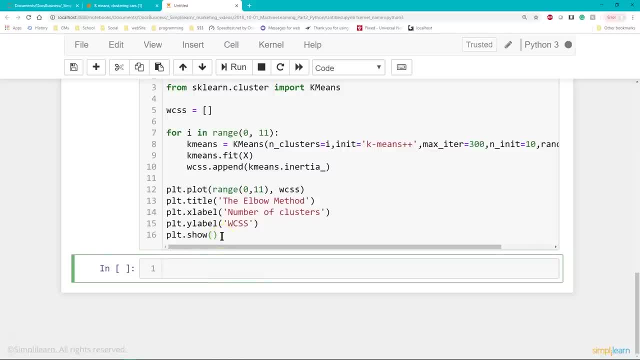 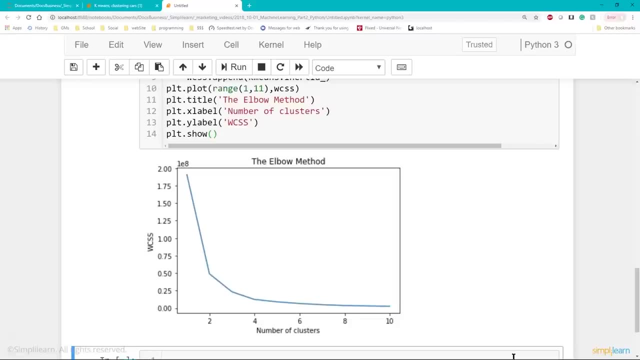 error on there And you can see we get a very nice graph. You can see a very nice elbow joint there at 2 and again right around 3 and 4, and then after that there's not very much. Now, as a data scientist, if I was. 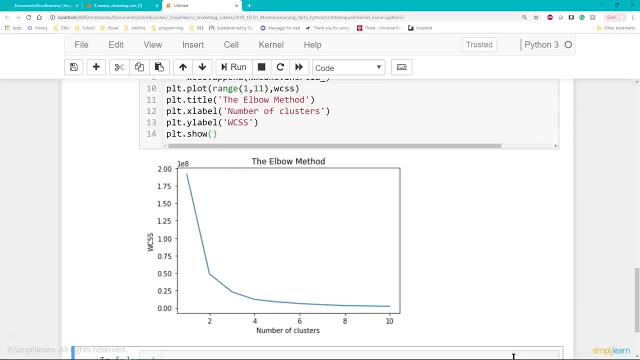 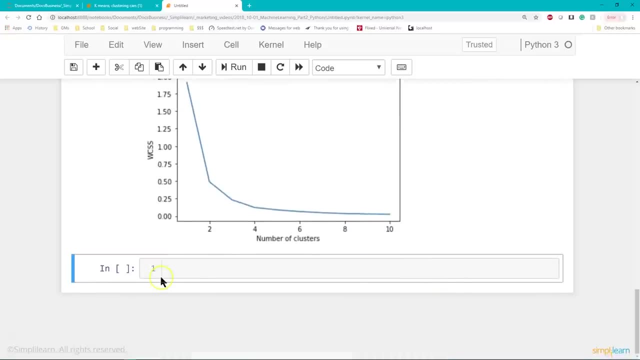 looking at this, I would do either 3 or 4 and I'd actually try both of them to see what the output looked like, And they've already tried this in the back. so we're just going to use 3 as a setup on here And let's go ahead and see what. 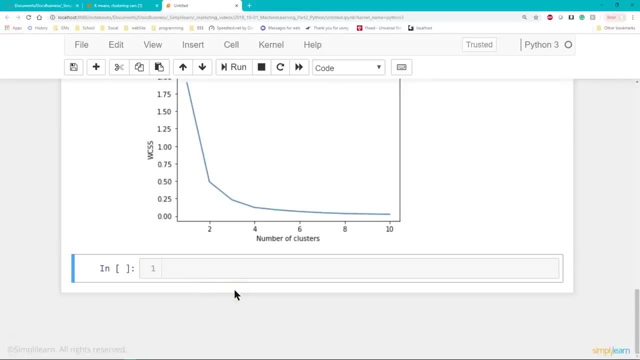 that looks like when we actually use this to show the different kinds of cars. And so let's go ahead and apply the k-means to the cars data set And basically we're going to copy the code that we looped through up above where. 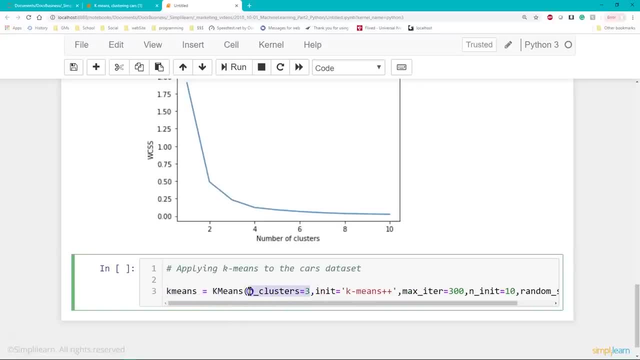 k-means equals k-means- number of clusters, and we're just going to set that number of clusters to 3.. Since that's what we're going to look for, And you can do 3 and 4 on this and graph them just to see how they come up differently, I'd be kind of 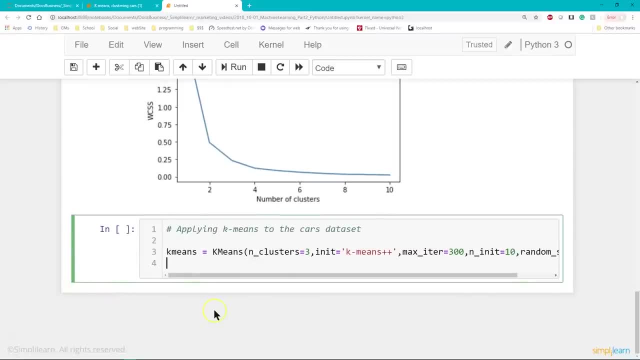 curious to look at that, But for this we're just going to set it to 3. Go ahead and create our own variable ykmeans for our answers and we're going to set that equal to kmeans, but we're not going to do a. 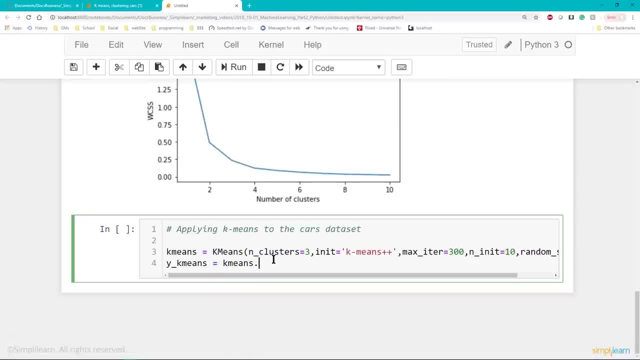 fit. We're going to do a fit. predict is the setup you want to use, And when you're using untrained models you'll see slightly different, because usually you see fit and then you see just the predict. But we want to both fit and predict. 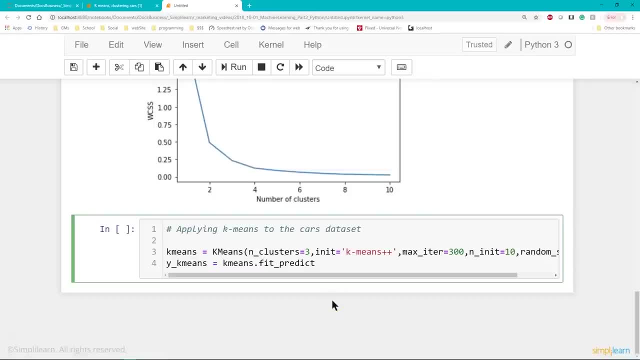 the k-means on this And that's fit. underscore predict. and then our capital X is the data we're working with. And before we plot this data, we're going to do a little panda's trick: We're going to take our x value and we're going to set x as. 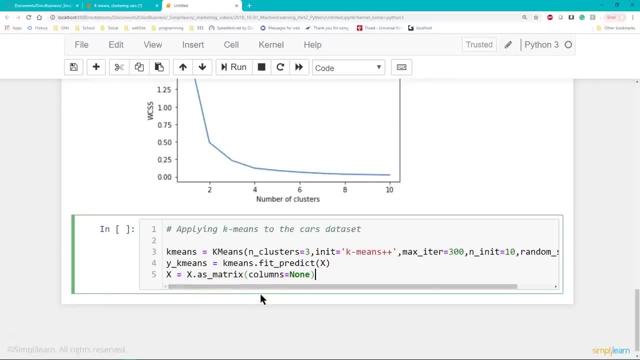 matrix. So we're converting this into a nice rows and columns kind of setup. But we want the. we're going to have. columns equals none. So it's just going to be a matrix of data in here And let's go ahead and run. 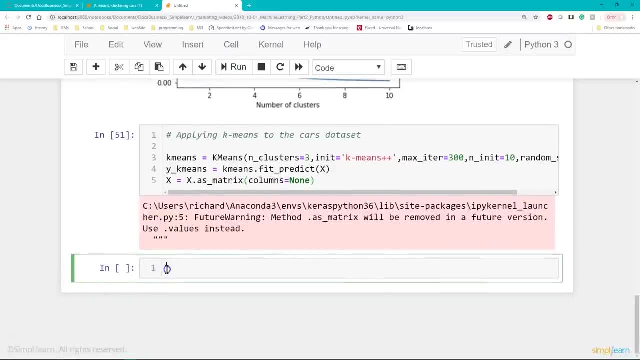 that A little warning. You'll see these warnings pop up because things are always being updated, So there's like minor changes in the versions and future versions. Instead of matrix- now it's more common to set it dot values instead of doing as matrix. 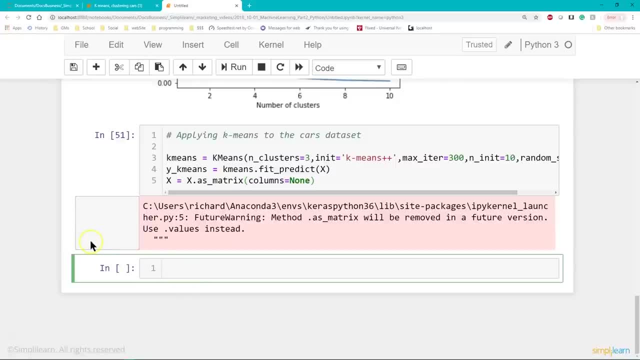 But math's matrix works just fine for right now And you'll want to update that later on. But let's go ahead and dive in and plot this and see what that looks like. And before we dive into plotting this data, I always like to take a look. 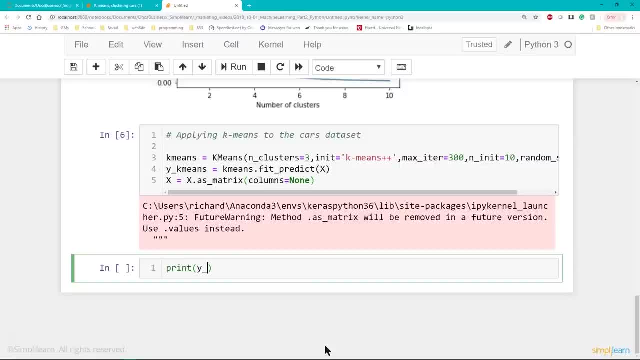 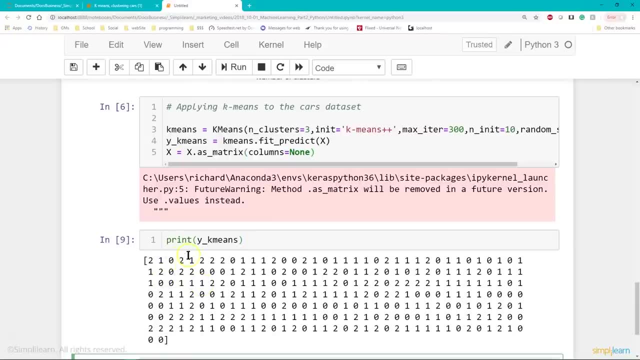 and see what I am plotting. So let's take a look at y. k means I'm just going to print that out down here And we see we have an array of answers. We have 2, 1 0, 2, 1 2. 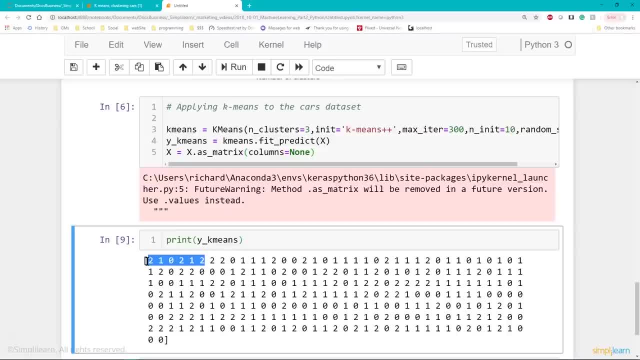 So it's clustering these different rows of data based on the three different spaces it thinks it's going to be. And then let's go ahead and print x and see what we have for x, And we'll see that x is an array, it's a. 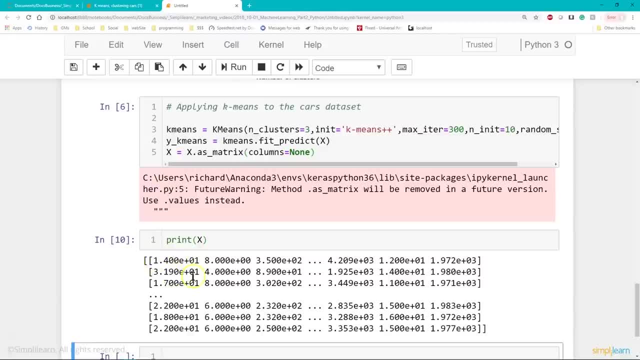 matrix. So we have our different values in the array And what we're going to do. it's very hard to plot all the different values in the array, So we're only going to be looking at the first 2, or positions 0 and 1.. 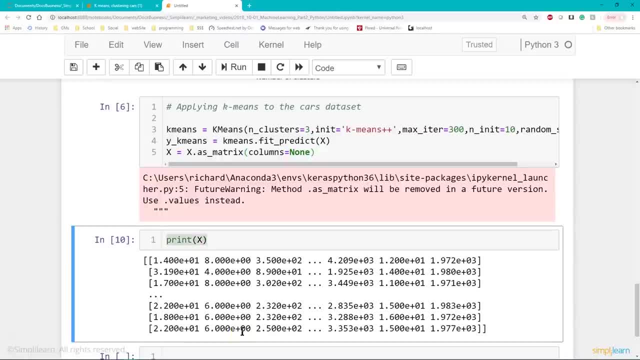 And if you were doing a full presentation in front of the board meeting, you might actually do a little different and dig a little deeper into the different aspects, Because this is all the different columns we looked at, But we'll only look at columns 1 and 2. 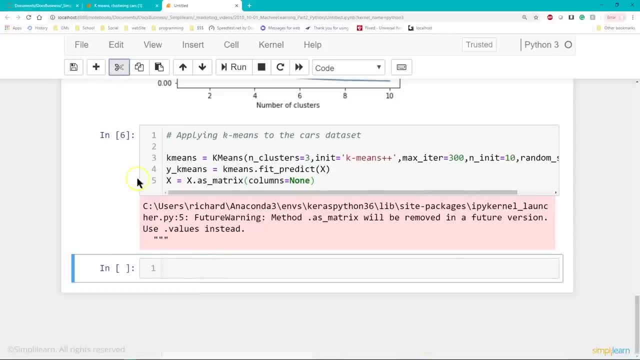 for this to make it easy. So let's go ahead and clear this data out of here And let's bring up our plot, And we're going to do a scatter plot here. So PLT scatter and this looks a little complicated, So let's explain what's going on with. 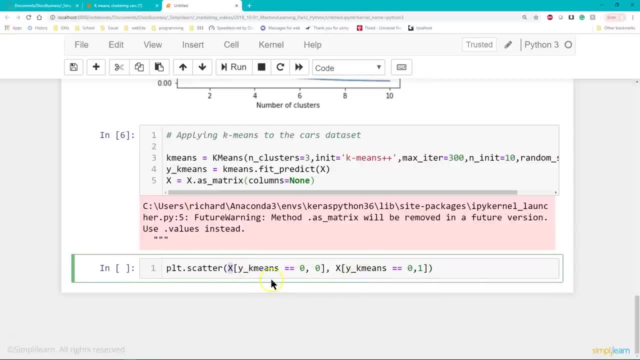 this: We're going to take the x values and we're only interested in y of k means equals 0, the first cluster, Okay. And then we're going to take values 0 for the x axes, And then we're going to do the same thing here. We're only 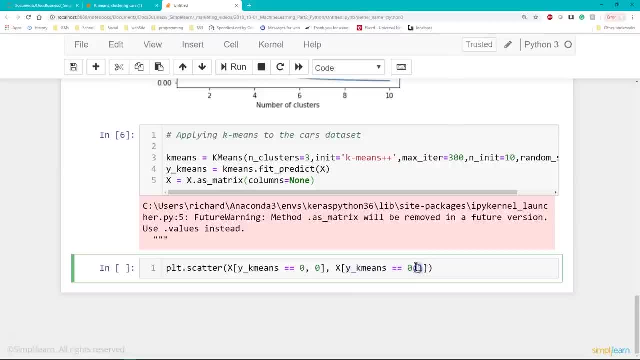 interested in. k means equals 0. But we're going to take the second column. So we're only looking at the first 2 columns in our answer or in the data, And then the guys in the back played with this a little bit. 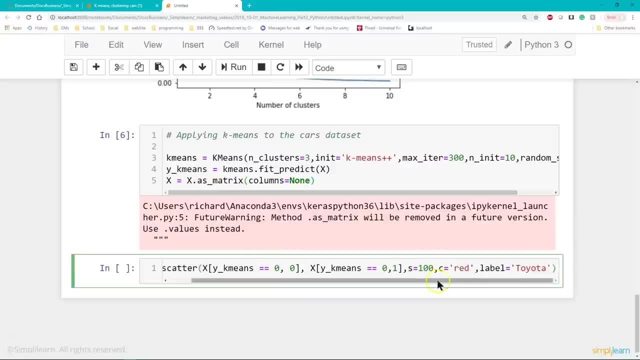 to make it pretty, And they discovered that it looks good if it has a size equals 100.. That's the size of the dots. We're going to use red for this one. And when they were looking at the data and what came out, 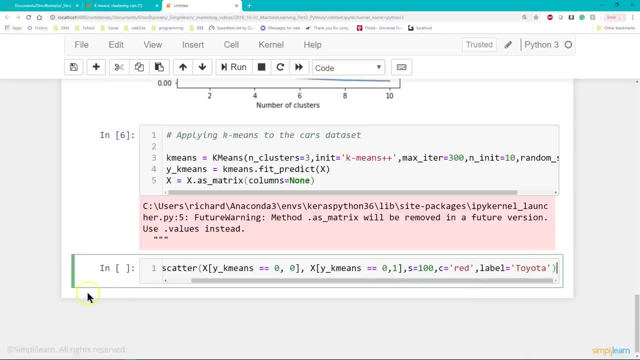 it was definitely the Toyota on this. We're just going to go ahead and label it Toyota Again. that's something you really have to explore in here. As far as playing with those numbers and see what looks good, We'll go ahead and hit enter in there. 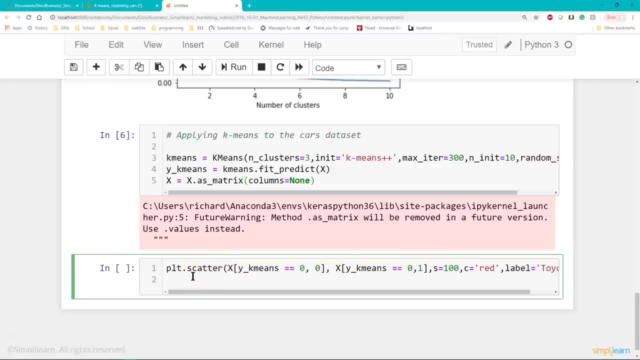 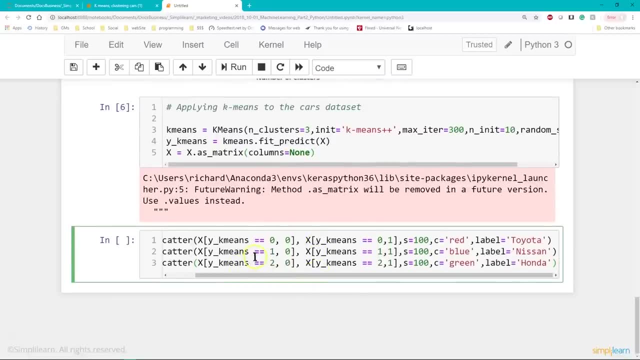 And I'm just going to paste in the next 2 lines, which is the next 2 cars, And this is our Nissan and Honda. And you'll see, with our scatter plot, we're now looking at where y underscore k means equals 1.. 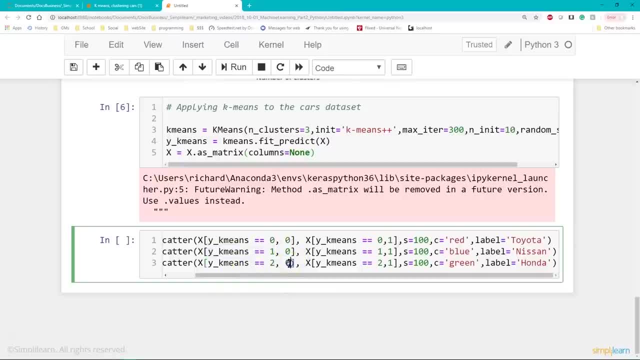 And we want the 0 column and y k means equals 2.. Again, we're looking at just the first 2 columns, 0 and 1. And each of these rows then corresponds to Nissan and Honda, And I'll go ahead. 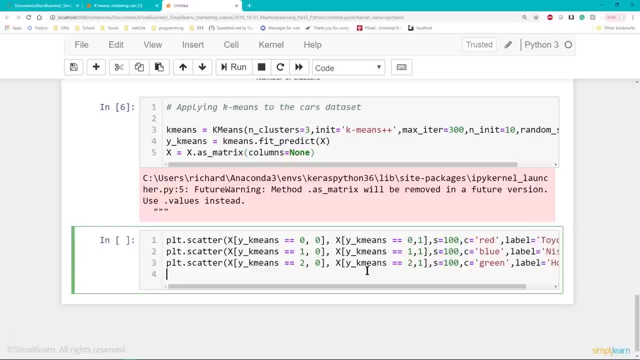 and hit enter on there. And finally let's take a look and put the centroids on there. Again, we're going to do a scatter plot And on the centroids you can just pull that from our k- means the model we created. 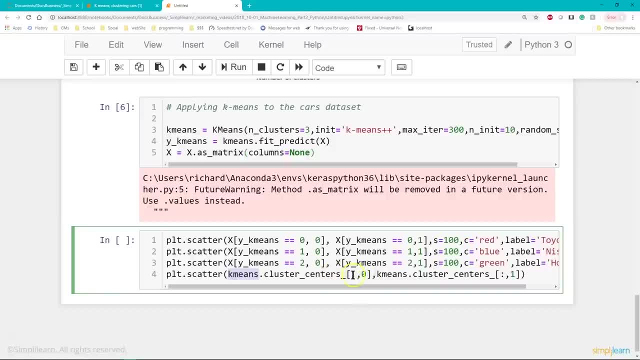 dot cluster centers, And we're going to just do all of them and the first number and all of them and the second number, which is 0, 1.. Because you always start with 0 and 1. And then we're playing. 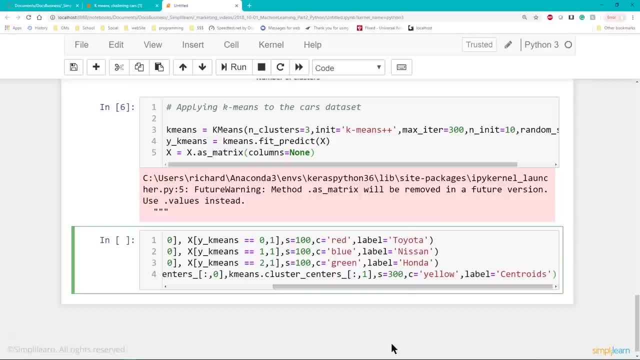 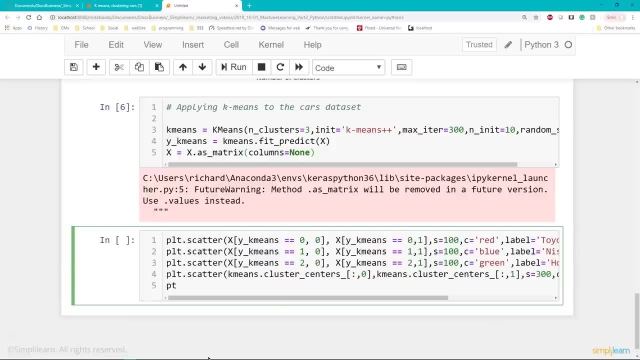 with the size and everything to make it look good. We'll do a size of 300.. We're going to go make the color yellow and we'll label them. it's always good to have some good labels, centroids. And then we want to do a title. 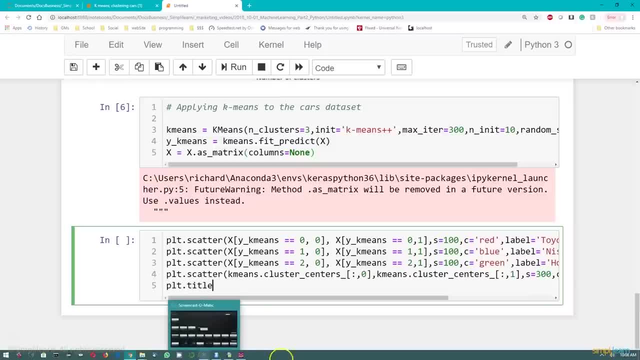 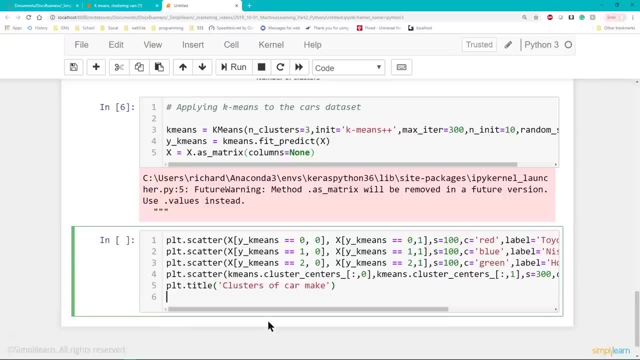 PLT title And pop up there PLT title because you always want to make your graphs look pretty. We'll call it clusters of car make, And one of the features of the plot library is you can add a legend. It'll automatically bring in it, since 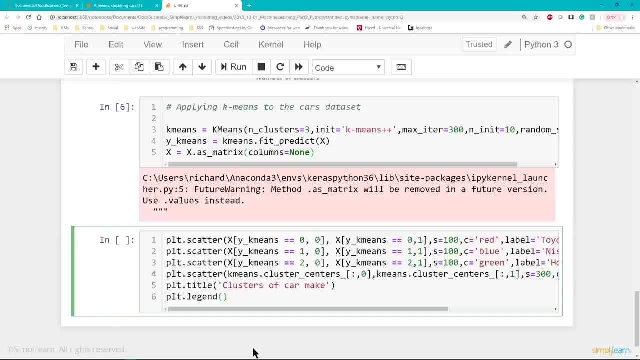 we've already labeled the different aspects of the legend with Toyota, Nissan and Honda. And finally, we want to go ahead and show So we can actually see it And remember it's inline, So if you're using a different editor, 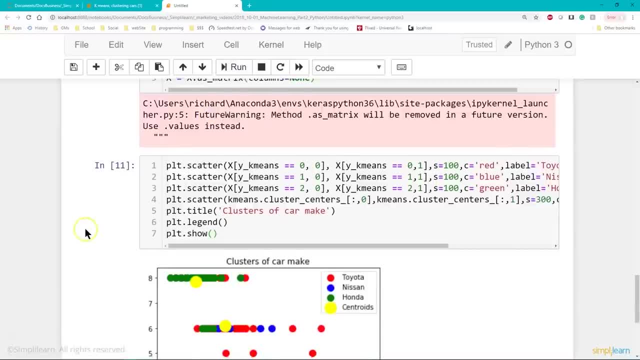 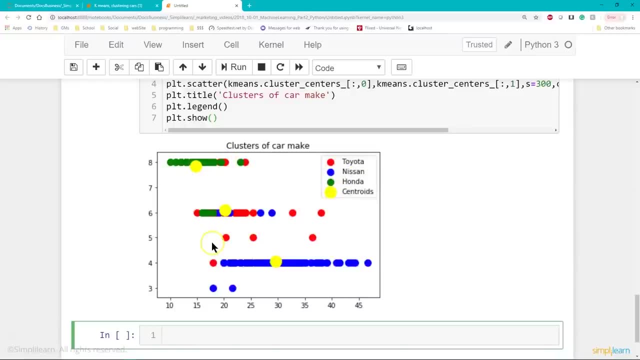 that's not the Jupyter Notebook. you'll get a pop up of this And you should have a nice set of clusters here. So we can look at this and we have clusters of Honda in green, Toyota in red, Nissan in purple And you can see where they put. 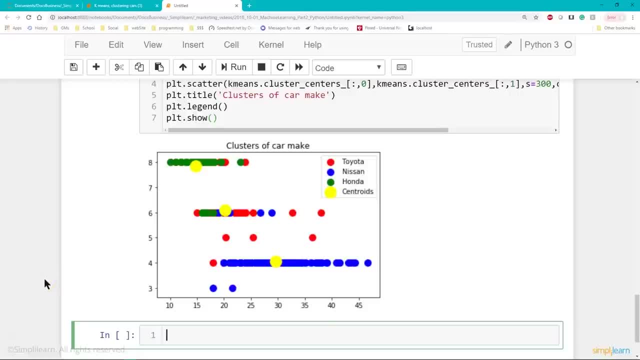 the centroids to separate them. Now, when we're looking at this, we can also plot a lot of other different data on here as far, because we only looked at the first two columns. This is just column one and two, Or zero one as you label. 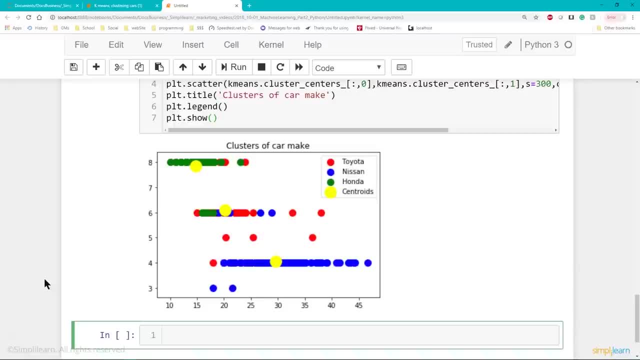 them in computer scripting. But you can see, here we have nice clusters of car make and we've been able to pull out the data And you can see how just these two columns form very distinct clusters of data. So if you were exploring new data you might take. 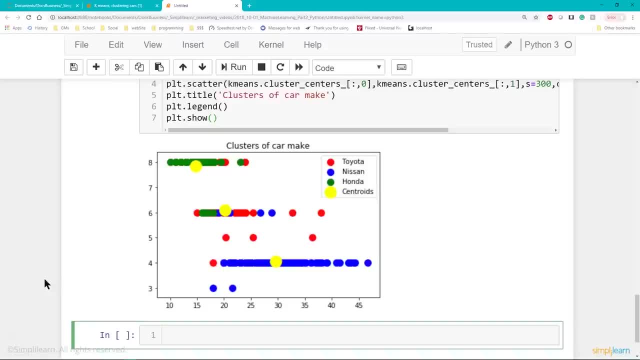 a look and say, well, what makes these different? Almost going in reverse, you start looking at the data and pulling apart the columns to find out why is the first group set up the way it is? Maybe you're doing loans and you want to go well, why is this group not defaulting? 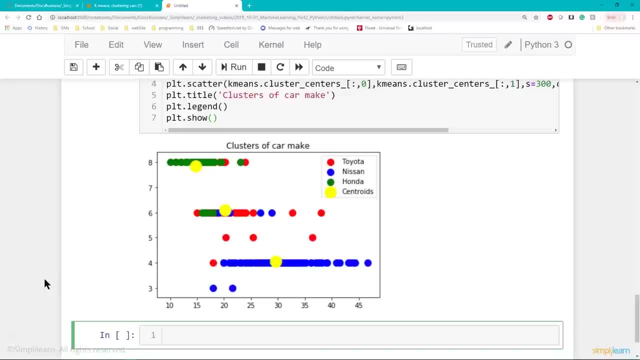 on their loans? And why is the last group defaulting on their loans? And why is the middle group- 50%- defaulting on their bank loans? And you start finding ways to manipulate the data and pull out the answers you want. So, now that you've seen how to use 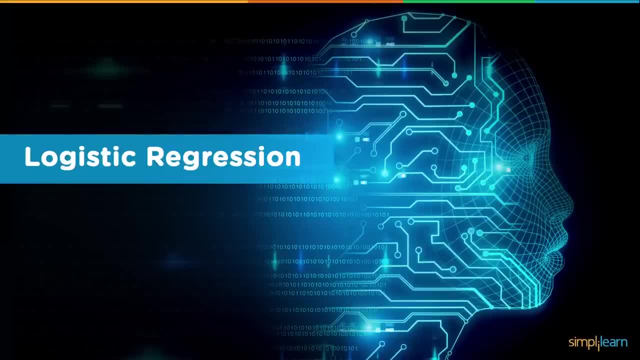 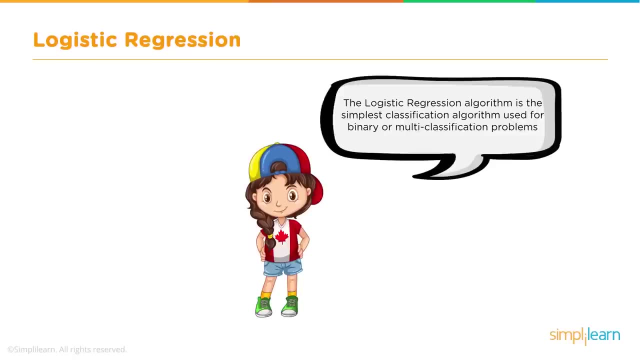 k-mean for clustering. let's move on to the next topic Now. let's look into logistic regression. The logistic regression algorithm is the simplest classification algorithm used for binary or multi-classification problems. And we can see: we have our little girl from Canada. 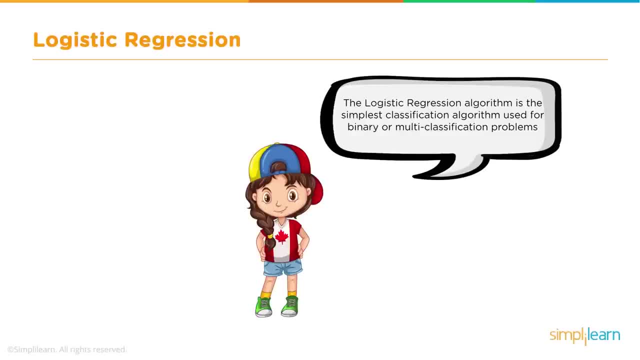 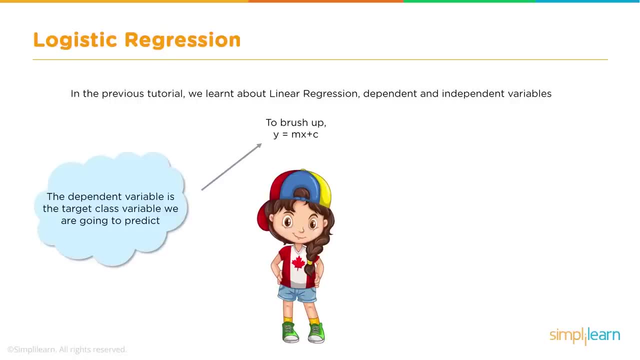 who's into horror books is back. That's actually really scary when you think about that with those big eyes. In the previous tutorial we learned about linear regression. We learned about independent and independent variables. So to brush up: y equals mx plus c. 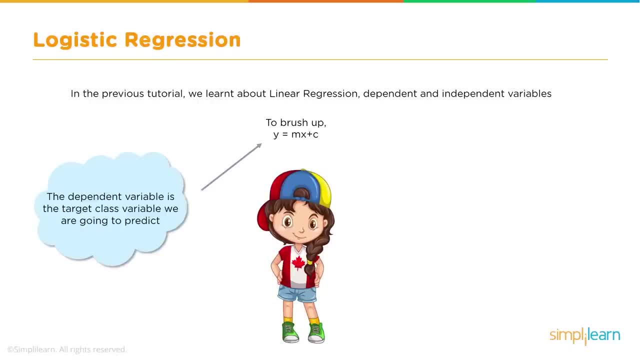 A very basic algebraic function of y and x. The dependent variable is the target class variable we are going to predict. The independent variables, x1 all the way up to xn, are the features or attributes we're going to use to predict the target class. 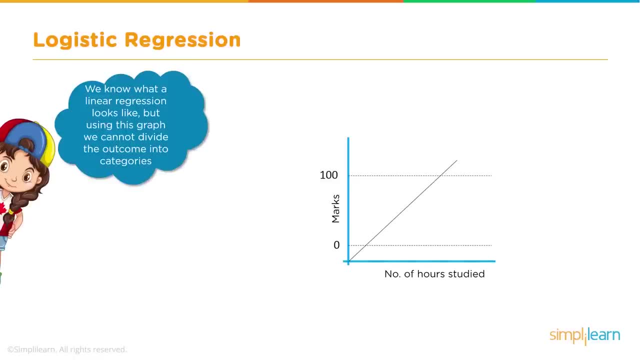 We know what a linear regression looks like, but using the graph, we cannot divide the outcome into categories. It's really hard to categorize 1.5, 3.6, 9.8.. For example, a linear regression graph can tell us that with increase, 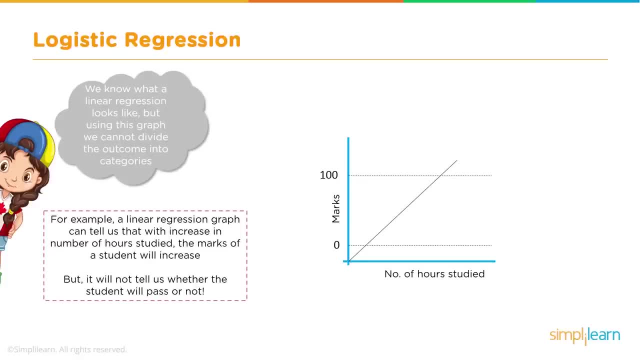 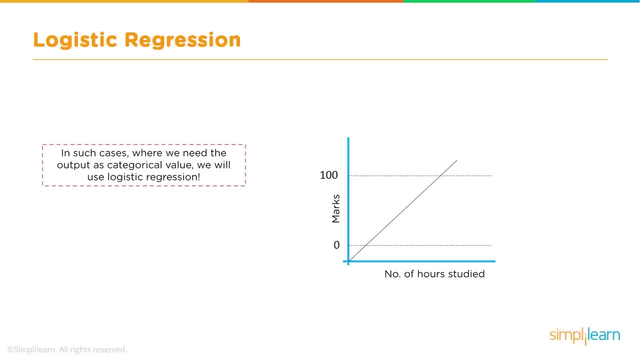 in number of hours studied, the marks of a student will increase, But it will not tell us whether the student will pass or not. In such cases where we need the output as categorical value, we will use logistic regression, And for that we're going to use the sigmoid function. 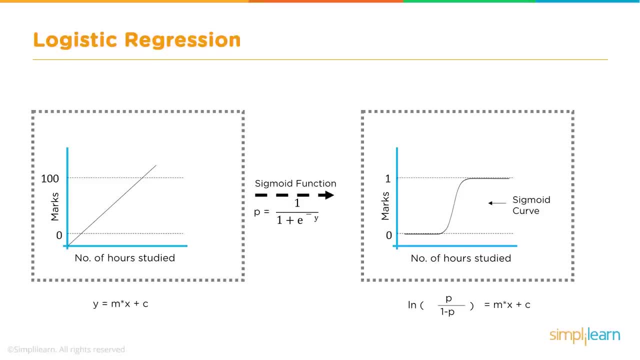 So you can see, here we have our marks 0 to 100, number of hours studied. that's going to be what they're comparing it to in this example, And we usually form a line that says y equals mx plus c, And when we use the sigmoid function. 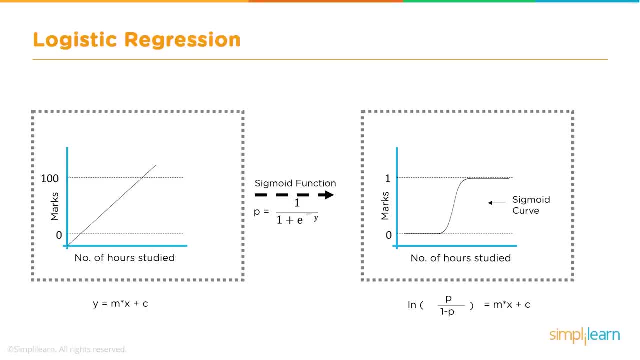 we have: p equals 1 over 1, plus e to the minus y, It generates a sigmoid curve. And so you can see right here, when you take the ln, which is the natural logarithm. I always thought it should be nl, not ln, that's just the inverse of e. 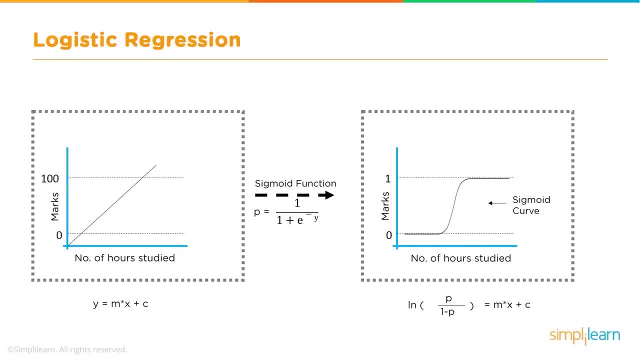 or e to the minus y, And so when we do this we get ln of p over 1 minus p equals m times x plus c. That's the sigmoid curve function we're looking for. Now we can zoom in on the function and you'll see that the function 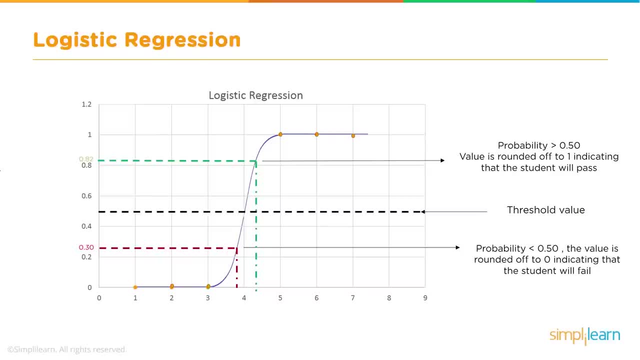 as it derives, goes to 1 or to 0, depending on what your x value is And the probability. if it's greater than .5, the value is automatically rounded off to 1, indicating that the student will pass. So if they're doing a certain amount of studying, 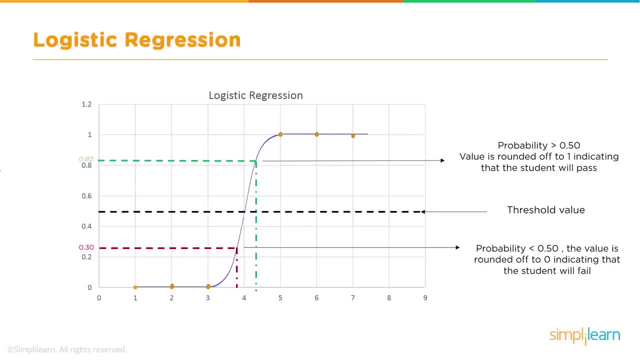 they will probably pass. Then you have a threshold value at the .5. it automatically puts that right in the middle usually, And your probability if it's less than .5, the value rounded off to 0, indicating the student, will fail. So if they're not studying very hard, 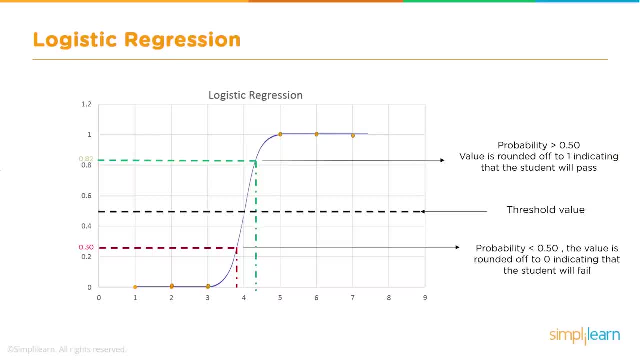 they're probably going to fail. This, of course, is ignoring the outliers of that one student who's just a natural genius and doesn't need any studying to memorize everything. That's not me, unfortunately. I have to study hard to learn new stuff. 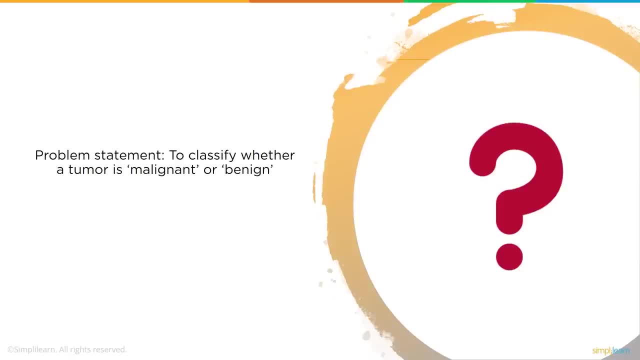 Problem statement To classify whether a tumor is malignant or benign. And this is actually one of my favorite tests to play with because it has so many features and when you look at them you really are hard to understand. You can't just look at them and know the answer. 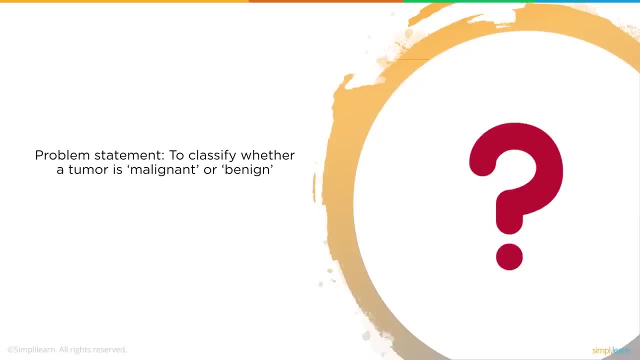 So it gives you a chance to kind of dive into what data looks like when you aren't able to understand the specific domain of the data. But I also want to remind you that, in the domain of medicine, if I told you that my probability was really good at classifying things, 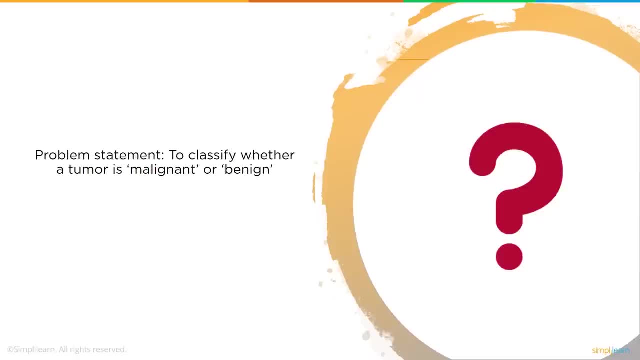 at, say, 90% or 95%, and I'm classifying whether you're going to have a malignant or a benign tumor. I'm guessing that you're going to go get it tested anyways. So you've got to remember the domain we're working with. 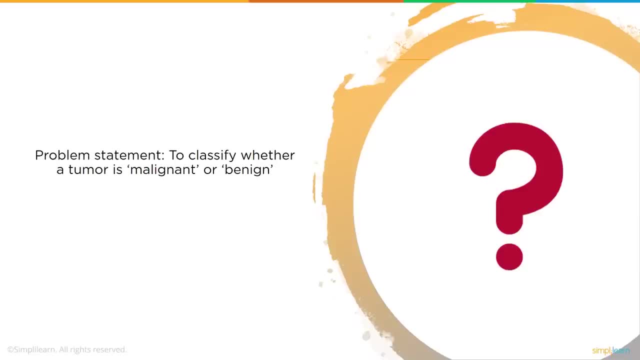 So why would you want to do that if you know you're just going to go get a biopsy? because it's that serious. This is like an all or nothing. Just referencing the domain it's important. It might help the doctor know where to look. 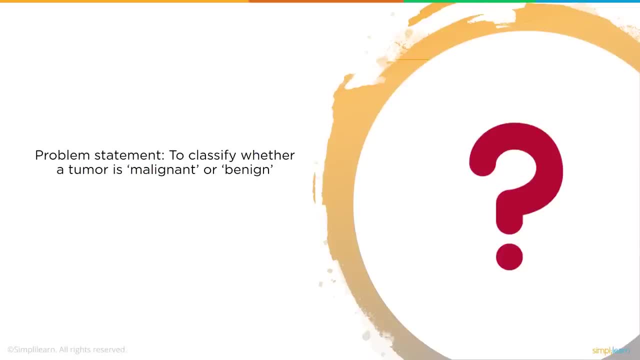 just by understanding what kind of tumor it is. So it might help them or aid them in something they missed from before. So let's go ahead and dive into the code and I'll come back to the domain part of it in just a minute. 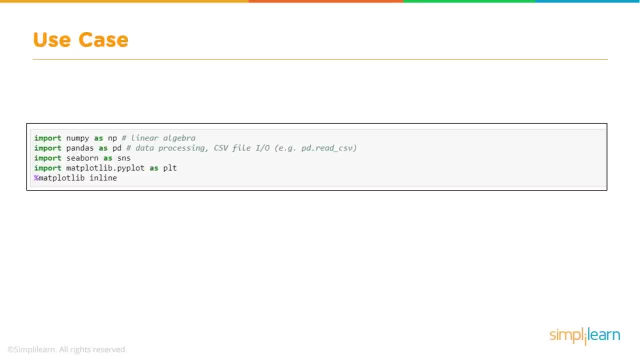 So use case, And we're going to do our normal imports here. We're importing numpy, pandas, seaborne, the matplotlibrary, and we're going to do matplotlibrary inline, since I'm going to switch over to Anaconda, So let's go ahead and flip over there. 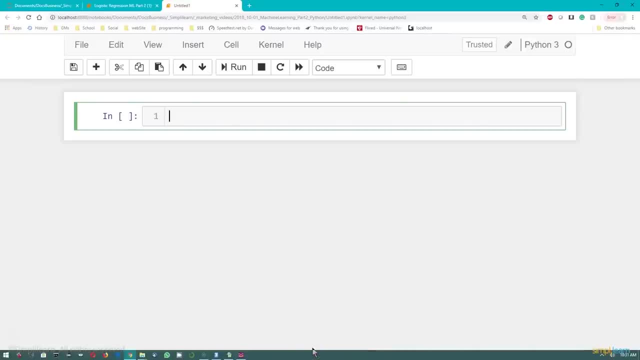 and get this started. So I've opened up a new window in my Anaconda Jupyter Notebook And, by the way, Jupyter Notebook, you don't have to use Anaconda for the Jupyter Notebook. I just love the interface and all the tools. 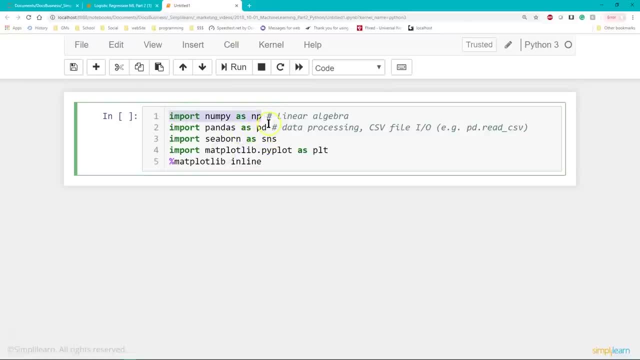 we have here. We have our numpy p for our numpy number array. We have our pandas pd. We're going to bring in seaborne to help us with our graphs as sns. So many really nice tools in both seaborne and matplotlibrary. 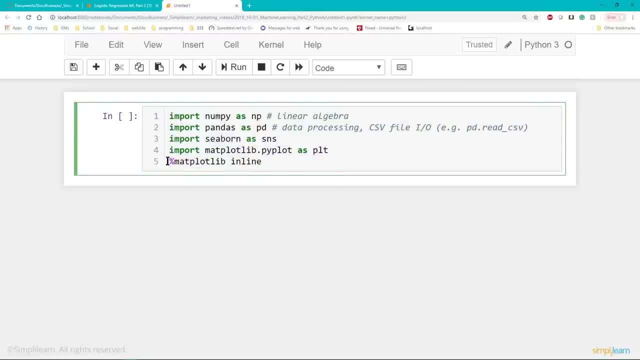 Then we'll do our matplotlibrarypiplot as plt and then of course, we want to let it know to do it inline. Let's go ahead and just run that. so it's all set up And we're just going to call our data data. 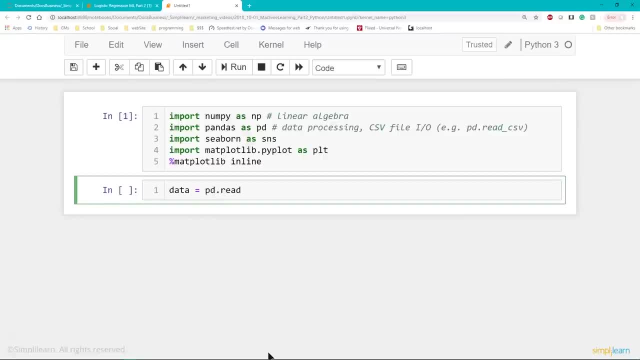 Not creative today. Equals pd, p2.csv file. So we'll use the pdread underscore csv And I happened to name the file. I renamed it. data for p2.csv. You can, of course, write in the comments below the YouTube and request. 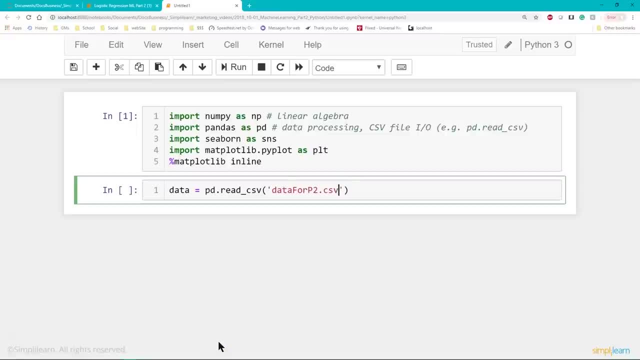 for the data set itself, or go to the Simply Learn website and we'll be happy to supply that for you. And let's just open up the data before we go any further. and let's just see what it looks like in a spreadsheet. So when I pop it open in a local spreadsheet, 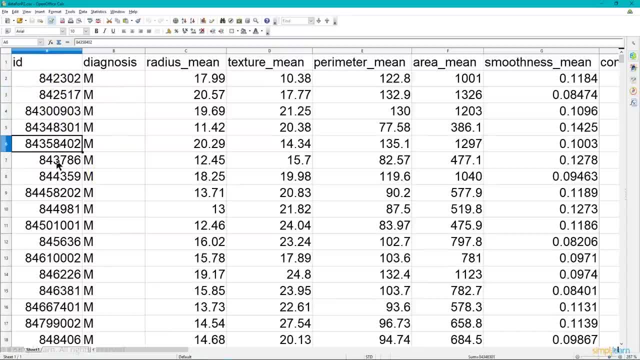 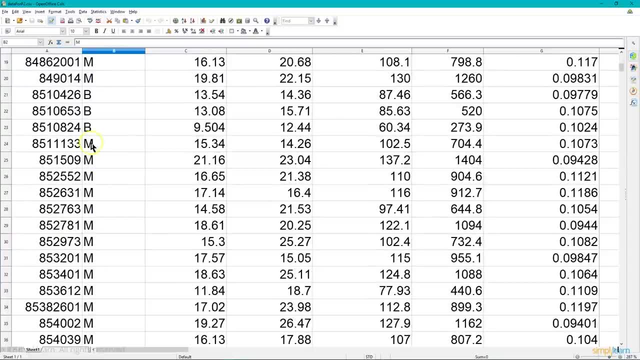 you can see it's separated variables. We have an ID, so I guess the categorizes for reference or what ID which test was done, The diagnosis, M for malignant, B for benign. So there's two different options on there And that's what we're going to try to predict. 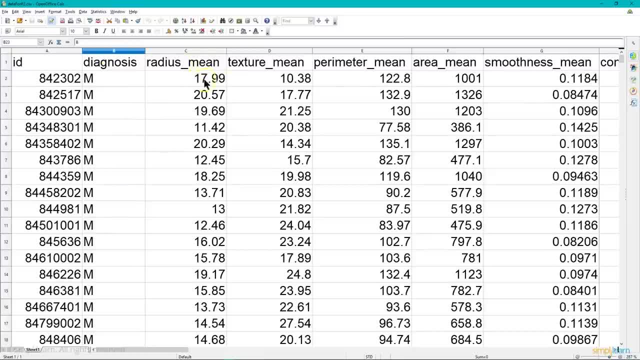 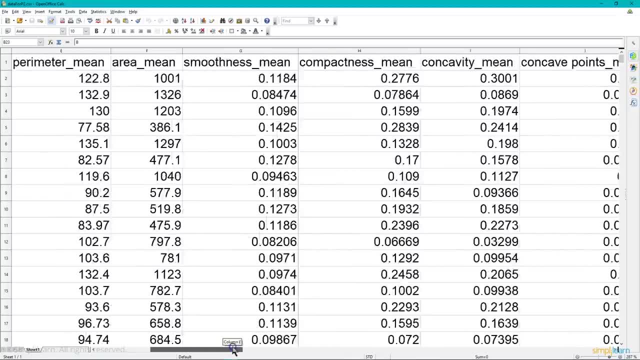 is the M and B and test it And then we have like the radius, mean or average, the texture, average perimeter, mean area, mean, smoothness. I don't know about you, but unless you're a doctor in the field, 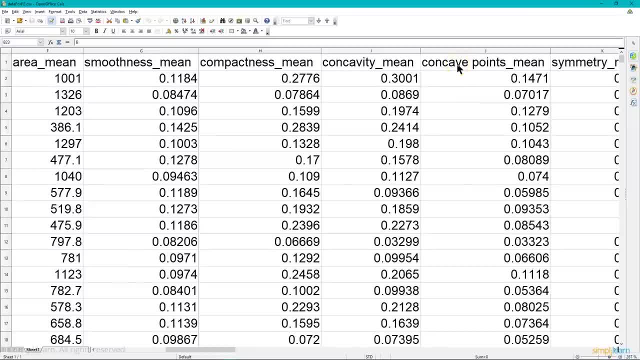 you can guess what concave means just by the term concave, But I really wouldn't know what that means in the measurements they're taking. So they have all kinds of stuff like how smooth it is the symmetry, And these are all float values. 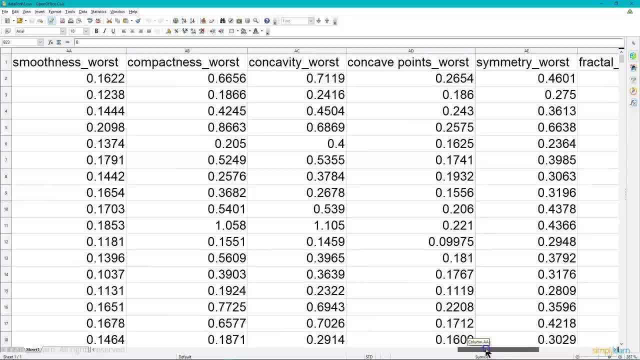 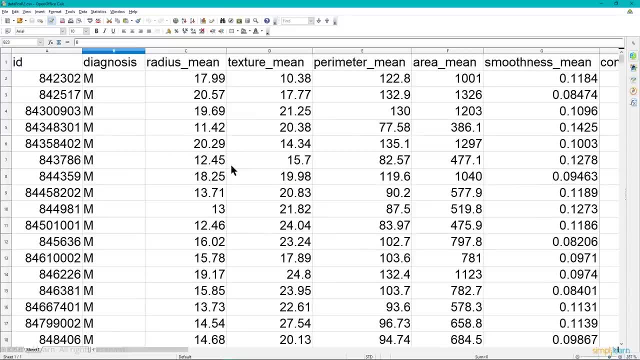 We can just page through them real quick And you'll see. there's, I believe, 36, if I remember correctly, in this one. So there's a lot of different values they take and all these measurements they take when they go in there and they take a look. 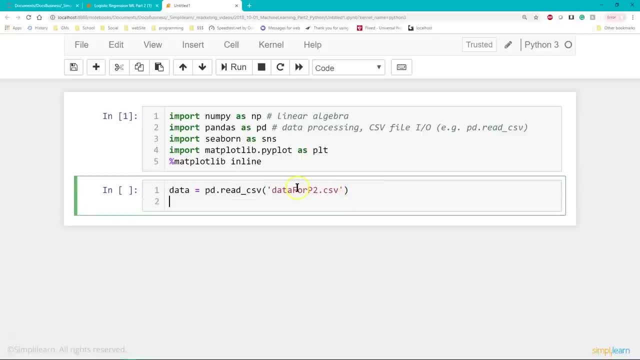 at the different growth, the tumorous growth. So back in our data. the folder is a code, So I saved this code in that folder. Obviously, if you have it in a different location, you want to put the full path in there. 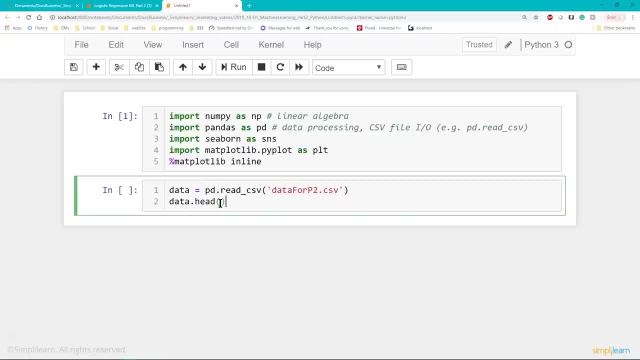 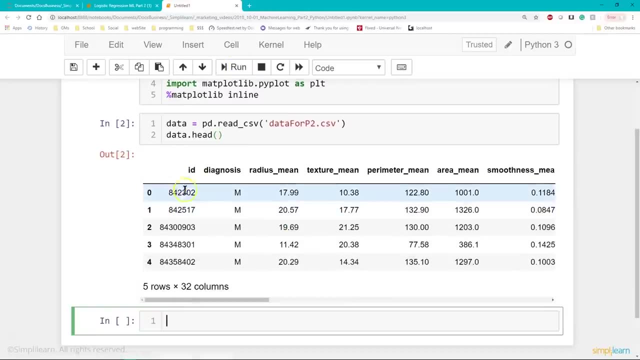 And we'll just do Panda's first five lines of data with the datahead. When we run that, we can see that we have pretty much what we just looked at. We have an ID, we have a diagnosis, If we go all the way across. 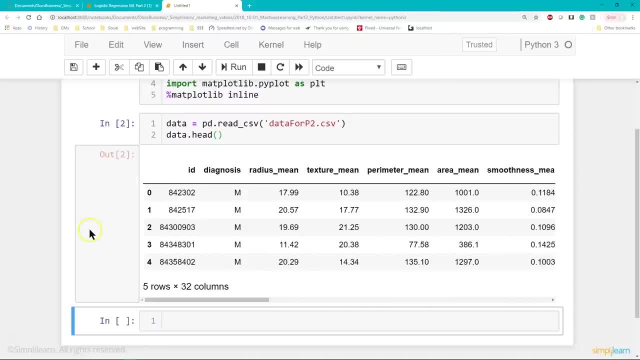 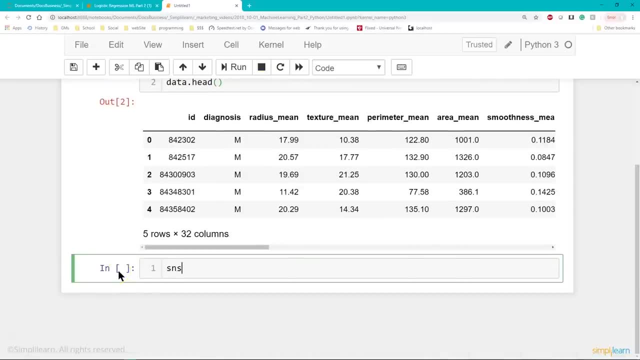 you'll see all the different columns coming across, displayed nicely for our data. And while we're exploring the data, our Seaborn, which we referenced as SNS, makes it very easy to go in here and do a joint plot. You'll notice it's very similar to. 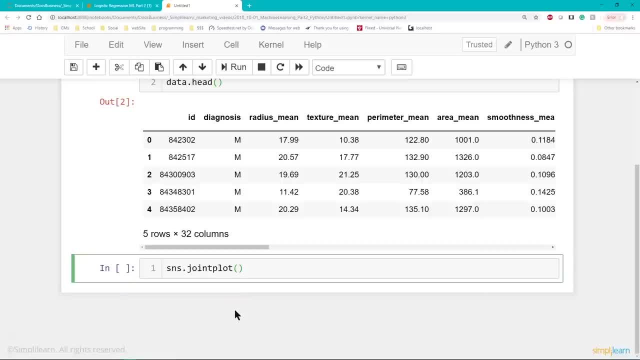 because it is sitting on top of the plot library. So the joint plot does a lot of work for us And we're just going to look at the first two columns that we're interested in: the radius mean and the texture mean. We'll just look at those two columns. 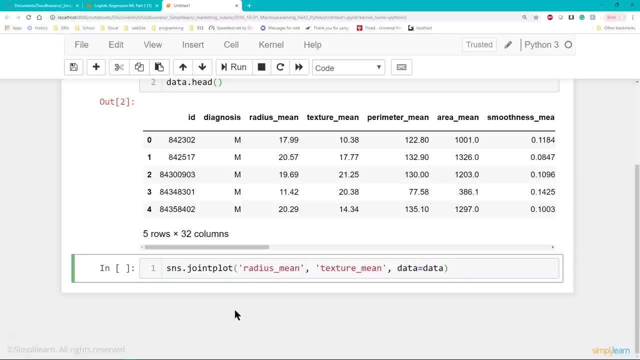 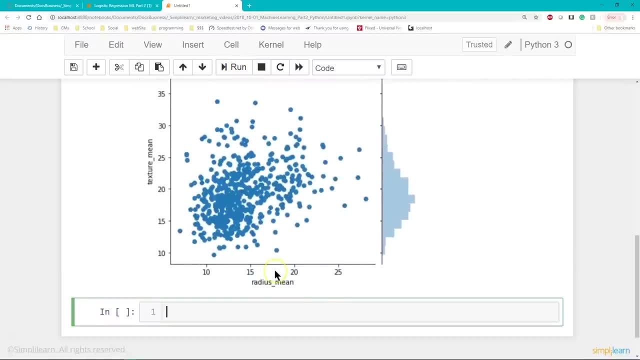 And data equals data. So that tells us which two columns we're plotting and that we're going to use the data that we pulled in. Let's just run that And it generates a really nice graph on here And there's all kinds of cool things. 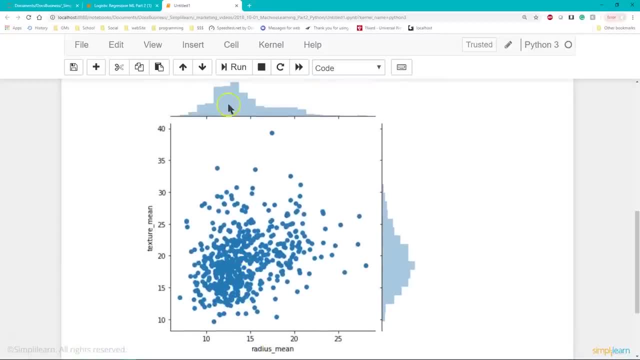 on this graph to look at. I mean we have the texture mean and the radius mean, obviously the axes You can also see- And one of the cool things on here is you can also see the histogram. They show that for the radius mean. 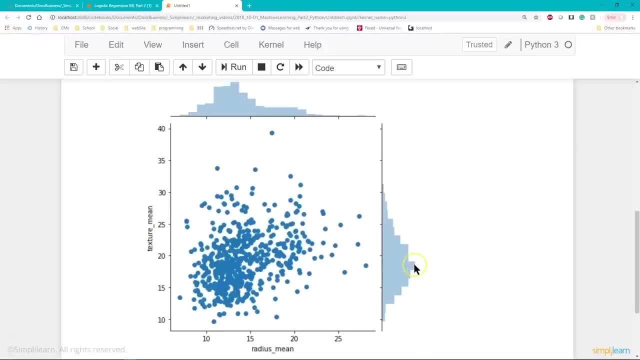 Where does the most common radius mean come up and where the most common texture is. So we're looking at the, The average texture, and on each radius it's average radius. on there It gets a little confusing because we're talking about the individual object's average. 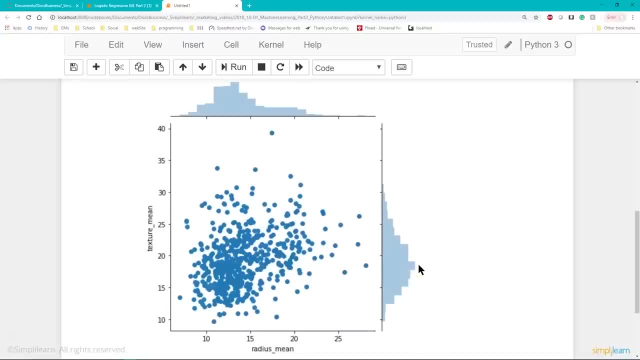 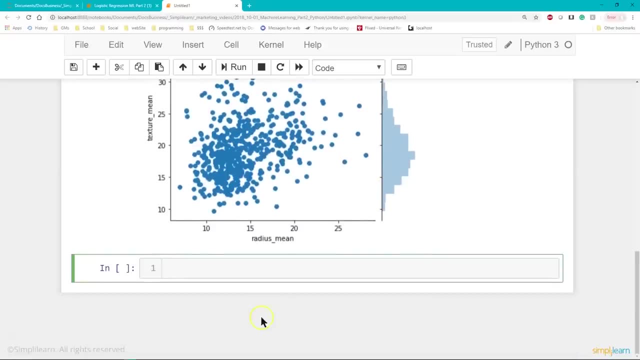 And then we can also look over here and see the histogram showing us the median or how common each measurement is. And that's only two columns, So let's dig a little deeper into Seaborn. They also have a heat map, And if you're not familiar with heat maps, 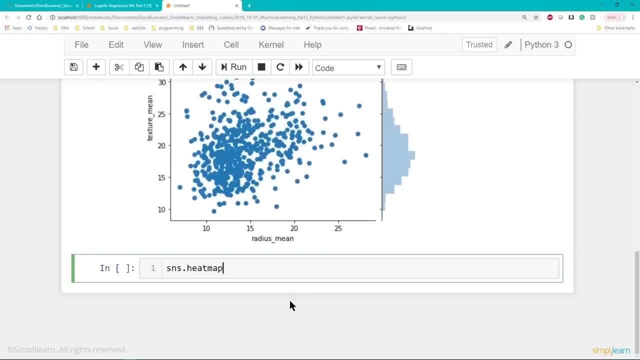 a heat map just means it's in color, That's all that means Heat map. I guess the original ones were plotting heat density on something And so ever since then it's just called a heat map And we're going to take our data. 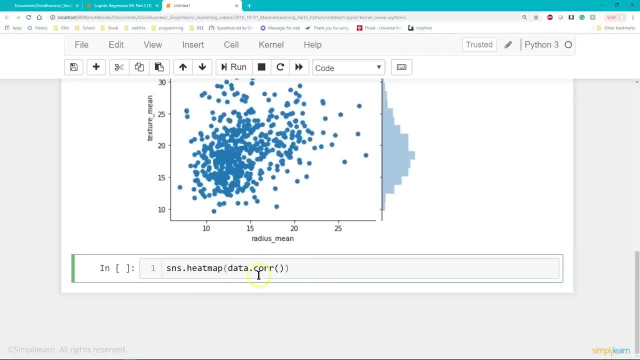 and get our corresponding numbers to put that into the heat map, And that's simply datacorr For that. that's a panda's expression. Just remember we're working in a panda's data frame, So that's one of the cool tools in pandas. 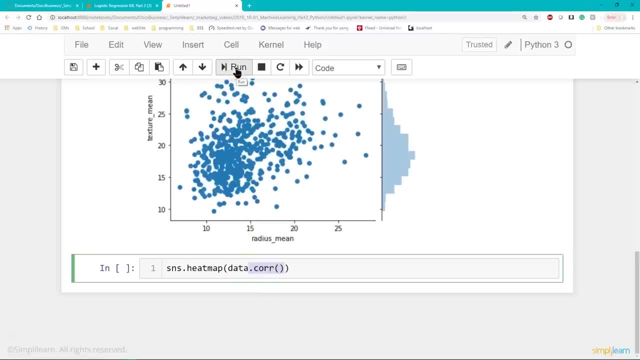 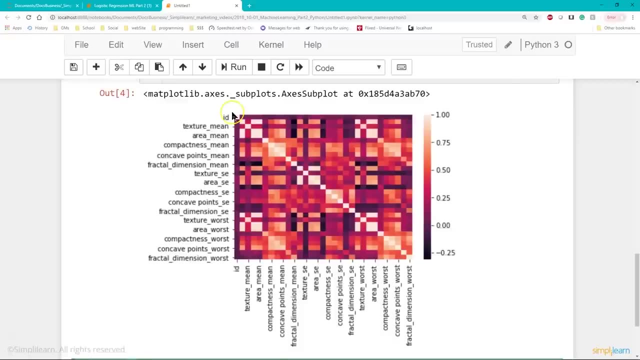 for our data And let's just pull that information into a heat map and see what that looks like, And you'll see that we're now looking at all the different features. We have our ID, we have our texture, we have our area, our compactness. 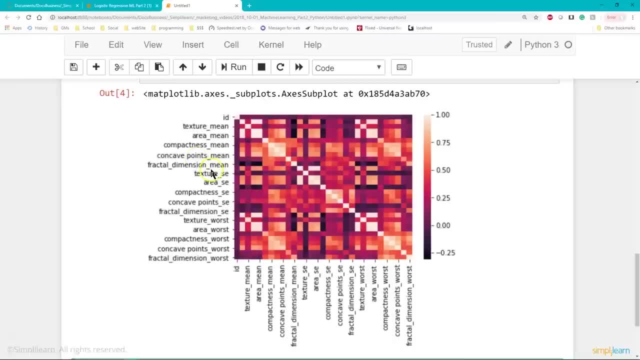 concave points. And if you look down the middle of this chart diagonal, going from the upper left to bottom right, it's all white. That's because when you compare texture to texture, they're identical, So they're a hundred percent. 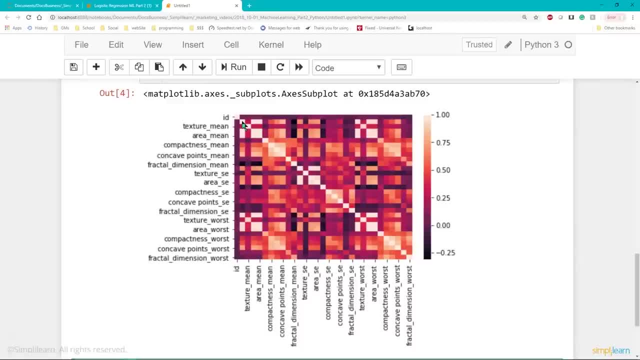 or in this case a perfect one in their correspondence. And you'll see that when you look at say area or right below it, it has almost a black on there in the texture. So these have almost no corresponding data. They don't really form a linear graph. 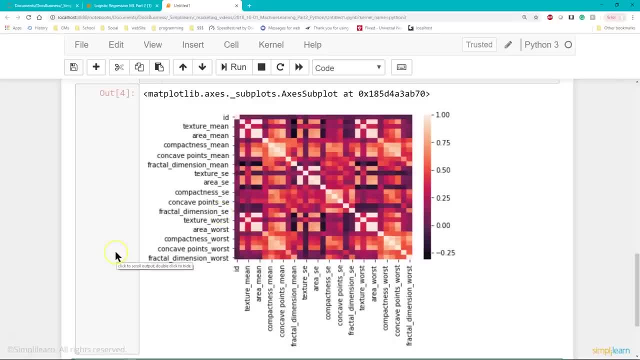 or something that you can look at and say how connected they are. They're very scattered data. This is really just a really nice graph to get a quick look at your data. It doesn't so much change what you do, but it changes verifying. 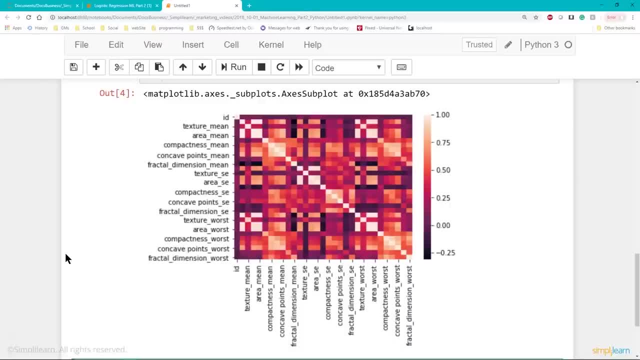 So when you get an answer or something like that, or you start looking at some of these individual pieces, you might go, hey, that doesn't match According to showing our heat map. this should not correlate with each other. You have to start asking: well, why? 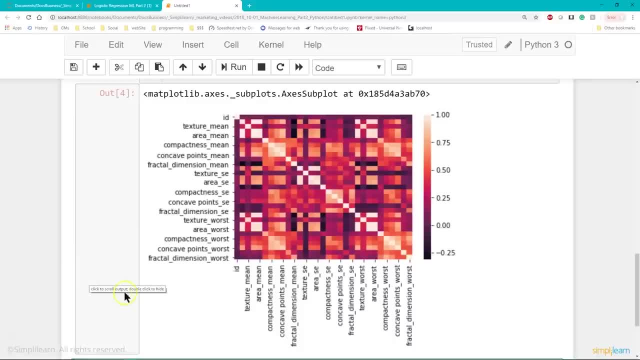 What's going on, What else is coming in there. But it does show some really cool information on here. I mean, we can see from the ID. there's no real one feature. that just says if you go across the top line. 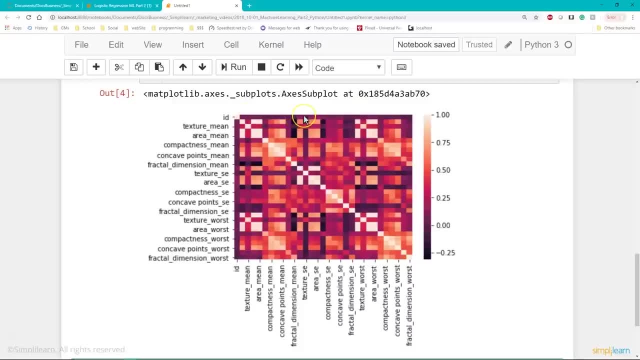 that lights up. There's no one feature that says hey, if the area is a certain size then it's going to be benign or malignant. It says there's some that sort of add up And that's a big hint in the data. 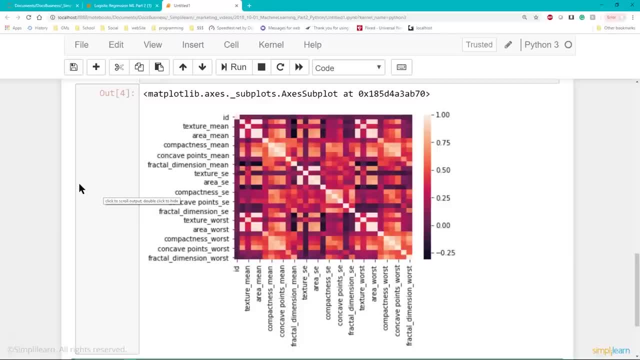 that we're trying to ID this. that's a big hint to us as data scientists to go: okay, we can't solve this with any one feature. It's going to be something that includes all the features, or many of the different features, to come up with a solution for it. 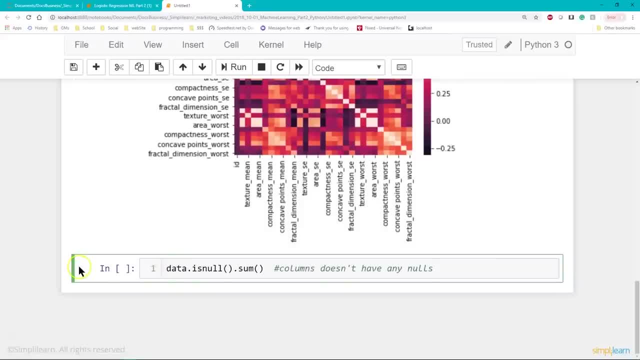 And while we're exploring the data, let's explore one more area and let's look at dataisNull. We want to check for null values in our data. If you remember from earlier in this tutorial we did it a little differently, where we added stuff up and summed them up. 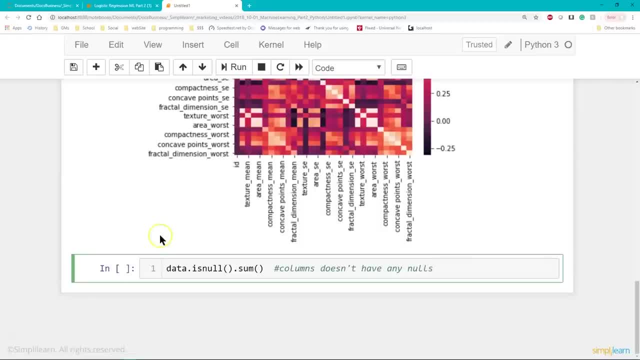 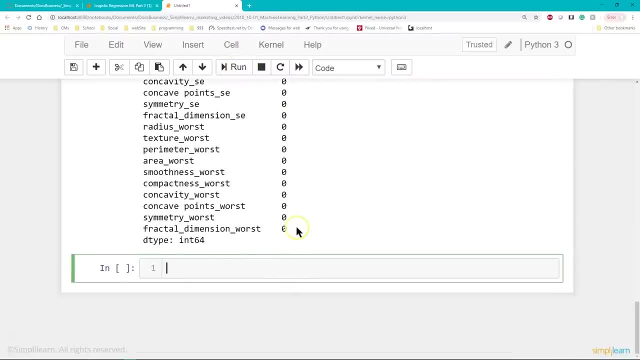 So what we're going to do right now is do it really quickly: dataisNull and summit, and it's going to go across all the columns. So when I run this, you're going to see all the columns come up with no null data. 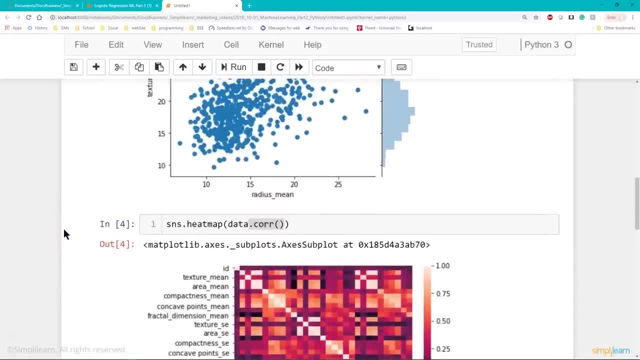 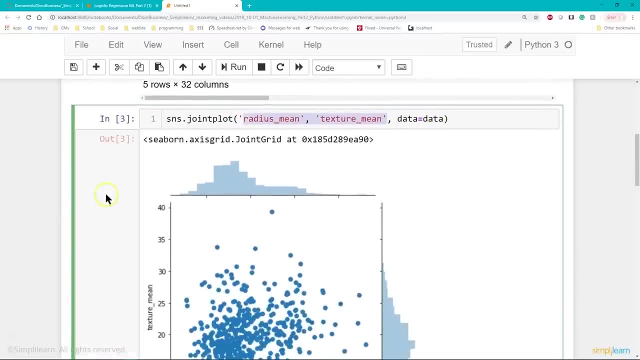 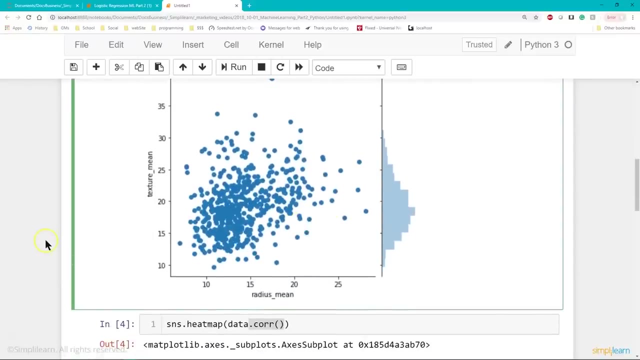 So we've just just to rehash these last few steps. we've done a lot of exploration. We have looked at the first two columns and seen how they plot with the seaborn, with the joint plot which shows both the histogram on the x and y coordinates. 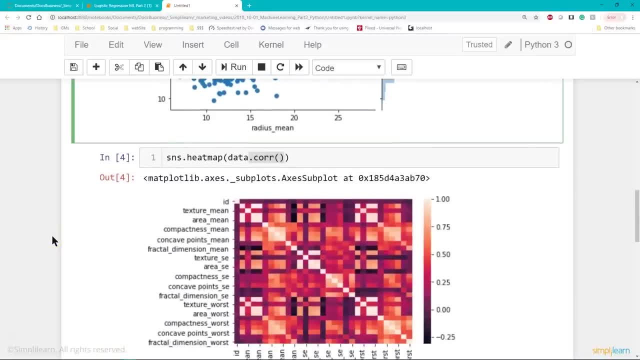 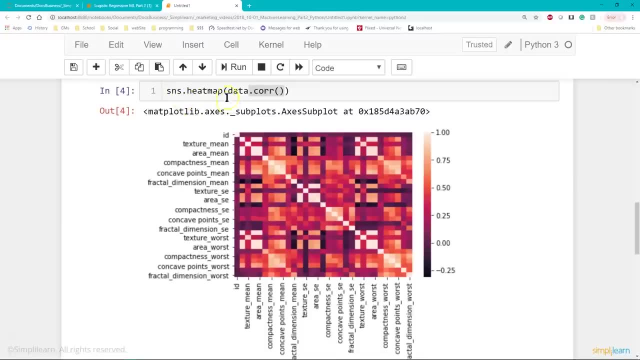 And obviously you can do that more in detail with different columns and see how they plot together. And then we took and did the seaborn heatmap, the snsheatmap of the data, And you can see right here where it did a nice job showing us. 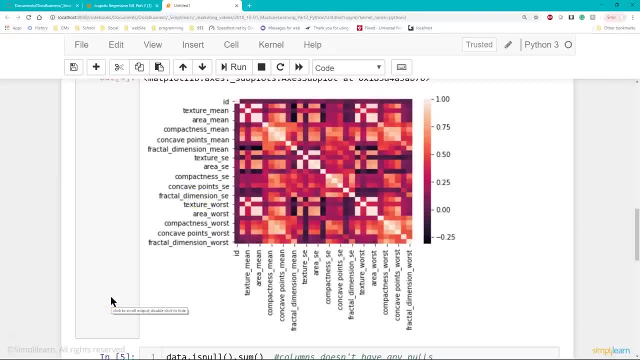 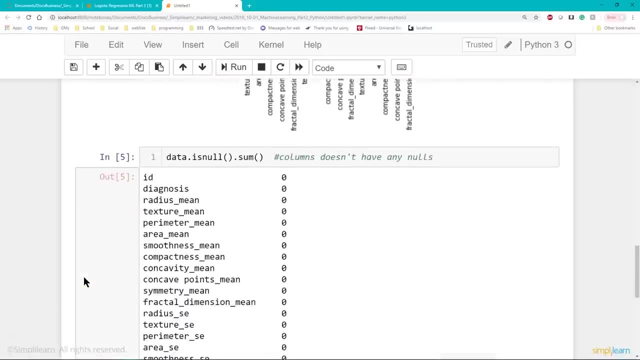 some bright spots where stuff correlates with each other and forms a very nice combination, or points of scattering points, And you can also see areas that don't. And then, finally, we went ahead and checked the data. is the data null value? Do we have any missing data in there? 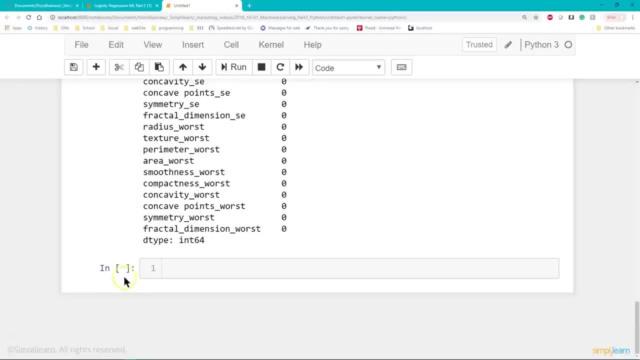 Very important step because it will crash later on. If you forget to do this step, it will remind you when you get that nice error code that says null values. So not a big deal if you miss it, but it's no fun having to go back. 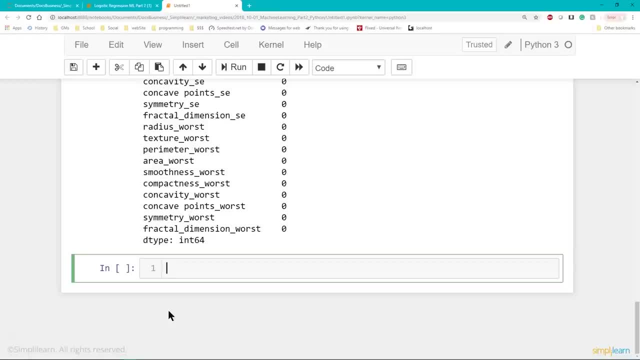 when you're in a huge process and you've missed this step. and now you're ten steps later and you've got to go remember where you were pulling the data in. So we need to go ahead and pull out our x and y. So we just put that down here. 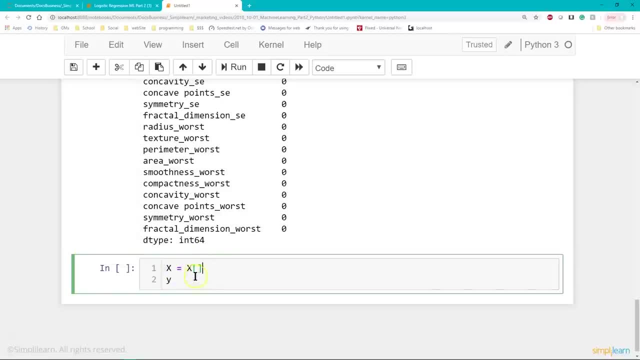 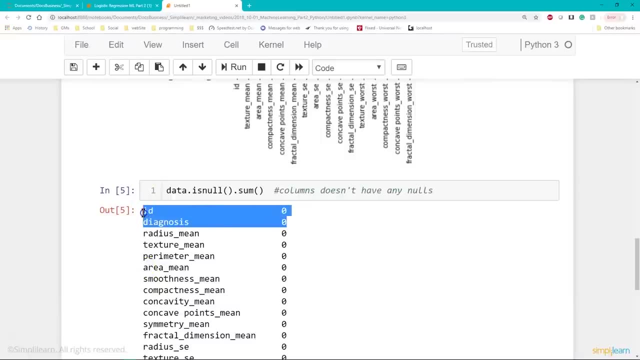 and we'll set the x equal to- and there's a lot of different options here. Certainly we could do: x equals all the columns except for the first two because, if you remember, the first two is the ID and the diagnosis. So that certainly would be an option. 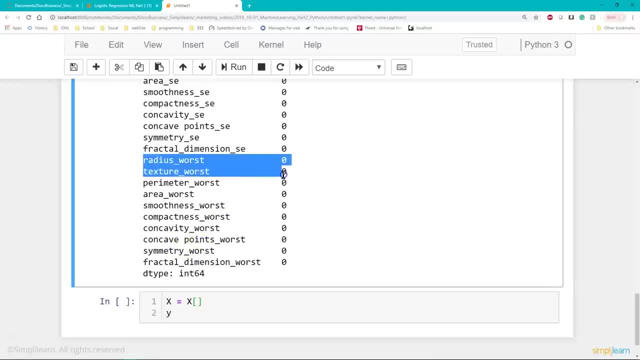 But what we're going to do is we're actually going to focus on the worst: The worst radius, the worst texture, parameter area, smoothness, compactness and so on- One of the reasons to start dividing the data up when you're looking. 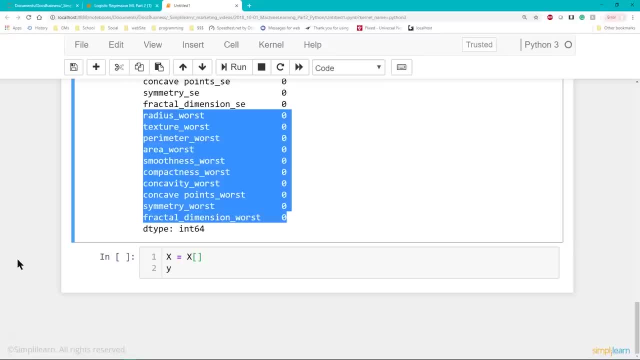 at this information is. sometimes the data will be the same data coming in. So if I have two measurements coming in to my model, it might overweigh them. It might overpower the other measurements because it's basically taking that information in twice. That's a little bit past the scope of this tutorial. 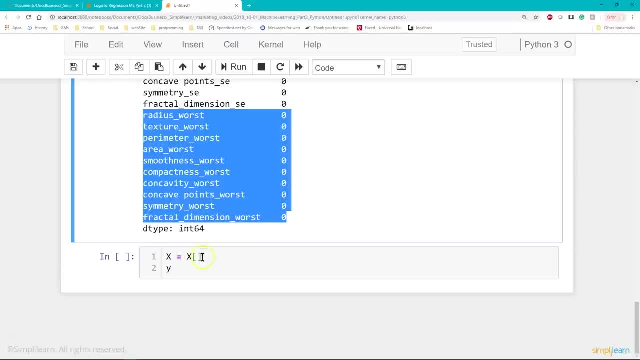 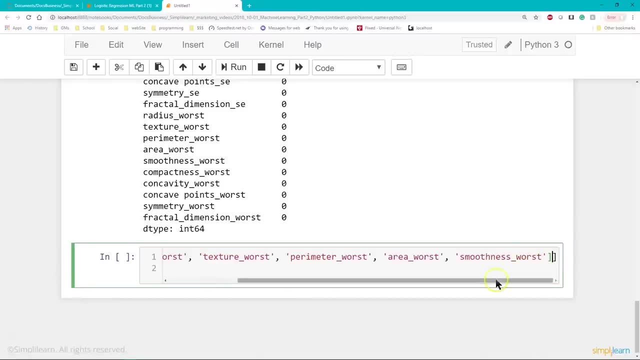 What I want you to take away from this, though, is that we are dividing the data up into pieces, and our team in the back went ahead and said: hey, let's just look at the worst. So I'm going to create an array, and you'll see this array. 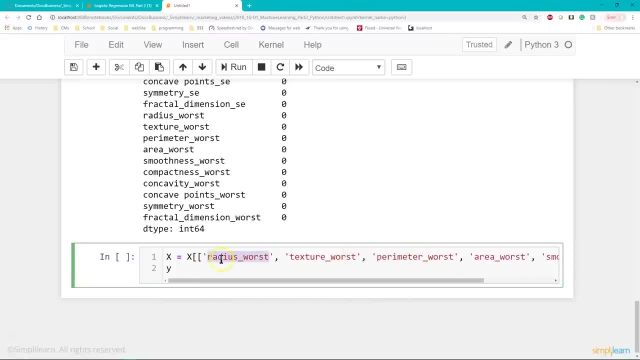 Radius worst, texture, worst, perimeter, worst. We've just taken the worst of the worst and I'm just going to put that in my x. So this x is still a panda's data frame, but it's just those columns And our y, if you remember correctly. 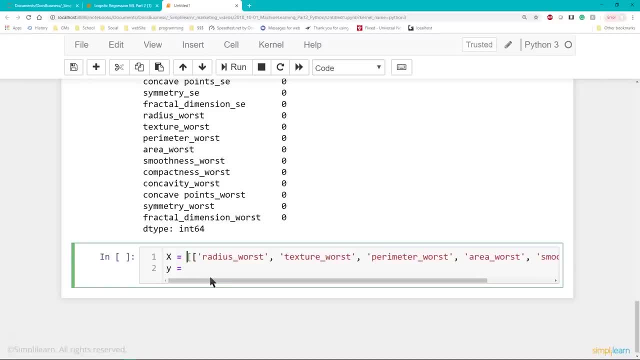 is going to be. it's not x, it's data. There we go, So x equals data, and then it's a list of the different columns, the worst of the worst, And if we're going to take that, we're going to have our answer for our y. 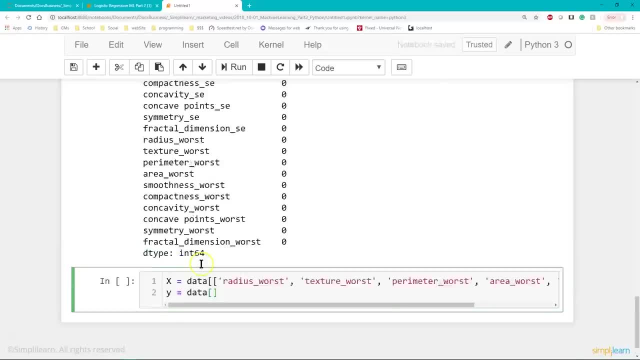 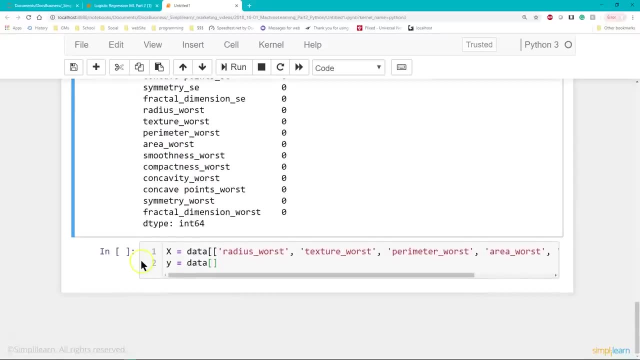 for the stuff we know And, if you remember correctly, we're just going to be looking at the diagnosis. That's all we care about is: what is it diagnosed? Is it benign or malignant? And since it's a single column, we can just do diagnosis. 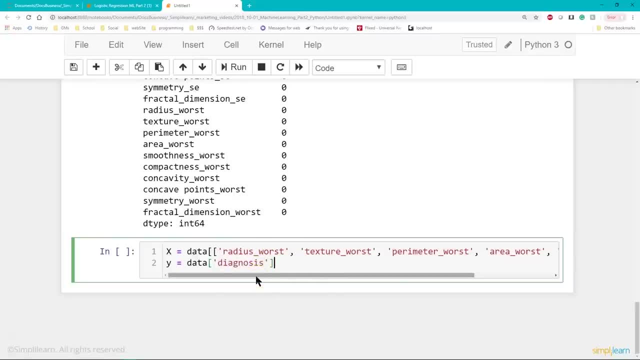 Oh, I forgot to put the brackets. There we go, Okay. So it's just diagnosis on there, and we can also real quickly do like xhead, if you want to see what that looks like, and yhead. So I'm going to go ahead and run this. 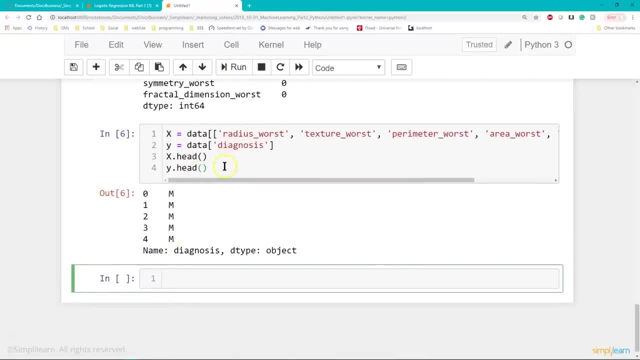 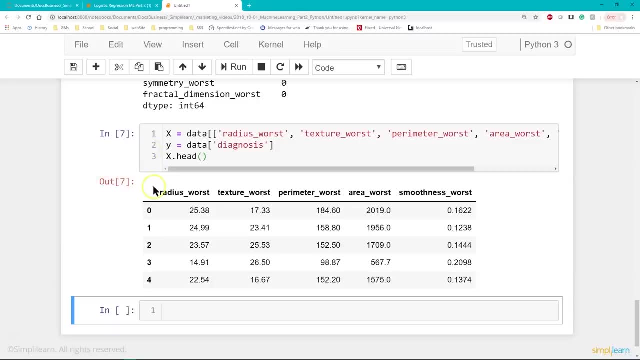 and you'll see it only does the last one. I forgot about that. if you don't do print, You can see that the yhead is just mm, because the first ones are all malignant And if I run this, the xhead is just the first five values. 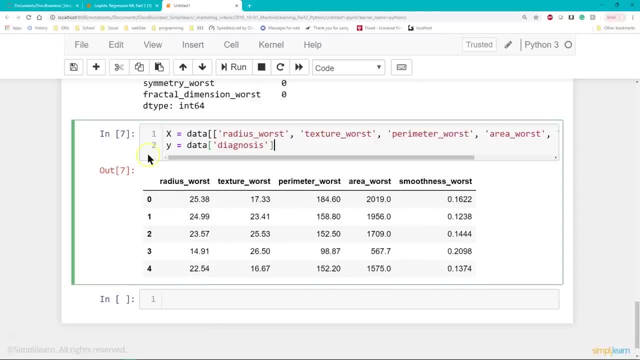 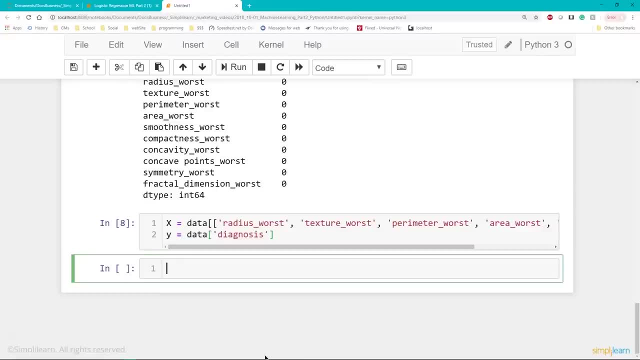 of radius worst, texture worst, parameter, worst area worst, and so on. I'll go ahead and take that out. So, moving down to the next step, we've built our two data sets, our answer and then the features we want to look at. 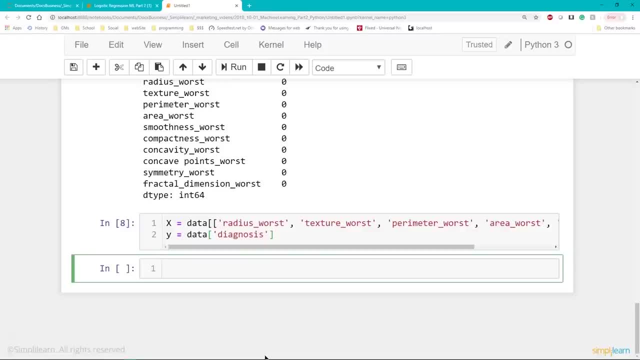 In data science it's very important to test your model. So we do that by splitting the data and from sklearn model selection we're going to import train test split. So we're going to split it into two groups. There are so many ways to do this. 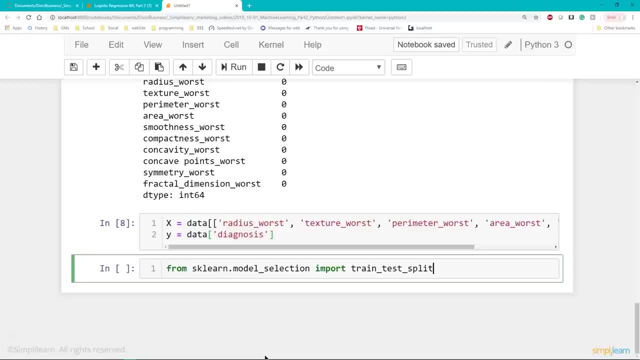 I noticed in one of the more modern ways. they actually split it into three groups and then you model each group and test it against the other groups And there's reasons for that, which is past the scope of this and, for this particular example, isn't necessary. 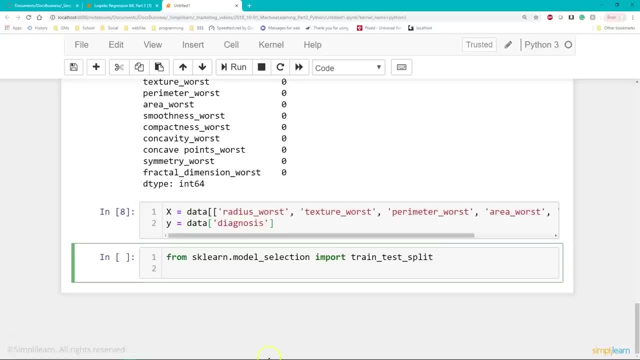 For this. we're just going to split it into two groups: one to train our data and one to test our data And the sklearnmodelselection. we have train test split. You can write your own quick code to do this, where you just randomly. 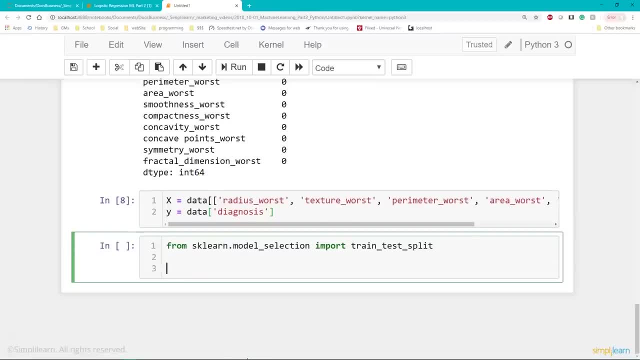 divide the data up into two groups, But they do it for us nicely And we can actually do it where we're going to generate four variables: capital X, train, capital X, test. So we have our training data we're going to use to fit the model. 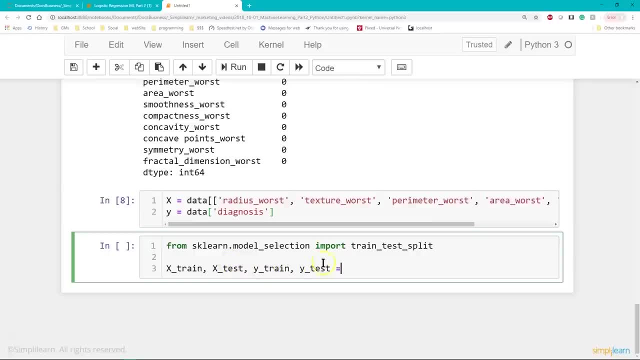 and then we need something to test it And then we have our Y train, so we're going to train the answer and then we have our test. So this is the stuff. we want to see how good it did on our model And we'll go ahead and take our train test split. 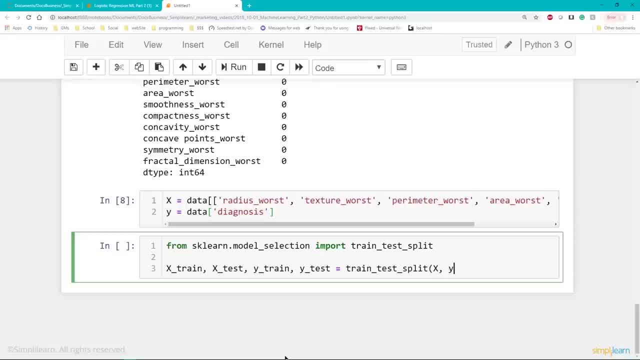 that we just imported And we're going to do X and our Y, our two different data. that's going in back came up and wanted us to go ahead and use a test size equals 0.3.. That's test underscore size, Random state. it's always nice. 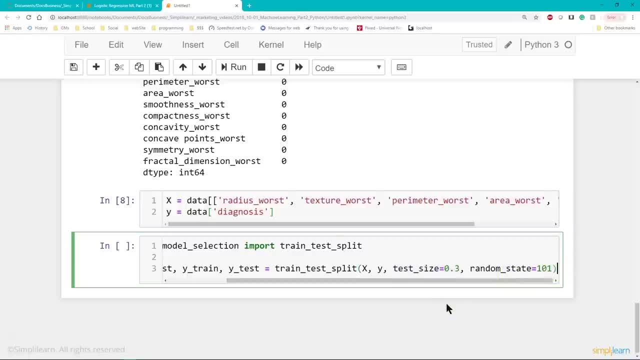 to kind of switch your random state around, but not that important. What this means is that the test size is. we're going to take 30% of the data and we're going to put that into our test variables- our Y test and our X test. 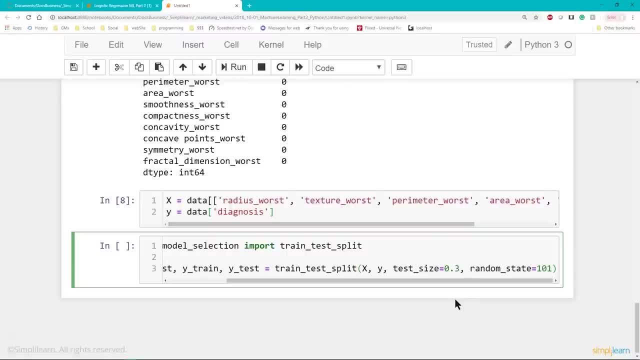 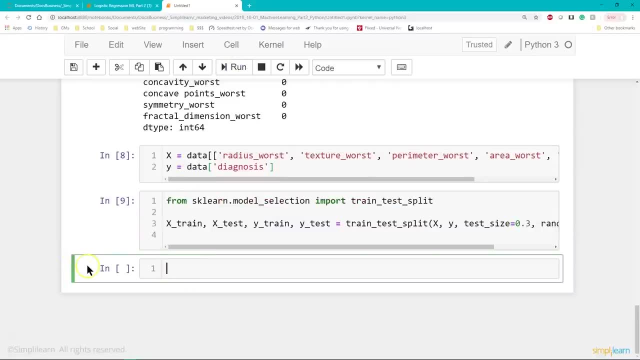 And we're going to do 70% into the X train and the Y train. So we're going to use 70% of the data to train our model and 30% to test it. So let's go ahead and run that and load those up. 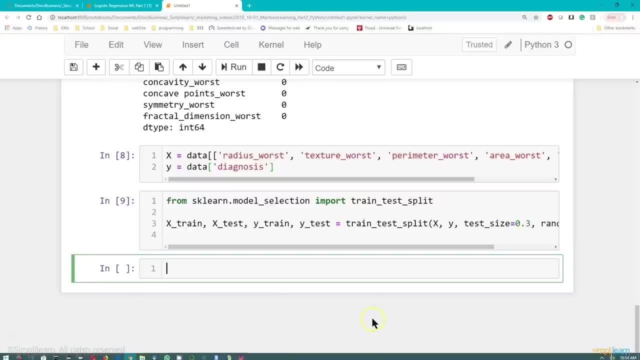 So now we have all our stuff split up and all our data ready to go. Now we get to the actual logistics part. We're actually going to create our model, So let's go ahead and bring that in from sklearn. We're going to bring in. 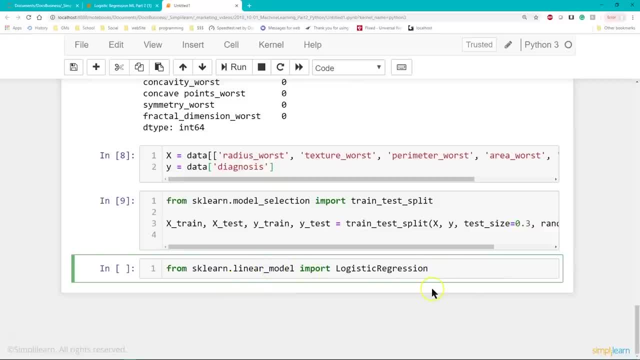 our linear model and we're going to import logistic regression. That's the actual model we're using And we'll call it log model Model And let's just set this equal to our logistic regression that we just imported. So now we have a variable. 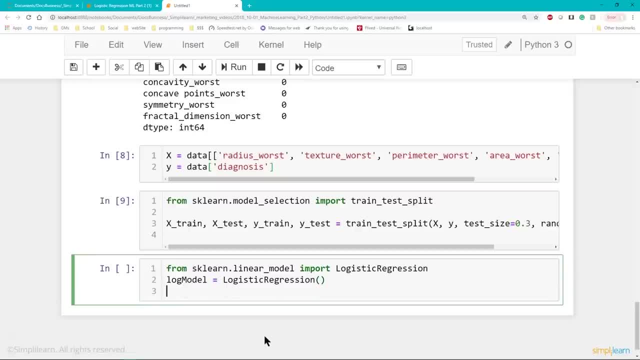 log model set to that class for us to use And with most of the models in the sklearn we just need to go ahead and fix it Fit, Do a fit on there, And we use our X train and we separate it out with our Y train. 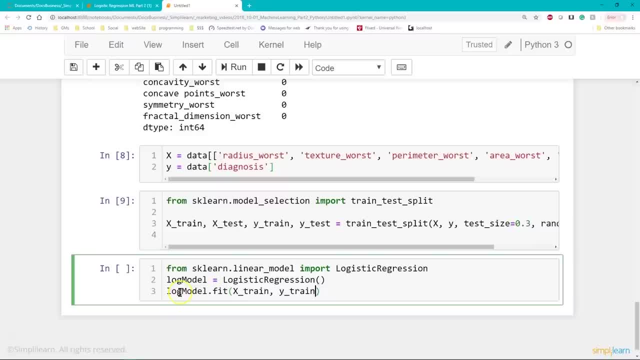 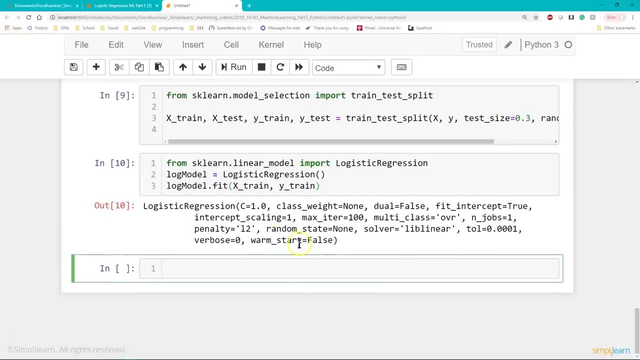 And let's go ahead and run this. So once we've run this, we'll have a model that fits this data, That 70% of our training data, And, of course, it prints this out that tells us how many different variables you can set on there. 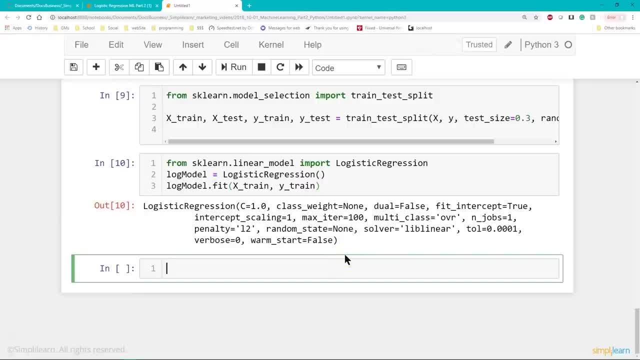 There's a lot of different choices you can make, But for WordDo we're just going to let all the defaults set. We don't really need to mess with those on this particular example. There's nothing in here that really stands out as super important, until you start. 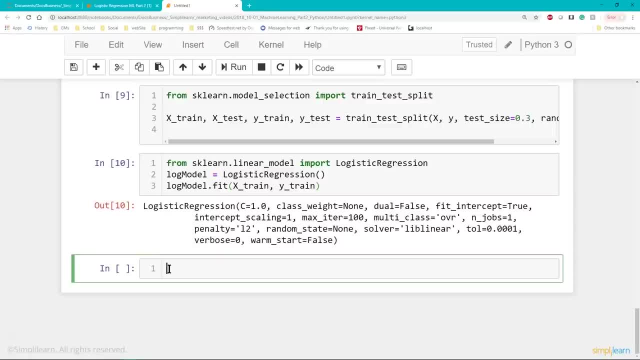 fine tuning it, But for what we're doing, the basics will work just fine. And then let's- we need to go ahead and test out our model. Is it working? So let's create a variable: Y predict. And this is going to be. 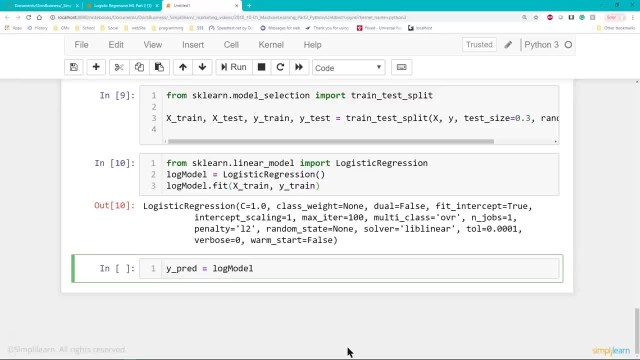 equal to our log model And we want to do a predict. Again, very standard format for the sklearn library is taking your model and doing a predict on it And we're going to test Y predict against the Y test. So we want to know what the model thinks it's going to be. 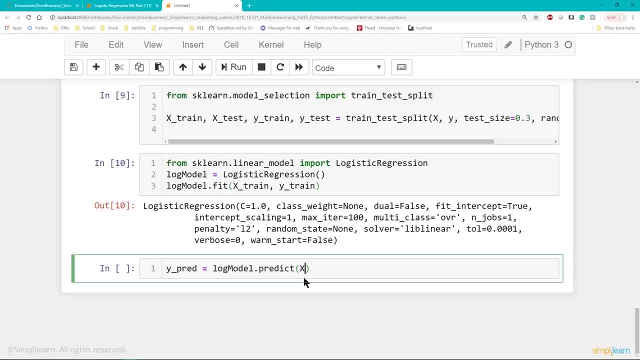 That's what our Y predict is And with that we want the X test. So we have our train set and our test set And now we're going to do our Y predict And let's go ahead and run that. And if we 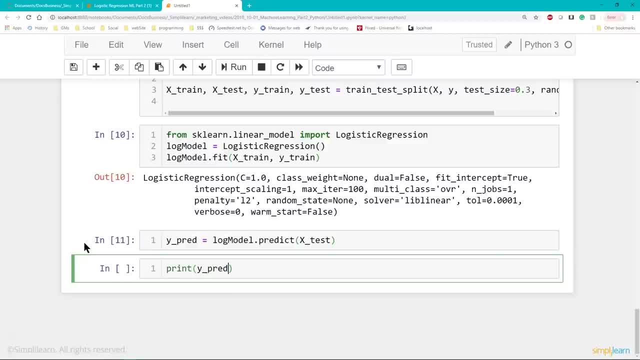 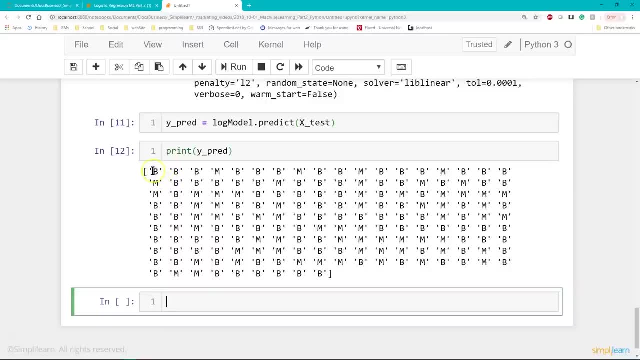 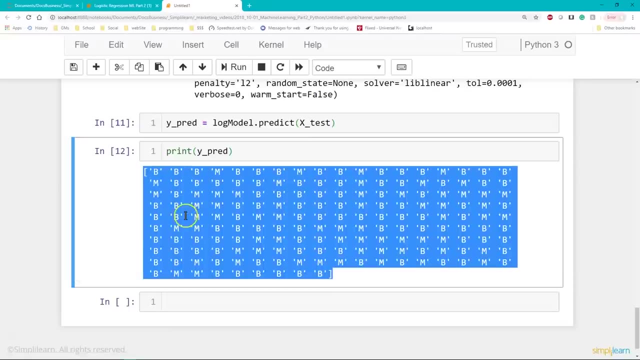 print Y: predict. Let me go ahead and run that, You'll see. it comes up and it prints a nice array of B and M for benign and malignant, For all the different test data we put in there. So it does pretty good. We're not sure exactly how. 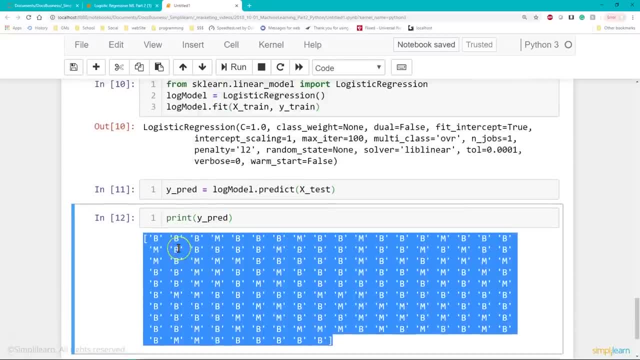 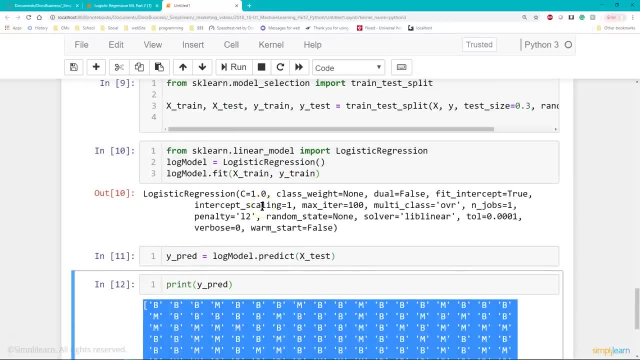 good it does, but we can see that it actually works and is functional. It was very easy to create. You'll always discover with our data science that as you explore this, you spend a significant amount of time prepping your data and making sure your data coming in is good. 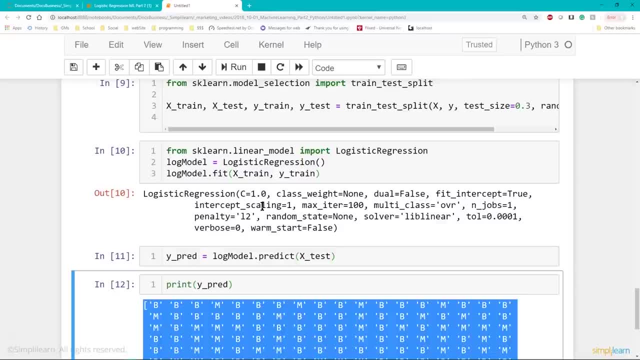 There's a saying: good data in good answers out, Bad data in bad answers out. That's only half the thing. That's only half of it. Selecting your models becomes the next part, as far as how good your models are. And then, of course, 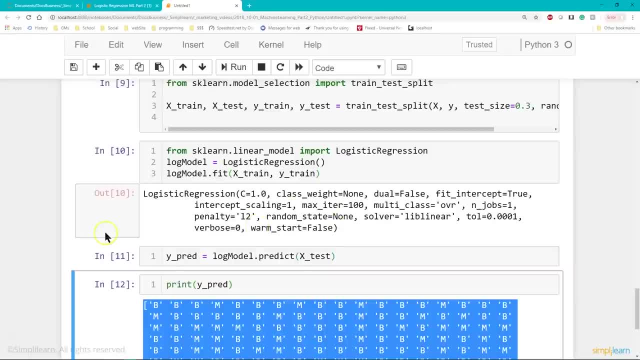 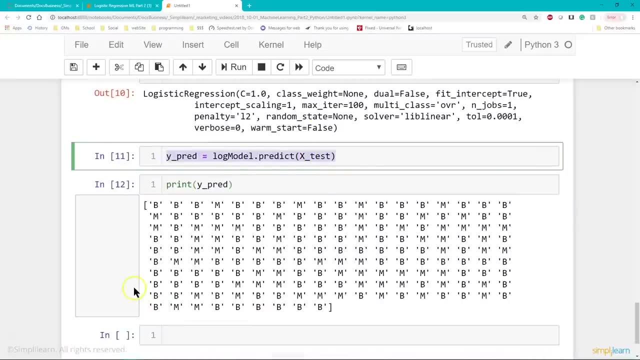 fine tuning it depending on what model you're using. So we come in here. we want to know how good this came out. So we have our Y predict here, log model predict X test. So for deciding how good our model is, we're going to go. 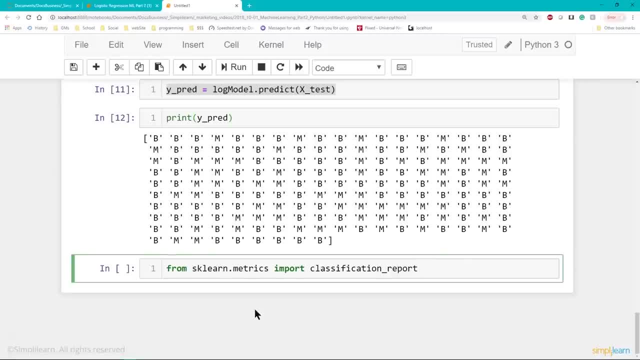 from the sklearnmetrics. we're going to import classification report And that just reports how good our model is doing And then we're going to feed it the model data. Let's just print this out And we'll take our classification report and we're going to put into there. 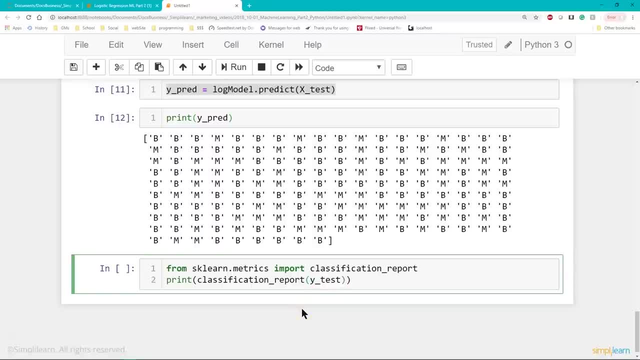 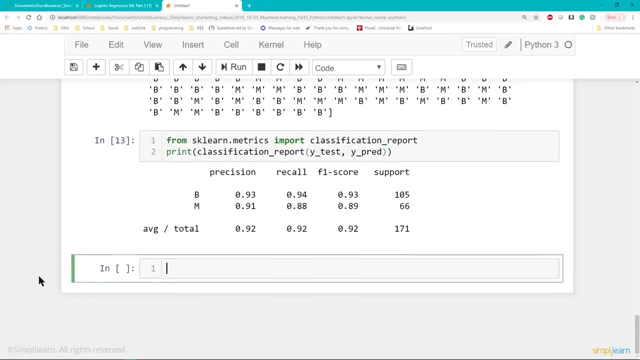 our test, our actual data. so this is what we actually know is true and our prediction, what our model predicted for that data on the test side. And let's run that and see what that does. So we pull that up, you'll see that we have. 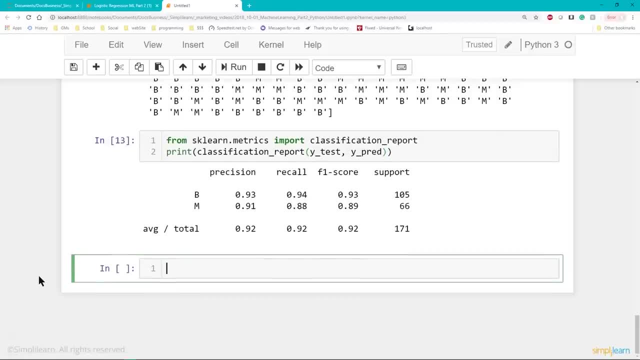 a precision for a benign and malignant B and M, And we have a precision of 93 and 91, a total of 92, so it's kind of the average between these two of 92.. There's all kinds of different information on here. Your F1 score. 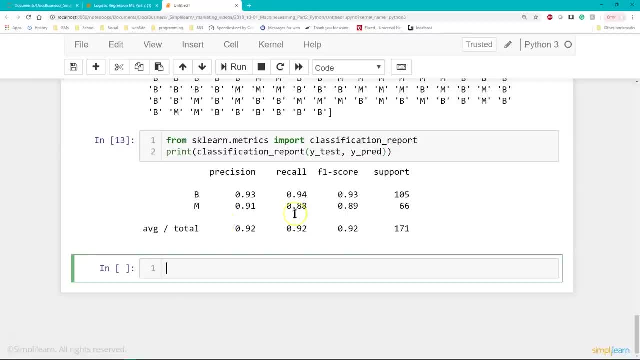 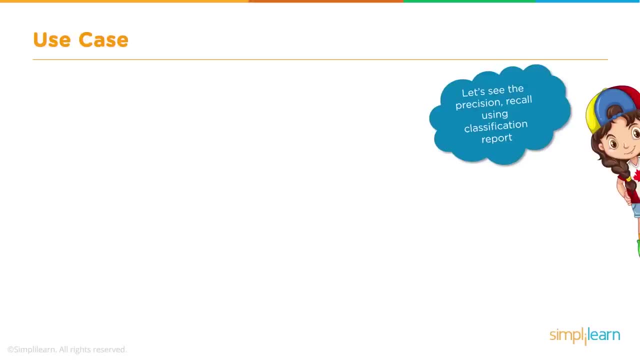 your recall, your support coming through on this, And for this I'll go ahead and just flip back to our slides that they put together for describing it. And so here we're going to look at the precision using the classification report, And you'll see, this is the same printout I had up. 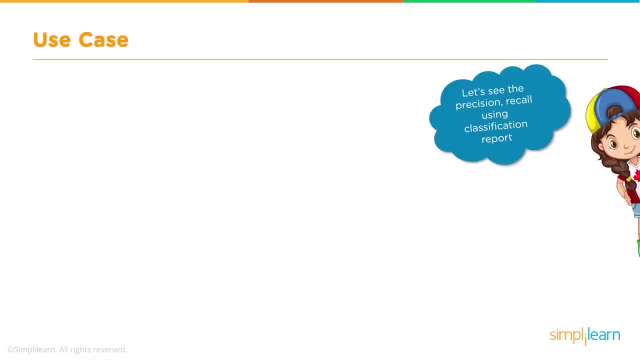 above. Some of the numbers might be different because it does randomly pick out which data we're using. So this model is able to predict the type of tumor with 91% accuracy. So we look back here. you'll see where we have benign and malignant. 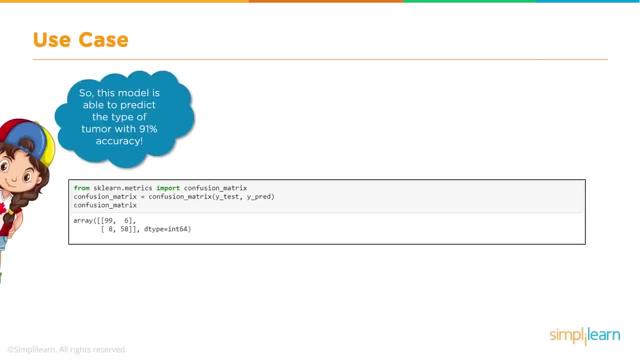 It actually is 92 coming up here. We're looking at about a 92, 91% precision And remember, I reminded you about domains And we're talking about the domain of a medical domain with a very catastrophic outcome, You know, at 91 or 92%. 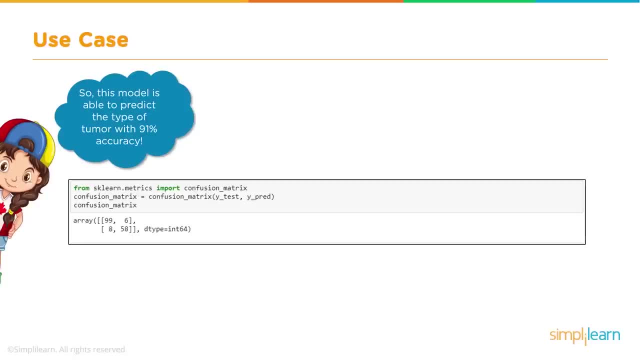 precision, you're still going to go in there and have somebody do a biopsy on it. Very different than if you're investing money and there's a 92% chance you're going to earn 10% and 8% chance you're going to lose 8%. 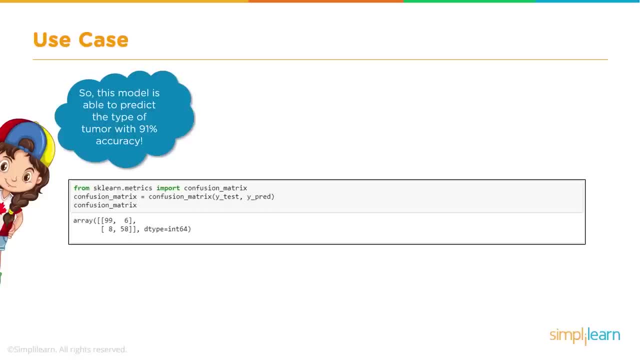 You're probably going to bet the money Because at that odds it's pretty good that you'll make some money And in the long run, if you do that enough, you definitely will make money. And also with this domain, I've actually seen them use. 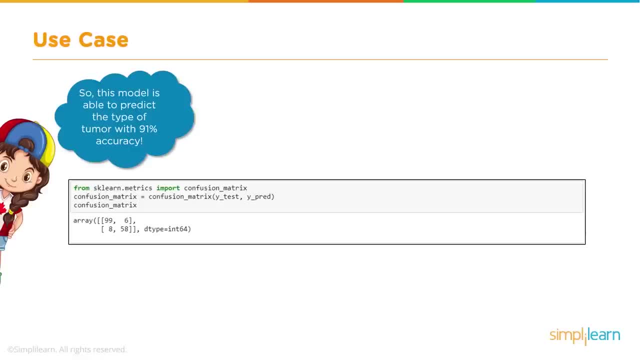 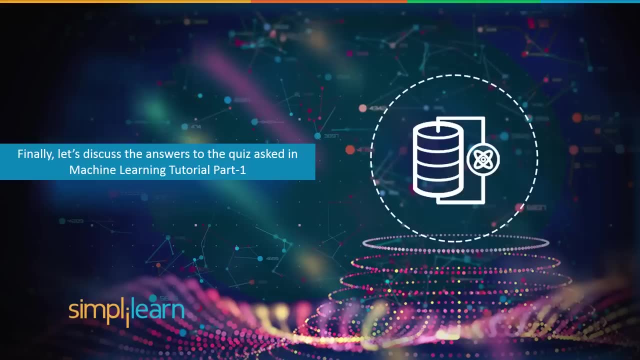 this to identify different forms of cancer. That's one of the things that they're starting to use these models for, Because then it helps the doctor know what to investigate. So that wraps up this section. Finally, we're going to go in there and let's discuss the answer to the quiz. 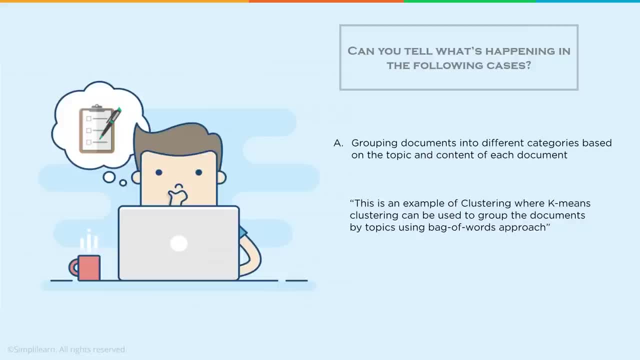 asked in Machine Learning Tutorial, Part 1.. Can you tell what's happening in the following cases? Grouping documents into different categories based on the topic and content of each document? This is an example of clustering where k-means clustering can be used to. 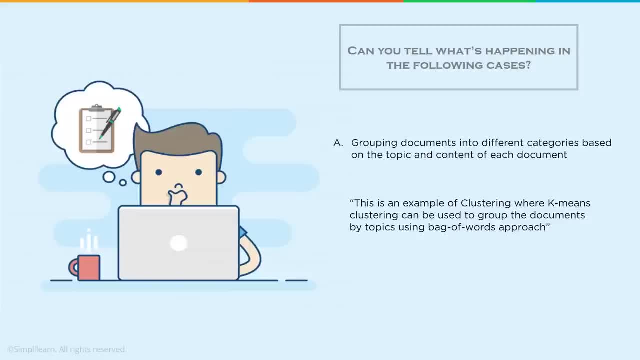 group the documents by topics using bag-of-words approach. So if you've gotten in there that you're looking for clustering- and hopefully you had at least one or two examples like k-means that are used for clustering different things- then give yourself a two thumbs up. 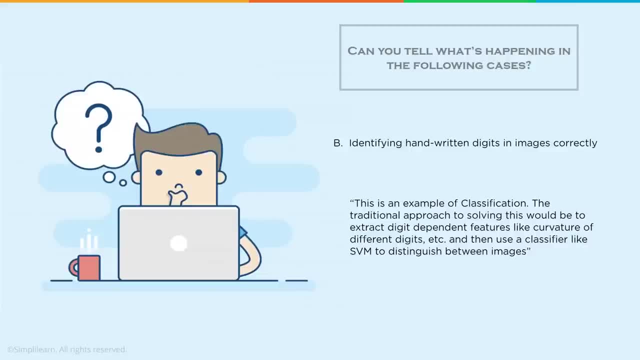 B- Identifying handwritten digits and images correctly. This is an example of classification. The traditional approach to solving this would be to extract digit-dependent features like curvature of different digits etc. And then use a classifier like SVM to distinguish between images. 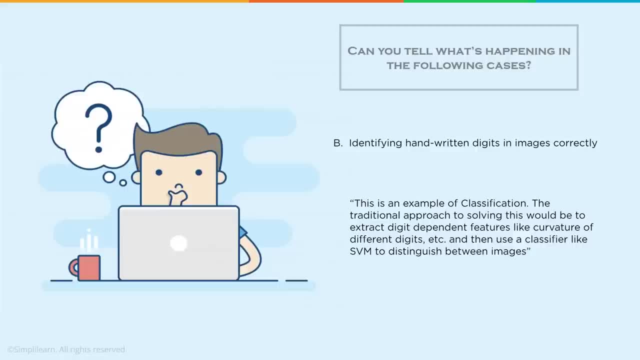 Again, if you got the fact that it's a classification example, give yourself a thumb up. And if you're able to go, hey, let's use SVM or another model for this, give yourself those two thumbs up on it. C Behavior. 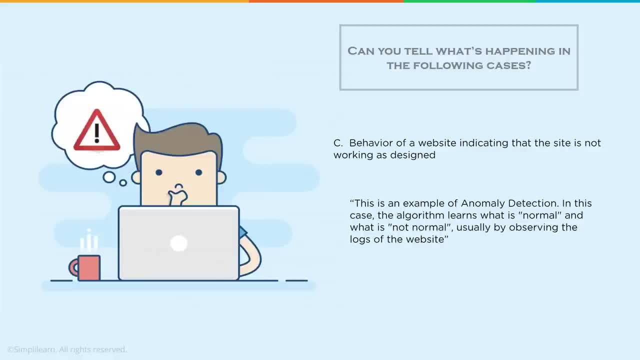 of a website indicating that the site is not working as designed. This is an example of anomaly detection. In this case, the algorithm learns what is normal and what is not normal, Usually by observing the logs of the website. Give yourself a thumbs up if you. 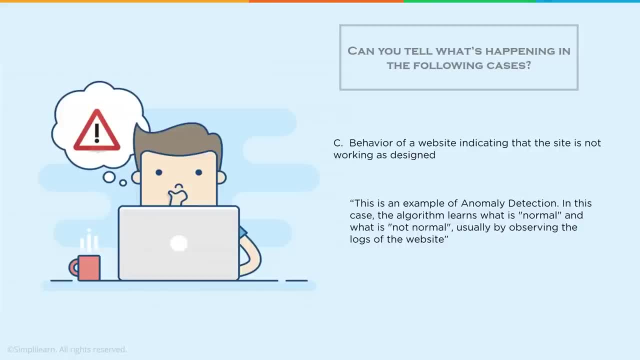 got that one And just for a bonus, can you think of another example of anomaly detection? One of the ones I use it for in my own business is detecting anomalies in stock markets. Stock markets are very fickled and they behave very radical, So finding 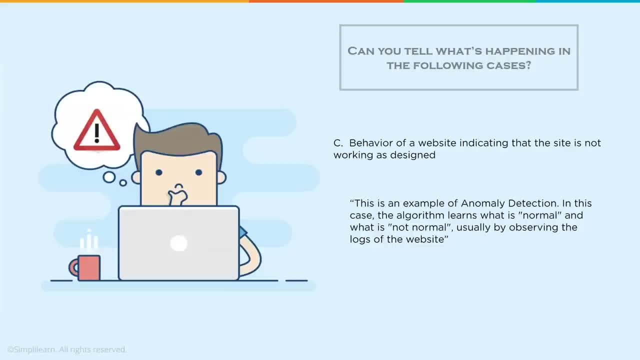 those erratic areas and then finding ways to track down why they're erratic. was something released in social media? It was something released. You can see where knowing where that anomaly is can help you to figure out what the answer is to it. in another area. 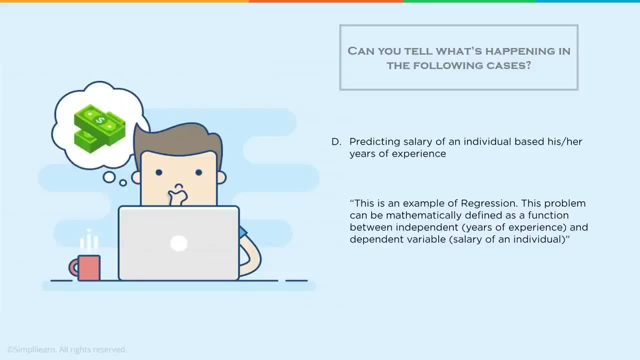 D, Predicting salary of an individual based on his or her years of experience. This is an example of regression. This problem can be mathematically defined as a function between independent years of experience and dependent variables- salary of an individual And if 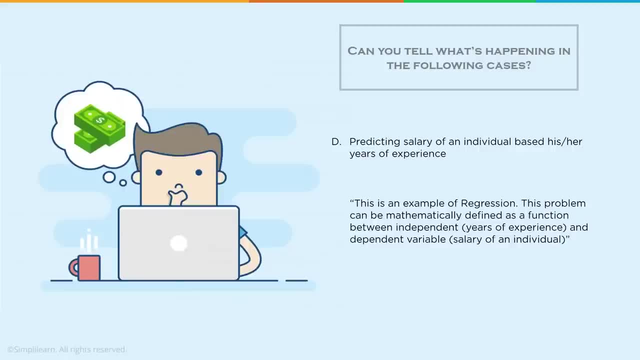 you guessed that this was a regression model, give yourself a thumbs up. And if you're able to remember that it is between independent and dependent variables and that terms, give yourself two thumbs up. Machine learning has improved our lives in a number of wonderful ways. 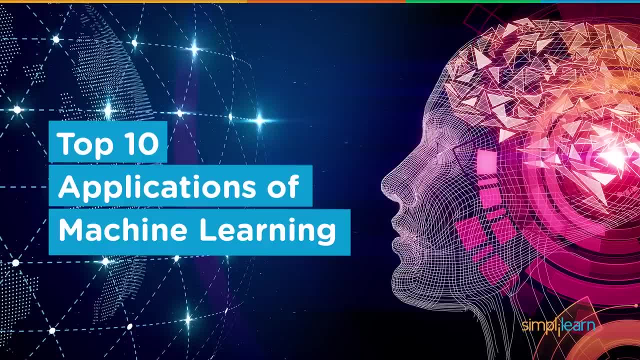 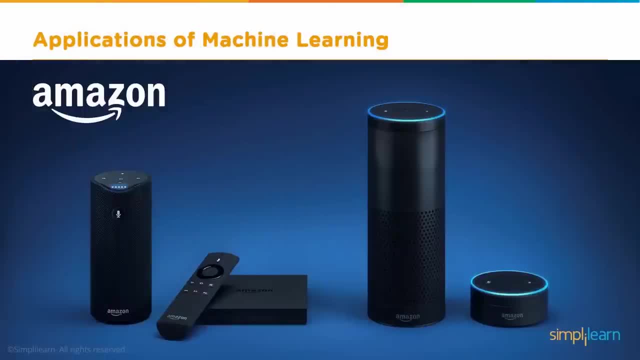 Today. let's talk about some of these. I'm Rahul from Simply Learn, and these are the top ten applications of machine learning. First, let's talk about virtual personal assistants: Google Assistant, Alexa, Cortana and Siri. Now we've all used one of these. 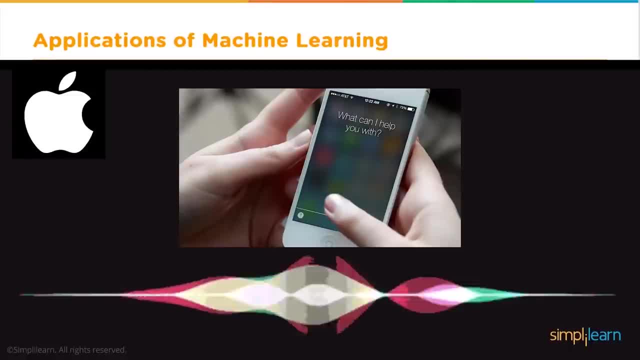 at least at some point in our lives. Now, these help improve our lives in a great number of ways. For example, you could tell them to call someone, You could tell them to play some music. You could tell them to even schedule an appointment. 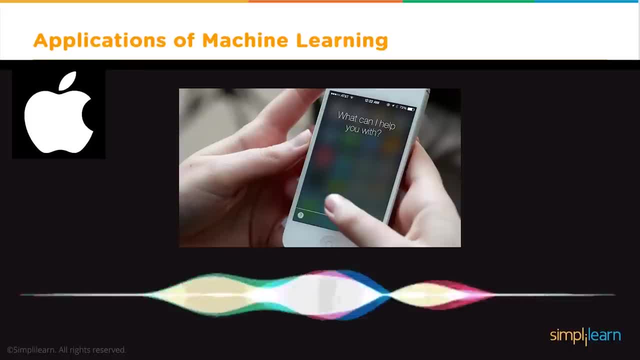 So how do these things actually work? First, they record whatever you're saying, send it over to a server, which is usually in a cloud, decode it with the help of machine learning and neural networks, and then provide you with an output. So if you've ever noticed, 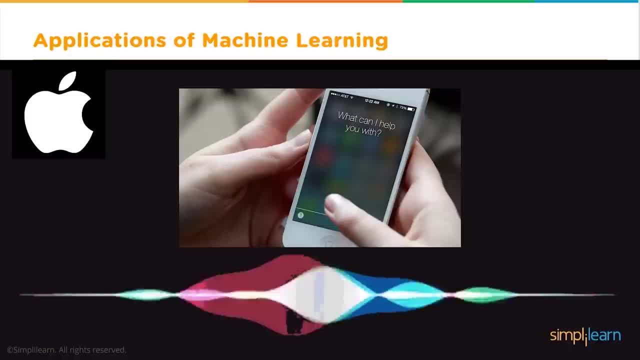 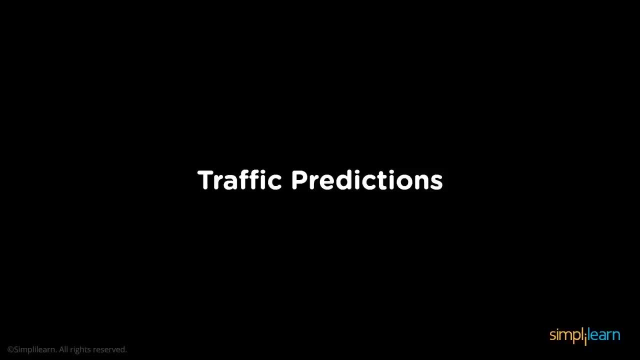 that these systems don't work very well without the internet. that's because the server couldn't be contacted. Next, let's talk about traffic predictions. Now, say I wanted to travel from Buckingham Palace to Lord's Cricket Ground, The first thing I'd 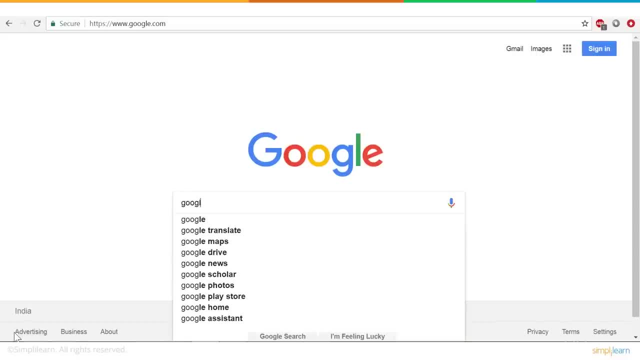 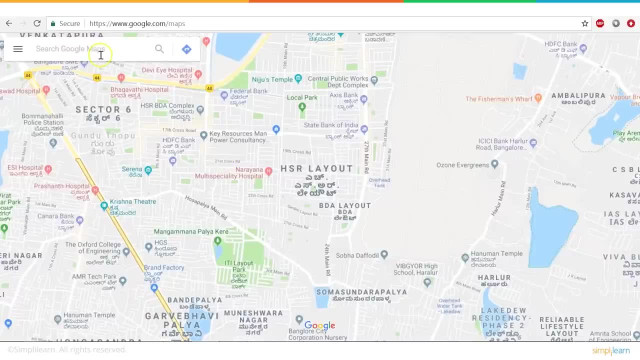 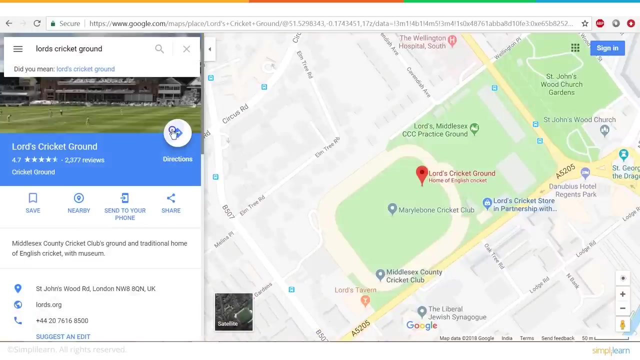 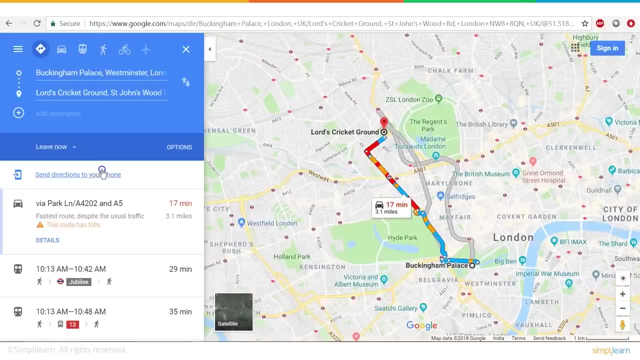 probably do is to get on Google Maps, So search it. So here we have the path you should take to get to Lord's Cricket Ground. Now here, the map is a combination of red, yellow and blue. 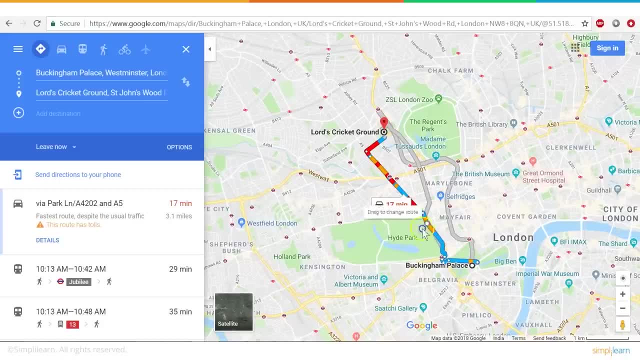 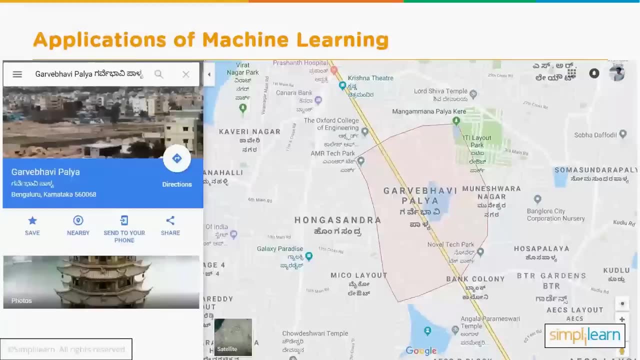 But the blue regions signify a clear road, That is, you won't encounter traffic there. Yellow indicates that they're slightly congested and red means they're heavily congested. So let's look at the map- a different version of the same map. 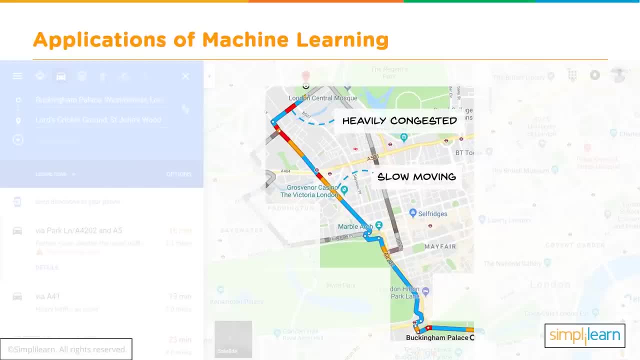 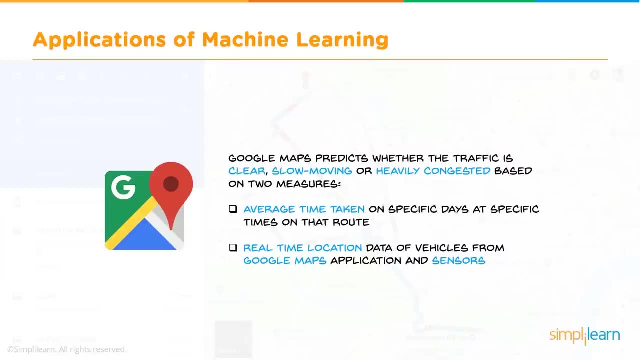 And here, as I told you before, red means heavily congested, yellow means slow moving and blue means clear. So how exactly is Google able to tell you that the traffic is clear, slow moving or heavily congested? So this is with the help of machine learning. 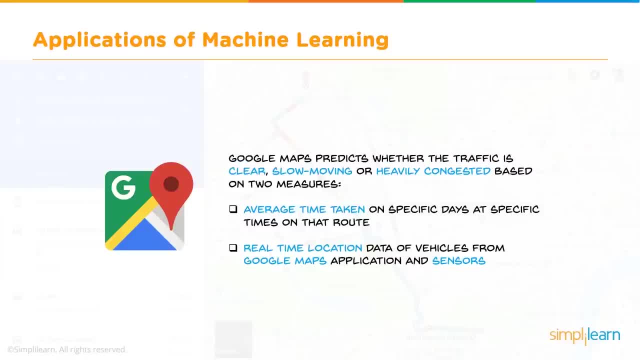 and with the help of two important measures. First is the average time that's taken on specific days at specific times on that route. The second one is the real-time location data of vehicles from Google Maps and with the help of sensors. 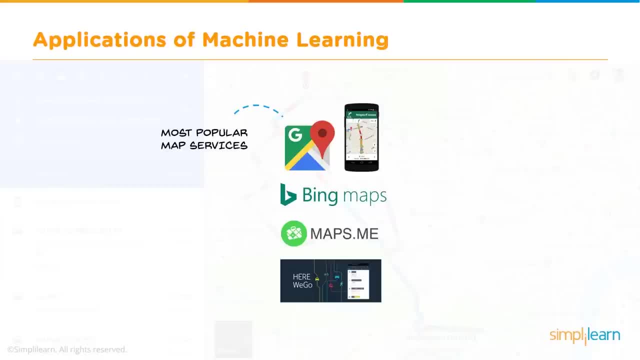 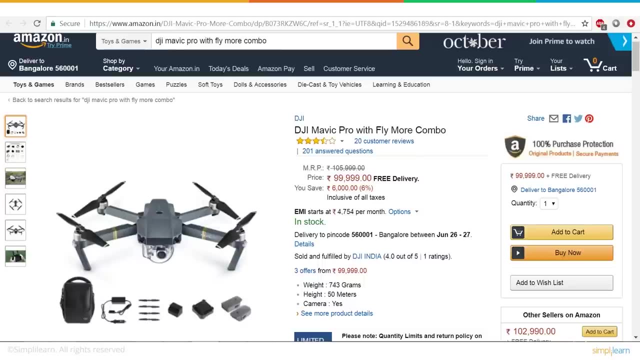 Some of the other popular map services are Bing Maps, Mapsme, and here we go. Next up, we have social media personalization. So say, I want to buy a drone and I'm on Amazon and I want to buy a DJI Mavic Pro. 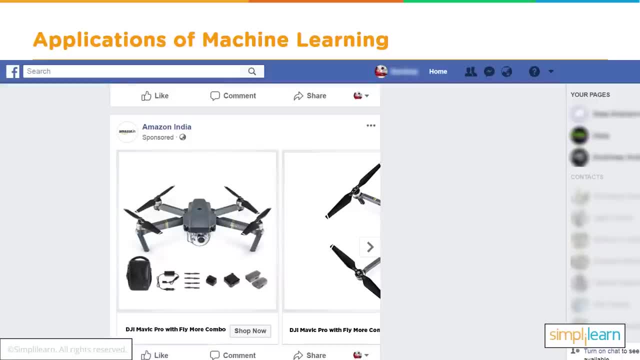 The thing is it's close to one lap, so I don't want to buy it right now, But the next time I'm on Facebook, I'll see an advertisement for the product. Next time I'm on YouTube, I'll see an advertisement. Even on Instagram. 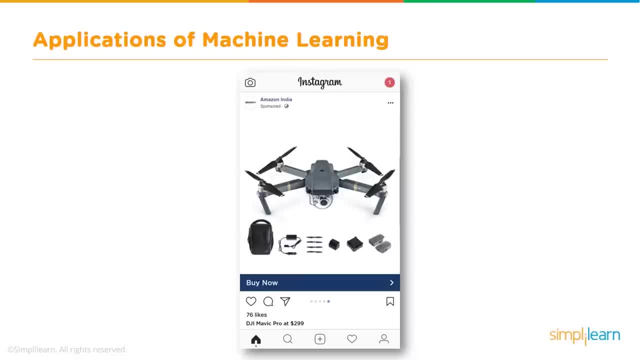 I'll see an advertisement. So here, with the help of machine learning, Google has understood that I'm interested in this particular product, Hence it's targeting me with these advertisements. This is also with the help of machine learning. Let's talk about email spam. 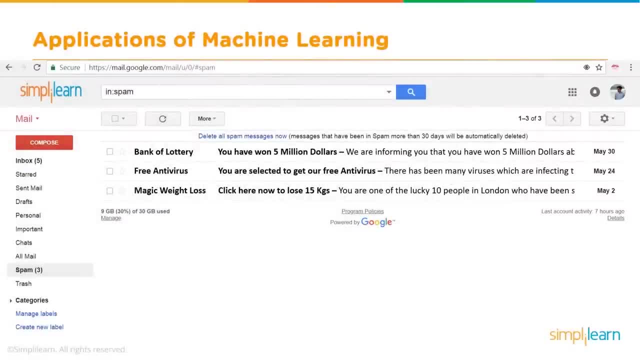 filtering. Now this is the spam that's in my inbox. Now how does Gmail know what's spam and what's not spam? So Gmail has an entire collection of emails which have already been labeled as spam or not spam. So, after analyzing, 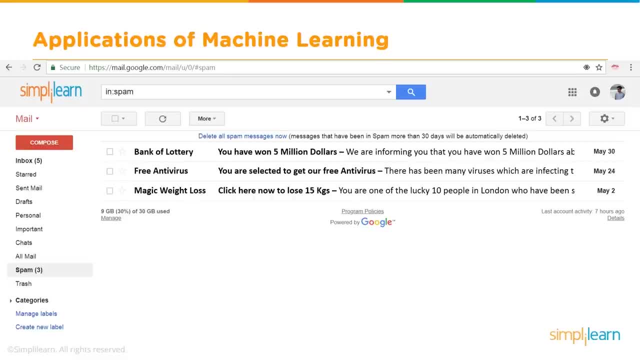 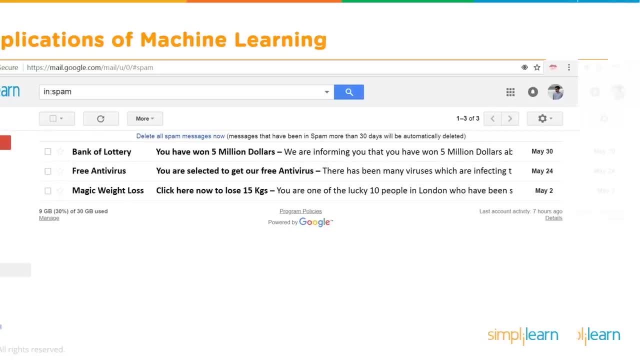 this data, Gmail is able to find some characteristics like the word lottery or winner. From then on, any new email that comes to your inbox goes through a few spam filters to decide whether it's spam or not. Now some of the popular 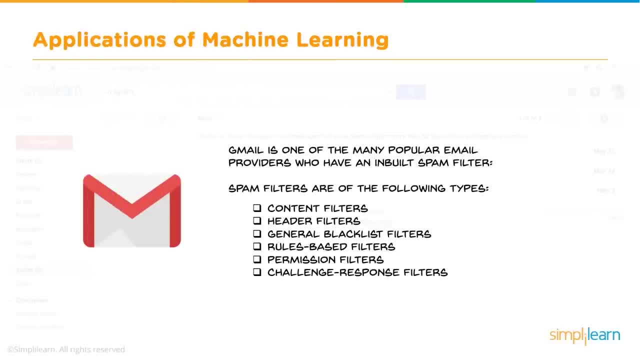 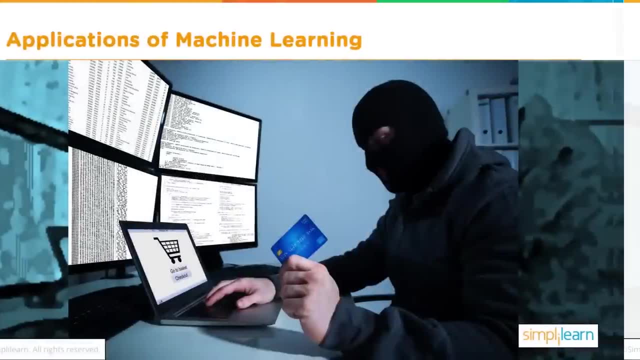 spam filters that Gmail uses is content filters, header filters, general blacklist filters and so on. Next, we have online fraud detection. Now there are several ways that online fraud can take place. For example, there's identity theft, where they steal your identity. 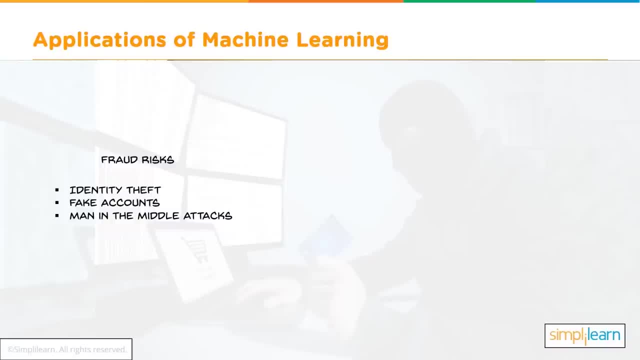 fake accounts, where these accounts only last for how long the transaction takes place and stop existing after that. and man-in-the-middle attacks, where they steal your money while the transaction is taking place. The feed forward neural network helps determine whether a transaction is genuine or fraudulent. 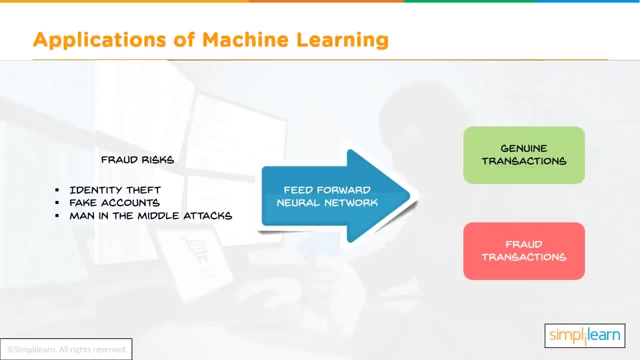 So what happens with feed forward neural networks are that the outputs are converted into hash values and these values become the inputs for the next round. So for every real transaction that takes place, there's a specific pattern. A fraudulent transaction would stand out because of the significant 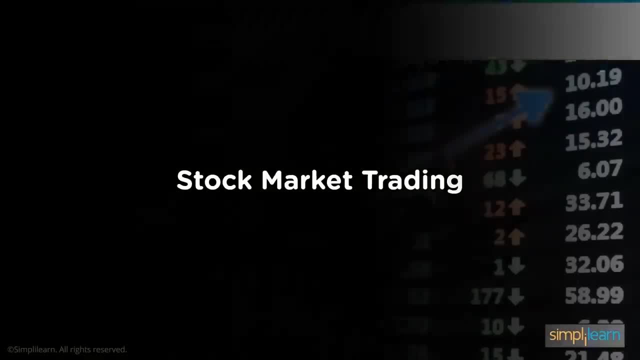 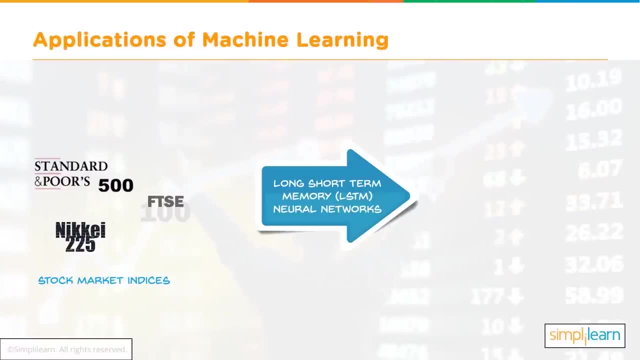 changes that it would cause with the hash values. Stock market trading. Machine learning is used extensively when it comes to stock market trading. Now you have stock market indices like Nikkei. They use long short-term memory neural networks. Now these are used to classify process. 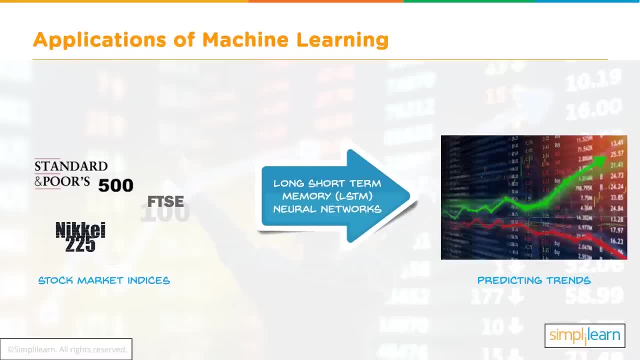 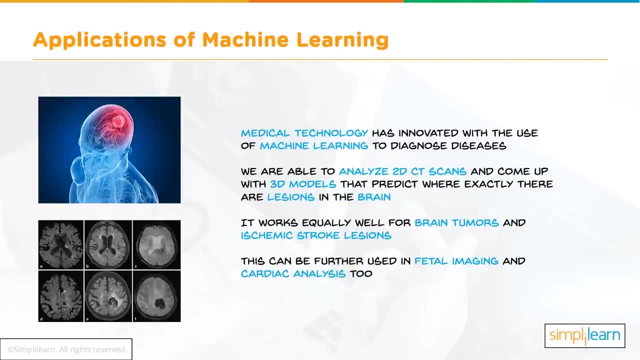 and predict data when there are time lags of unknown size and duration. Now this is used to predict stock market trends. Assistive medical technology: Now medical technology has been innovated. With the help of machine learning, diagnosing diseases has been easier, from which we can. 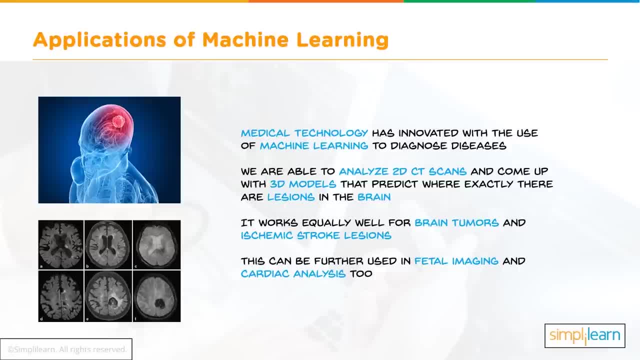 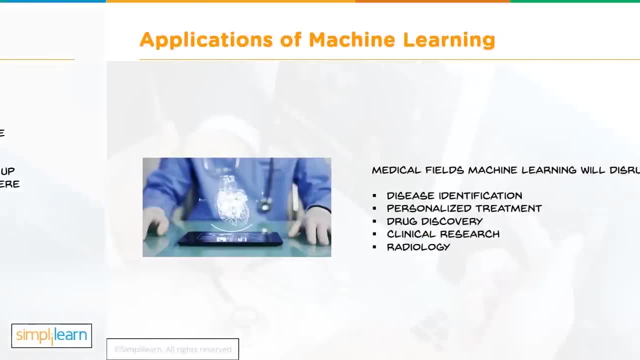 create 3D models that can predict where exactly there are lesions in the brain. It works just as well for brain tumors and isochemic stroke lesions. They can also be used in fetal imaging and cardiac analysis. Now some of the medical fields that. 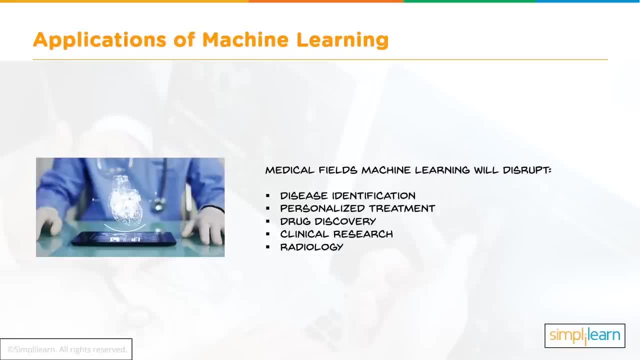 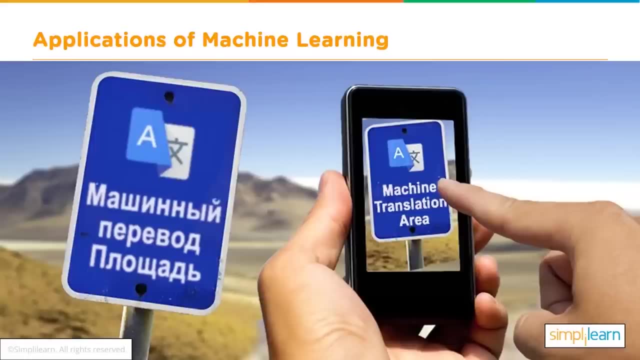 machine learning will help assist in is identification, personalized treatment, drug discovery, clinical research and radiology. And finally we have automatic translation. Now say, you're in a foreign country and you see billboards and signs that you don't understand. That's where automatic. 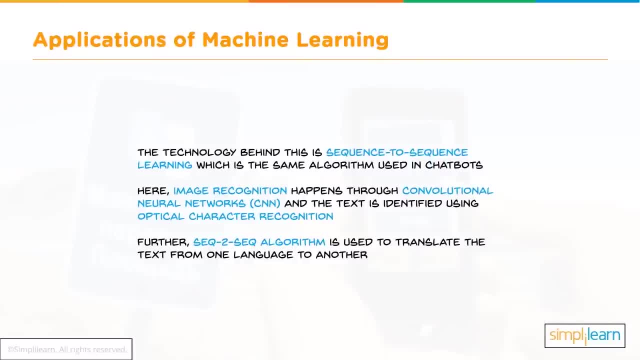 translation comes of help. Now how does automatic translation actually work? The technology behind it is the same as the sequence-to-sequence learning, which is the same thing that's used with chatbots. Here the image recognition happens using convolutional neural networks and 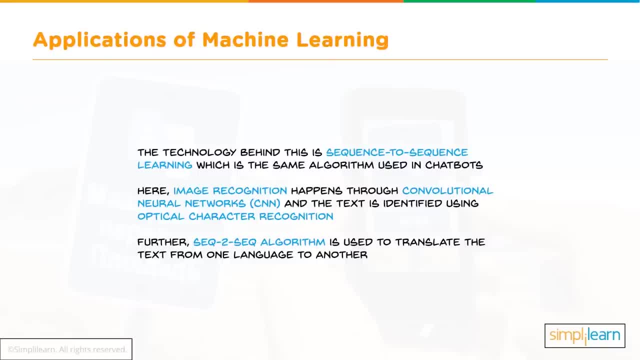 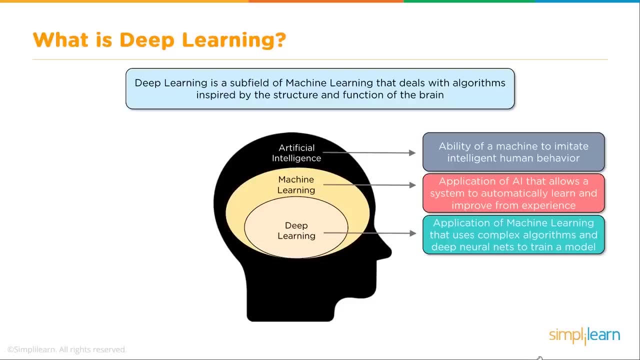 the text is identified using optical character recognition. Furthermore, the sequence-to-sequence algorithm is also used to translate the text from one language to the other. Welcome to deep learning in Python. Deep learning is a subfield of machine learning that deals with algorithms inspired by the structure. 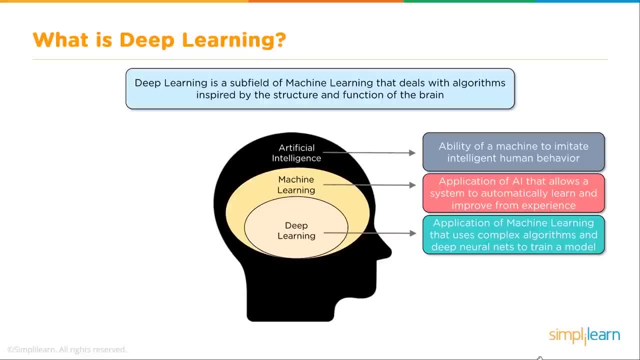 and function of the brain And you can see we have a nice picture here. We have artificial intelligence, which is kind of the big bubble that encompasses all these different things we're talking about. This is the ability of a machine to imitate intelligent human behavior. 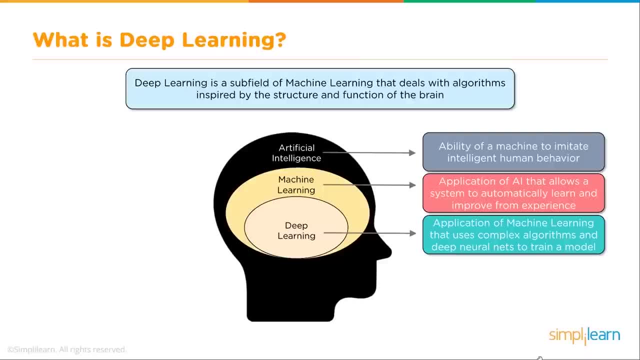 And in there we have machine learning application of AI that allows a system to automatically learn and improve from experience, And if you looked at any of our other videos, you'll see that there are a lot of videos. You'll know that machine learning, 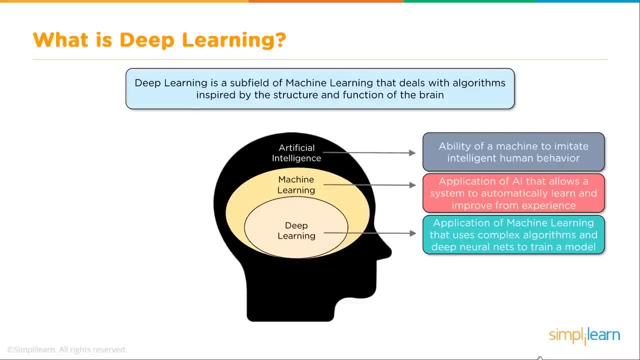 covers a lot. so deep learning is a subcategory of that. But don't forget, machine learning has all kinds of other tools that people use to do very basic descriptive and predictive and post-scriptive analytics. And then you have deep learning application of machine. 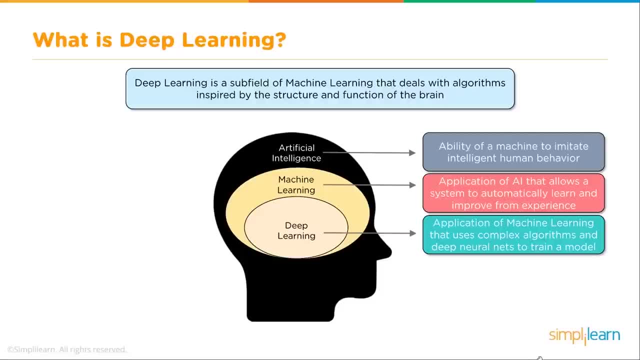 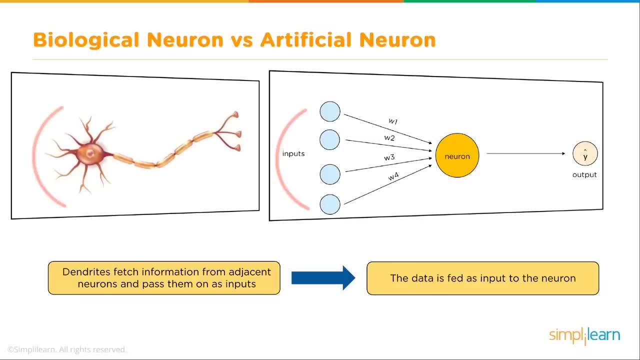 learning that uses complex algorithms and deep neural nets to train a model. Let's take a look at the biological neuron versus the artificial neuron. Now, remember, in the human brain- and this is true for most animals- there are a lot of different. 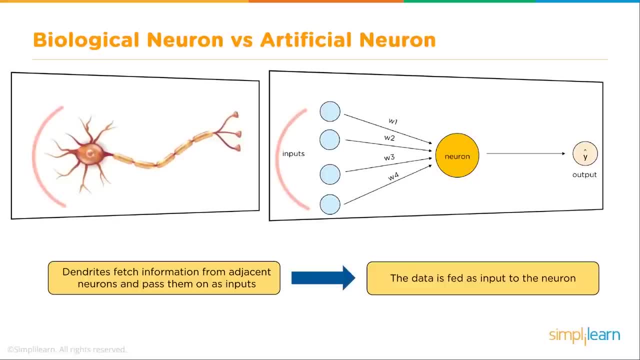 neural networks that are used to train a model. Now let's take a look at the neurons going on. So this is a very basic one. I mean, there's hundreds of different cells involved. So when we talk about neural networks- and this is why I say it's 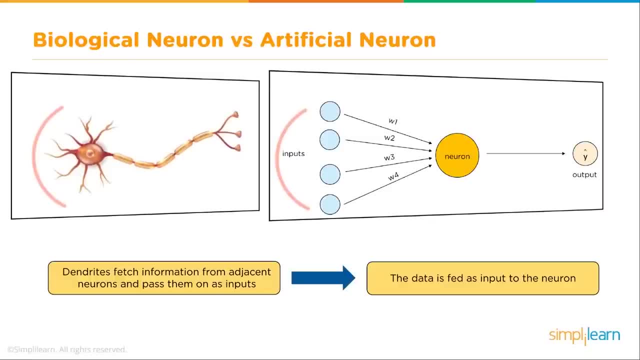 in a very infant stage. they're really basing it on just the most basic thing that we're able to figure out going on in the neural networks, And you can see right here we have dendrites, fetch information from adjacent neurons and pass them on as inputs. So you have your. 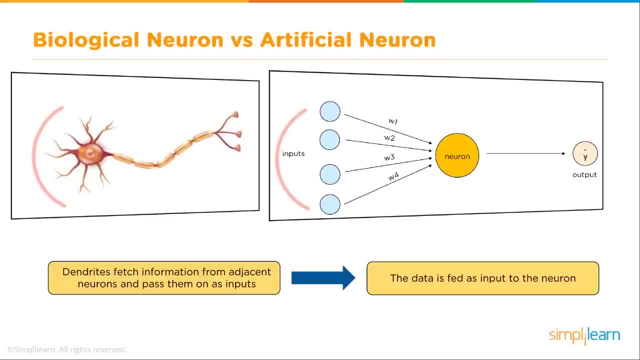 data coming in and your data going out. Any computer model should be looking at that: what's coming in, what's going out. The data is fed as an input and then the data is fed as an output to the neuron. So when we look at the artificial neuron, 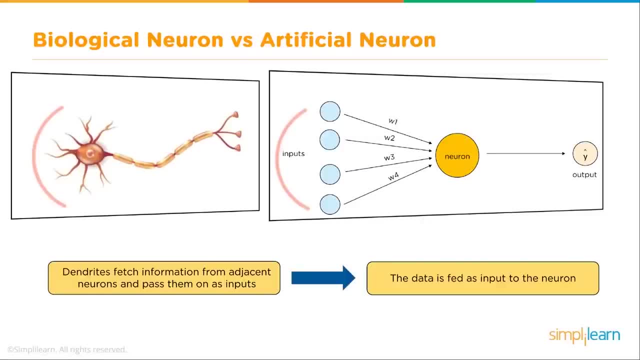 you can see, we have our inputs. they come in, each one is specially weighted into the neuron and then the neuron has an output: The cell nucleus processes, the information received from the dendrites and the neuron processes, the information provided as inputs. Axons are the cables. 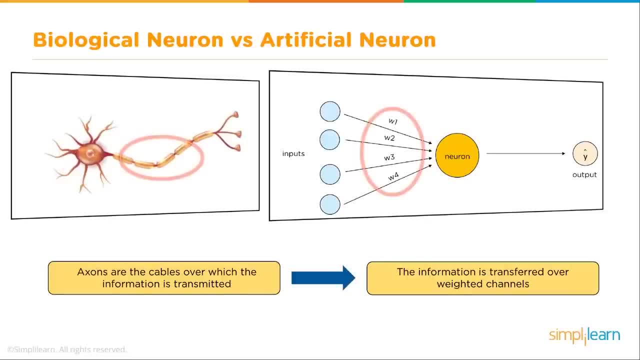 over which the information is transmitted, And the information is transferred over weighted channels. So you can look at that. I mentioned weights briefly but you alter the data coming in, So those weights are what causes the data to process different information coming. 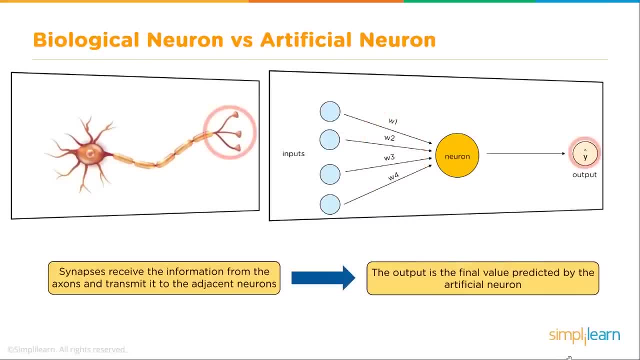 in to be weighted differently and processed differently, And the synapses receive the information from the axons and transmit it to the adjacent neurons. That's in your biological model. And then, when we look at the artificial neuron, the output is a final value predicted by 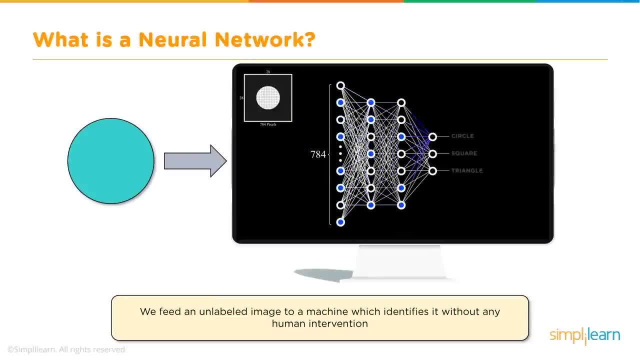 the artificial neuron. So as we dig deeper into looking at the theory behind the neural network and we kind of flip back and forth between these, because there's two huge aspects of it. One is from the outside: what are you seeing and what's? 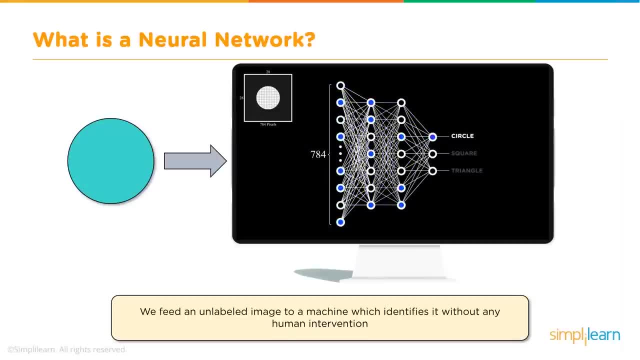 going on from the inside, so you can find out how to do what you need to do and give the best results you can. And we start off with what do we feed? We feed an unlabeled image to a machine which identifies it, without any human. 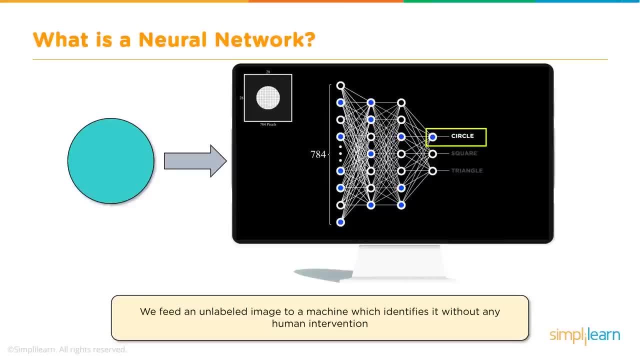 intervention. And so you can see, here we have a circle that comes in at 784 pixels and it comes in by 28 by 28.. And you can see how it colors in the circle on there And we put a triangle in The triangle. 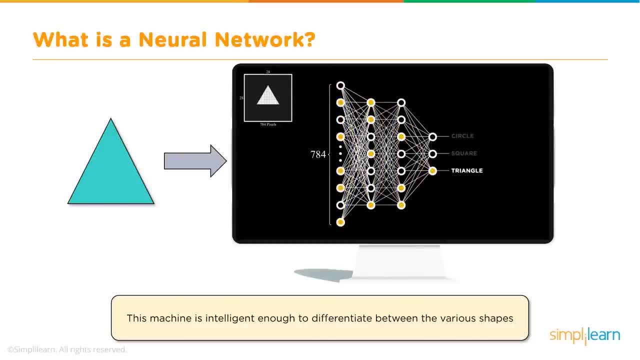 in also comes in as 28 by 28 and it has 784 pixels. So you'll see, between these two, both of them are 784 pixels. This machine is a little bit more complex. This machine is intelligent enough to differentiate between the various shapes. 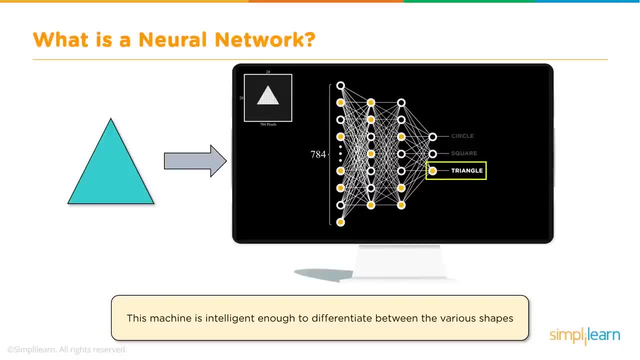 So that's what we want to use our neural network to do- is to say: hey, this is a circle, this is a triangle. That's more of a categorical. You can also do a regression model, where you're actually putting out a float value or a numerical. 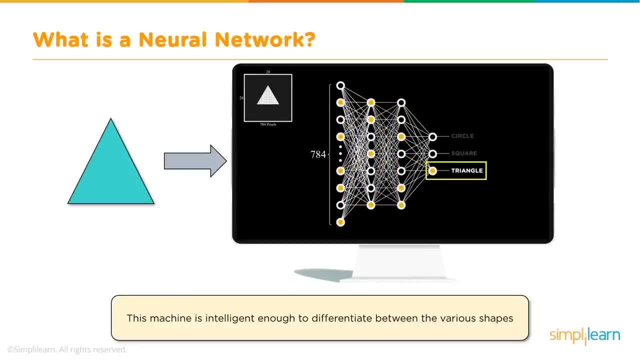 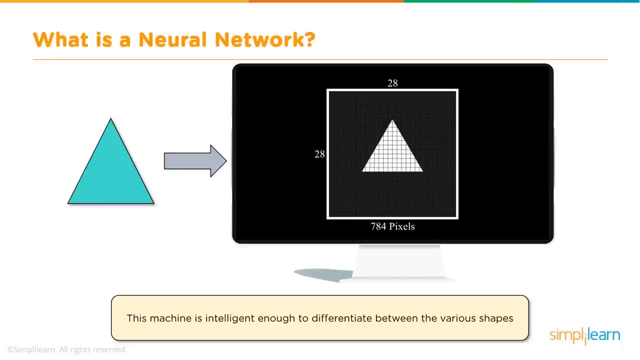 value. We'll be looking at the true-false or the categorical model, mostly because that's where you usually start at The difference. there is no real difference when you, as far as the way the internal functioning goes, when you start flipping between them, other than well, we'll talk. 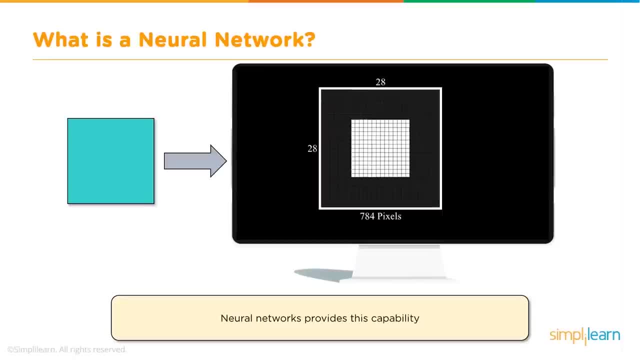 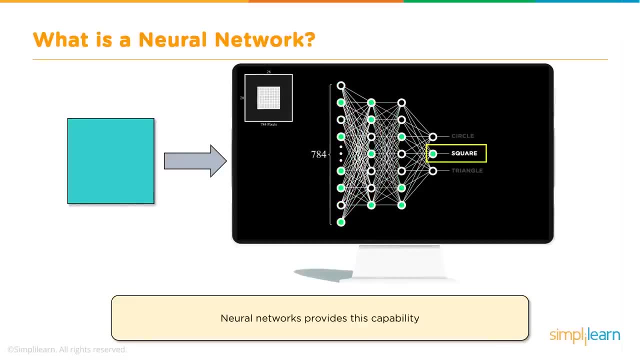 about that in a minute. So you can actually go between the two quite easily, And the neural network provides this capability, So we're going to use this capability to look between those two. One of the things I want you to note in here is that we're 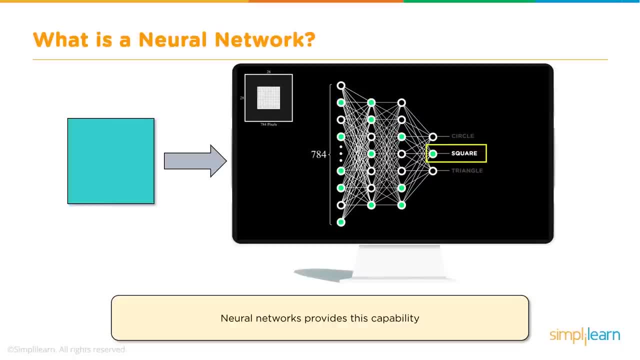 looking at 784 pixels. We're looking at 784 inputs. That's very different than stock with a high-low or last year's sales based on date. We're looking at just a couple of numbers and they're very clear. they're numbers. They're. 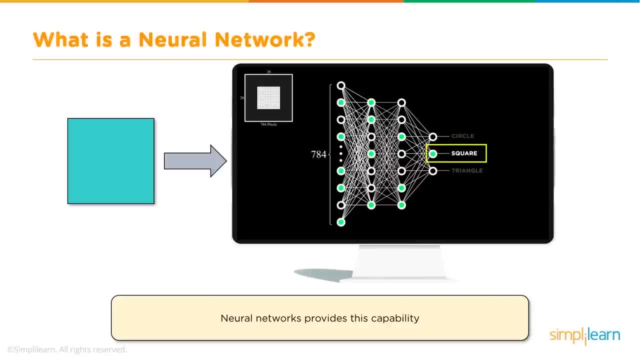 very clear what they are, which is something you'd put into a machine learning linear regression model. This is where we step out from that, in that we're looking at complex patterns, and how do you figure those complex patterns out? So a neural network is a system. 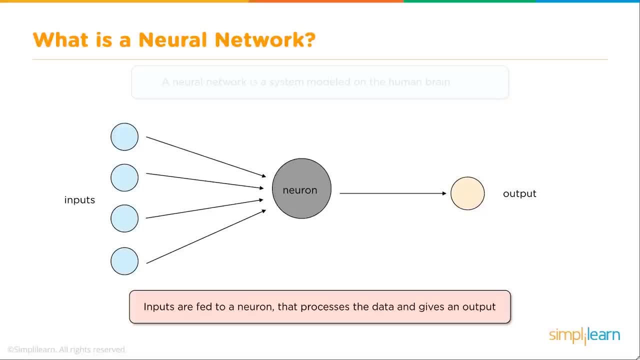 modeled on the human brain And we looked at that, Comparing the two. let's go ahead and look deeper into the neural network itself. We have our inputs coming in, So the inputs are fed to a neuron that processes the data and gives us an. 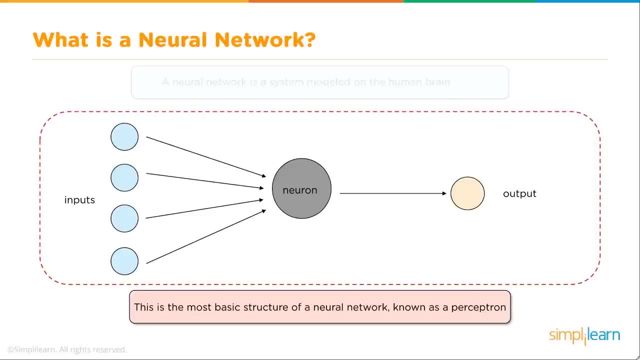 output. Input and output. This is the most basic structure of a neural network known as a perceptron. So if you see the term perceptron, that's what we're talking about. We're talking about this box of inputs and an output. However, 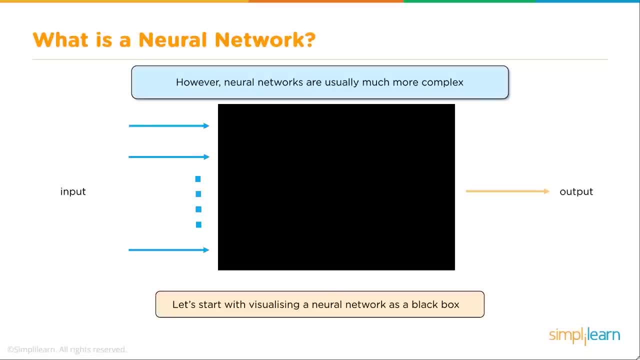 neural networks are usually much more complex. Let's start with visualizing a neural network as a black box, And I always loved that symbol. It's a black box. It's kind of magical. We have our inputs coming in and we want certain. 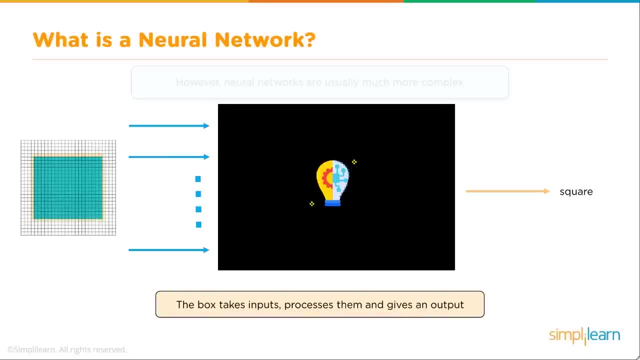 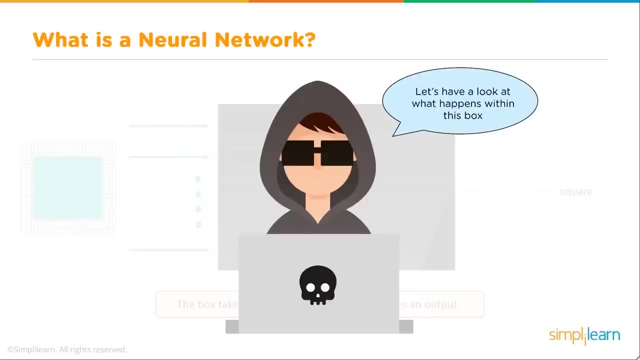 outputs. The box takes inputs, processes them and gives an output. Let's have a look at what happens within this box And you can see me there in my secret agent. get up, I got my hidden hood and everything. I guess I'm part of the black. 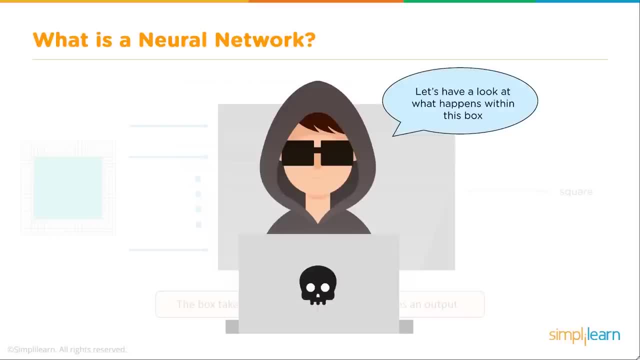 skull or something like that group. So let's take a look at what happens within this magic box And remember we're skipping back and forth between the theory of what's going on in the box, which you have to know how to fine tune. 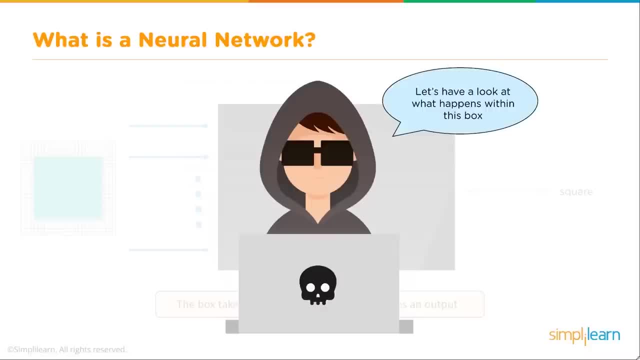 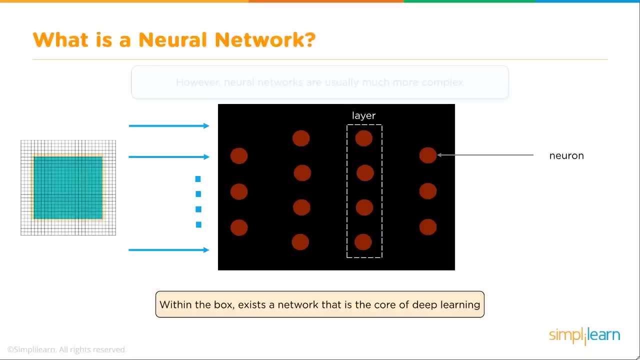 and how to build, versus looking at it from the outside. We're programming this box and we have an input and an output to the box as a whole. Within the box exists a network that is a core of deep learning, And you can see, here we're. 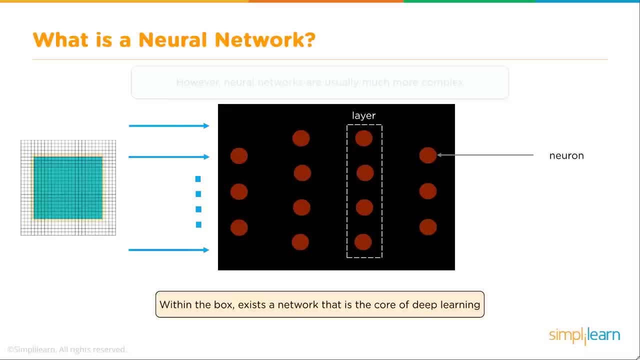 showing one layer And we have our grid coming in. The network consists of layers of neurons. Each neuron is associated with another neuron And each neuron is associated with a number called the bias. And you can think of the bias if you overly simplify this and we're doing a. 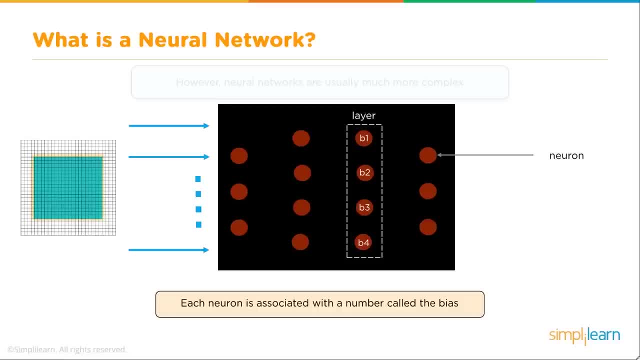 linear regression model. this is your y-intercept in your Euclidean geometry. You have to have something that offsets it, And so you always have a bias. in these cells, Neurons of each layer transmit information to neurons of the next layer over channels, And so you can. 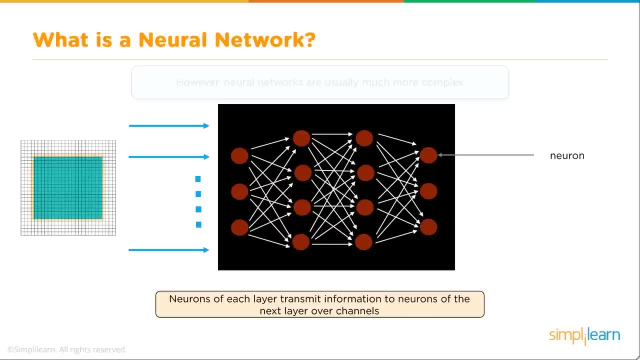 see each of our layers going through from left to right. These channels are associated with numbers called weights. These weights, along with the biases, determine the information that is passed over from the neuron to neuron. So just like the bias is your y-intercept, 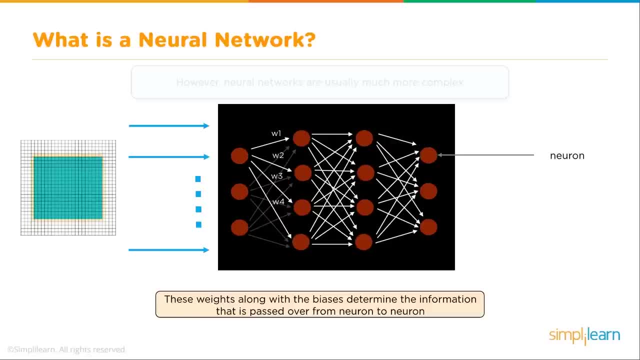 in Euclidean geometry you can look at the one weight. Remember, this is very complicated, so we're not looking at just one weight. You can look at the weight as your slope of the line. Or, if you're doing, x equals my plus c, it would. 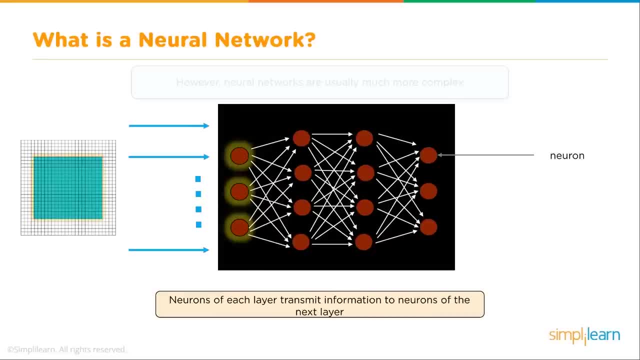 be the m value. Neurons of each layer transmit information to neurons of the next layer And you can see here as they light up, going across into the final layer And then to the output, And in this case the output is going to be: 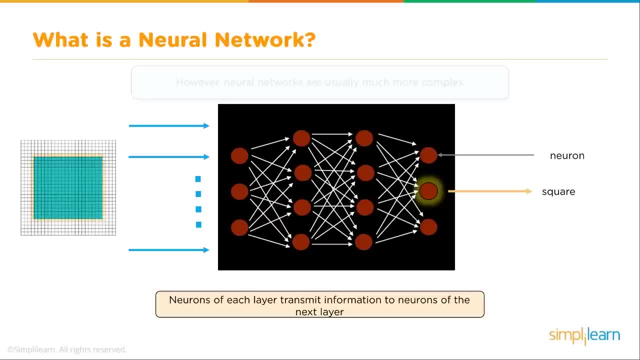 either x equals my plus c or the second layer is going to be either a square in this one or it might light up the other one, which is a circle. The output layer emits a predicted output, So in this case we're looking at a. 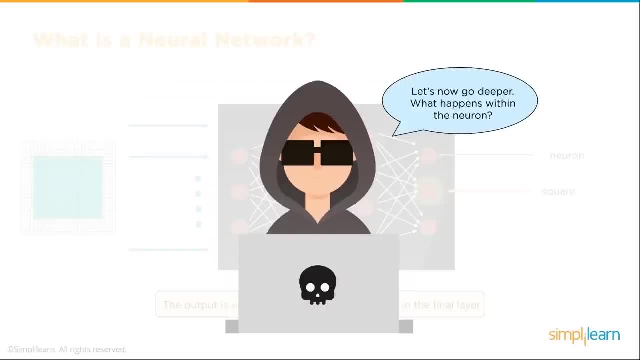 classification: True, false? Is it a circle, Is it a triangle, Is it a square? Let's now go deeper. what happens within the neuron? So we're going to dig deeper and start getting a little bit closer to some of the math. Don't worry, you don't. 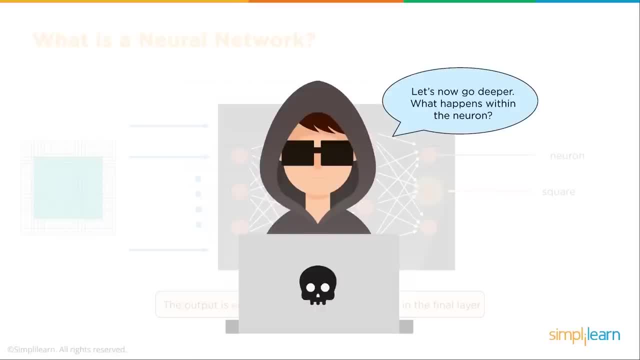 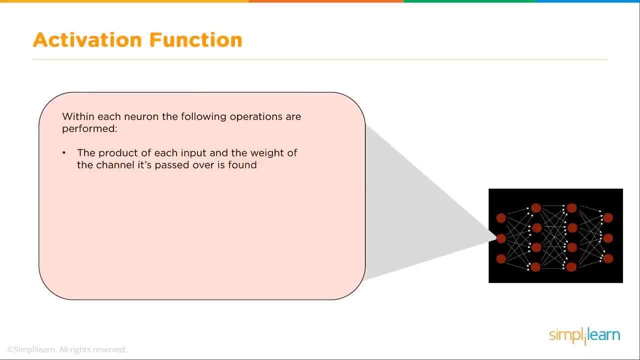 have to be a calculus expert or know your differential equations. Even though this is one giant differential equation, you don't need to understand those to be true. In each neuron, the following operations are performed: The product of each input and the weight of the channel. 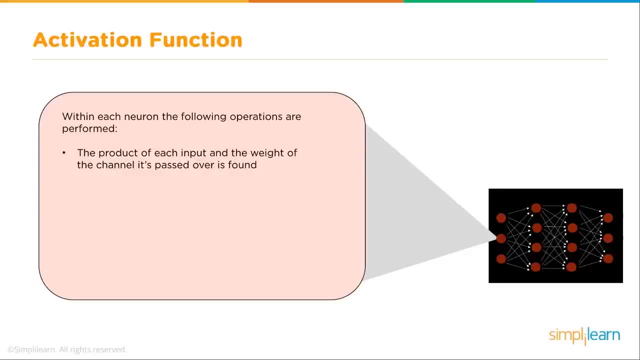 it's passed over is found. This is simply addition. We're going to sum up the weight times, the output from the previous channel and plus the bias. Some of the weighted products is computed. This is called the weighted sum. Bias unique to the neuron is added to the. 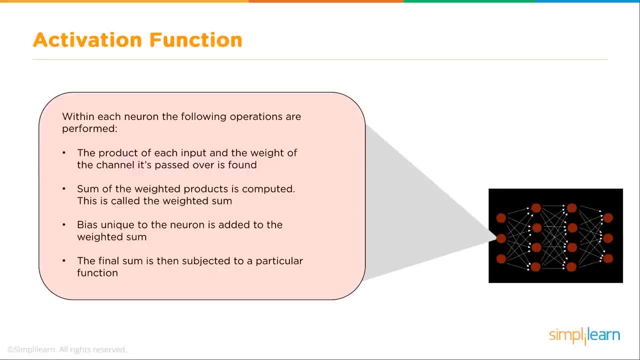 weighted sum. The final sum is then subjected to the particular function, And we'll discuss that particular function. That part is really important because those functions have a huge impact on how well your model performs under different conditions. The final sum is then subjected to a particular. 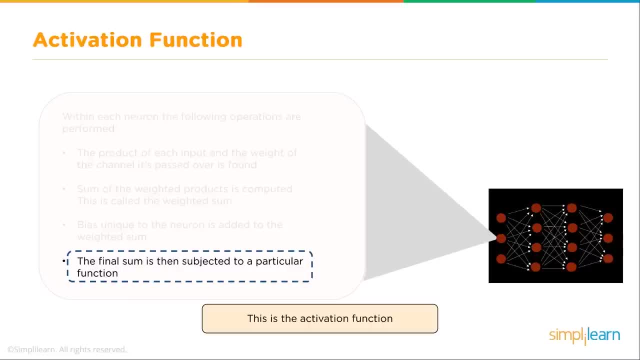 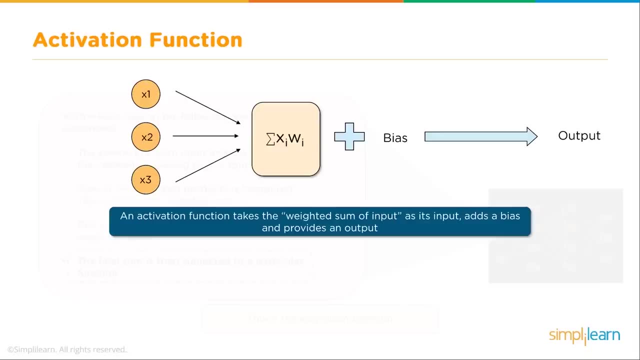 function. This is the activation function. So if you ever hear the term activation function, that's what we're talking about: What activates this cell and what doesn't. As we dig deeper into activation function, an activation function takes the weighted sum of the 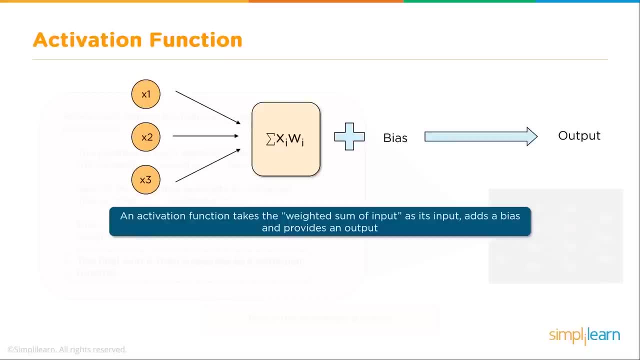 input, as its input adds a bias and provides an output. And a lot of times you'll actually see one formula for the sum, of the weighted sum and the bias. You'll just see that as a single line of everything added together. And here 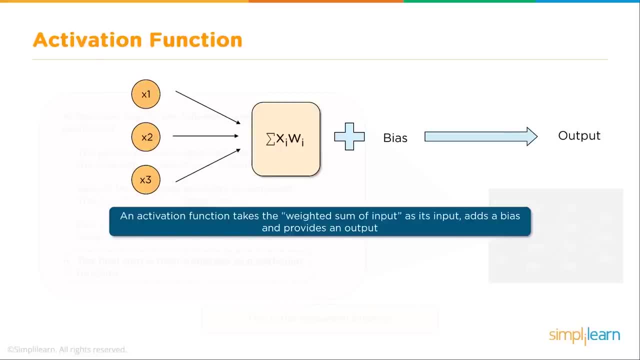 we've broken it apart because it makes it clear that this bias is not computed the same as the weighted sums. Here are the most popular types of activation function, And I always find these interesting because at one point I was sitting at a table with a gentleman who 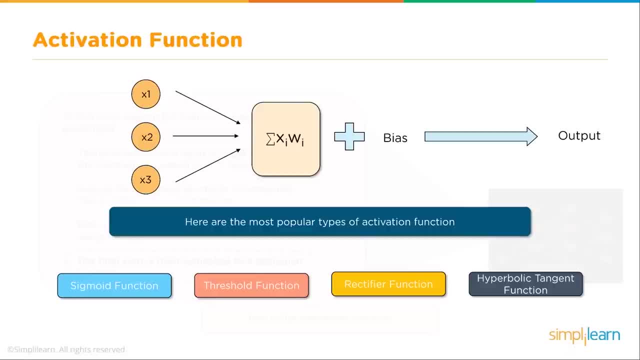 was finishing his PhD. He was in his last year And he said he went through all this stuff and he ended up just trying the four different activation functions on this particular problem he was working on. So knowing the math behind it doesn't necessarily mean you're going. 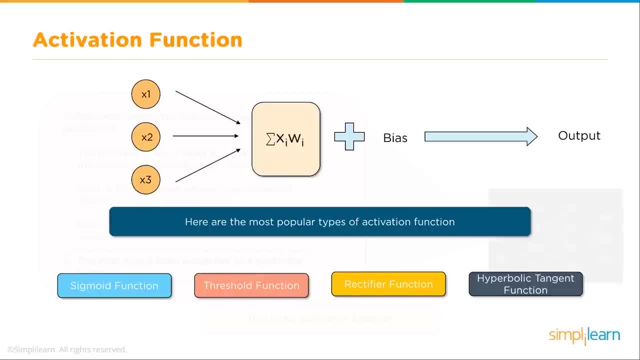 to know it right away. So even somebody who might have a PhD and be doing the calculations on this comes back out of it and ends up just trying the different activation functions to see what's going to make a difference, And a lot of times that's a final step. That's the kind of 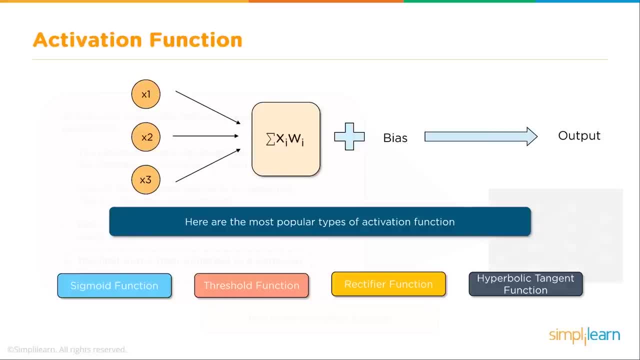 thing where you've built your whole model. you've come back and you're like: wait a minute, can I do a better deal with the sigmoid function or the threshold or the rectifier? Knowing what they're doing is important so you can explain it to somebody else. And again, 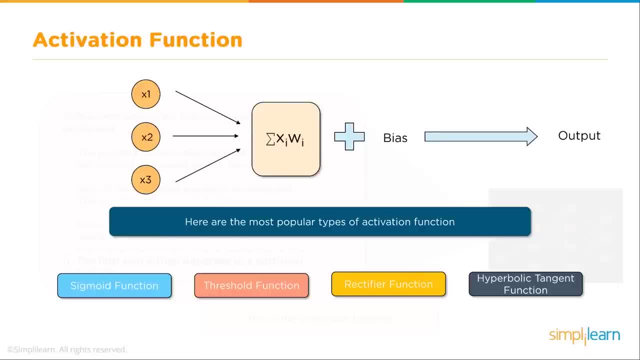 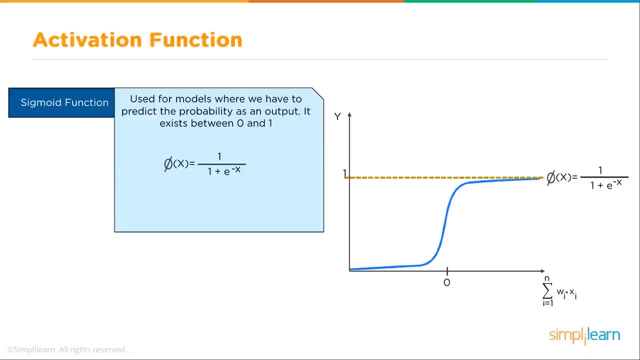 you don't want to take down the full server farm just to test out your three different series. You take a small portion of that data, test it and then you put it through to the big data. So let's take a look at this. We have the 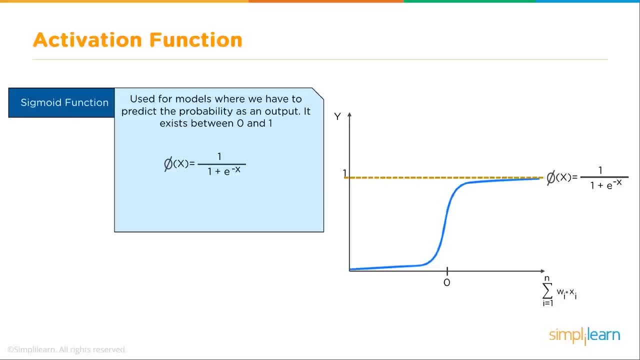 sigmoid function, and it's used for models where we have to predict the probability as an output. It exists between 0 and 1.. And you'll see that's true of all of our activation functions. we're working with Either the cell's on 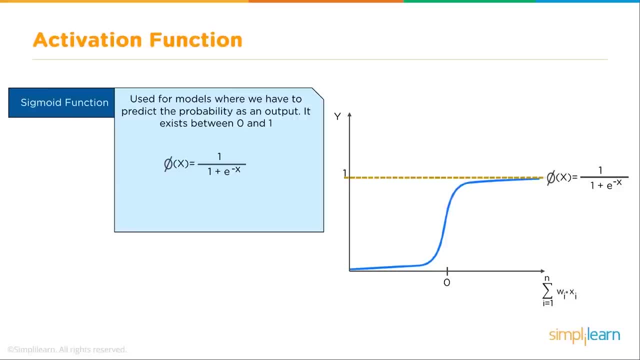 or off, It's true or false, And there might be a little variation in there which, as an output, could be used to determine the certainty in your solution. So if you're getting a .7 with this activation function, it might be well, I'm not sure if that's really a. 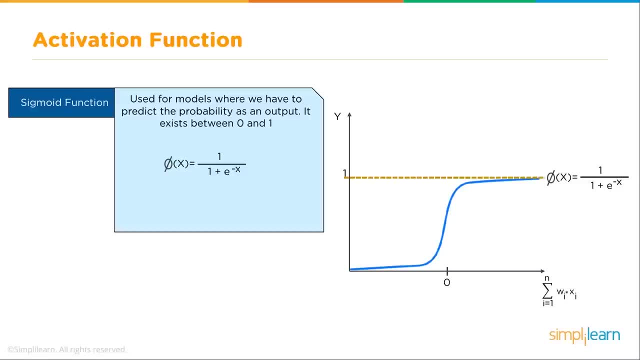 square, or I'm not sure that's really a triangle, And that might be a flag for it to be looked at by a human observer. at least in today's models where we're at right now And you can see here we have the formula is simply equals 1 over. 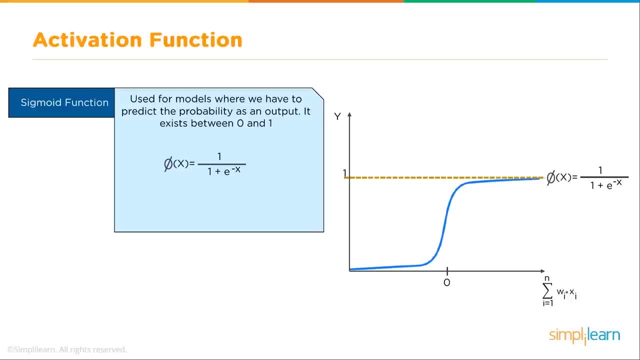 1 plus e to the minus x, where x is your value coming in, And it's going to give you a result that looks very similar to the graph on there, which is somewhere between 0 and 1.. And right in the middle there's a huge kind of you can go. 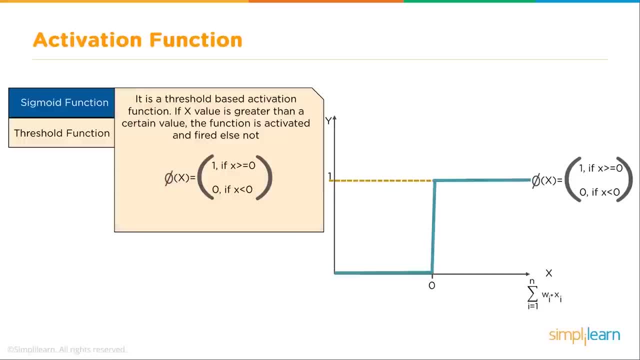 through all the different values and uncertainties involved. So the sigmoid function is probably the default on most of them. The next one is the threshold function. It is a threshold based activation function. If x value is greater than a certain value, the function is activated and fired, else not. 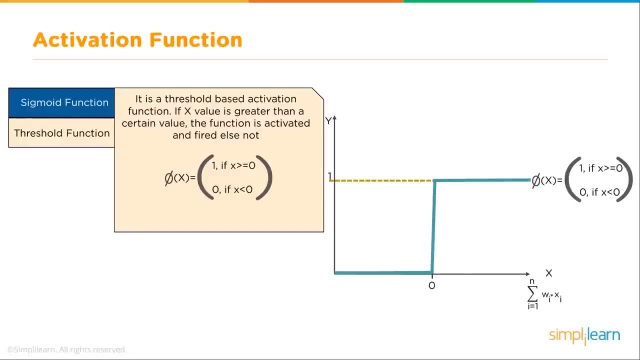 Pretty straightforward: Yes, no, true, false. I don't want to test for improbabilities, I just want a straight answer. I don't want to know if there's a partial value on there. It either is true or it's false. And the rectifier. 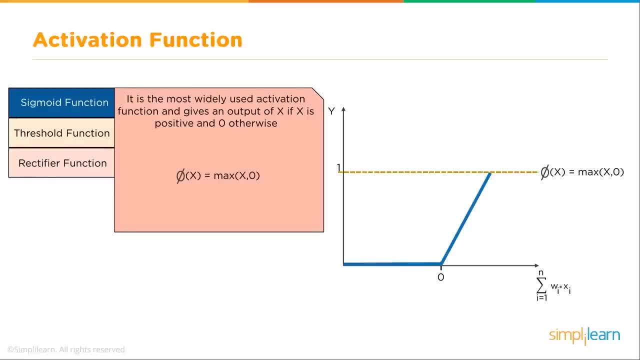 function. it is the most widely used activation function. I would debate that. Rectifier is a pretty common one, although I see that the sigmoid function used to be the basic one, But it's up there. The rectifier function is very commonly used. It gives the output of x. 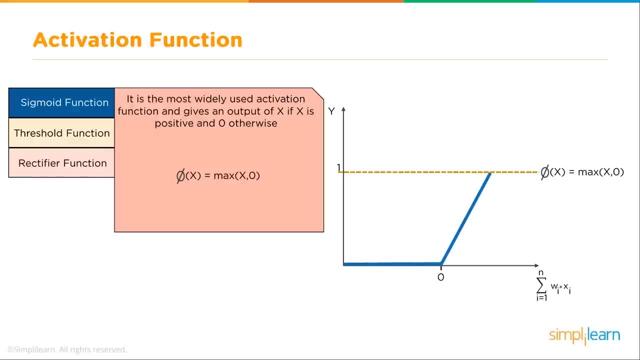 if x is positive and 0 otherwise, And you can see here again just like it's either kind of get a value going up there. So max of x, of 0. So it's again, it's like the threshold function. Yes, no, true. 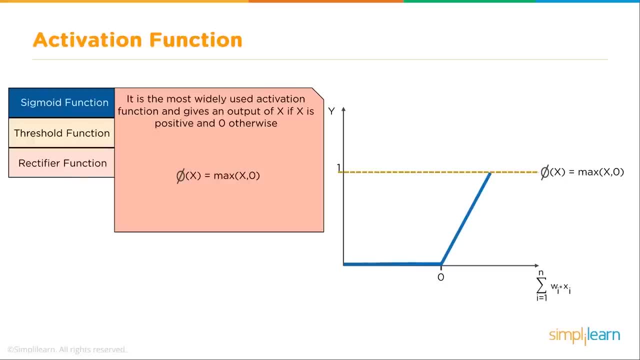 false. It's either 0 or it's some kind of positive or it's negative. So it's either 0 or it's some kind of progressive value, And then we have the rectifier function. I would argue with this because the sigmoid function used to be. 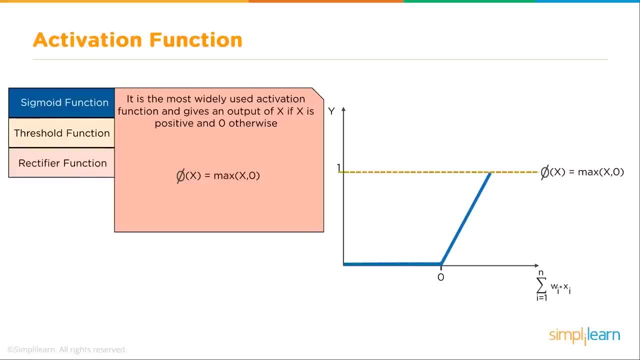 the most common one, But with the rectifier function it now says it is the most commonly used or widely used activation function and gives an output of x if x is positive and 0 otherwise. This is kind of nice because it now says absolutely not, or it gives you a value. 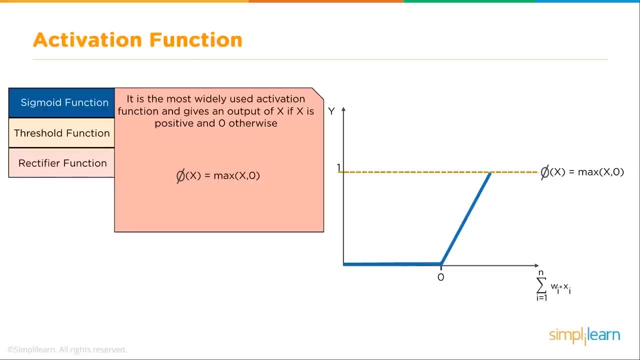 of probability. Now, when I say a value of probability, be very careful there- I'm not saying that it's going to tell you this is 75% chance of success, There's no chance of being a circle. I'm going to tell you that it says hey. 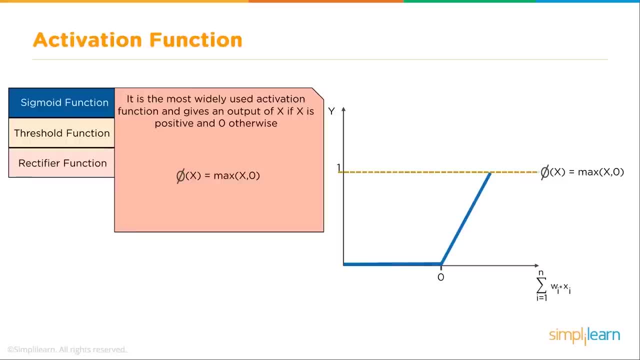 if this says 0.1, it probably needs to be looked at. or 0.2 or 0.3. It's going to depend on your data as to what that value means. In general, that just means it's flagging it that if it's not a 1,. 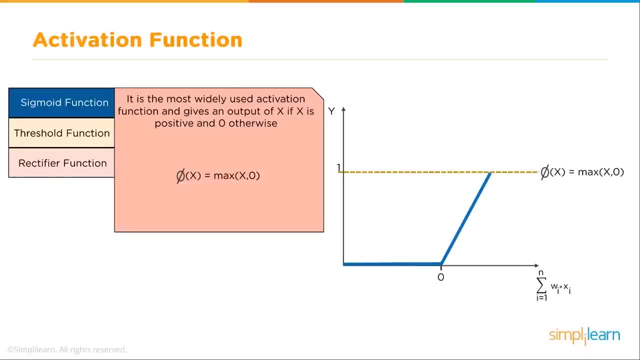 then chances are it needs to be looked at by a person and re-evaluated, And there's a hyperbolic tangent function. This function is similar to sigmoid function and is bound to a range of minus 1 to 1.. So you can see, there's our. 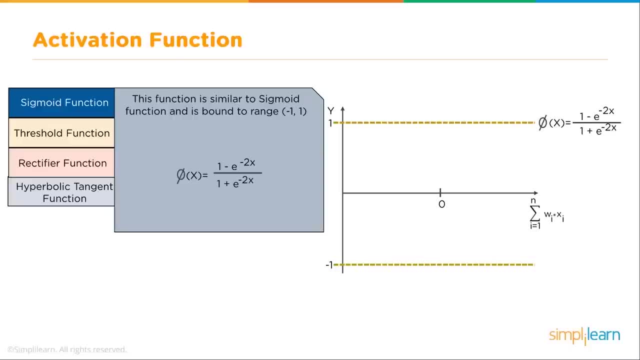 1 minus e to the minus 2x and 1 plus over, 1 plus e to the minus 2x. Again, it's very similar to the sigmoid function. The bonus of the hyperbolic function is you have that variable coming through the middle. So again, you. 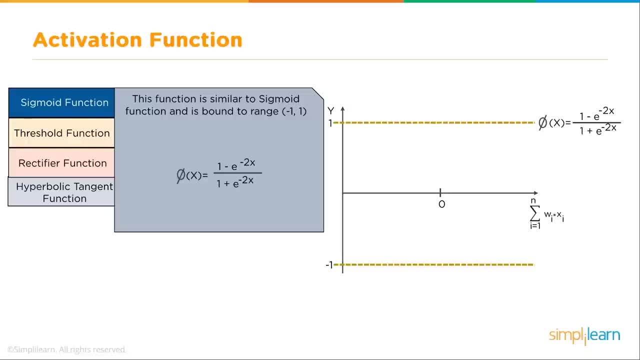 can look at it and you have a little bit more weight as far as you can process that down the line. That's a little bit more advanced than what we're looking at right now And a lot of times it's not even necessary in a lot of our different 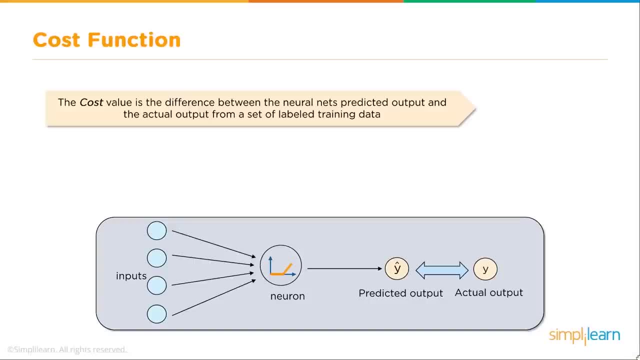 uses for these activation functions. Now we looked at activation functions and I kind of said those are a little bit like a black box, because even if you know all the math, a lot of times you end up just playing with them to find out what works. 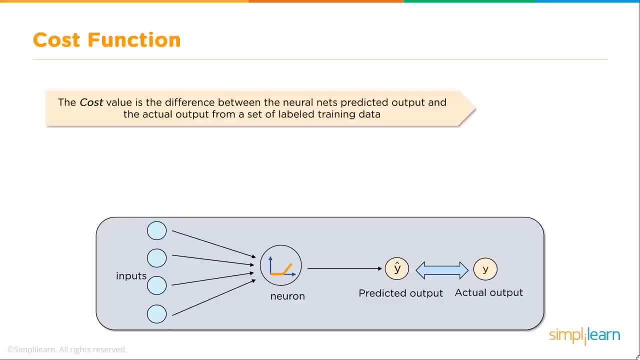 And it also depends on what model you're working with, whether you need a flat, yes, no, true, false, or you need to have something in the middle that says, hey, this isn't quite a 1. You might need to. 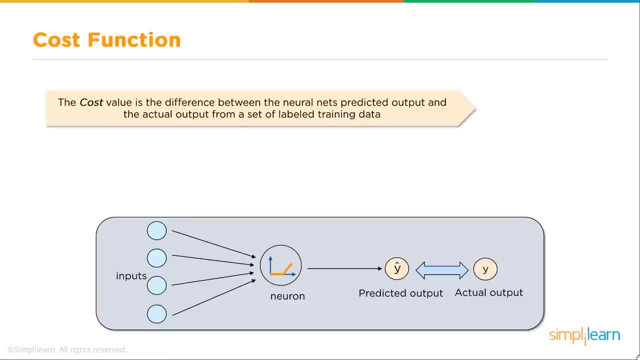 process this with the human intervention And you can look at that. One example would be self-driving cars. You don't want a car to be yes, no, I'm going to go through the light. You want it to be like: okay, if it's almost yes, maybe we stop. 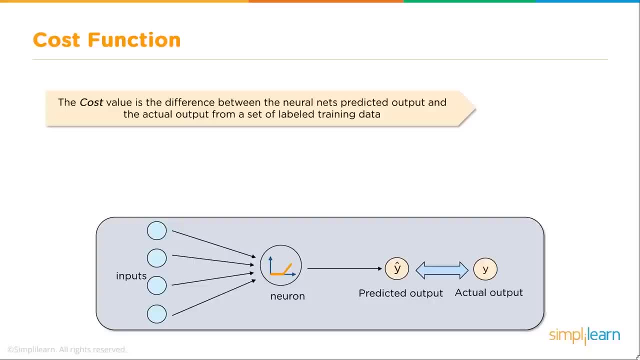 and have human intervention so we don't get an accident. Cost function is something you can really see and measure. the cost value is the difference between the neural nets predicted output and the actual output from a set of labeled training data. So we have our group of. 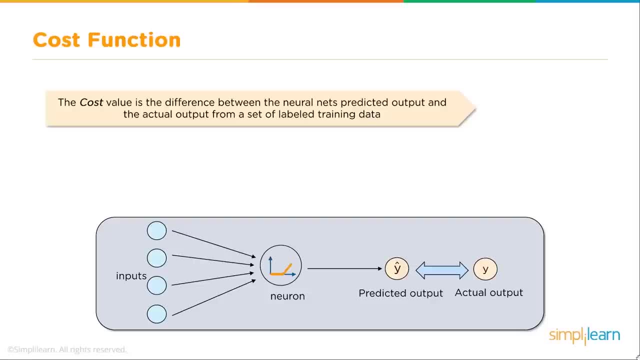 data. that's a square circle and since we're looking at geometrical shapes, we've had somebody already labeled that data. They've already said this is a triangle, this is a square, And so if this is coming up and it's giving us and 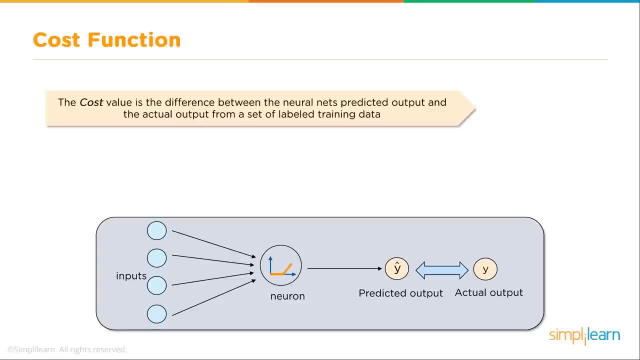 saying a square is a triangle and it's saying a triangle is a circle, the output is wrong, And so that output can then be measured in the versus the actual output, and that's the cost. You might also hear this as error, because that's the error value being returned. 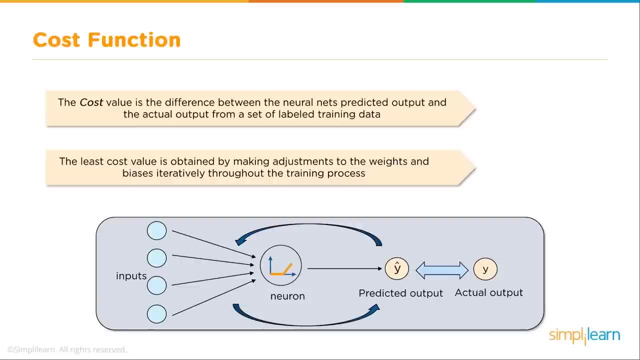 How far off is it? And what we're looking for is the least cost or the least error value, And it's obtained by making adjustments to the weights and biases iteratively throughout the training process, And this is called back propagation, And we're going to look in. 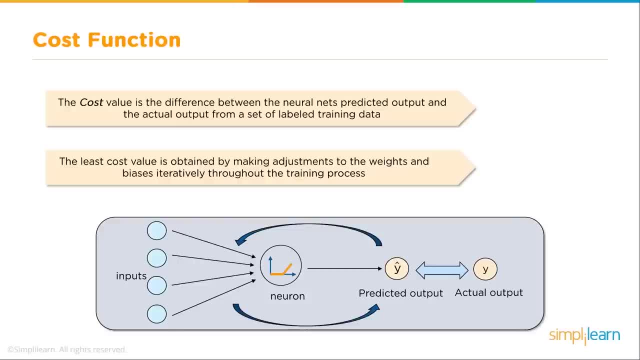 that a little deeper as we look into an example. It's really hard to see when you're just looking at arrows without actual numbers and where that flow is coming from. But you can look at this as here's our inputs. They put out a. 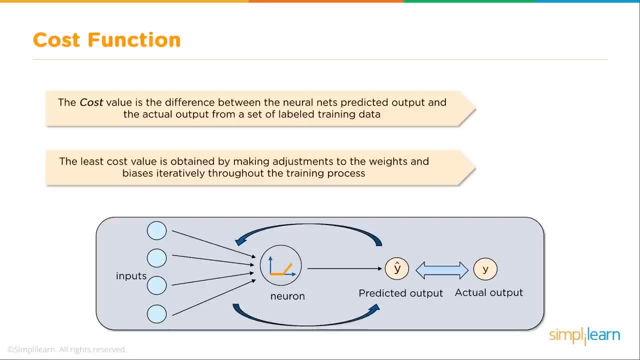 prediction. and then the prediction comes out and says: hey, we've already labeled this data because we're in training mode and the training data is off. This is the cost. Can we send that error or that cost back and adjust those weights? And we do. 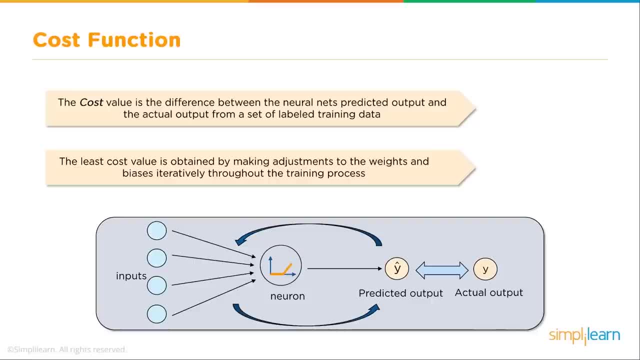 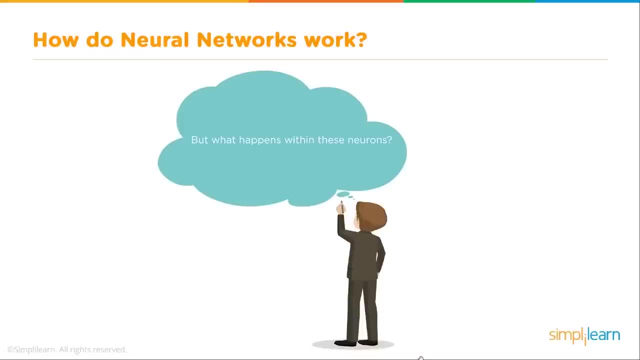 it in very small increments across large amounts of data, so that those weights minimize that cost or that error. But what happens within these neurons? So let's look at a little example of this Kind of helps. if you have some kind of visual, Let's build a neural network that. 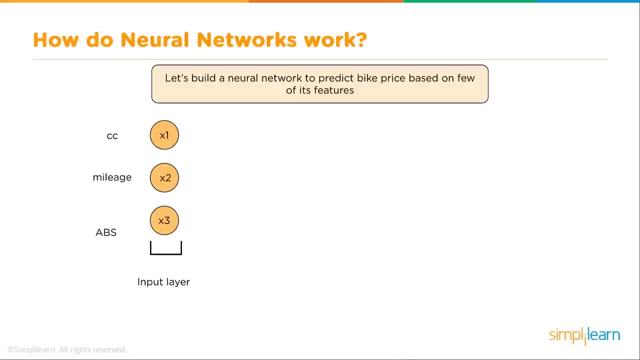 predict bike prices based on a few of its features And we'll see. here we have our CC, our mileage and our ABS, And these are our three input layers, And then we have the bike price and the output layer. Now it 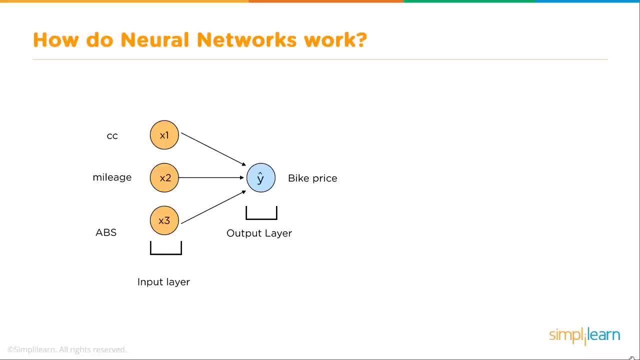 doesn't do us very good to just pump it in from the beginning and pump it out And, to be honest, I would use a machine learning linear regression model on this, since these are just straight numbers. But because we want a simple example, we're going to put this through and show. 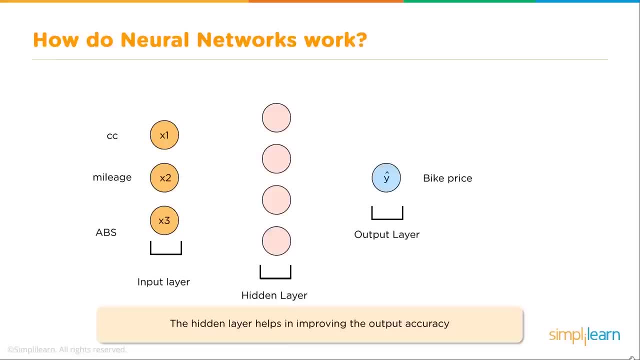 you as a neural network what that looks like, And we've got to put a hidden layer in there. The hidden layer helps in improving the output accuracy And you can see it does a bunch of ORs. So it might say: hey, when we compare these. 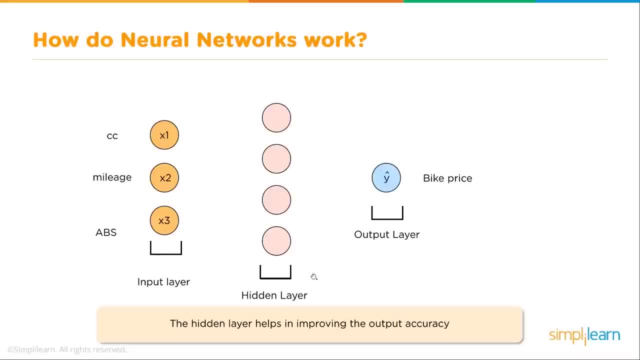 three values. on the first, hidden layer neuron, we're looking at one set of features And then we might weight them in the second one. So these are a bunch of different ORs, kind of how the math comes out in behind the scenes. And then 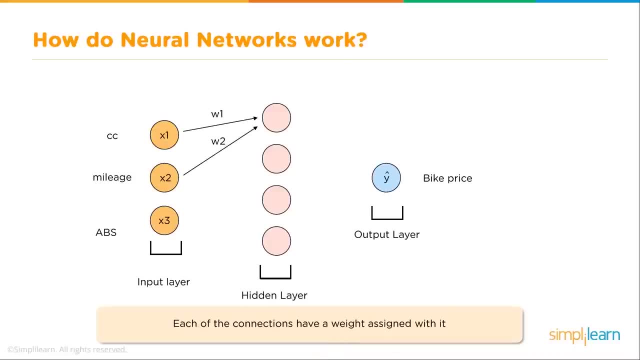 they go out, of course, to the bike price or the output layer, And each of the connections have a weight assigned with it And you'll see, here we have mileage CC with the weight 1 and weight 2 going into our first neuron, And you'd. 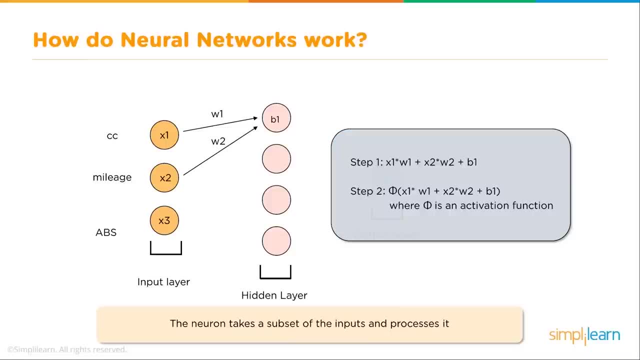 also have your ABS going in there, And so X1 times weight 1 plus X2 times weight 2, plus the bias of 1.. And step 2 is our activation, the activation function coming in there. When does this fire And the neuron takes a subset of. 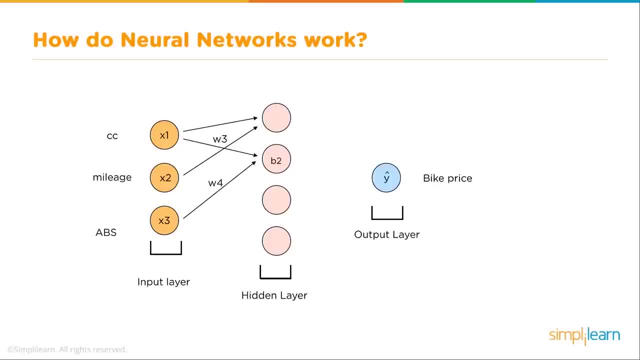 the inputs and processes it. And then we go through and we do that with the second hidden layer, neuron, and the third one, and so on. So you process each layer in order, going forward. Now what I told you. this is in its infant stage. They 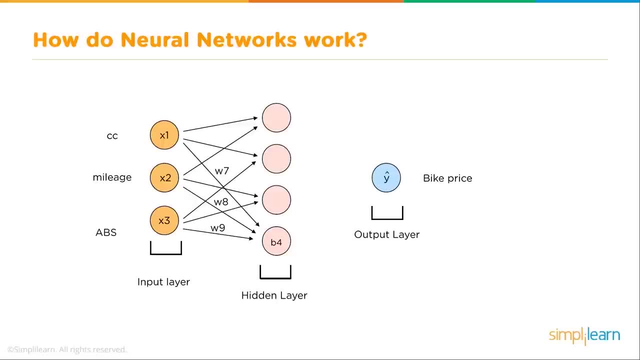 now have neurons that fire into the same layer or back a layer, so that you now have a time series And there's all kinds of wild things that they're experimenting with on these layers. This basic setup has been around since the mid-90s. It's only now, because of our 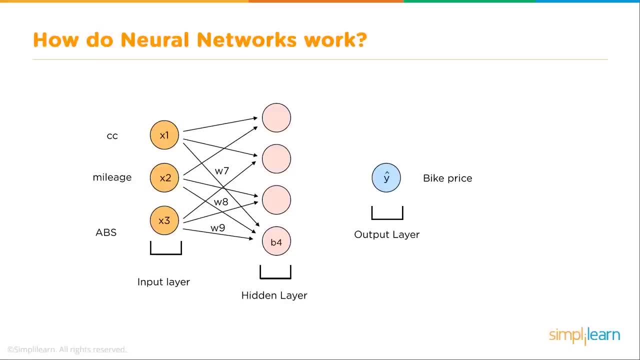 technology that it's open to almost everybody to play with it- And that's why I say this is in an infant stage in development- is this: basic math is here, but what we can do with it is amazing. And what they're actually doing with all. 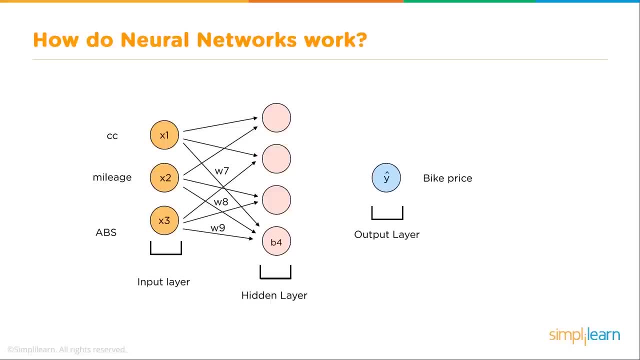 these different things is amazing, And so we're just at the beginning of how to use all these different tools in our deep learning and our neural networks, And so what we've done is we've computed the information reaching the neurons in the hidden layer is subjected to the 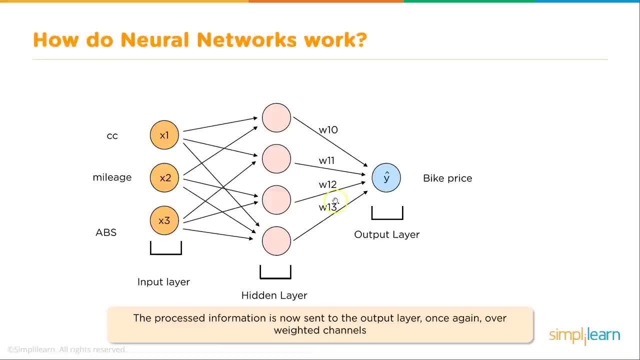 respective activation function, And so each one of these fires an activation output, and then those are each weighted to the final output layer. So the processed information is now sent to the output layer once again over weighted channels, And you could look at this as each one of these is I always look at 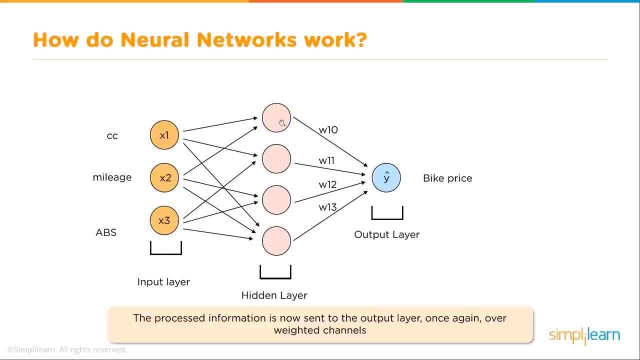 this as, like a group of people, They're all looking at the bulletin board and the first person says: this is what I project- cells for the company- and the second person says: I project the data for the product. So the third person says: this is what I project for the product and the 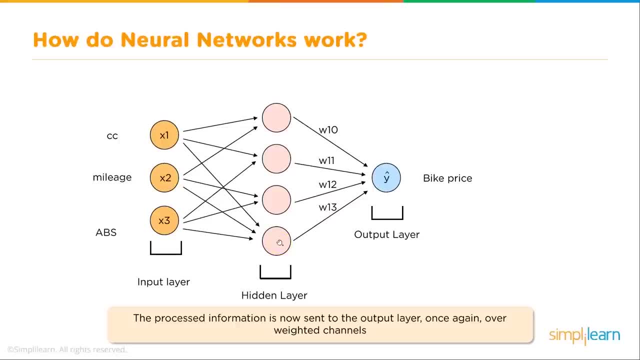 fourth person says: this is what I project for the product. So you can see that there's different ways to do that. So again, you can see that the executives are weighted based on their expertise. So your accountant might have a very high weight where maybe your janitor has a. 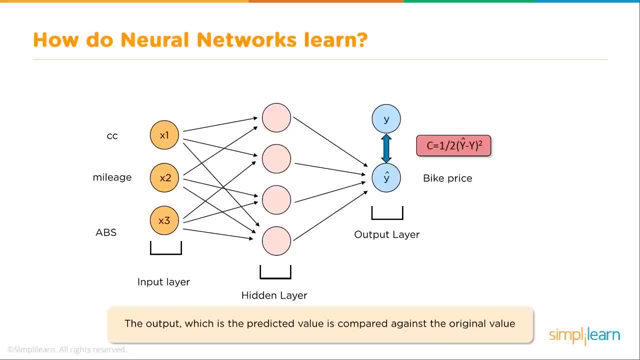 very low weight because their expertise is not in accounting. And then that goes into the output layer. And once in the output layer it goes, the output, which is the predicted value, is compared, determines the error prediction and reports it back to the neural network. 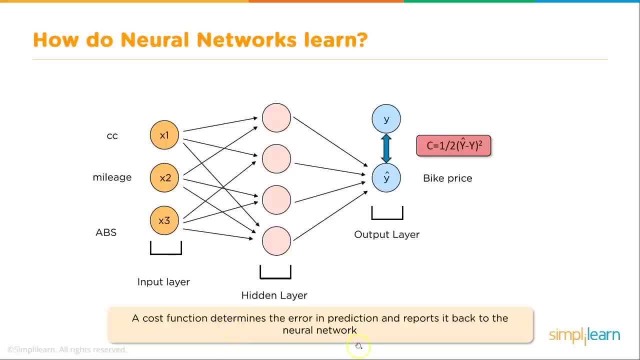 So this is the cost, This is how far off it is. This is your error coming back and, as you can see, this is back propagation going on. So now our error is going in reverse, because we know we're not completely correct on this particular channel. 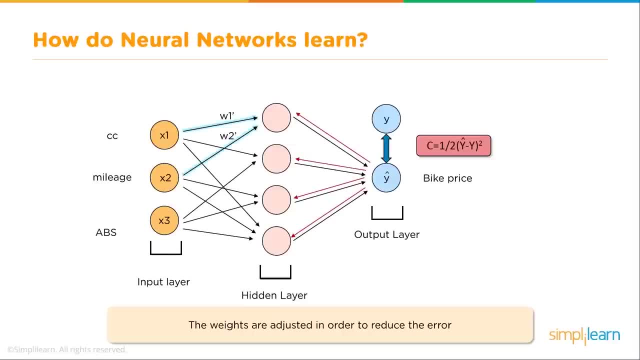 The weights are adjusted in order to reduce the error. So each time we go back, we are changing those weights to reduce that error and we change them in small increments. You don't want to fit one input. Remember you might have a data pool with a terabyte of data. 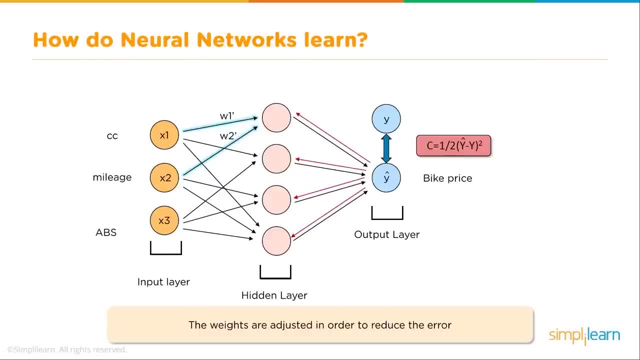 You don't want to solve for the first set of data that comes in and that be the main solution, because everything else will be off. This is going to confuse you. That's also called a bias. So we have the bias in the cell where we're adding a value, kind of like the y intercept. 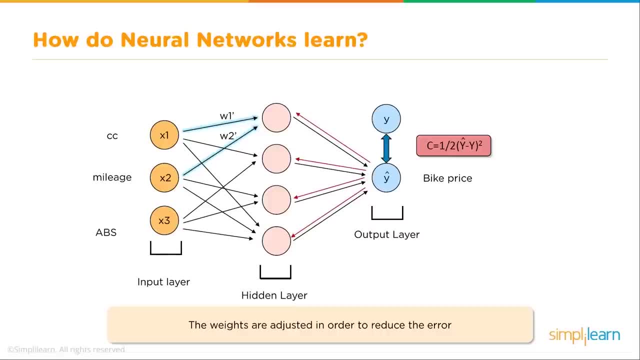 and we have a bias of the whole neural network which means that it's weighted towards one set of answers. So we want to make small changes in these weights so we don't create a bias. And the weights are very important. These are adjusted in order to reduce the error or the cost. 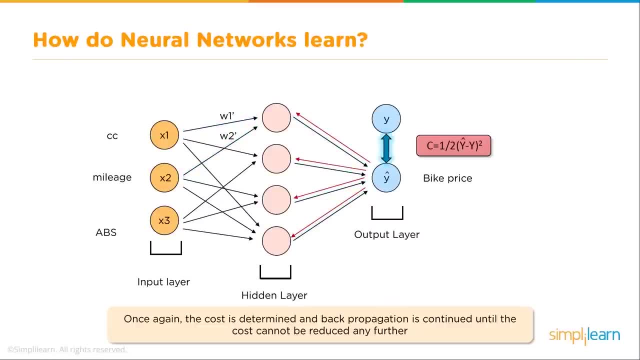 The network is now trained using the new weights. Once again, the cost is determined and back propagation is continued until the cost cannot be reduced any further. So let's go ahead and plug in values and see how our neural network works. So here we come in here, and initially our channels are assigned with random weights. 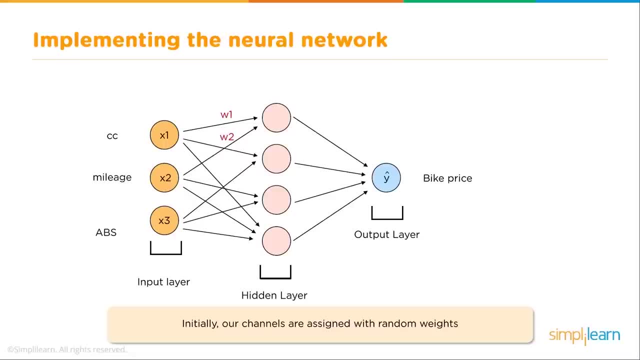 This is important because if you assign them all with the same weight, you might be able to reproduce it. but it turns out that if I put all my weights as one or all my weights as zero, It takes longer to train where if you have random weights, they already have like a little. 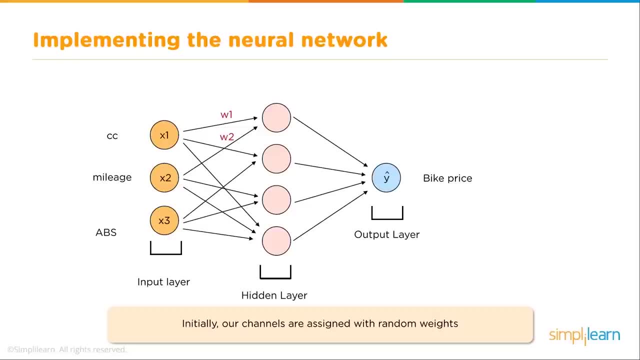 bit of adjustment and ors built in and that will give us a better answer and train faster. Our first neuron takes a value of mileage and cc as inputs. So here comes our computation, whatever those inputs are, and we do that again with the second neuron with those values coming in. 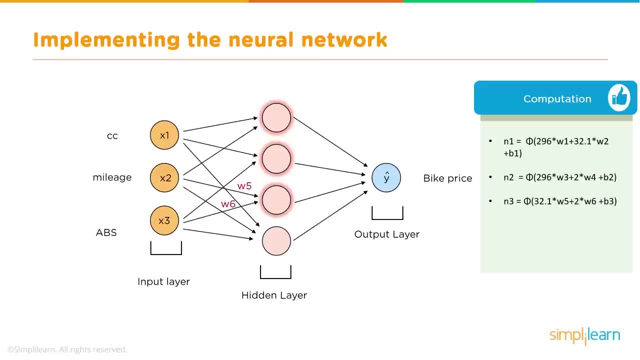 You can see, here we have weight three and so on, and then our third neuron coming down and of course, our fourth neuron. So we're adding all these different values coming in here in our hidden layer. The process value from each neuron is sent to the output layer over weighted channels. 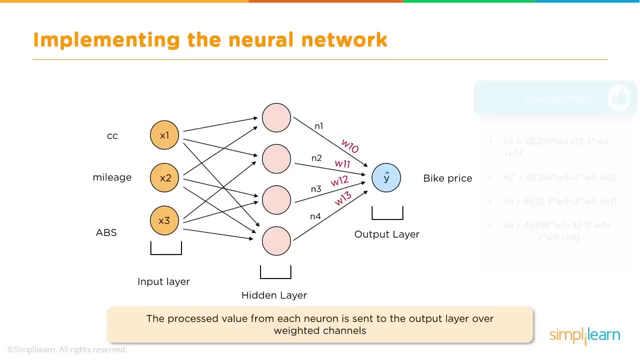 So again, here's our weights coming in, and we have N1, N2, N3 and N4.. Once again, the values are subjected to the activation function and a single value is emitted as the output. On comparing the predicted value to the actual value, we clearly see that our network requires. 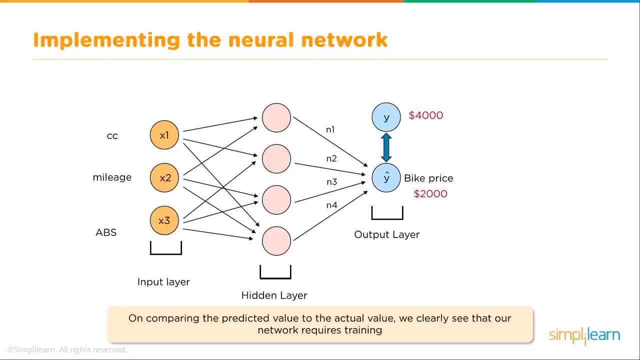 training. So here we have it that our bike price we put out. we thought it was worth 2,000 on our random weights and the bike actually was 4,000 on there. I'm guessing that's not US dollars, Because that would be a very expensive bike, but maybe it is. 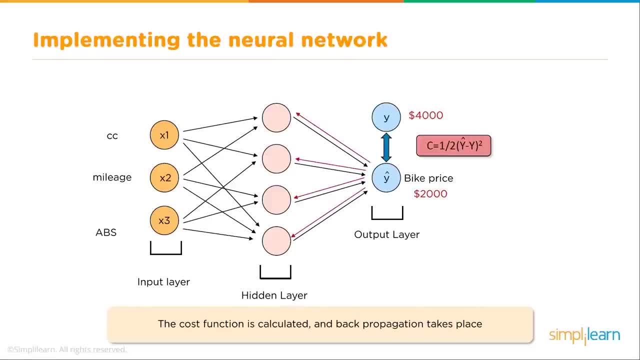 There's some 2,000, 4,000 dollar bikes out there. The cost function is calculated and back propagation takes place. This is pretty simple. you can look at that as we're subtracting one value from the other, we square it and then we take half of that. 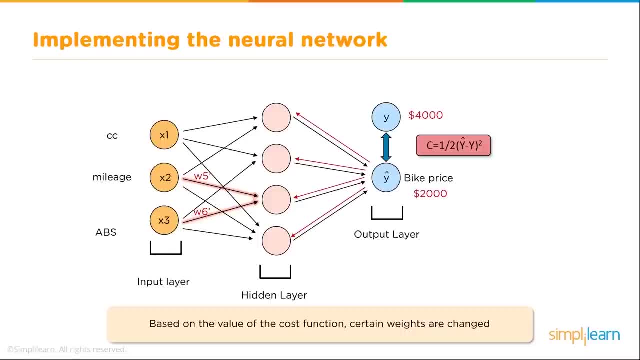 And that is propagated back up and each layer generates its own errors. Let's go back one, because you have your predicted y and your actual y. That goes back to the first layer and then, based on the value of the cost function, certain weights are changed. 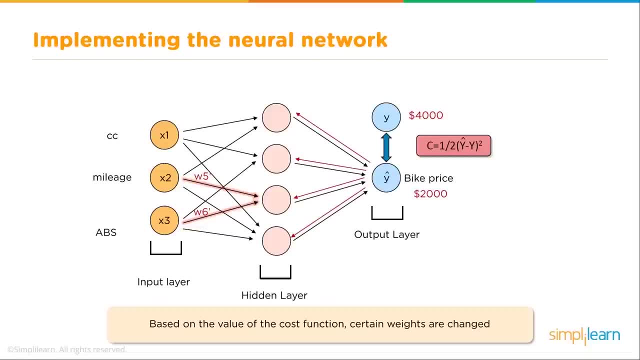 So when we look at the next layer, that error is not the original 4,000 minus 2,000 squared divided by 2. This error is based on the error of each cell generated. How far off is that cell as far as its weights? 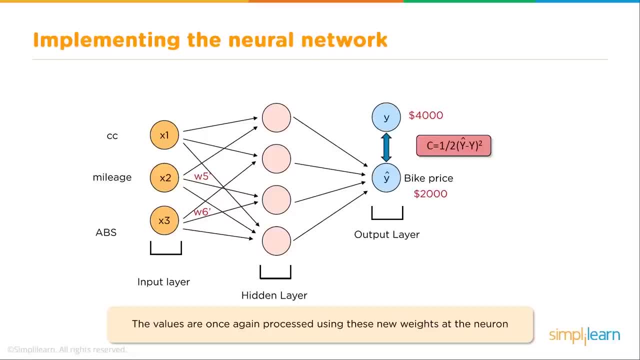 We're not going to show you. it's actually a very complicated differential equation and you can probably write it out if you wanted to. You just write out each formula that goes into the next level and you add them all together and you can write it out all the way through. 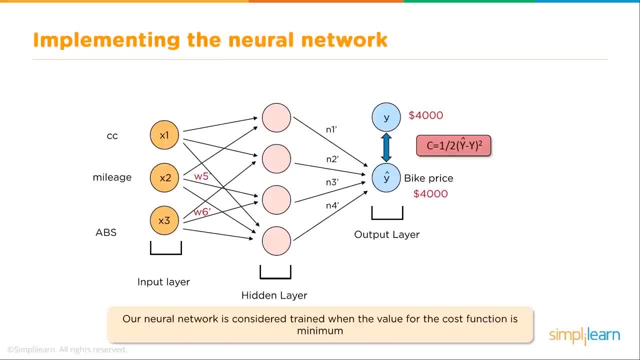 Computers make it, so you don't have to. And our neural network is considered trained When the value for the cost function is the value of the cost function, So when we get our error way down as low as we can, that's when our neural network is. 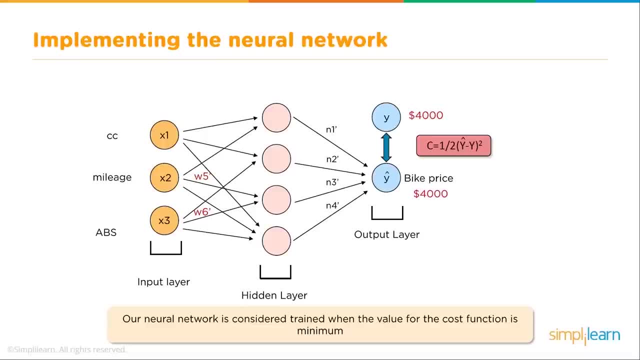 trained And just recently they've come up with all kinds of different means for measuring that particular value, A little bit beyond the scope of today's neural network, but you can actually see how far do you do this until the neural network doesn't need to be trained anymore and you can overtrain. 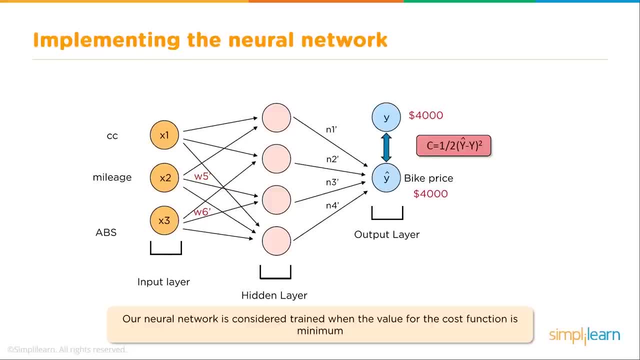 a neural network. Now, the tools that we're looking at automatically let you know when to stop, which is really nice. And that is just. We're at the beginning stages in neural networks and it's just really cool what they can do now and how much of it's automated and how much of it is experimental right now. 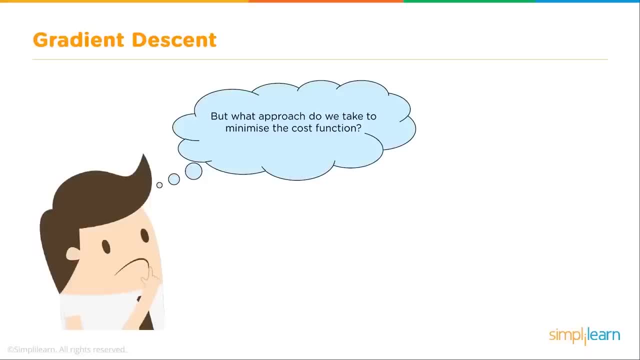 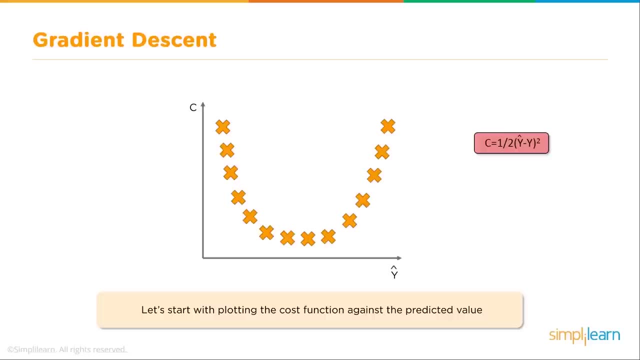 Let's take a look at gradient descent. But what approach do we take to minimize the cost function? So here we have a nice error thing coming in. This is our cost or our error. Let's start with plotting the cost function against the predicted value. 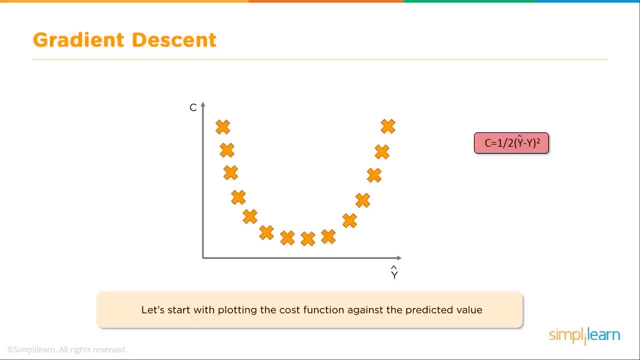 And so you can see they've fed in multiple y's and these are the errors coming in and the cost of each of these inputs and changes going in. So we're going to take a look at gradient descent. Let's see what's going on. 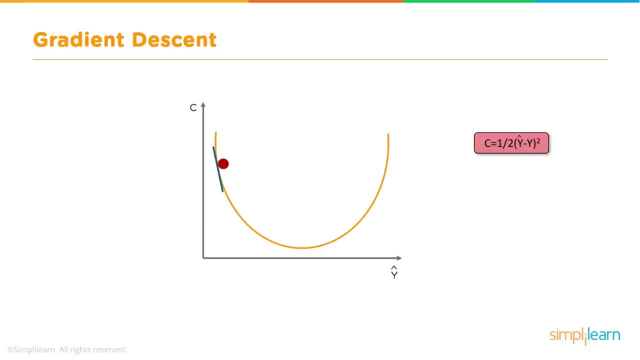 Note, we start at a random point on the curve. So usually you put in, you know you pick up your data and you randomly pick where to start in your data. A lot of times you just run it from the beginning because you're going through so much data. 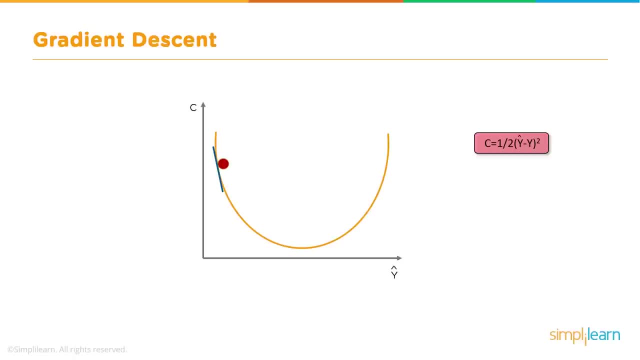 it's not that big of a deal, But you start with one point going in, So your forward propagation goes through and you're going to go ahead and find your cost or your error. It points out on the curve and you can see how we're plotting it right here. 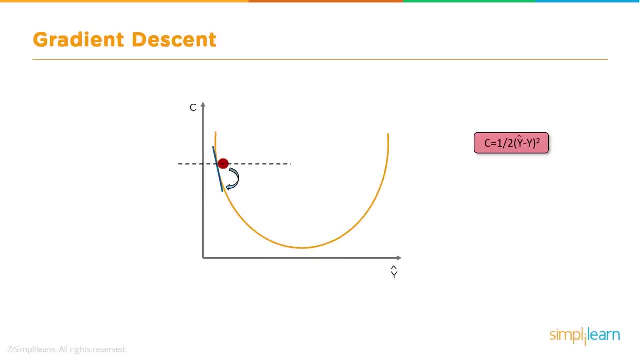 Since the gradient at this point is positive, we may move right. So we're going to move a little bit to the right on here, And this time the gradient is negative, we move a little bit to the left. Eventually, we try out the point where the gradient is zero. 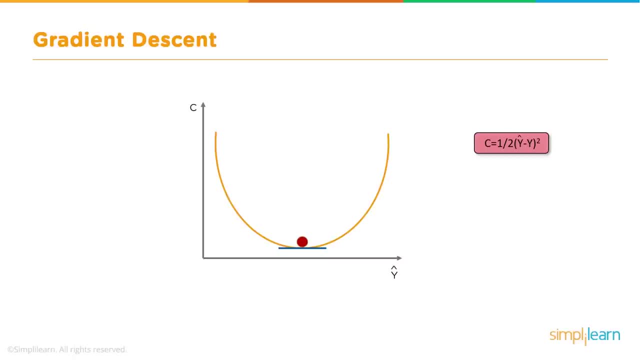 This is the least value of cost function. You have to be a little careful with this, because this particular I mean they make it look nice and simple in this graph. Sometimes these curves look like stair steps, and so there is global minimums and then there. 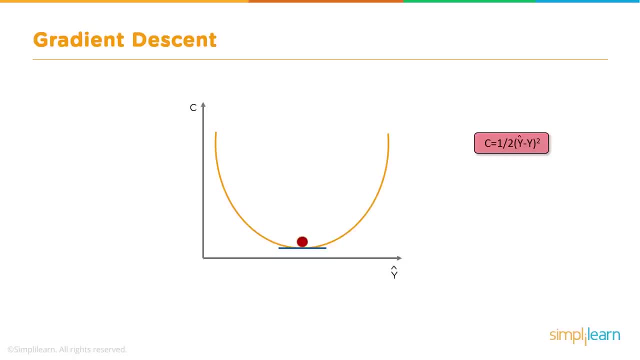 is local. There might be a local point where the gradient is zero, but it's not the global one. So it might be way off to the left, where it just happens to step up, Step down a little bit and you think you're in the right gradient. 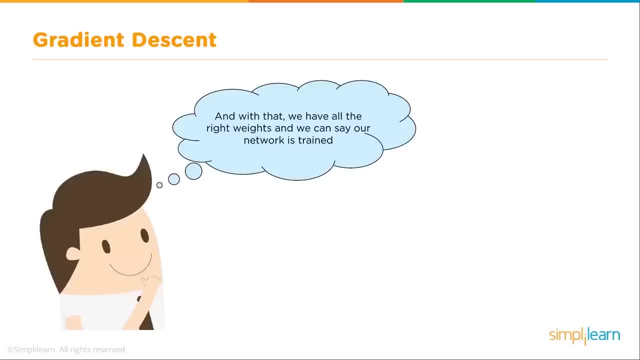 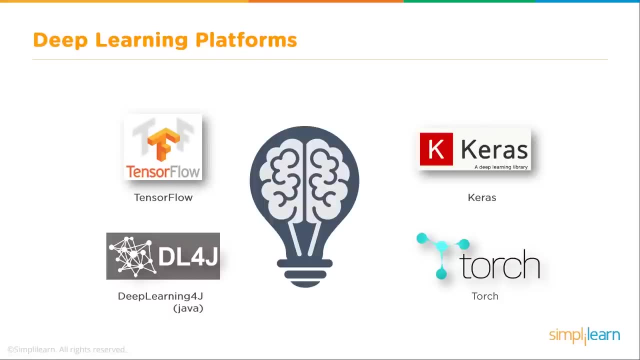 And with that we have all the right weights. We can say our network is trained. So here we have just some major. these are some of the big names out there right now in development for deep learning platforms- TensorFlow, which we'll actually do an example in a minute. 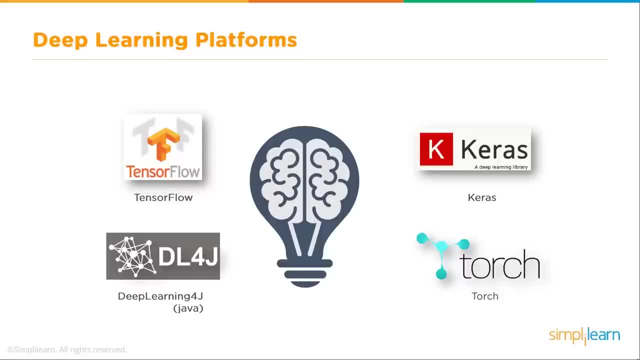 Deep learning for J, which is in the Java platform, so if you're a Java programmer. By the way, TensorFlow is accessed. most people are using Python to access it, but it is a system that's kind of separate from a lot of the programming languages. 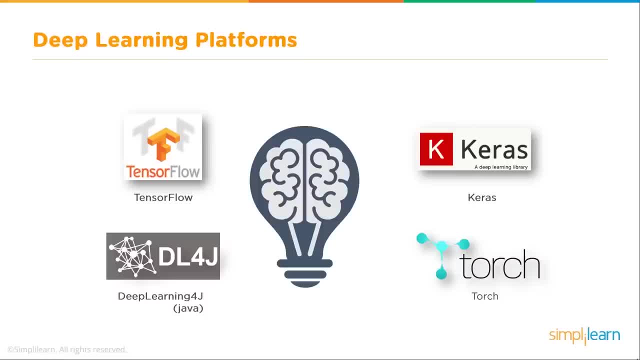 It's a lot more flexible as far as use. Deep learning for J is Java based. And then Keras is just exploding right now, and this is interesting. Keras is working with TensorFlow. It actually can sit on top of TensorFlow and it can also do its own thing. 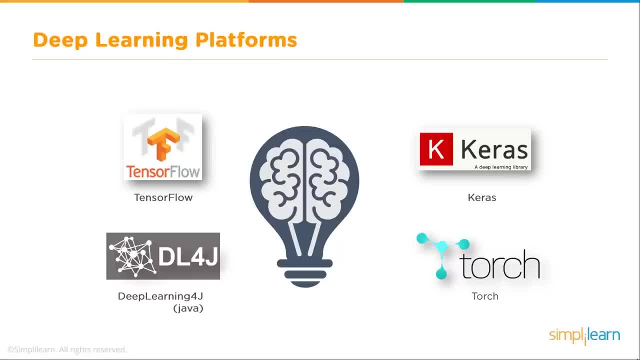 So if you're studying deep learning or getting into it, you'll want to know the basics of TensorFlow, but you're also going to want to know the upper level of Keras sitting on top of TensorFlow. We're just looking at TensorFlow today, though, in our example. 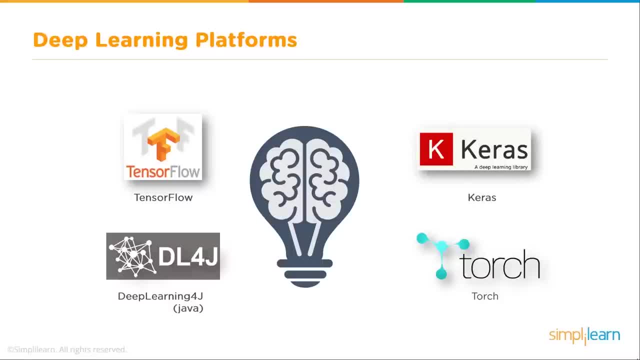 And there's also Torch on there. There's a bunch more that we didn't list on here. Even sklearn, or the side package in Python, has a neural network. you can program a very basic one, And it is the same basic one that you could do in TensorFlow if you stripped everything. 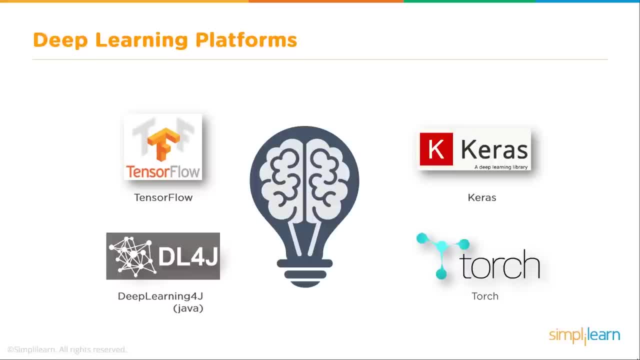 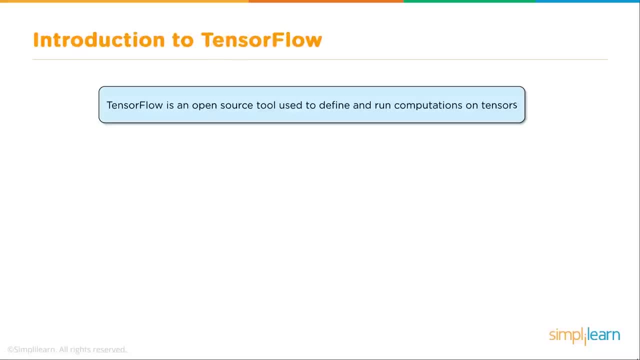 out of it. And then TensorFlow has a lot of tools they've added in, and so has Keras, But we're going to be looking specifically at TensorFlow in our example, And TensorFlow is an open source tool used to define and run computations on what they 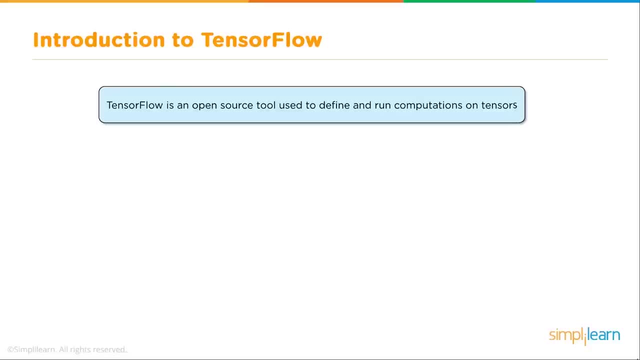 call tensors Very common language now, So more and more we see the term tensor as being a standard In the deep learning language, And this was originally developed by Google. So let's take a little bit in there. What are tensors? Tensors are just another name for arrays. 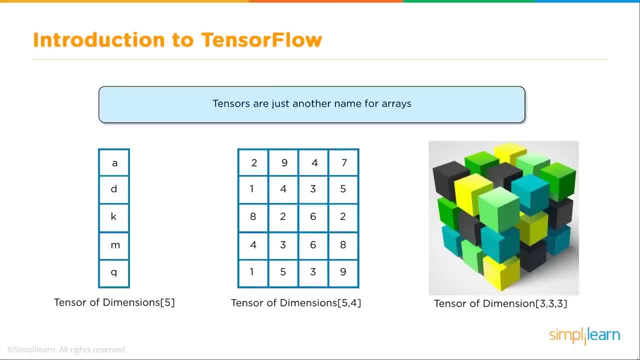 So a tensor of dimension 5.. You can see here we have A, B, K, M, Q, whatever. So it's an array coming in And the tensor of dimension 5,, 4, more like a picture. Very common to see that in a picture. 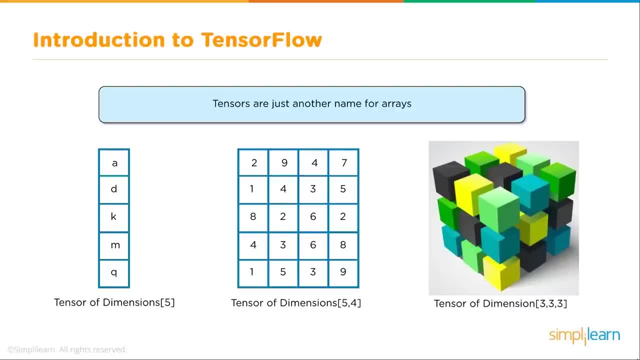 You can also see a tensor even more detailed in a picture as we go to the next one: Tensor of dimension 3,, 3, 3.. This is 3D space. You might have a picture that also has colors. That might be the third dimension. 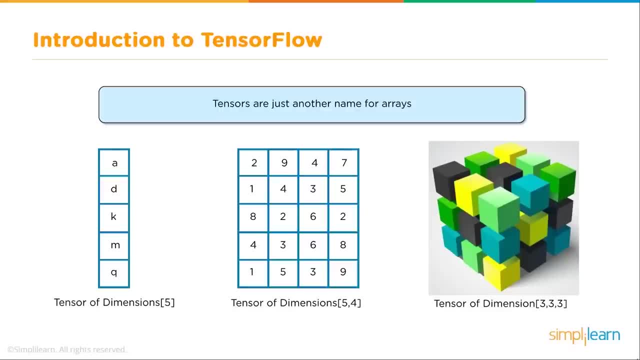 You might have four dimensions, because you have both your grid and your different color channels and your Z plot. You can see where you can now process a very high level set of data coming in, Whether as an image or features. They could be features that have nothing to do with images. 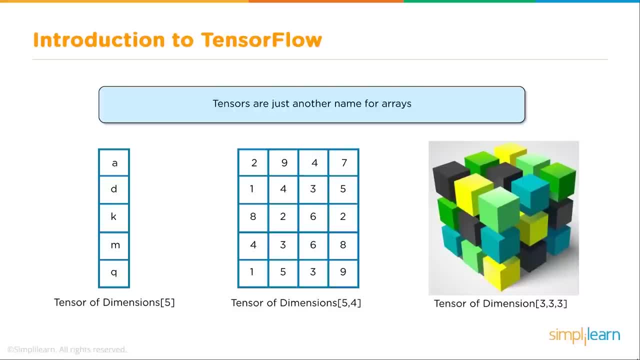 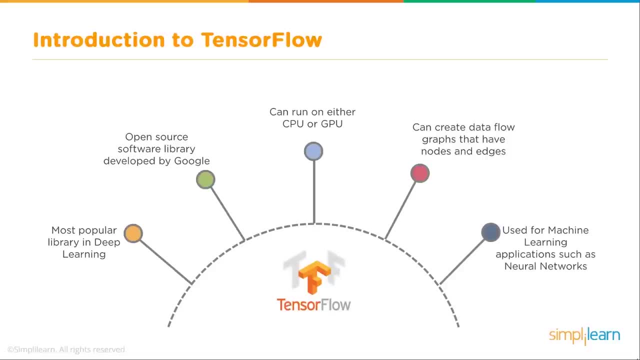 So there's a lot of stuff you can do now with the tensors coming in. This is where the term TensorFlow comes from, So we have right now that TensorFlow is the most popular library In deep learning, And I did mention Keras now works with TensorFlow. 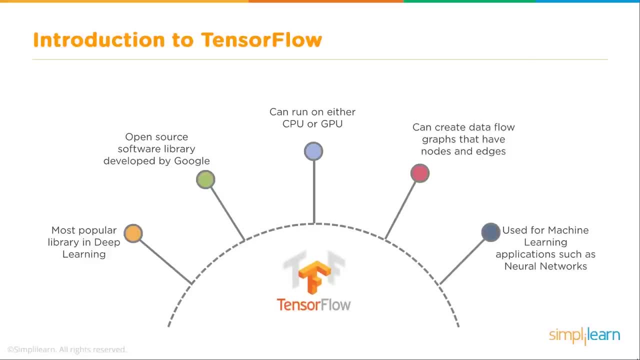 So there's a lot of stuff you can do between the two. It's an open source software library developed by Google. So they hit a roadblock and they realized, hey, this is an infant stage technology. You know, we thought it was going to be the next greatest thing. 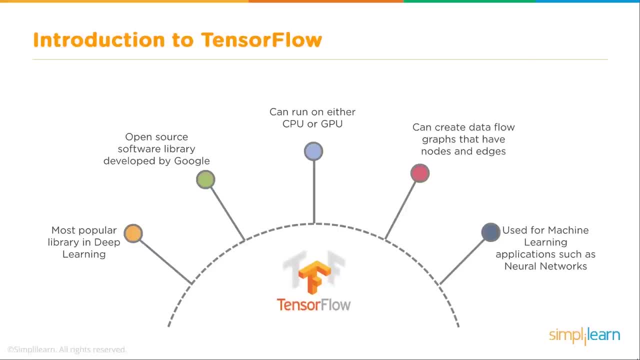 And we were going to have a hold on it, But it's really infant as far as how it's applied and what we can do with it. Let's open source it so everybody can work on it. Let's take it to the next level. 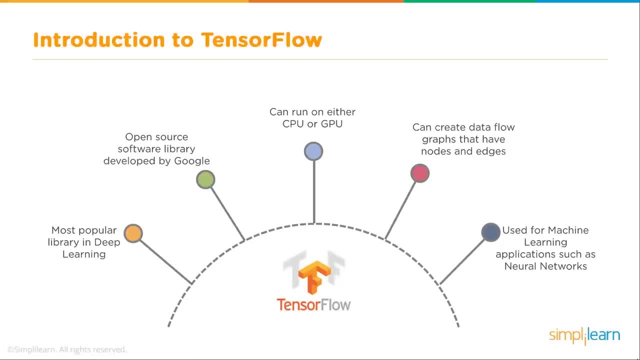 And that's really what open source does to a lot of these packages when they're released And you can run on either a CPU or a GPU. So, when we look at the details, if you have your graphic processing units, what's nice about those is they run a lot faster. 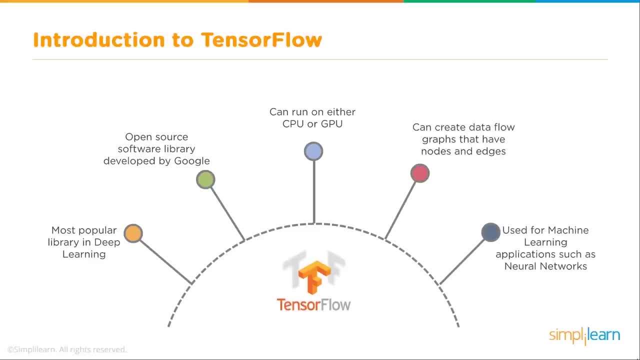 The downside is you have to play with them a little bit to get them up and running And it's a hardware upgrade. When we run it, I'll be running it in the CPU mode. I have played with it in my GPU on my personal computer. 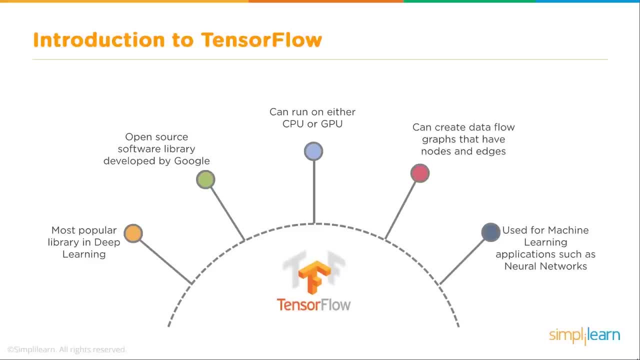 You know it does increase the processing. But I did run into some version problems with my Python and stuff like that, And when I did finally work it out I went back to the CPU because it didn't increase my speed enough for what I was working on. 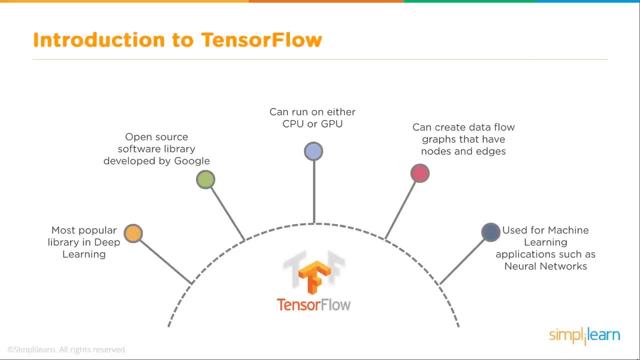 But in a larger group you might be able to put that on. If you're working with a larger stack of computers, you might want to run it in the GPU. You can create a data flow graphs that have nodes and edges. So there's our edges coming in. 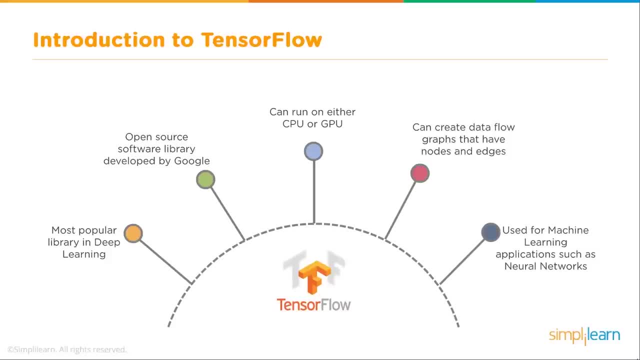 We didn't talk about edges, But that's a very up and coming way of looking at your analytical data- is: how do different nodes connect? What do those edges look like in between them? And it's used for machine learning applications such as neural networks. 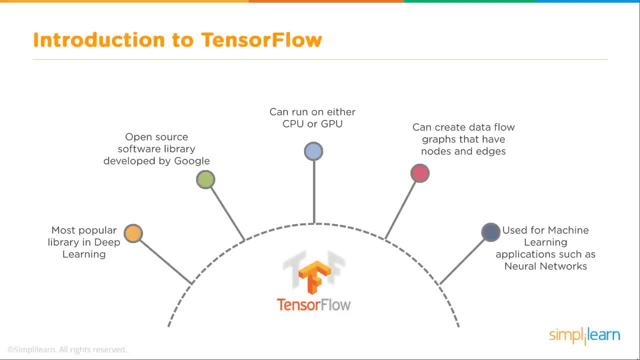 It is mostly a neural network, But they have all kinds of tools which sit on top of our basic neural network. They have new stuff evolving into the TensorFlow library, So it's very much just exploding. Great time to jump into TensorFlow because there's 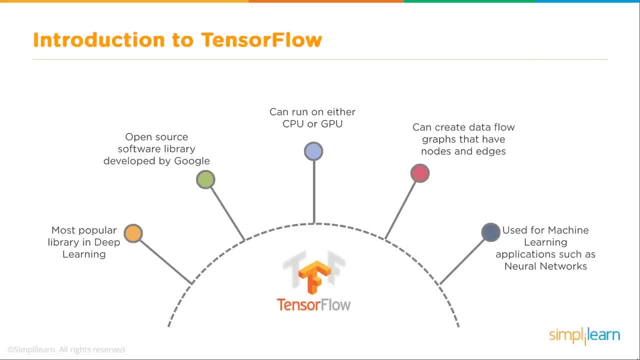 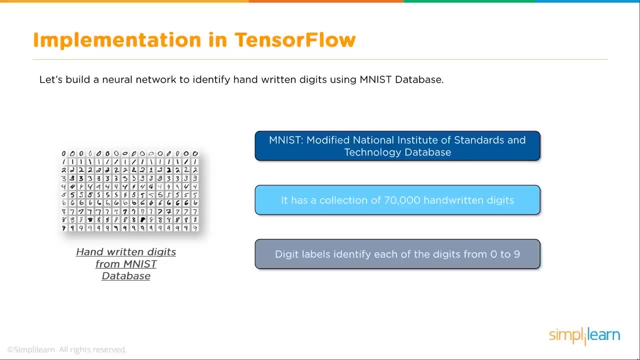 all kinds of cool things we're doing with it and all kinds of cool applications you can now use TensorFlow for. So let's take a look at implementation in TensorFlow, And we're going to build a neural network to identify handwritten digits using the MNIST database or the M-N-I-S-T database. 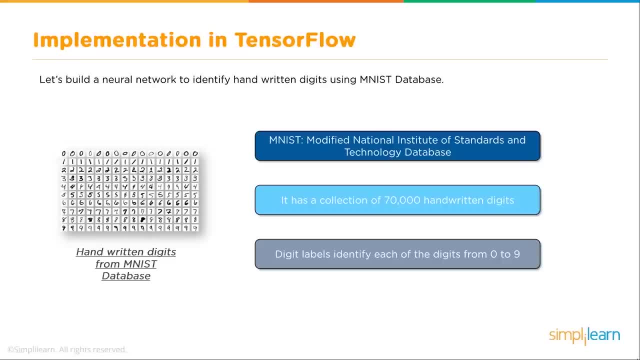 And that stands for MNIST, That stands for Modified National Institute of Standards and Technology Database. It is a collection of 70,000 handwritten digits And the digit labels identify each of the digits from 0 to 9.. This is a cool example, because it's simple enough. 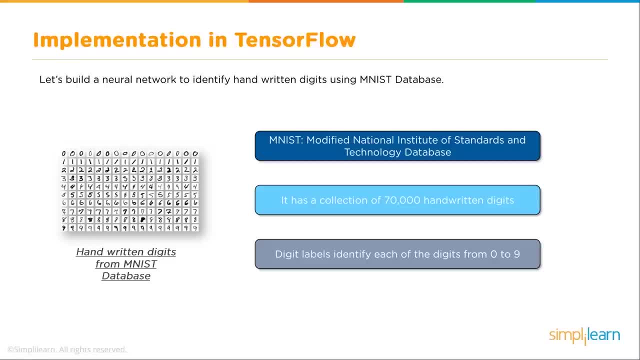 that you could actually run this through some basic machine learning, categorizing algorithms and train them And you'll get about the same answer because, again, it's a simple grid. The digits on the grid don't have a huge amount of variation, like you would say, an automated driving car looking 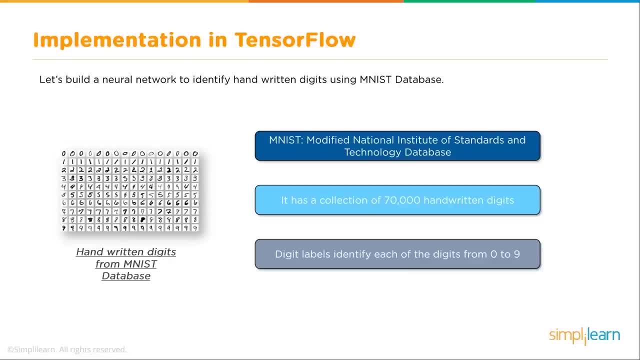 at the environment. So you could still do this with a lot of your different linear models and stuff like that. You could solve this And you'll get about the same answer. When I ran a comparison between TensorFlow and between some basic regression models or category models in machine learning, 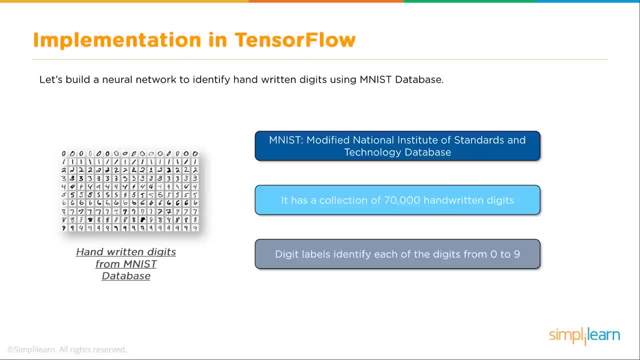 they came up pretty even as far as their output. So this is kind of where we start to see the complexity of something coming in, in this case a tensor or a grid of information where the deep learning model does as good as the regular models. 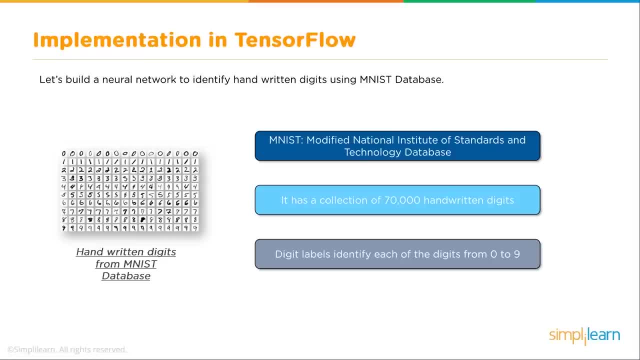 And when you get past this kind of complexity and features, suddenly the neural networks come up with better answers, better solutions and a better build. And that's why there's such a move into neural networks is we live in a complicated world And it's just really cool we can do with this. 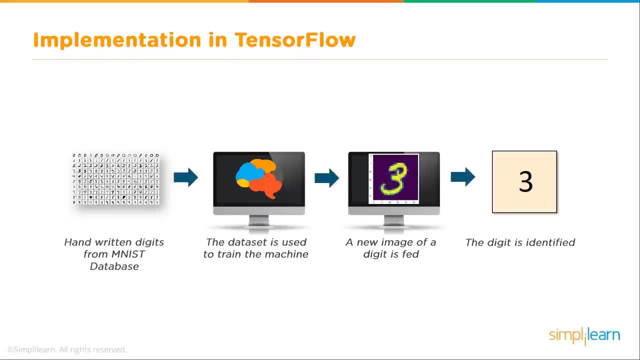 So the handwritten digits from the NIST database they come in, The data set is used to train the machine. A new image of a digit is fed and the digit is identified. And if you've looked at any of our other machine learning tools where we're doing training, where we train our model to fit, 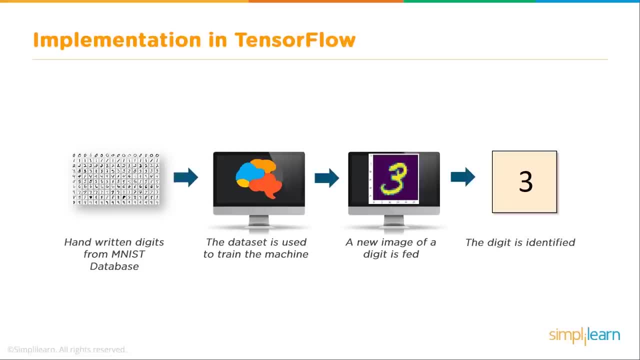 and then you test it out. this will look pretty familiar And there is some tools out there for, say, untrained categorizing, where it's just looking for features that fit together. So there are tools that don't need that training, But this is where we're talking about neural networks. 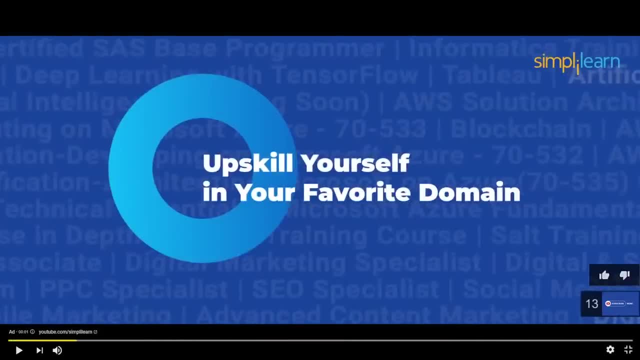 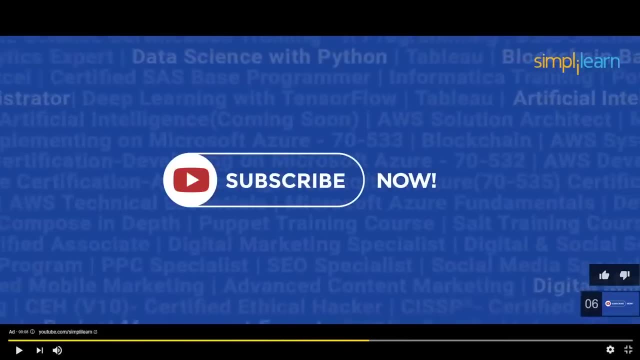 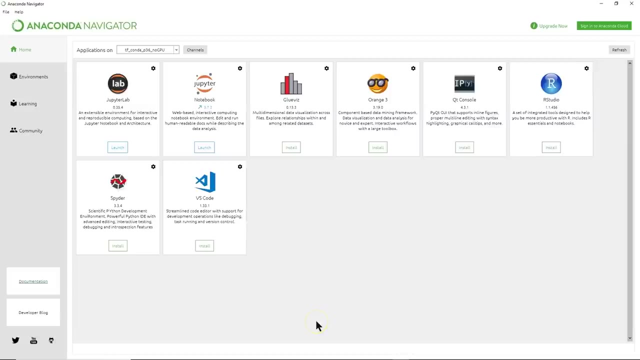 We do need to train them, And this is what we're looking at. So for this I'm going to use the Anaconda Navigator, just because it's a very nice visual tool. You might be in PyCharm or one of your other IDEs for editing Python, because we are looking 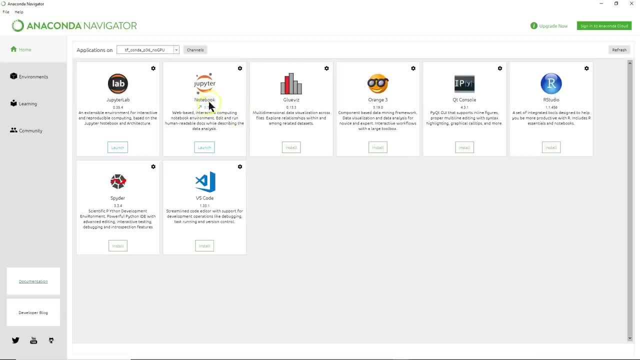 at Python, TensorFlow And under Anaconda. we have the Notebook, which is something we use pretty regularly, And they have the JupyterLab. The JupyterLab is the Jupyter Notebook, but with tabs and a few new features, So we'll be using the Jupyter Notebook. 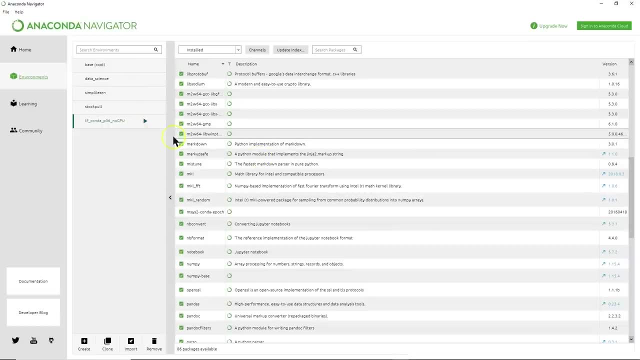 And under the Environment you'll want to go ahead, and if you haven't yet, you'll see that I have a number of different setups in here. Right now I have the Python version 3.6 and the TensorFlow. In this case I have TensorFlow 1.12.. 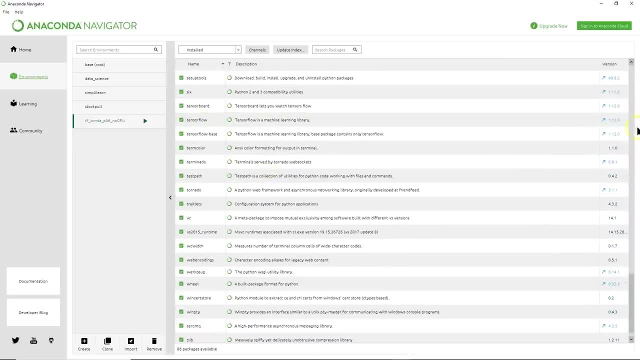 If we scroll down, you can see that Here we go: TensorFlow and its version 1.12.. And in here, if you haven't yet, you'll need to install those and go in and just open our terminal. And if you've never used the Anaconda Navigator, you can do that here. 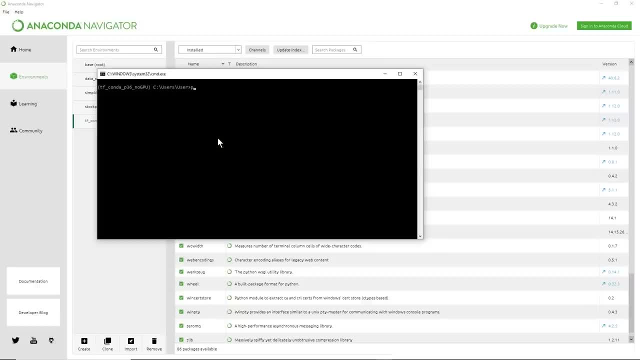 The Anaconda or, if you're in your other thing, you might have something simple like pip. Conda is what I use for my install and you can simply do conda, install tensorflow. That should bring in the most current version. Now, when I installed this a few months ago, Python version. I'm not going to run this. because I already have it installed on here. Python version 3.7, the newest one out- still had a couple glitches with the TensorFlow. I believe they fixed it as of writing of this, but I'm going to stick with 3.6, just so I. 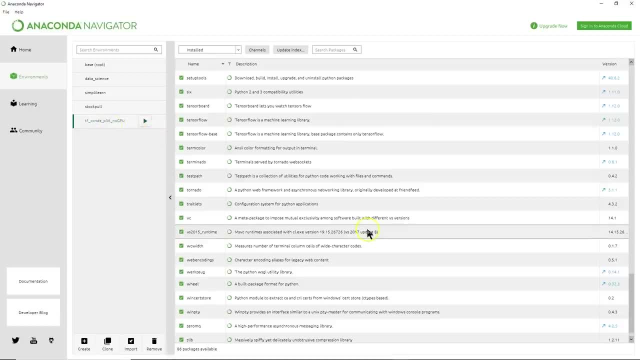 don't get any surprises on there. So this is Python version 3.6 with TensorFlow 1.12 on here, And if you haven't installed it yet, you also want to install numpy for this example. That's numbers, Python or N-U-M-P-Y and you can just simply run install on there. 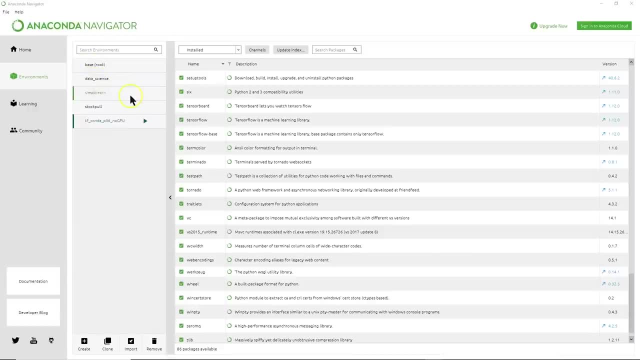 Keep in mind: if you're in Anaconda and you've created one of these environments specific to this, keep with conda. if you're going to use conda, If you're going to use pip, keep with pip. Don't install one package with pip and one under conda. 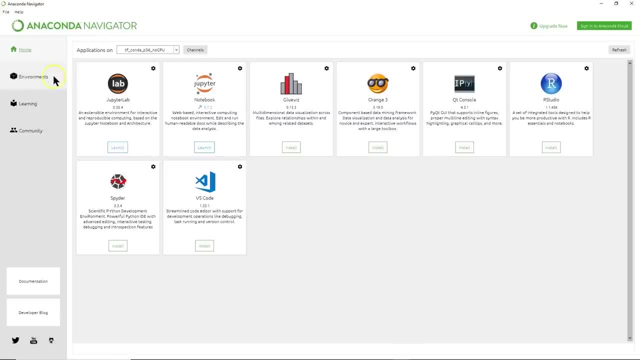 Because that's how they track those version numbers and how they fit together, and you can end up with a problem. Pip doesn't see conda, and vice versa. So just keep that in mind when you're running your installs. We'll go ahead and open up JupyterLab and we're going to launch that. 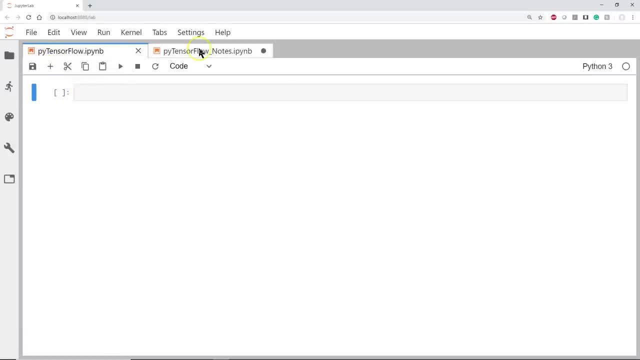 So here's my JupyterLab. One of the really cool features of JupyterLab is you have tabs now so you can open up multiple notebooks. This is nice because I have my notes I'm working on and then our actual window. we're looking. 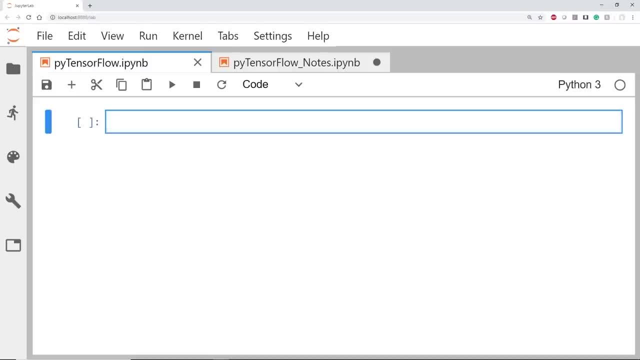 in And we'll go ahead and zoom in a little bit here. There we go, So you have a nice, Hopefully easy to see, And then we'll go ahead and do a simple Get our imports out of the way. So we're going to import our TensorFlow as tf. 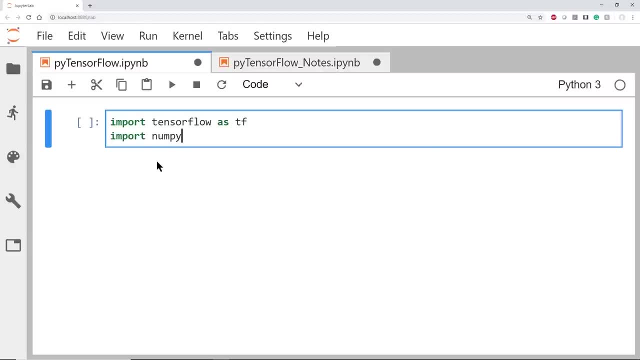 That's pretty much a standard for TensorFlow, NumPy, our numbers, Python as py And we'll import our matplotlibrary as plt. Again, these are very common, So if you see tf or py or plt, this is a standard that most people use. 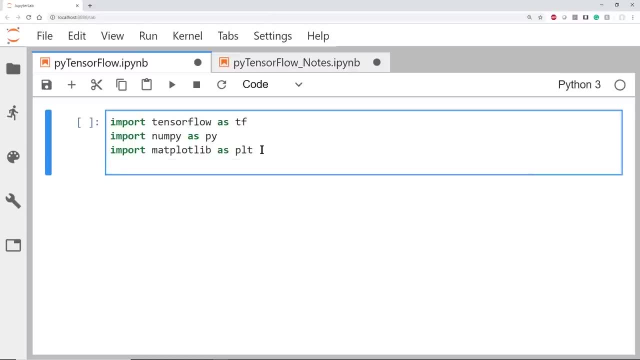 Do you have to? No, You can just do import numpy instead of doing as py, And then from TensorFlow: TensorFlowexamplestutorials. This is always nice because they actually include the data set we're going to play with. So we're going to import input data. 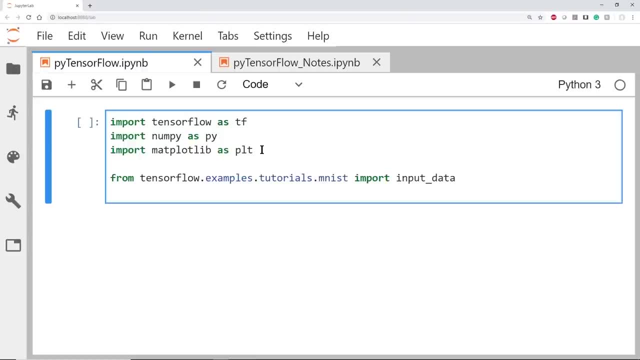 So there's our data coming in. That's all we're doing is telling it this is where it's coming from. And if we're going to tell it where it's coming from, we need to go ahead and create a variable with that information in it. 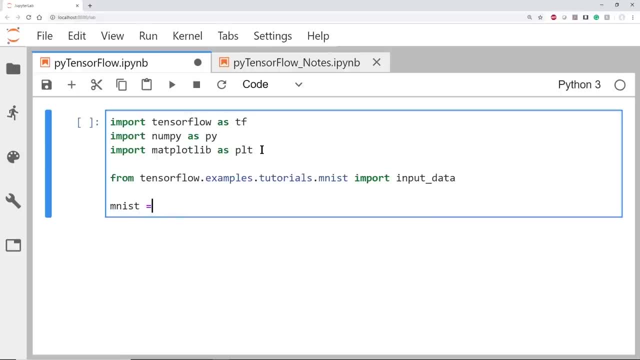 And we'll just call this mnist, nist or minst. You know, I don't really know how they pronounce that. I should probably look that up. It's a very common data set to use And there's our input data. 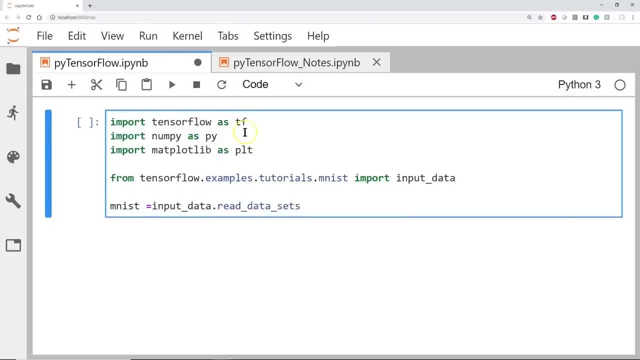 And we're going to read data sets And this is: If you look at this, we imported input data from our TensorFlow And so this is a TensorFlow read statement for their tutorials. So this isn't like some special Python setup, This is just their setup. 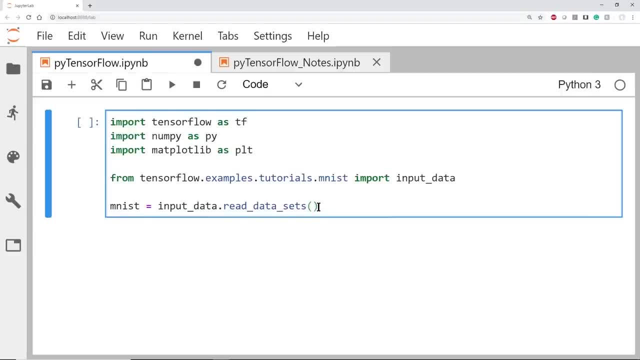 It makes it easy to pull it in. So once we get into their data sets, we need to go and tell it what kind of data set. And again, this is what we brought in, but it's going to be the ninst data. 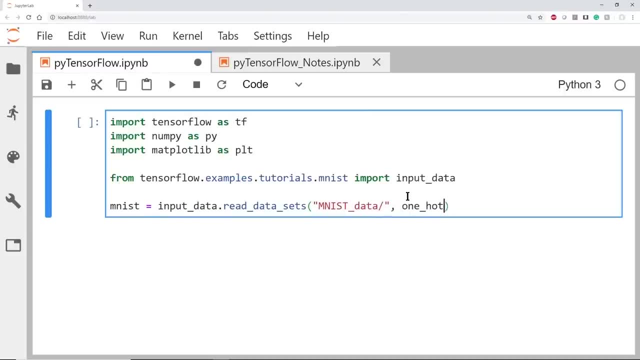 And this part is very important- One hot equals one minst. That's true. This means that instead of importing a value from zero to nine, we evaluate the data set. It's going to bring it in as one hot. Whenever you see one hot encoder, we're flattening that out. 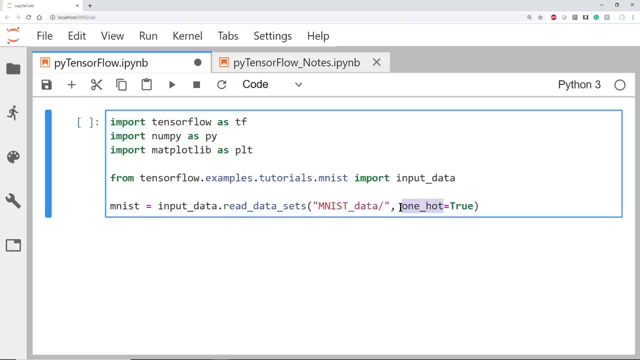 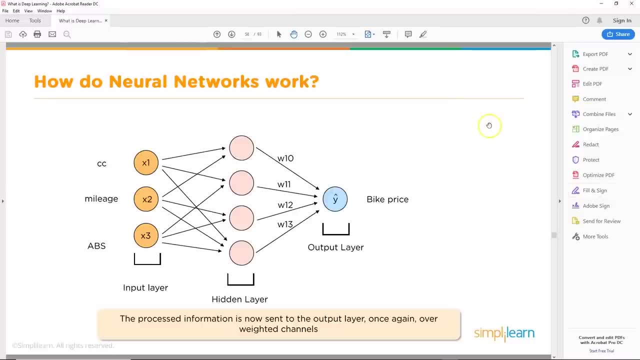 And we have true false for zero, true false for one, true false for two. So our output, if you remember from our output, from the slide we did earlier, in this case I grabbed the one for bike price. It doesn't really matter which one we use. 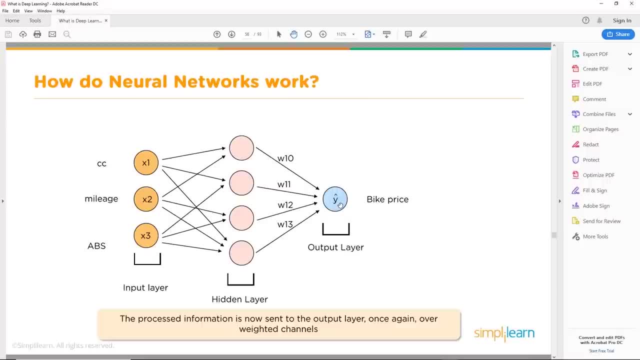 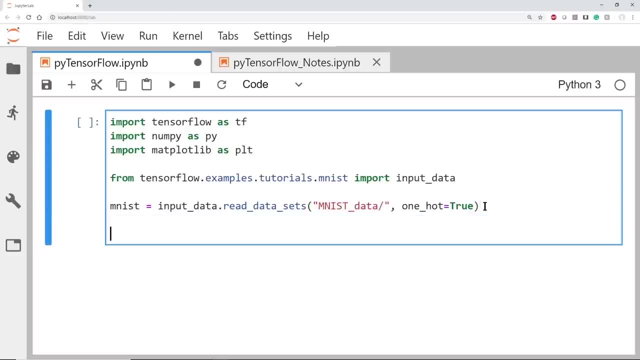 This has one output, So we have our bike price On this. we're going to have, Instead of one output, we're going to have, ten outputs representing each of the digits in there, And this code really isn't going to show us anything. 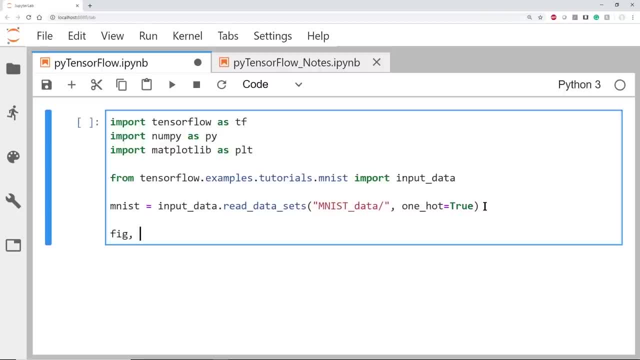 It's good to see what we're actually looking at. So let's go ahead and do a figure ax equals, go into our plot library, subplots ten, comma, ten, And that is, if you remember, we talked about tensor, tensor being data coming in. 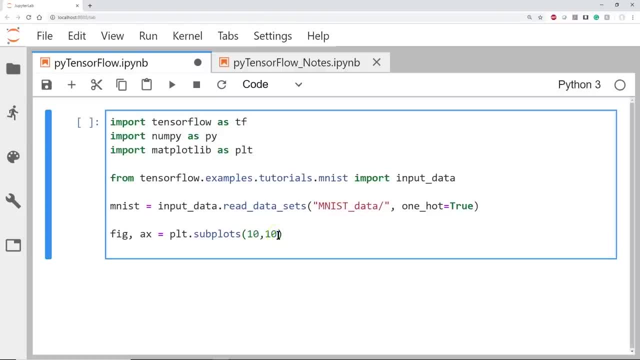 This is a ten by ten grid, or a hundred pixels on there, And if we're going to display it, let's go do k zero. Okay For i in range ten, just a simple loop through on the data. let's do what is it for j in? 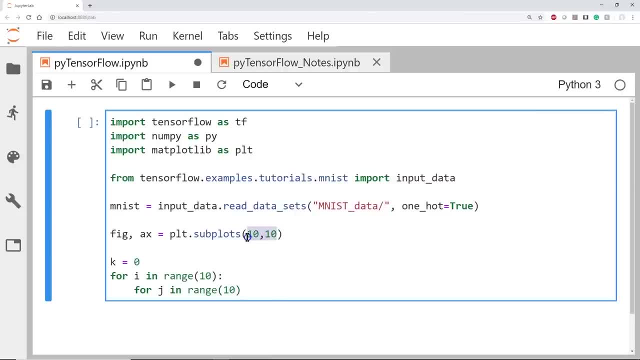 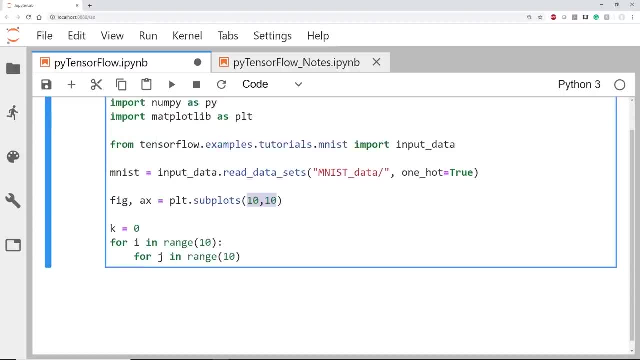 range ten. So I actually misquoted that ten. ten by ten is not the actual size of the pixels. The actual pixels are going to be when we look at the shapes, and we'll get into that in just a second here. We'll take a quick look at the shape on there. 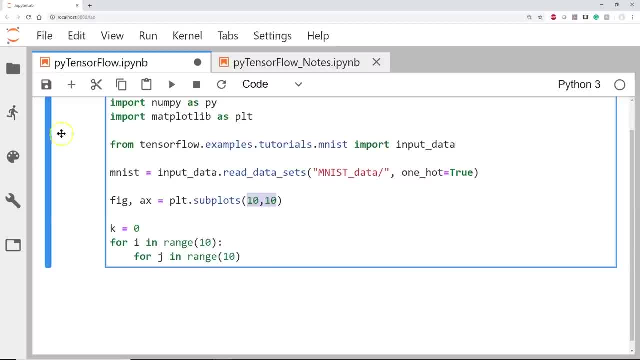 It turns out they're. what are they? they are, I believe, twenty-eight by twenty-eight. So let's take a look at that And we're just going to plot these. What are we looking at? What are we working with? 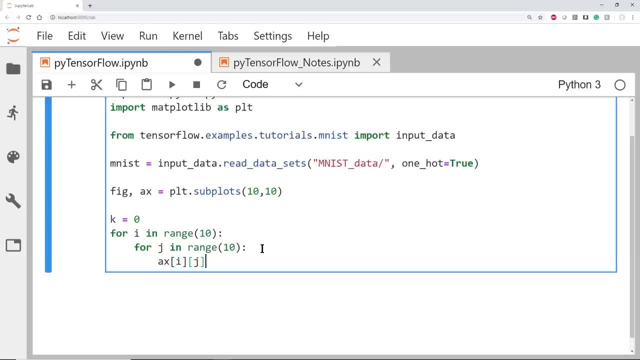 As a data scientist, you should always be looking back at your data and seeing what it looks like You can get that human perspective, because you just never know. You know the computer might put something out that looks makes no sense, and at that. 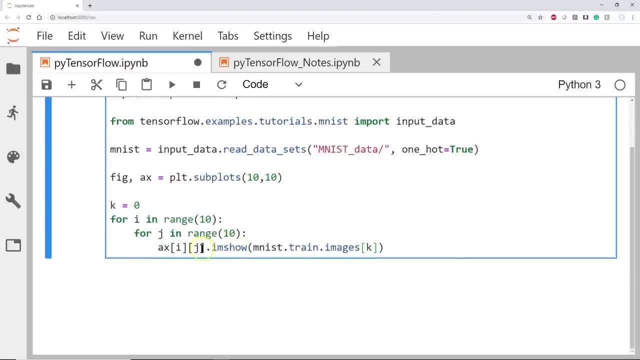 point. you want to go back and reevaluate what you did. So we're going to go ahead and plot. We're going to plot ten digits. you know ten of the digits by ten of the digits, and here's our ax. We'll create the ij on our subplots and we're going to do an image show. 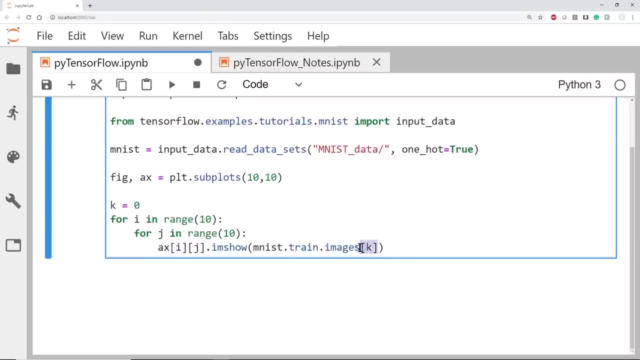 We're going to look at the training image for images of k And then we want our subplots. Okay, We're going to reshape this, We're going to reshape this and we're going to reshape this twenty-eight by twenty-eight. 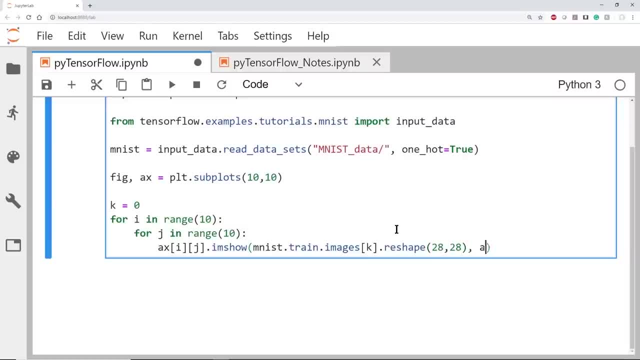 That's how I knew I had it wrong is because I looked down my notes and I was like: oh no, that says twenty-eight, It's not ten by ten, And I should know that already, because I've done enough messing with this data set. that. 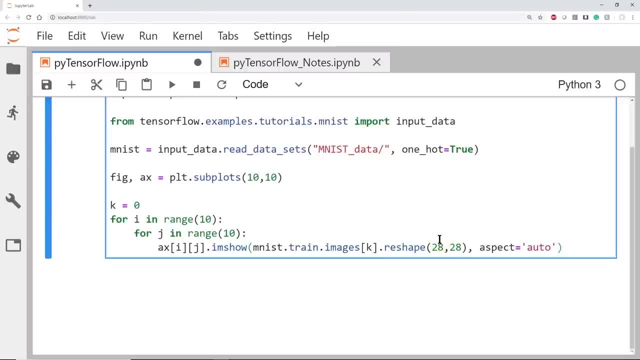 I should remember, But it's twenty-eight by twenty-eight and the aspect we're going to do is auto And this is all. if you look at this, here's our variable nist. The nist is coming from data set. 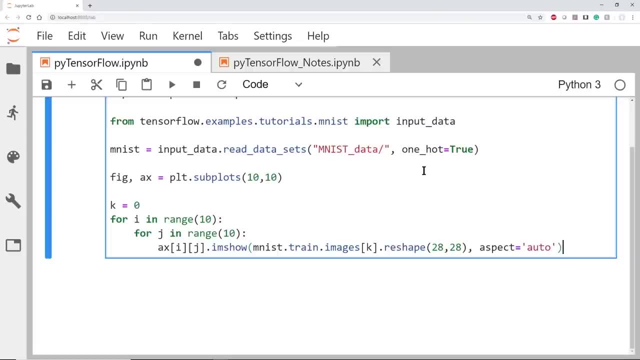 So this is all part of the tftensorflow learning or examples tutorial in there, And then we'll go ahead and do k. Okay Plus equals one, so we just keep paging through our different images and let's see what that. 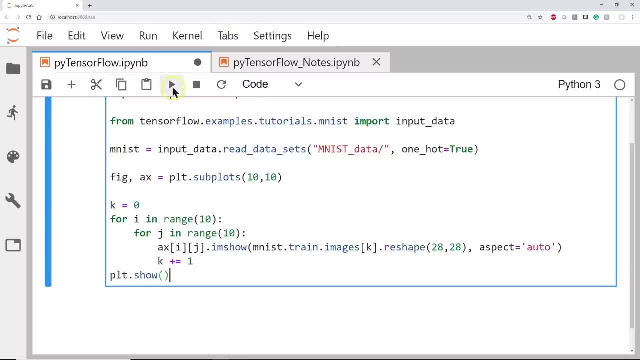 looks like Let's go ahead and do a plot show And we'll go ahead and run this so we can take a look and see what we have here. And so we have a nice plot here and you can just see that we have some random numbers. 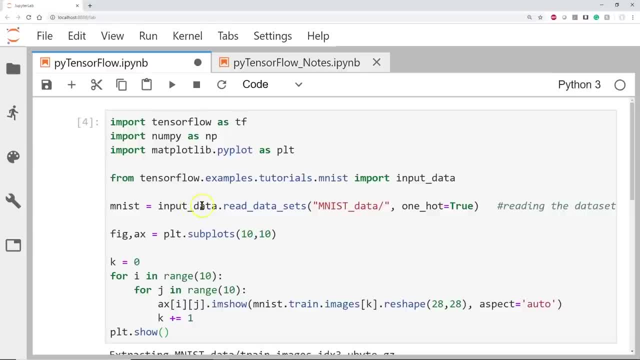 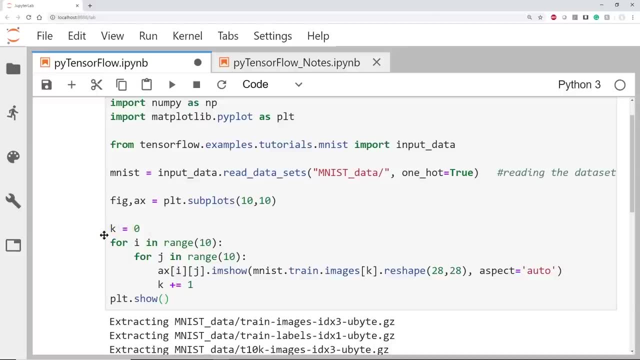 showing up in each one of these little subplots. If you're wanting a copy of this code, put a note down in the YouTube video and let us know, or come visit us at wwwsimplylearncom and we'll send you out a copy of what we're. 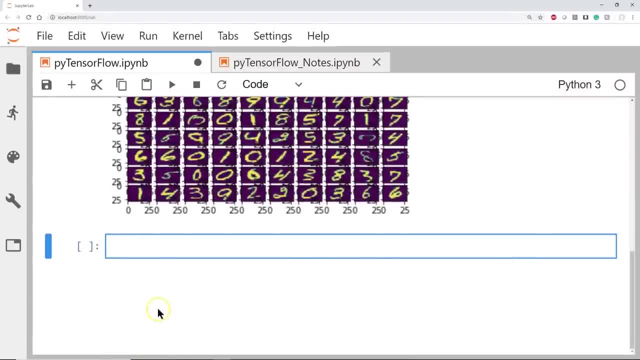 working on and get a copy of that for your own setup. So now we've taken a look and we can just see here's our pictures that are coming on. We've plotted them, so we have an idea of what we're looking at. 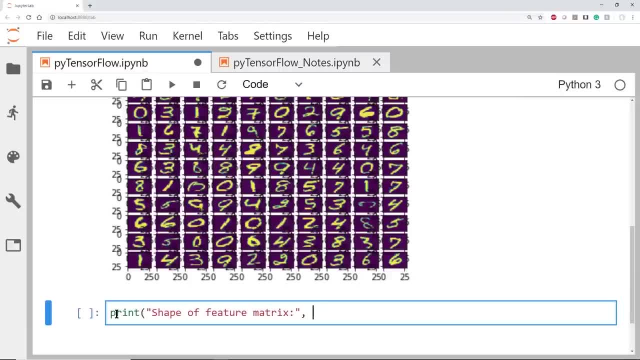 Let's go ahead and print. let's look at the shape of the features. So when we have this, we have our nist train images and we'll do the shape on there. Let's take a look and just see what we're looking at as far as our count and everything. 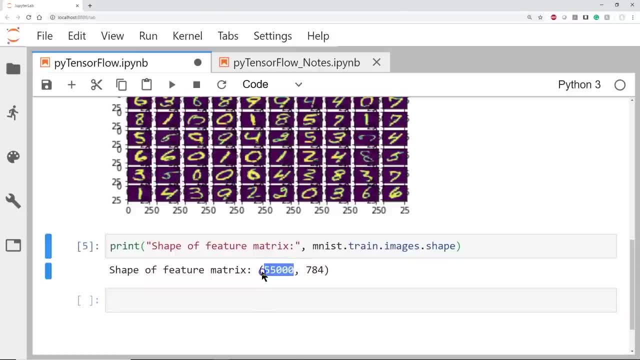 And so you can see, here we have 55,000, that's basically how many images we have, and this by 784.. Okay, So in this data set there's also our labels, so let's take a look at that. 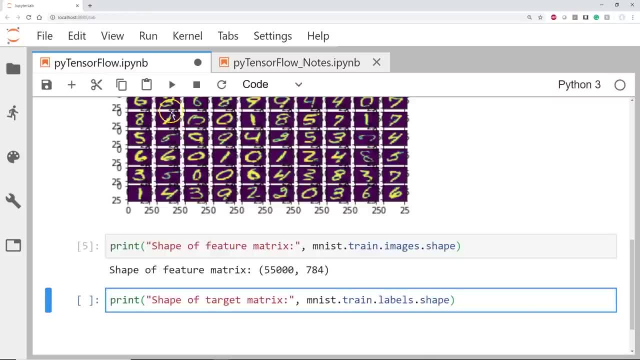 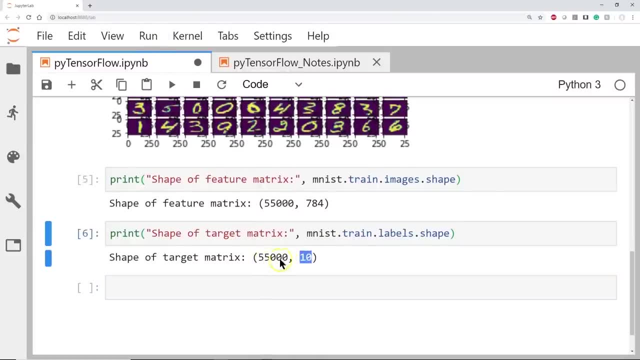 We have our nist train labels shape. Let's take a look and see what that looks like, And there we have 10, because there's 10 digits, so we brought in, that's our output we're looking at, And so we have, there we go, 55,000, they match. they should match because you should. 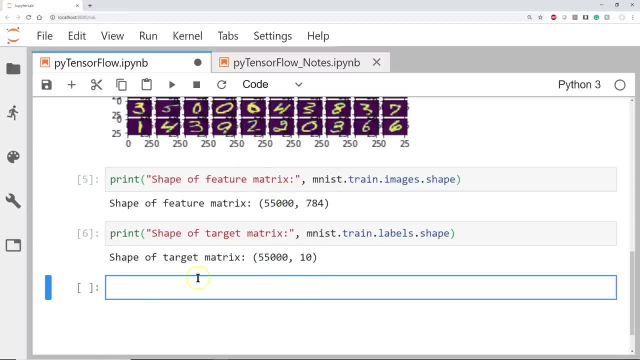 have equal numbers in both of those you know. here's our data in and here's our answer. If you remember, this is a bunch of zeros and each one will be 0001,. would be what letter four? something like that. 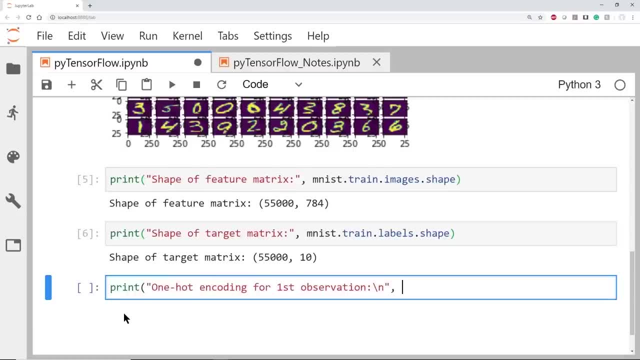 So let's take a look at what our one hot image is. Let's see what encoding did for the first observation, And this is when we're exploring data. you really want to dig in there and just see what the heck am I looking at? 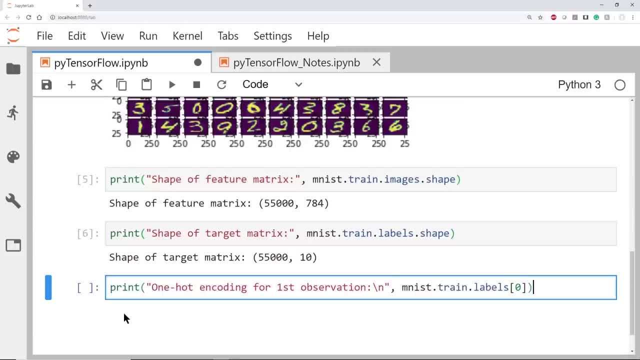 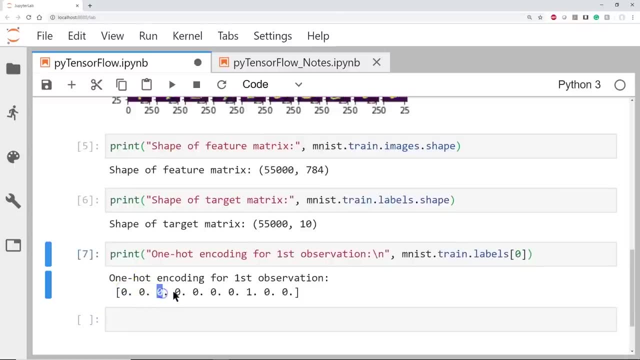 So we're going to look at the labels- and this would be the first label that comes up And we'll go ahead and run this And we look at that. you can see, this is what I'm talking about: Zero, zero. our one is zero. two is zero. three is zero. four is zero. five is zero. 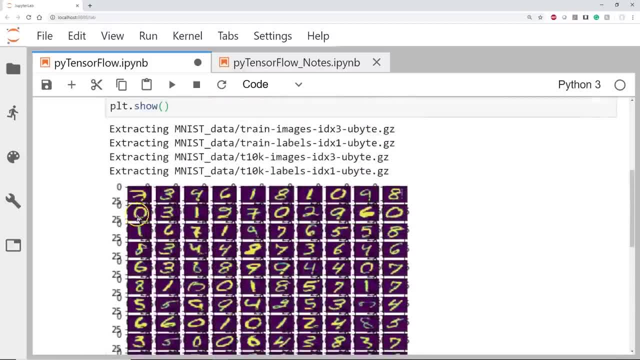 six is zero, seven equals one. So our very first label is a seven, but our very first label comes up that it's a seven, And so we don't have like: zero, three, four, five, zero, six, zero, seven equals one. So our very first label is a seven, but our very first label comes up that it's a seven. So our very first label is a seven, but our very first label comes up that it's a seven. So our very first label is a seven, but our very first label is a seven, and that comes. 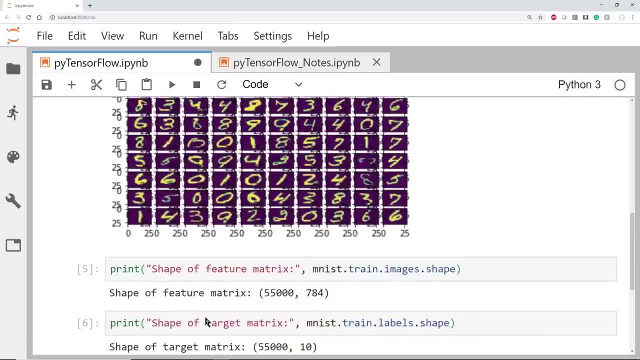 from zero to nine and once you go through nine we have a bunch of zeros and just the one to mark it as a seven on here. So now we've kind of looked a quick look at the data And in here you might ask some questions like: what is 784?? 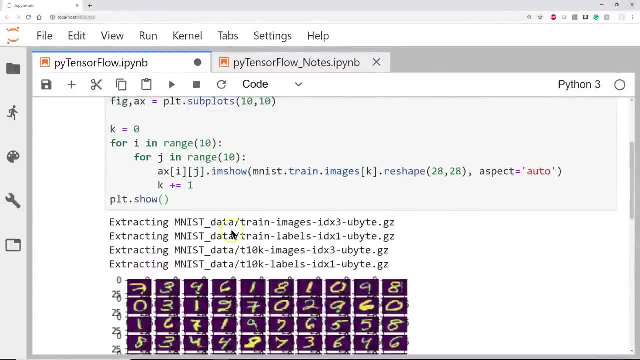 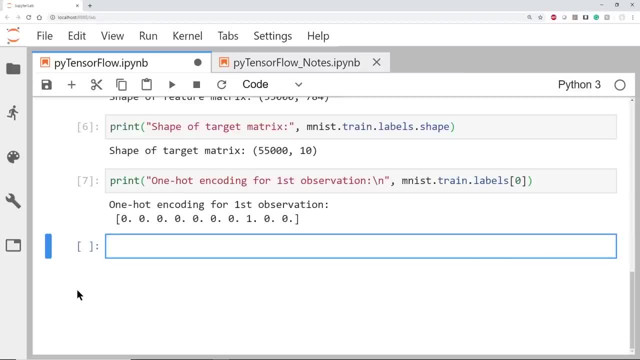 24 times 24.. Remember, that's the size of our grid on there or our tensor coming in. So 784 is a set up on there And we've gone through all this. viewing the data, We'll go ahead and start looking at our tensor flow. 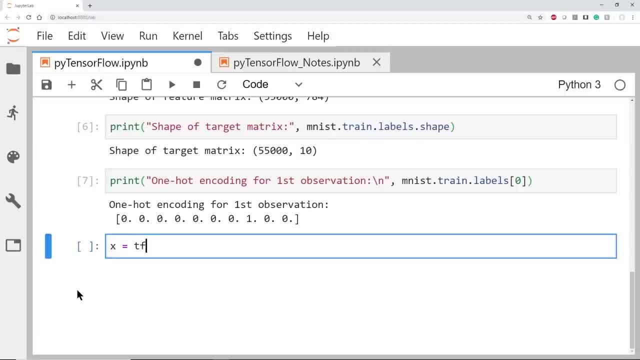 So let's take our x variable. This is going to be our training set. We'll do a placeholder and then we're going to have these come in as float. now, if i remember correctly, they're actually, you know, zero or one for the values, because they're either, but we have them coming in as a. 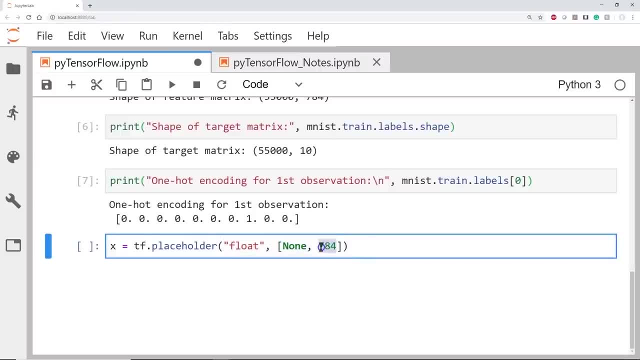 float value and we have a little bit of a shape coming in here and there's our 784, uh. so we let it know that this is what's what our input is for our tensorflow and this is our training set. so we'll just put a label on there to help us track that train set and then w and with w, we'll go. 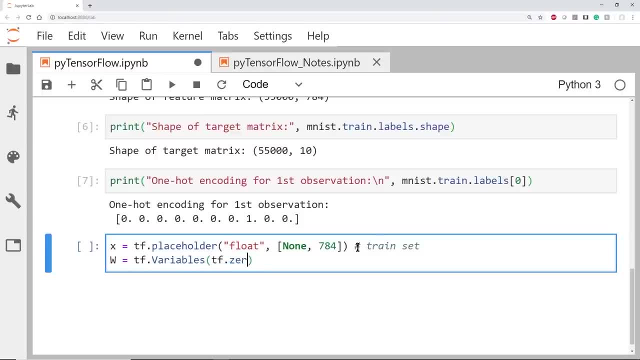 ahead and do tf variables, and we'll do this as zeros variables, tf zeros, and we'll set this as 784 by 10, 10 being the output, 784 being our number of variables in, and this is our weights. remember, we have a bias in there too, and i'll go back over this in just a second as we see how that fits. 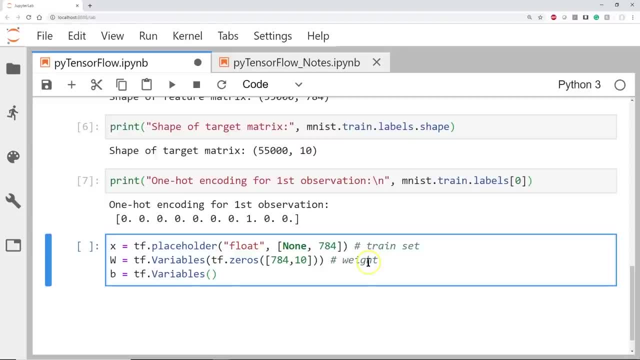 together in our tensorflow and we'll do this one with our variables. again, we have 10, so we're going to do the bias, we do it the same kind of format and setup on here and so we'll do that as as tf zeros of 10. so just create an array of 10. 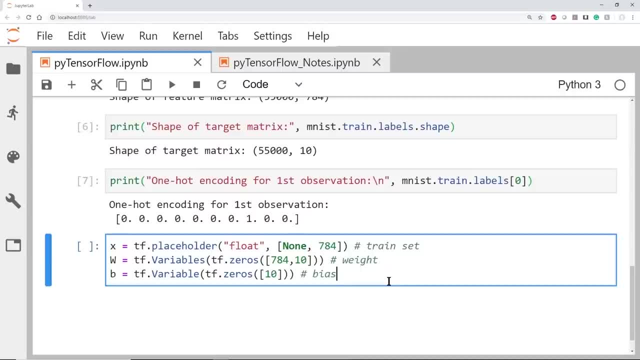 there and this is our bias. so, with these three lines, um, and there's actually, they're coming out with the eager execution which would bypass some of what we're doing, but this is important to understand- is, the first thing you have to do with tensorflow is we have to allocate a space for the 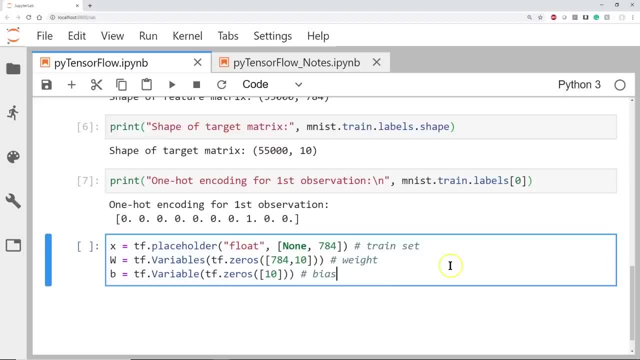 variables and our tf placeholder and our tf variable with our weights and our biases. this actually hasn't done anything, you yet? so all it is is placeholders. that's why it's okay to use zeros. you could have just as easily used ones or anything else, and it wouldn't matter. the next stage is to go ahead and set up some of 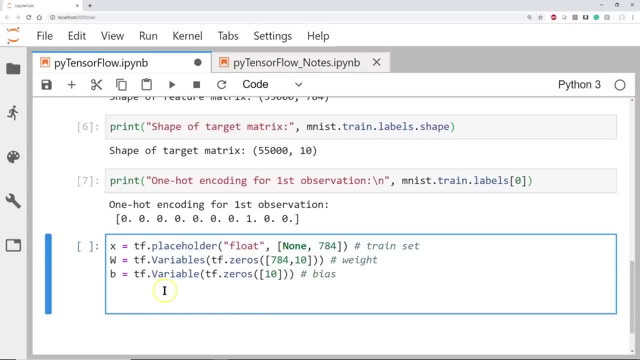 the functions going on. but before we do that, just note that this hasn't done anything, even if i execute it. all it's done is created placeholders until we do the final initialization, and so we need to go ahead and set up. we'll do. y equals tfnnsoftmax and the code for this is tfmatmul xw. 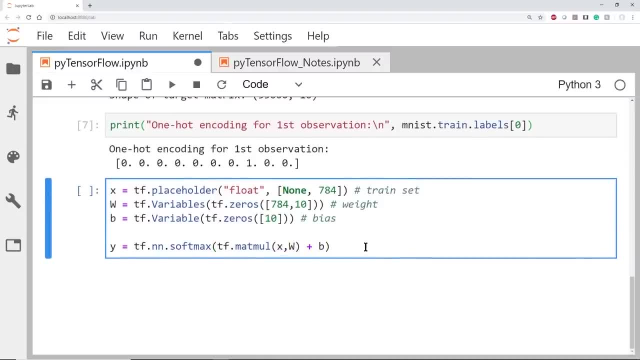 plus b, and this is our sum. let's just put a note here so we can keep track of what's going on. we're finding weighted sum of inputs plus the bias. uh, so there's our plus b, the bias, and then we need to go ahead, keep them. let's do y underscore and again another placeholder, and this one will set. 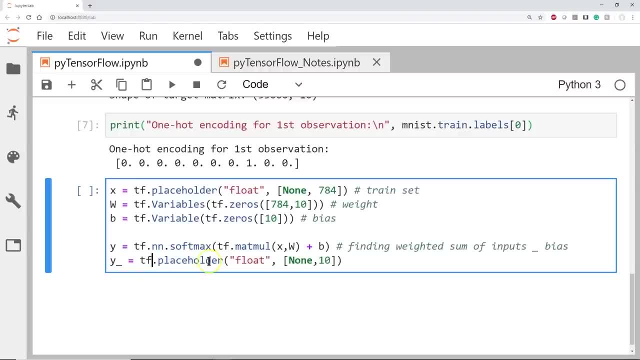 it actually will put in as tf placeholder on here. tf placeholder float none 10. there's our one hot encoder going on there. so our 10 values coming out and we'll do a cross entropy on here and this is going to be minus tf reduce sum and we'll do y. here's our. 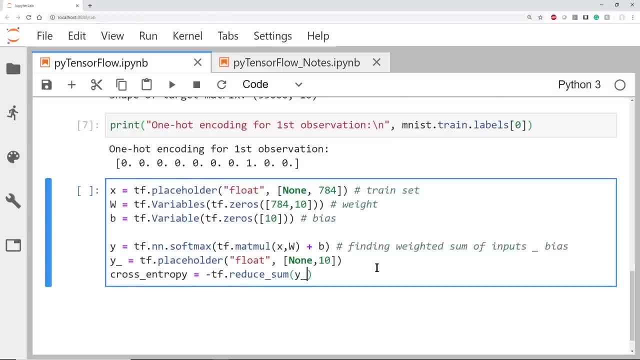 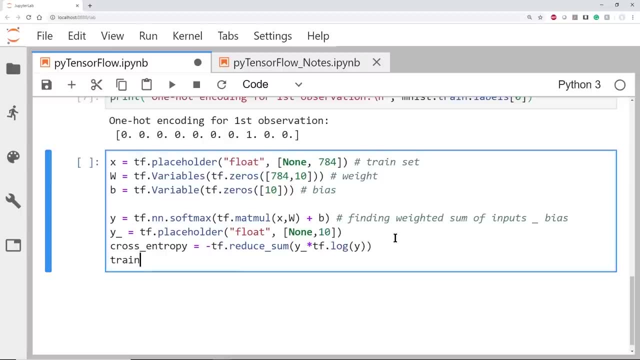 y underscore, which is, remember, we have your y output and your actual output. so this will be our y underscore times, the tf log of y and then, finally, before we do the actual initialization of all our variables, we'll set up our train step. this equals our gradient descent optimizer. very, 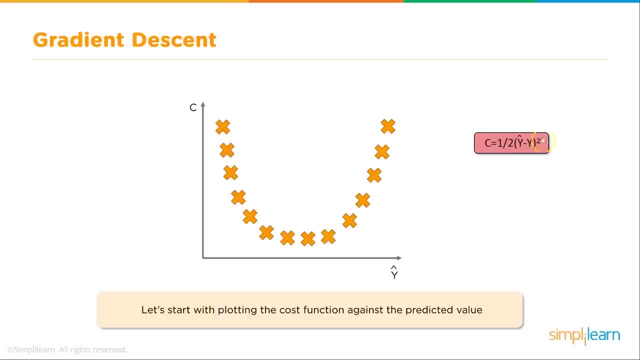 important, remember, we looked at that chart on our slides and so we've set up all these formulas and here's our gradient descent optimizer and as it keeps looking, it keeps looking for that zero value. that's what we're doing with that particular formula. so let's take a look and see what we're. 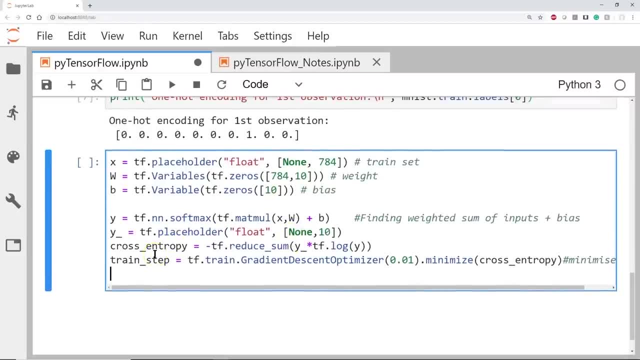 doing here? we just put together all of our pieces for tensorflow and you know the devil's in the details. we have here our training set coming in. we have to put a placeholder on there. we have our variables with their weights, we have our biases coming out and then we put in our the weighted sum. so here's uh, summizing our summation. 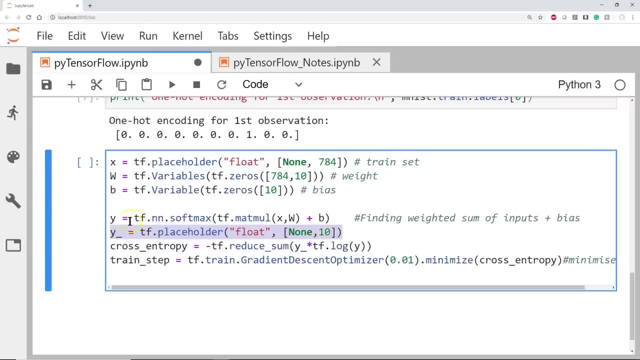 here. then we have our y variable output. so there's our y, how it works, and then of course the actual output on there, and then we have our cross entropy coming in and that's our minus tf. dot reduce sum the y times the tf log of y and then the training step gradient descent optimizer. 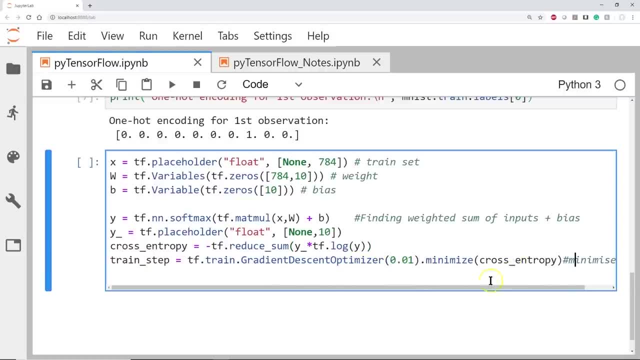 we're using a 0.01 in this and we're going to minimize cross entropy, so we're going to let it do all the work you. So, once we've set up all of these different layers we've allocated for them, we need to go ahead and initialize them. 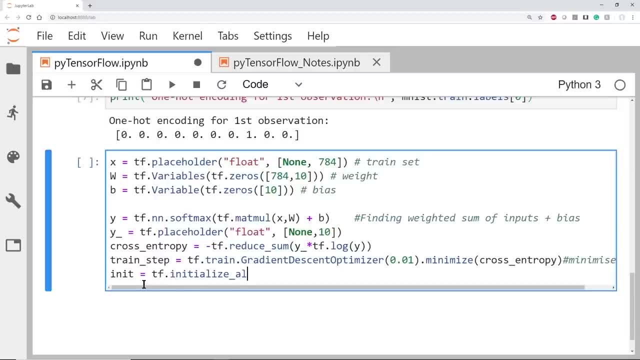 So we're gonna do an init, tf, initialize, and it's gonna be all variables. One of the cool things is they're in the process of doing away with this, So all these steps would be bundled into one instead of having to have placeholders. 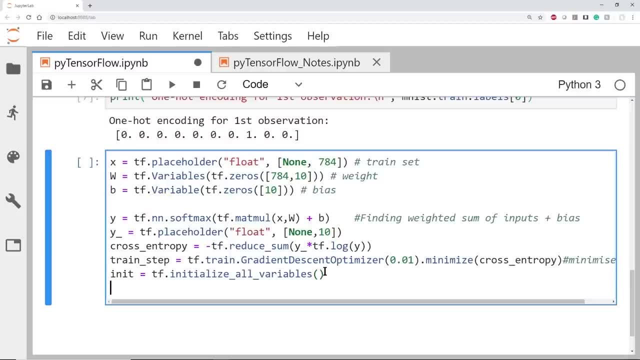 you initialize them in the same process, going on, And then finally, everything in TensorFlow is based on your session. Now this is changing that. there's other options to be able to run this, but we wanna go ahead and do a session. There's our tf, which is a tf session. 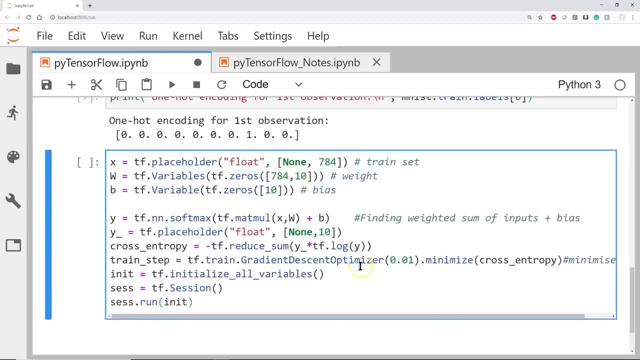 And then we wanna go ahead and do session run, And what are we gonna run? Well, we did initialization of all our variables, So this is what we're running And this is where, actually, once we do this, we actually create our TensorFlow object. 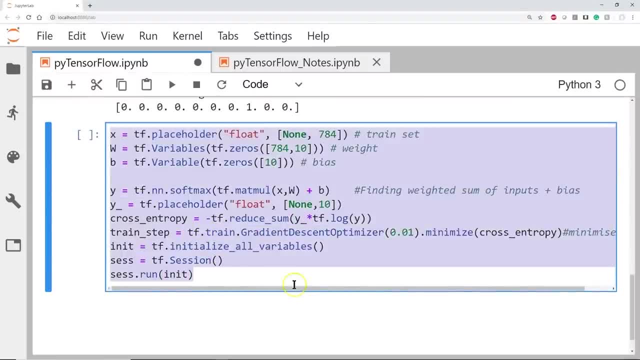 So this whole piece of code right here is our TensorFlow object. We have our input coming in with our weighted variables coming in, our softmax for our metamil going out. How does it add it together for our y value? Then we have the actual float value coming out. 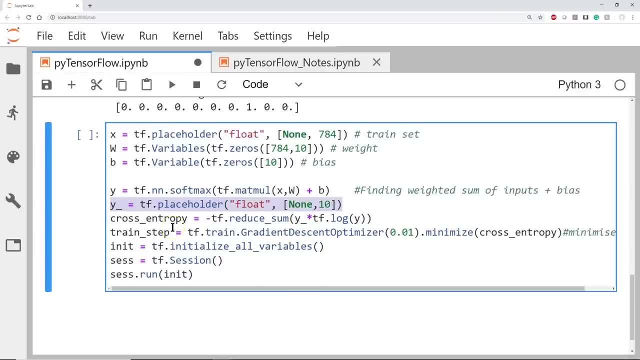 checking on our all the way down So you can see all the different stages going through that we're setting up, And this is one of the reasons that a lot of people like TensorFlow is because you can designate all these different pieces one step at a time. 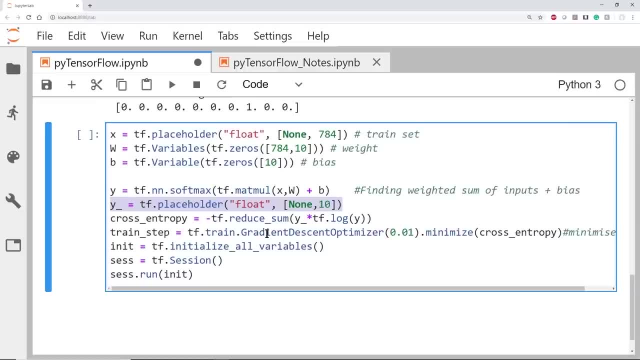 This is also one of the reasons people don't like TensorFlow is because you have to designate all the different layers coming down, And there's a lot of steps being made right now to minimize this, to make it either easier to automate, to automate it, or to allow you to do more complicated things. 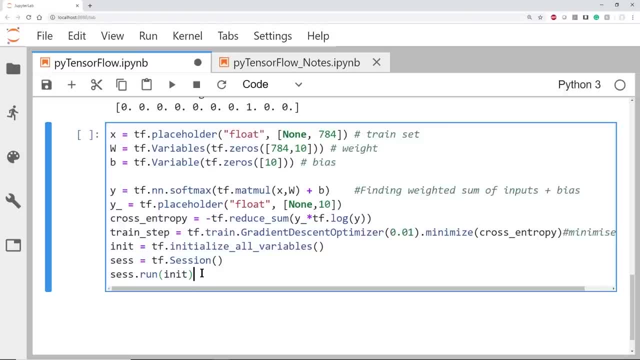 And all those steps are still at play. So it's worth looking into the more advanced version of what's going on with Keras on top of TensorFlow. It's also important to understand what's going on in these individual levels If you're going to play with them. 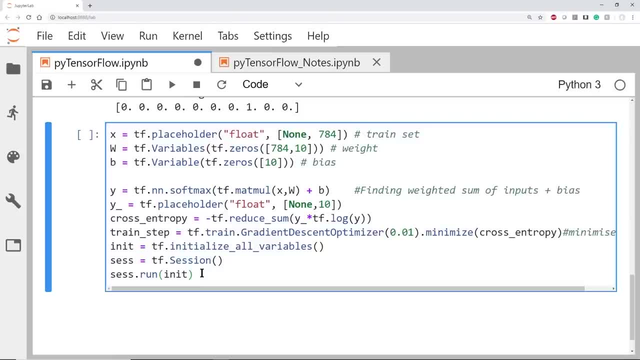 it's important to understand: Hey, what's going on with the finding the weighted sum of the inputs plus the bias Cause? there's other ways to do that. There's all kinds of other tools in there now, but this is the basic setup that you want to do. 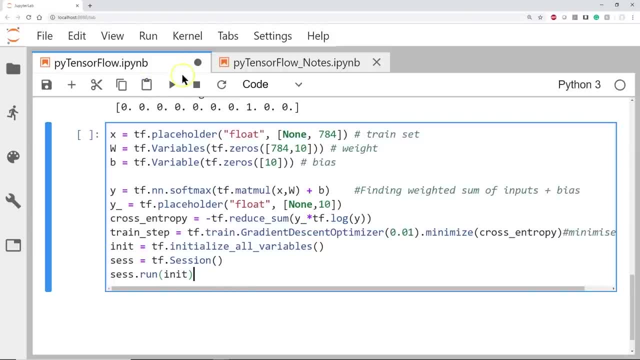 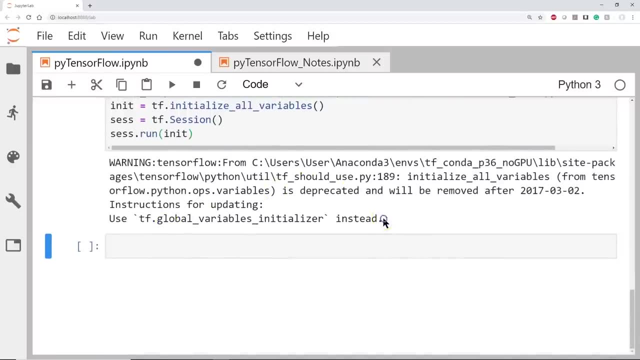 on a TensorFlow coming in And we want to go ahead and just run and admit our TensorFlow. So let's go ahead and do that. Let's run this. We do get a warning here because there's a move to use global variables. This is one of the changes they're making. 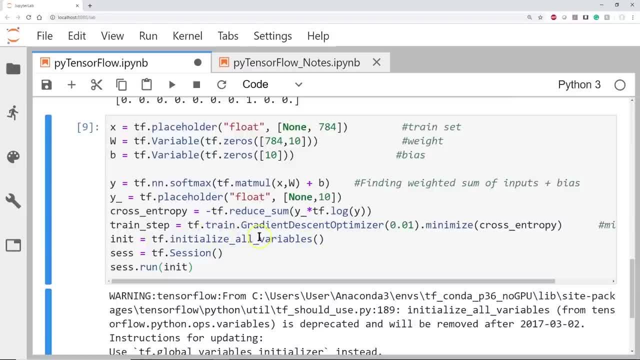 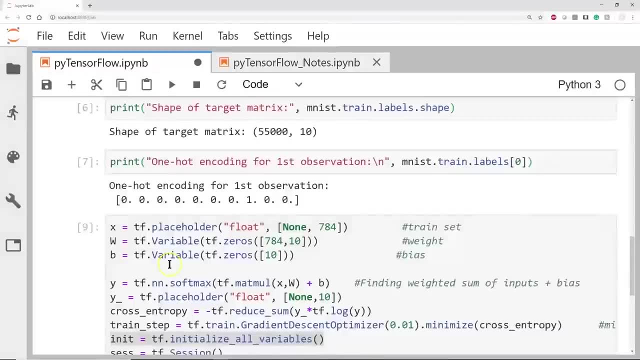 but as far as this example, it's not going to make a difference because we're doing once we initialize it. this is initializing our variables And again, these are only placeholders up here until we initialize them, And I would highly suggest put a note down there. 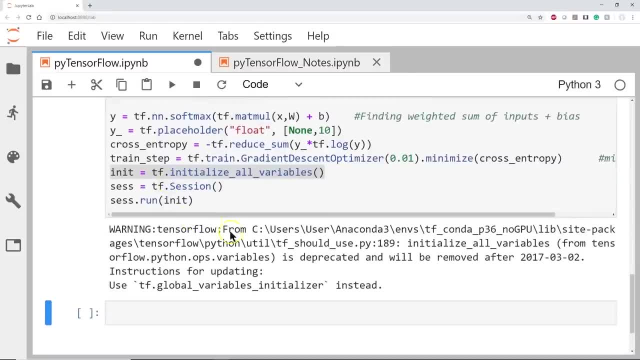 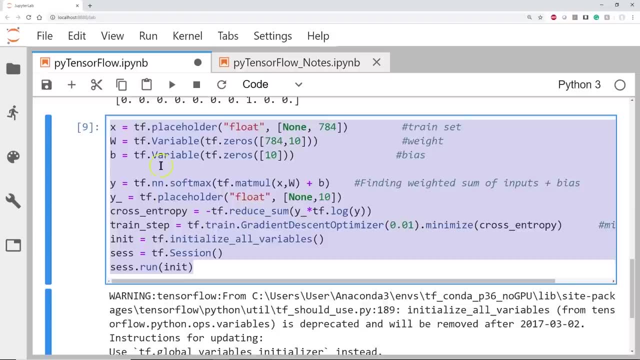 or go over to simplylearncom and let them know and have them email you a copy of the code So you can actually play with this code right here, Because this is the body of what's going on in TensorFlow. This is the build in neural networks. 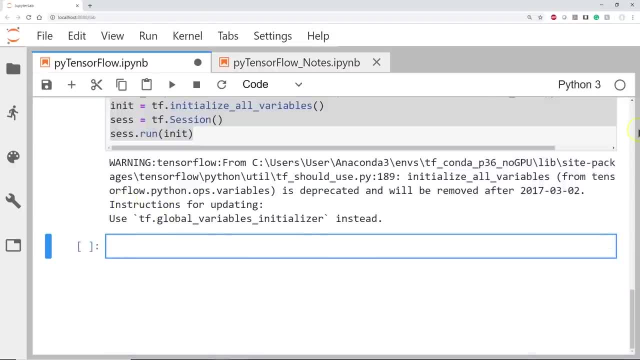 And then, once we've done that, now comes kind of the fun part is: we need to go ahead and train it. So we've created our TensorFlow, We've created our network And now we need to go ahead and train it. So let's put together that training code. 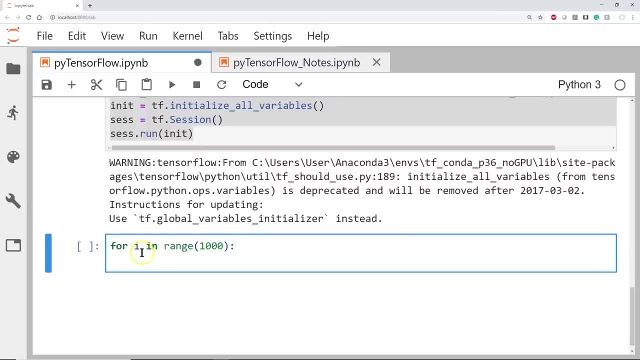 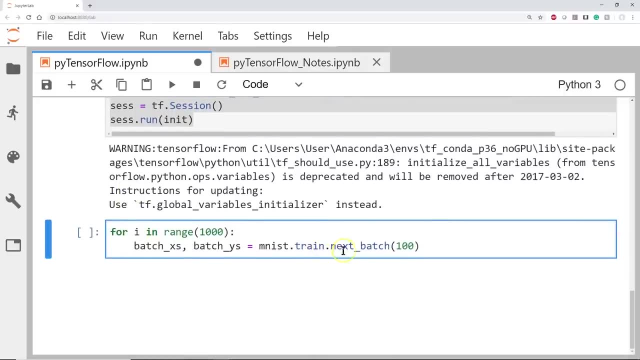 And let's just do for I in range 1,000, 0 to 1,000.. So we're just going to look at the first 1,000 in our training And the way we pull that data from our minstrain. 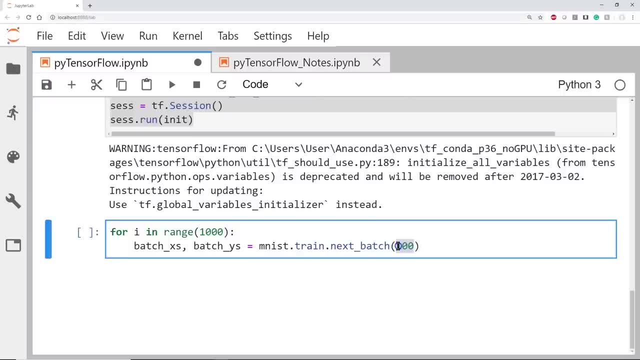 the next batch of 100, so you look at this, We're going to be doing groups of 100. And then there's going to go through 1,000 of them. This is very important that TensorFlow builds this in. This is one of the downsides of doing sklearn. 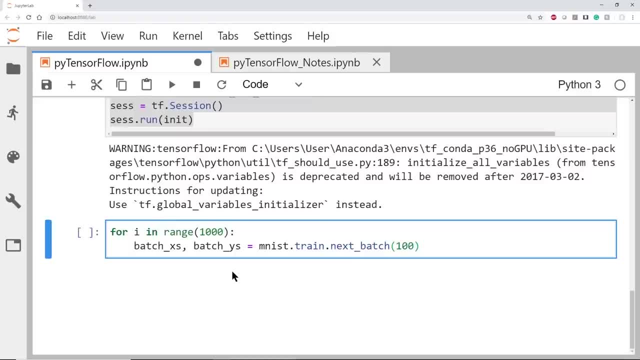 or one of the older packages, is they don't let you batch groups in. They wanted to have it all up front. And then you have to build your own batch programs. right now, This lets us go ahead and do that, And you can see, here we have batch x of s, batch y of s. 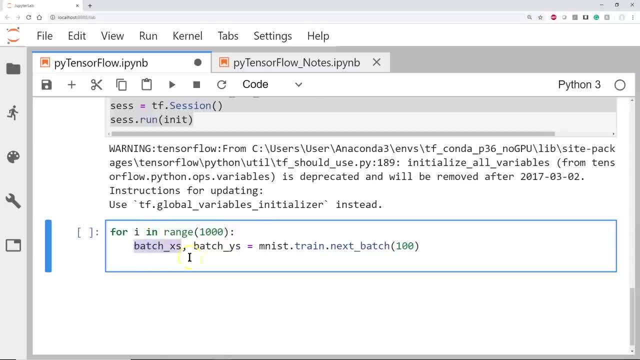 So there's our x and our y. You can look at this: There's our training of x and our training of y, or the data in and the answer in, And then we simply do our session run. So here's our session that we've created. 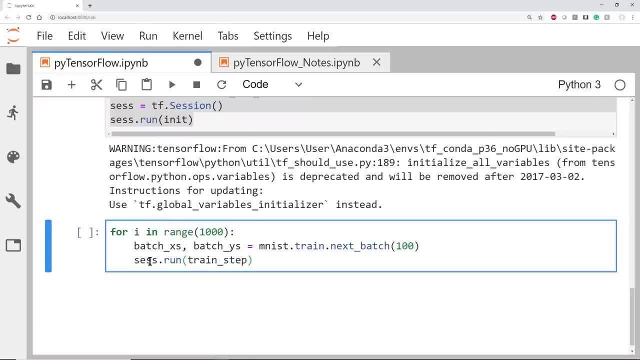 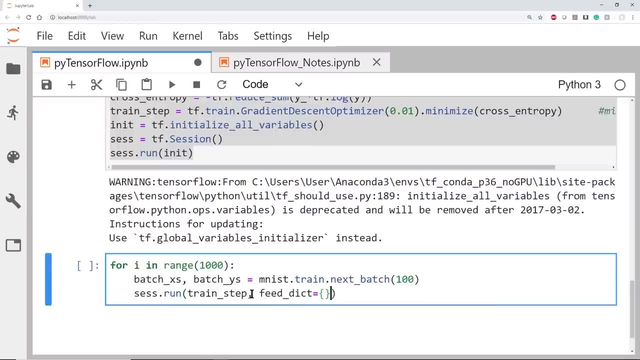 We're going to run it And we want to do the train step. Remember, we initialized our train step up here in our tf, And so there's our train step feed. It's a dictionary Dictionary coming in which we're going to create right. here is x is our batch x of our sample. 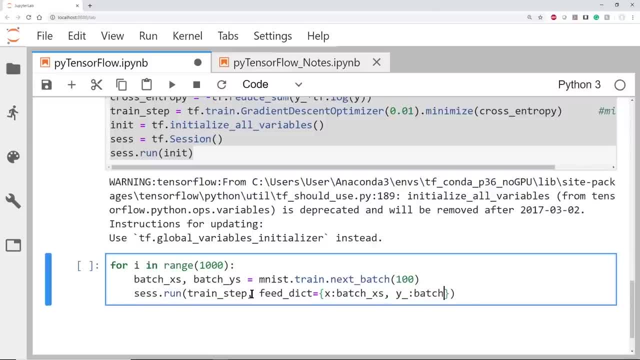 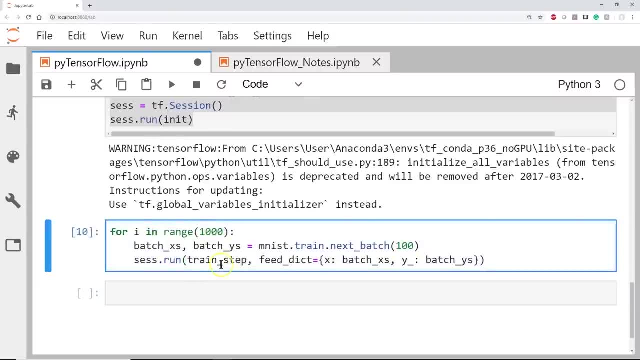 comma and our y underscore is going to be our batch of our y sample, And so this goes through And we've now hit the Run button And we've trained our session. We've trained this setup on here, And once we've trained it, then we 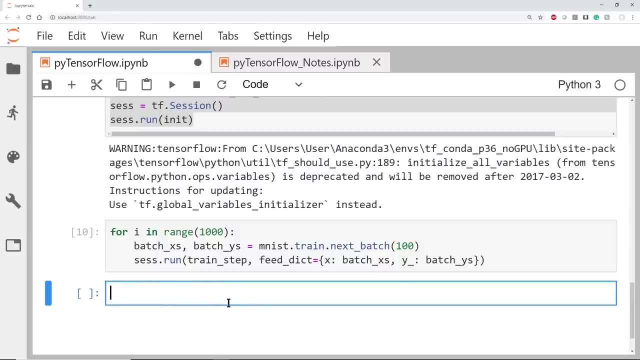 need to go ahead and find out how good our accuracy was and actually start running some predictions through there. So we'll go ahead and create a correct prediction And this is where our tfequal we'll use our argmax y of 1 and tfargmax of y of underscore. 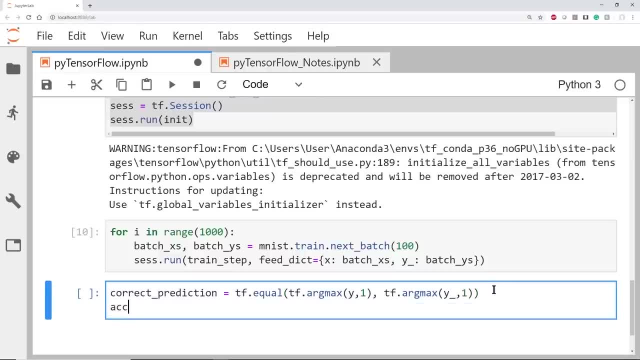 of 1 to help us get the correct predictions on there, And then we want to use that to feed into to an accuracy, And so our accuracy is going to be tfreducemean And we'll take that and we'll do a cast. 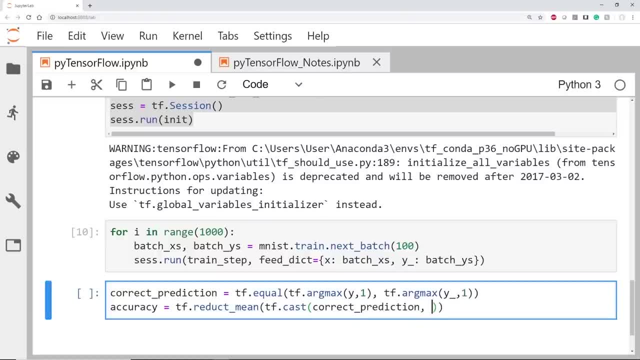 This is the correct prediction that we're sending in there, And it is a float value. Keep it simple And let's go ahead and print this out so we can see what we're looking at. So what are we printing out? We need to do a session run. 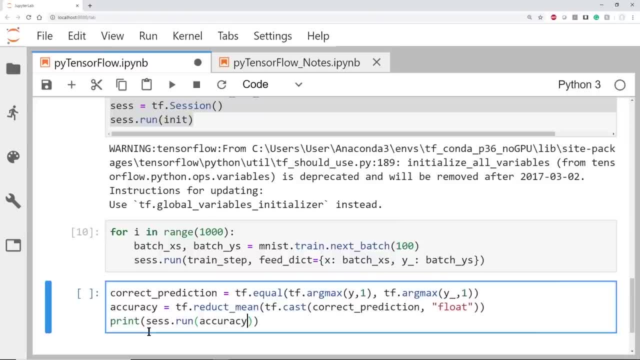 This session run is going to be on the accuracy. Where did accuracy comes from? This is our. we're casting our tf on there with the correct predictions on that. So here's our accuracy Feed in. so it needs a dictionary for the data coming in. 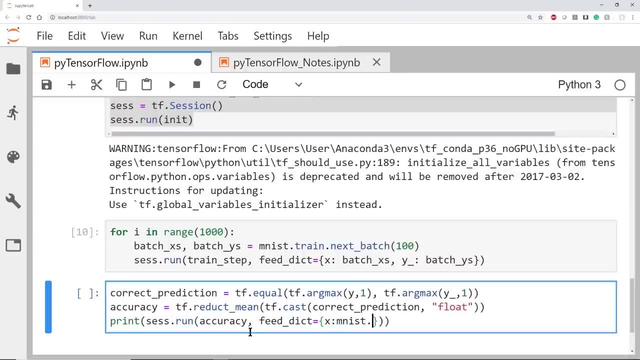 We're going to create our dictionary, And x is going to be our NIST test images And y underscore there is going to be our NISTtestlabels. Let me just double check and make sure I have that typed in there correctly. There we go. 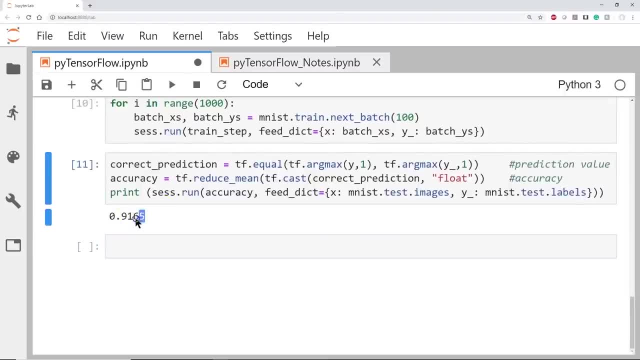 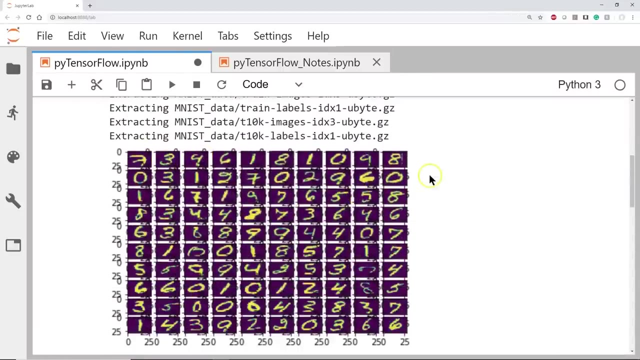 And let's go ahead and run that and see what comes up, And we end up with a 0.9165 for our accuracy, which means our trained neural network does a pretty good job letting us know what these different symbols are And guessing that a 7 and a 3 and a 4, something that, as humans, 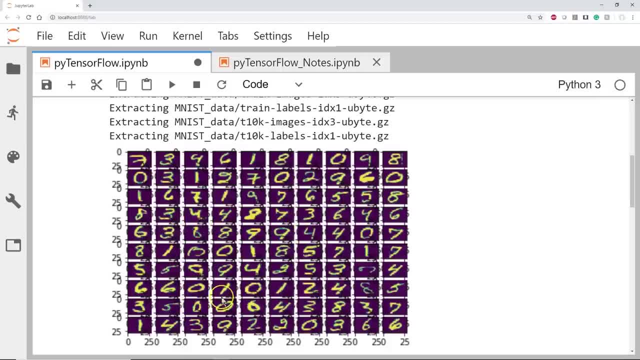 we kind of take for granted. I even have trouble reading this, So I don't know if I would be able like that first one. I would sit there for a long time figuring out that's a 7 versus a 2. That could have easily been a 2 to me. 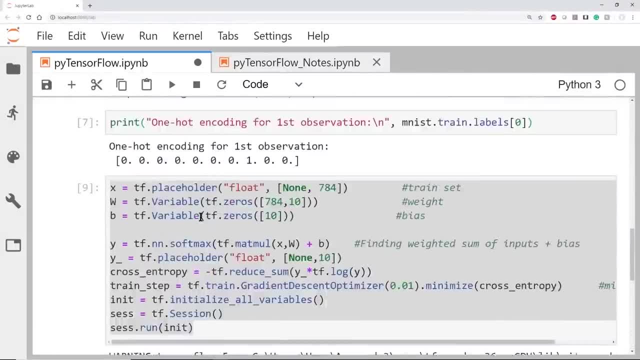 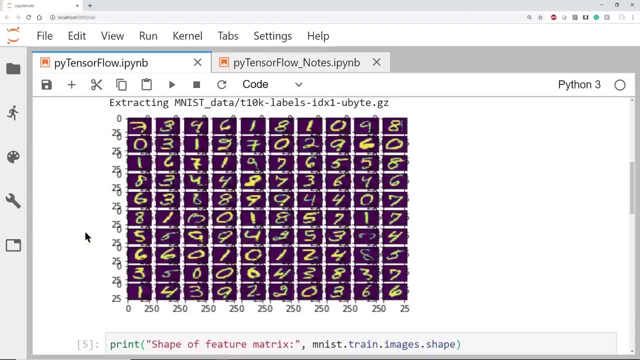 So you can see, we do a pretty good job analyzing this data, And this is used to analyze something very complicated on these images, Very different than just a straight value of cost of cells. And here's our return and our marketing. We can now create this nice neural network that 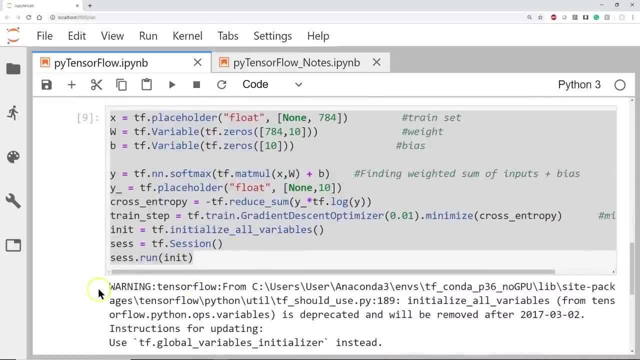 does all kinds of cool things. Now we've covered a number of really cool things here in our SimplyAlert. Hopefully you've had a chance to explore. You'll have a chance to get in there and dig into TensorFlow and all the upcoming cool things connected to TensorFlow. 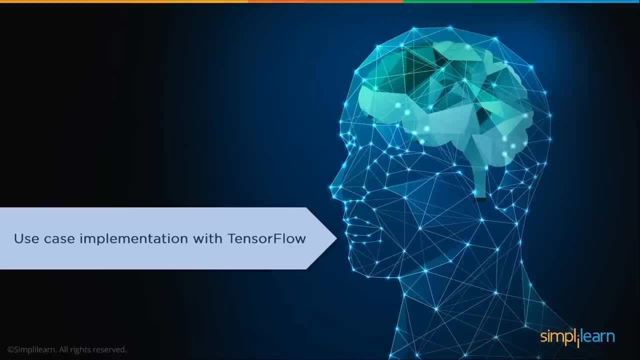 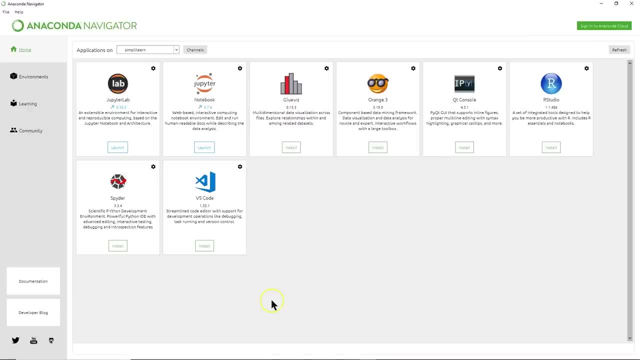 What we'll do is we'll go ahead and dig into use case implementation with TensorFlow To do that I'm actually going to go into. in this case I'll be using the Anaconda Navigator And you can use either JupyterLabs. 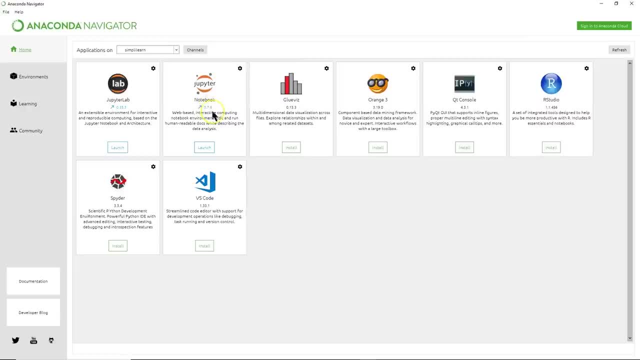 or Jupyter Notebook. Most people are very familiar with Jupyter Notebook. It's very commonly web-based. The JupyterLab is the next version of Jupyter Notebook And it just lets you have multiple tabs open when you're working on it. 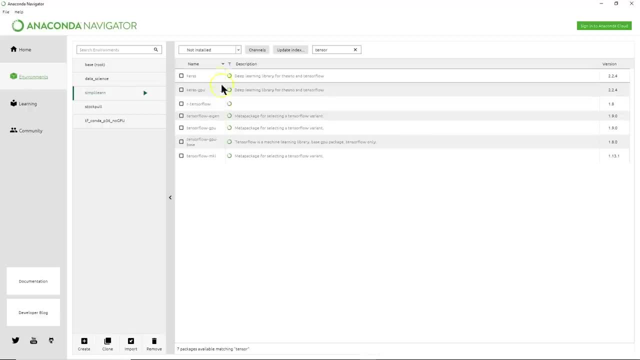 And if you're using Anaconda, you'll go under environments And you'll want to make sure that you have your TensorFlow installed, And you can simply. we'll do this. I have it installed, But you could do all. We'll do all. 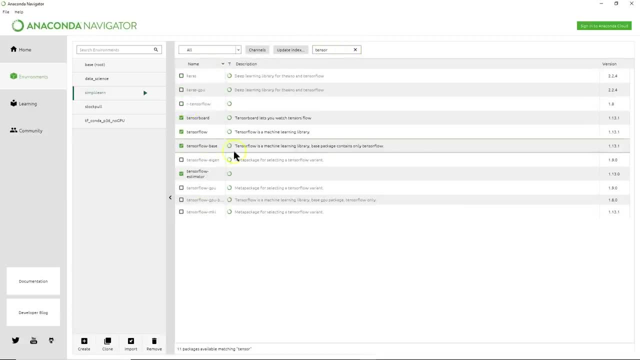 You can do a search under all for TensorFlow And you can see all the different tensors. It's actually installed. We installed in here version 1.1.3.1.. If it wasn't, you could check the box and then run the install on there. 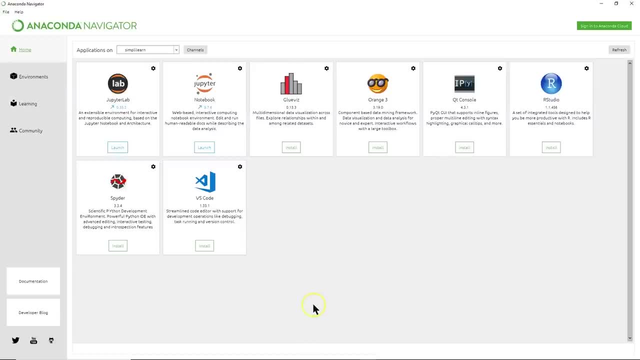 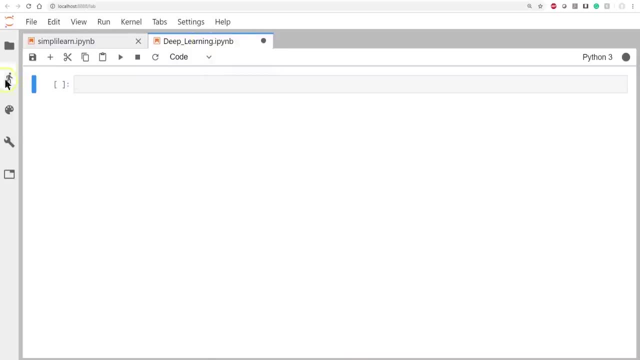 And it'd bring it right in. But we'll go and start up our JupyterLab, which is going to open up. in this case, I use Google Chrome And in our JupyterLab or Jupyter Notebook, if you're in the notebook, you only have one tab. 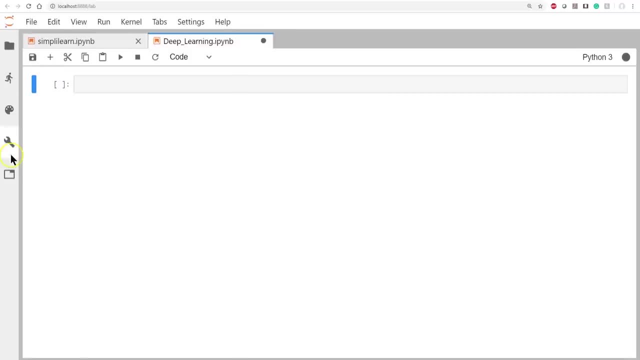 And you won't have the added options, like there's a folder and different things you can do in the lab that you can't do in the notebook, But everything we're going to do you can easily do in the notebook And you'll start up a new project. 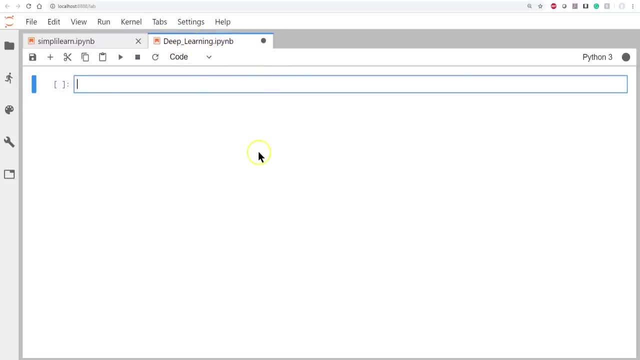 Deep learning is what I'm going to call this And if you're not familiar, you can definitely. we have some tutorials out on the use of Jupyter Notebook and how to run it and set it up and things like that. The most basic is, we put our code in here. 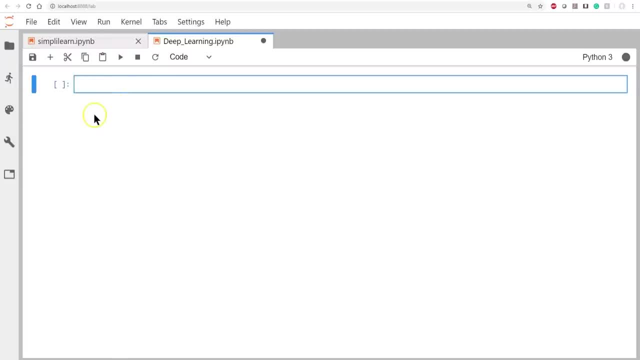 It has a nice display, a nice interface, especially for data science. I can display all kinds of things on this page And then you can just run this page right here. There's no code in it, so it's not going to show any thing until I put some code in there. 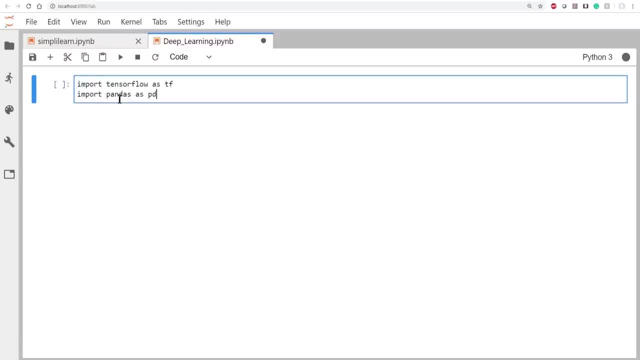 And, of course, you can cut your cells and things like that. So the first thing we want to do is we want to import our tools. Now, if you haven't remember, you've got to. You've got to install TensorFlow. 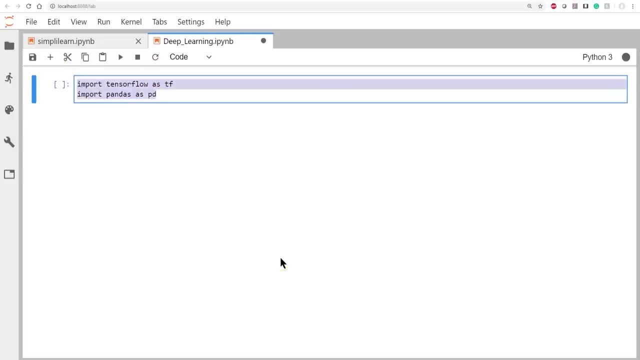 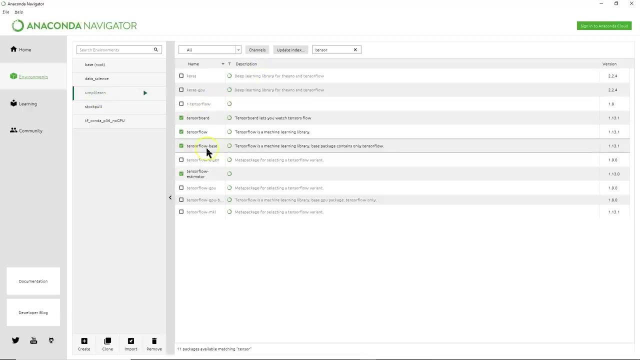 And we'll also use Pandas. Pandas is a nice database setup And that again is underneath your environment And you can see here. whatever you're working on, I simply learned setup where I've installed TensorFlow and Pandas in here. 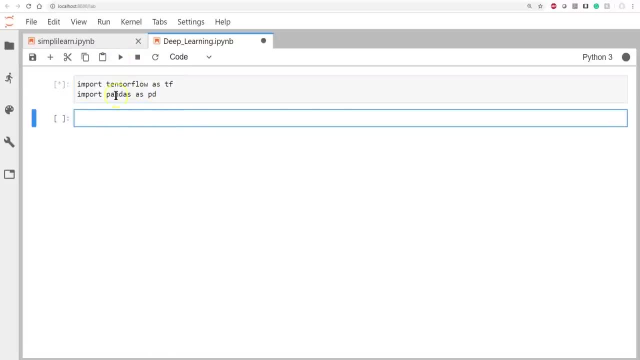 And I'll simply go up here and run this. I'm not going to see anything. so we've just imported those into our notebook that we're working on. So those are now available to us, And it helps to have some data to work with. 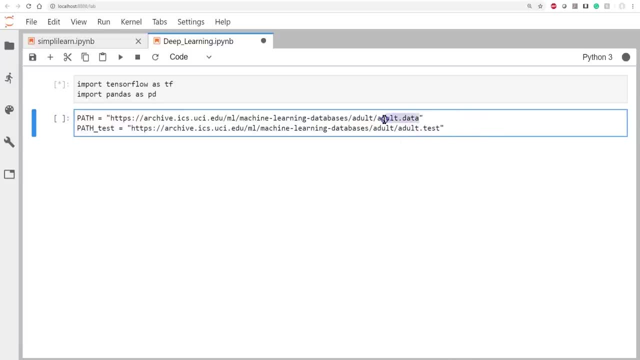 And we have here. I'm going to create a path and a test path And we'll go ahead and let's just just highlight this whole path And you can always post a note, either down below in the YouTube video or you can post a note on simplylearncom. 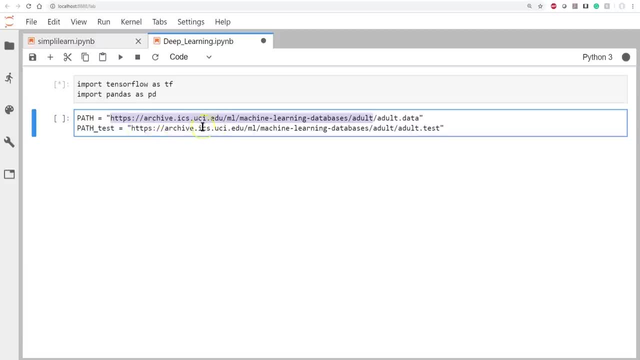 and ask for this path if you're not quite picking it up, But it is over here at the UCI EDU on their setup And it's in their archive, So it's archiveicsuciedu forward. slash ML for machine learning. slash machine. 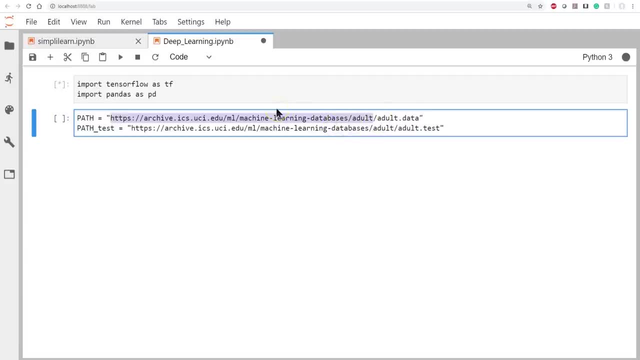 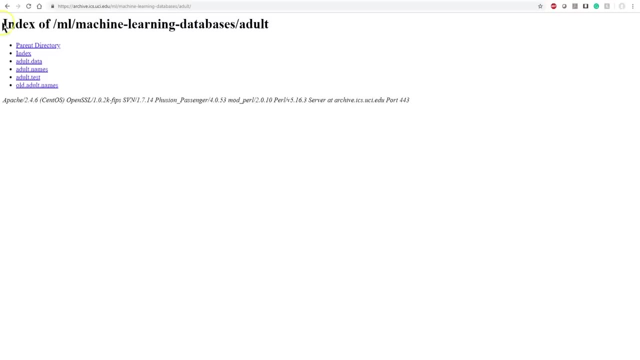 dash learning, dash databases, slash adult. That's quite a mouthful, And in this case we have adult data and adult test. But let's go ahead and just take a look at that. Let me just paste that right in there to our browser window. 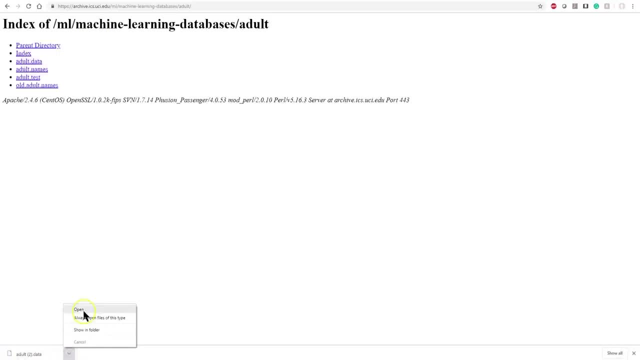 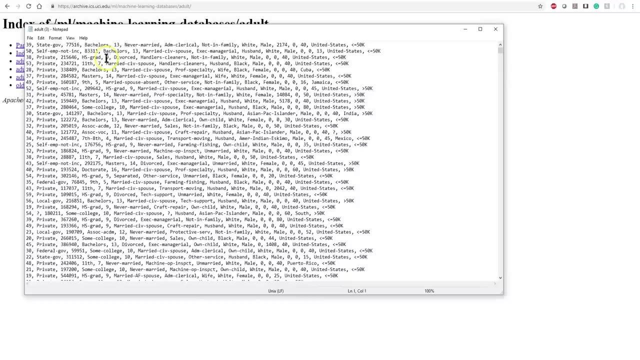 And here's our adult data And if I click on there it's going to come down as a download. I'm going to go ahead and open it as a text in my notepad, And the guys in the back were kind enough to look up to find out what the actual columns were. 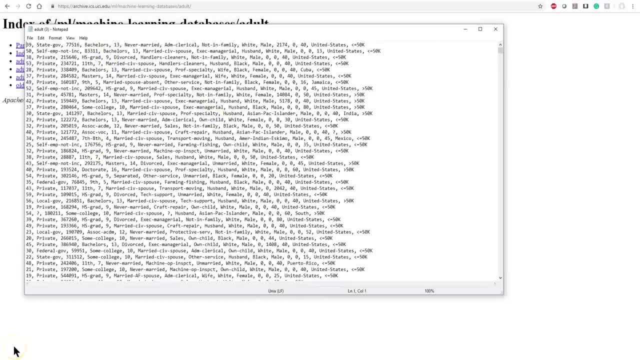 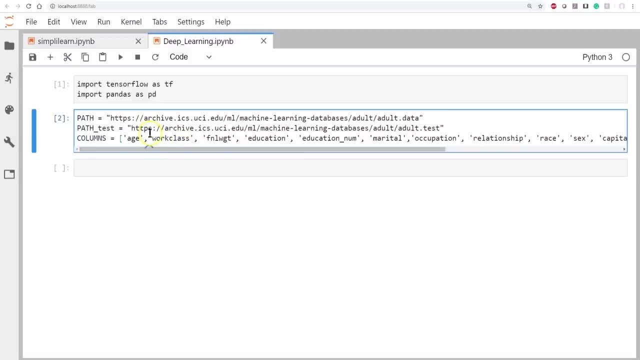 in this coming across. So let me go ahead and take that to pull that information. It doesn't matter whether I put it before or below, because these are just variables, But we can see here that we have age, work class, final WGT. 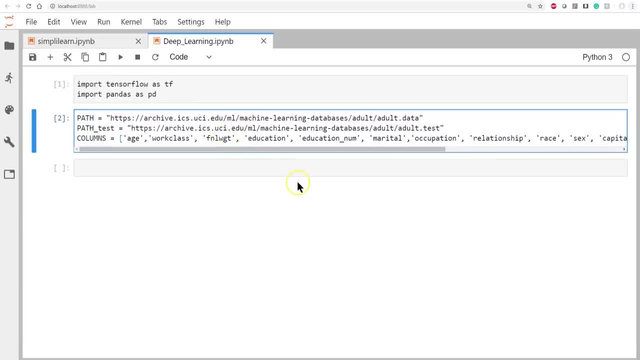 I'm guessing that's final. We'll look that up in just a second to see what that matches In fact. let's pull that up and just put them next to each other so we can kind of see what we got here. So we have age. 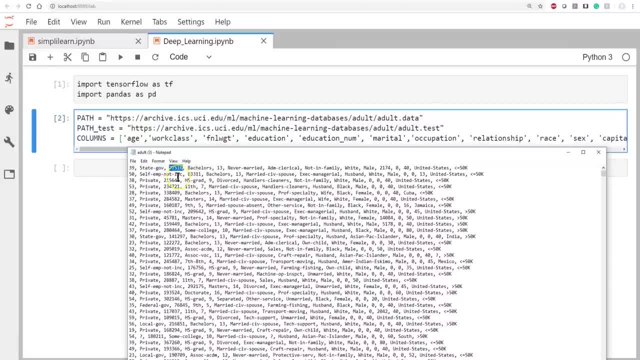 We have our working class state gov. Maybe final wage $77,516.. Education of bachelors: education number 13,. marital, never married admin, clerical relationship not in family, so on and so on. 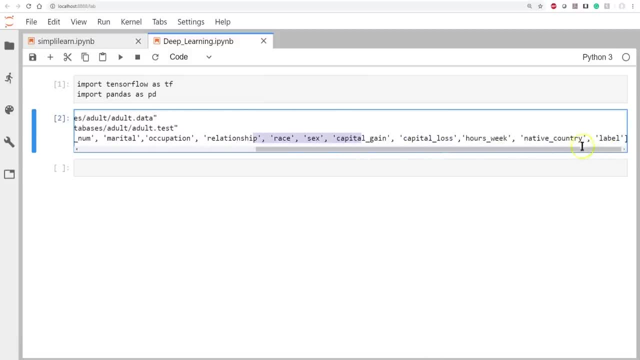 So it goes all the way across here, And so we've pulled out this information: Native country label, et cetera. We'll go ahead and run this, And so now we've loaded all our different paths And this path. by the way, this is the same columns on here. 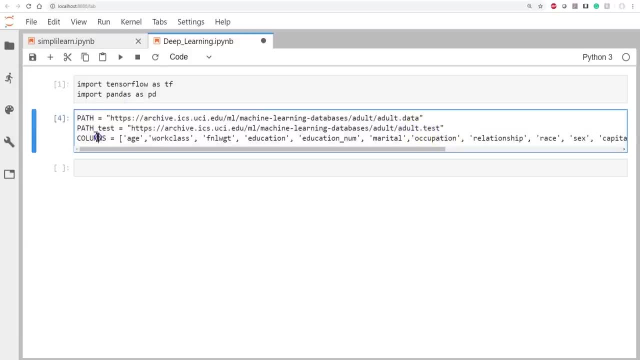 So I don't need to create a separate columns on the adult test. And once we've run this, we've set those variables, Let's go ahead and pull that data in, And to do that we'll use pandas And we'll create a dftrain, a dftest. 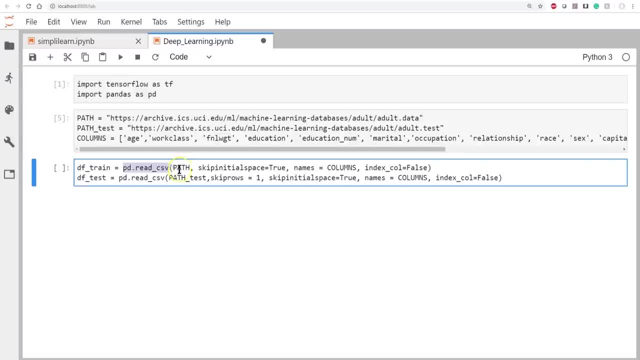 Each one's going to have our pdforpandasreadcsv. It'll have our path. we put in there our path test The first one. we'll go ahead and skip initial space. true names columns: There's our columns in there. 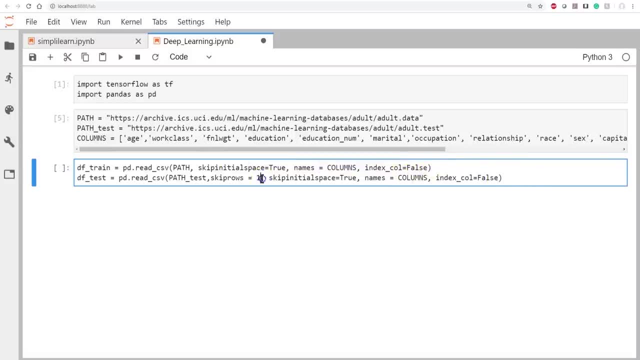 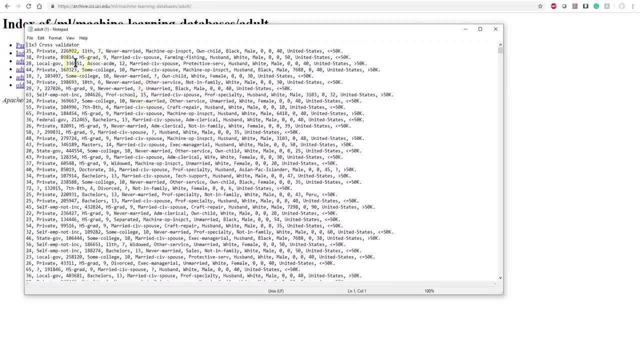 Index column equals false. There's no index column On the second one. if we went back into here and we open up adult test, let me just go ahead and open that up pad. You'll see there's an actual row up here. we want to skip. 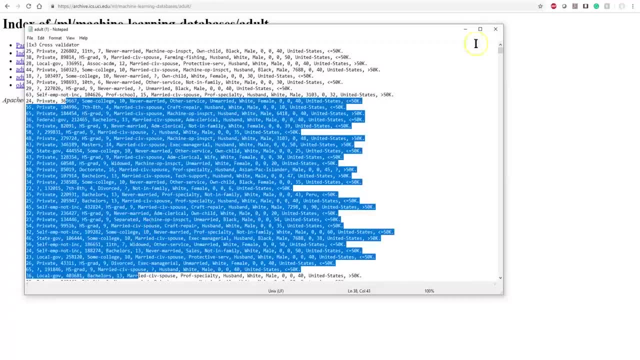 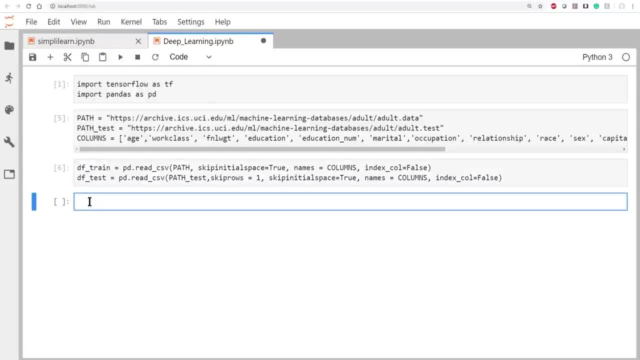 1 by 3 cross validator with all the same data in it. So we're looking at the same data in there And here. we're going to go ahead and bring in our data And then, once you bring it in, it's always nice to see what kind of shape your data is in. 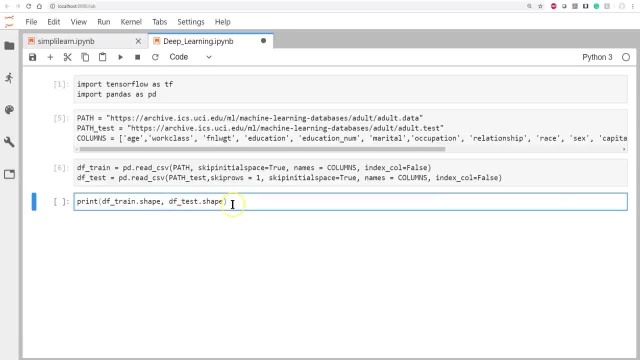 And, of course, when we talk about shape, we're talking about how many rows and columns, not whether it's been lifting weights. We can see here we have. each one has 15 columns And that goes with our columns right here. If we counted them, there's going to be 15.. 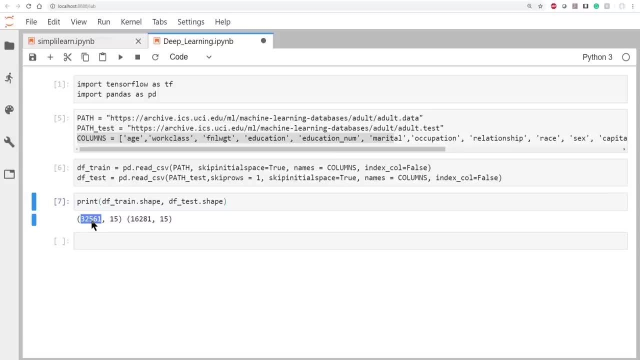 And the first data set has 32,561 rows, where the second one has 16,281 rows, And it's also good to see just how the data came in. So we'll use the pandas dtypes. We'll run that. 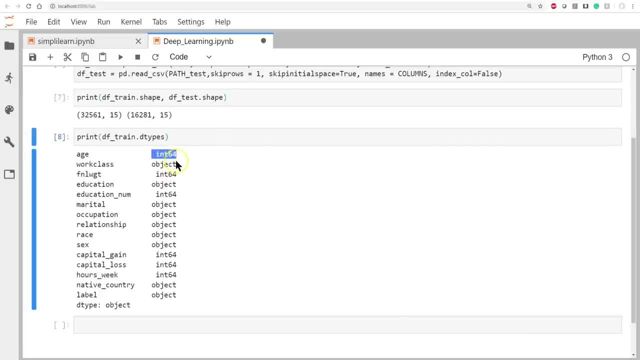 And you can see here where age came in as an integer, Integer, 64.. Working class as an object, which makes sense. And then we have our fnlwgt, the education, as objects. Or well, this is an integer, integer object. so on. 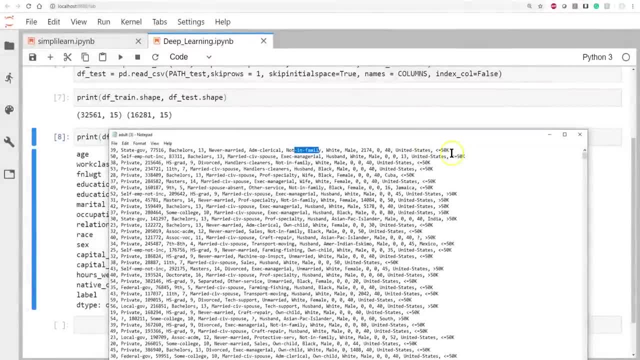 all the way down And if we flash back to the data, we look at the last column- It's less than, or equal to, 50k And if we scroll down enough we'll see it's also greater than, or equal to 50k. 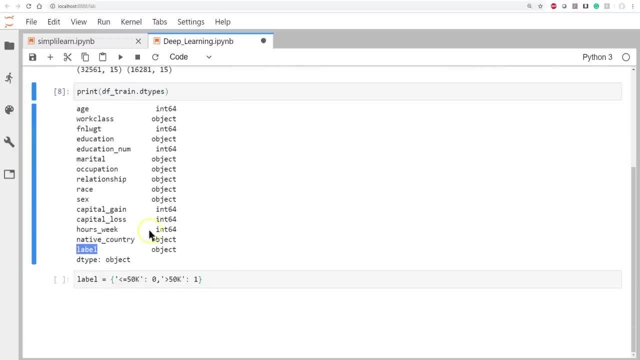 So we'd like to kind of give that its own special setup on that label. So on that feature, we're going to set the label equal to. if it's less than or equal to 50k, it's going to be 0.. 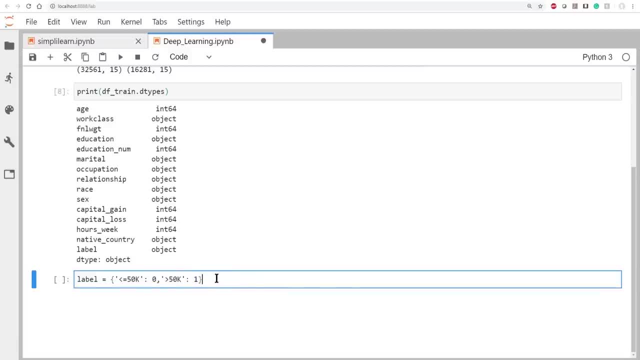 And if it's greater than or equal to 50k, it's going to be 1.. So it's one or the other. That's always an easy thing to read. And then we can take this and we can go: dftrainlabel equals. 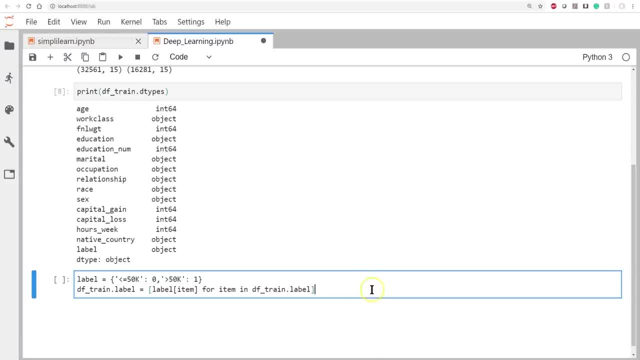 label item for item in dftrainlabel, And this just loops through all the labels. There's a lot of ways we can do this. Pandas, this might be actually kind of a slower way. There's a way to do just that setup. 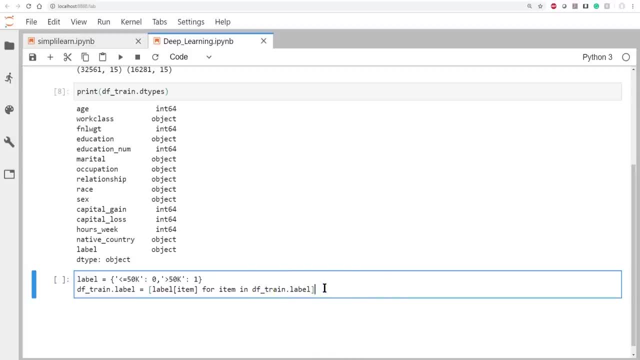 and do the logic within the setup instead of doing a loop, But for this this thing will work fine. We're not dealing with a lot of data. It's a large data set, but it's not that big of a data set as data goes. 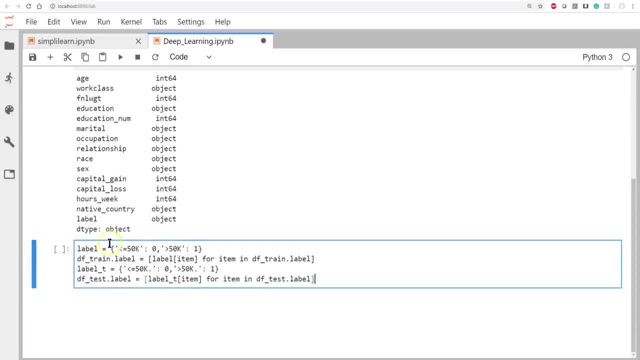 And we also want to do it for our test data. I didn't really mention that we created two data. We're looking at two different data sets: One, we're going to train the data And then we're going to take it and run the test data. 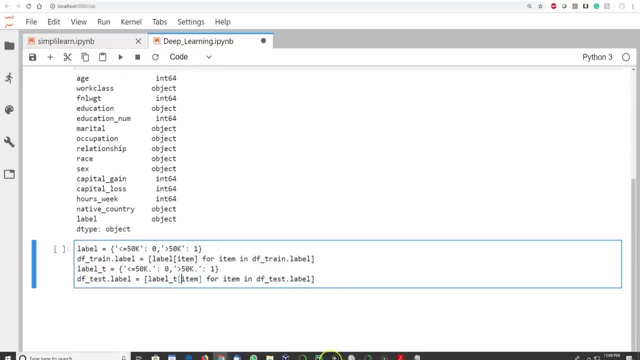 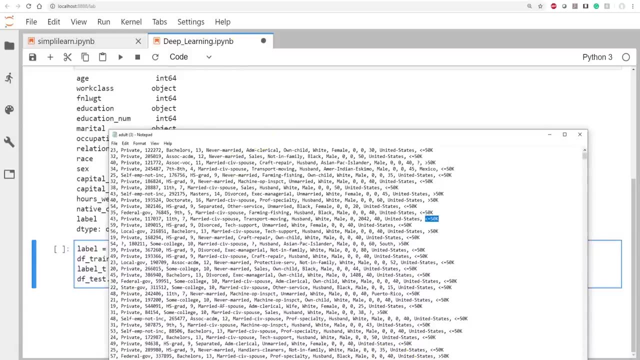 to see if it works. So we have our two different data sets And we didn't catch it off the bat. If you were pulling up this, you're going to pull up one. This is the training set, And if we go back in here and open up the test set, 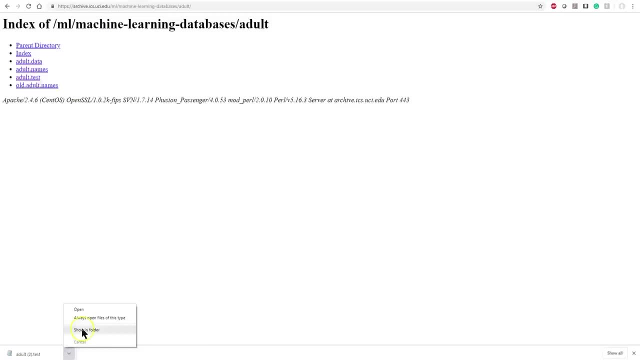 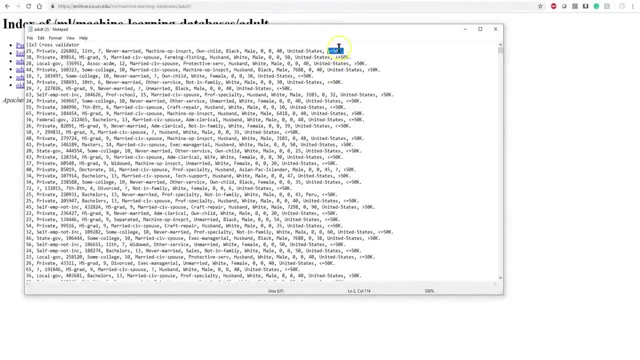 let me just go back and do that Adult test. One of the things that we didn't notice that you'll want to pull up is at the end. there's a period, So we're preprocessing our data. We want to make sure that we include. 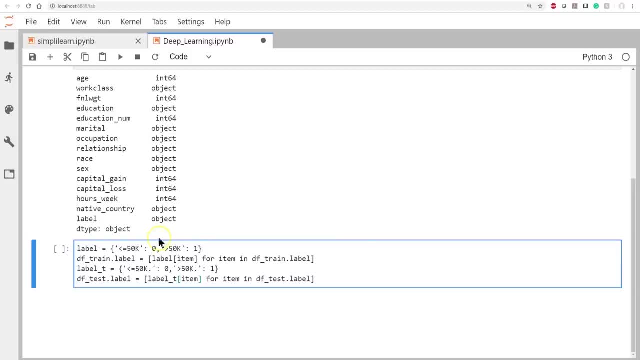 that period in every line on the second setup. So I go back to my Jupyter notebook. I've got to have a label t which is less than or equal to 50k period, or greater than or equal to 50k period for one. 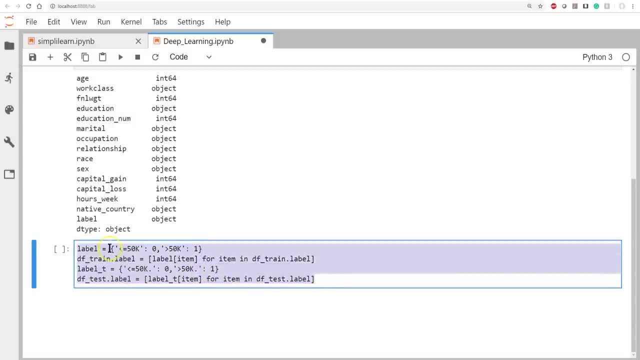 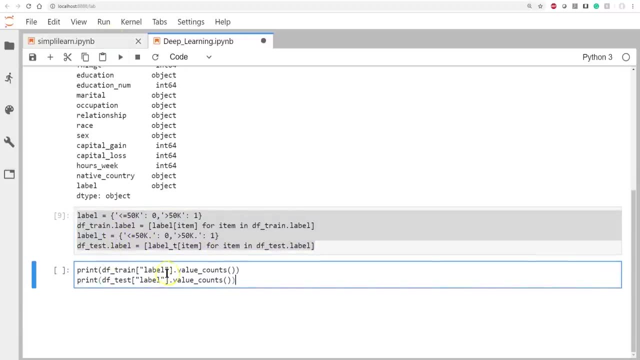 Otherwise it's doing the exact same thing. We're going to change the df train label and the df test label to 0 or 1.. We'll just run that. We'll go ahead and print The df train label- dot value counts and the df test label- value counts. 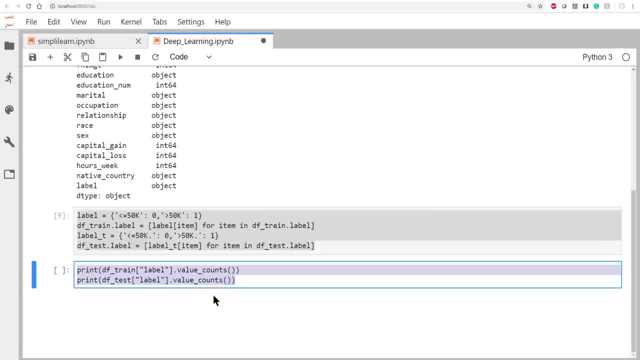 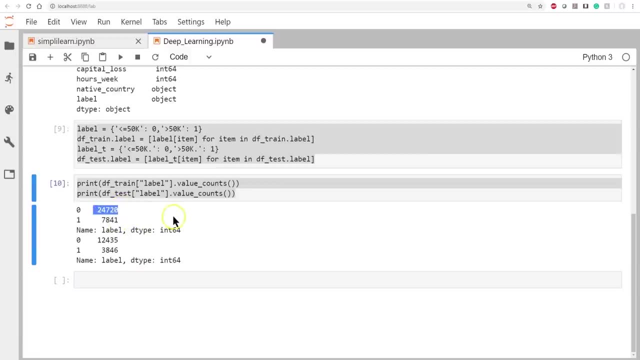 This is always a good idea because we want to know: is there any weird stuff going on there? If there's null values, stuff like that, this will turn up on that setup And we can see here we have zeros, how many zeros, how many ones. 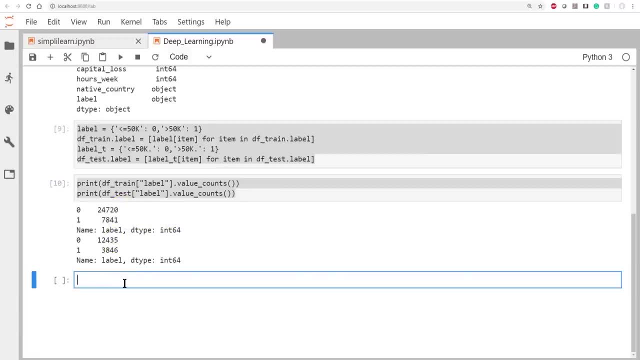 and so on on there. Just a quick view of the data that we're going through And if we go back up here, go ahead and print the train d types again And we run that. You can actually run it up there and it'll give you the new answer, because this loaded. 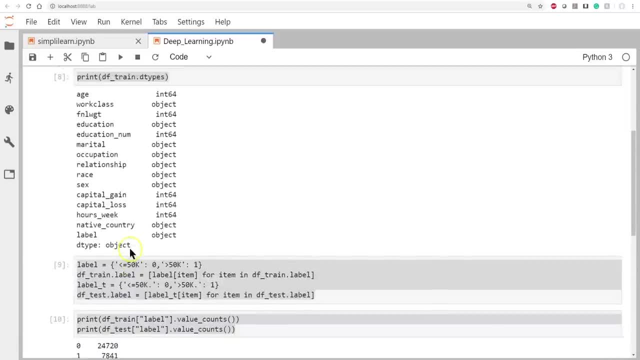 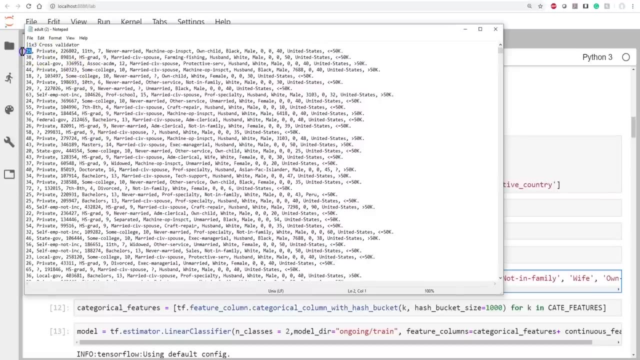 this information. We now see it's an integer And if you go back up here, it was an object, So that makes life a little easier. as far as what we're doing with this Now, at this point we're going to look at the data and we can see we have a lot of numbers. 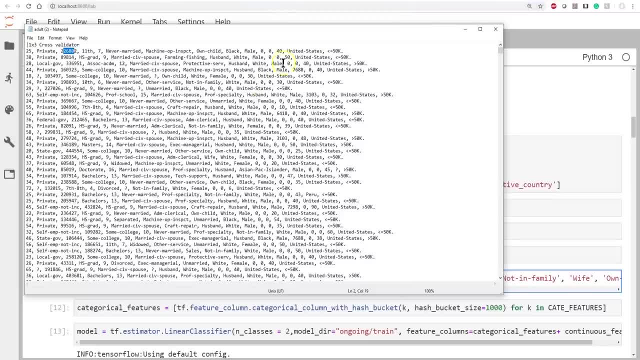 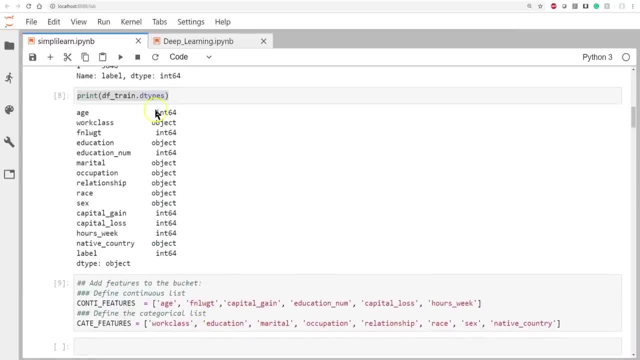 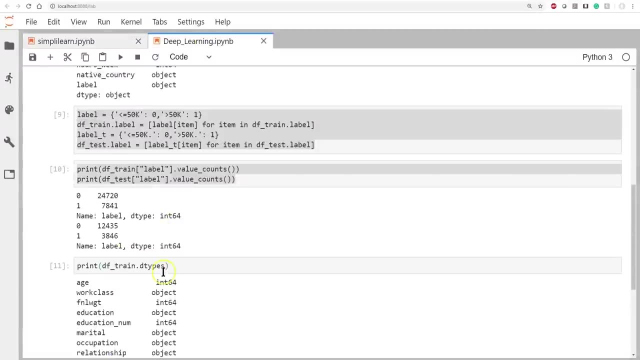 and we have a lot of categories in here. So categories would be: United States male never married versus seven, And we can also see that when we looked at this, we have our integers, we have our objects, working class- So the next thing we want to do on there is we want to go ahead and take that. 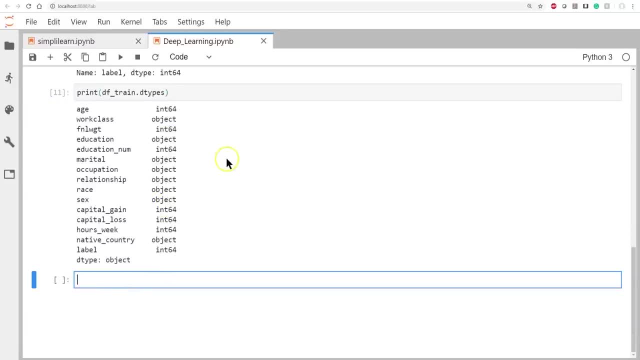 We have integers and the objects and we want to bring that down here. We want to create those categories in a way that the computer can see them And we'll start with our continuous features like age. we can see age integer. FNLWGT is: 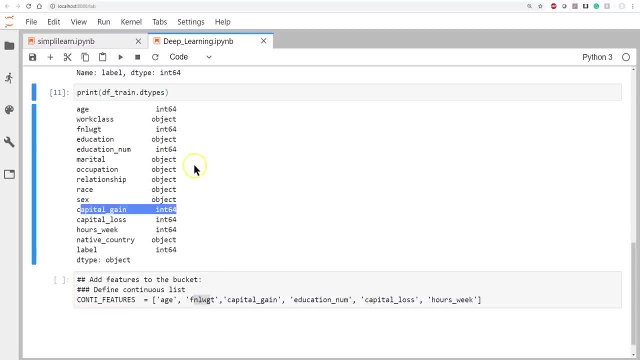 an integer. capital gain is an integer. educational number: there's our educational numbers and integer and so on. So if we're going to have these as continuous features where they're an integer, we also need to make a list of the categorical features we want to work with. 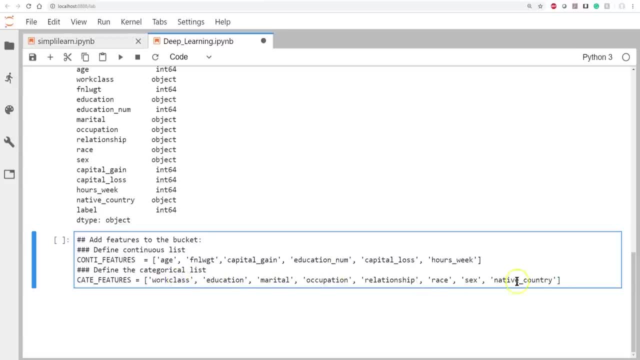 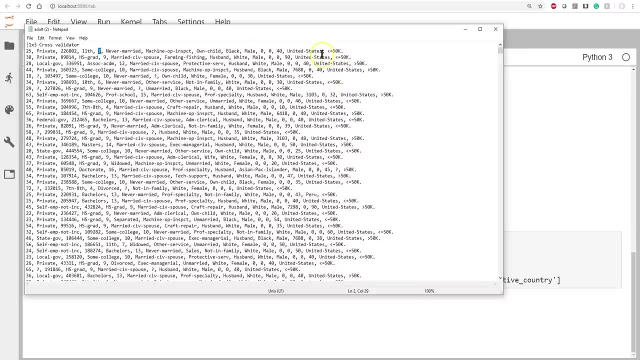 Such as working class, education, marital occupation, relationship, race, sex and native country, And again, these are all objects. So that makes sense, And when we flip back over to the data, we can see here we're actually looking at United. 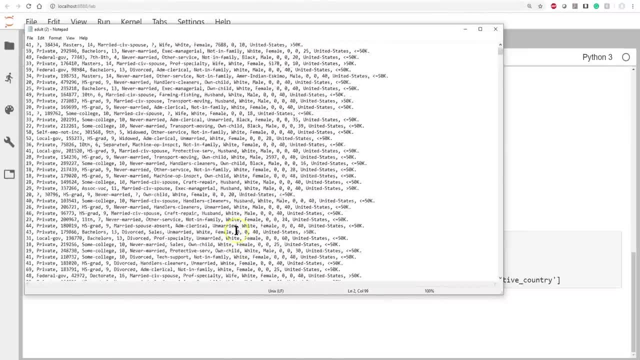 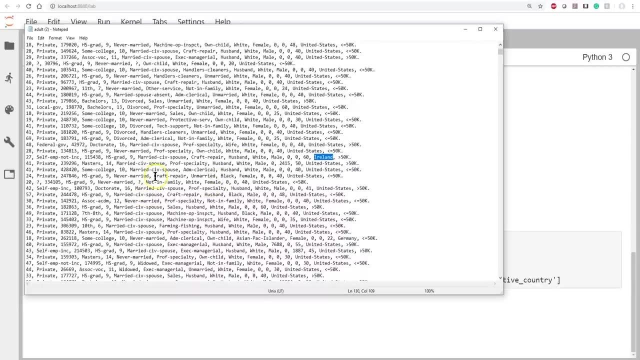 States. If we continue down, see if I can find another one. there's a lot of United States on this particular one. I was getting worried there for a second that we only had United States and it was a very biased census, which it probably is for wherever it came from. 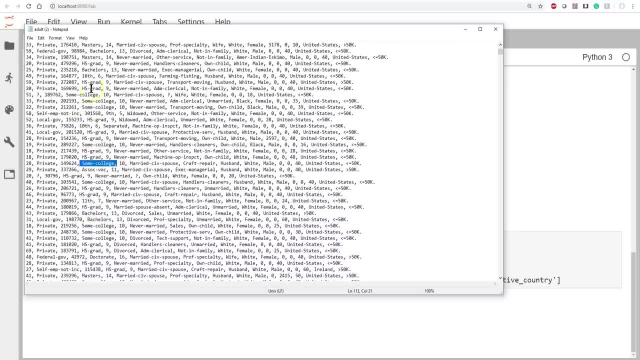 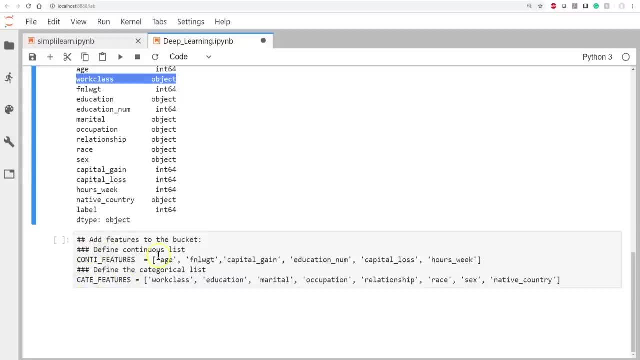 And, of course, bachelors, associate vocational, some college. so you can see this is more categorical versus an actual number. So now we have our categorical and we have our continuous features And this is just the list of these. So let's go ahead and run that and load that list in there so we can now start manipulating. 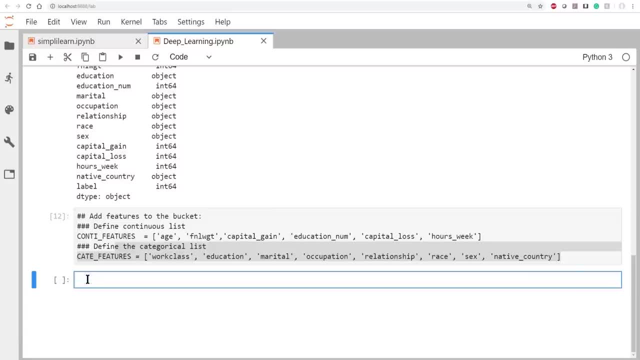 our data with it. Now we get our first line of tensor flow code, which is exciting, and we're going to create a variable continuous features. And what we're doing in here is we're going to go into tf feature columns. So we have the feature columns, we're going to set those up. 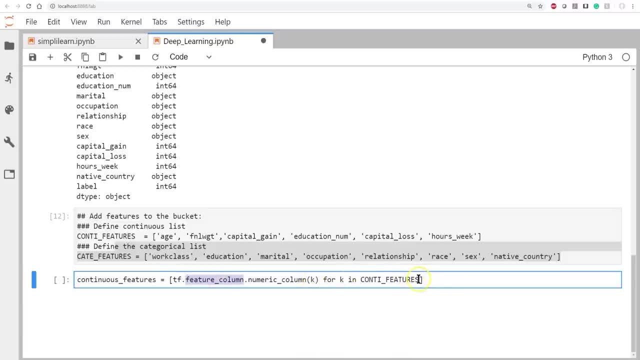 Numeric columns K, K in continual features. So this is going to go in here and says each one of these is a continual feature and we're going to feed that into the feature column. Not very exciting on the output because we're just creating this variable here, letting 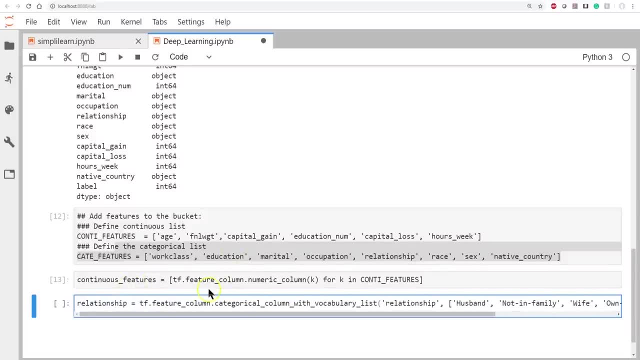 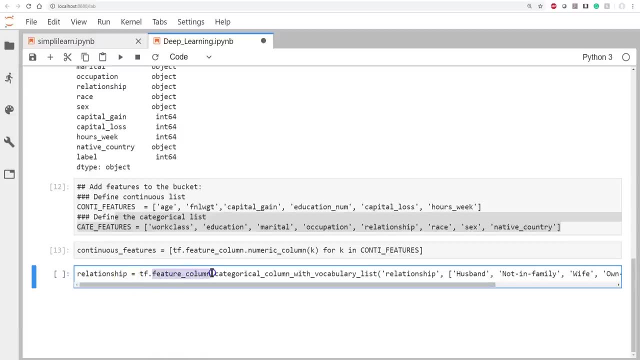 it know what columns are what, Then we're going to create a relationship setup, So we have continuous features, and then we have a relationship And again we're doing tf, but in this case we use feature column. So, just like this one, we're telling it feature column. 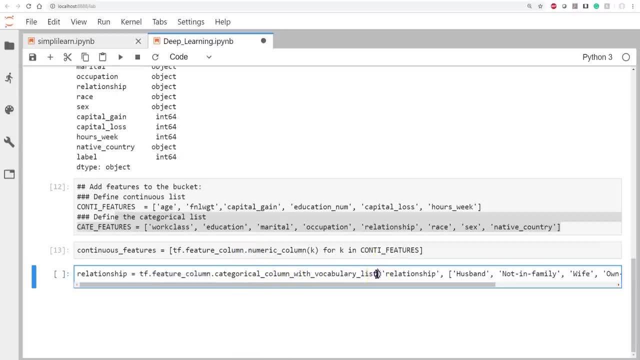 And now we do categorical column with vocabulary list. So that's one of the things we can do with tensor flow And we're going to feed it one. we have a relationship And so we're just drilling down to the relationship column And these are the options they had. 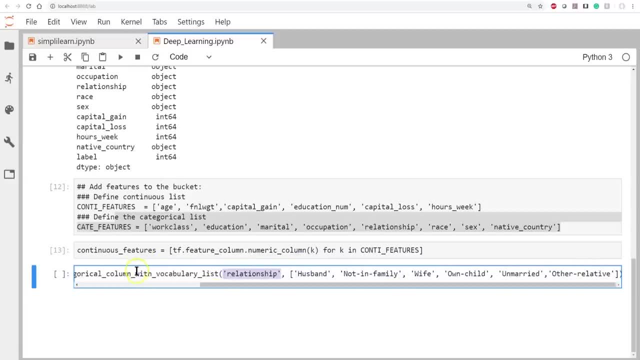 So this is going to be the vocabulary attached to this column And we'll go ahead and run that. so we load up our relationship. And then we're going to do one more way of loading. In this one we're going to do categorical features. 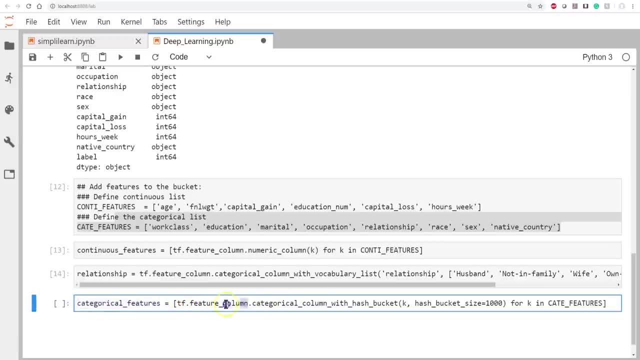 And so in categorical features, we're going to do tf feature column. There's our command, We've already seen it, We've seen it before And it's going to be categorical column with hash bucket. We're going to create buckets. 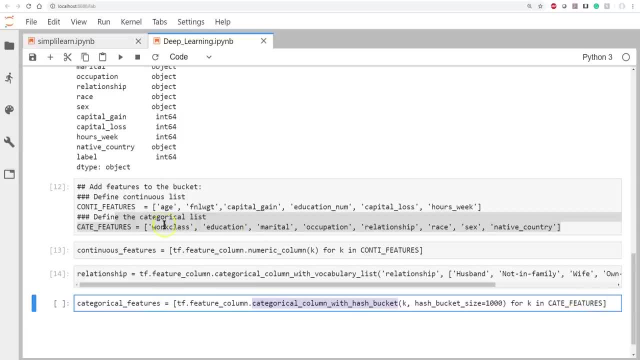 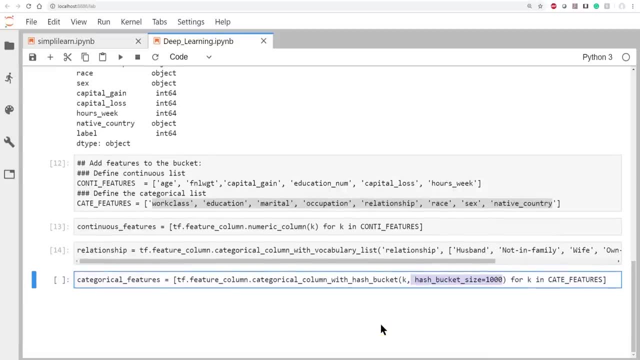 In this case for k and categorical features. So it's going to create a bucket for each one of these categorical features And the bucket size is 1,000.. So we're looking at and we've actually kind of repeated something. 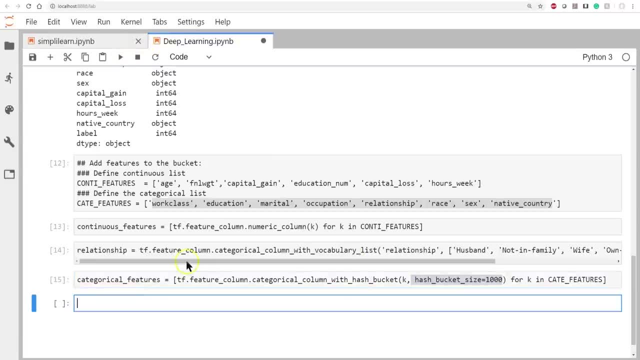 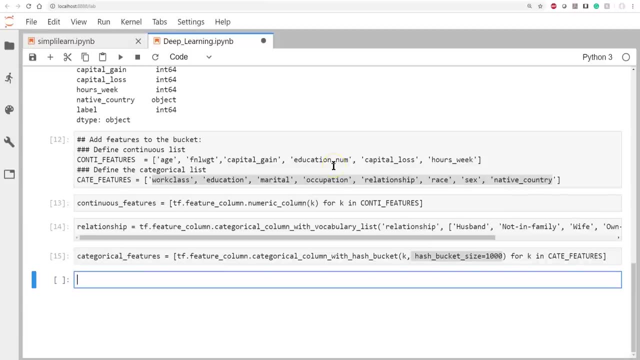 because relationship is also in the bucket setup on there. But we wanted to show you three major ways of loading in your different features. One is our features that we know where it's going to be a number, So our continuous features. then we can set it as a relationship. 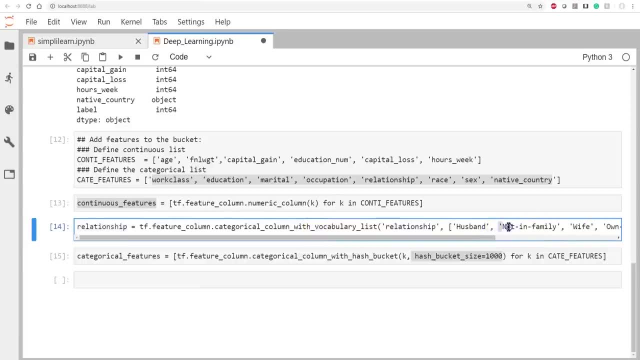 In this case we actually created a vocabulary husband not in family, very clear vocabulary on there, And then we also are loading just general categories into buckets. You can set different bucket settings in. here We went ahead and just went with 1,000. 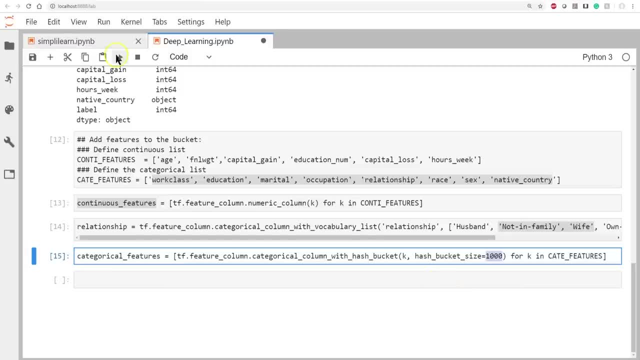 So pretty much everything. since there's not a huge number of categories, each one gets their own kind of bucket setup in there And as far as the initial setup, we need to go ahead and create a model. So this is where it starts to come together. 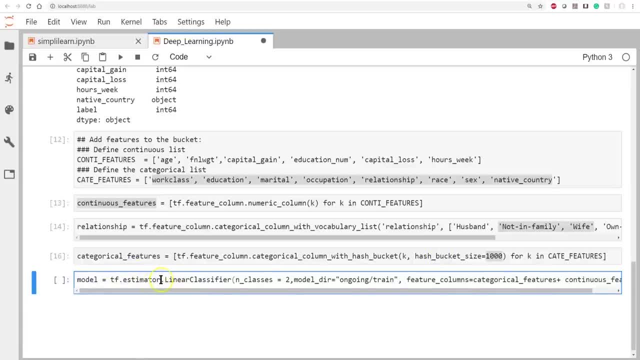 We've as far as the pre-setup, we have our TF, we have an estimator. we're going to do linear classifier on the estimator in classes equals two. So we know there's only two classes we're looking at. We have ongoing train feature columns and then we have our different. we have categorical. 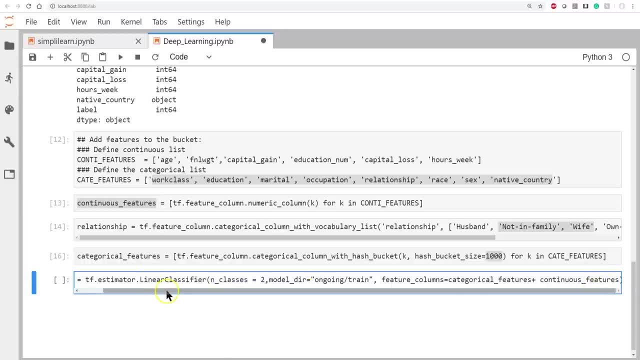 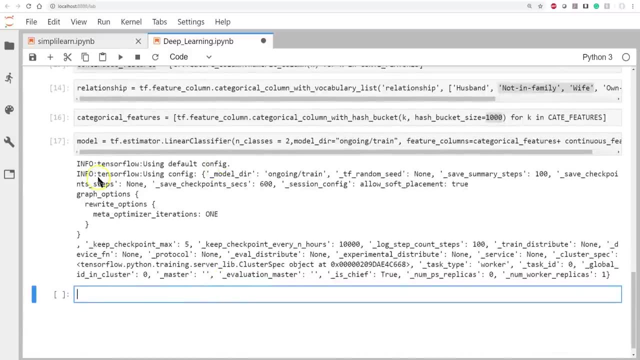 features plus continuous features. So this basically creates our model. what data is going in? And we'll go ahead and run this And you can see here that it gives us a little information that we had our TensorFlow using default config. You can change. there's a lot of defaults you can change as far as the model directory. 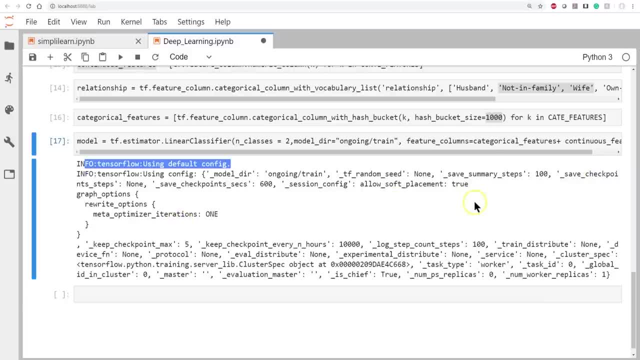 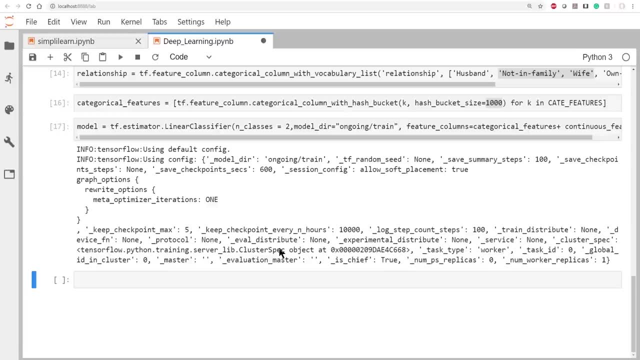 random seed saving, summary checkpoints, there's all kinds of things. you can go in here and set up, Rewrite options, keep checkpoint mix, et cetera. At this point, the model hasn't done anything. All we've done is create the model. 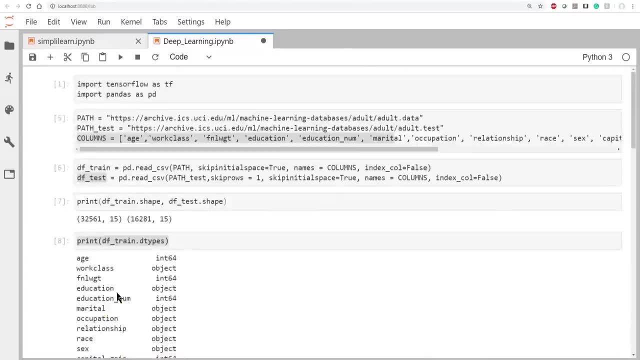 So let's just do a real quick rehash of what we've done so far. What we started off with is we grabbed some data, in this case an adult and adult test. We have a training data set and a test data set. 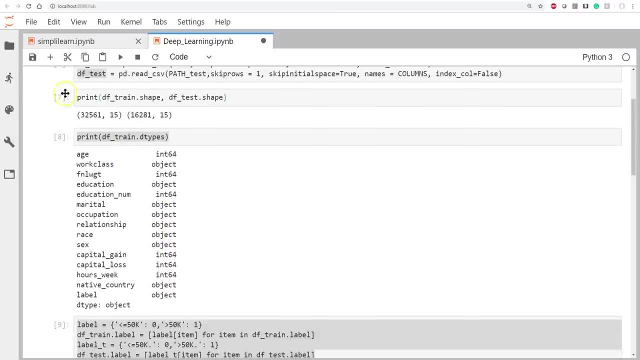 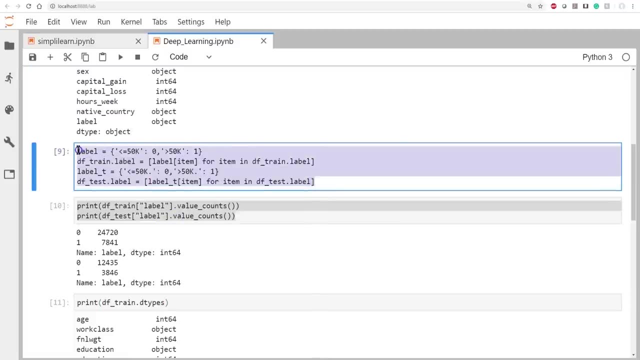 We've got the columns up. We took a very short, brief exploration of the data and its shape. as far as what we're working with, We changed our label around a little bit so that the label makes a little bit more sense of 01.. 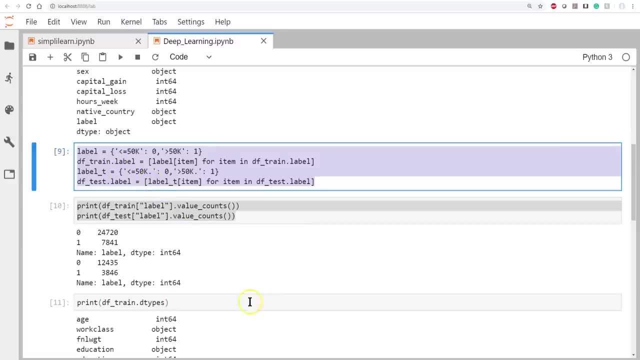 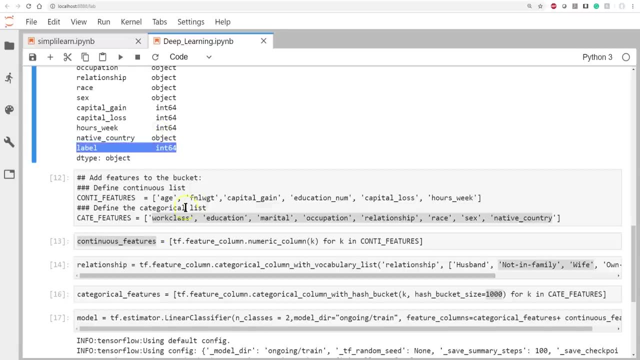 Instead of for the machine, it's easier to spit out a 0 or a 1.. We can look up here. we double check to make sure how many 0s and 1s we have. Double check our data, make sure it's integer 64, nothing weird's going on. 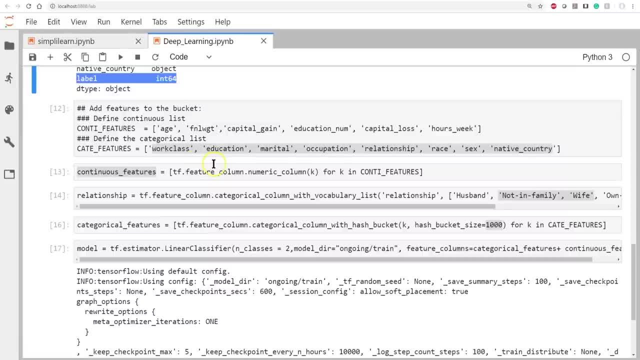 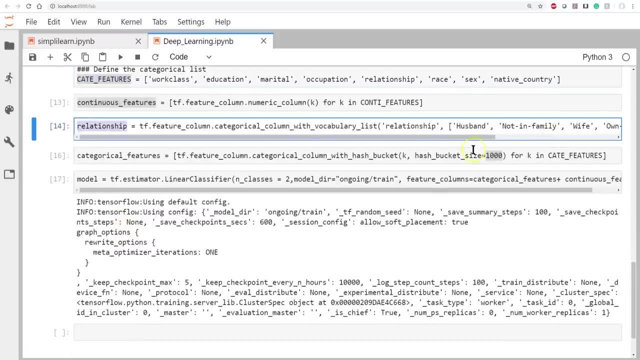 And then we looked at three different ways that we can kind of label the data as far as the way we're going to read it. We have our continuous features and our categorical features. Here's our relationship, which is one of them. When we went ahead and created our model, we did not put the relationship in here, which 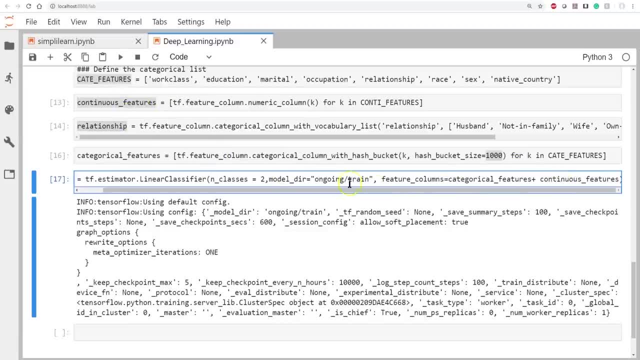 you can do. You can actually maybe take it out of categorical and then have its own on here instead of having categorical features and continuous features and so on. So we've created our setup for our model. The next thing we need to do is we need to go ahead and create a function letting it. 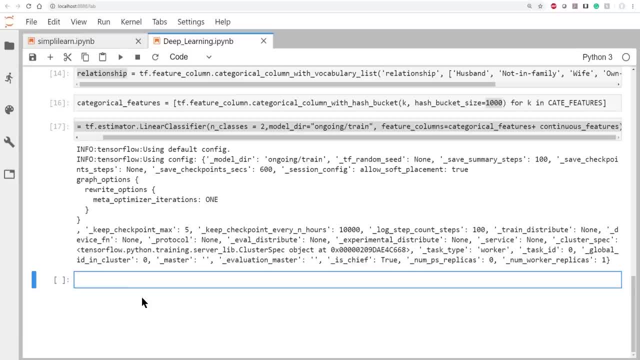 know how to read the data into our model, How are we going to train it? And let's go ahead and create two variables. The first one is going to be features- This is just all the features that are in there- And then the second one is going to be our label. 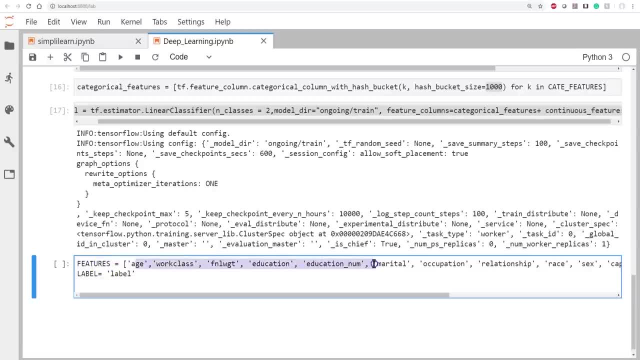 And this is basically. we're looking at all the different information we can put into it, and then is that person, based on that information, going to make less than or greater than 50K? That's what that comes down to. Now, the next part, the definition we're going to create, has a lot in it, and we're going 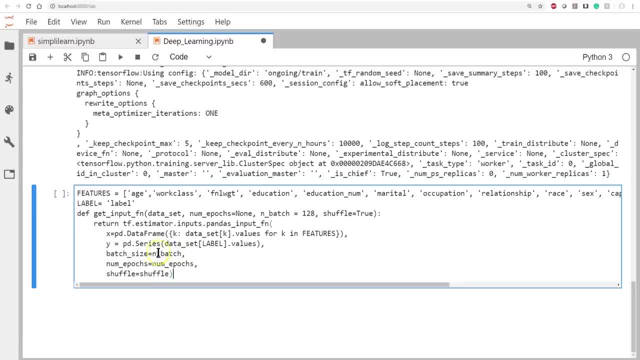 to feed this definition into our model training. So there's a lot of stuff that goes on here. First we'll call it get input and function def. get input function. We have our data set. number of epics equals none, in batch equals 128, shuffle equals. 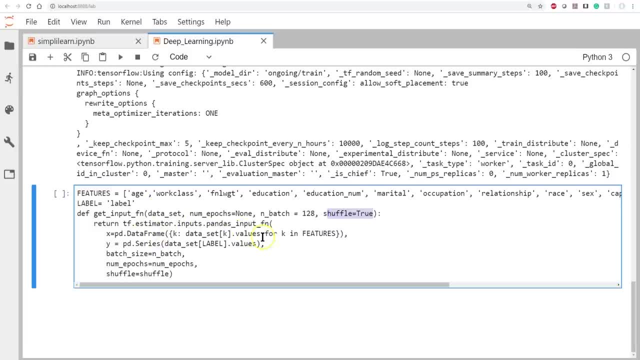 true. So we're running this and this is going to return a tf estimator inputs, pandas input function, And in this case it's going to be x equals our PD data frame. k data set, k values for k in features. Y is PD series data set label values. 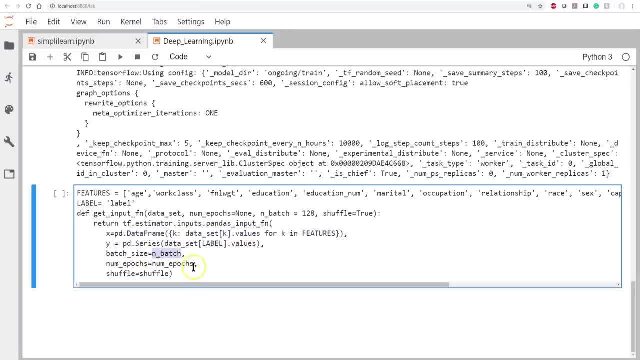 Batch size. Size equals in batch. Number of epics equals number of epics. Shuffle equals shuffle. So in here we're passing in the number of epics We're not too worried about. we're going to just go once through the data because there's 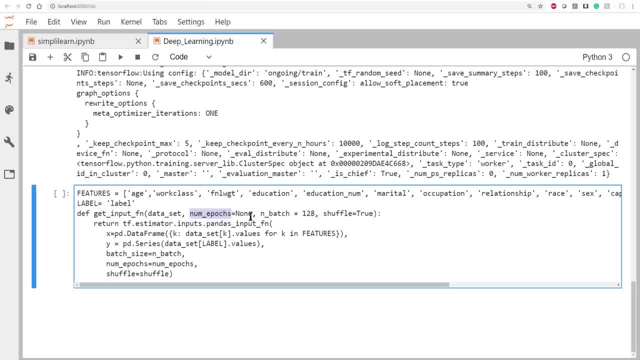 a lot of data in there, We don't need to rerun it. Epics is: how many times do you cover all the data? And then how many groups of data do you pull in and batch at a time? So we're only going to look at 128, do the reverse propagation, like we talked about? 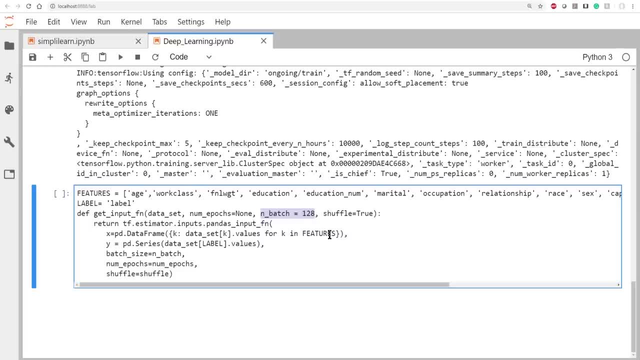 and then it'll go to the next batch, and the next batch, and the next batch and it shuffles them. So shuffle means that we're randomly picking where they're coming from. Again, we're not too worried about the number of epics for this particular model. 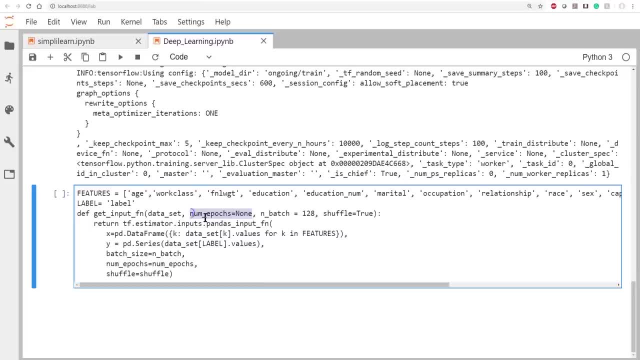 Depending on how much data you have and depending on what you're running. it depends on how many epics you need to run, And there's a lot of rules on how many epics you need to run. One of them is if your training data and your testing data, because you'll check your testing- 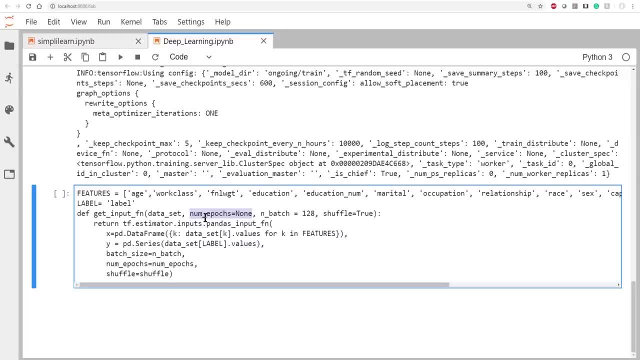 data against your training data. If your testing data starts having better results than your training data, that means you're no longer fitting towards the data, but you're fitting to the answer. So it's kind of these little weird things you start to on here. 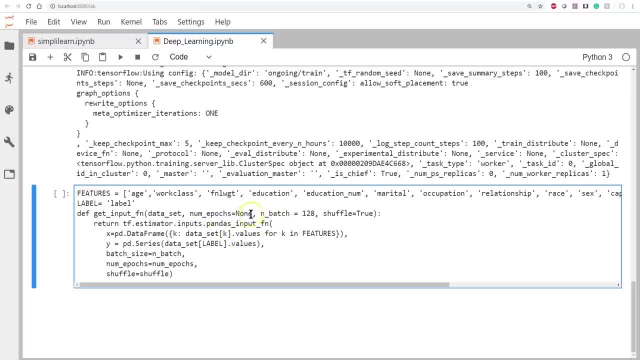 And TensorFlow is really cool because it actually checks a lot of that for you. But we're just going to set number of epics equal to zero and then we have our data set going in, So we're creating our get function. How do we get the data into training our model? 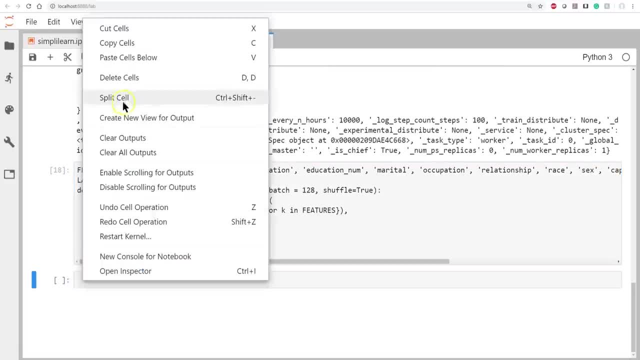 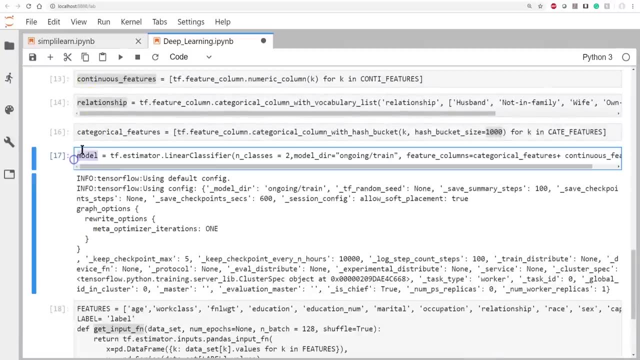 And we'll go ahead and run that. So now we have our data function and now it knows where the data is coming from. So we need to go ahead and train it, And that's simply. we take our model we created way up here. 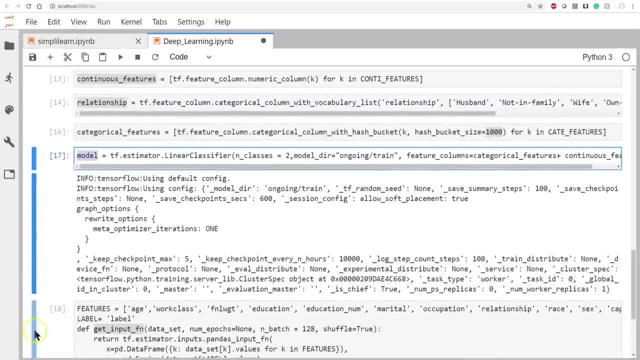 That's where we take the model there. We've told it where it's coming from, And then we're going to run it. And then we're going to run it. It knows what columns it's going to pull in, so it knows what columns it's looking. 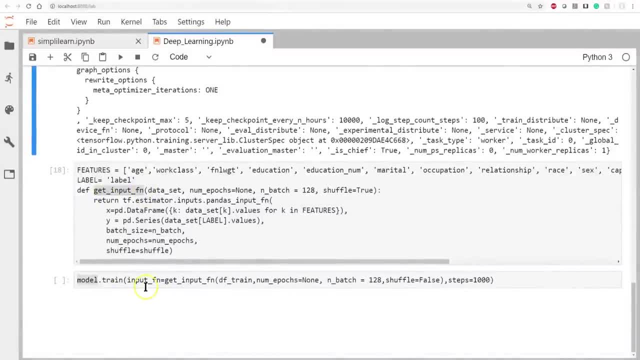 at know what the definition, where it's going to get the information from. So now we want to go ahead and train it, And here's our input function equals, in this case, get input function. And here we tell it that our data set is a df train. number of epics equals none, which 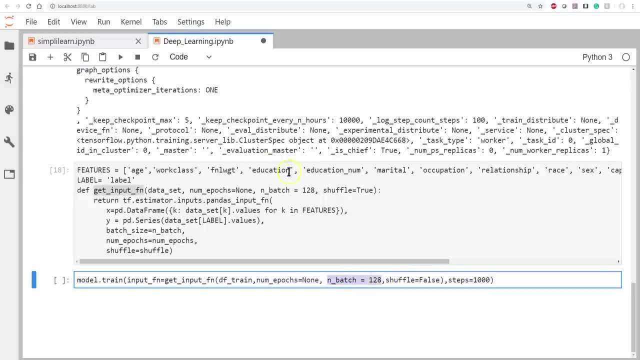 is already automatically set up there in batch equals 128, which is what we have up here. Shuffle equals false And we're going to do 1,000 steps, So we're actually going to go through 128 steps. We're going to do that 1,000 times. 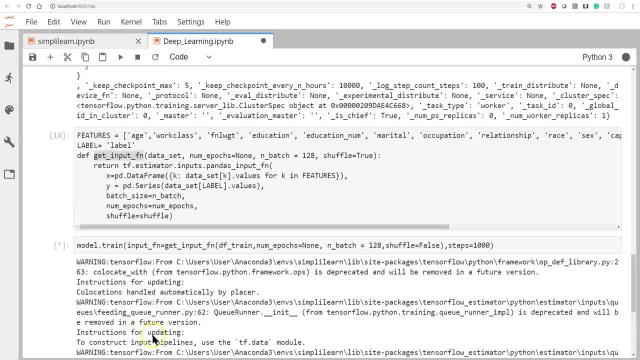 And we'll go ahead and run this And I just ran an update, so it's going to give me some warnings because of that update And then we're back here and it's still going To construct pipelines. use tf data module. 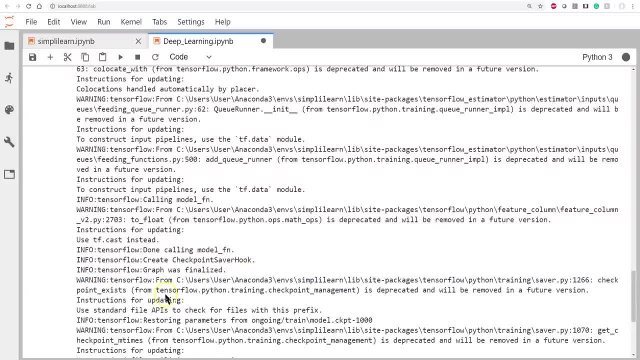 Not a big problem. Let me let it go ahead and run all the way through on here And it takes it just a moment. There we go, There's our 1,000 coming out And, as you can see here, here's checkpoints for 1,000, ongoing training: 1,001, global. 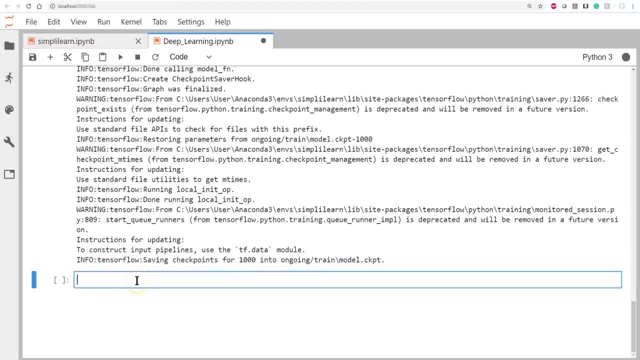 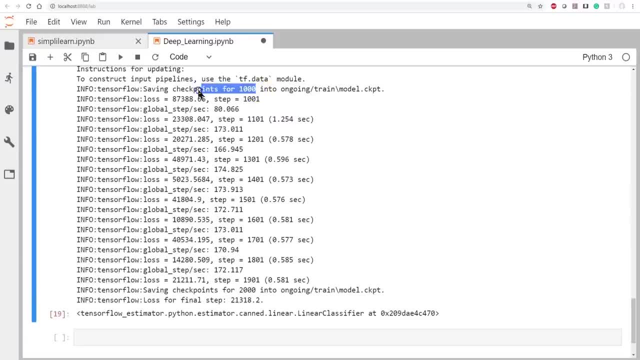 One of the things we didn't cover is we do it in small increments So it's not all done like one error goes all the way back. You'd only do a part of that error And each one sends back a little piece, so you slowly adjust your different weights going. 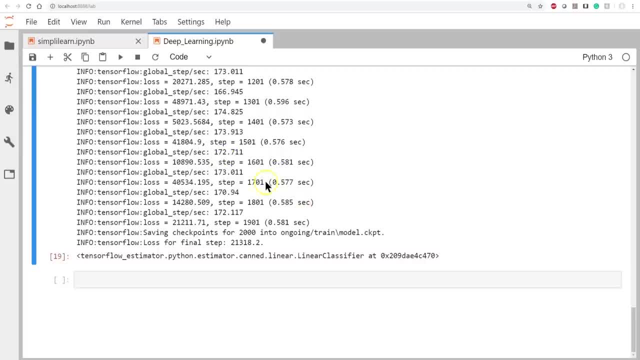 all the way back, And then, if you're gonna train your model, we wanna know how it did, So make sure that you Will be able to get that interesting model in order to show what you can do. So it's now working. 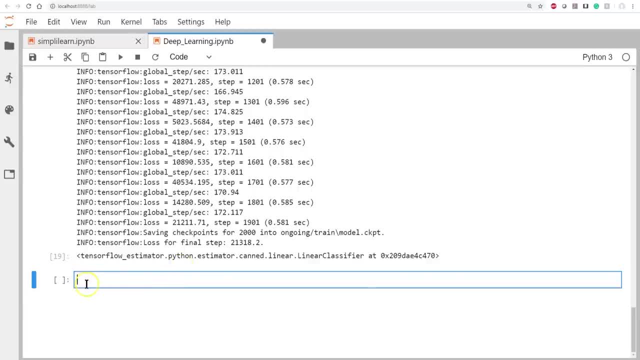 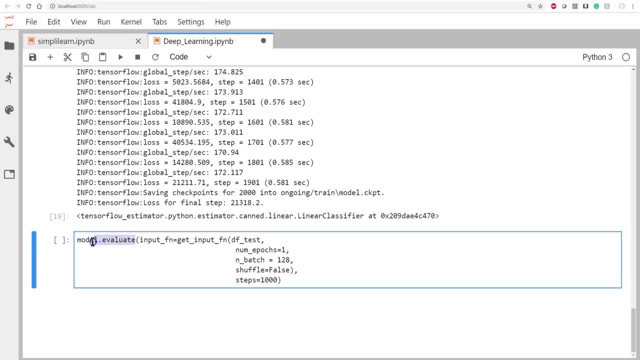 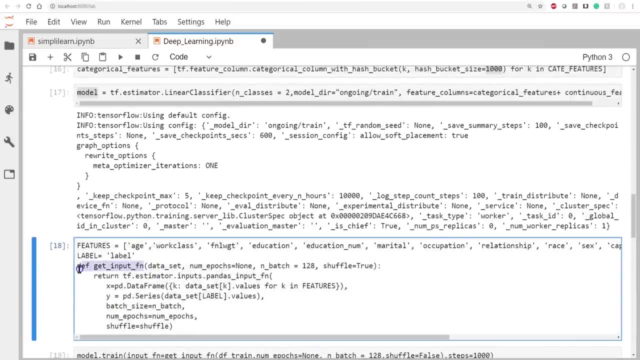 Like I said, we're at 1,000 variables. I punish that model. So we're going to do model evaluate and our input function equals. remember our input function up here that we created Way up here. We're going to take this input function and instead of the data set that's coming in, we put in the data set here for training. 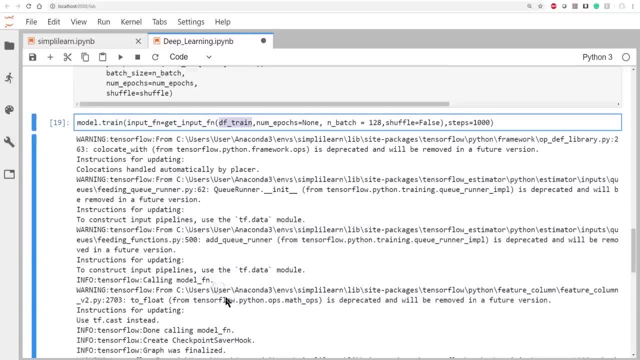 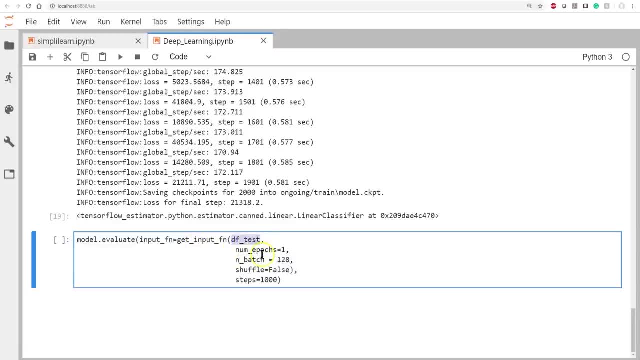 Where's our training input train? There we go: df underscore train. Now we're going to go ahead and evaluate, and here it is: get input function test. So we're going to test the data out. Number of epics: one. 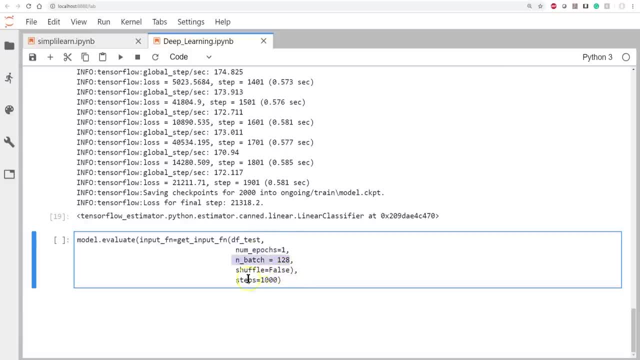 We don't need to rerun it more than once Per batch. 128. So on shuffle and steps, 1,000.. So we're going to go ahead and evaluate this. Let's just see how good our test data did, how good our model was programmed on our training data and how it evaluates on the test. 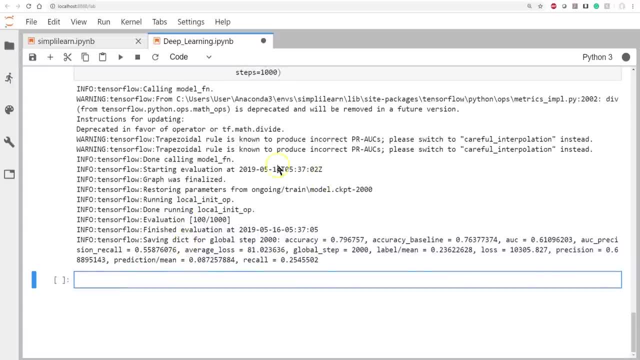 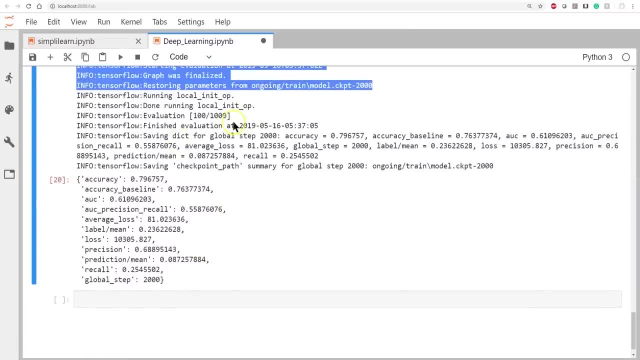 And we can see it going on down here where it's got. the evaluating Graph was finalized. Let me just highlight that Ongoing model checkpoint TensorFlow running local init evaluate 100 out of 1,000, and so on, And once it gets to the end we get a nice output. 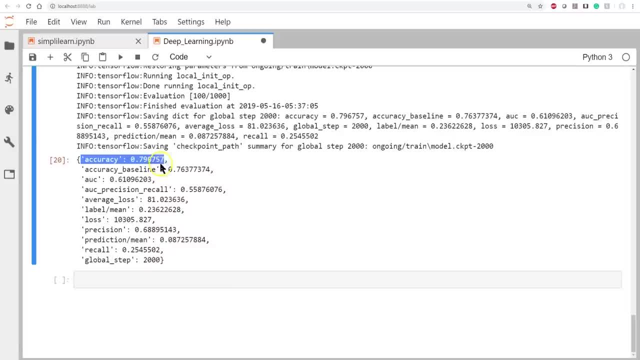 Here we have an accuracy, in this case of 0.79, with a baseline of 0.76.. So now we've created a model, Let's go ahead and tweak it a little bit. So we have our accuracy up here. 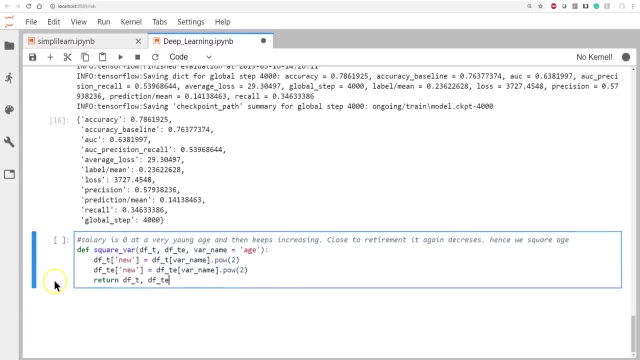 What we're going to do is we're going to look at age And let's just go ahead and create a new square value for age. And the reason we want to look into the square value of age is we know that if you really look through the data. 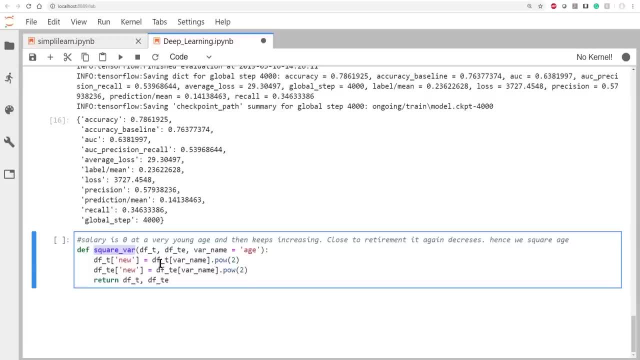 you'll find that as a young person, the age keeps increasing And as you get close to retirement it begins to decrease. So we square the value of age And that's very data-specific. when we're looking at data, You'll find that any kind of data that has that kind of like uptick and downtick- 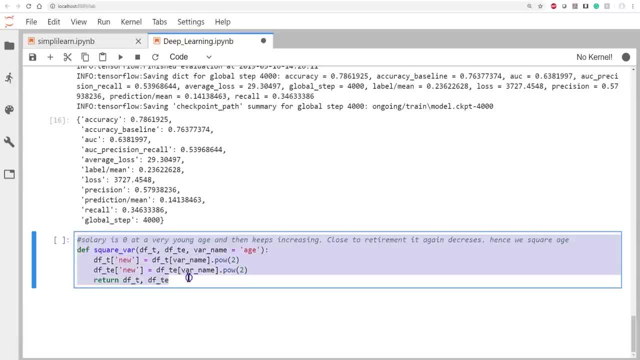 by squaring it or square rooting it, you can get some very different results. And so we're going to go ahead and square our age. And this is kind of it's interesting because at this point, even at the beginning of this, 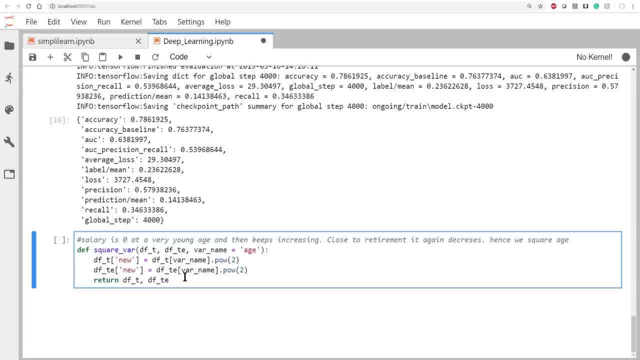 we're focused on deep learning and on TensorFlow. But before I would begin even looking at any of this, I would have probably run some kind of heat map or some kind of evaluation in R or sklearn And Python to find out the correlation between different features, to see just how well they correlate to each other. 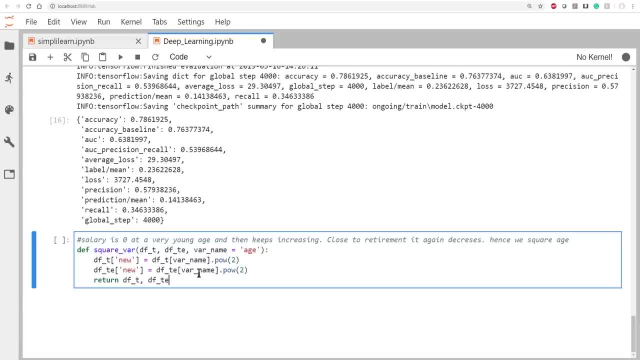 And there certainly are some wonderful tools for that, because sometimes you can just mark off some features and other features you bring in. But for the deep learning we can see how we can just dump it all in there and let it sort it out itself. 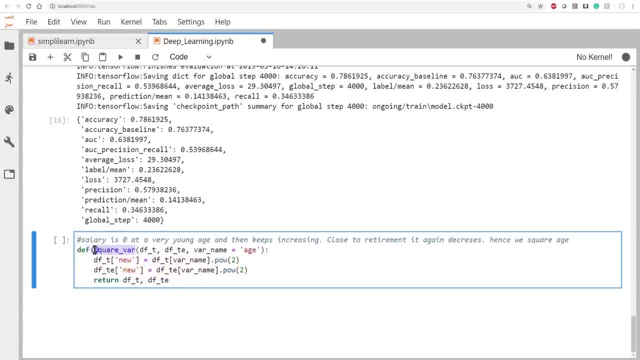 And we're going to just write a quick little function here. to take the square variable In this case we have DFT, DFTE- This is our training and your test variable and the variable age coming in, And we just want to go ahead and create a new under DFT. 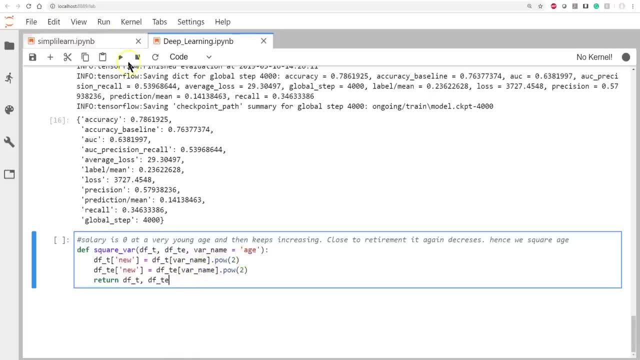 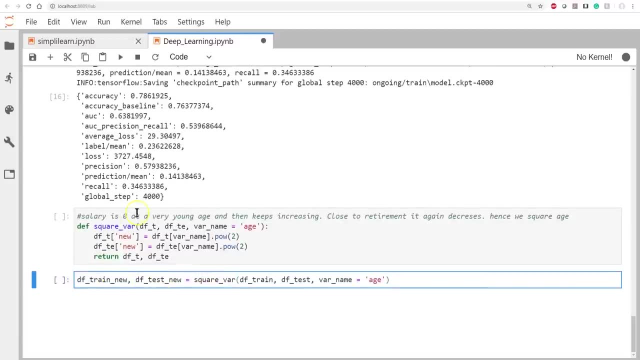 And that's going to be the variable name that we put in there, which will be age. So let's load this. Here's our functions now loaded, And certainly we could have just done that as a line of code. But you start to get the feeling that when you build these functions, 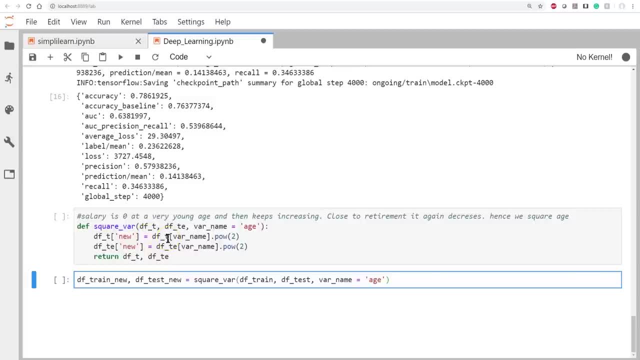 you can now use this function if you had a number of different features that had this kind of quality to them. And we have our DFTRAIN new. So we're going to create a new training and a new test And it's going to equal the square variable DFTRAIN or DFTEST. 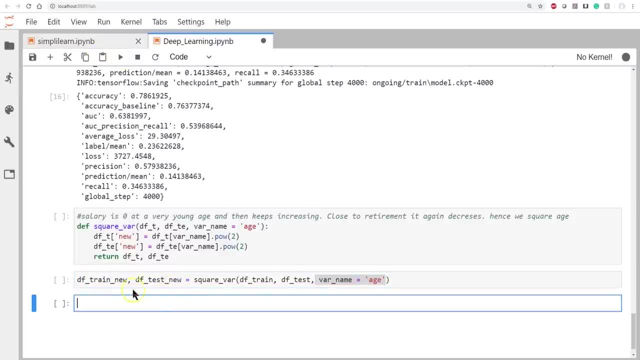 And the variable name is age. Let's just go ahead and run that. So now we have our new, Our DFTRAIN, DFTRAIN new and DFTEST new And, just like we did before, let's just double check the shape of our data and make sure it all matches. 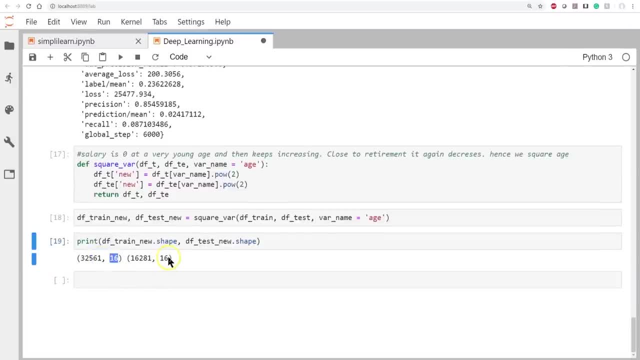 And when we look at the output here, really what's important is that each one of these has 16 features in it. We want to make sure we're not getting something weird on there, And our training set has 32,561 rows in it. 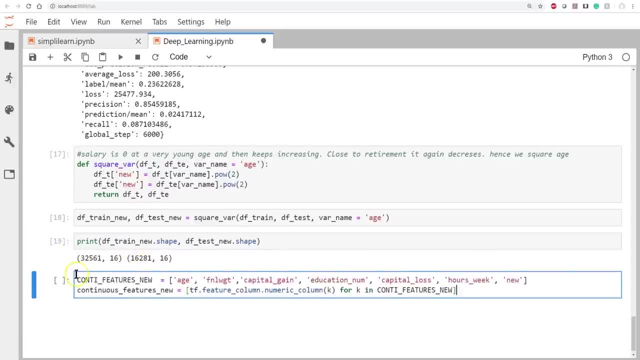 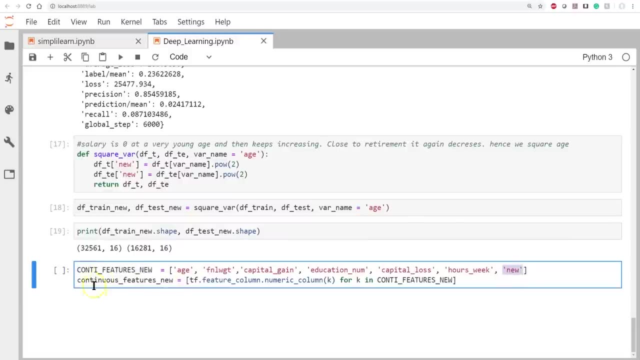 And this one has just over 16,000 in there And everything's pretty much the same, except that in our continuous features new, we now have the new column We put in there, So we need to change that. And we have our continuous features new down here which we're going to load up with our TF feature column numerical. 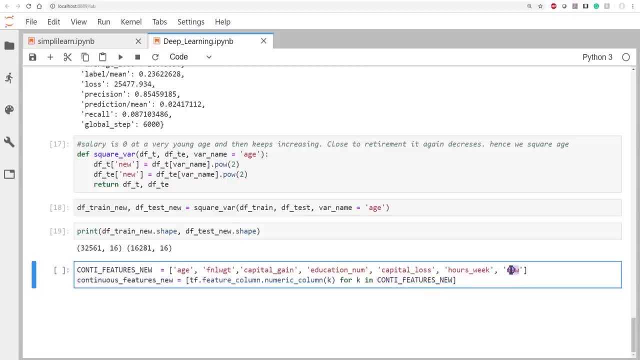 This would all look familiar, because we just did this, And so we're going to load that up with the new being, the new value in there, And let's go ahead and run that And we'll create a model that we'll call it model one. 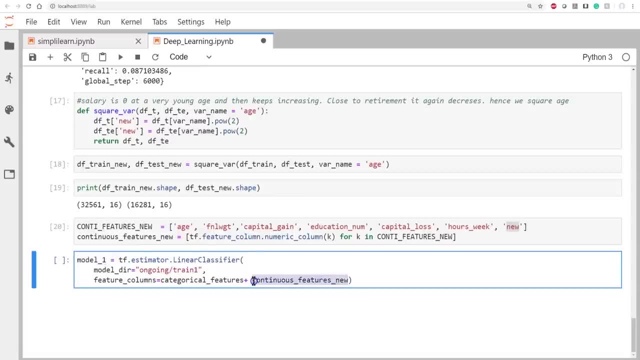 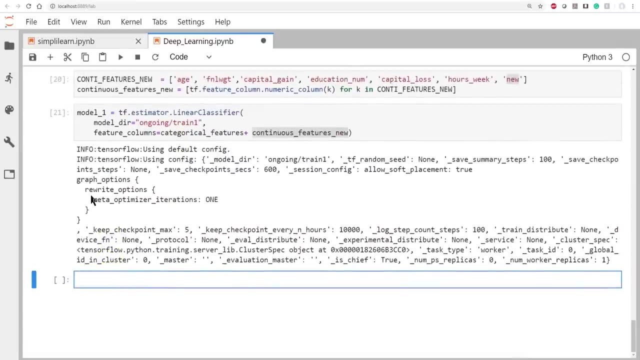 And this is the same that we did before, except now we have our continuous features- new in here. So here's our new model, In this case, model one instead of model, And we're going to build that model right there Now. we haven't trained it. 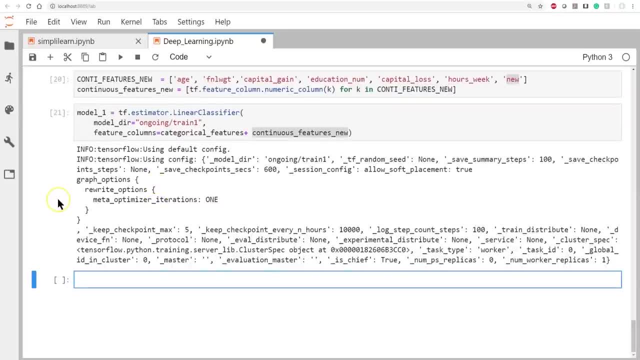 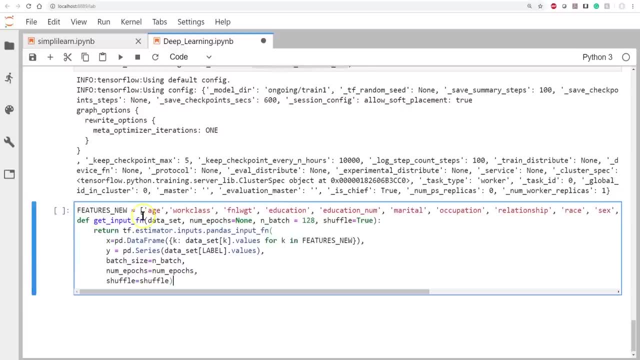 All we've done is told it where to get the data And how to get the data and what features are coming in. We haven't actually told it everything on the features coming in, Because we still need to also build our get input function. 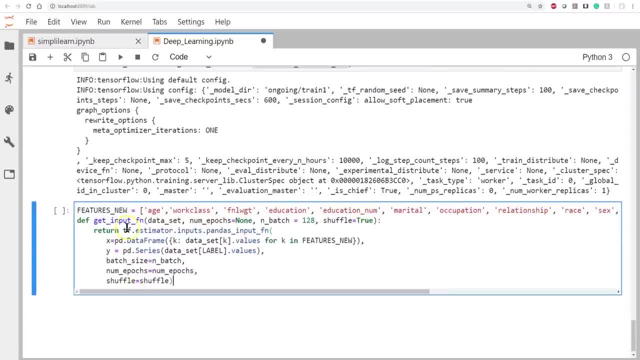 So where's the input coming from? So we built the model with the features in it, And now we need to go ahead and create our get input function. This is the same as before, But you'll see we now have it with the data set coming in. 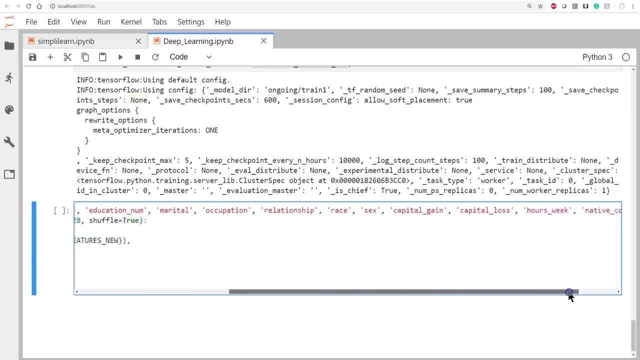 It's going to be the same data set up here, And so if we scroll a little bit to the right, we should see the new, And there it is Sure enough. there's our new on the right, And so let's go ahead and run that. 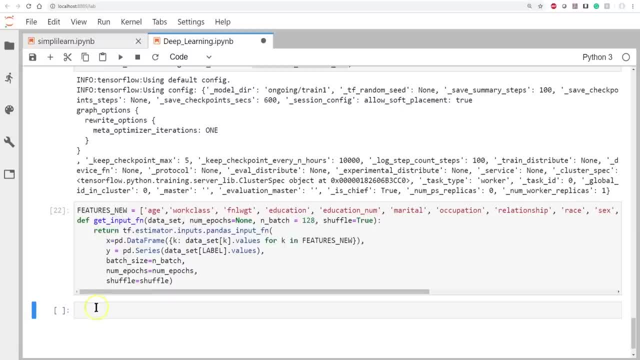 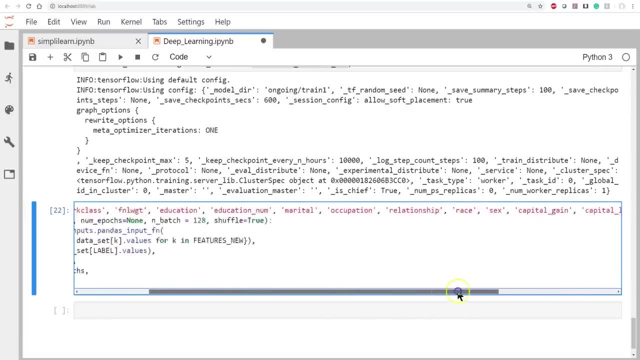 Now we've defined our model, We've defined where the information is coming from And again, you can go back and review the first part, Because this is identical that we did before, Except now we have new as the column for the age. 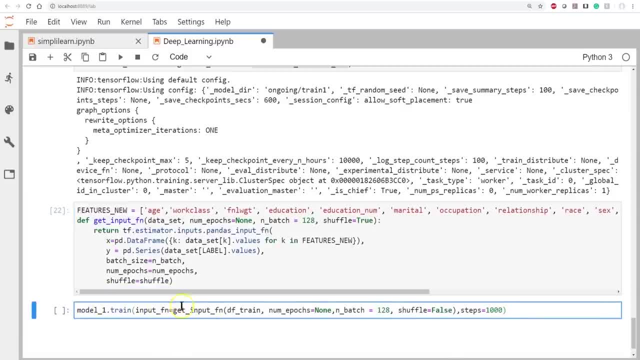 And we'll go ahead and do our model one And let's go ahead and train it. There's our input function: get input function that we defined up here. DF train is going to be the same And everything else is going to be the same. 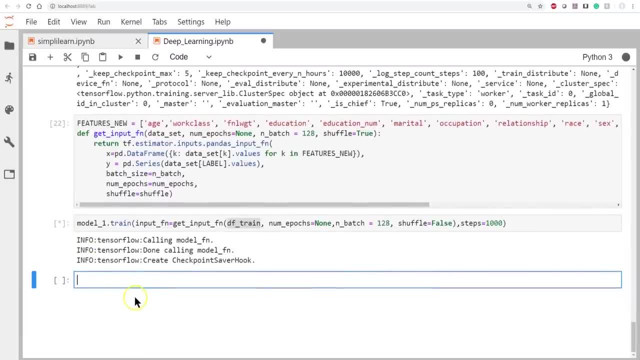 Let's go ahead and run that And it should go through here and run the tensor info coming in And it's going to go through. in this case we have steps 1,000 shuffling, So it's going to go randomly. 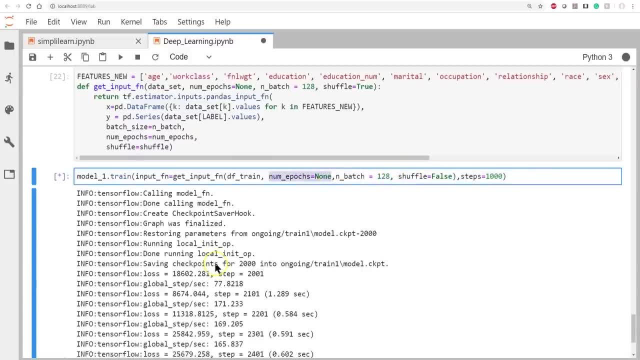 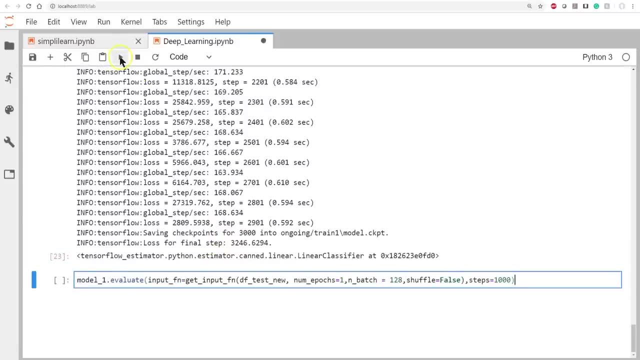 128 per batch, And then the epics is automatic. We're not worried about that today. So now we have a trained TensorFlow model And with our new model, just like we did before, we want to go ahead and evaluate it. 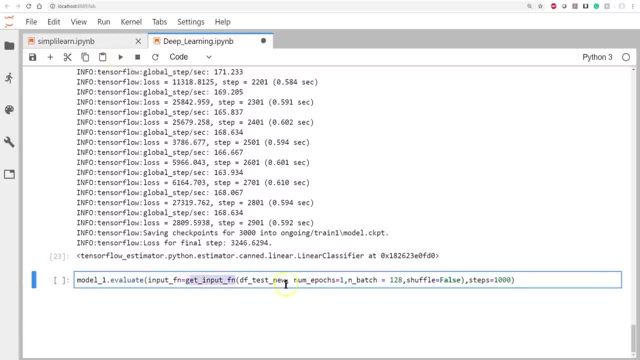 So it's the same setup we had before, with our same get input function, With our DF test new in here coming in. So there's our new data coming in. And this is really common when you're doing these models: You make little tiny tweaks to see if you can improve it. 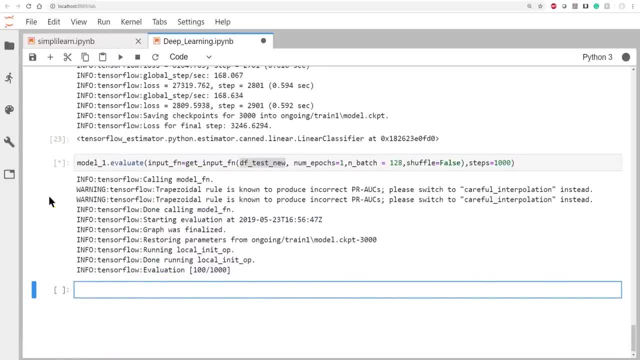 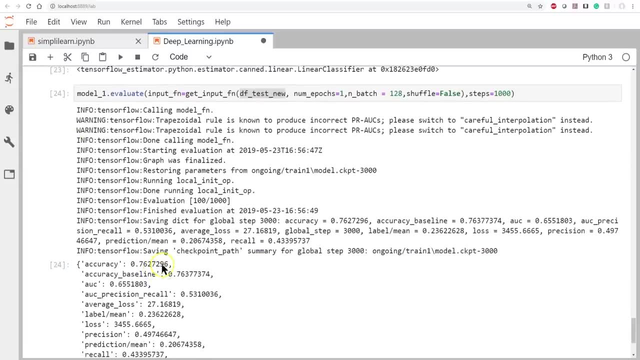 One of the best articles I read recently was: you build your model to fail. You want a running model so that you actually have something to compare against, And then you continually tweak it until you get a better accuracy. Now I don't expect the accuracy necessarily to get better on this. 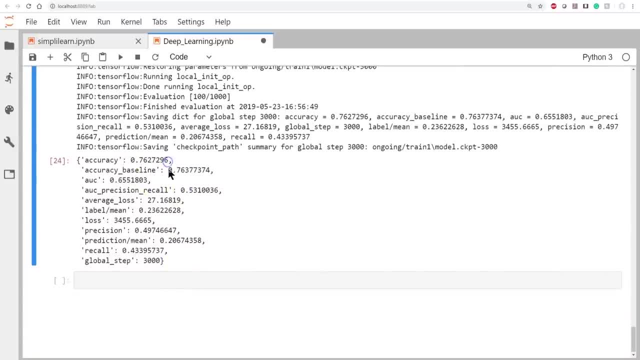 because of the way we partition the data. But we can see here we now have an accuracy of 0.76, which is a little bit over the baseline, And it's about what I would have expected it to be, kind of the same. 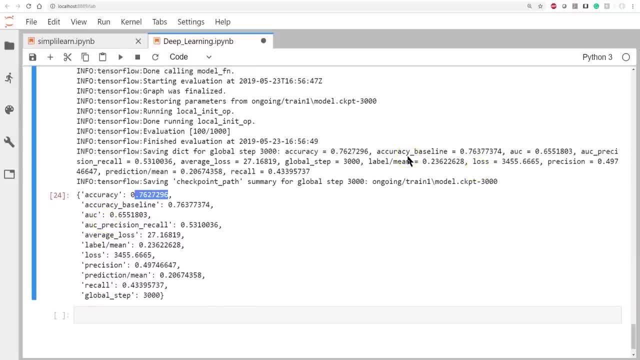 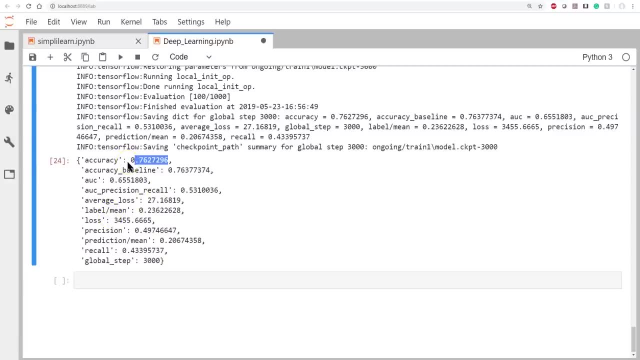 The reason is because we split the data at the 50, the people making over 50K and those making less, And so the age factor shouldn't be a huge factor. It would be if we were looking at more discrete buckets like 40 to 50,, 50 to 60,, 60 to 70. when we create buckets, 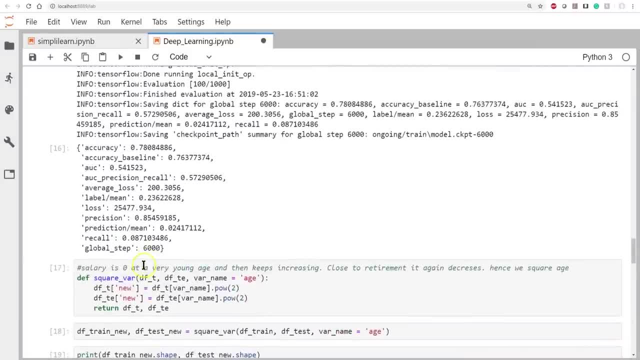 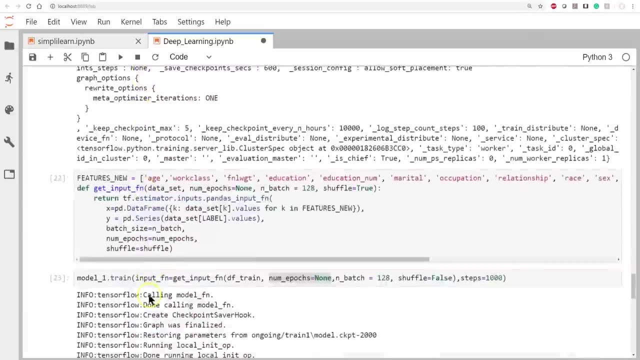 But in this I didn't really expect it to go up that much. In fact we could probably run it a dozen times, which would be very bad data science, And we see we actually had a slightly better one up here, But our baseline accuracy was 0.76.. 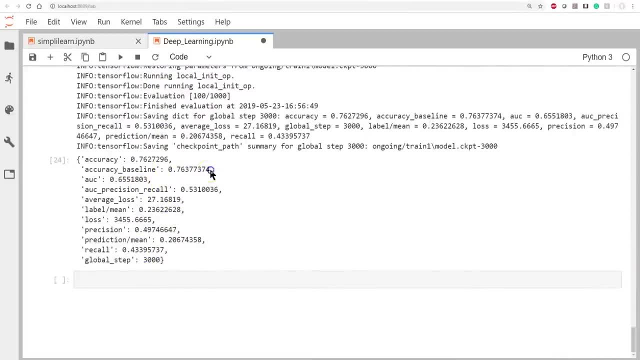 And we come down here and we still see here's our accuracy baseline 0.763.. That didn't really change And you know the accuracy didn't really go up that much. I could hit the run button And a few times I would probably upbeat the one above. 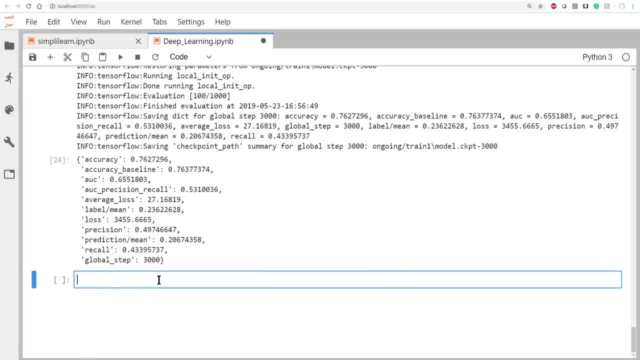 It's not a big change, But that's all right. This is how we learn. This is how we go through and figure out what's going to work with our data and what's not, What's going to improve the quality of our data so we have a better prediction, and what's not. 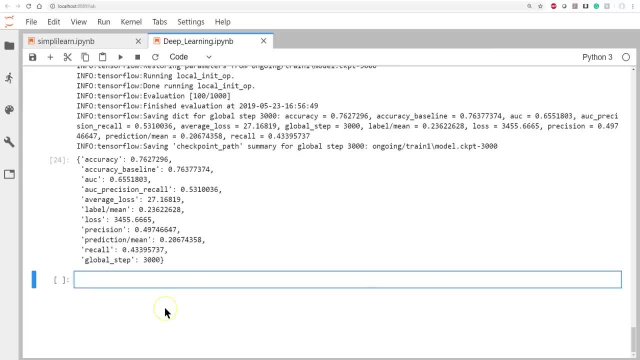 And we can now go ahead and utilize this model. This is where it gets exciting: when you're actually working with somebody or with your clients, And you come in and you say, OK, here's my predictions. We're going to create a list. 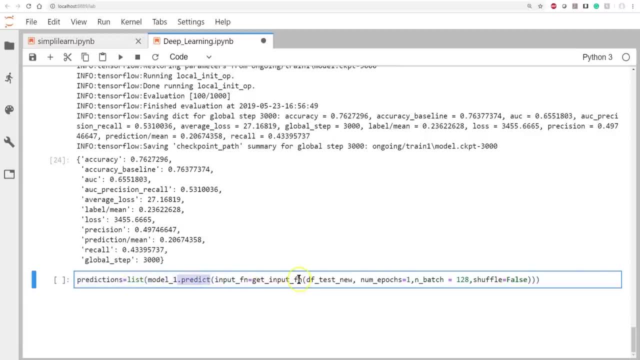 And we're going to use model one And we're going to predict And our input function is get input function dftestnew. Again, this probably doesn't make too big of a difference, But we'll go ahead and stick with the new data we created. 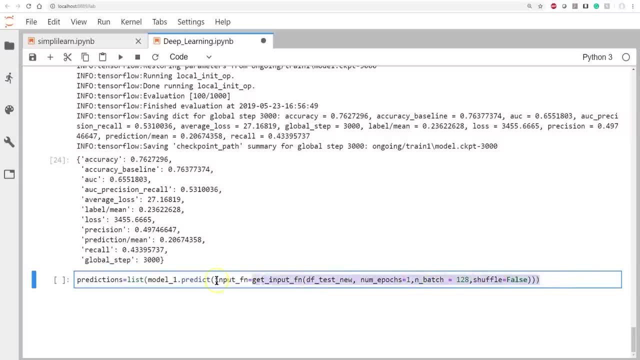 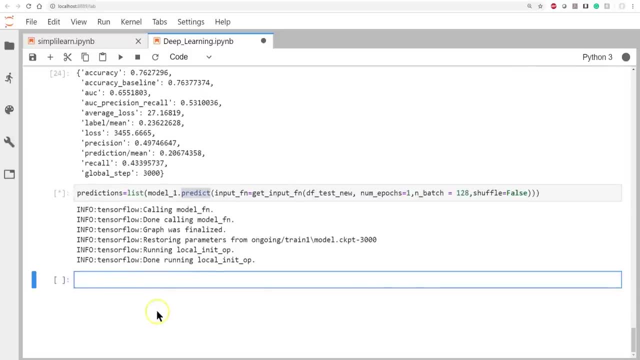 Number of epics: 1, batch 128.. So all this should look pretty familiar, But we're running the prediction, So we're going to load all our predictions into the predictions And let's go ahead and run that And you'll see it go through the TensorFlow setup. 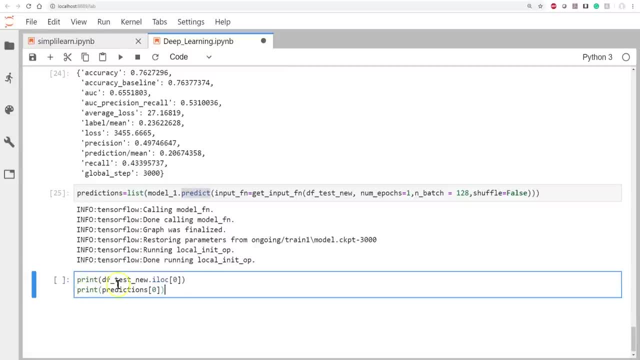 So it's running, done running local ops, And then let's just go ahead and print the dftestnew ilocation 0,. so row 0. And we're going to look at the predictions also for the same location: 0.. 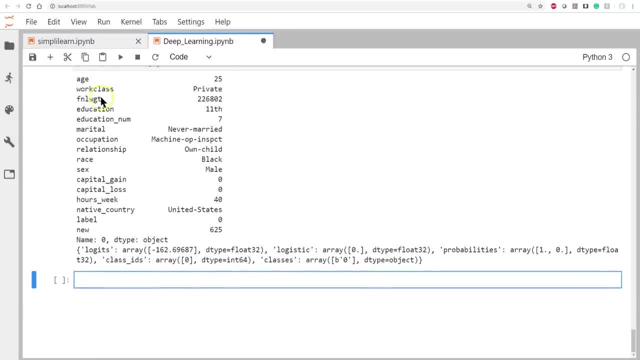 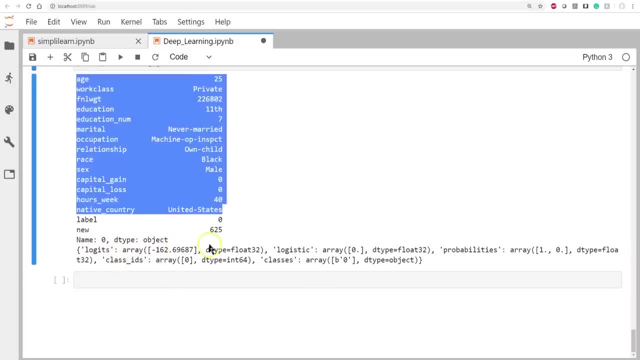 Let's go ahead and run that And we can see here that we have age 25, work class, private. It has all the information coming in for that individual And then it comes down here And we go ahead and get our prediction. 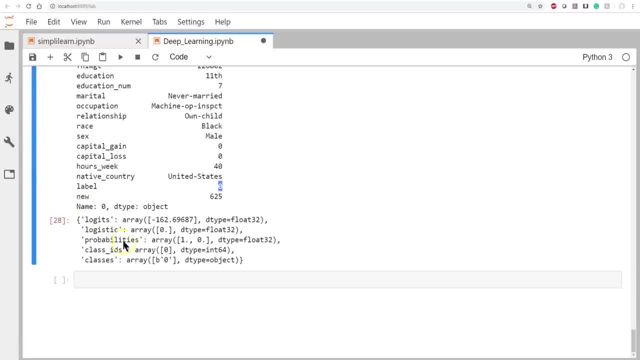 And in this particular instance there's our label 0. And then we come down here And we see it takes a little bit for the setup to look up, But there's our array, which also returns a 0. And it has information for us on there: probabilities, logistics on here. 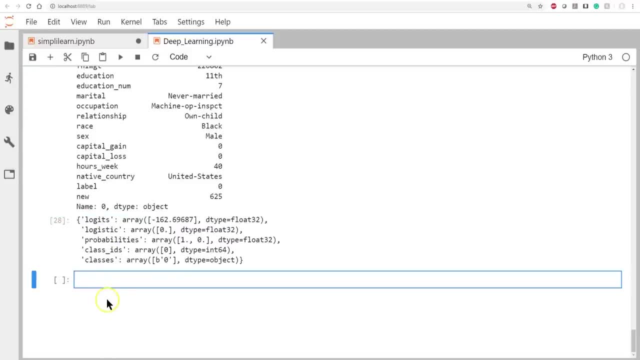 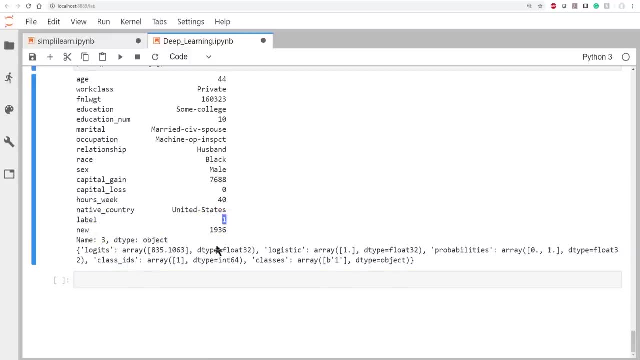 So you can see there's all kinds of additional information you can pull from this, And likewise We could do it for position 3.. Let me go ahead and run that, And what's kind of nice about this is you can now see here's label 1.. 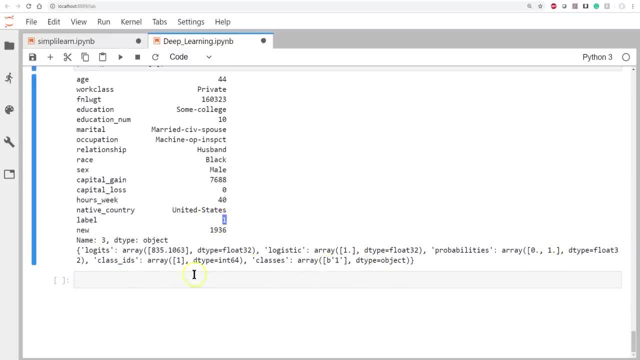 And here's our logistics output. And again we have to kind of hunt for it a little bit in this particular setup, But here's the output array And there's our 1.. And they match Label 1, 1.. 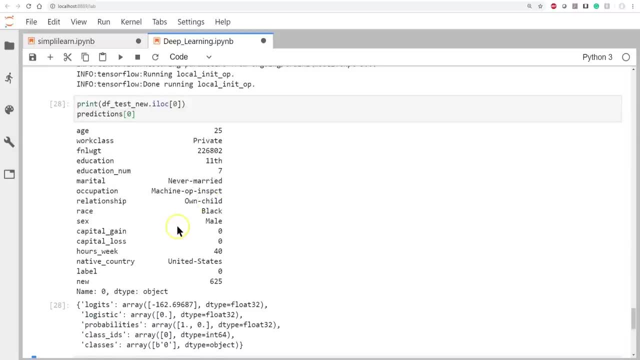 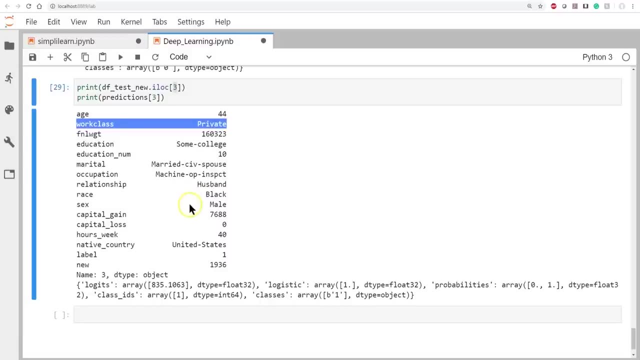 So we predicted for the very first one location, 0, that it's going to be a 0 on the label. It's going to make under 50,000.. And the individual in 2, working class, private, whatever setup on here, capital gain, capital loss, etc. 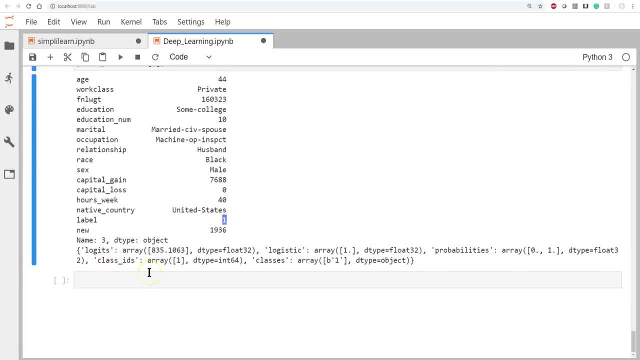 And the individual in 2, working class, private, whatever setup on here- capital gain, capital loss, etc. It came up as 1.. Meaning they're going to make over 50,000.. So we covered a lot. I mean, this is the basics. 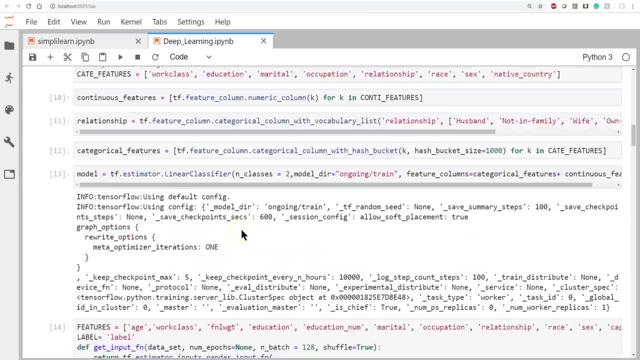 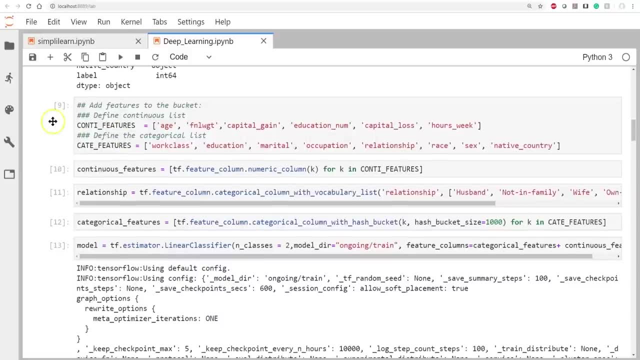 And you can see as you dig deeper when you look at some of this code. Let me just go back up here. We're way back up here at the very top, A little too far overshot As we start working in. here we have 1 defining your features. 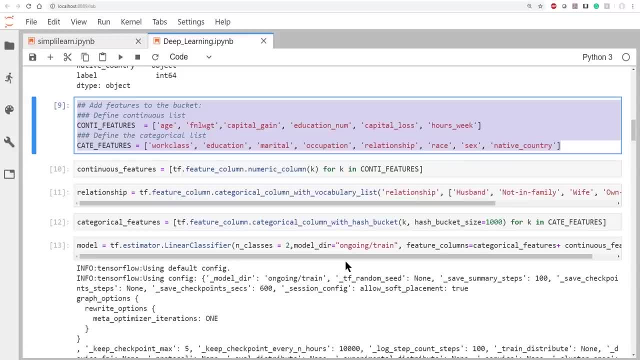 And at this point we didn't show this, but I would probably use either Python or R to show a relationship correlation, Because they have some really easy packages in there to pull that up So you can see what features are really connected and how they're connected. and then we showed you different features, like 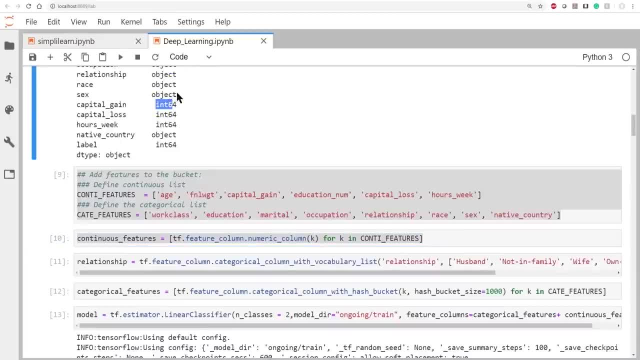 we have ones that are integers and then we have ones like sex that are objects, your zero one, your male or female, your same thing with a race, probably have just a maybe 16 different races listed there, necessities, things like that native country again that's. you don't have like infinite number of. 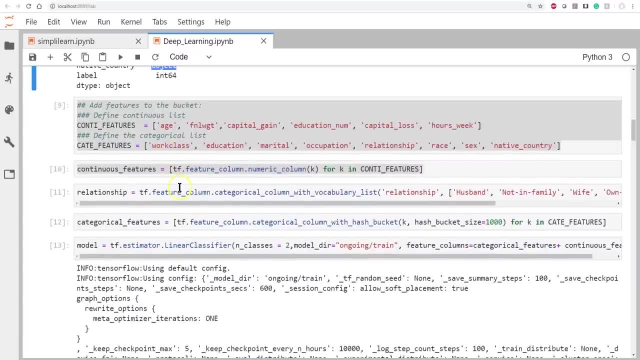 native countries. you just have a handful. so we look at this, we have our features, we looked at that, we have our continuous features, like age, which is a number, or, in this case, an integer, and education number, how many years, and so on, along with your race, your sex, your relationship, which? 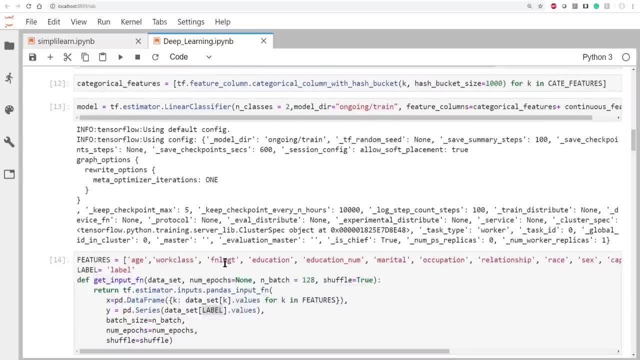 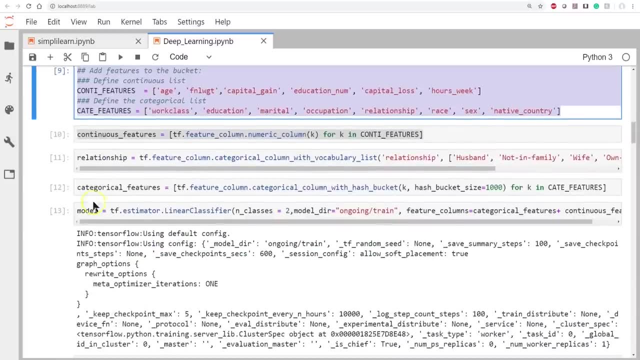 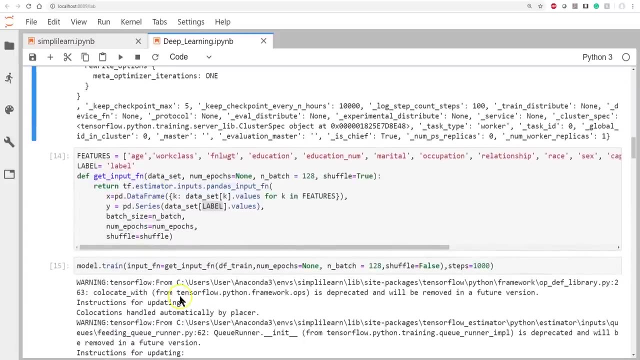 are just very abbreviated categorical data. so we looked at that, we went in there and we showed you how to. where was it here? we go, go back up here so we create our model. the model knows what categories are coming in. that's really important and this is probably the one of the more complicated parts of 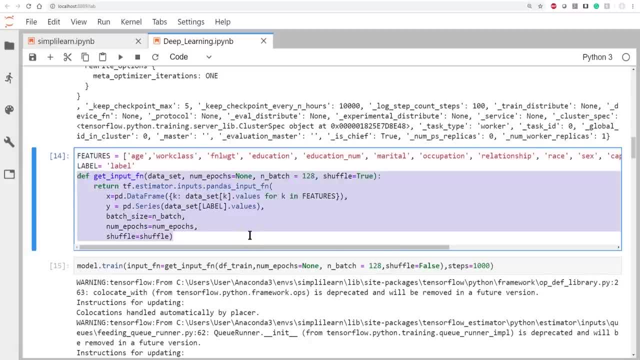 this is our input function and this input function is so important, so I want to just rehash the input function for that reason. this lets us know how we're pulling the data. it lets us know if we're gonna go through all the data 20 times, or we're gonna let the, or we're just gonna let tensorflow. 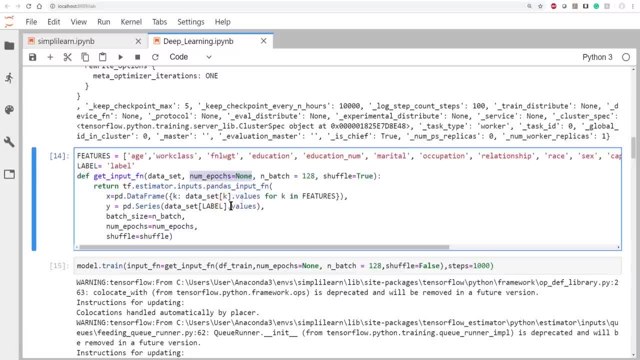 itself keep going until the training model reaches a point. that point is based on what they call bias. you can become biased on your training data and so when it hits a certain point where it becomes overly biased to just that data, then it doesn't really work really good in the outside world. you start losing. 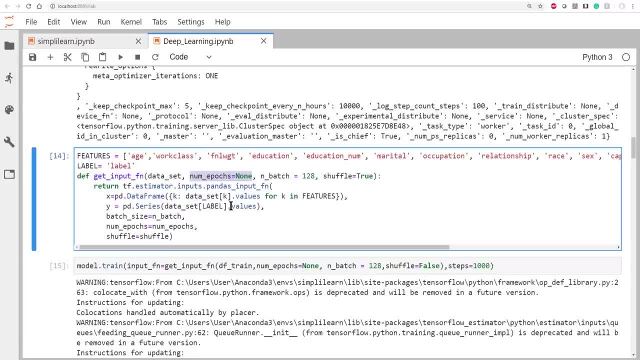 when I keep it generic but as close as possible to the right answer. so generic answers for a huge amount of data, and then we have our batch size- are we gonna shuffle it, which we did? and then also our estimator inputs- see of your estimator function here, and then, of course, where the actual 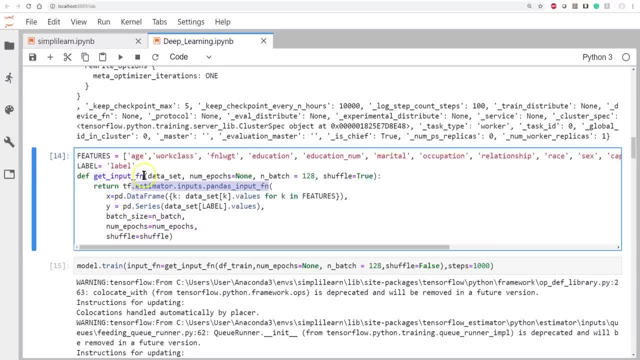 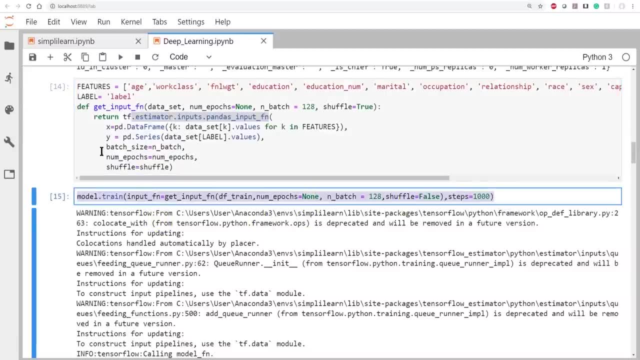 data is coming from. so you can see all this is in that get input function. that's where a lot of the work comes in: putting this together and then we train our model. that's pretty straightforward: once you have your input function and all your setup, training the models quick and then we go ahead and 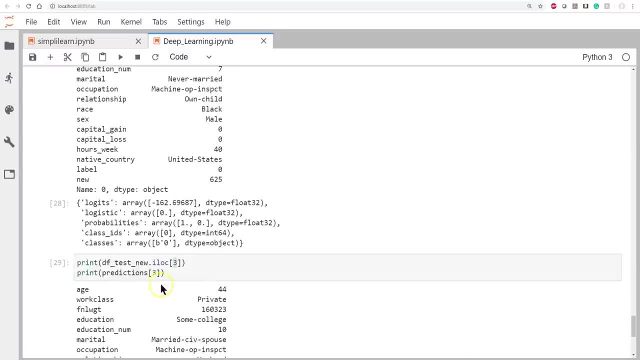 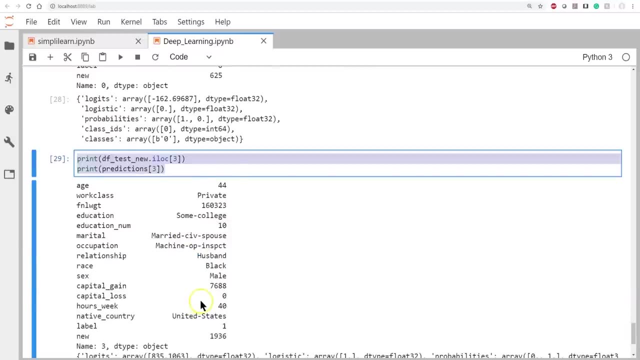 evaluate and then we can go ahead and create a predict and then you know, look at our predictions and how they work on individuals. so it's pretty gives you a whole roundabout set up on here and how this is set up and how it's working. certainly there are a lot more things you can do with. 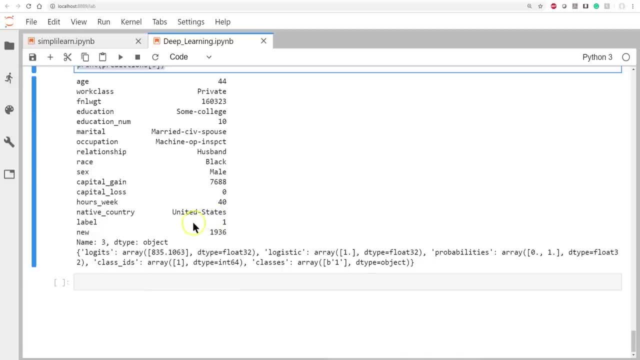 tensorflow. this is the basic tensorflow and it's always developing, so it's exciting. this is gonna be one of the most exciting fields right now because it is really in an infinite stage and just exploding in the market. in today's exciting world of AI, artificial intelligence, we're going 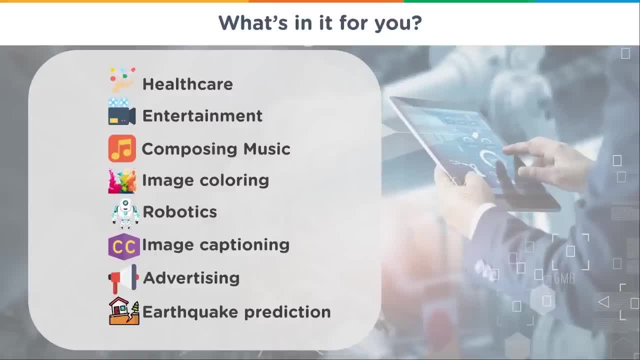 to cover some of the many uses as being applied to health care, entertainment, composing music, image coloring, robotics, image captioning, advertising, earthquake prediction, and there's many more. it's just an exciting time to be in the field of AI and deep learning and artificial intelligence now. all these fields are just booming. it's just amazing what's going on. 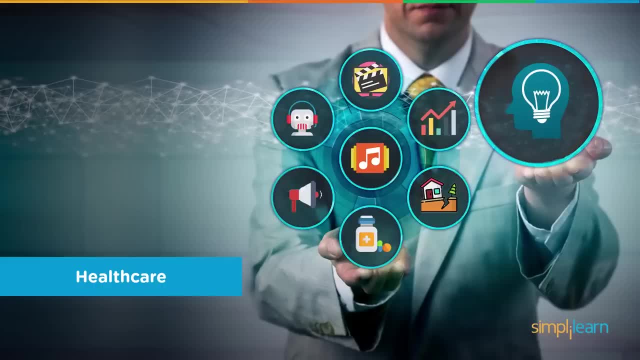 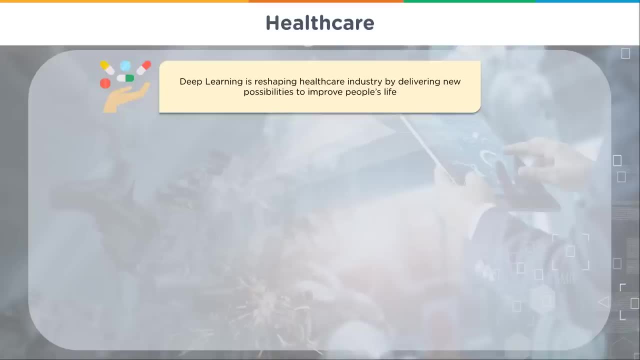 so let's take a quick glance at some of the things going on, and we'll start with our health care. when we take a look at health care, deep learning is reshaping health care industry by delivering new possibilities to improve people's lives, and we have computer-aided disease detection. I know a 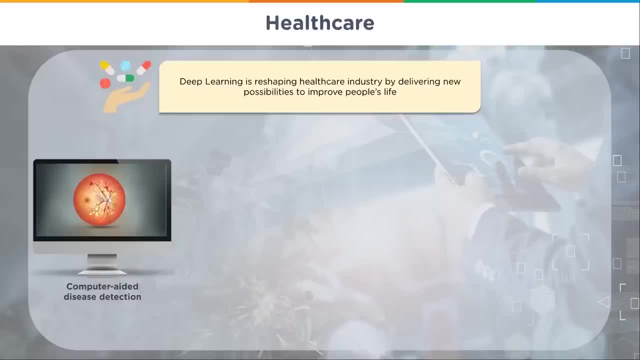 number of startups have come up where they're working on. you take a picture like if you have some kind of irritation or rash and they use that. or even you know some infection in the eye and they use the deep learning to help identify what it is. hey, this. 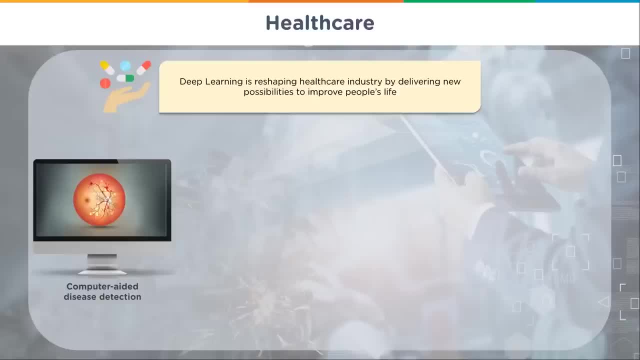 is 99.99%, nothing, don't worry about it. or this is 93% chance. it usually doesn't come out 93% chance if you do deep learning, but it says, hey, you know, you should probably take this into the doctor, you know, have them take a look at it and see what it is. these are the things that could be analyzing. 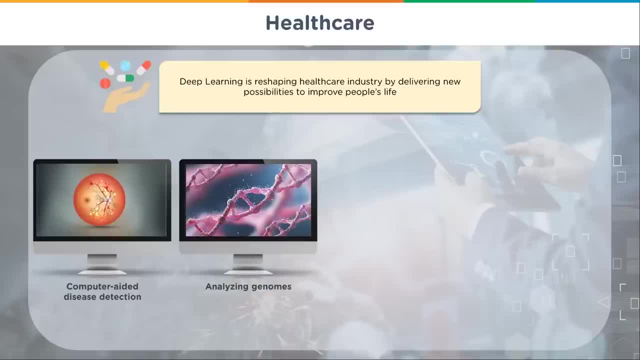 genomes. that's a big one, very controversial nowadays with all the different genome editing and options they have and things they're doing. but deep learning is definitely diving into the genome projects. we have discovering new drugs and this- there's so many directions for new drugs going on. it's like one of the booming industries, especially. 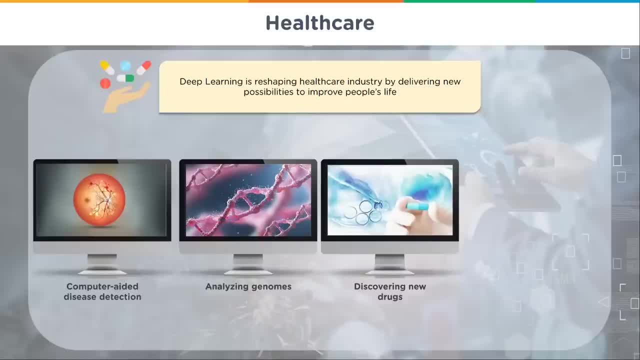 in the US but all across the world, and they range from exploring different plants and the opening up of, let's say, marijuana in the US and a number of cities are exploring that for medical use- to how do you reprogram t-cells in the human body to combat disease. there's whole industries. 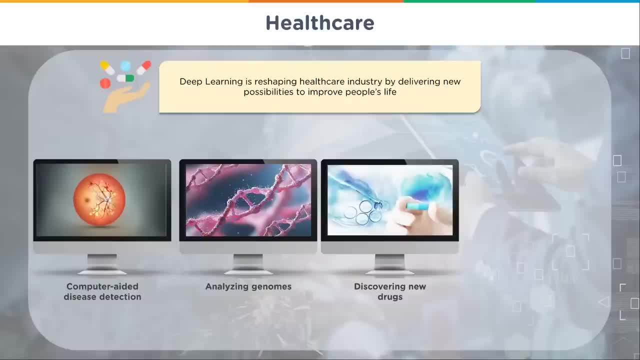 and data analysis. another one is chemistry. how do you use a chemical cell or a chemistry molecule, a chemical molecule to imitate the t-cell, so you can then put those molecules in there and then they grab the disease cells out, or the cancer cells or whatever out, just like the human body? 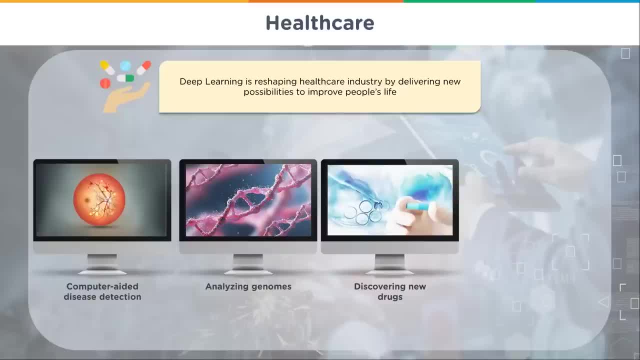 would so discovering new drugs and how to apply, that is just a huge industry. all these are huge industries. and medical imaging- we'll even take a glance closer at that. but being able to analyze, you know, you get your MRI, you get your CAT scans. the doctors can spend a long time looking at those. 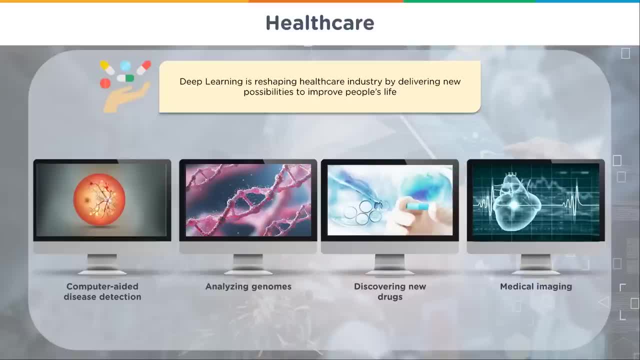 and taking careful measurements, and most of that's done by hand, but it's really important that you start applying deep learning. that deep learning can do a lot of that work. not only do it the same, but it'll be uniform from one hospital to the next, meaning that, as a 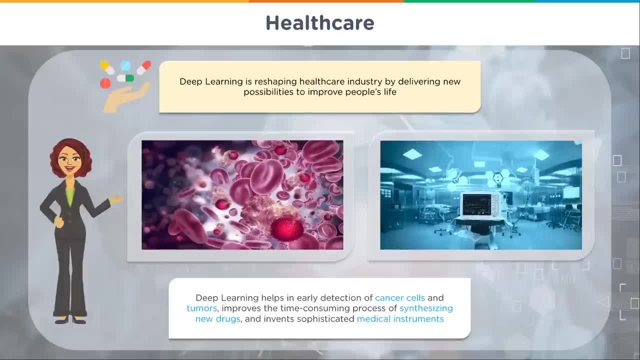 industry. it continues to progress and you get better results and better services. so deep learning is reshaping healthcare industry by delivering new possibilities to improve people's life, and deep learning helps in early detection of cancer cells and tumors, improves the time-consuming process of synthesizing new drugs and inverse sophisticated medical instruments. 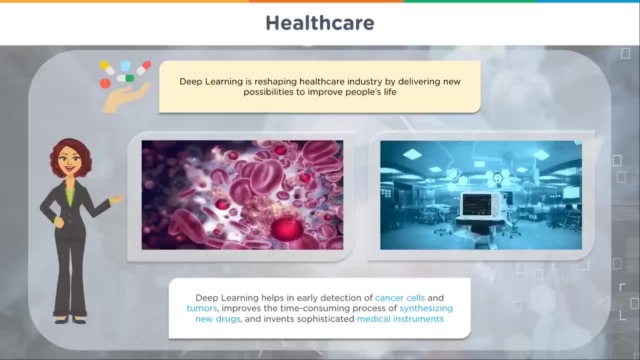 and not even sophisticated. they're using iPhones and deep learning to help with medical diagnosis. so it's at all levels. it's just amazing what they're doing in the healthcare industry with deep learning and they've just barely tapped what there's possible they're just now evolving into. 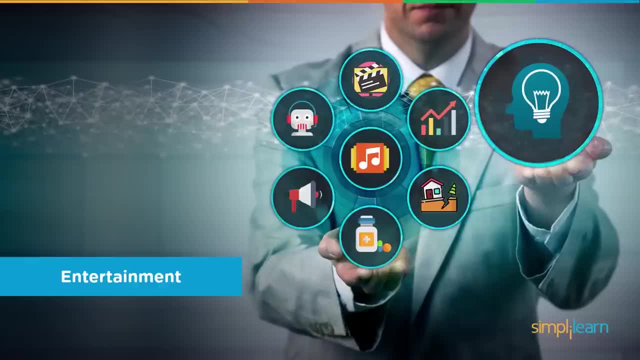 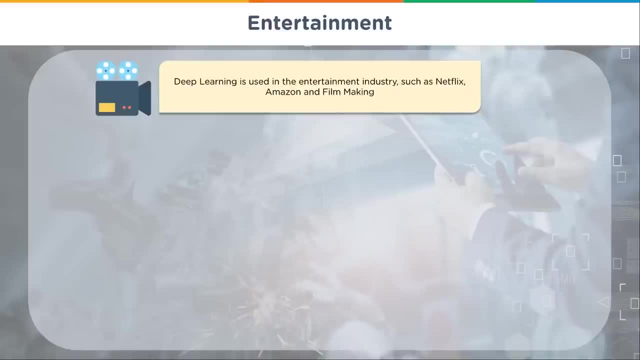 the beginning of this, where it's exploding out there. so entertainment, that's always a fun one. a lot of people go into the entertainment and deep learning because it's just fun. you know what's my favorite movie? all that fun stuff. deep learning is used in the entertainment industry. 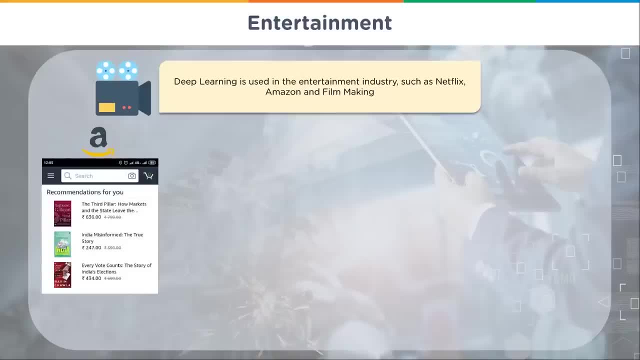 such as Netflix, Amazon and filmmaking and you have like your recommendations. that's probably the most common one you see and you can see here where they have India transform the true story. the third pillar, now markets in the state leave. so it comes up and says, hey, this is based on whoever. 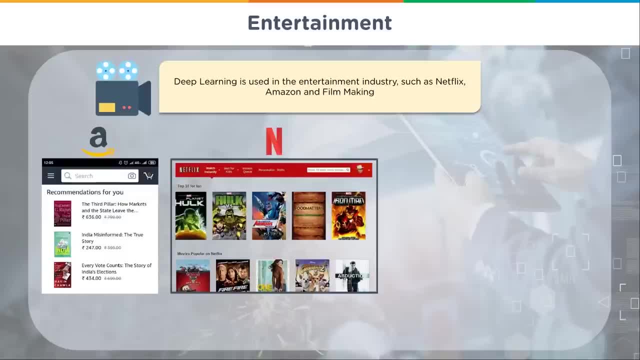 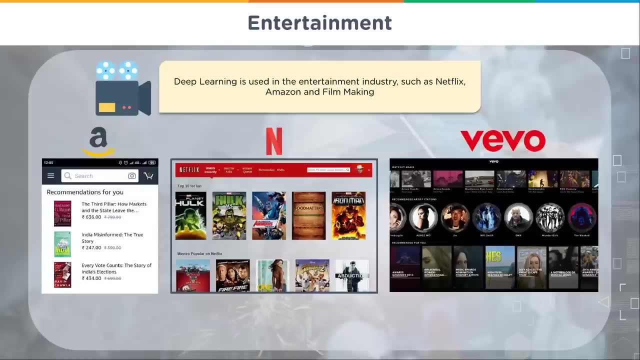 and of course, this is showing up on Amazon or Amazon Prime. Netflix does a good job of grouping movies for you and says: since you like these movies, you might like these movies over here. same thing with Vivo. it does that also. Amazon, Netflix and Vivo use recommender systems to provide. 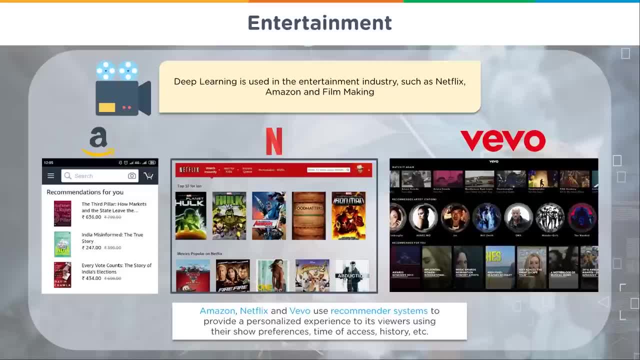 experience to its viewers using their show preferences, time of access, history, Etc. so really, this is one of the cool things is, instead of having to dig for the information, deep learning starts doing that for you. so instead of spending hours trying to figure out what you want to watch, 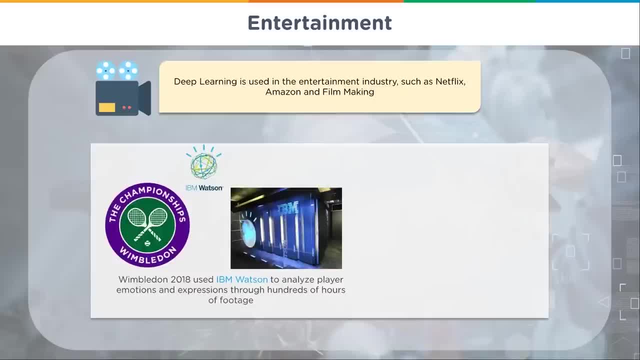 you can actually just enjoy the movies and have them come up. deep learning is used in the entertainment industry, such as Netflix, Amazon and filmmaking. continue on in deep learning. we have things like the IBM Watson. this is just really cool. I didn't know this till I read this till we. 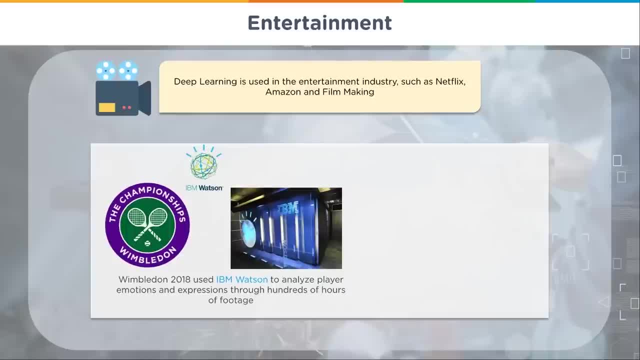 did this slide? Wimbledon 2018 used IBM Watson to analyze player emotions and expressions through hundreds of hours of footage and then it auto generated highlights for the telecast so you can imagine somebody sitting there looking through all the boring stuff. I want to look at the interesting stuff. it helps. 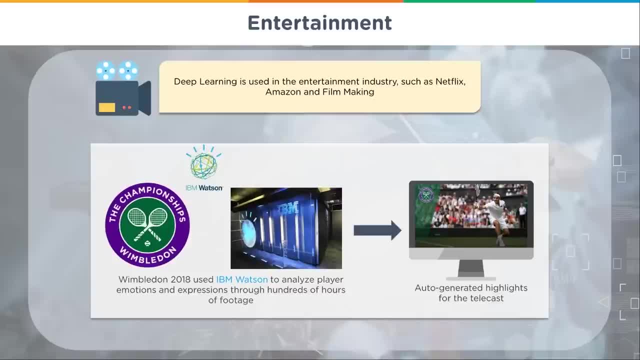 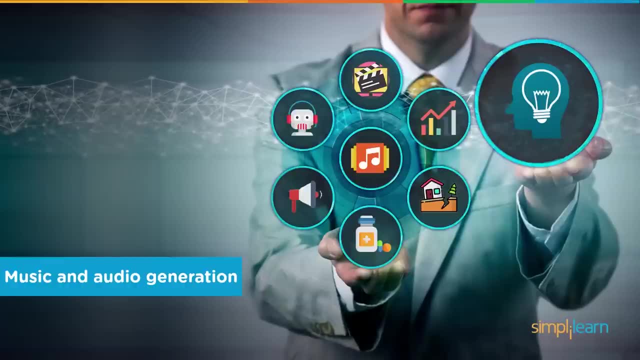 us sort that out again. you know, just like the Netflix and referral, it helps you find your choices without having to do all the heavy work of digging through really bad B rated movies and music and audio generation- another huge part of the industry- and this kind of blends right. 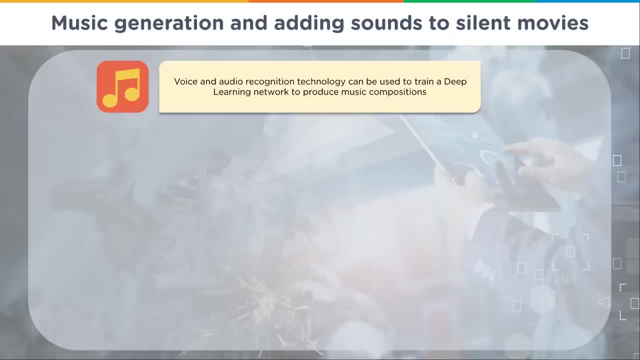 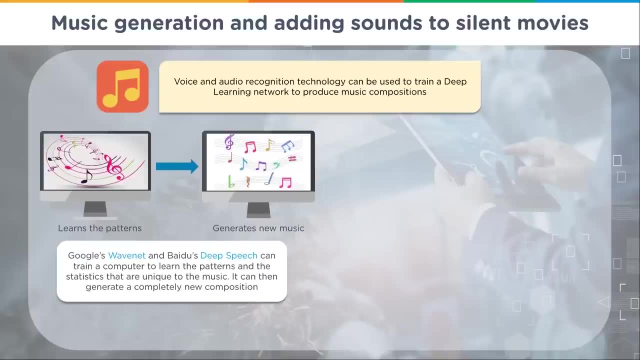 in with video and movie making. voice and audio recognition technology can be used to train deep learning Network to produce music compositions so it learns the patterns and generates new music. Google's WaveNet and Beidou's deep speech can train a computer to learn the patterns and the 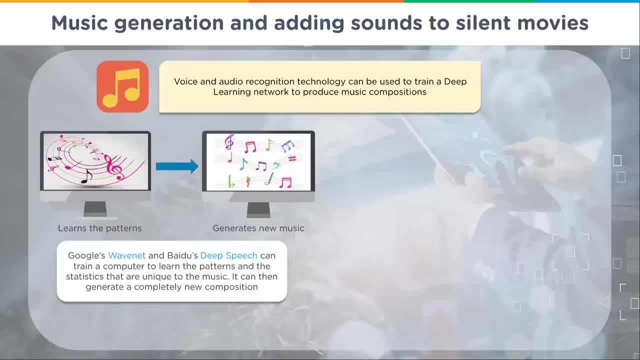 statistics that are unique to the music. it can then generate a complete new composition. that's a little scary. I always thought that creativity would always be the human factor, that we'd always have our creativity. but you know, computers can do some of that too, and then we have 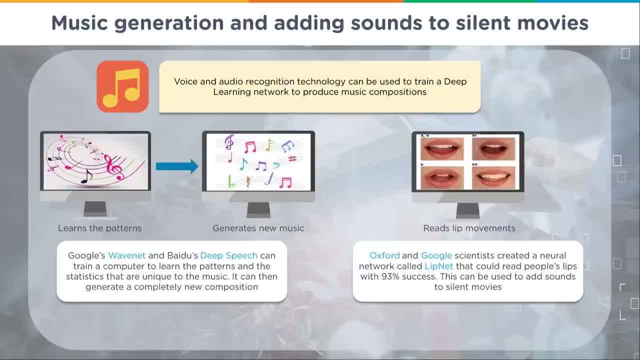 our reads, lip movements. Oxford and Google scientists created a neural network called lipnet that could read people's lips with 93 success. this can be used to add sounds to silent movies. I like that. it'd be fun to hear what they actually were saying back there. they probably said: 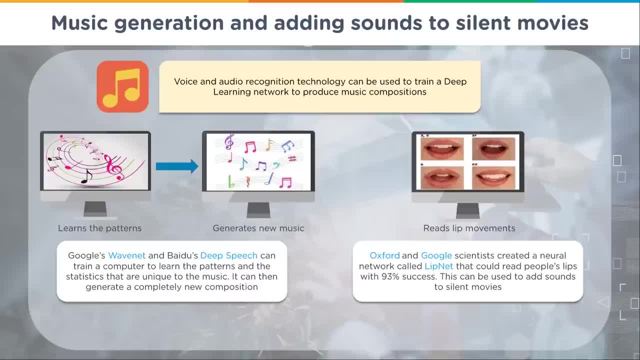 something totally different than what's actually on the movie. that'd be pretty funny. on the scary note, this would allow surveillance equipment to pull what people are saying, even if they're really far away, as long as they can see the lips. that's a little scary. coloring images and videos. 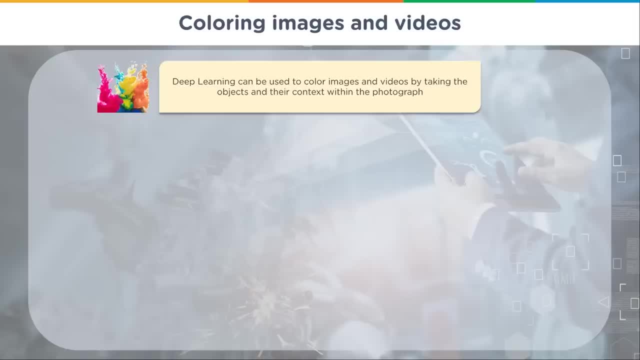 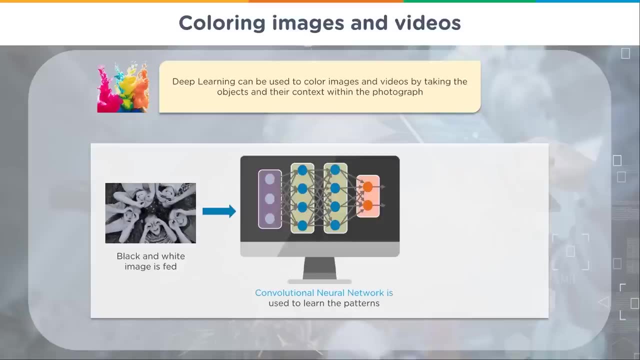 deep learning can be used to color images and videos by taking the objects and their context within the photograph. so you have your black and white image is fed in and you have a convolutional neural network is used to learn the patterns and usually you train it. you train it with hundreds of black and white photos that you 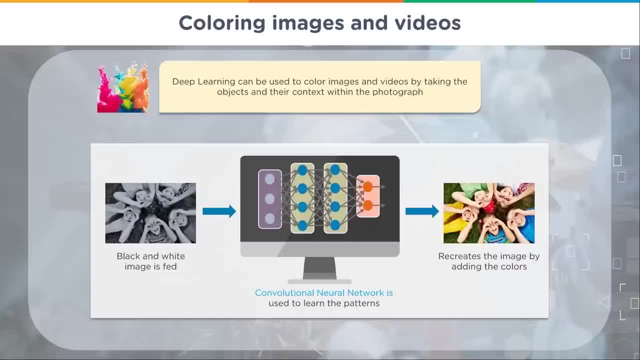 already have the color image for, so you know what to expect. and they take the new one and it recreates the image by adding the colors, and this is also used in the movie industry to add in special effects. there's all kinds of cool things they can do with this. it goes way beyond. 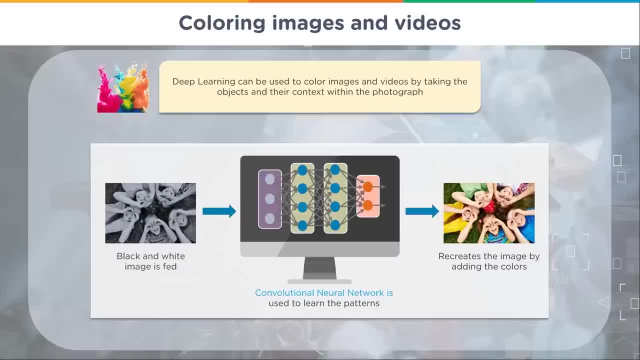 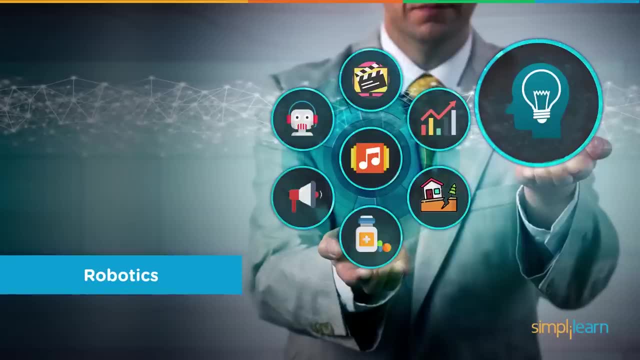 just coloring pictures. of course, the coloring pictures is something that you can probably do in your own lab on your own computer and build your own neural network to do that. robotics- one of my favorites robotics- all these tools that make them so exciting- is that you can go out and even now used to be. you'd have to spend four, five, six, ten. 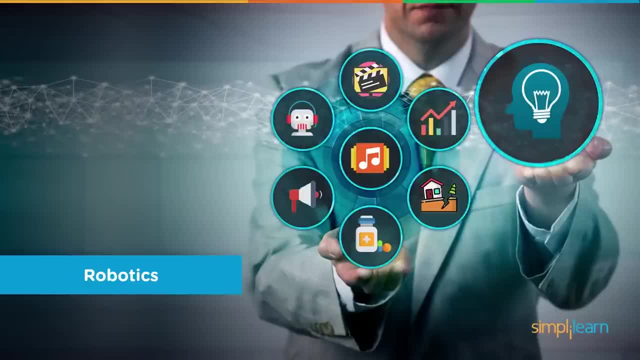 thousand US dollars to buy your own robot and then start programming it and doing neural networks. now it's around two thousand dollars and that continues to plummet. there's even kid robots- much cheaper- robotic hands- all of that that you can purchase and generate your own neural network and start trying to figure. 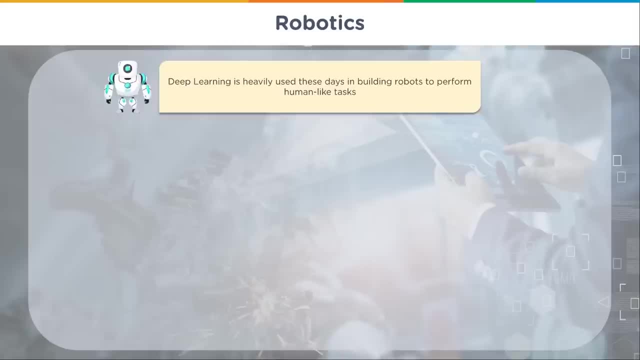 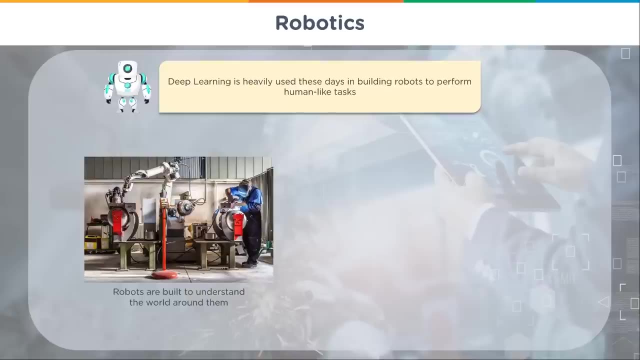 out how to get it to do things, and so we talk about deep learning. it's heavily used these days in building robots to perform human-like tasks. robots are built to understand the world around them- very important how to figure out what's what I remember. if you go back 20 years, they could not. 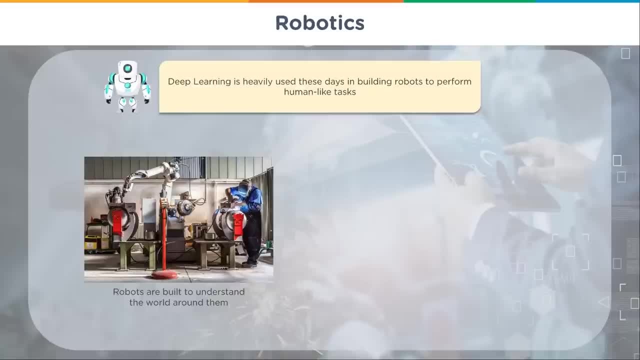 get a robot to figure out the difference between a Coke can and a pencil, because they're both cylinders and it. just they just had no idea how to do that back then. you know they did. the beginning of this- really the neural networks- was mid-90s, where it started, really taken off and the theory started. 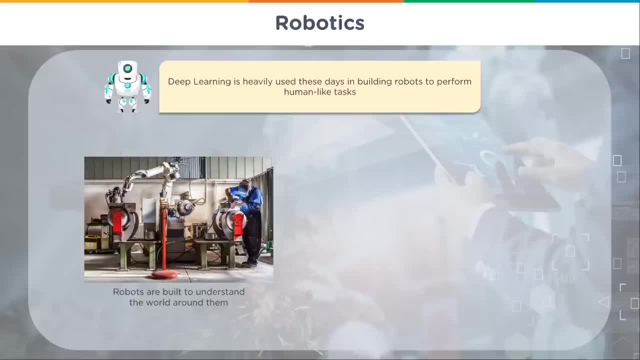 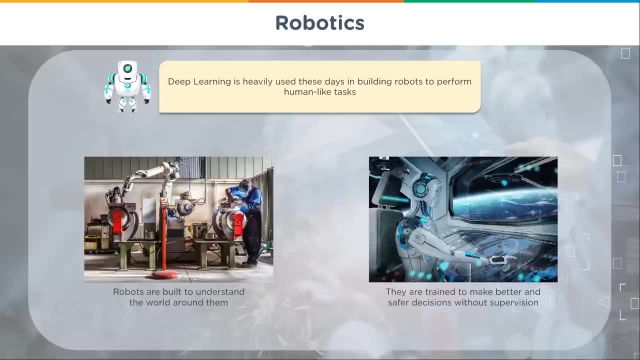 coming in, and so you go back to that time and figuring out those differences was almost impossible before then and they trained to make better and safer decisions without supervision, and you can see in this case, you know, in outer space, having a robot up there, uh, you know, the window blows out. 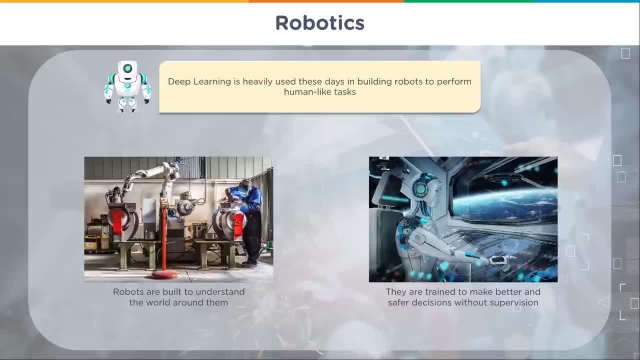 air pressure is lost. the robot is, you know, not going to be hurt by it, because they don't need air and oxygen and their decisions usually, instead of being like a human's tired- in this case, the robot never is tired. so you know, there's definitely a lot of tasks for a robot that can be used to. 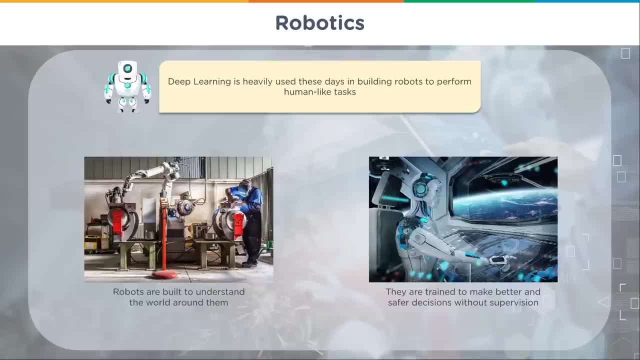 replace humans would be safer. think uh nuclear reactors that melted down after the tsunami in Japan. using robotics to go in there and clean up would be really important, instead of putting a person in a hazmat suit that might or might not protect him from the radiation in Boston Dynamics. 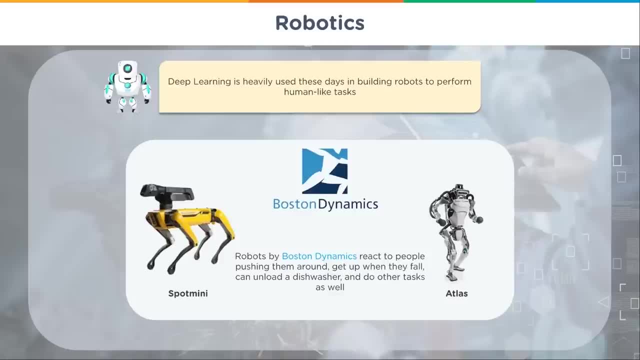 we have a spot mini. he's fun to watch if you ever pull up the video. or the Atlas robots by Boston Dynamics react to people pushing them around, get up when they fall, can unload a dishwasher and do other tasks as well. so we're starting to see this kind of robotics. 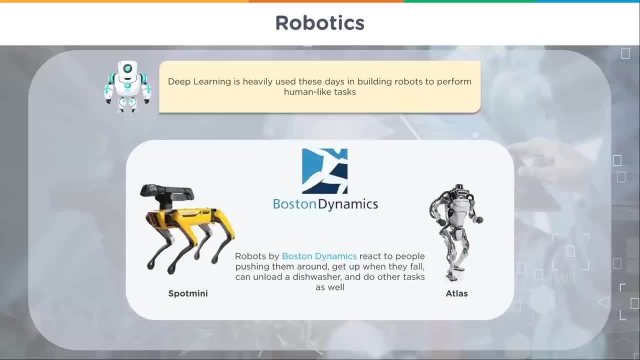 coming into the house. the Atlas obviously is a very expensive robot but there is certainly more common ones you can actually bring into the house. and then spot mini is fun to watch run. you can I forget how fast he goes, but he goes pretty fast. image caption generation another into part of. 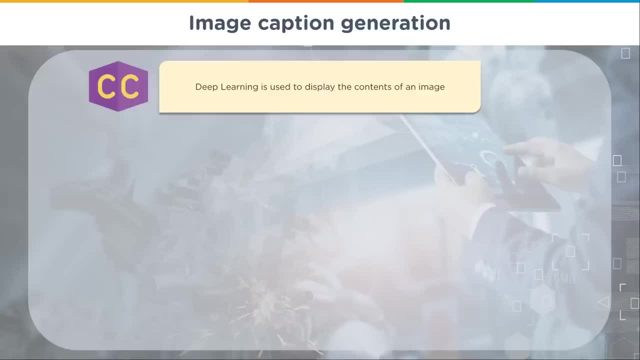 the industry in deep learning. deep learning is used to display the contents of an image. I love this with my Google photos. the system is trained with very large convolutional neural networks for detecting objects in the photographs. then a recurring neural network like an lstm is used to 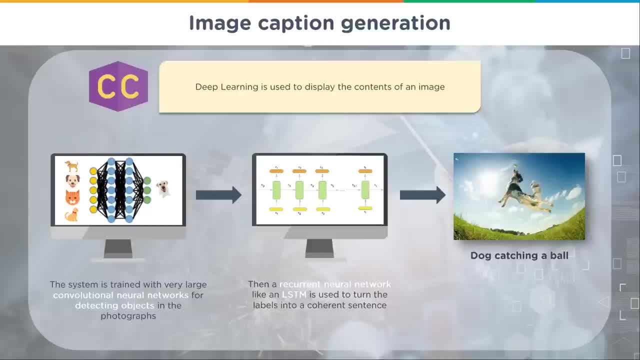 turn the labels into coherent sentence: dog catching a ball. so this is awesome. this is like you go into your Google photos and you say, hey, I want all the pictures of my dog, or I want all the pictures of kids or whatever it is, and they get to the point where you can now do, I want pictures where my dog 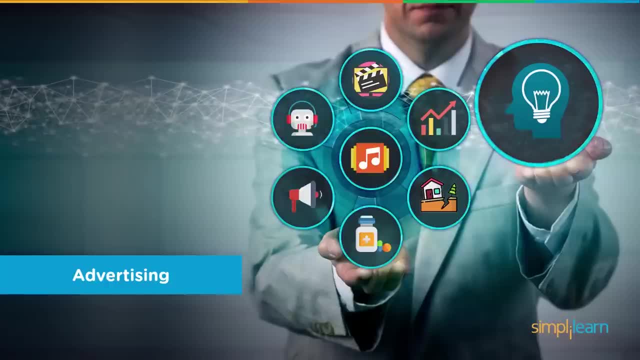 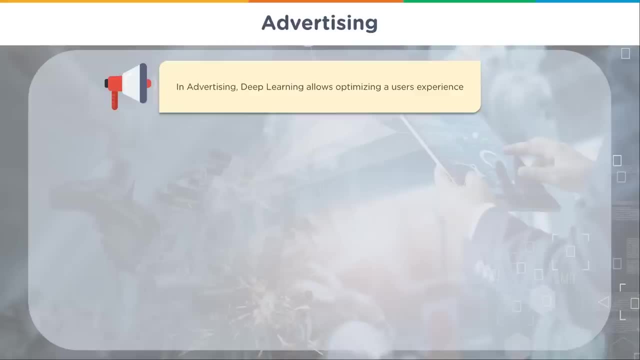 is catching the ball. advertising. one of the better paid fields in AI is in marketing and advertising, especially if you are working on bonuses and commissions, so advertising an advertising. deep learning allows optimizing a user's experience. so deep learning helps publishers and advertisers to increase the relevancy of the ads and boost the 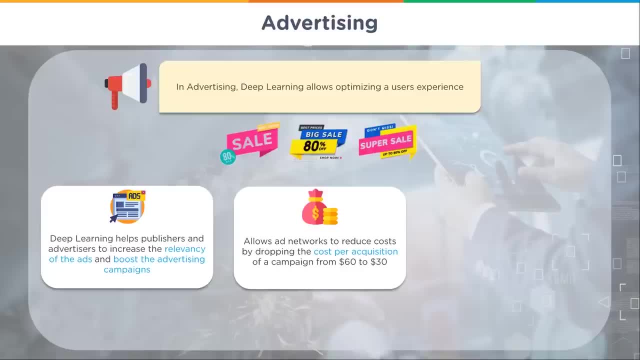 advertising campaigns. allows a network to reduce cost by dropping the cost per acquisition of a campaign from 60 to 30 dollars. create data-driven predictive advertising, real-time bidding of their ads and Target display advertising. and again, this goes from experimental where I'm just going to. 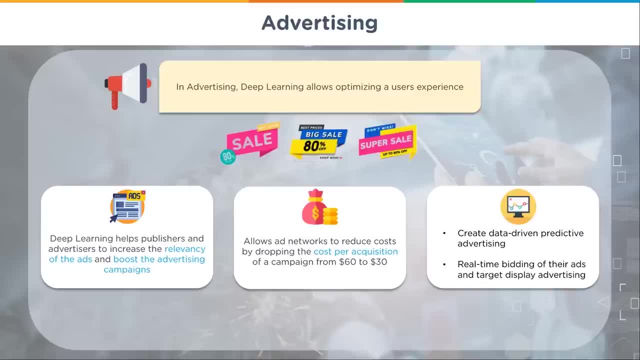 guess what people want and we'll put out a pink sign that says you want to add on widget to your order. well, nobody wants widgets and nobody wants to see the pink sign. maybe you got three people want to see the pink sign and you find out that the blue sign- a lot of people are reading that and they really want. 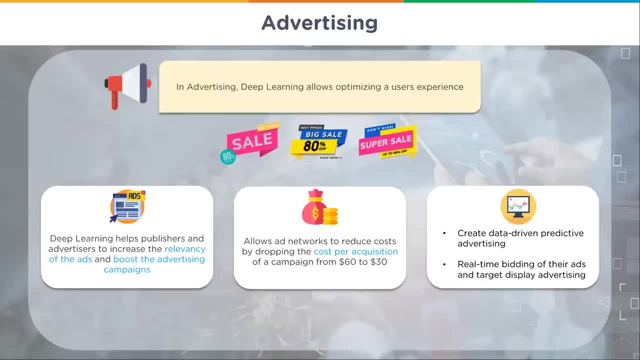 a widget number two, whatever that is. so when you talk about advertising, it also deals with marketing and also preference of merchandise. so it becomes really huge as far as what you're advertising and generating profit and sells for a company and that's across the board, whether you're. 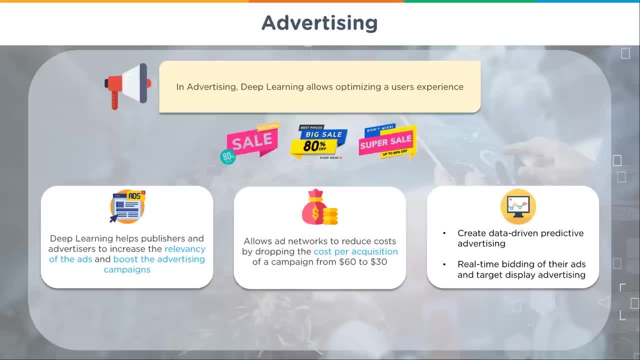 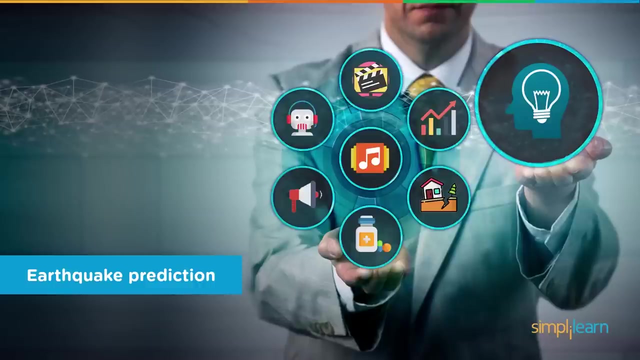 talking big real estate or property management and rentals, or Amazon uses this for all their. Now we're getting to something. uh, safety, human safety, you can also think weather predictions, all those fun things. deep learning model can be used to predict earthquakes by using a mass transfer model. 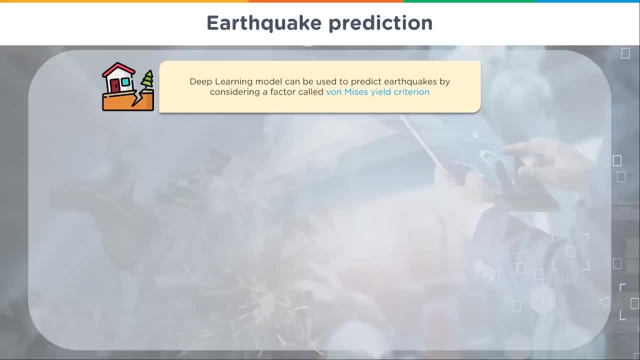 considering a factor called von Mises' yield criterion. Scientists at Harvard used deep learning to teach a computer to perform viscoelastic computations- that is quite the mouthful- which are used in prediction of earthquakes. This application helped to improve the earthquake calculation by 50,000 percent. That's amazing. We went from just guessing when an earthquake's. 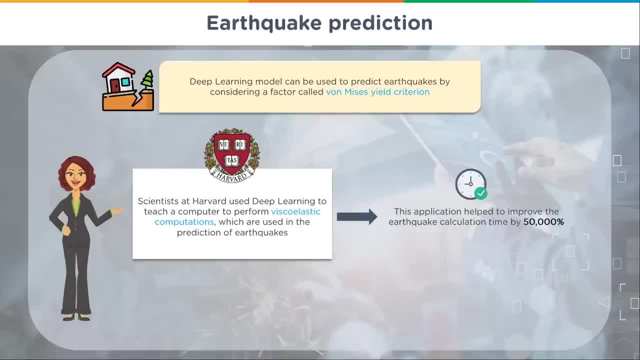 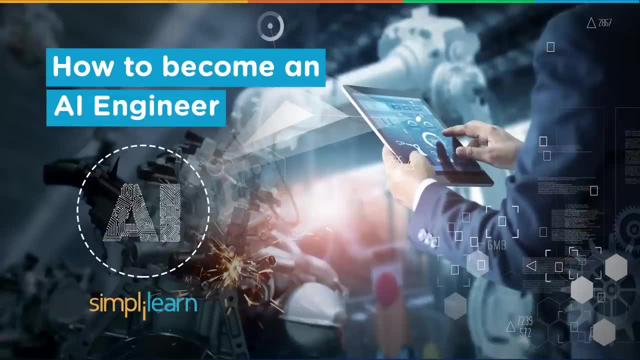 going to happen where we have almost no reliability to being able to have a decent guess as when the earthquakes are going to hit. That's pretty impressive. Hi guys, I'm Rahul from Simply Learn, and today I'm going to tell you how you can become an AI. 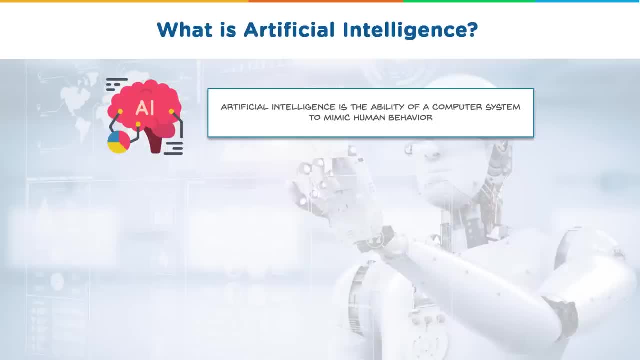 engineer. So, first off, let's ask the important question: what is artificial intelligence? Now, artificial intelligence is the ability of a computer system to mimic human behavior. Now, this is the sort of intelligence that's demonstrated by machines, and this is in. 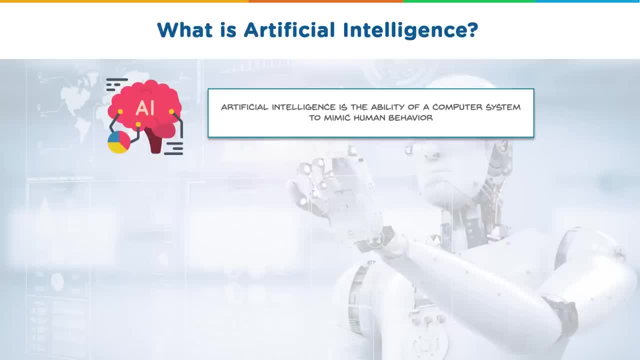 contrast to natural intelligence that's shown by humans as well as animals. So how does artificial intelligence work? Firstly, it learns from pathogens. Now, whatever machines that are artificially intelligent learn from their actions, which are positive or negative. Now, with this new information, the machine is able to make corrections. 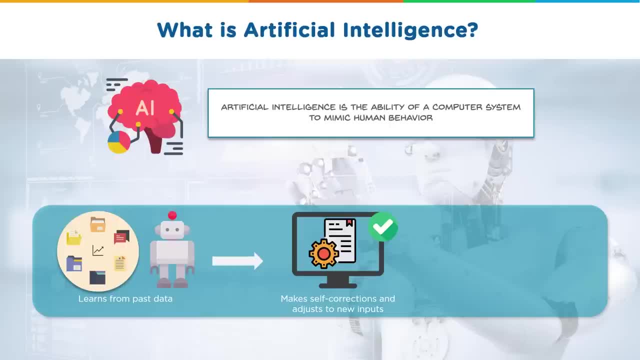 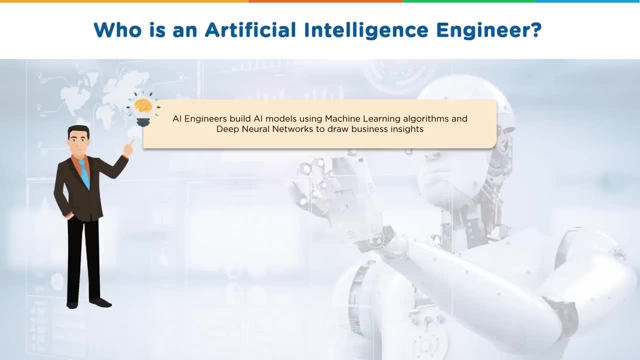 to itself so that these problems don't resurface, and make some adjustments to handle new inputs. And finally, the machine is able to perform human-like tasks. So who is an artificial intelligence engineer? An AI engineer builds AI models using machine learning algorithms and deep learning neural networks to draw business insights. Now these insights can be used to make business. 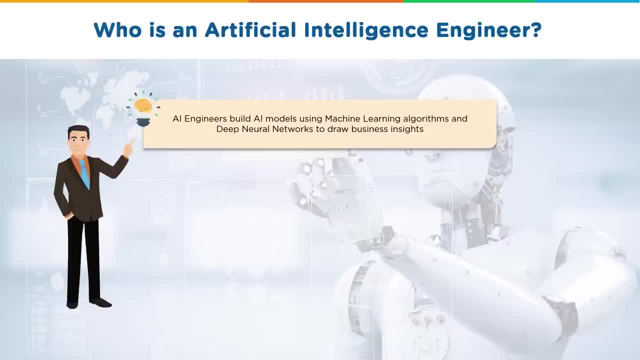 decisions that affect the entire organization. Not to mention, they also create weak or strong AIs, depending on what goal they want to achieve. Now, AI engineers have a sound understanding of programming, software engineering as well as data science. They use different tools and techniques. 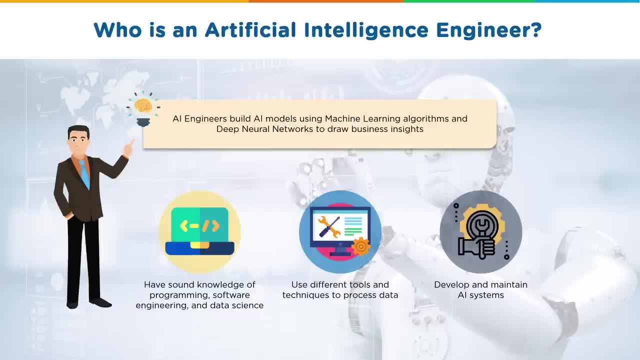 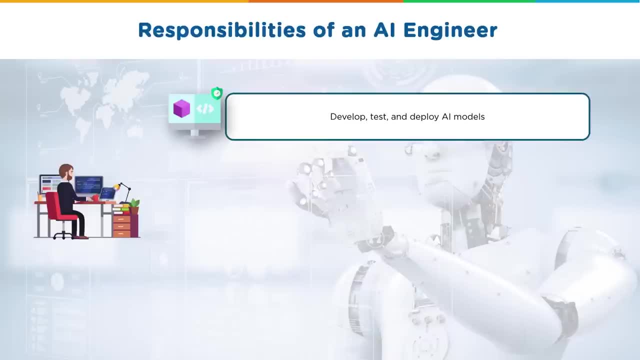 so that they can process data and they develop, as well as maintain, AI systems. Now let's talk about the responsibilities of an AI engineer. Firstly, they need to develop, test and deploy AI models. This can be done through a number of different programming algorithms, like random. 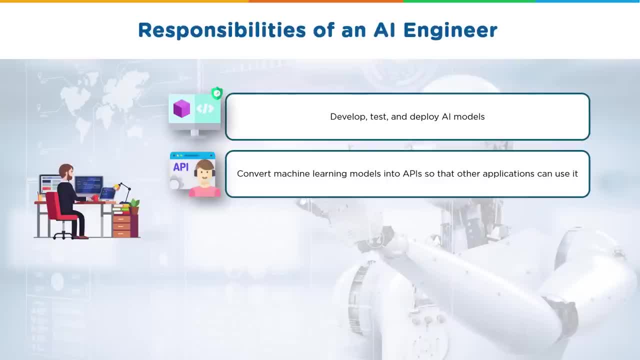 logistic regression, linear regression and so on. They need to be able to convert the machine learning models into APIs or application program interfaces so that other applications can use it. They're responsible for building AI models from scratch and help the different components of the organization, such as product managers and stakeholders, understand what 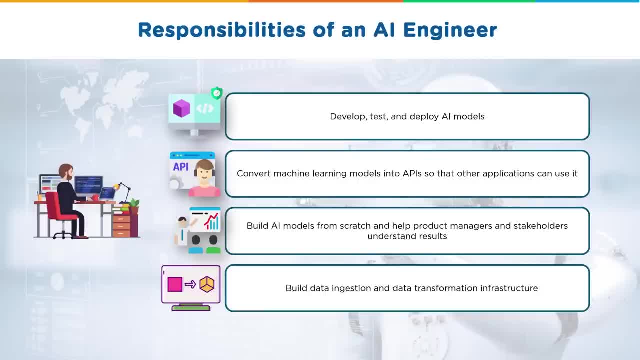 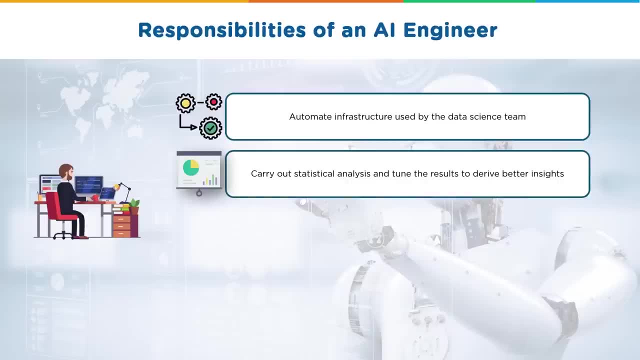 they stand to gain from the model. They need to build data ingestion and data transformation infrastructure. They need to automate infrastructure that's used by the data science team. They need to be able to perform statistical analysis And tune the results so that the organization can take better informed decisions. They need 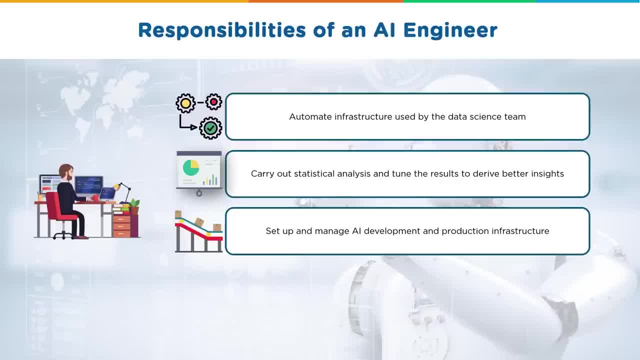 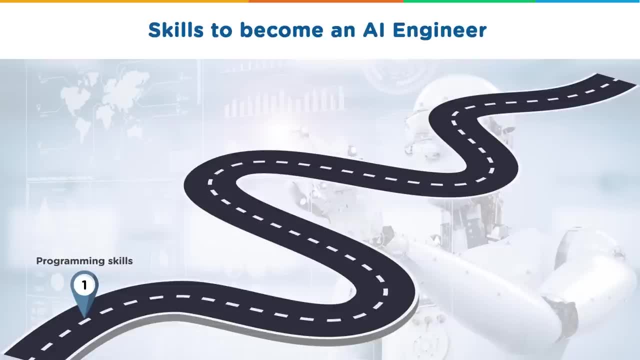 to set up, as well as manage, AI development and product infrastructure, And they need to be good at teamwork, since they'll be coordinating work with teams of data as well as business analysts. Next up, let's talk about the skills required to become an AI engineer. First off. 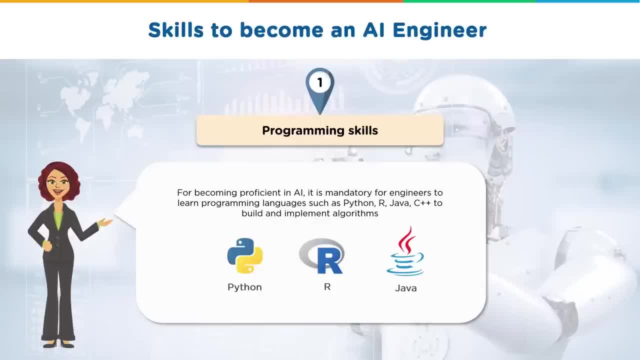 programming skills Now. the first skill required to become an AI engineer is programming skills Now. for you to become well versed in AI, it is very important that you start learning programming languages such as Python, R and Python Now. the first skill required to become 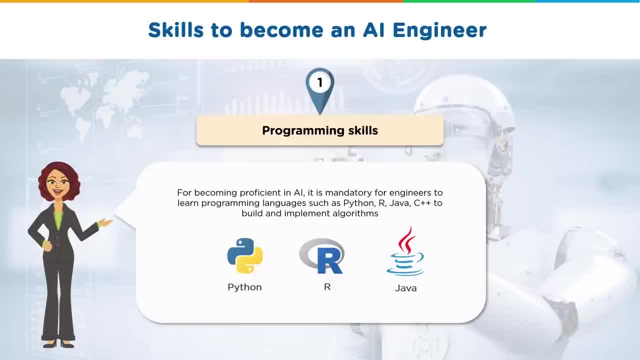 an AI engineer is programming skills. Now, for you to become well versed in AI, it is very important that you start learning Python, R, Java and C++ so that you're able to build as well as implement. So that you'll be able to build as well as implement models. The 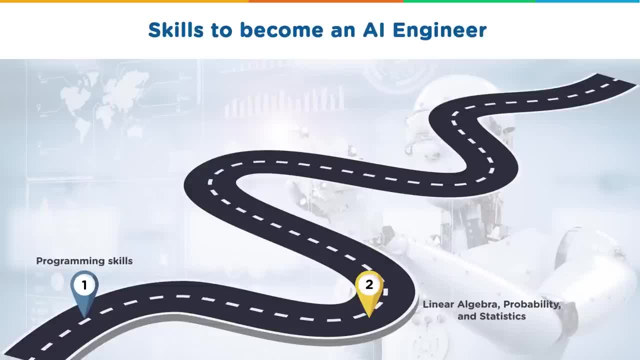 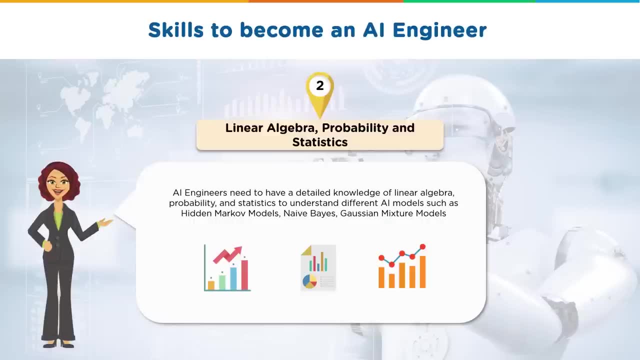 second skill required is linear algebra, probability and statistics. Now, to understand as well as implement different AI models, such as Hidden Markov Models, Naive Bayes, Gaussian Mixture Models, Linear Discriminant Analysis, and so on, you need to have detailed knowledge. 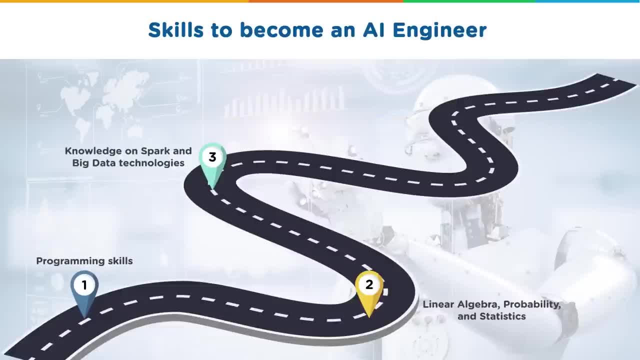 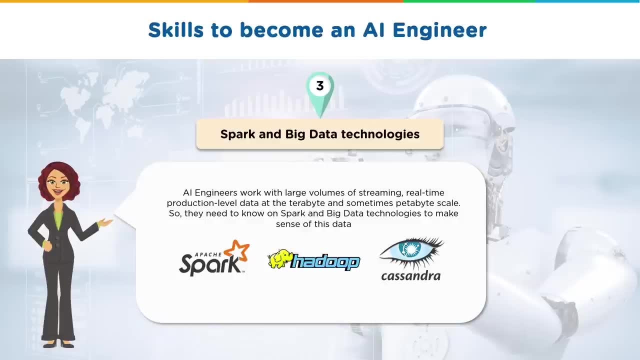 of linear algebra, probability and statistics. The third skill required is knowledge about Spark and Big Data technologies. Now, since AI engineers work with large volumes of data, which could be streaming or real-time production-level data, production-level data in terabytes or even petabytes, they need 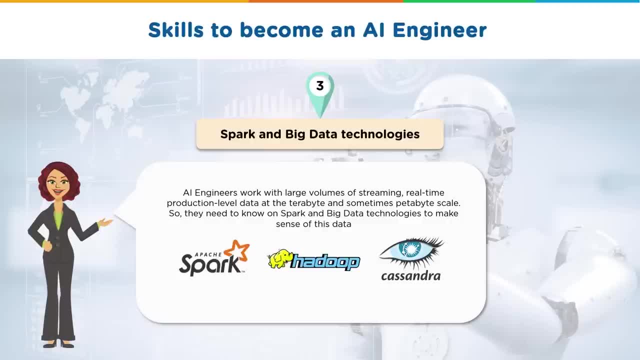 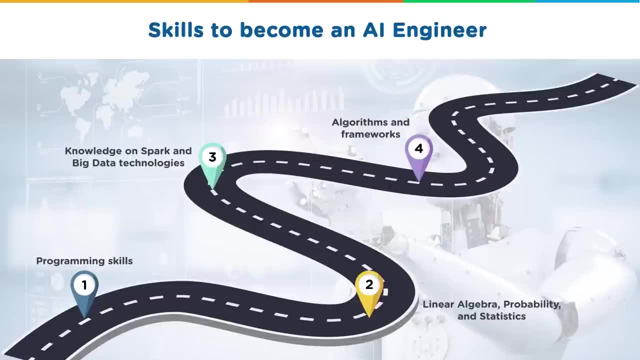 to know about Spark and other Big Data technologies. to make sense of this, Along with Apache, Spark, you could also use other Big Data technologies like Hadoop, Cassandra and MongoDB. The next skill that you require is to be well versed with algorithms and frameworks. 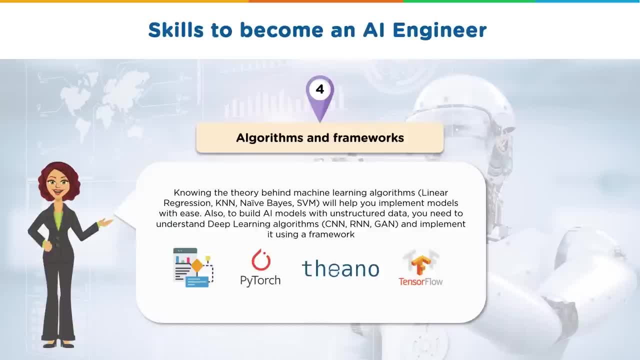 Now understanding how machine learning algorithms like linear regression, KNN, Naive Bayes, SVNM and so on can be applied to programming and programming. Now for you to become well versed. SVM and others work will help you implement machine learning models with ease. 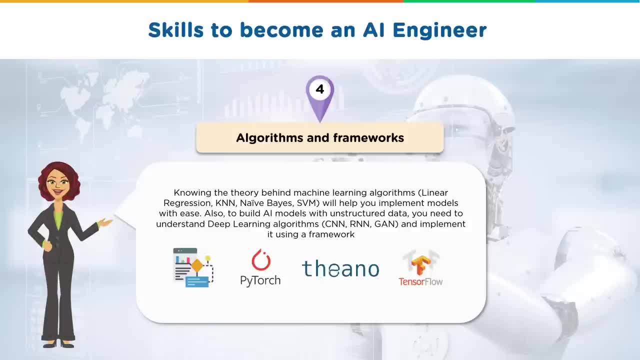 Also, to build AI models with unstructured data, you need to understand deep learning algorithms like CNN, which is the Convolutional Neural Network, RNN, which is the Recurrent Neural Network, and GAN, which is the Generative Adversarial Network, so that you can implement. 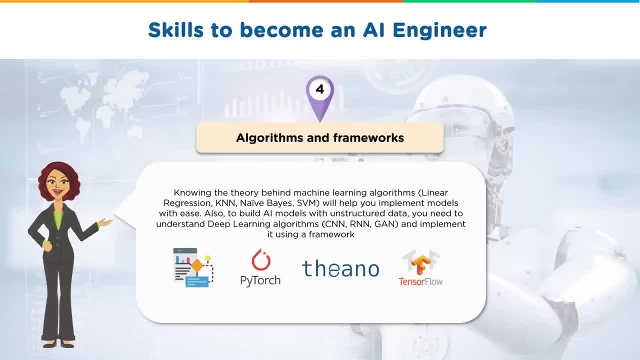 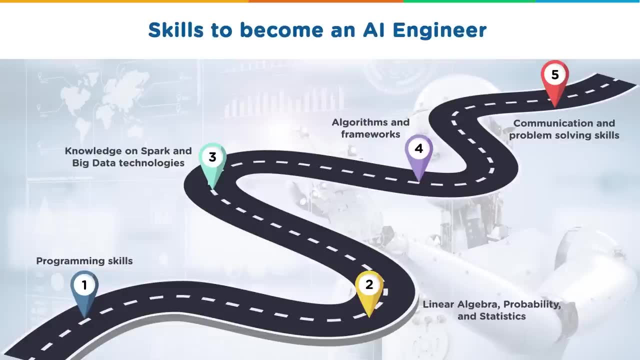 it using a framework. Some of the frameworks used in artificial intelligence are PyTorch, Theano, TensorFlow and Caffe. The final skill required to become an AI engineer is communication and problem solving skills. Now you need to be very good at communication so that you are able to pitch your product. 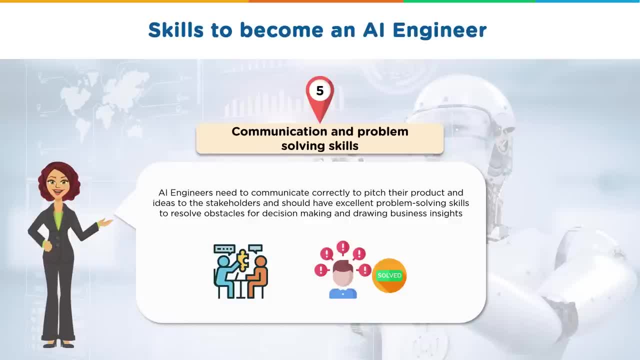 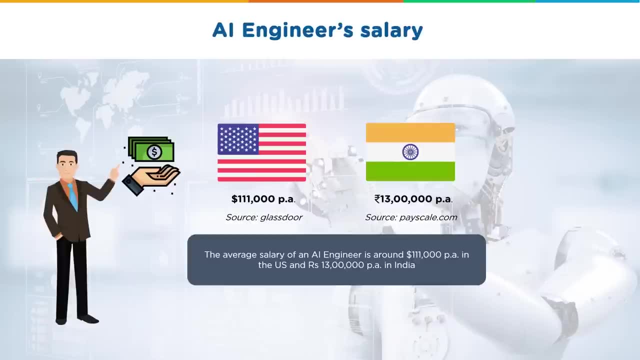 and idea to the stakeholders. You should also have excellent problem solving skills to resolve obstacles for decision making and draw helpful business insights. Now let's talk about an AI engineer's salary. The average salary of an AI engineer is $111,000 per annum in the United States and Rs 13. 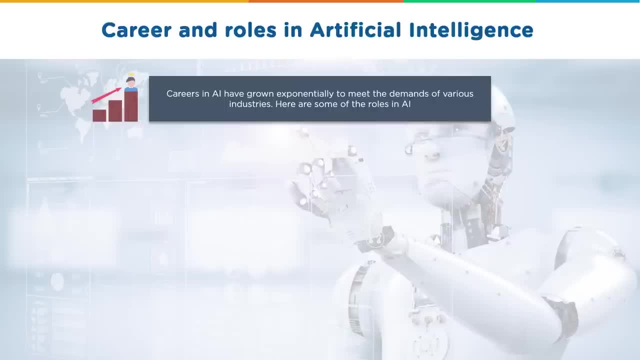 lakhs per annum in India. Now let's talk about the career and roles in artificial intelligence. Since several industries around the world use AI to some degree or the other, there has been an exponential growth in the career opportunities within the field of AI. 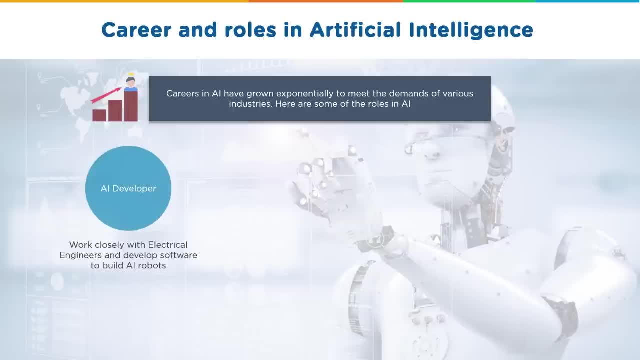 Let's have a look at some of these job roles. First off, we have AI Developer. Now these individuals work closely with electrical engineers and develop software to create artificially intelligent robots. Next up, we have AI Architect. Now these people work closely with clients so that they can provide business as well. 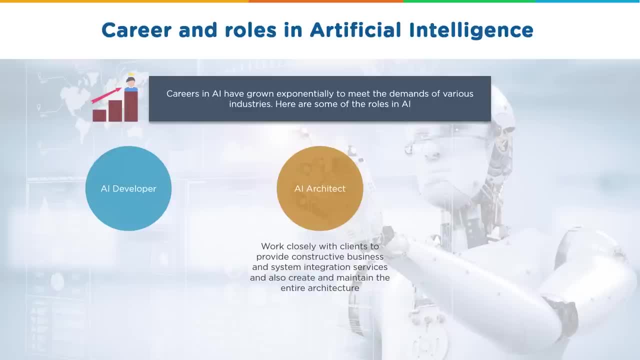 as system integration services, while at the same time creating and maintaining the industry. Next up, we have AI Architect Now. these individuals build predictive models using vast volumes of data, have in-depth knowledge of machine learning algorithms, deep learning algorithms and deep learning frameworks. 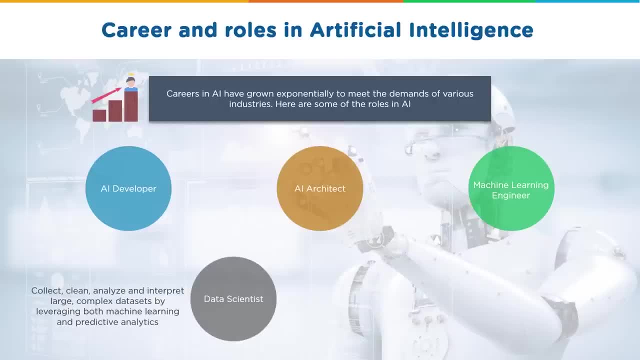 Next up, we have Data Scientists. Now, data scientists collect, clean, analyze and interpret large and complex datasets by leveraging both machine learning and predictive analytics. And finally, we have BI Developer, or Business Intelligence Developer. They are responsible for designing, modeling and analyzing complex data to identify business. 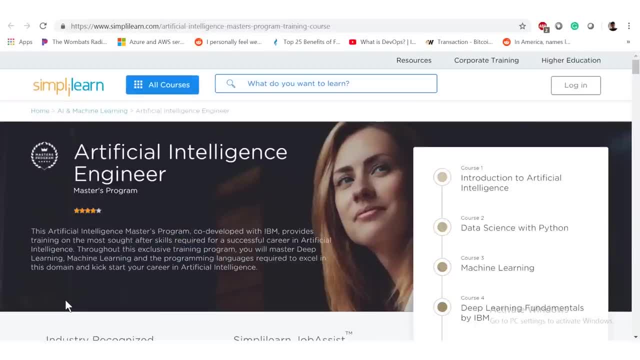 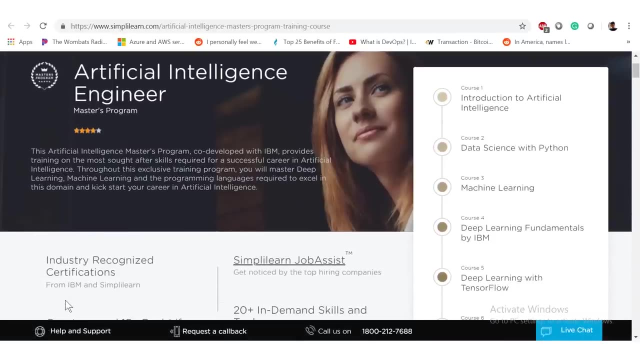 as well as market trends. So how can SimpliLearn help you? SimpliLearn has now tied up with IBM and is offering the AI Engineer's Master's Program. This program consists of a number of different courses, such as Introduction to Artificial Intelligence, Data Science with Python, Machine Learning, Deep Learning, Fundamentals by IBM. 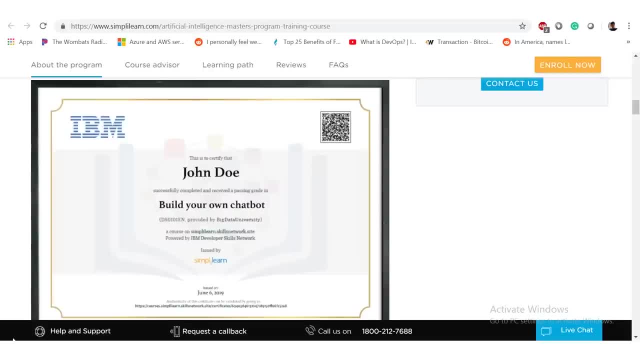 Deep Learning with TensorFlow and the AI Capstone Project. After completing this course, you'll get a second chance to learn more about AI. You'll get a certificate from both IBM as well as SimpliLearn, which is recognized across the world. IBM is the second largest predictive analysis and machine learning solutions provider globally. 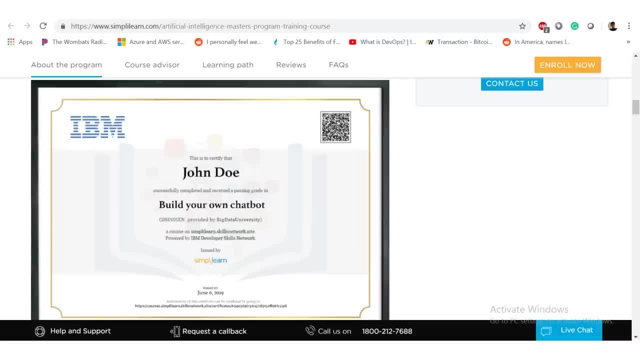 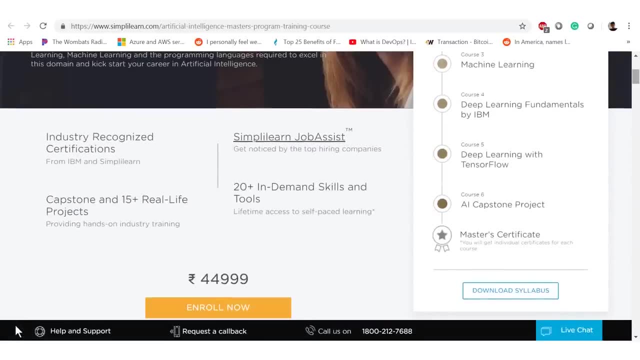 A joint partnership with SimpliLearn and IBM introduces you to integrated blended learning and making you an expert in artificial intelligence and data science. The program, co-developed with IBM, will make you industry ready for artificial intelligence as well as data science job roles. As a benefit, you get SimpliLearn Job Assist. 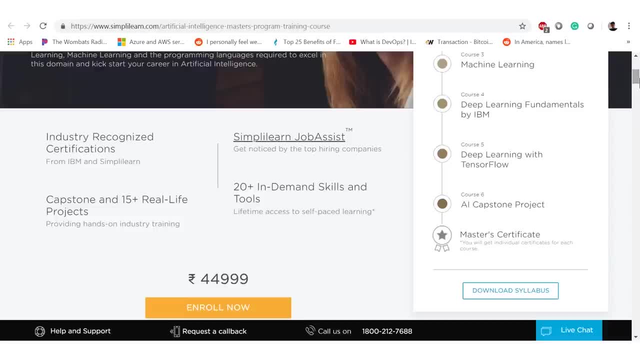 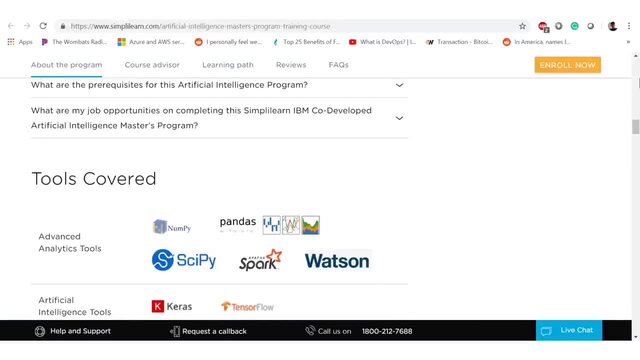 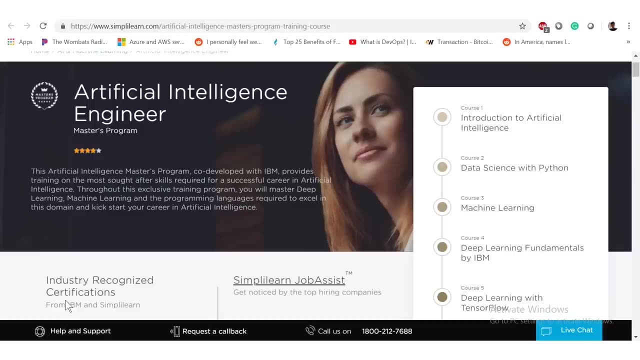 You perform Capstone and 15-plus real-life projects and assistance with 20-plus in-demand skills and tools, Tools such as NumPy, SciPy, Apache, Spark, Watson, Keras, Python, R and much more. You also have certain other benefits, such as access to exclusive forums which are moderated. 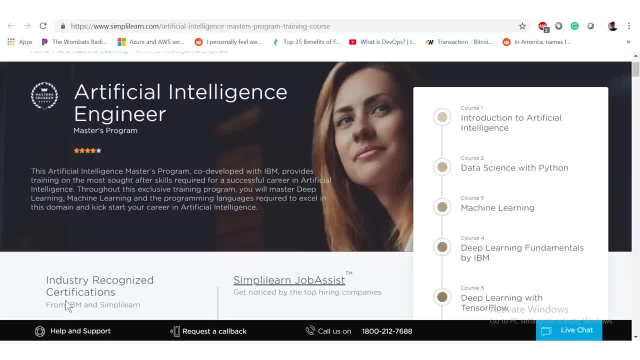 by expert, faculty and industry thought leaders. $1200 worth of IBM Cloud credits that you can leverage for hands-on exposure. access to IBM Cloud platforms such as IBM Watson, which is IBM's own supercomputer, and other software for 24-7 practice. access to digital. 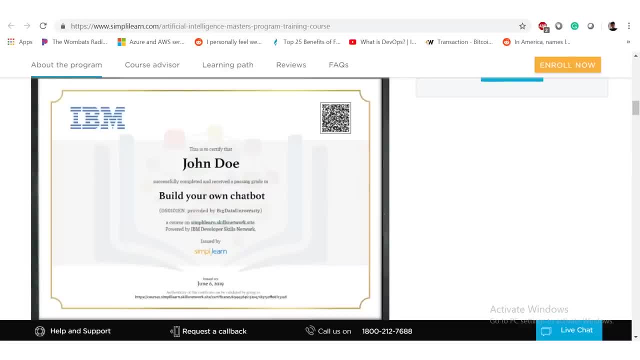 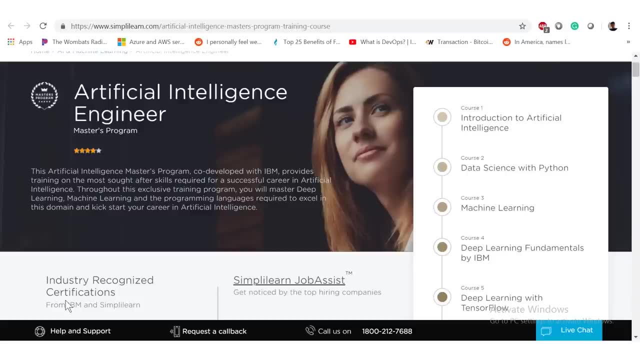 badges from IBM and, of course, the industry recognized Master Certificate from SimpliLearn. So if your dream is to become an AI engineer, I suggest you go on to SimpliLearncom and get started on your journey to getting certified and getting ahead. 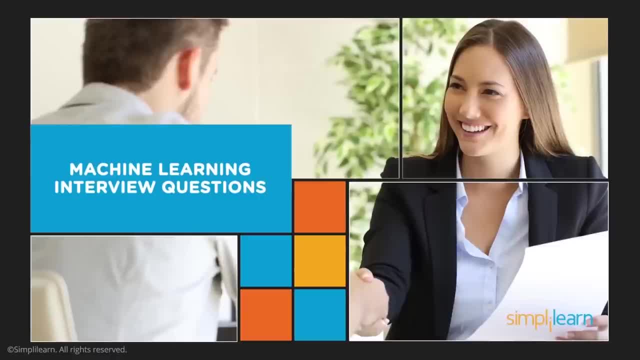 Hello everyone, welcome to this session. I'm Mohan from SimpliLearn, and today we'll talk about interview questions for machine learning. Now, Interviews can probably help you when you're attending interviews or machine learning positions, and the attempt here is to probably consolidate 30 most commonly asked questions and to help 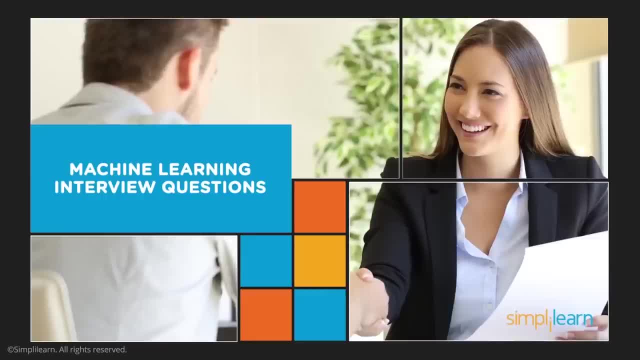 you in answering these questions. We tried our best to give you the best possible answers but of course what is more important here is rather than the theoretical knowledge you need to kind of add to the answers or supplement your answers with your own experience. 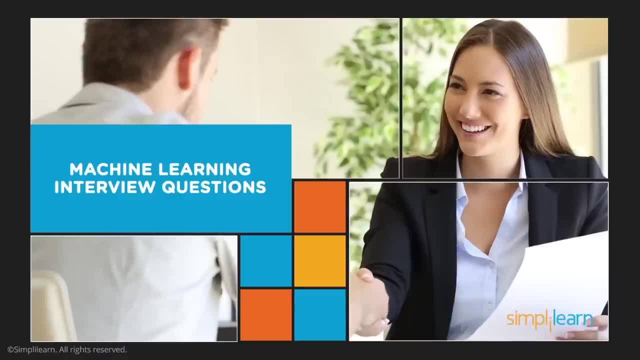 So the responses that we put here are a bit more generic in nature, so that if there are some concepts that you are not clear, this video will help you in kind of getting those concepts cleared up as well. But what is more important is that you need to supplement these responses with your own. 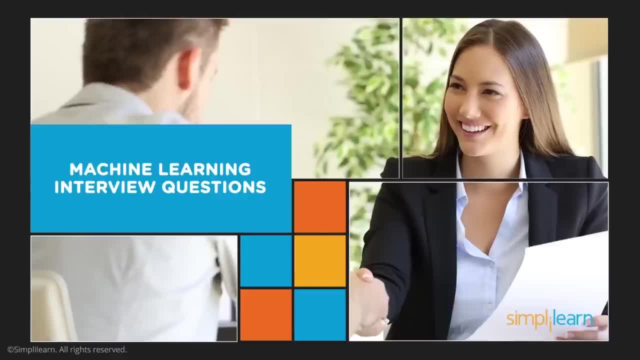 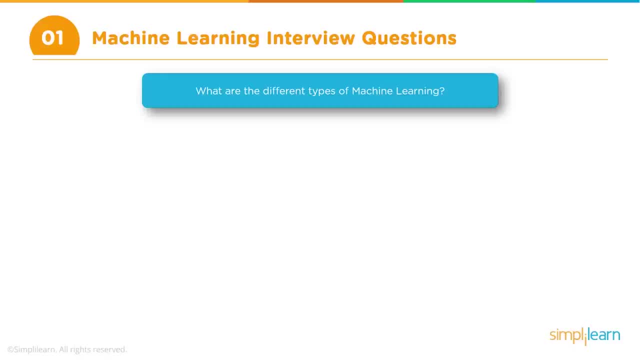 practical experience. Okay, So with that, let's get started. So The first question that you may face is: what are the different types of machine learning? Now, what is the best way to respond to this? There are three types of machine learning. 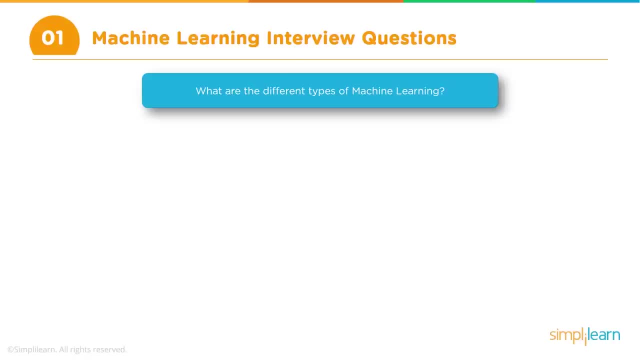 You read any material, you will always be told there are three types of machine learning. but what is important is you would probably be better off emphasizing that there are actually two main types of machine learning, which is supervised and unsupervised. And then there is a third type, which is reinforcement learning. 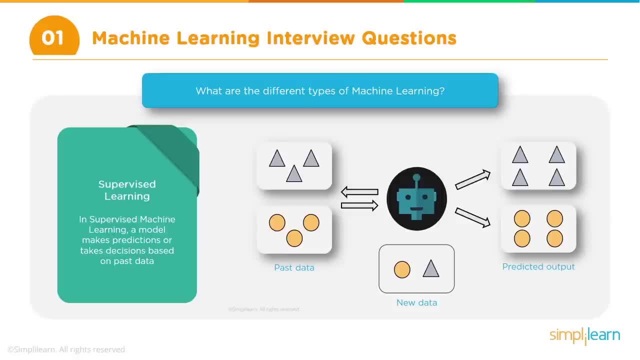 So supervised learning is Okay. This is where you have some historical data and then you feed that data to your model to learn. Now you need to be aware of a key word that they will be looking for, which is labeled data Right. 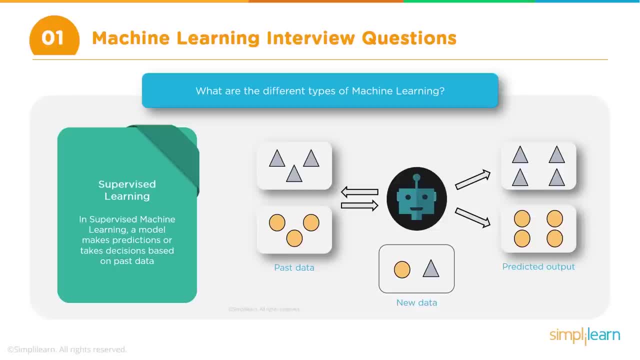 So if you just say past data or historical data, the impact may not be so much. you need to emphasize on labeled data. So what is labeled data Basically? let's say, if you're trying to do train your model for classification, you need 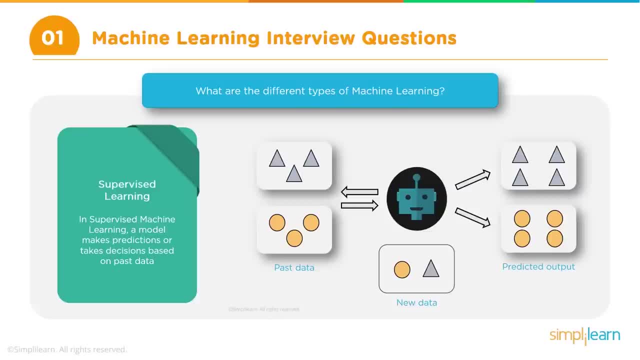 to be Aware of, for your existing data, which class each of the observations belong to right. So that is what is labeling. So it is nothing but a fancy name. you must be aware. But just make it a point to throw in that keyword labeled. 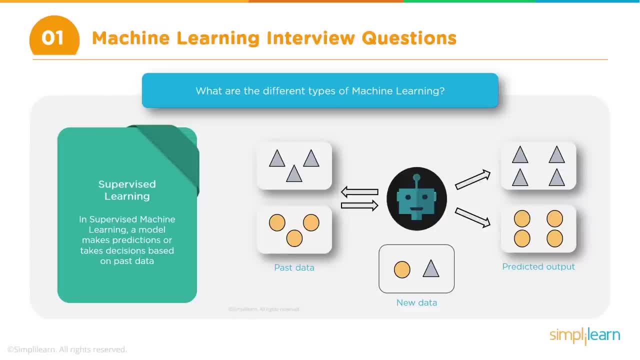 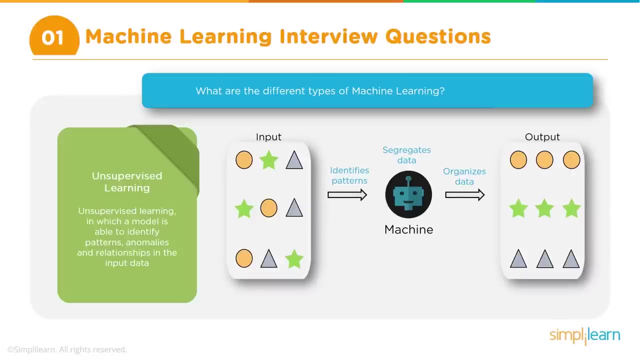 So that will have the right impact. Okay, So that is what is supervised learning: when you have existing labeled data which you then use to train your model. that is known as supervised learning, And unsupervised learning is When you don't have this labeled data. 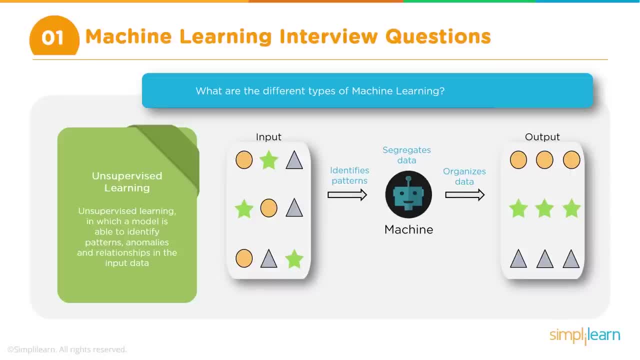 So you have data, it is not labeled, So the system has to figure out a way to do some analysis on this. Okay, So that is unsupervised learning, And you can then add a few things like: what are the ways of performing supervised learning? 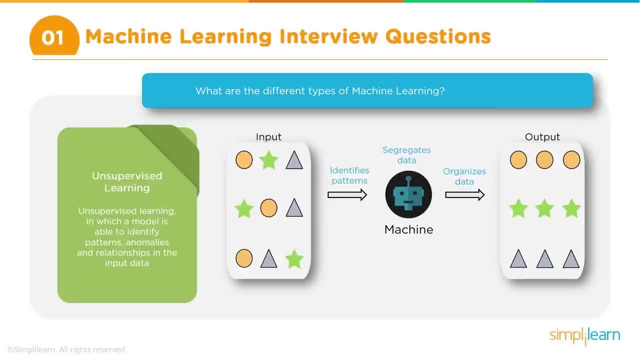 and unsupervised learning, or what are some of the techniques? So, supervised learning, we perform, or we do regression and classification. and unsupervised learning, We do clustering. Okay, So clustering can be of different types. Similarly, regression can be of different types, but you don't have to probably elaborate. 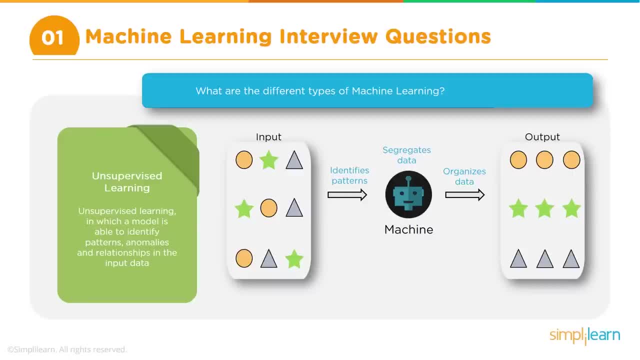 so much. If they are asking for just the different types, you can just mention these, and just at a very high level. But if they want you to elaborate, give examples, then of course I think there is a different question for that. 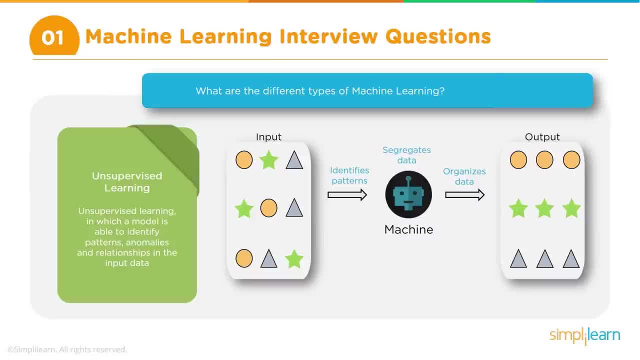 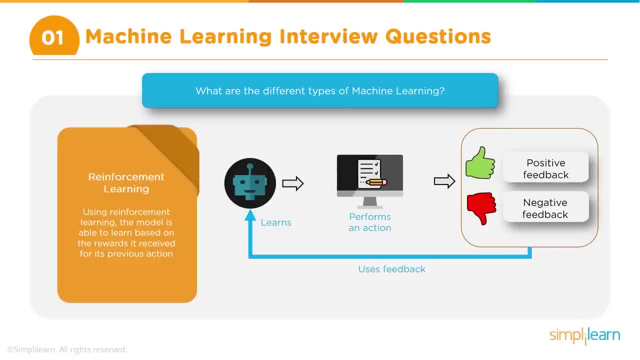 We will see that later. Then the third: So we have supervised, then we have unsupervised, and then reinforcement. You need to provide a little bit of information around that as well, because it is sometimes a little difficult to Come up with a good definition for reinforcement learning. 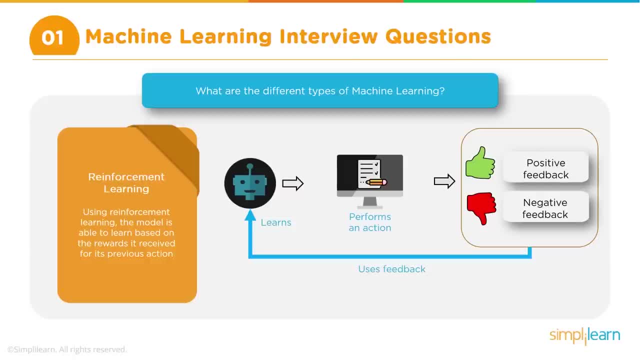 So you may have to a little bit elaborate on how reinforcement learning works, right? So reinforcement learning works in such a way that it basically has two parts to it. One is the agent and the environment, and the agent basically is working inside of this. 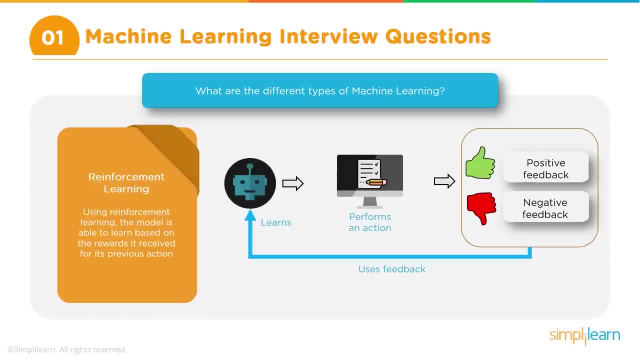 environment and it is given a target that it has to achieve And every time it is moving in the direction of the target. so the agent basically has to take Some action And every time it takes an action which is moving the agent towards the target right. 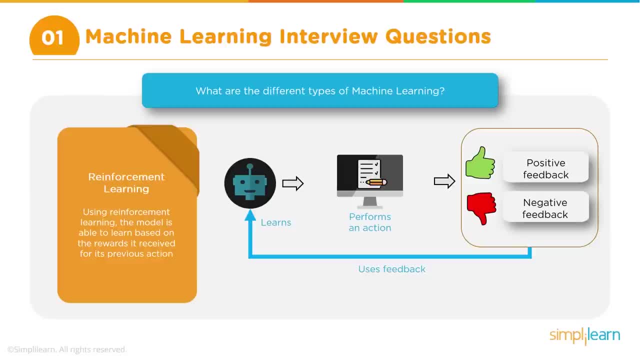 Towards a goal- a target is nothing but a goal- Then it is rewarded, And every time it is going in a direction where it is away from the goal, then it is punished. So that is the way you can a little bit explain. 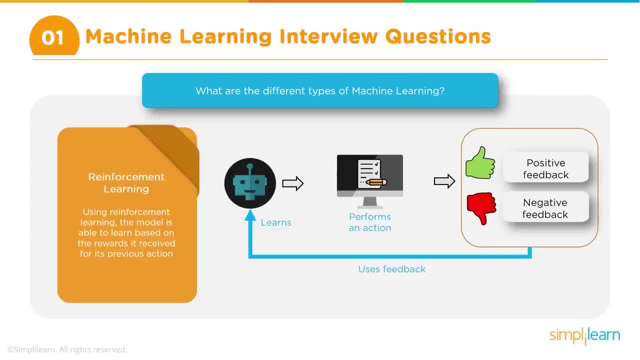 And this is used primarily or very, very impactful, or teaching the system to learn games, and so on. Some examples of this are basically used in AlphaGo. You can throw that as an example where AlphaGo used reinforcement learning to actually learn to play the game of Go and finally it defeated the Go world champion right. 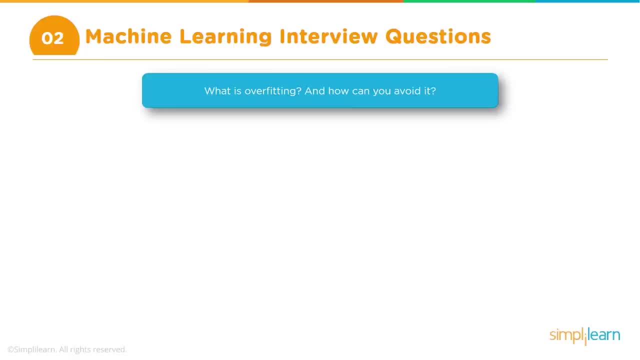 This much of information. that would be good enough. Okay, Then there could be a question on overfitting. So the question could be: what is overfitting and how can you avoid it? So what is overfitting? Okay, Let's just try to understand the concept, because sometimes overfitting may be a little. 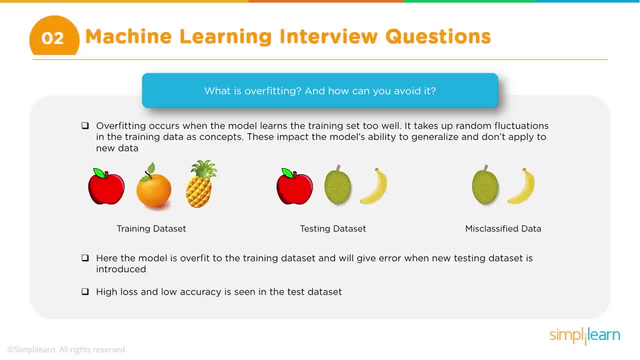 difficult to understand. Overfitting is a situation where the model has kind of memorized the data. So this is an equivalent of memorizing the data. So we can draw an analogy so that it becomes easy to explain this. Now let's say you're teaching a child about recognizing some fruits or something like. 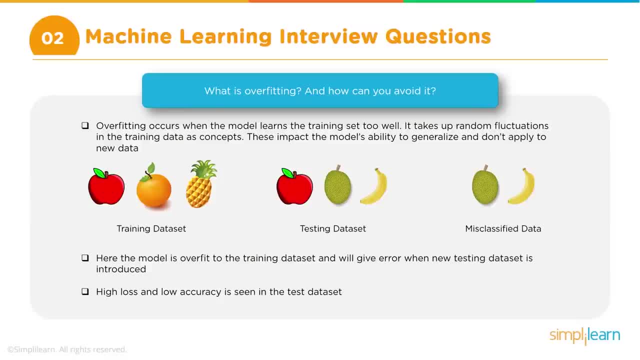 that, Okay, And you're teaching this child about recognizing, let's say, three fruits: apples, oranges and pineapples. Okay, So this is a small child and for the first time, you're teaching the child to recognize fruits. Then, so what will happen? 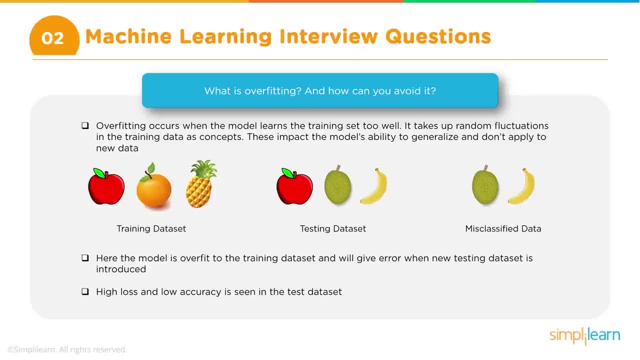 So this is very much like that is your training data set. So what you will do is you will take a basket of fruits which consists of apples, oranges and pineapples, Okay, And you take this basket to this child, and there may be, let's say, hundreds of these. 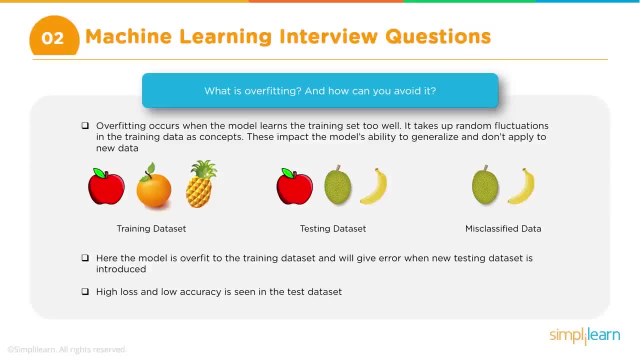 fruits. So you take this basket to this child and keep showing each of this fruit, And then first time obviously, the child will not know what it is. So you show an apple and you say: Hey, this is apple. Then you show maybe an orange and say: this is orange, and so on and so forth. 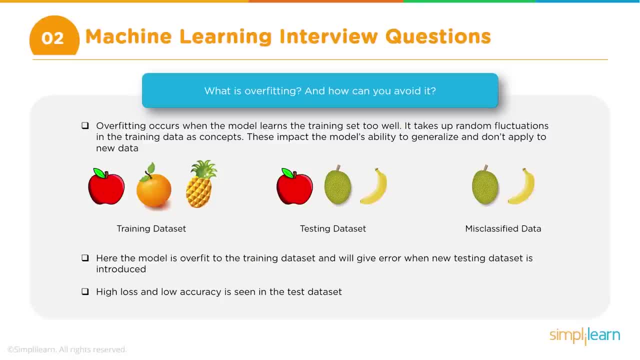 And then again you keep repeating that right. So until that basket is over. this is basically how training work. in machine learning also, That's how training works. So till the basket is completed, maybe a hundred fruits. you keep showing this child. 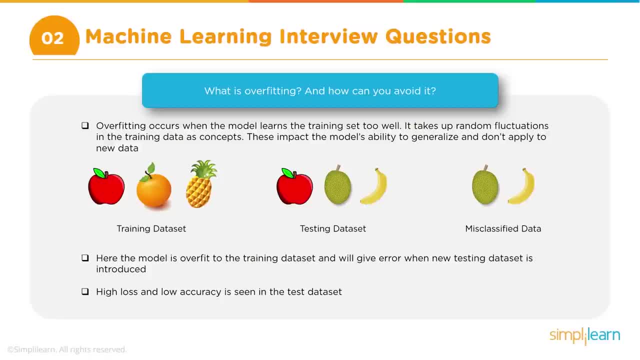 And then the process. what has happened? the child has pretty much memorized these. So Once you finish that basket right, By the time you are halfway through. the child has learned about recognizing the apple, orange and pineapple. Now what will happen after, halfway through? initially, you remember it made mistakes in 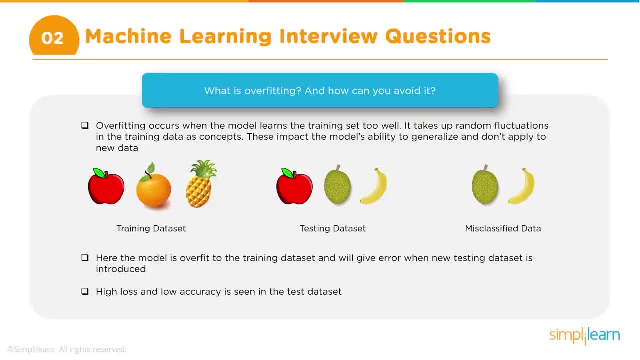 recognizing. but halfway through, now it has learned. So every time you show a fruit, it will exactly a hundred percent accurately, it will identify it. It will say: the child will say: this is an apple, this is an orange. And if you show a pineapple it will say: this is a pineapple. 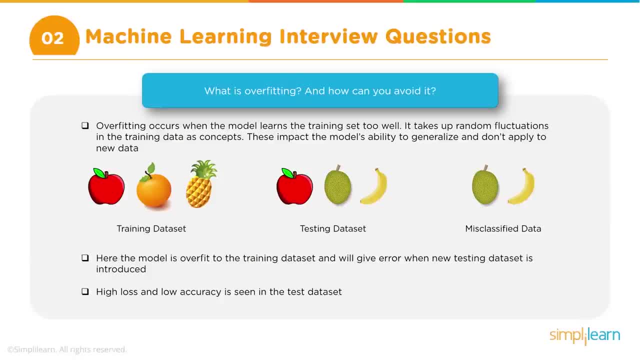 Right, So that means The child has already seen this data. Now let's say you bring another basket of fruits and it will have a mix of maybe apples, which were already there in the previous set, but it will also have in addition to apple. 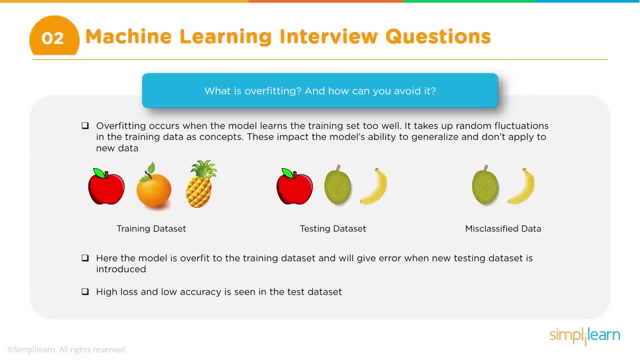 it will probably have a banana or maybe another fruit like a jackfruit, right? So this is an equivalent of your test data set, which the child has not seen before. Some parts of it It probably has seen, like the apples it has seen, but this banana and a jackfruit it has. 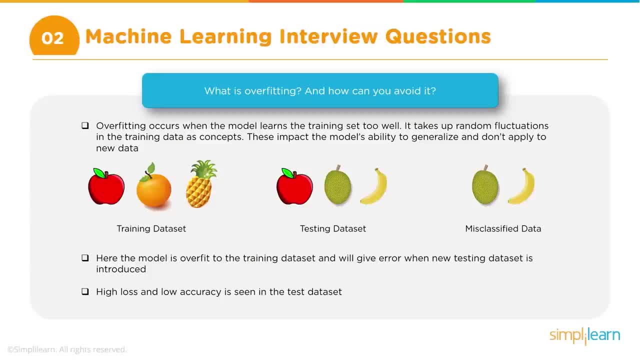 not seen. So then what will happen in the first round, which is an equivalent of your training data set towards the end, it has a hundred percent. It was telling you what the fruits are, right: Apple was accurately recognized, Orange was accurately recognized and pineapples were accurately recognized, right. 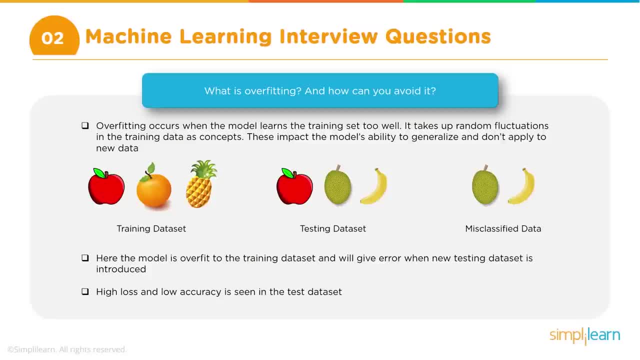 So that is like a hundred percent accuracy. But now, when you get another, a fresh set, which were not part of the original one, what will happen? All the apples maybe it will be able to recognize correctly, but all the others, like the jackfruit. 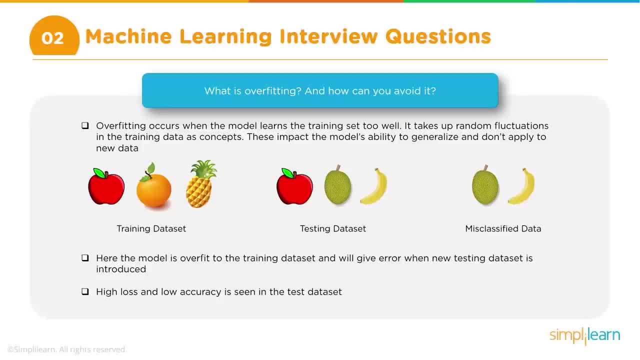 or the banana Will not be recognized by the child, right? So this is an analogy. This is an equivalent of overfitting. So what has happened during the training process? It is able to recognize or reach a hundred percent accuracy, maybe very high accuracy. 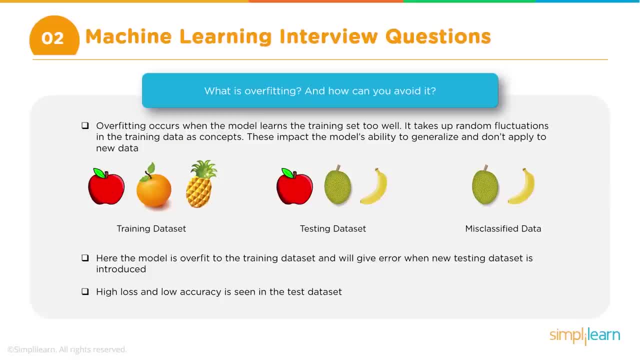 Okay, And we call that as very low loss, right? So that is the technical term. So the loss is pretty much zero and accuracy is pretty much a hundred percent, Whereas when you use testing, there will be a huge error, which means the loss will be. 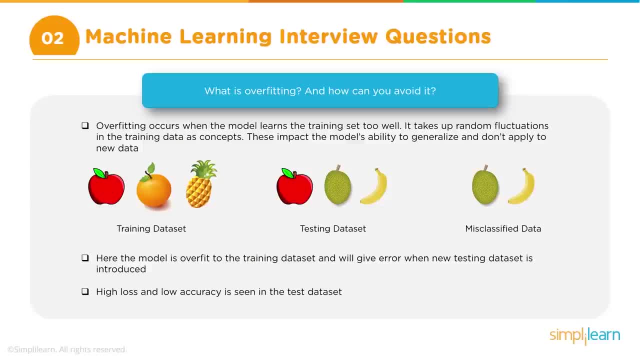 pretty high, Okay, And the accuracy will be also low- Okay. This is known as overfitting. This is basically a process where training is done, training processes. It goes very well, almost reaching a hundred percent accuracy, but while testing it really, 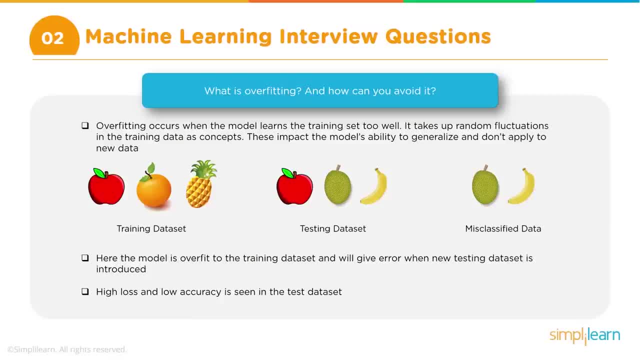 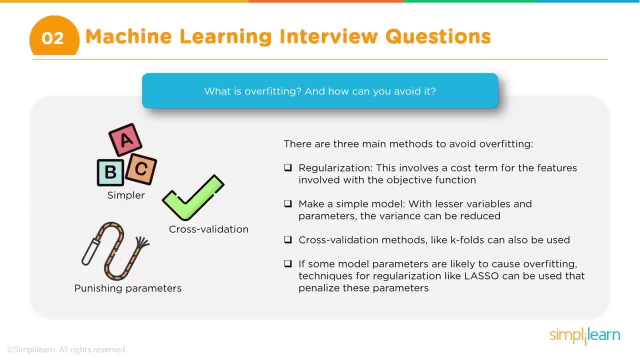 drops down. Now how can you avoid it? So that is a extension of this question. There are multiple ways of avoiding overfitting. There are techniques like what you call regularization. that is the most common technique that is used for avoiding overfitting. 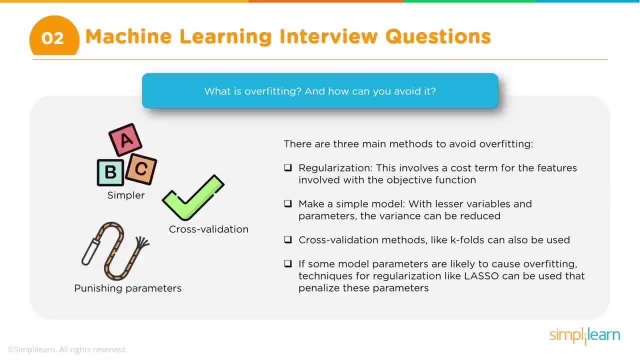 Okay, And within regularization there can be a few other subtypes, like dropout in case of neural networks and a few other examples. But I think if you give example or if you give regularization as the technique, probably that should be sufficient. So there will be some questions where the interviewer will try to test your fundamentals. 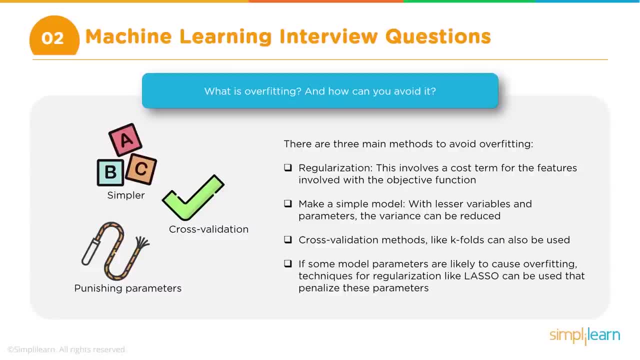 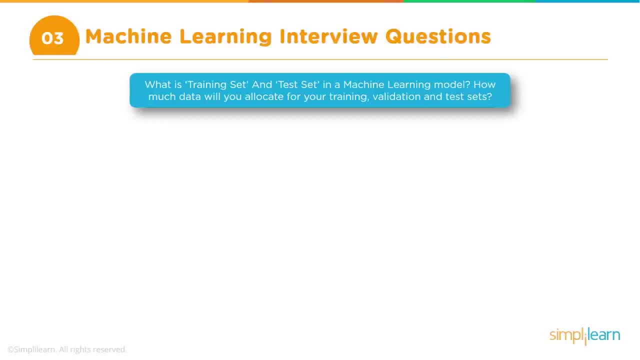 and your knowledge and depth of knowledge and so on and so forth. And then there will be some questions which are more like okay, Questions which are more like quick questions that will be more to stump you, Okay. Then the next question is around the methodology. 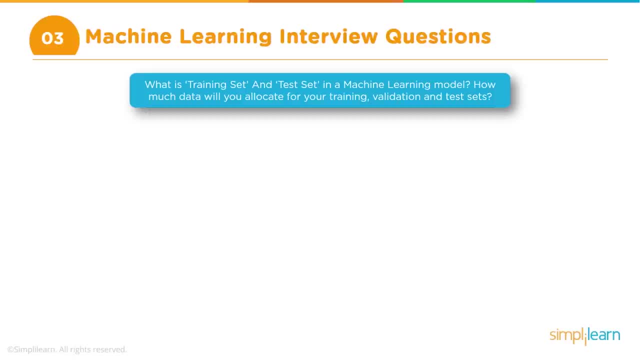 So when we are performing machine learning training, we split the data into training and test, right? So this question is around that. So the question is: what is training set and test set in machine learning model and how is the split done? So the question can be like that: 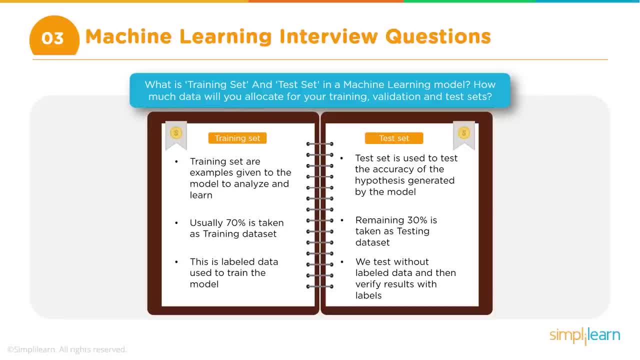 So in machine learning, when we are trying to train the model, so we have a three step process: We train the model and then we test the model And then, once we are satisfied with the test, only then we deploy the model. So what happens in the train and test is that you remember the labeled data. 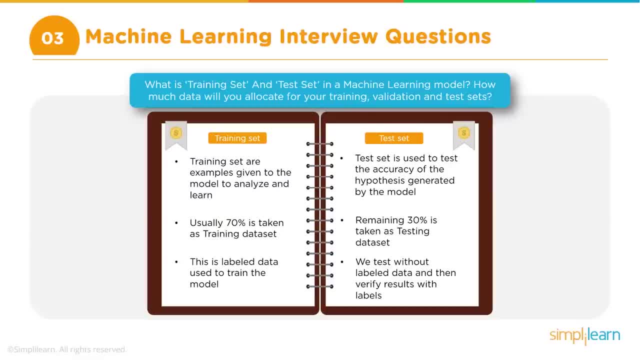 So let's say you have a thousand records with labeling information. Now one way of doing it is you use all the thousand records for training and then maybe right, which means that you have exposed all this thousand records during the training- And then you take a small set of the same data and then you say, okay, I will test it. 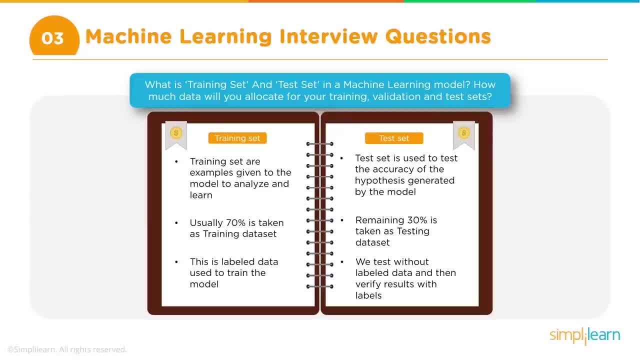 with this, Okay, And then you probably what will happen? You may get some good results right, But there is a flaw there. What is the flaw? This is very similar to human beings. It is like you are showing this model, the entire data, as a part of training. 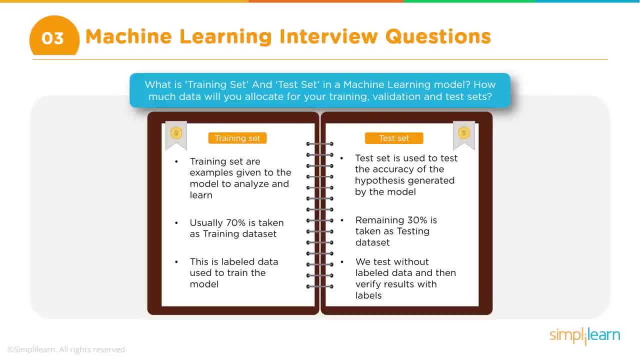 Okay, So obviously it has become familiar with the entire data. So when you're taking a part of that again and you're saying that I want to test it, obviously you will get good results. So that is not a very accurate way of testing. 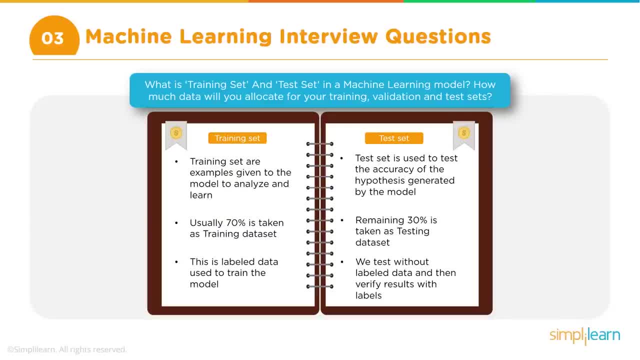 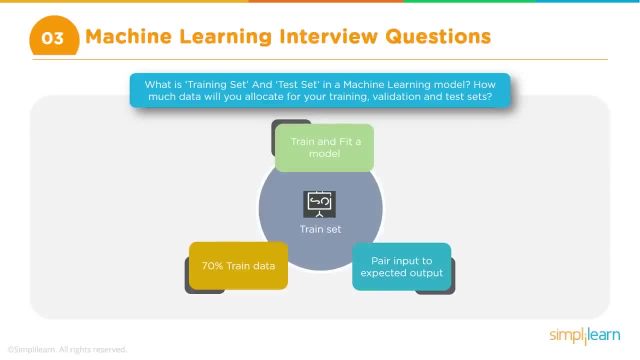 So that is the reason. what we do is we have the label data of this thousand records or whatever We set aside before starting the training process. we set aside a portion of that data and we call that test set and the remaining we call as training set. 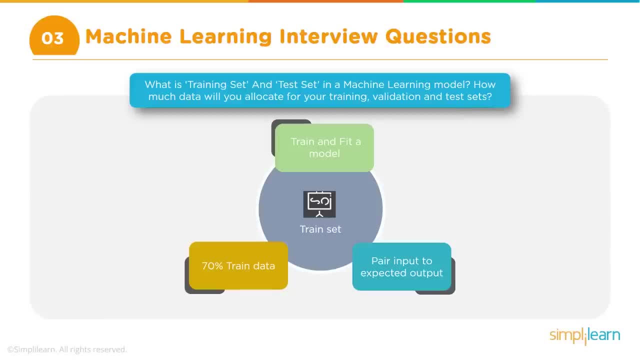 And we use only this for training, our model. Now, the training process, remember, is not just about passing one round of this Data set. So let's say now your training set has 800 records. It is not just one time you pass this 800 records. 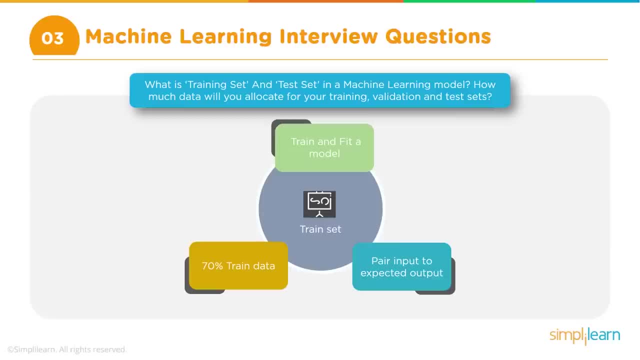 What you normally do is you actually, as a part of the training, you may ask this data through the model multiple times. So this thousand records may go through the model maybe 10,, 15,, 20 times, till the training is perfect, till the accuracy is high, till the errors are minimized. 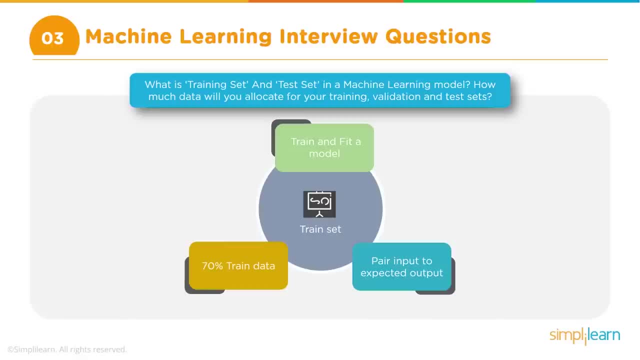 Okay Now so, which is fine, which means that your- that is what is known as the model- has seen your data and gets familiar with your data. And now, when you bring your test data, what will happen is: this is like some new data. 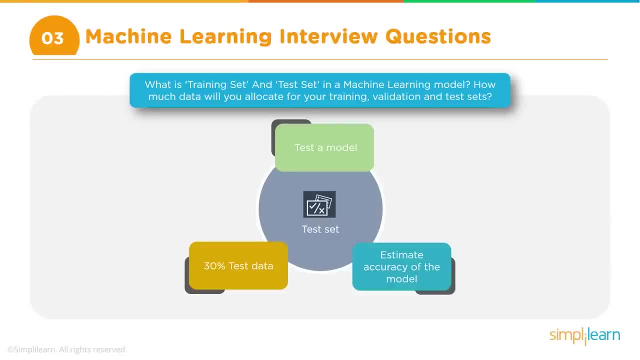 because that is where the real test is. Now you have trained the model and now you are testing the model with some data which is kind of new. That is like a situation, like a realistic situation, because when the model is deployed, that is what will happen. 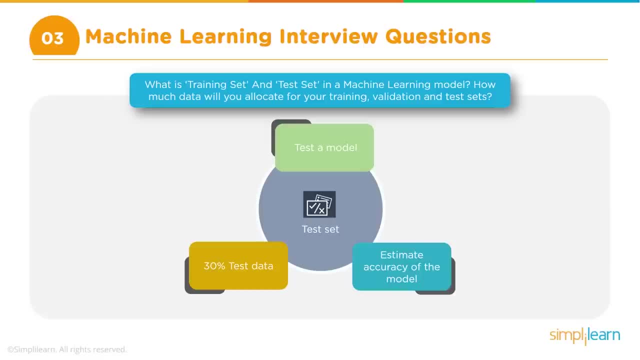 It will receive some new data, not the data that it has already seen, Right. So this is a realistic test. So you put some new data. So this data which you have set aside For the model, it is new And if it is able to accurately predict the values, that means your training has worked. 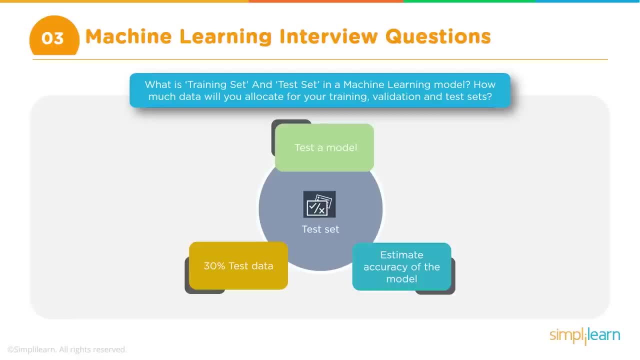 Okay, The model got trained properly. But, let's say, while you're testing this with this test data, you're getting a lot of errors. That means you need to probably either change your model or retrain with more data and things like that. 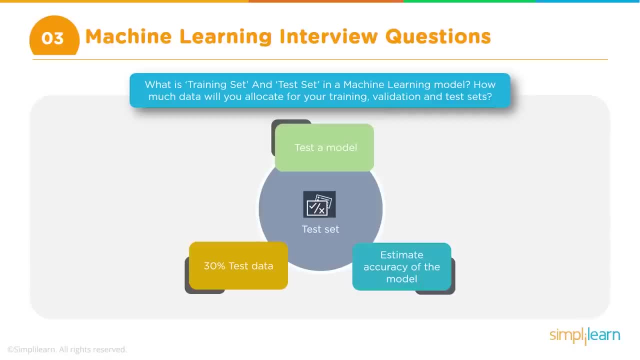 Now coming back to the question of how do you split this? What should be the ratio? There is no fixed number. Again, this is like individual preferences. Some people split it into 50-50, 50% test and 50% training. 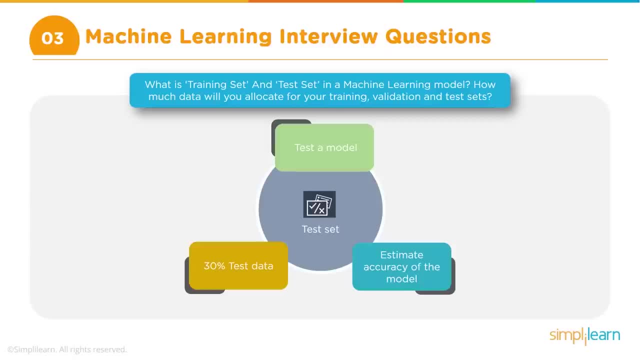 Some people prefer to have a larger amount for training and a smaller amount for test, So they can go by either 60-40 or 70-30, or some people even go with some odd numbers, like 65-35 or 63.33 and 33,, which is like one third and two thirds. 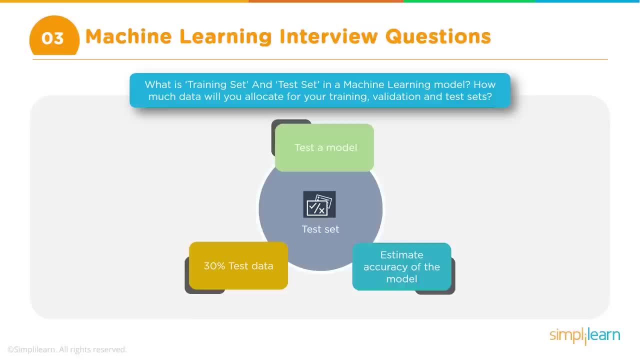 So there is no fixed rule that it has to be something. The ratio has to be this. You can go by your individual preference. Okay, Then you may have questions around data handling, data manipulation or what do you call data management or preparation. 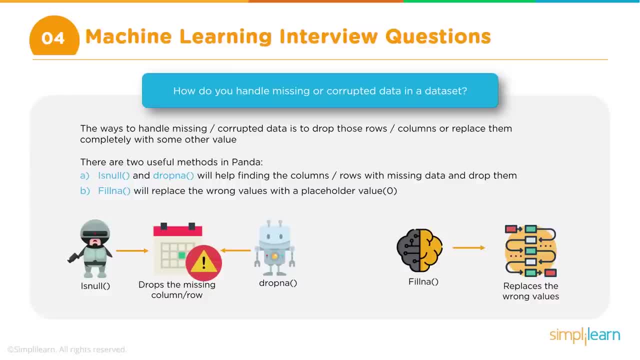 So these are all some questions around that area. There is, again, no one answer, one single good answer to this. It really varies from situation to situation and depending on what exactly is the problem, what kind of data it is, how critical it is, what kind of data is missing and what is. 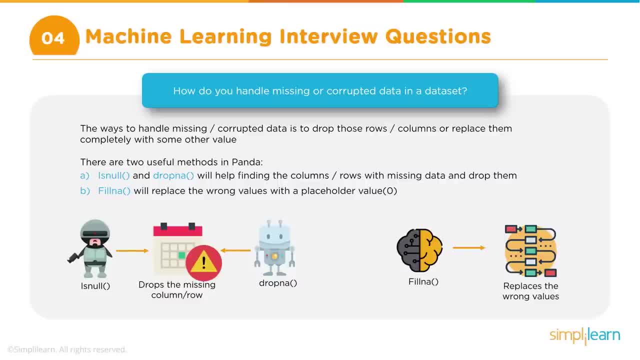 the type of corruption? So there are a whole lot of things. This is a very generic question and therefore you need to be a little careful about responding to this as well, So probably have to illustrate this again. If you have experience in doing this kind of work in handling data, you can illustrate. 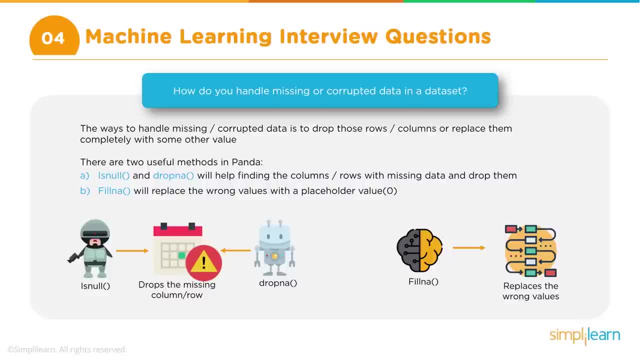 with examples, saying that I was on one project where I received this kind of data. These were the columns where data was not filled, or these were the this many rows where the data was missing. That would be, in fact, a perfect way to respond to this question. 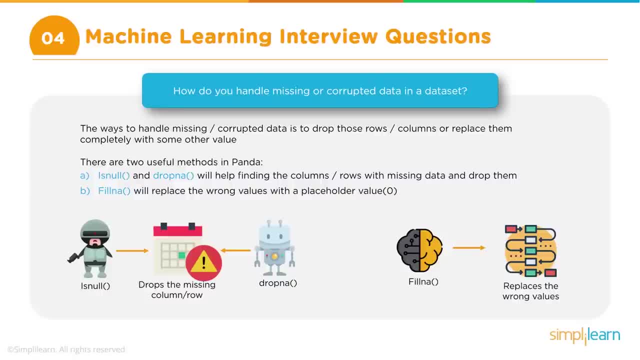 Okay. So if you don't have that, obviously you have to provide some good answer. I think it really depends on what exactly the situation is, and there are multiple ways of handling the missing data or corrupt data. Now let's take a few examples. 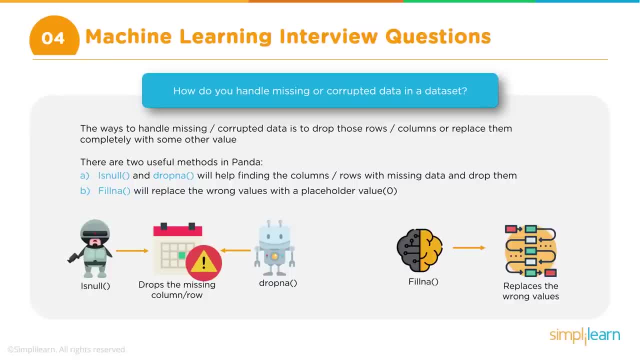 Now, let's say you have data where some values in some of the columns are missing and you have pretty much half of your data having these missing values in terms of number of rows. Okay, That could be one situation. Another situation could be that 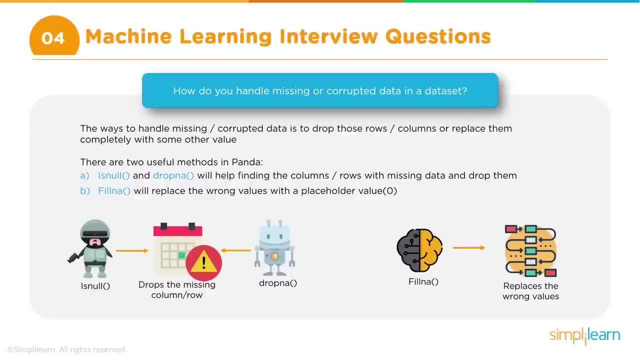 You have. How many records are data missing? but when you do some initial calculation, how many records are corrupt, or how many rows or observations, as we call it, has this missing data? Let's assume it is very minimal, like 10%. okay, 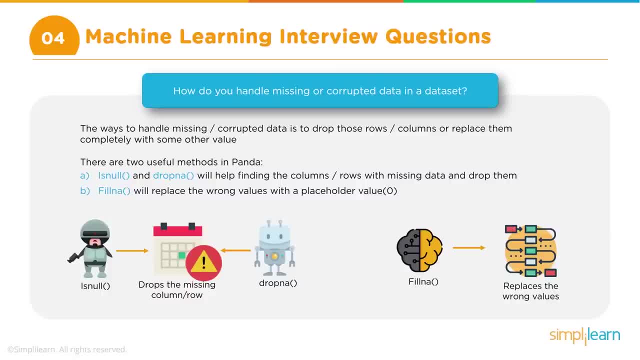 Now between these two cases, how do you so? let's assume that this is not a mission critical situation And in order to fix this 10% of the data, the effort that is required is much higher, And obviously effort means also time and money. 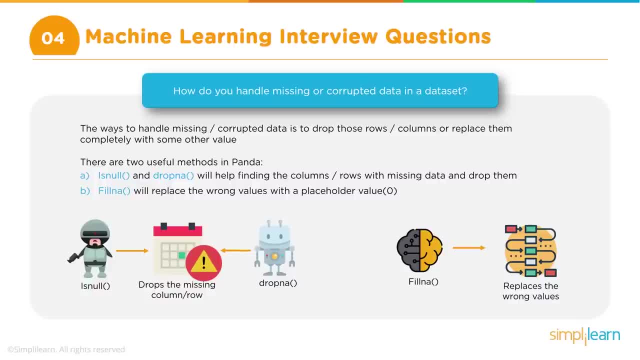 Okay, Okay, Okay. So it is not so mission critical and it is okay to, let's say, get rid of these records. So obviously one of the easiest ways of handling the data part or missing data is remove those records or remove those observations from your analysis. 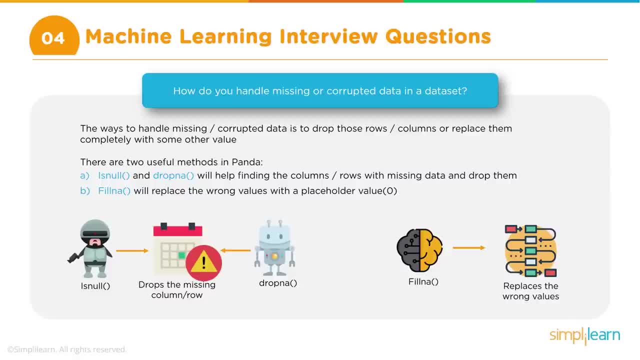 So that is the easiest way to do. But then the downside is, as I said in as in the first case, if, let's say, 50% of your data is like that because some column or the other is missing, So it is not like every in every place, in every row, the same column is missing. but 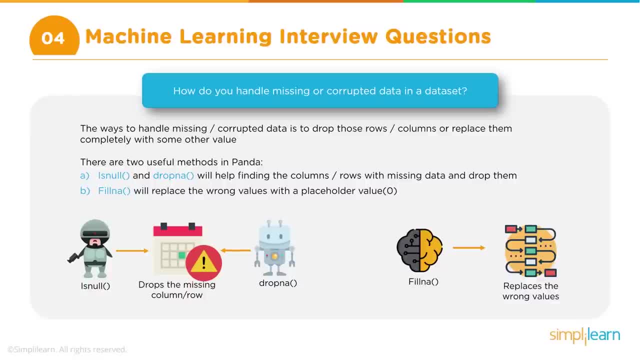 you have in maybe 10% of the records. column one is missing and another 10%, column two is missing, another 10% column three is missing, and so on and so forth. So it adds up to maybe half of your data set. 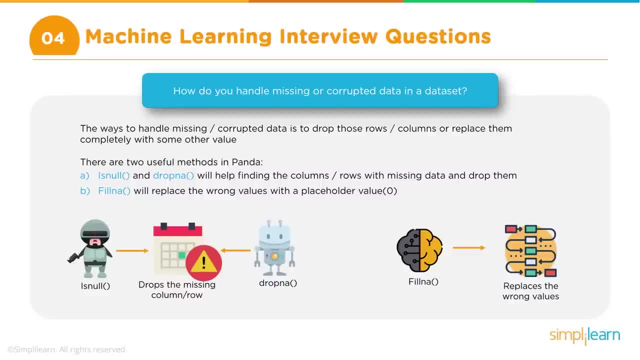 So you cannot completely remove half of your data set, then the whole purpose is lost. Okay, So then how do you handle? Then you need to come up with ways of filling up this data with some meaningful value. right, That is one way of handling. 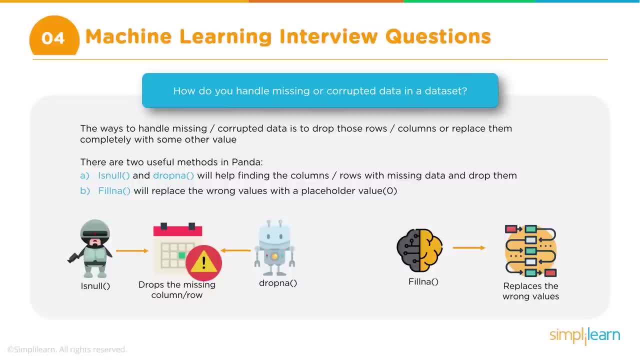 So when we say meaningful value, what is that meaningful value? Let's say, for a particular column. You might want to take a mean value for that column and fill wherever the data is missing. fill up with that mean value, So that when you're doing the calculations your analysis is not completely way off. 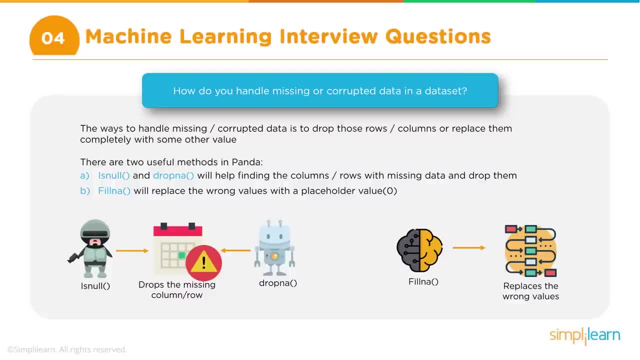 So you have values which are not missing, first of all, so your system will work. Number two: these values are not so completely out of whack that your whole analysis goes for a toss right. There may be situations where if the missing values, instead of putting mean, maybe a good. 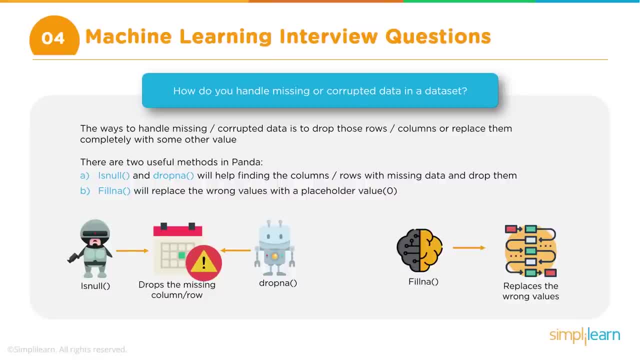 idea to fill it up with the minimum value Or with a zero. So, or with a maximum value again. as I said, there are so many possibilities, So there is no like one correct answer for this. You need to basically talk around this and illustrate with your experience, as I said, 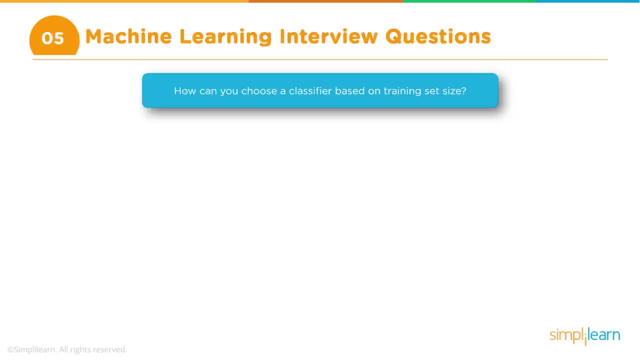 that would be the best. Otherwise, this is how you need to handle this question. Okay, So then the next question can be: how can you choose a classifier based on a training set data size? So again, this is one of those questions where you probably do. 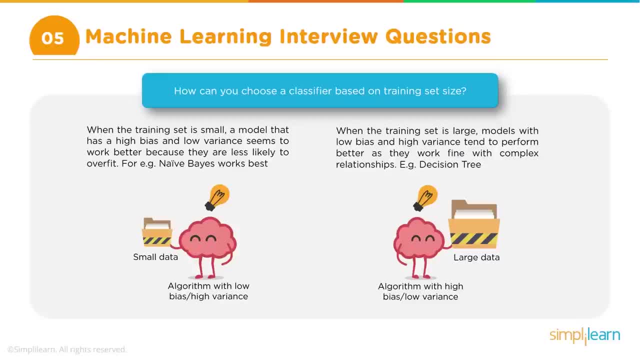 Okay, You do not have like a one size fits all answer. First of all, you may not, let's say, decide your classifier based on the training set size. Maybe not the best way to decide the type of the classifier. And even if you have to, there are probably some thumb rules which we can use. but then 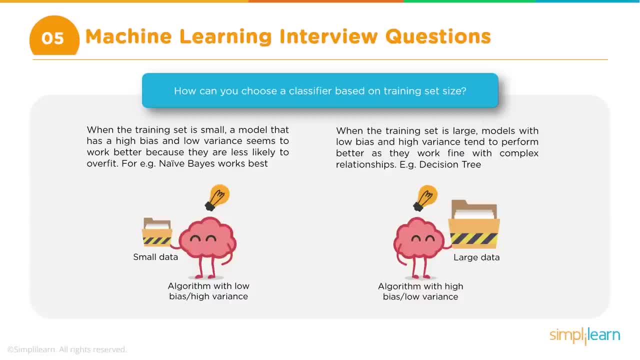 again every time. so, in my opinion, the best way to respond to this question is you need to try out few classifiers, irrespective of the size of the data, And you need to then decide, on your particular situation, which of these classifiers are. 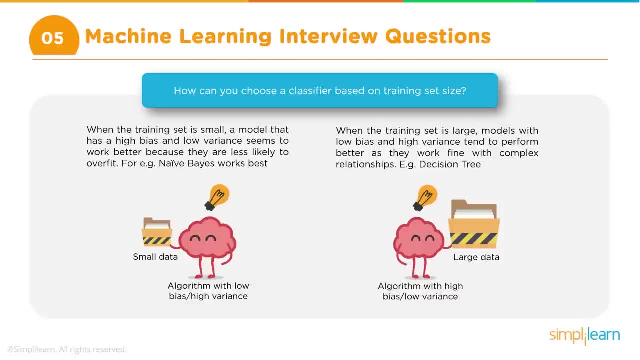 the right ones. This is a very generic issue, So you will never be able to just by if somebody defines a problem to you and somebody, even if they show the data to you or tell you what is the data or even the size of the data. 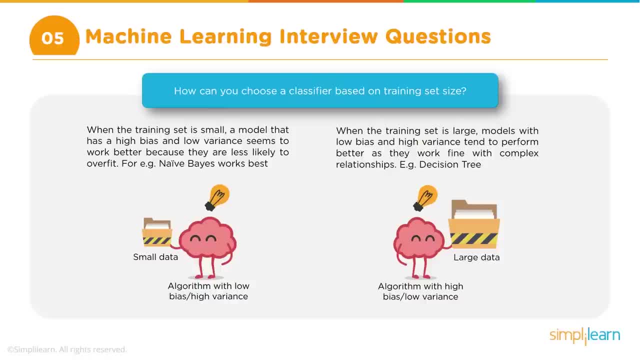 I don't think there is a way to really say that, yes, this is the classifier that will work here. No, that's not the right way, So you need to still, you know, decide. Okay, So test it out, get the data, try out a couple of classifiers, and then only you will be. 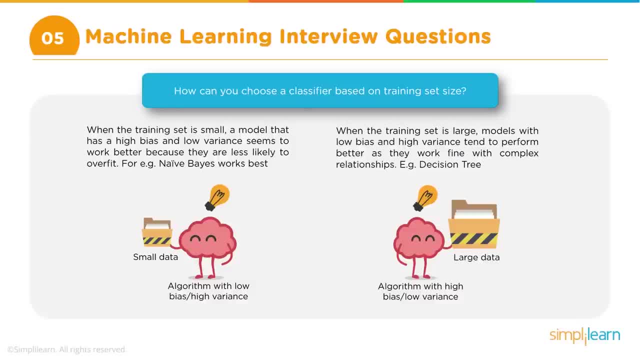 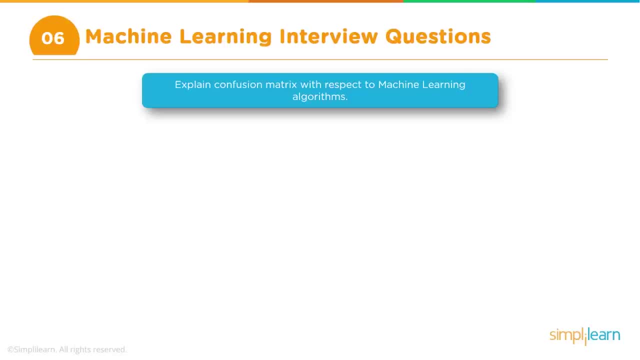 in a position to decide which classifier to use. You try out multiple classifiers, see which one gives the best accuracy, and only then you can decide. Then you can have a question around confusion matrix. So the question can be explained: confusion matrix- right? 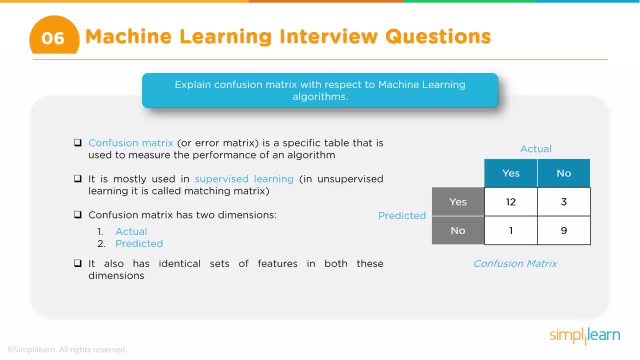 So confusion matrix. I think the best way to explain it is by taking an example and drawing like a small diagram. Otherwise it can really become tricky. So my suggestion is to take a piece of pen and paper and explain it by drawing a small matrix. 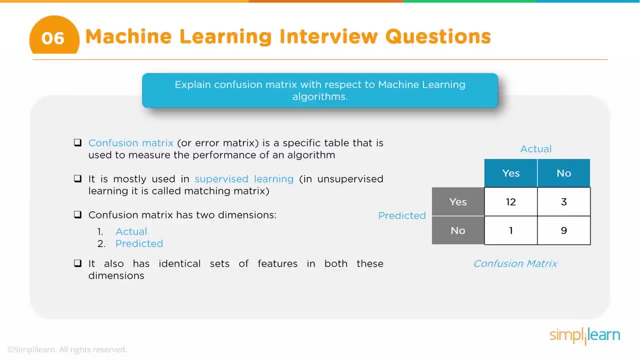 And confusion matrix is about to find out. this is used especially in classification learning process, And when you get the results- and the model predicts the results- you compare it with the actual value and try to find out what is the accuracy. Okay, So in this case, let's say this is an example of a confusion matrix. 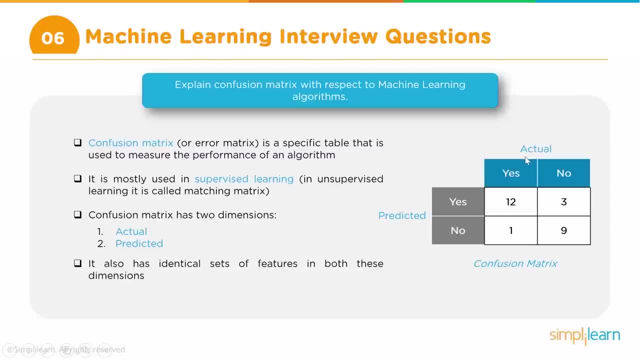 And it is a binary matrix. So you have the actual values, which is the labeled data right And which is so you have how many yes and how many no. So you have that information and you have the predicted values: how many yes and how. 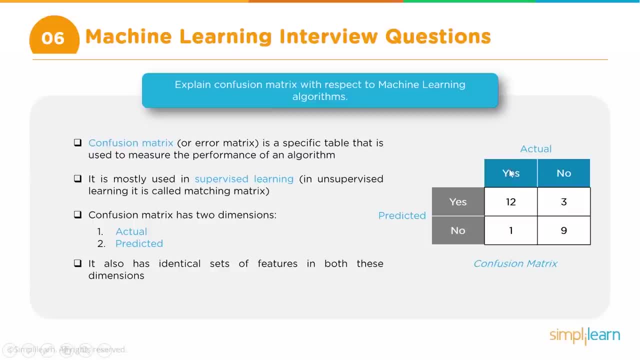 many, no right. So the total actual values: the total yes is 12 plus 1, 13,, and they are shown here, And the actual value no's are 9 plus 3, 12.. Okay, So that is what this information here is. 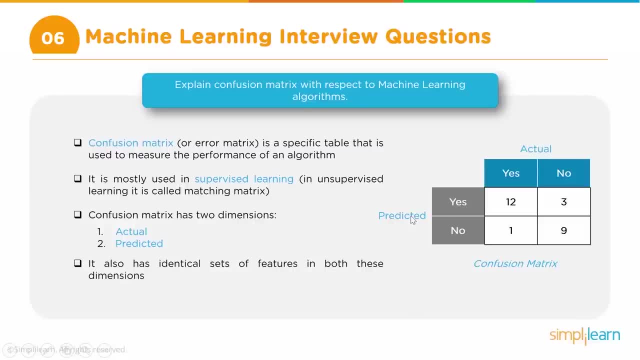 Okay. So this is about the actual and this is about the predicted. Similarly, the predicted values there are: yes are 12 plus 3, 15 yeses and no are 1 plus 9, 10 no's. Okay. 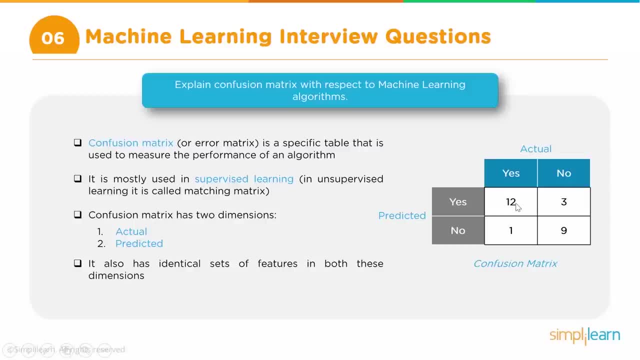 So this is the way to look at this confusion matrix. Okay, And out of this, what is the meaning conveyed here? So there are two or three things that needs to be explained outright. The first thing is for a model to be accurate, the values across the diagonal should be high. 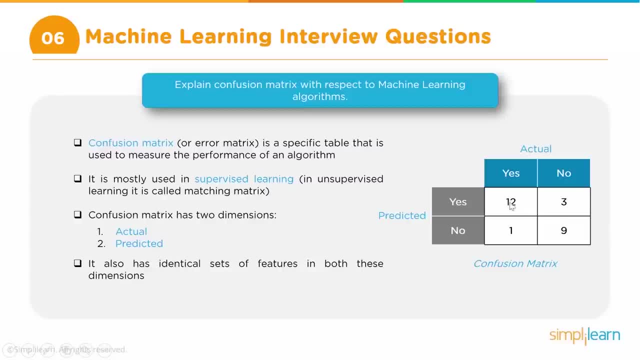 like in this case. right, That is one Number two. the total sum of these values is equal to the total observations in the test dataset. So in this case, for example, you have 12 plus 3, 15 plus 10, 25.. 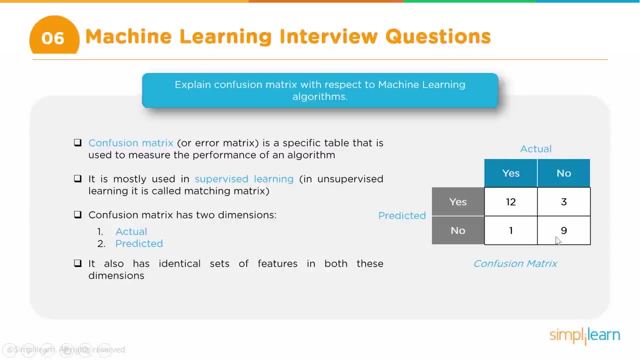 So that means we have 25 observations in our test dataset. Okay, So these are the two things. you need to first explain that the total sum in this matrix the numbers is equal to the size of the test dataset and the diagonal values indicate the. 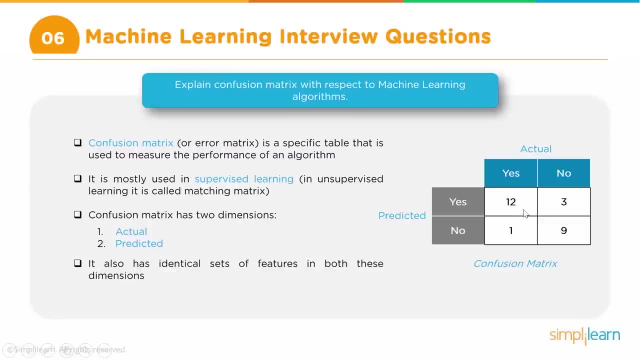 accuracy. So just by looking at it you can probably have an idea about: is this an accurate model? Is the model being accurate? If they're all spread out equally in all these four boxes, that means probably the accuracy is not very good. 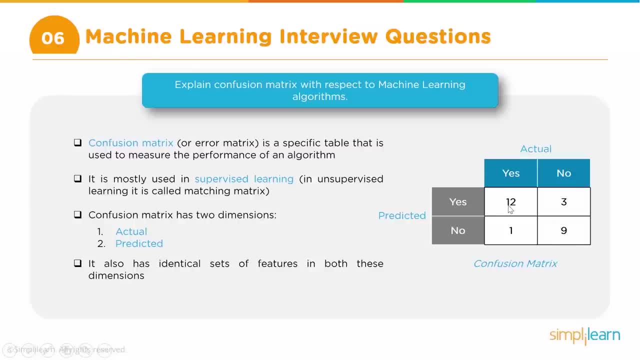 Okay, Now how do you calculate the accuracy itself, Right? How do you calculate the accuracy itself? So it is a very simple mathematical calculation. You take some of the diagonals, right? So in this case, it is 9 plus 12, 21 and divide it by the total. 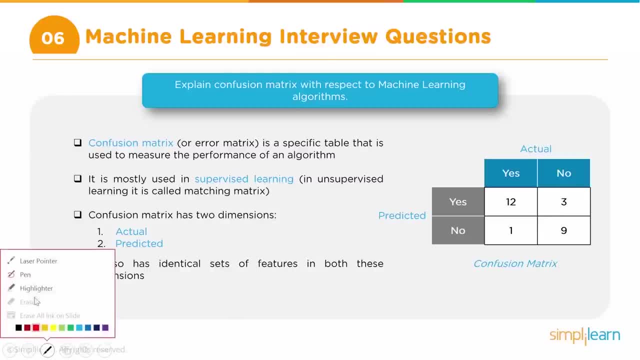 So in this case, what will it be? Let's me take a pen. So your, your diagonal values, is equal to. if I say D is equal to 12 plus nine, So that is 21,. right, And the total data set is equal to right. we just calculated, it is 25.. 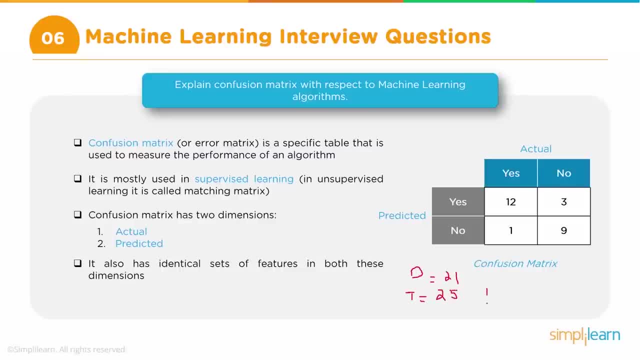 So what is your accuracy? It is: 21 by your accuracy is equal to 21 by 25.. And this turns out to be about 85%, Right? So this is 85%. So that is our accuracy. Okay, So this is the way you need to explain: draw diagram, give an example and maybe it may. 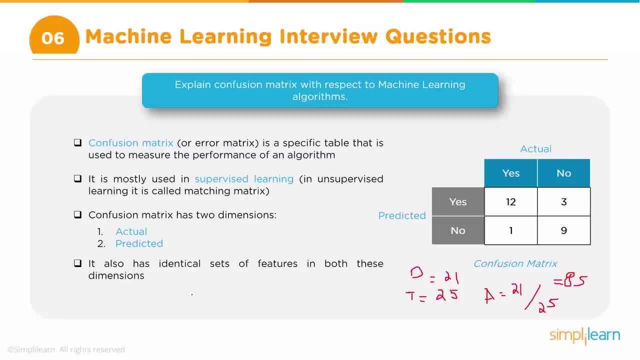 be a good idea to be prepared with an example so that it becomes easy for you. You don't have to calculate those numbers on the fly, right? So a couple of hints are that you take some numbers which are with, which add up to a 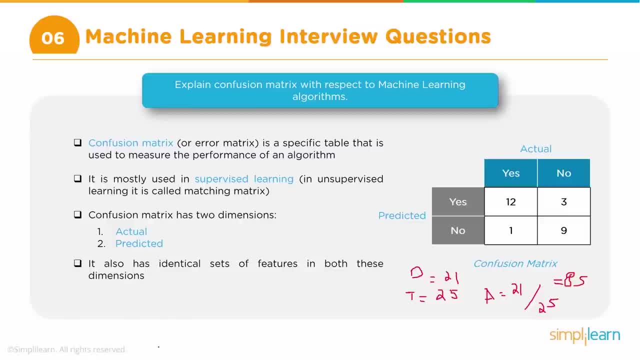 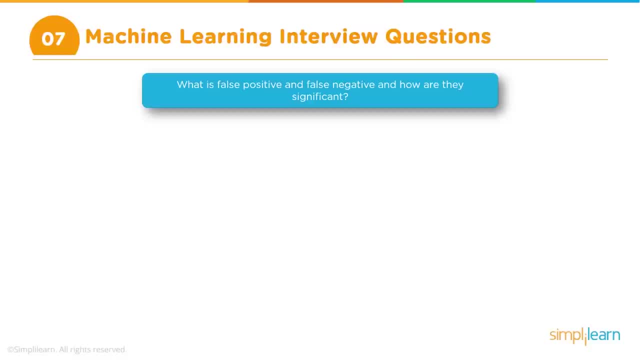 hundred. That is always a good idea, So you don't have to really do this complex calculations. So the total value will be a hundred and then diagonal values. you divide. once you find the diagonal values, That is equal to your percentage. Okay. 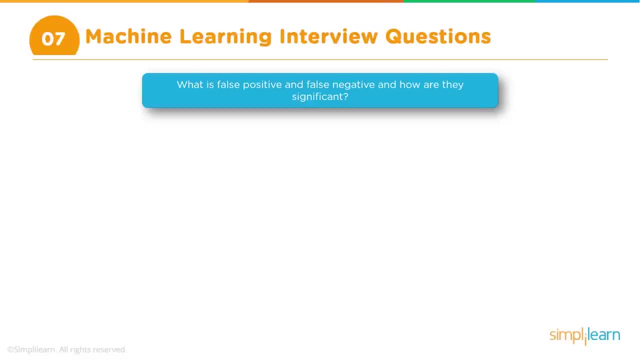 All right, So the next question can be a related question about false positive and false negative. So what is false positive and what is false negative? Now, once again, the best way to explain this is using a piece of paper and pen. otherwise, 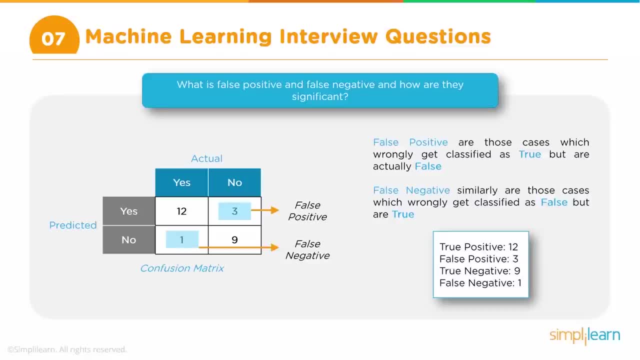 it will be pretty difficult to explain this. So we use the same example of the confusion matrix and we can explain that. So a confusion matrix looks somewhat like this, Okay, And when we just take a, yeah, it looks somewhat like this, and we continue with the previous. 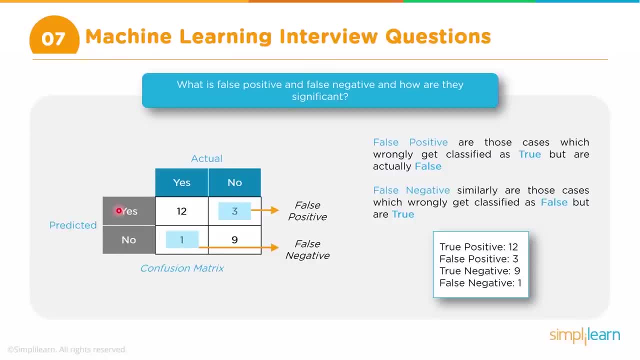 example where this is the actual value, This is the predicted value And in the actual value we have 12 plus 1, 13 yeses and 3 plus 9, 12 nos And the predicted values there are 12 plus 3, 15 yeses and 1 plus 9, 10 nos. 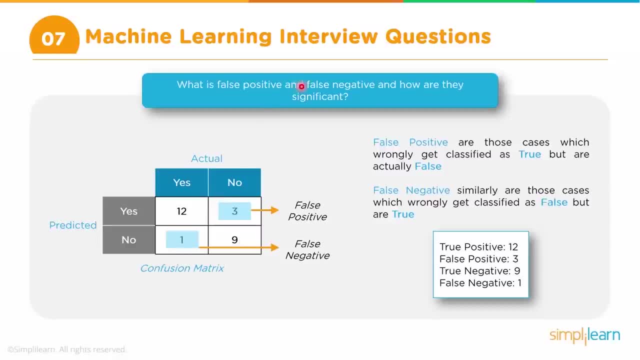 Okay, Now this particular case, which is the false positive. What is a false positive? First of all, the second word which is positive, okay- is referring to the predicted value. So that means the system has predicted it as a positive, but the real value? 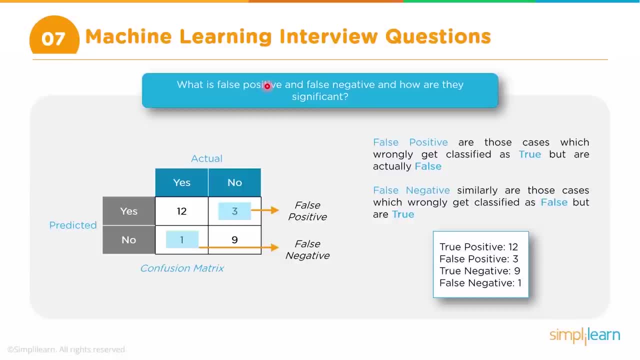 So this is what the false comes from, but the real value is not positive. Okay, That is the way you should understand this term: false positive or even false negative. So false positive, So positive is what your system has predicted. So where is that system predicted? 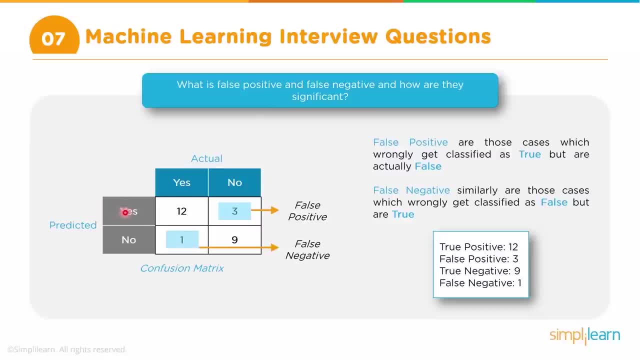 This is the one Positive is what? Yes, So you basically consider this row: Okay. Now, if you consider this row, so this is, this is all positive values, This entire row is positive values. Okay Now, the false positive is the one with where the value- actual value- is negative. 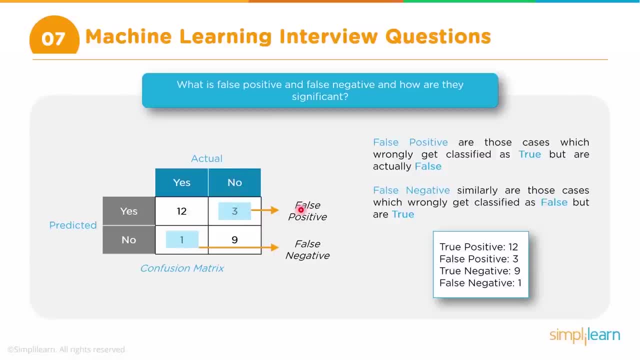 Predicted value is positive, but the actual value is negative. So this is a false positive right, And here is a true positive. So the predicted value is positive and the actual value is also positive. Okay, This is making sense. Now let's take a look at what is false negative, false negative. 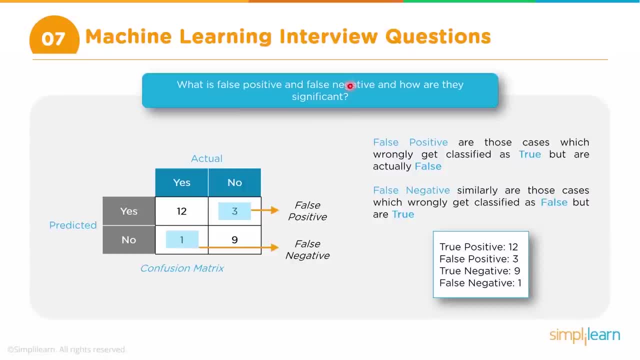 So negative is the second term. That means that is the predicted value that we need to look for. So which are the predicted negative values? This row corresponds to predicted negative values. All right, So this row corresponds to predicted negative values and what they're asking for: false. 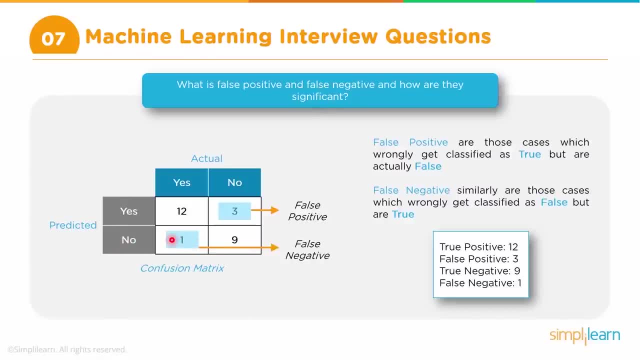 So this is the row for predicted negative values And the actual value is this one right, This is predicted negative and the actual value is also negative. Therefore, this is a true negative. So the false negative is this one: predicted is negative, but actual is positive, right. 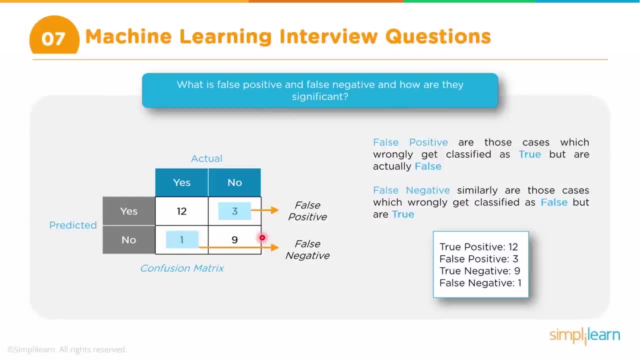 So this is the false negative. So this is the way to explain and this is a way to look at false positive and false negative Same way. there can be true positive and true negative as well. So, again, positive, the second term you will need to use to identify the predicted row. 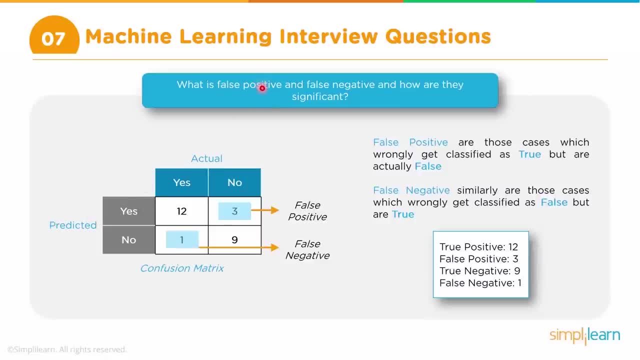 Right. So if we say true, positive, positive we need to take for the predicted part. So predicted positive is here, Okay. And then the first term is for the actual. So true, positive, So true in case of actual is yes, right. 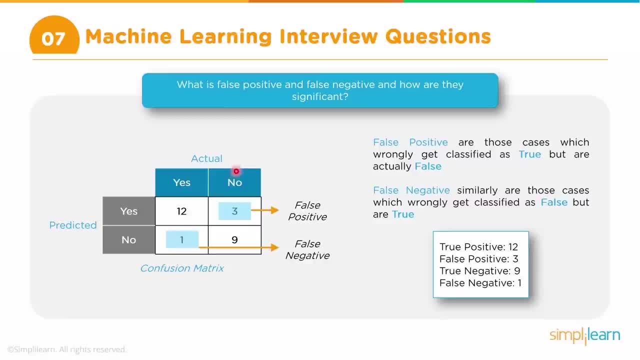 So true, positive is this one, Okay, And then, in case of actual the negative now we are talking about, let's say true, negative, true, negative, Negative is this one, and the true comes from here. So this is true, negative, right. 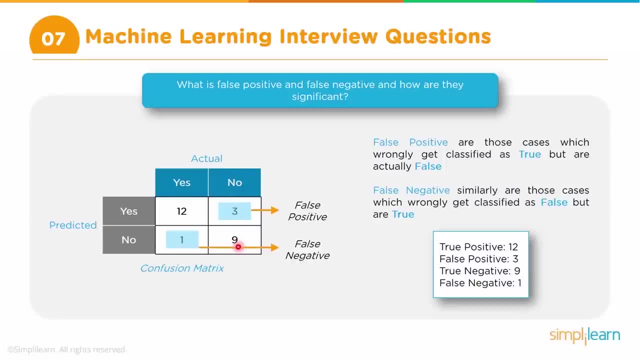 Nine is true, negative, The actual is negative, The actual value is also negative and the predicted value is also negative. Okay, So that is the way you need to explain this: the terms false positive, false negative and true positive, true- negative. 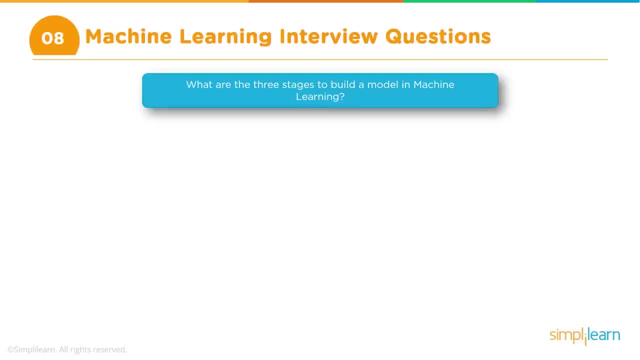 Then you might have a question like: what are the steps involved in the machine learning process? Or what are the three steps in the process of developing a machine learning model? right, So it is around the methodology that is applied. So, basically, the way you can probably answer in your own words. 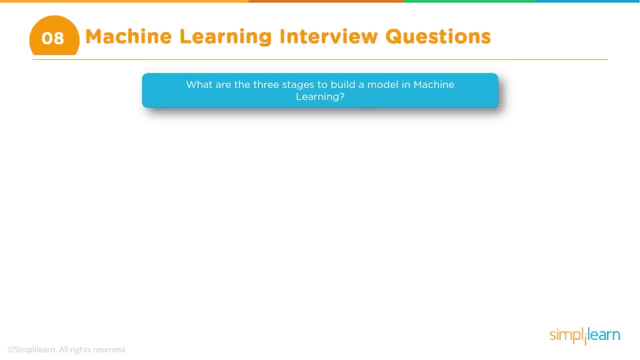 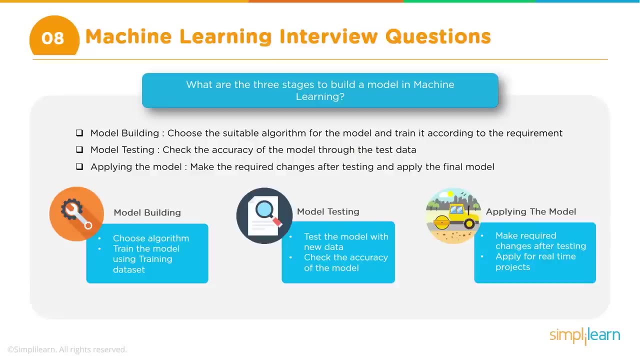 But the way the model development of the machine learning model happens is like this. So first of all you try to understand the problem and try to figure out whether it is a classification problem or a regression problem. Based on that, you select a few algorithms and then you start the process of training. 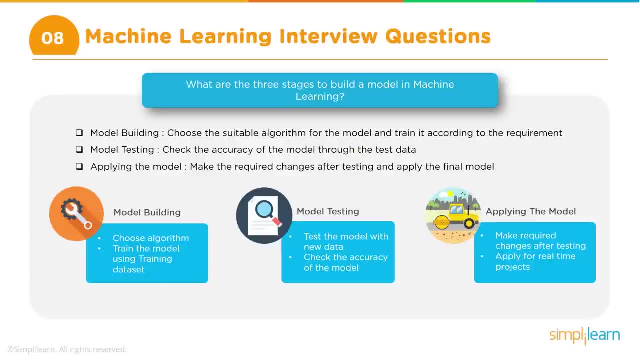 these models. Okay, So you can either do that or you can. after due diligence, you can probably decide that there is one particular algorithm which is most suitable. Usually it happens through trial and error process, but at some point you will decide. 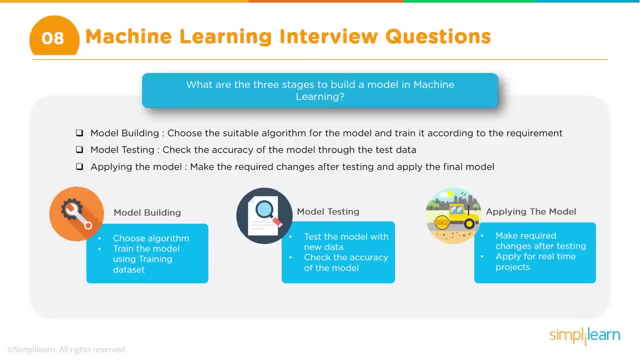 that, okay, this is the model we are going to use. Okay, So in that case, we have the model algorithm and the model decided and then you need to do the process of training the model and testing the model, And this is where, if it is supervised learning, you split your data, the label data, into training. 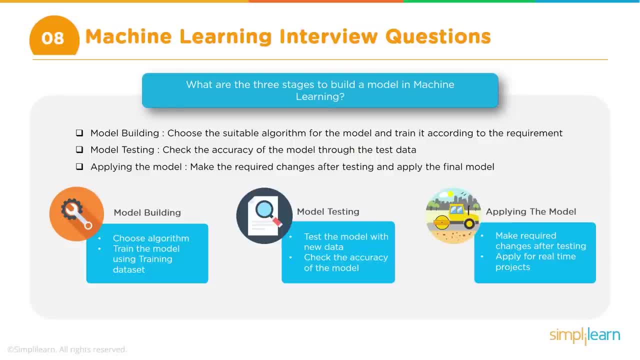 data set and test data set and you use the training data set to train your model and you use the test data set to check the accuracy, whether it is working fine or not. So you test the model before you actually put it into production, right? 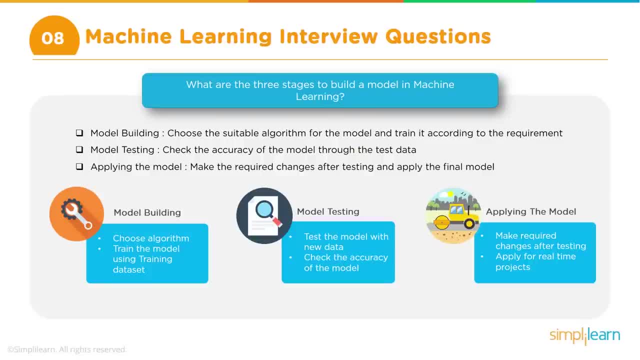 So once you test the model, you're satisfied it's working fine. Then you go to the next level, which is putting it for production, And then in production obviously new data will come and the inference happens. So the model is readily available. 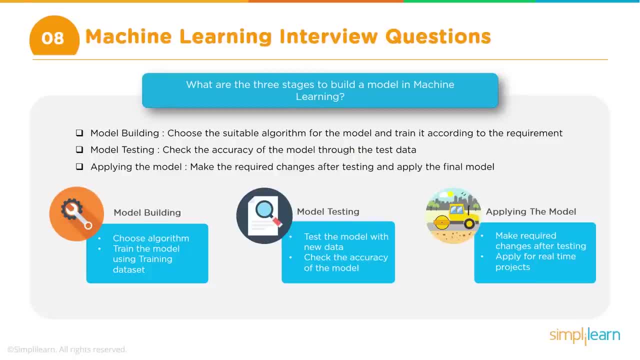 And only thing that happens is new data comes and the model predicts the values, whether it is regression or classification. Now, So this can be an iterative process, So it is not a straightforward process where you do the training, do the testing and then 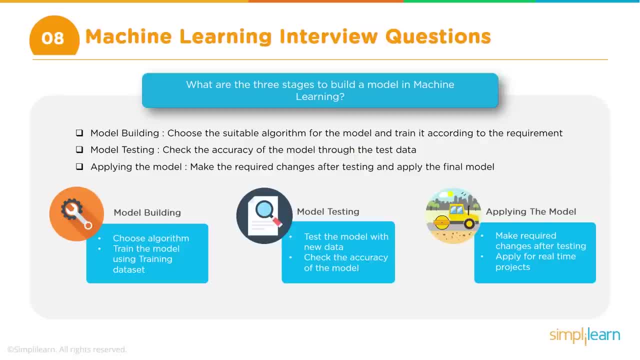 you move it to production now. So during the training and test process, there may be a situation where, because of either overfitting or things like that, the test doesn't go through, which means that you need to put that back into the training process. 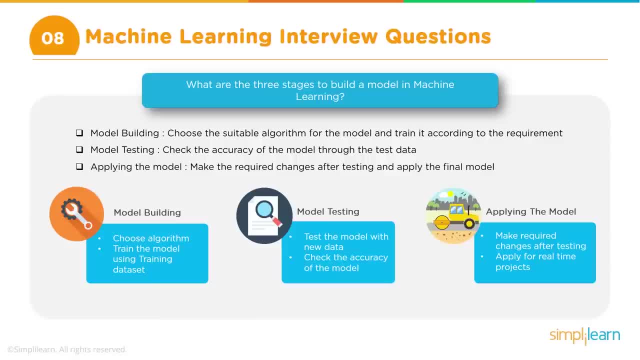 So that can be an iterative process. Not only that, even if the training and test goes through properly and you deploy the model in production, there can be a situation that the data that actually comes, The real data that comes with that, this model is failing. 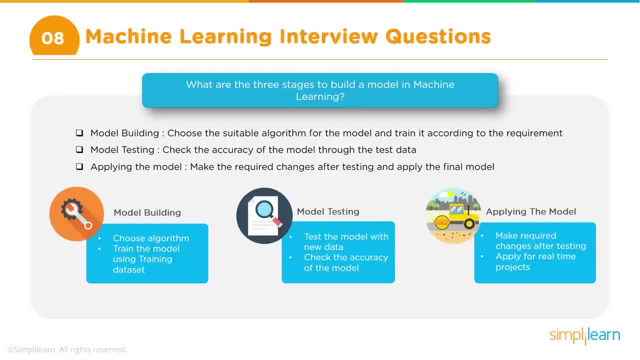 So, in which case you may have to once again go back to the drawing board, or initially it will be working fine, but over a period of time, maybe due to the change in the nature of the data- once again the accuracy will deteriorate. 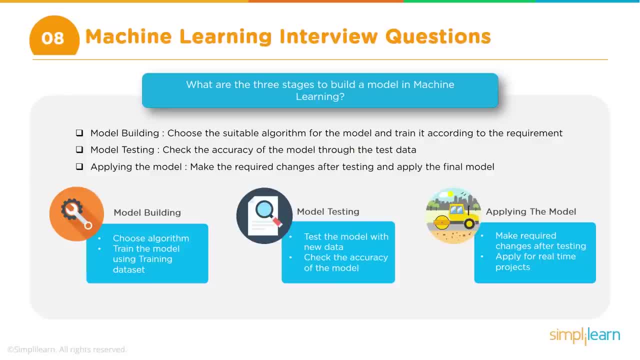 So that is again a recursive process. So once in a while you need to keep checking whether the model is working fine or not And, if required, you need to tweak it and modify it, and so on and so forth. So net-net. 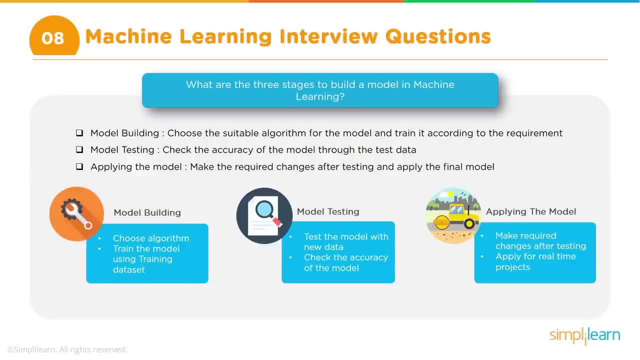 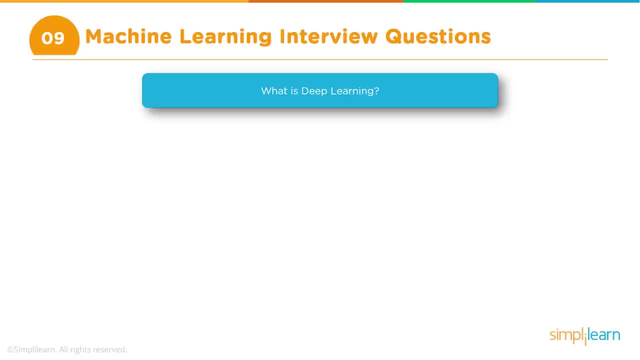 This is a continuous process of Okay, From tweaking the model and testing it and making sure it is up to date. Then you might have question around deep learning. So, because deep learning is now associated with AI, artificial intelligence and so on, So can be as simple as what is deep learning? 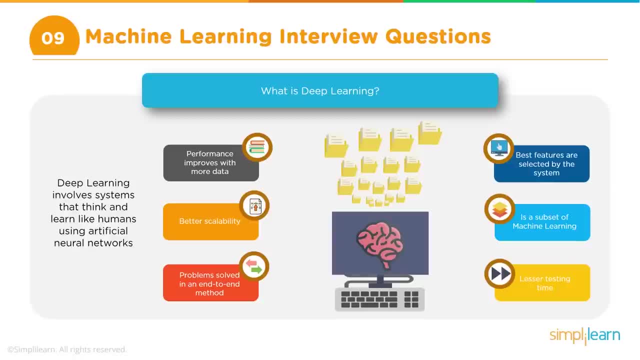 So I think the best way to respond to this could be: deep learning is a part of machine learning, And then, obviously, the question would be: then what is the difference? right? So deep learning, you need to mention there are two key parts that interviewer will be. 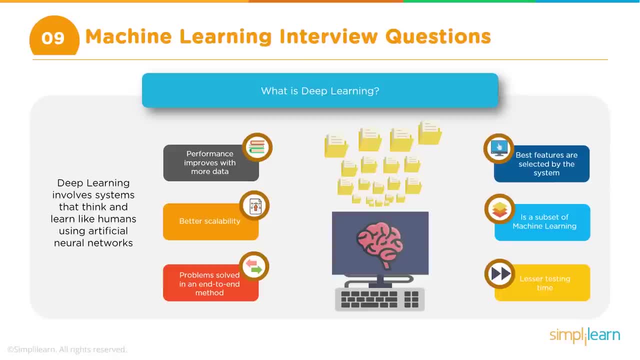 looking for when you are defining deep learning. So first is, of course, deep learning is a subset of machine learning. So machine learning is still the bigger, let's say, scope, and deep learning is one part of it. So then, what exactly is the difference? 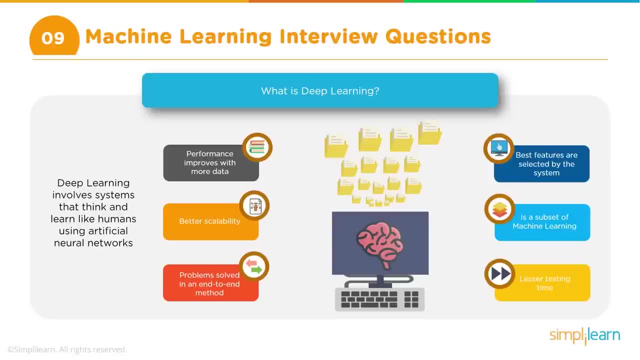 Deep learning is primarily when we are implementing these, our algorithms, or when we are using neural networks for doing our training and classification and regression and all that right. So when we use neural network, then it is considered as Deep learning, and the term deep comes from the fact that you can have several layers. 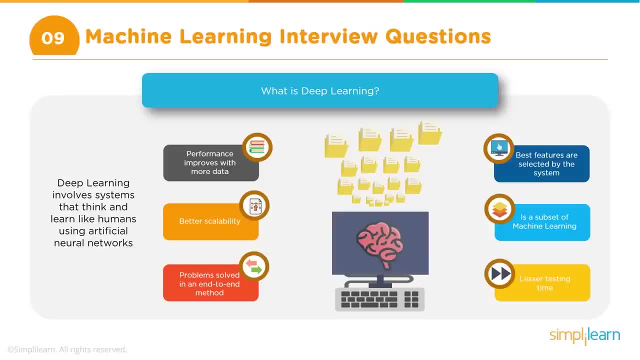 of neural networks, and these are called deep neural networks and therefore the term deep learning. The other difference between machine learning and deep learning, which the interviewer may be wanting to hear, is that in case of machine learning, the feature engineering is done manually. 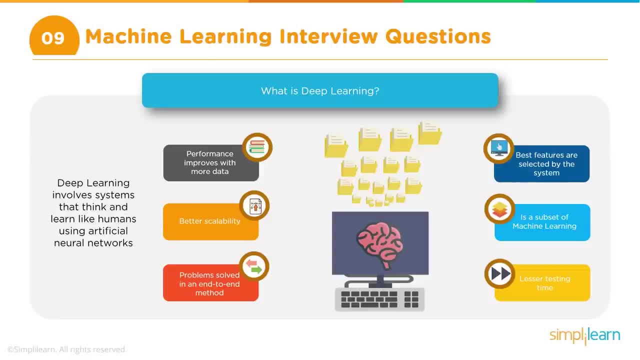 What do we mean by feature engineering Basically when we are trying to train our model? What do we mean by feature engineering Basically? We have our training data right, So we have our training label data and this data has several, let's say, if it is a regular 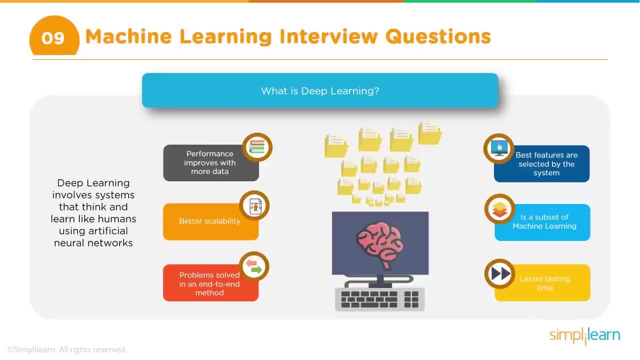 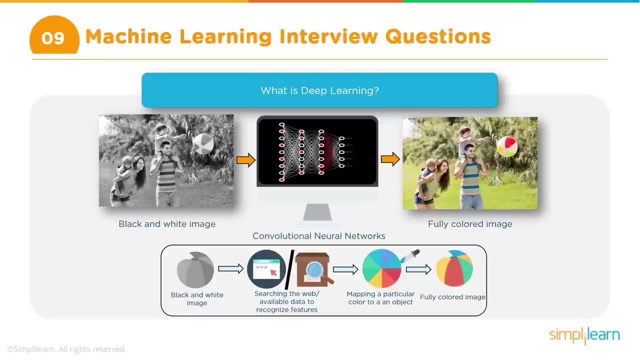 table. it has several columns. Now each of these columns actually has information about a feature right? So if we are trying to predict the height, weight and so on and so forth, So these are all features of human beings. let's say we have census data and we have 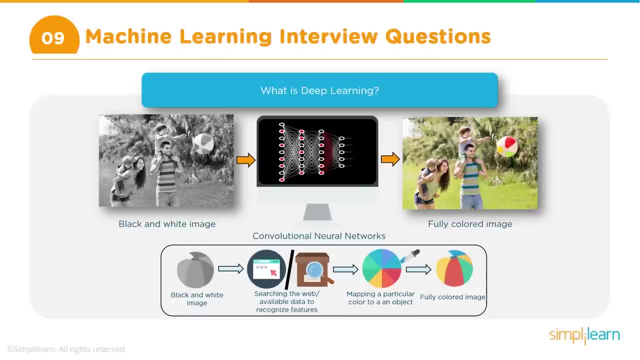 all this. So those are the features Now. there may be probably 50 or a hundred. in some cases there may be a hundred such features. Now all of them do not contribute to our model, right? So we, as a data scientist, we have to decide whether we should take all of them, all the 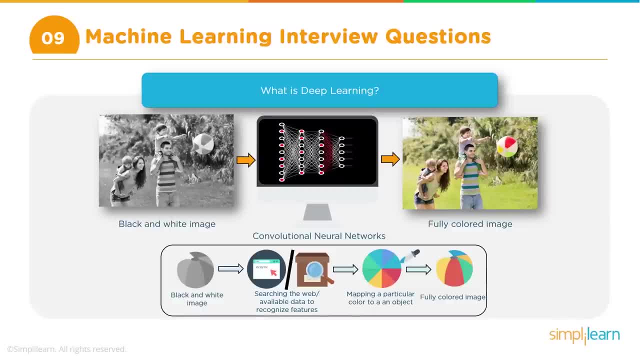 features, or we should throw away some of them, Because again, if we take all of them, number one, of course your accuracy will probably get affected. But also there is a computational part. So if you have so many features and then we have so much data, it becomes very tricky. 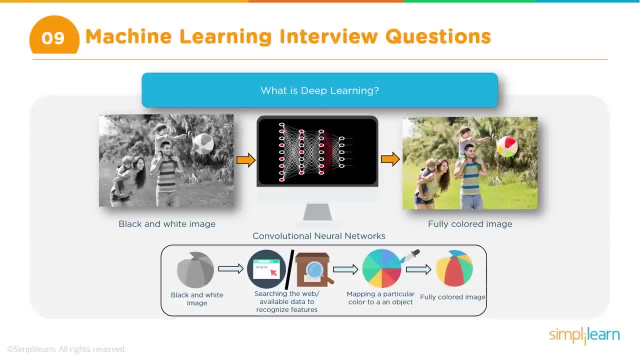 So in case of machine learning, we manually take care of identifying the features, Identifying the features that do not contribute to the learning process, and thereby we eliminate those features, and so on. right, So this is known as feature engineering, And in machine learning we do that manually. 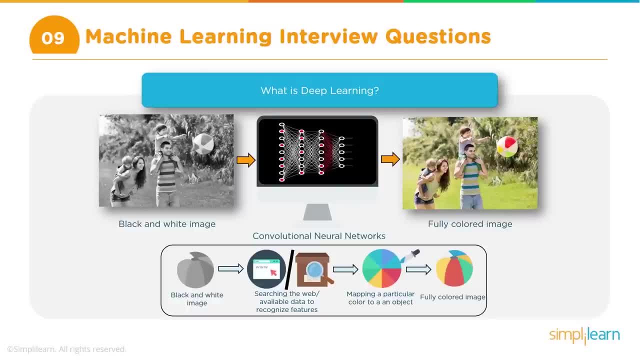 Whereas in deep learning, where we use neural networks, the model will automatically determine which features to use and which to not use, And therefore feature engineering is also done automatically. So this is an explanation. These are two key things. Probably You can add value to your response. 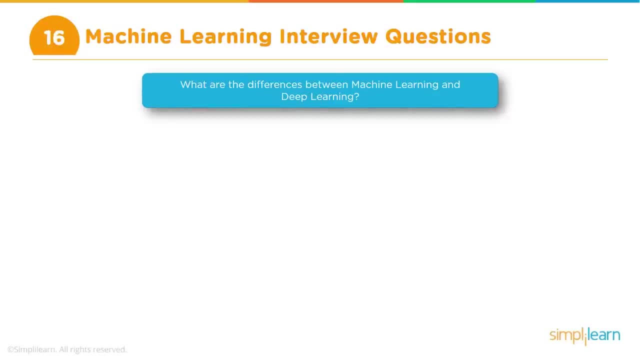 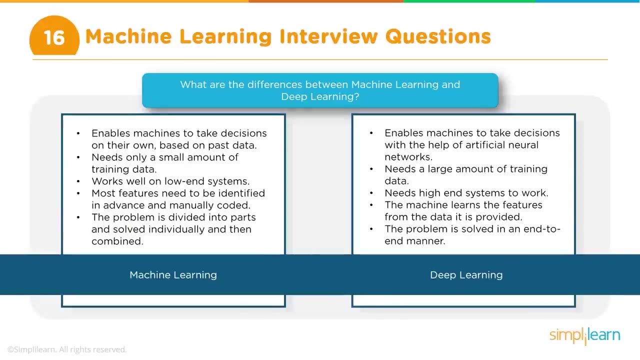 All right. So the next question is: what is the difference between, or what are the differences between, machine learning and deep learning? So here this is a quick comparison table between machine learning and deep learning. And: in: machine learning enables machines to take decisions on their own, based on fast. 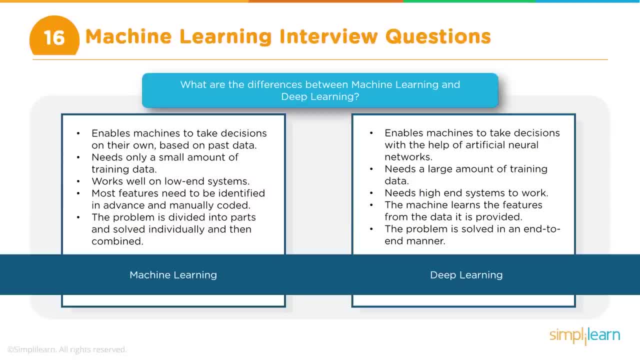 data. So here we are talking primarily of supervised learning, And it needs only a small amount of data for training and then works well on low end systems. So you don't need large machines And most features need to be identified in advance and manually coded. 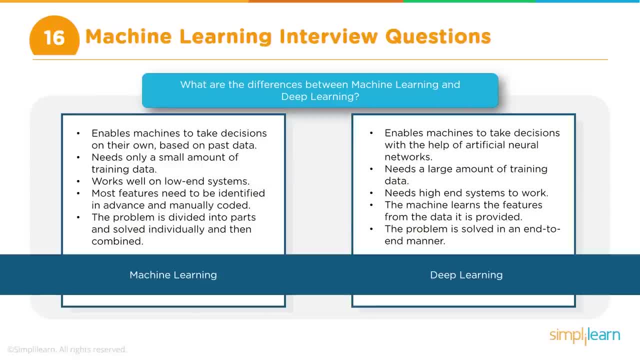 So basically the feature engineering part is done manually and the problem is divided into parts and solved individually and then combined. So that is about the machine learning part In deep learning. deep learning basically enables machines to take decisions with the help of artificial neural networks. 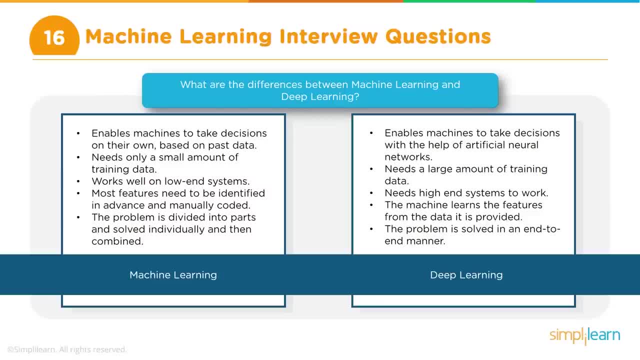 So here in deep learning we use neural networks. So that is the key differentiator between machine learning and deep learning. And usually deep learning involves a large amount of data and therefore the training also requires- usually the training process requires- high-end machines because it needs. 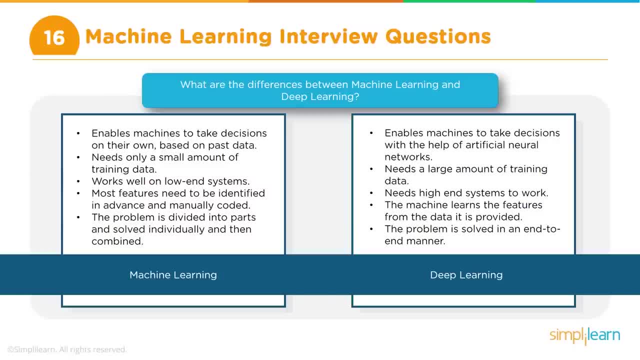 a lot of computing power And the machine learning features are, or the feature engineering is done automatically. So the neural networks takes care of doing the feature engineering as well, And in case of deep learning, therefore, it is said that the problem is handled end-to-end. 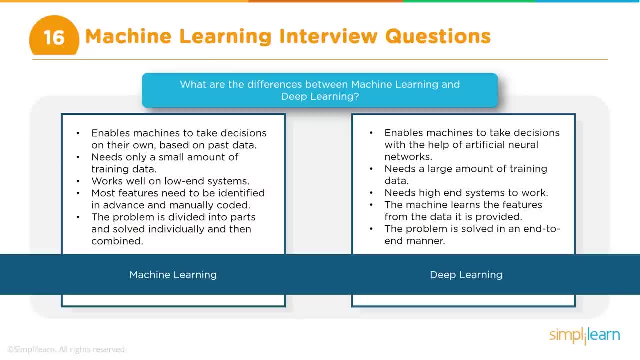 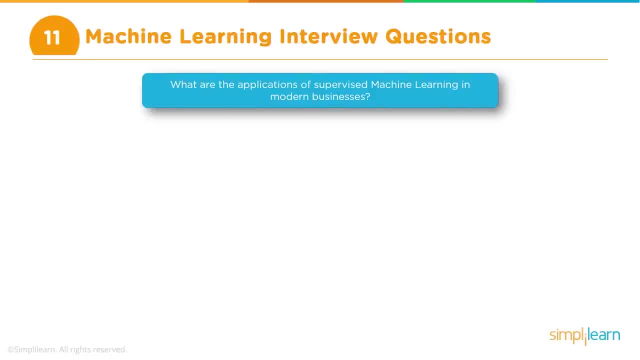 So this is a quick comparison between machine learning and deep learning. Thank you. In case you have that kind of a question, Then you might get a question around the uses of machine learning or some real-life applications of machine learning in modern business. The question may be worded in different ways, but the meaning is: how exactly is machine 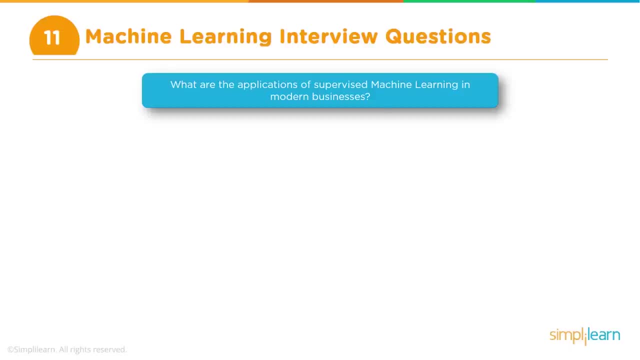 learning used or actually supervised machine learning? It could be a very specific question around supervised machine learning. So this is like give examples of supervised machine learning, use of supervised machine learning in modern business. So that could be the next question. So there are quite a few examples or quite a few use cases, if you will, for supervised 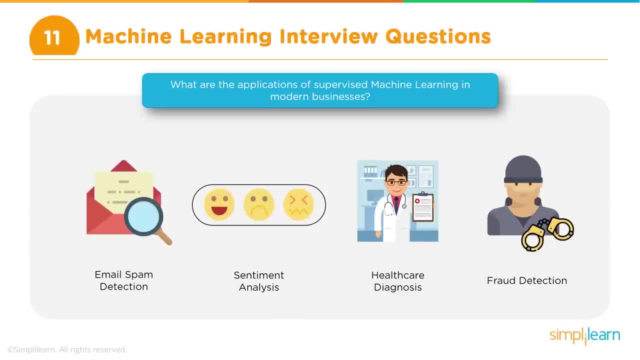 machine learning. The very common one is email spam detection, So you want to train your application or your system to detect between spam and non-spam. So this is a very common business application of supervised machine learning. So how does this work? The way it works is that you obviously have 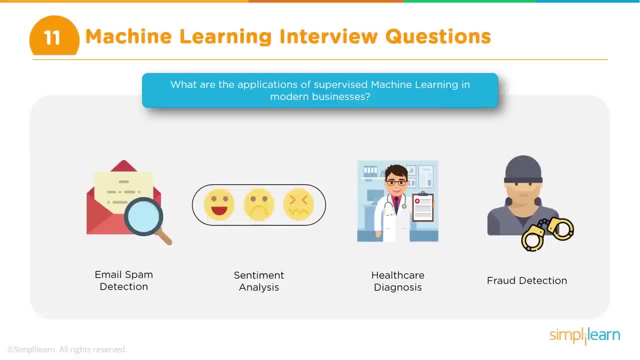 Historical data of all of your emails and they are categorized as spam and not spam. So that is what is the labeled information. And then you feed this information or all these emails as an input to your model right, And the model will then get trained to detect which of the emails are, to detect which is. 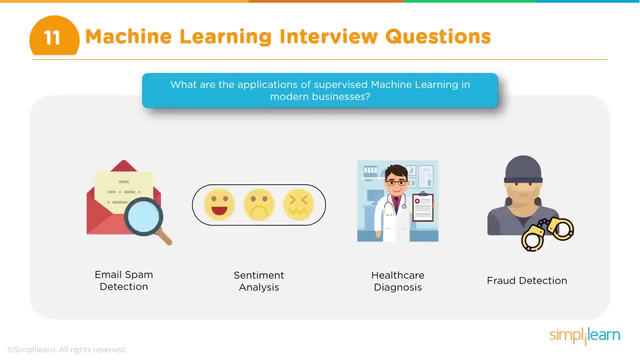 spam and which is not spam. So that is the training process and this is supervised machine learning, because you have labeled data, You already have emails Which are not spam, Which are tagged as spam or not spam, and then you use that to train your model, right? 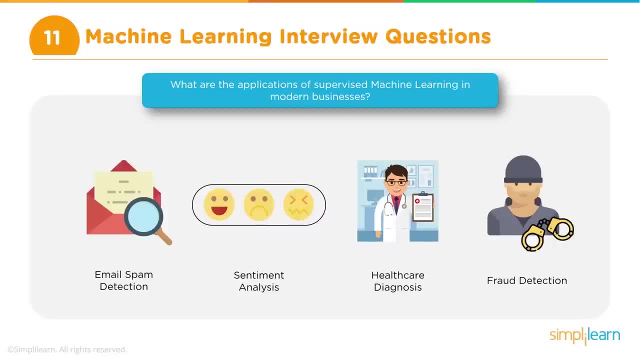 So this is one example. Now there are a few industry specific applications for supervised machine learning. One of the very common ones is in healthcare diagnostics. In healthcare diagnostics you have these images and you want to train models to detect whether, from a particular image, whether it can find out if the person is sick or not. 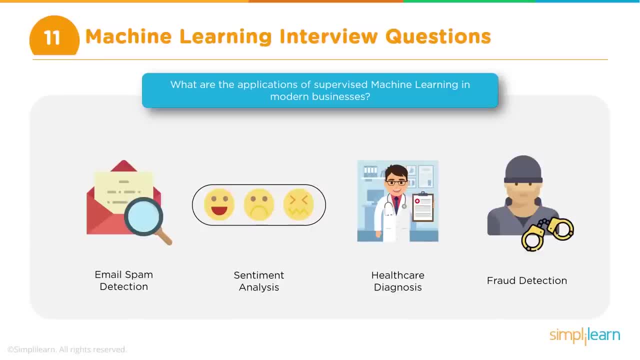 whether a person has cancer or not, right? So this is a very good example of supervised machine learning. Here, the way it works is that existing images- it could be x-ray images, it could be MRI or any of these images- are available and they are tagged saying that, okay, this x-ray image. 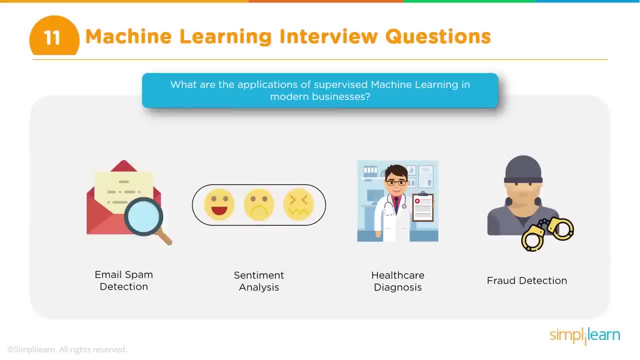 is defective, or the person has an illness, or it could be cancer, whichever illness, right? So it is tagged as defective or clear or good image and defective image, something like that. So we come up with a binary- or it could be multi-class as well- saying that this is defective. 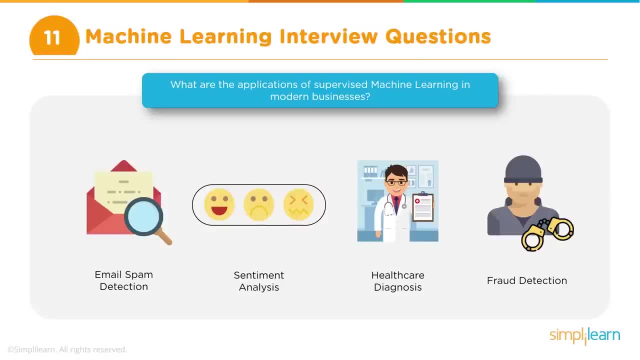 to 10%, this is 25% and so on. but let's keep it simple. You can give an example of just a binary classification. that would be good enough. So you can say that in healthcare diagnostics using image, we need to detect whether a person 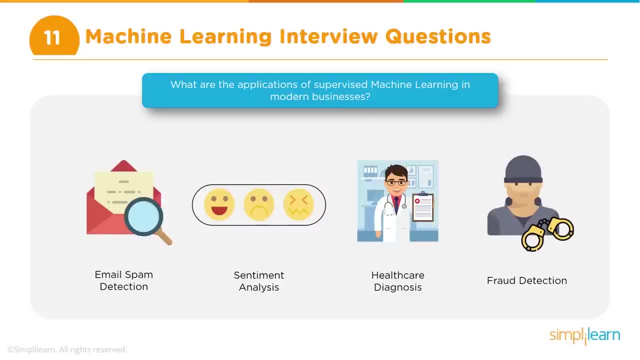 is ill or whether a person is having cancer or not. So here the way it works is you feed labeled images and you allow the model to learn from that so that when new image is fed it will be able to predict whether this person is having that illness or not, having cancer or not. right, 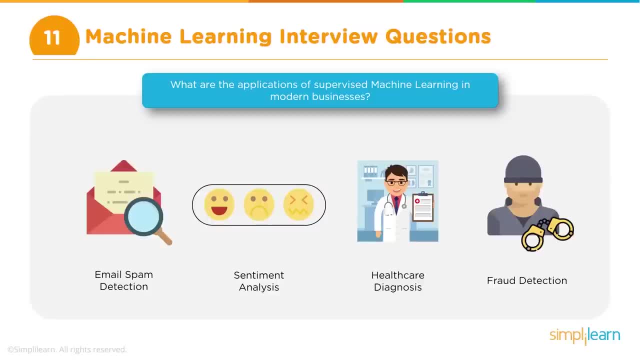 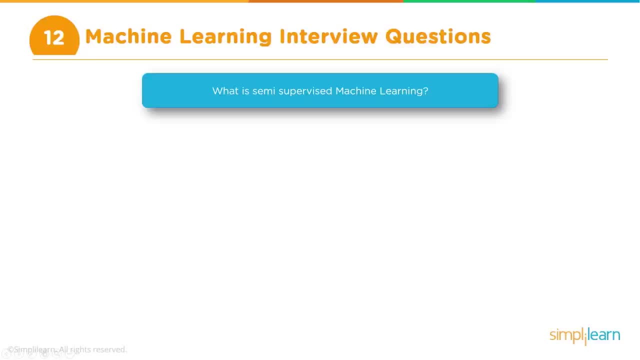 So I think this would be a very good example for supervised machine learning in modern business. All right, then we can have a question like: so we've been talking about supervised and unsupervised, and so there can be a question around semi-supervised machine learning. 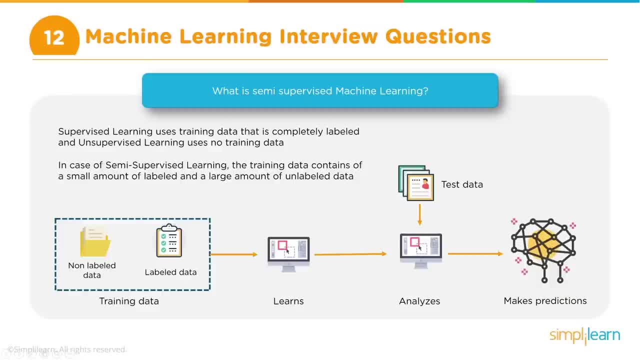 So what is semi-supervised machine learning? Now, Semi-supervised learning, Okay, So there are two things, such as it falls between supervised learning and unsupervised learning, but for all practical purposes it is considered as a part of supervised learning. 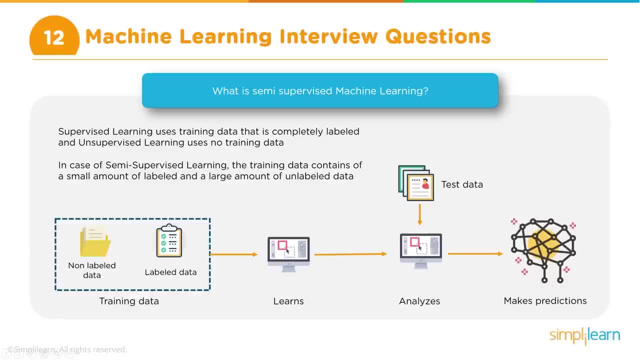 And the reason this has come into existence is that in supervised learning you need labeled data. So all your data for training, your model, has to be labeled. Now this is a big problem in many industries or in many under many situations getting 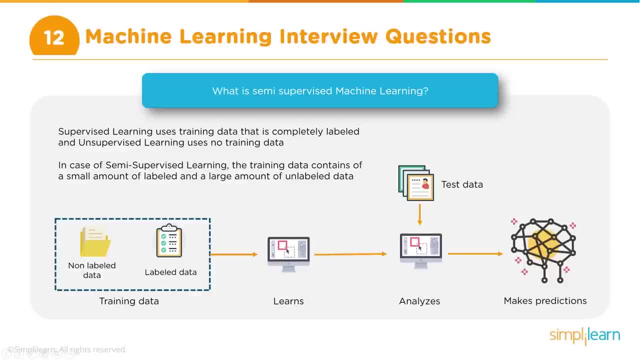 the labeled data. Yeah, It's not that easy because there's a lot of effort in labeling this data. Let's take an example of diagnostic images. We can just, let's say, take x-ray images. Now, there are actually millions of x-ray images available all over the world, but the problem 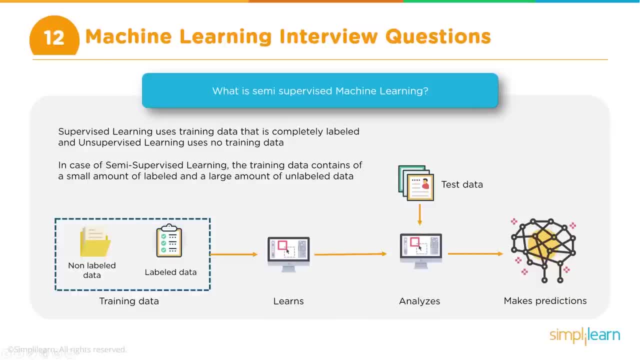 is, they are not labeled, So their images are there, but whether it is defective or whether it is good that information is not available along with it right In a form that it can be used by a machine, which means that somebody has to take a look. 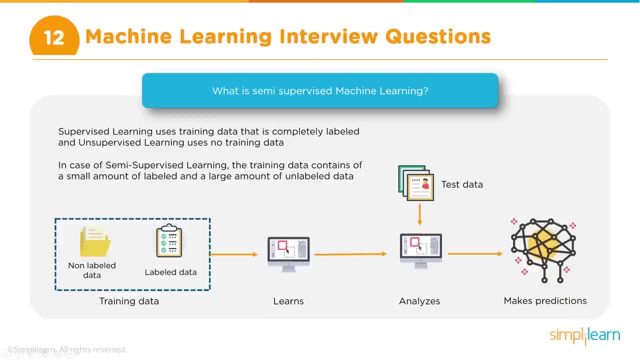 You take a look at these images and usually it should be like a doctor and then say that: okay, yes, this image is clean and this image is cancerous, and so on and so forth. Now, that is a huge effort by itself. So this is where semi-supervised learning comes into play. 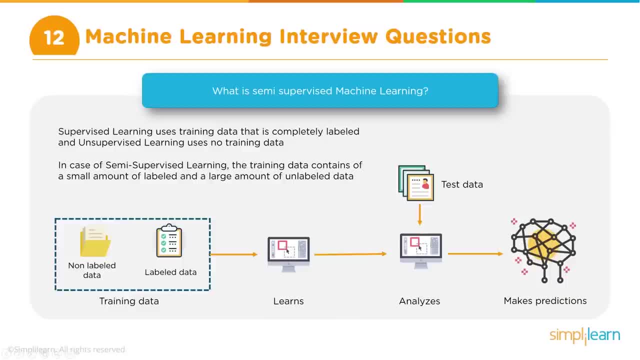 So what happens is there is a large amount of data, maybe a part of it is labeled. Then we try some techniques to label the remaining part of the data so that we get completely labeled data, and then we train our model. So I know this is a little long winding explanation, but unfortunately there is no quick and easy. 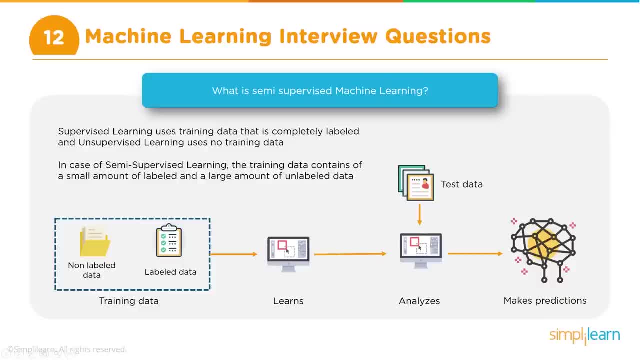 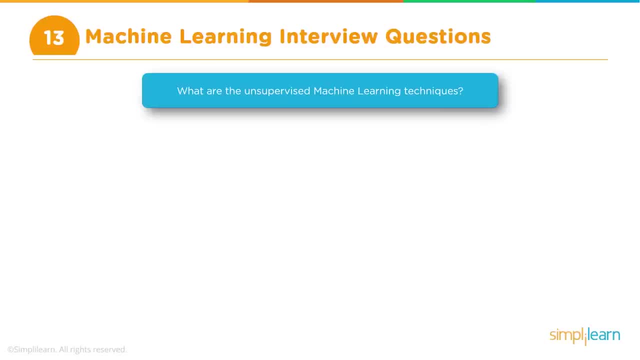 definition for semi-supervised machine learning. This is the only way, probably, to explain this concept. We may have another question as what are unsupervised machine learning techniques or what are some of the techniques used for performing unsupervised machine learning? So it can be worded in a different way. 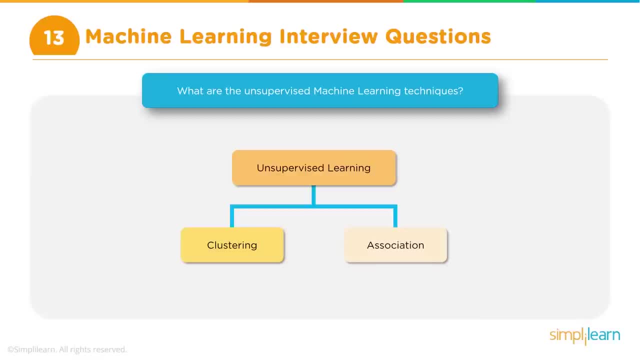 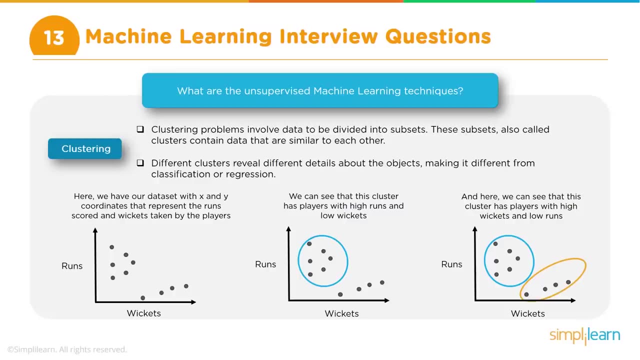 Okay, So how do we answer this question? So unsupervised learning. you can say that there are two types: clustering and association. And clustering is a technique where similar objects are put together and there are different ways of finding similar objects, So their characteristics can be measured and if they have most of the characteristics, 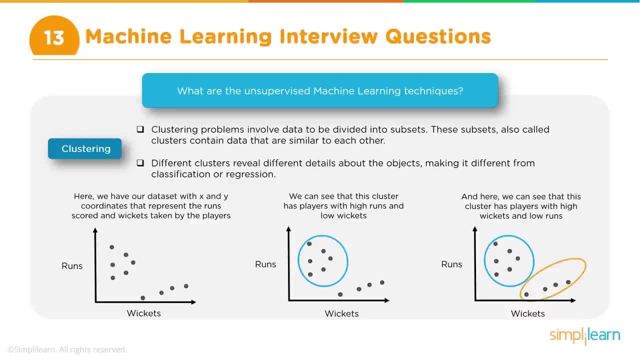 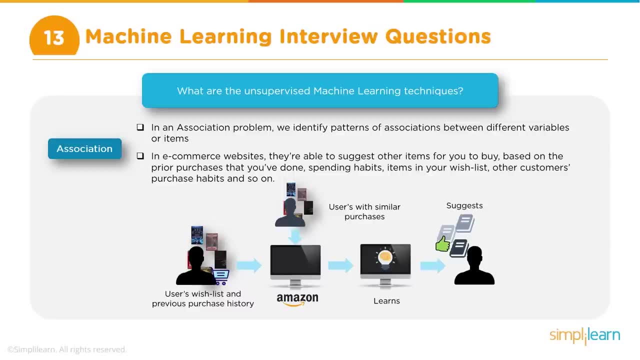 if they are similar, then they can be put together. This is clustering, Then association you can. I think the best way to explain association Is with an example. in case of association, you try to find out how the items are linked. 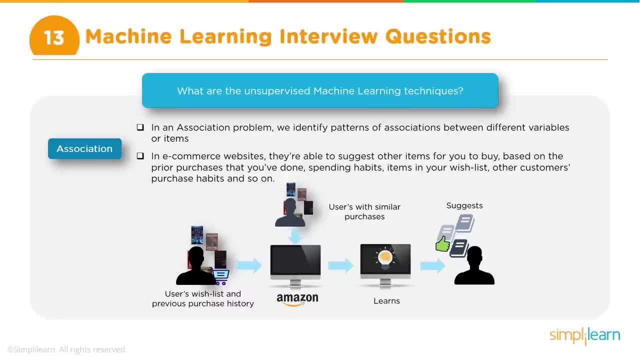 to each other. So, for example, if somebody bought, maybe, a laptop, the person has also purchased a mouse. So this is more in an e-commerce scenario, for example, so you can give this as an example. So people who are buying laptops are also buying a mouse. 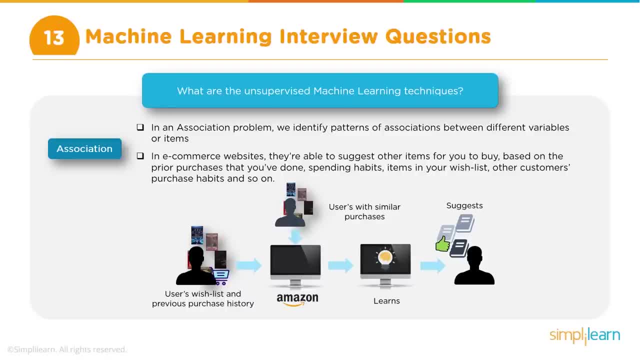 So that means there is an association between laptops and mouse. Or maybe people who are buying bread are also buying butter, So that is a association that can be created. So this is unsupervised learning one of the techniques. Okay, All right. 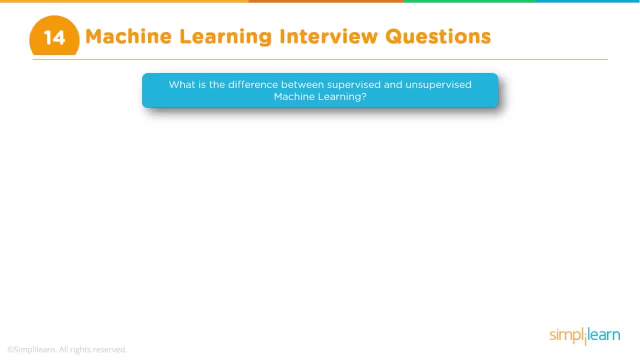 Then we have a fundamental question: What is the difference between supervised and unsupervised machine learning? So, machine learning, these are the two main types of machine learning: supervised and unsupervised. And in case of supervised- and again here probably the key word that the person may- 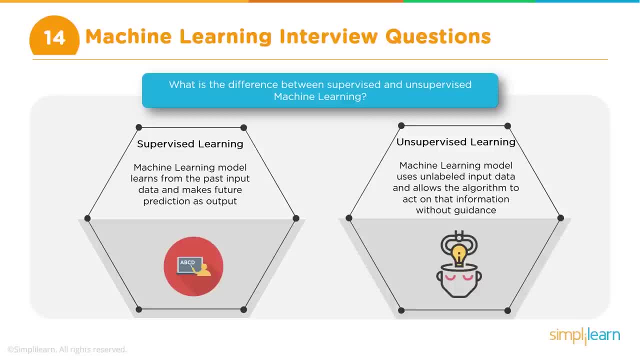 be wanting to hear is labeled data. Now, very often people say we have historical data and if we run it it is supervised, And if we don't have historical data, yes, but you may have historical data, but if it is not labeled, then you cannot use it for supervised learning. 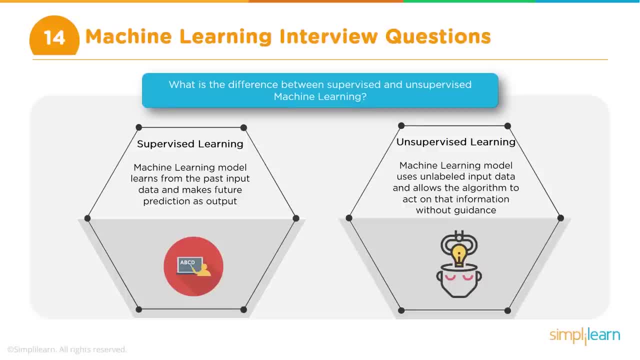 So it is. it's very key to understand that we put in that keyword labeled okay. So when we have labeled data for training our model, then we can use supervised learning, And if we do not have labeled data, then we use supervised learning. 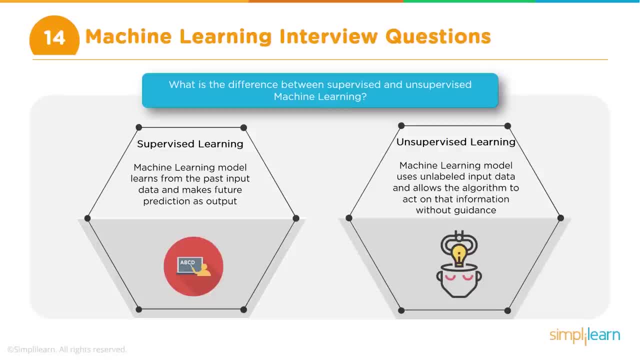 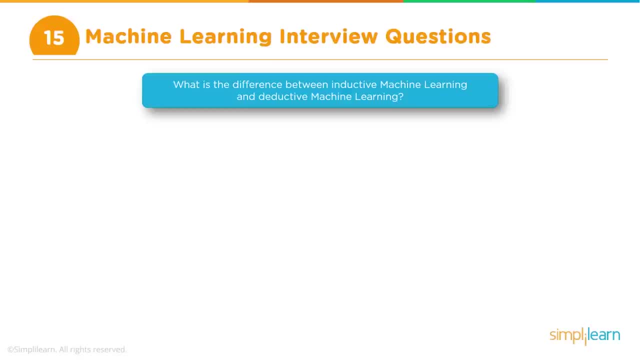 Okay. Okay, Then we use unsupervised learning, And there are different algorithms available to perform both of these types of trainings. So there can be another question a little bit more theoretical and conceptual in nature. This is about inductive machine learning and deductive machine learning. 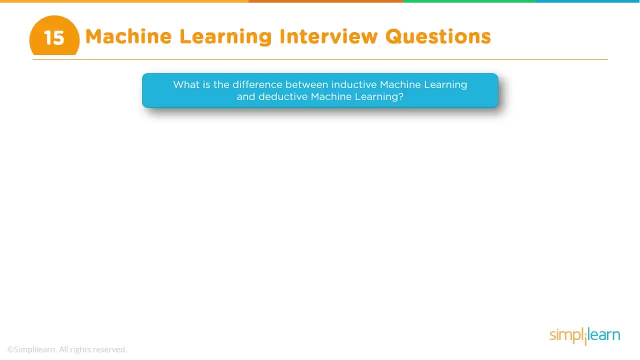 So the question can be: what is the difference between inductive machine learning and deductive machine learning, or somewhat in that manner, so that the exact phrase or exact question can vary. They can ask for examples and things like that, but that could be the question. 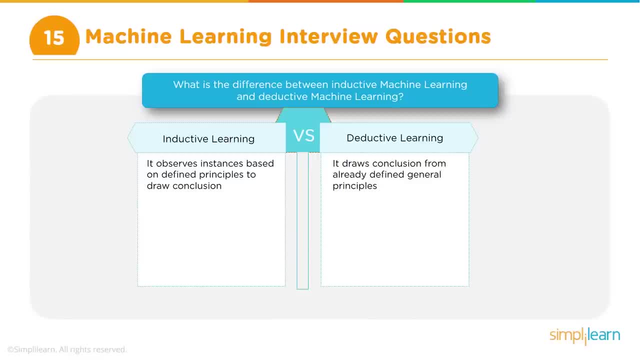 So let's first understand what is inductive and deductive training. Inductive training is induced by somebody and you can illustrate that with a small example. I think that always helps. So whenever you're doing some explanation, try as much as possible, as I said, to give. 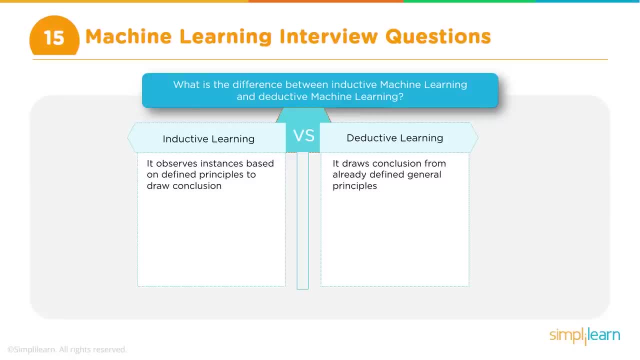 examples from your work experience or give some analogies, and that will also help a lot in explaining as well and for the interviewer also to understand. So here we'll take an example. Okay, So we'll take an example, or rather we will use an analogy. 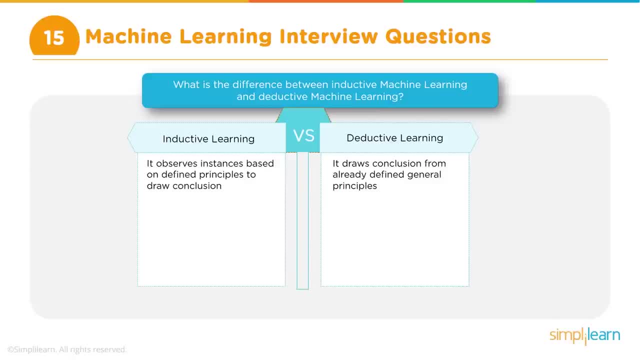 So inductive training is when we induce some knowledge or the learning process into a person without the person actually experiencing it. What can be an example? So we can probably tell the person, or show a person a video, that a fire can burn, burn his finger or fire can cause damage. 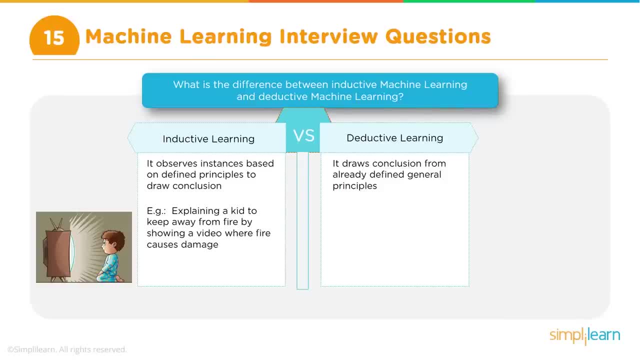 So what is happening here? This person has never probably seen a fire Or never seen anything getting damaged by fire. But just because he has seen this video, he knows that, okay, fire is dangerous And if a fire can cause damage, right. 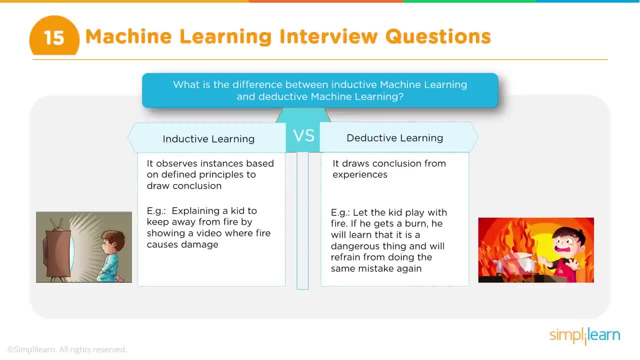 So this is inductive learning. compared to that, what is deductive learning? So here you draw conclusion, or the person draws conclusion out of experience. So we will stick to the analogy. So, compared to the showing a video, let's assume a person is allowed to play with fire. 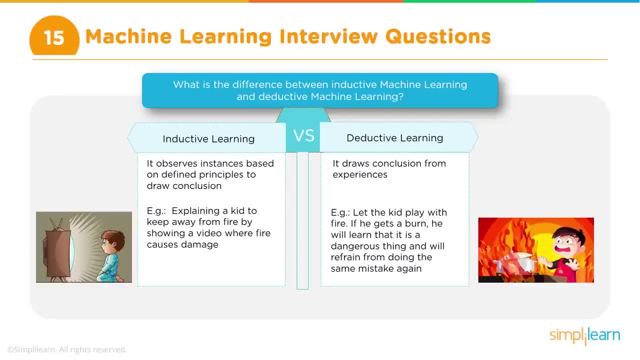 right. And then he figures out that if he puts his finger, it's burning, or if throw something into the fire, it burns. So he is learning through experience. So this is known as deductive learning. okay, So you can have applications or models that can be trained using inductive learning or 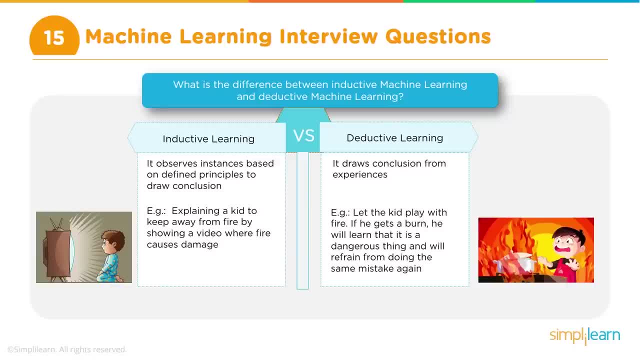 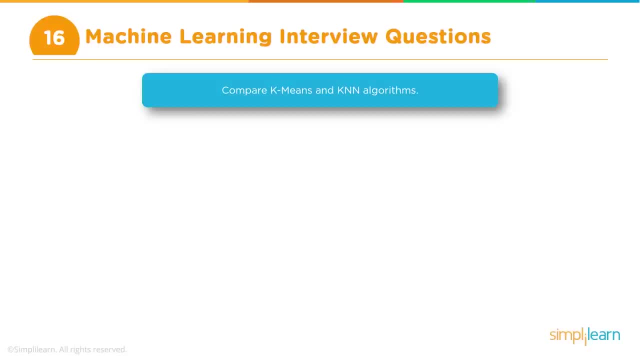 deductive learning. All right, I think probably that explanation will be sufficient. The next question is: are KNN and K-means clustering similar to one another? Or are they similar? Are they same right? Because that the letter K is kind of common between them. okay. 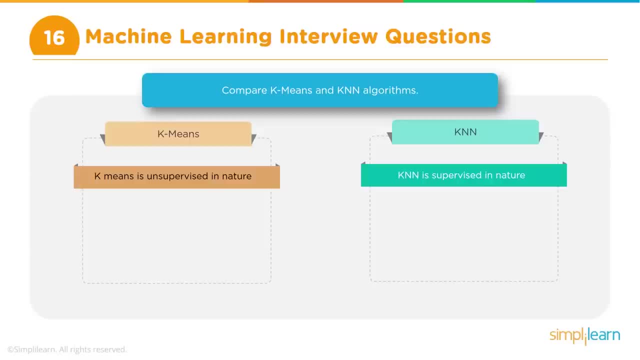 So let us take a little while to understand what these two are. One is KNN and another is K-means. KNN stands for K- nearest neighbors, and K-means, of course, is the clustering mechanism. Now, these two are completely different, except for the letter K being common between them. 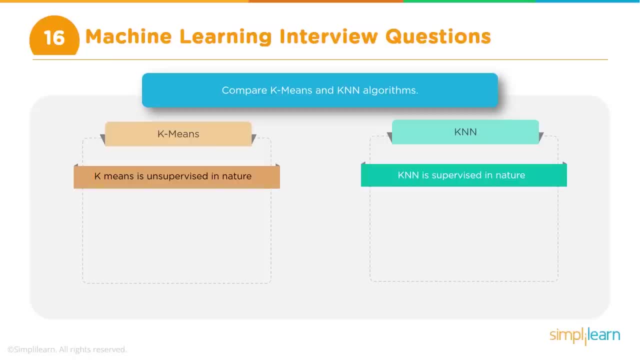 KNN is completely different. K-means clustering is completely different. KNN is a classification process And therefore it comes under supervised learning, whereas K-means clustering is actually unsupervised. Okay, When you have KNN, when you want to implement KNN, which is basically K- nearest neighbors- 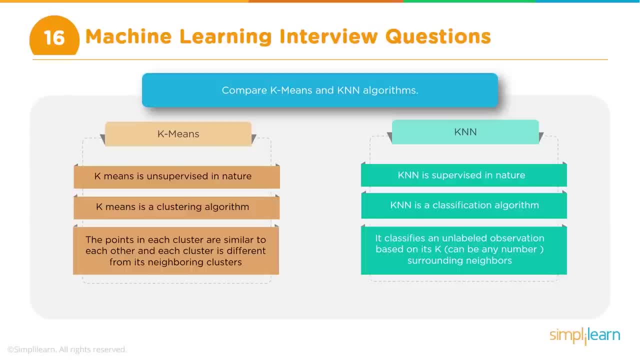 the value of K is a number, So you can say K is equal to 3,. you want to implement KNN with K is equal to 3.. So, which means that it performs the classification in such a way that how does it perform the? 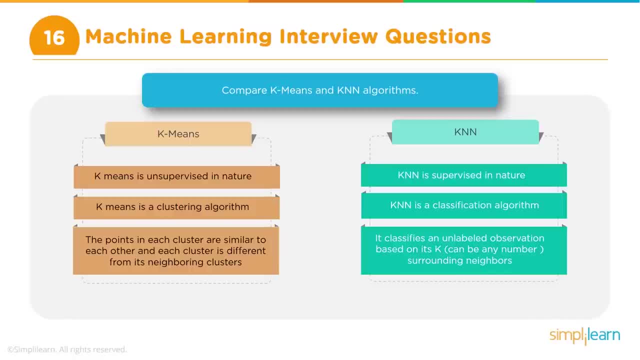 classification. So it will take three nearest objects. Okay, That's why it's called nearest neighbor. So basically, based on the distance, it will try to find out its nearest objects, that are, let's say, three of the nearest objects, and then it will check whether the class they. 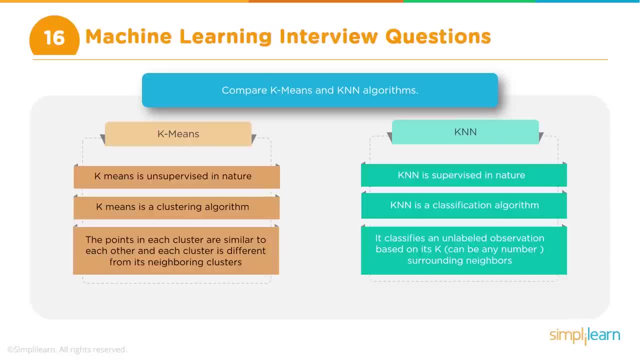 belong to which class, right? So if all three belong to one particular class, obviously this new object is also classified as that particular class. but it is possible that they may be from two or three different classes. Okay, So let's say they are from two classes, and then if they are from two classes, now, usually 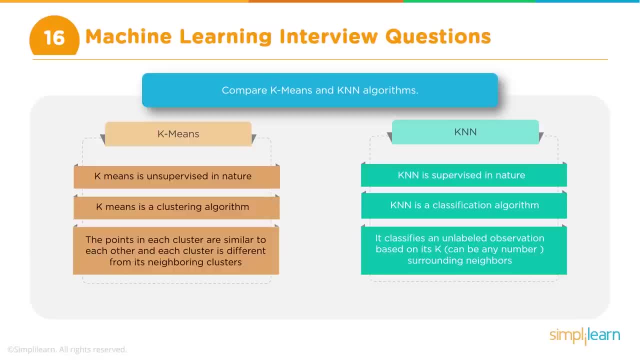 you take an odd number, you assign an odd number to. so if there are three of them and two of them belong to one class and then one belongs to another class, So this new object is assigned to the class to which the two of them belong. 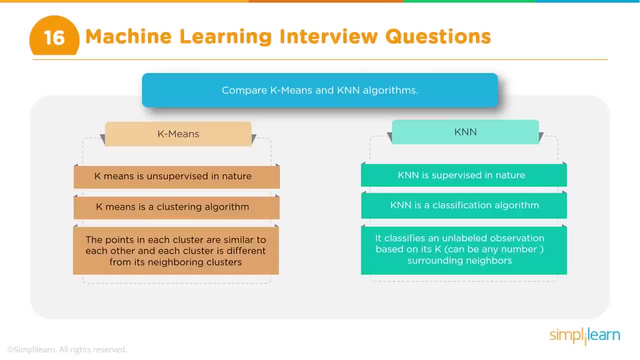 Now, the value of K is sometimes tricky: whether should you use three, should you use five, Should you use seven? That can be tricky because the ultimate classification can also vary. So it's possible that if you're taking K as three, the object is probably in one particular class. 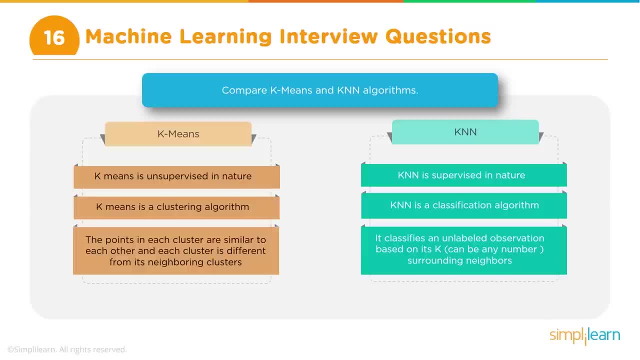 But if you take K is equal to five, maybe the object will belong to a different class, because when you're taking three of them, probably two of them belong to class one and one belong to class two, Whereas when you take five of them, it is possible that only two of them belong to class. 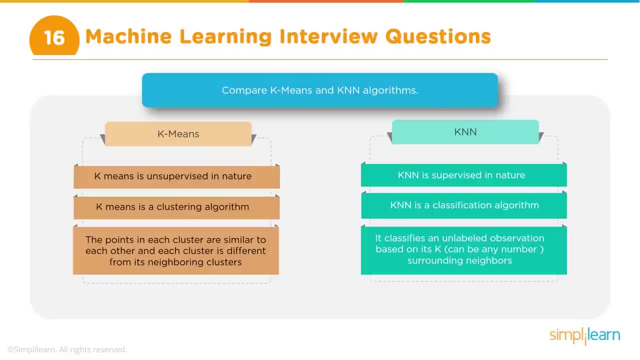 one and three of them belong to class two. So, which means that this object will belong to class two, right? So you see that. So it is. the class allocation can vary depending on the value of K. Okay Now, K means, on the other hand, is a clustering process, and it is unsupervised. where what? 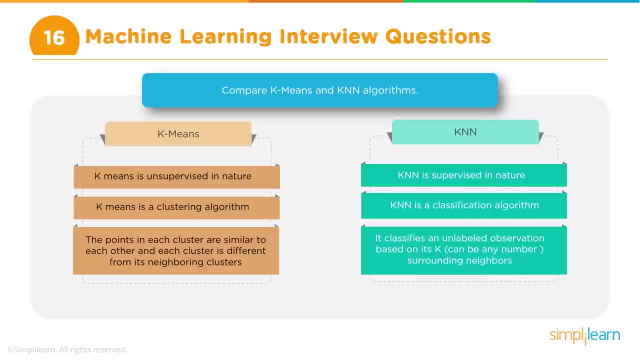 it does is the system will basically identify how the objects are, how close the objects are with respect to some of their features. Okay, And but the similarity, of course, is the letter K, And in case of K means also we specify its value, and it could be three or five or seven. 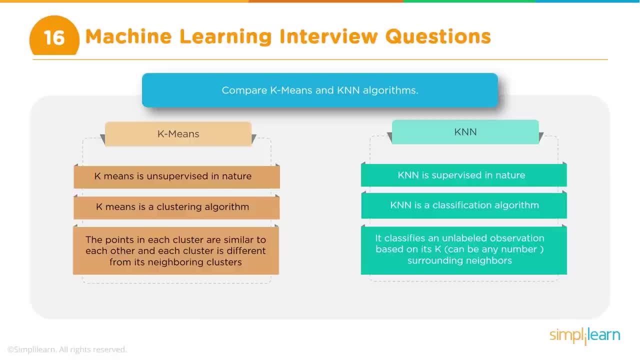 There is no technical limit as such, but it can be any number of clusters that you can create. Okay, So based on the value that you provide, the system will create that many clusters of similar objects. So there is a similarity to that extent that K is a number in both the cases, but actually 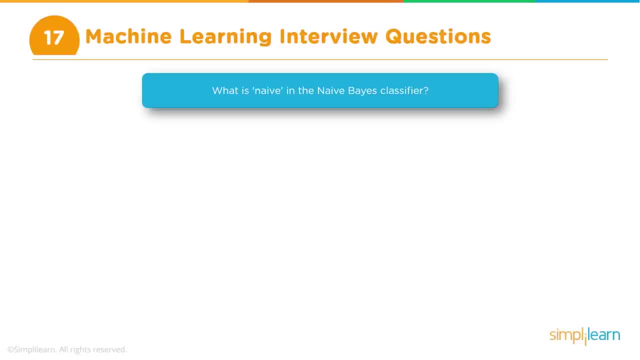 these two are completely different processes. We have what is known as naive Bayes classifier, and people often get confused, thinking that naive Bayes is the name of the person who found this classifier or who developed this classifier, which is not a hundred percent true. 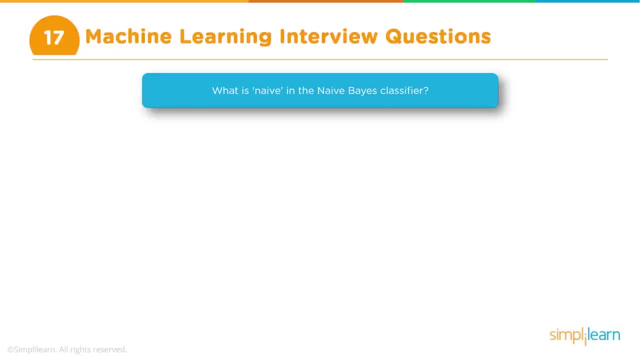 Bayes is the name of the person, BA Y S Is the name of the person, But naive is not the name of the person, right? So naive is basically an English word And that has been added here because of the nature of this particular classifier. 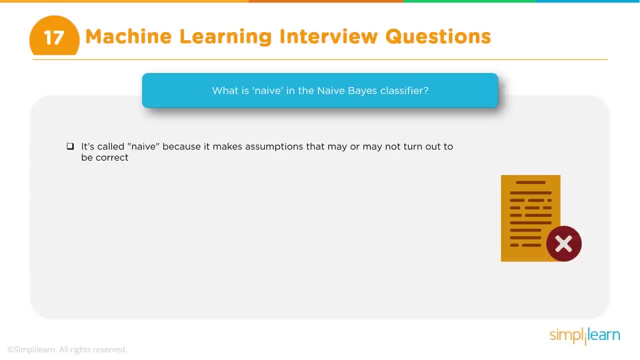 Naive Bayes classifier is a probability based classifier And it makes some assumptions that presence of one feature of a class is not related to the presence of any other feature of maybe other classes. right So, which is not very strong or not a very 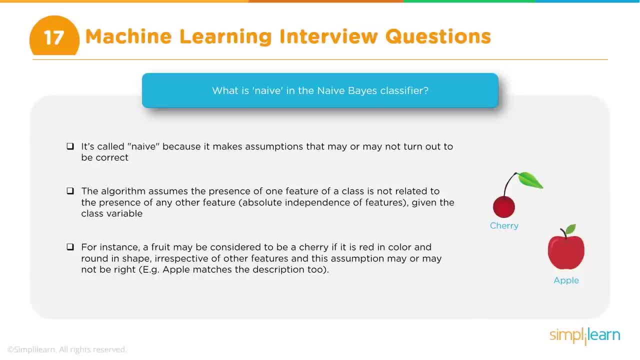 What do you say? accurate assumption, because these features can be related and so on. But even if we go with this assumption, this whole algorithm works very well, even with this assumption, and that is the good side of it. But the term comes from that. 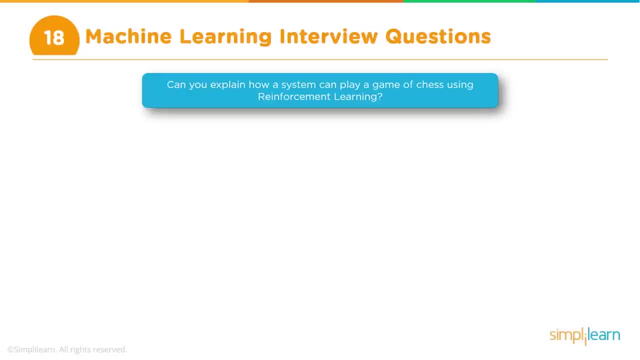 So that is the explanation that you can. then there can be question around reinforcement learning. It can be paraphrased in multiple ways. One could be: can you explain how a system can play a game of chess using reinforcement learning? Or it can be any. 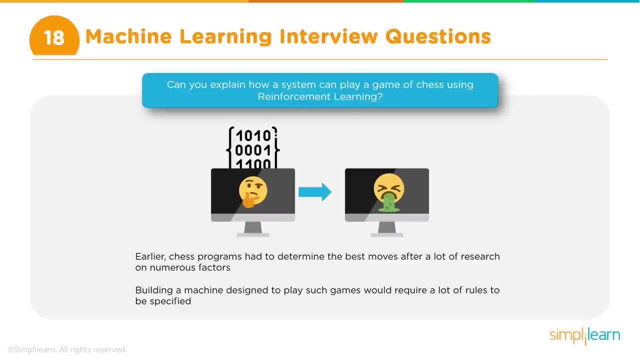 So the best way to explain this is again to talk a little bit about what reinforcement learning is about and then elaborate on that to explain the process. So, first of all, reinforcement learning has an environment and an agent, and agent is basically performing some actions in order to achieve a certain goal. 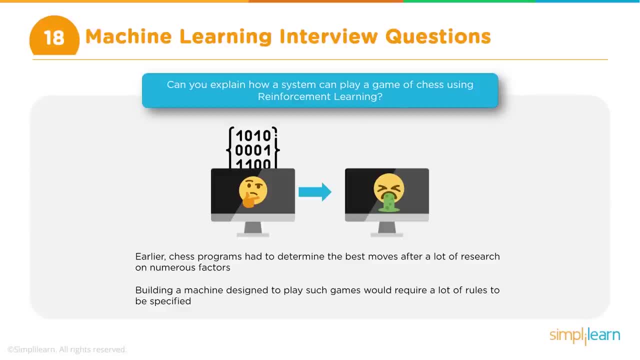 And this goals can be anything either. If it is related to game, then the goal could be that you have to score very high, score high, value high. Or it could be that your number of lives should be as high as possible. Don't lose life. 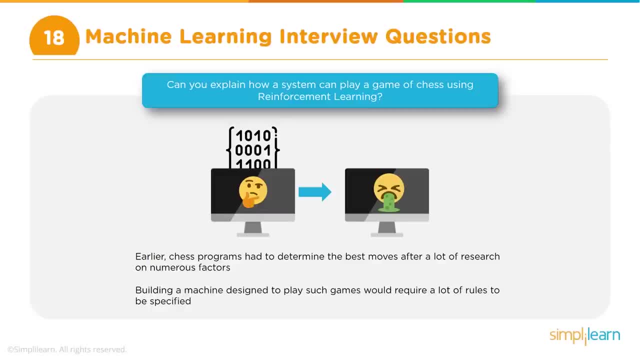 So these could be some of them. A more advanced examples could be for driving the automotive industry: self-driving cars. They actually also make use of reinforcement learning to teach the car how to navigate through the roads, and so on and so forth. That is also another example. 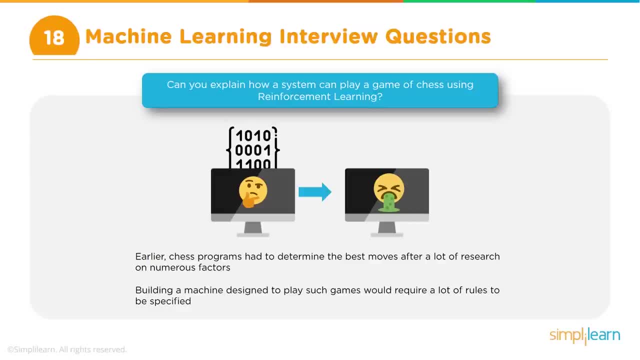 Now, how does it work? So if the system is basically there is an agent and environment, And every time the agent Takes a step or performs a task which is taking it towards the goal, the final goal, let's say to maximize the score, or to minimize the number of lives and so on, or minimize the debts, for 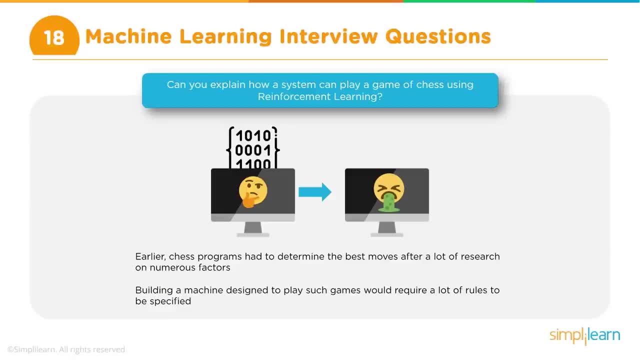 example, it is rewarded and every time it takes a step which goes against that goal and contrary or in the reverse direction, it is penalized. Okay, So it is like a carrot and stick system. Now, how do you use this to create a game of chess or to create a system to play a game of chess? 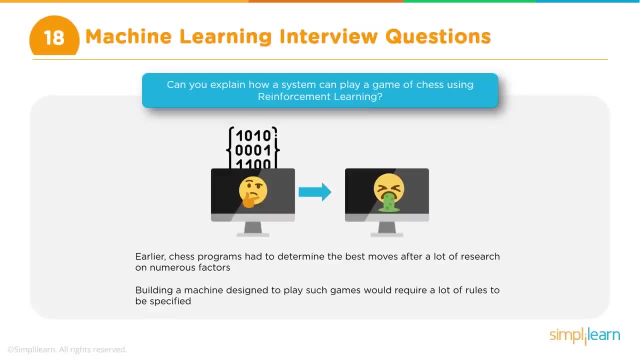 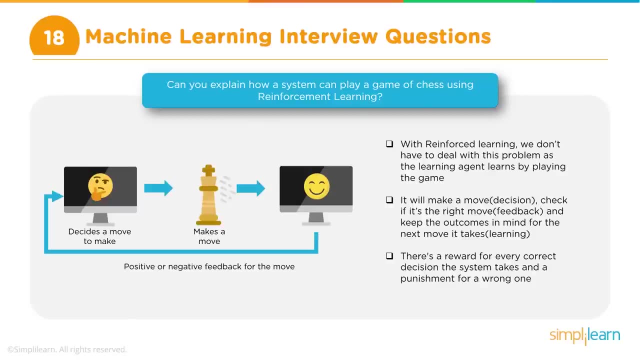 Now the way this works is- and this could probably go back to this AlphaGo example, where AlphaGo defeated a human champion- So the way it works is in reinforcement learning. the system is allowed. for example, in this case we are talking about chess- 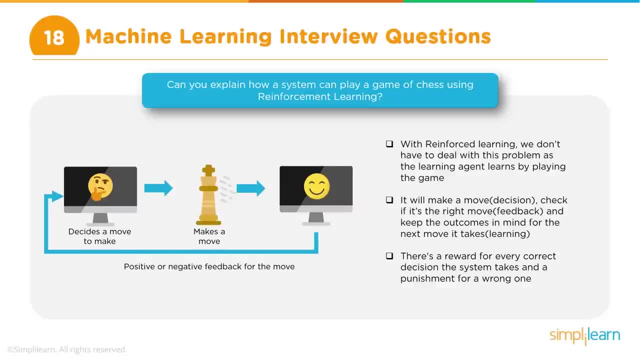 So we allow the system to first of all watch playing a game of chess. So it could be with a human being, or it could be the system itself. There are computer games of chess right. So either this new learning system, 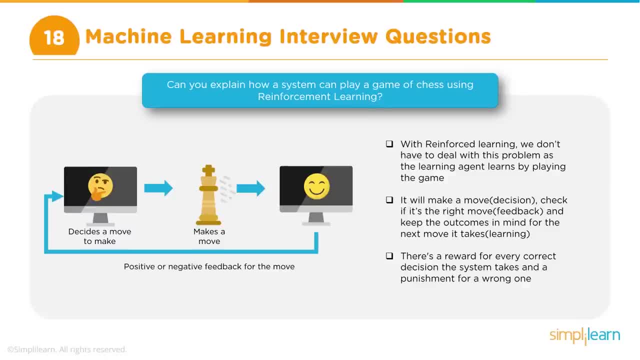 The system has to watch that game or watch a human being play the game, because this is reinforcement. learning is pretty much all visual. So when you're teaching the system to play a game, the system will not actually go behind the scenes to understand the logic of your software, of this game or anything like that. 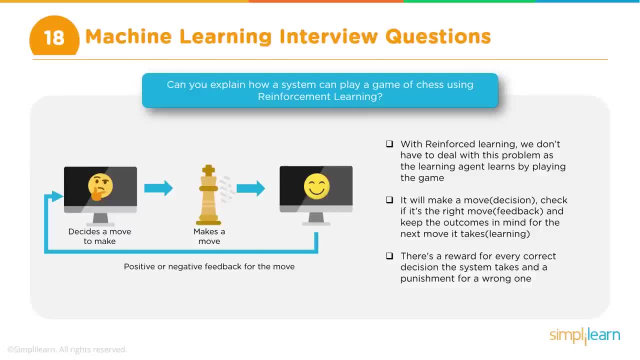 It is just visually watching the screen and then it learns. Okay, So reinforcement learning to a large extent works on that. So you need to create Mechanism whereby your model will be able to watch somebody playing the game and then you allow the system also to start playing the game. 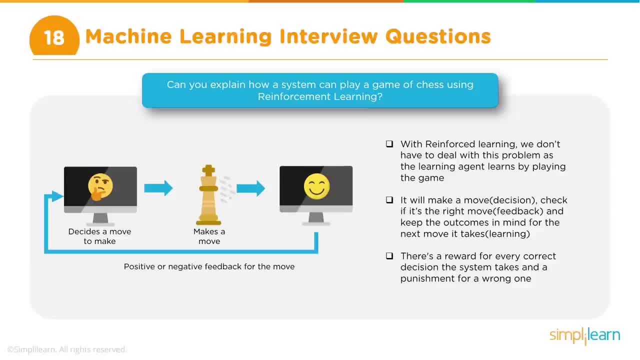 So it pretty much starts from scratch. Okay, And as it moves forward it's right. at the beginning the system really knows nothing about the game of chess. Okay, So initially it is a clean slate. It just starts by observing how you're playing, so it will make some random moves. 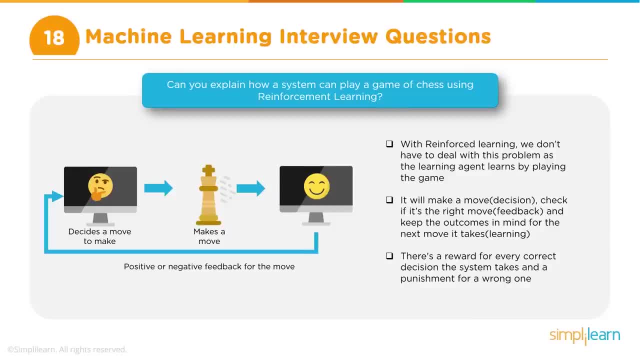 And keep losing badly, But then what happens is over a period of time. so you need to now allow the system or you need to play with the system, not just one, two, three, four or five times, but hundreds of times, thousands of times, maybe even hundreds of thousands of times. 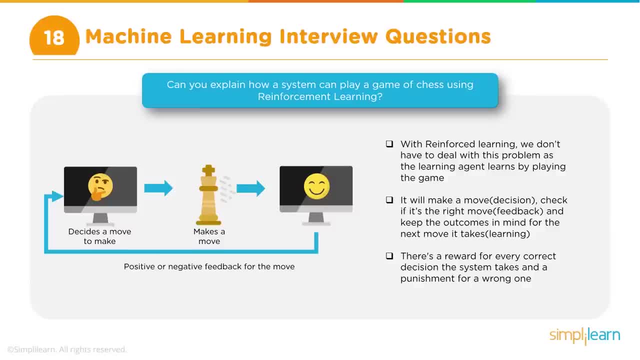 And that's exactly how AlphaGo has done. It played millions of games between itself and the system right. So for the game of chess also, you need to do something like that. You need to allow the system to play chess And then learn on its own over a period of repetition. 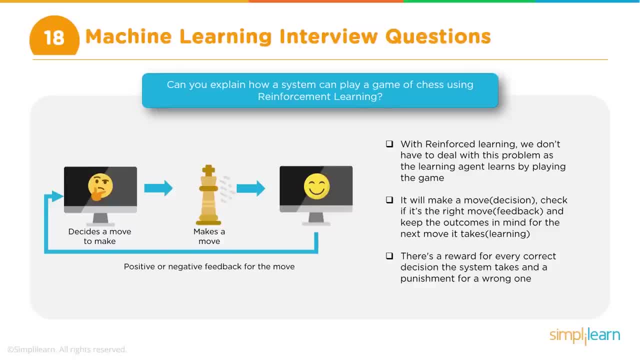 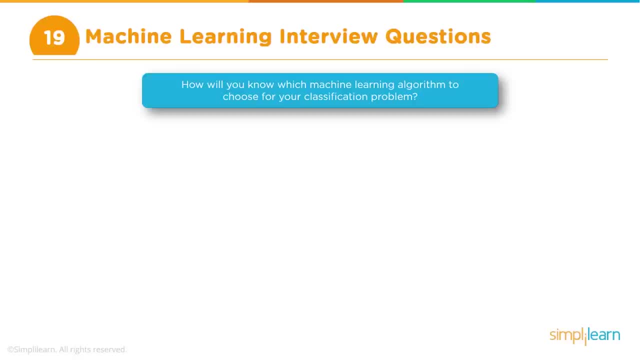 So I think you can probably explain it to this much to this extent, and it should be sufficient. Now this is another question which is again somewhat similar, but here the size is not coming into picture. So the question is: how will you know which machine learning algorithm to choose for your classification problem? 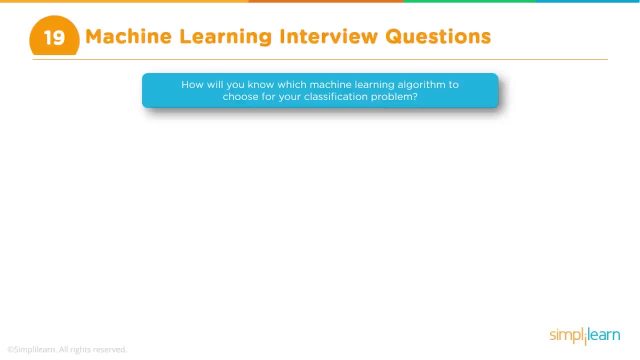 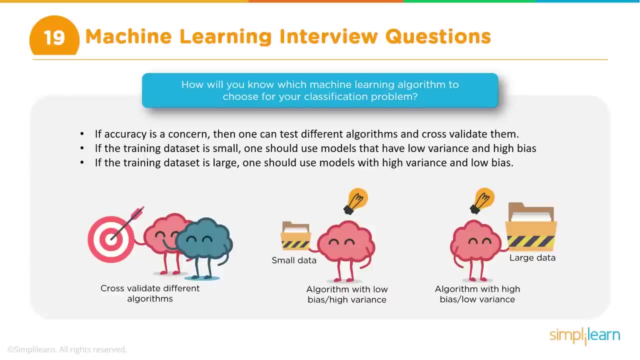 Now, this is not only classification problem. It could be a regression problem. I would like to generalize this question. So if somebody asks you, how will You choose, how will you know which algorithm to use? The simple answer is: there is no way you can decide exactly, saying that this is the algorithm I'm going to use in a variety of situations. 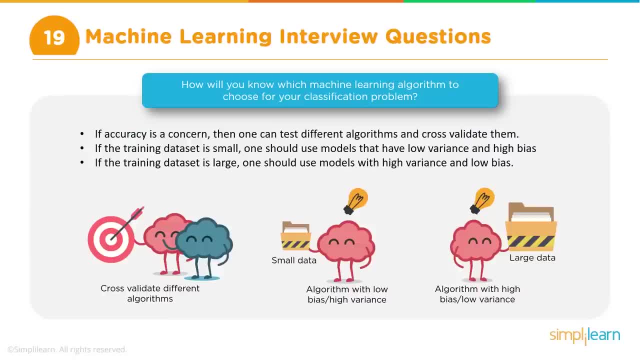 There are some guidelines like, for example: you will obviously, depending on the problem, you can say whether it is a classification problem or a regression problem, And then, in that sense you are kind of restricting yourself to: if it is a classification problem- there are, you can only apply a classification algorithm, right? 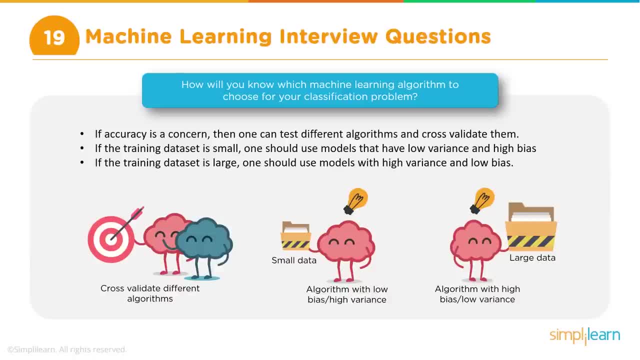 To that extent you can probably, let's say, limit the number of algorithms. But now, within the classification algorithms you have decision trees, you have SVM, you have logistic regression. Is it possible to outright say yes for this particular problem? 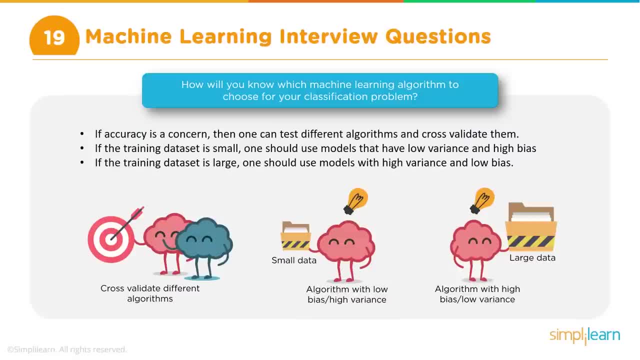 Since you have explained this, now this is the exact algorithm that you can use. That is not possible. Okay, so we have to try out a bunch of algorithms, see which one gives us the best performance and best accuracy, And then Decide to go with that particular algorithm. 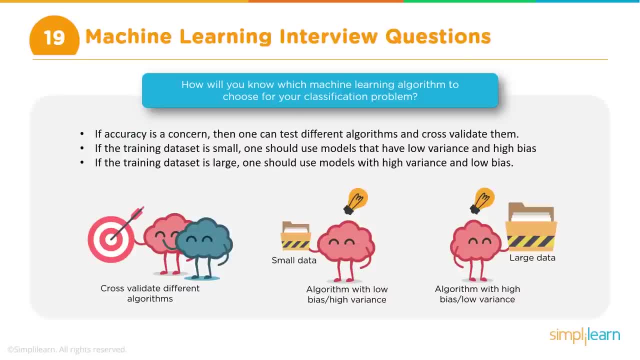 So in machine learning a lot of it happens through trial and error. There is no real possibility that anybody can, just by looking at the problem or understanding the problem, tell you that okay, in this particular situation, this is exactly the algorithm that you should use. 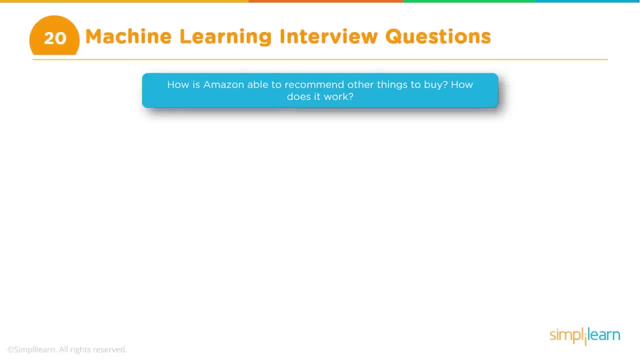 Then the questions may be around application of machine learning, And this question is specifically around how Amazon is able to recommend other things to buy. So this is around Recommendation engine: How does it work, How does the recommendation engine work? So this is basically the question is all about. 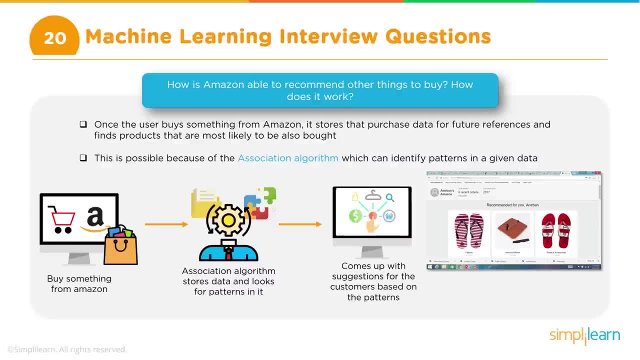 So the recommendation engine again works based on various inputs that are provided. Obviously, something like, you know, Amazon. a website or e-commerce site like Amazon- collects a lot of data around the customer behavior- Who is purchasing what, And if somebody is buying a particular thing, they're also buying something else. 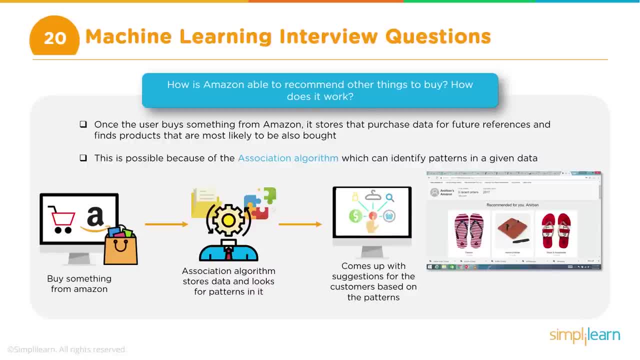 So this kind of association right. So this is the answer. As for supervised learning we talked about, they use this to associate and link or relate items, and that is one part of it. So they kind of build association between items, saying that somebody buying this is also buying this. 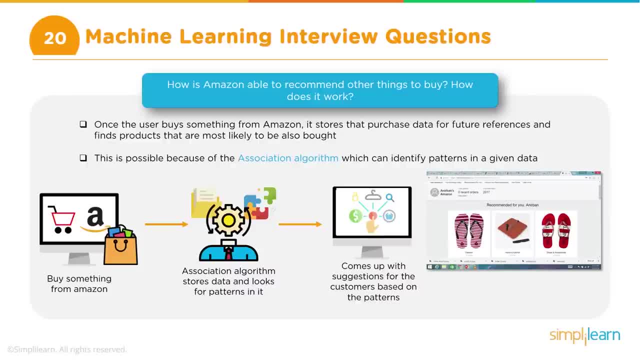 That is one part of it. Then they also profile the users right based on their age, their gender, their geographic location. They will do some profiling And then, when somebody is logging in and when somebody is shopping, the kind of mapping of these two things are done. 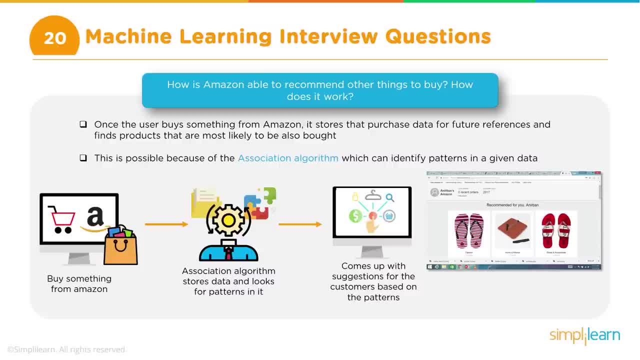 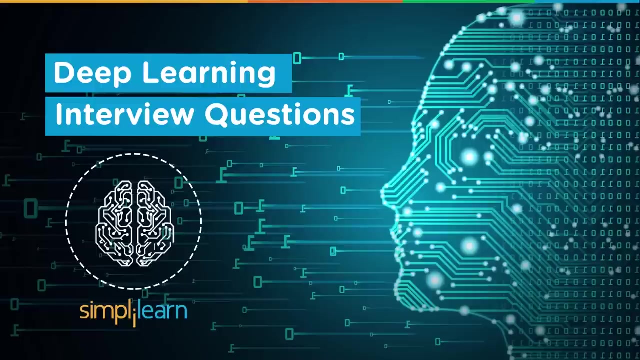 to identify. obviously, if you have logged in, then they know who you are and your information is available, like, for example, your age, maybe your gender, and where you're located, what you purchased earlier, right? so all this is taken and the recommendation engine basically uses all this information and comes up with recommendations for a particular user. today, we're going to help you. 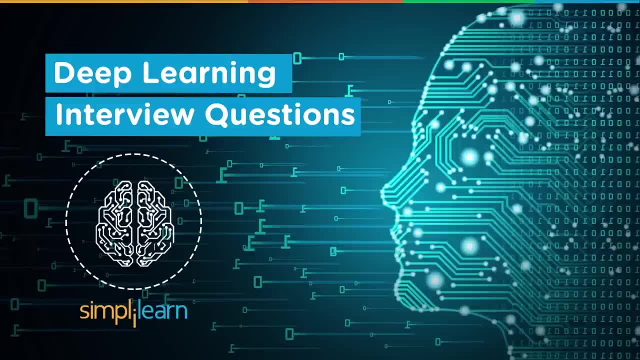 prepare for interview questions dealing with deep learning, and we're going to go from the very basics of neural networks and deep learning into some of the more commonly used models so you can have an understanding of what kind of questions are going to come up and what you need to know. 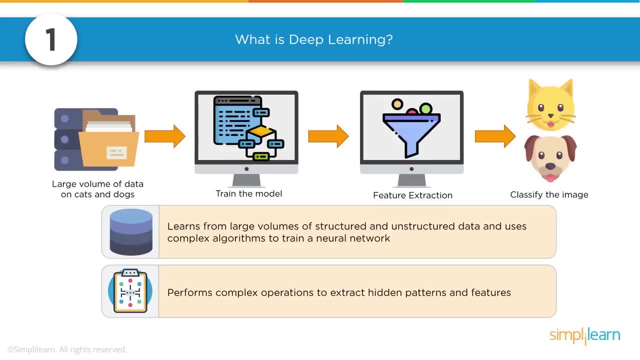 in interview questions. we'll start with a very general concept of what is deep learning. this is where we take large volumes of data, in this case on cats and dogs or whatever. a lot of times you use a training setup to train your model, remember. it's kind of like a magic black box. 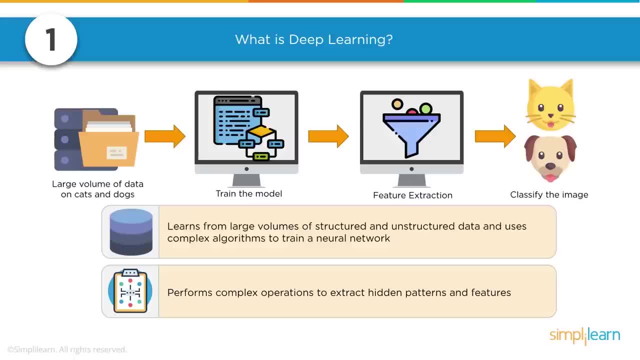 going on there. then we use that to extract features or extract information- in this case, classify the image of a cat and a dog. so the primary takeaway we're talking about deep learning is it learns from large volumes of structured and even unstructured data and uses complex algorithms to train neural network. it also performs complex operations to extract hidden. 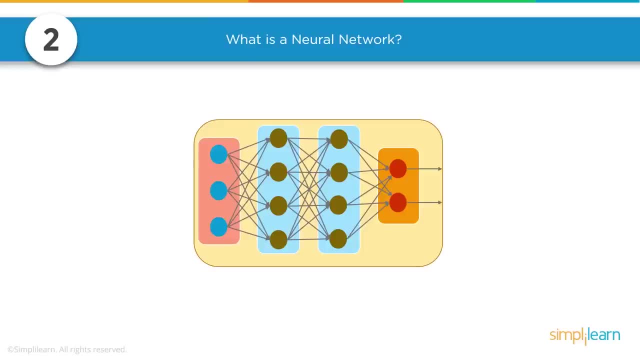 patterns and features and if we're going to discuss deep learning in this very simplified overview and we also have to go over what is a neural network. this is a common image you'll see of a drawing of a cat and a dog, and it's it's a human brain inspired system which replicate the way humans 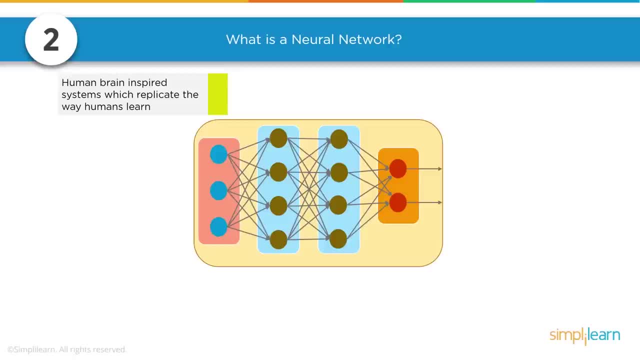 learn. so this is inspired how our own neurons in our brain fire, but at a much simplified level. obviously it's not ready to take over the human population and be our leader yet- not for many years. it's very much in its infant stage, but it's inspired by how our brains work and they use a lot. 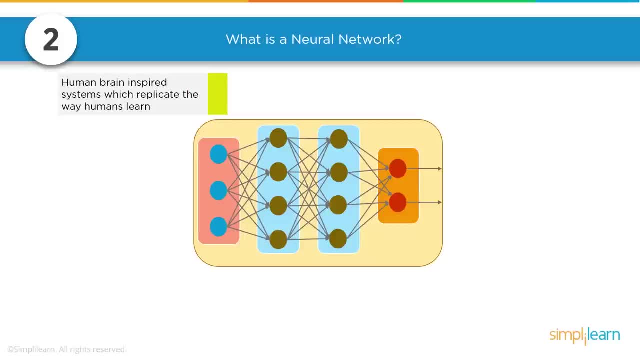 of other inspirations. you can study brains of moths and other animals that they've used to figure out how to improve these neural networks. the most common one consists of three layers of network, and this is generally how you view these networks: is you have an input? you have a hidden? 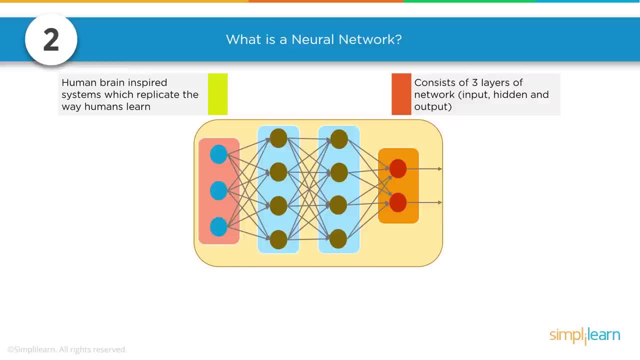 layer and an output and the neural network is broken up into many pieces. but we focus just on the neural network. it's always on the hidden layers that we're making all the adjustments and figuring out how to best set up those hidden layers for their functions, to both train faster 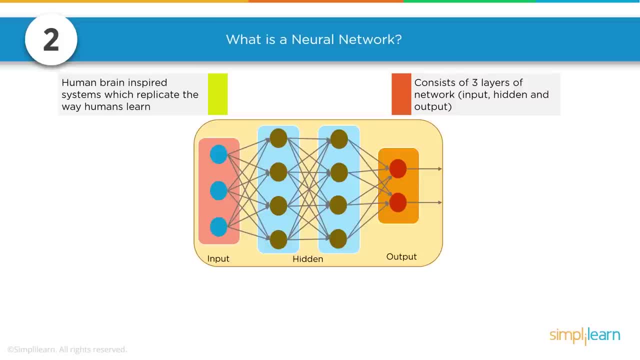 and to function better. when we look at this, of course, we have our input, hidden and output. each layer contains neurons called as nodes, perform various operations and you can see here we have the list of the nodes. we have both our input nodes and our output notes, and then our hidden layer notes and it's used in deep learning algorithm like CNN, RNN, GAN, etc. we'll 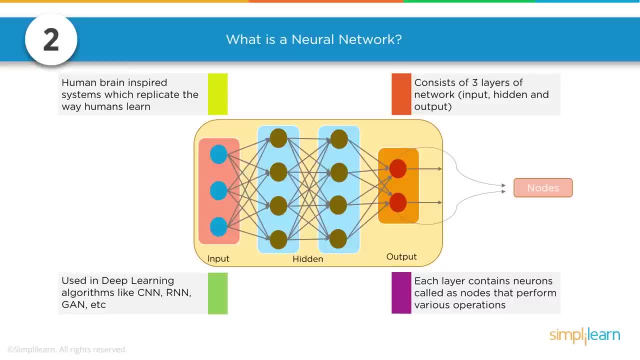 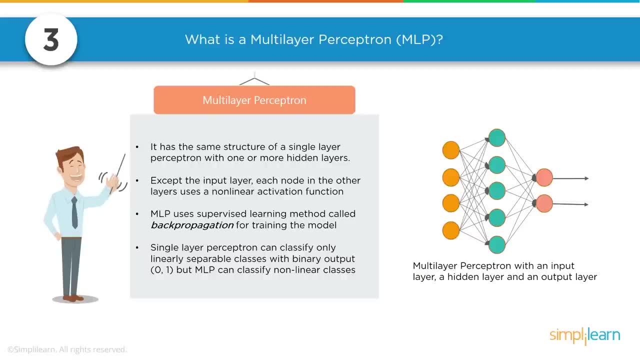 address some of these models a little closer, at least the most common models, as we go down the list and we study the deep learning and the neural network framework. let's start with what is a multi-layer perceptron, or MLP? a lot of time is it referred to and you'll see these abbreviations. 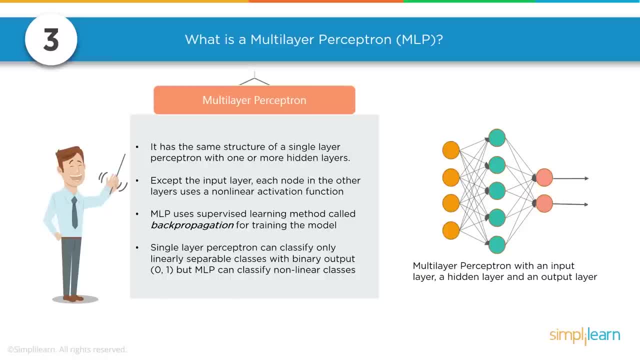 I'll be honest, I have to write them down on a piece of paper and go through them, because I never remember what they all mean, even though I play with them all the time. what is a multi-layer perceptron? well, if you look at the image on the right, it's very. 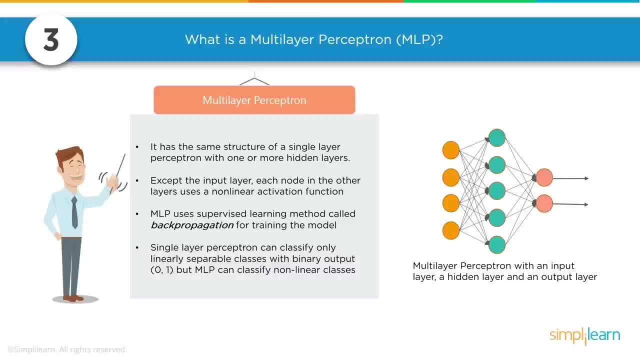 similar to what we just looked at. you have your input layer, your hidden layer and your output layer, and that's exactly what this is. it has the same structure of a single layer, perceptron, with one or more hidden layers. except the input layer, each node in the other layers uses a non-linear 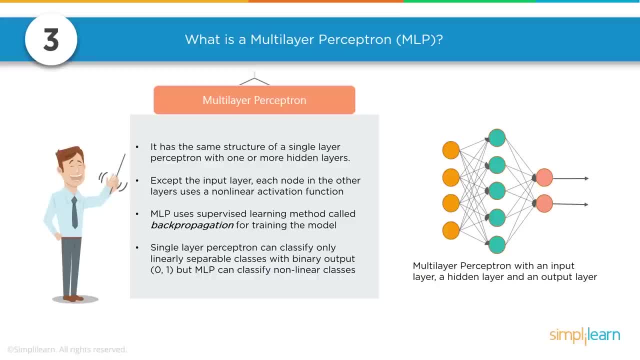 activation function. what that means is your input layers, your data coming in, and then your activation function is based upon all those nodes and weights being added together and then it has the output. MLP uses supervised learning method, called back propagation, for training the model. very key word there is back. 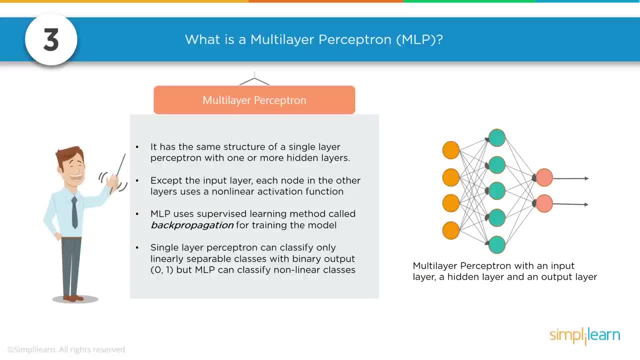 propagation single layer perceptron can classify only linear, separable classes with binary output 01, but the MLP can classify non-linear classes. so let's break this down just a little bit. the multi-layer perceptron with an input layer and a hidden layer and an output layer, as you see that. 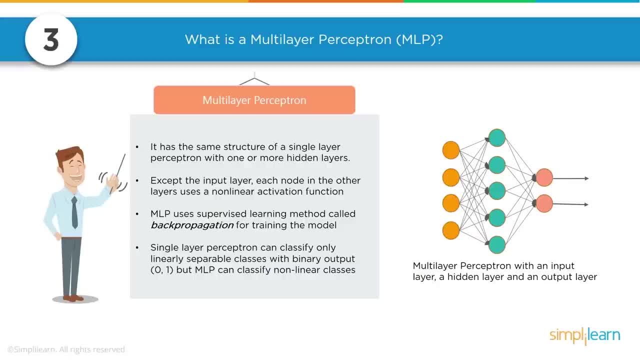 is the output layer, so it's a set of numbers and weights, depending on how your setup is. that then goes to the next layer, that then goes to the next hidden layer- if you have multiple hidden layers- and finally to the output layer. the back propagation takes the error that it sees. so, whatever the 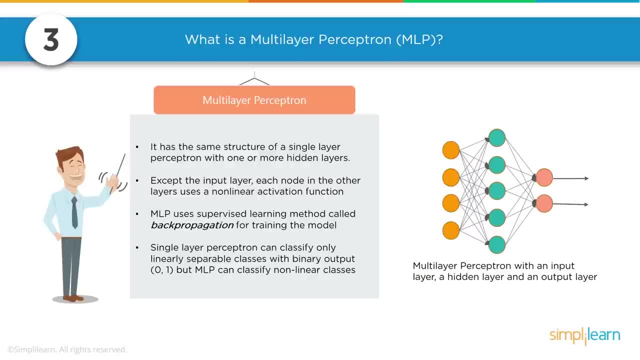 output is it says hey, this has an error to it, it's wrong, and then sends that error backwards from where it came from, and there's a lot of different functions used to train this based on that error and how that error goes backwards in the nodes. so forward is you get your answers, backward is for. 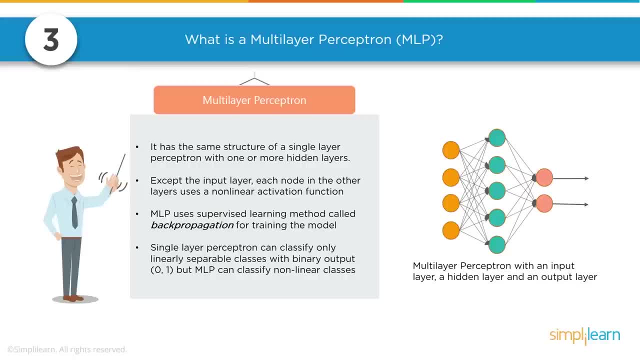 training. you see this every day. even my google pixel phone has this. it they train the neural network, which takes a lot more data to train than it does to use, and then they load up that neural network into. in this case, I have a pixel 2 which actually has a built-in neural network for. 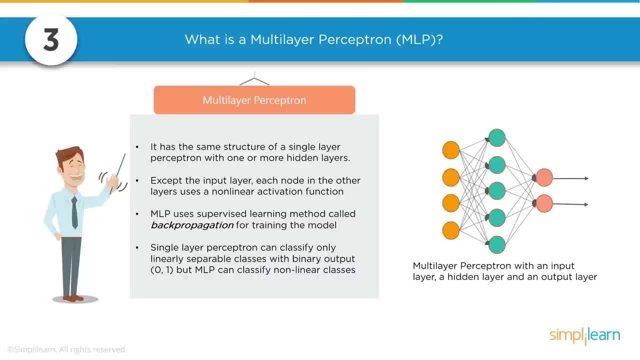 processing pictures, and so it's just the forward propagation I use when it processes my photos, but when they were training it, you use the back propagation to train it with the errors they had. we'll be coming back to different models that are used for right now though: multi-layer. 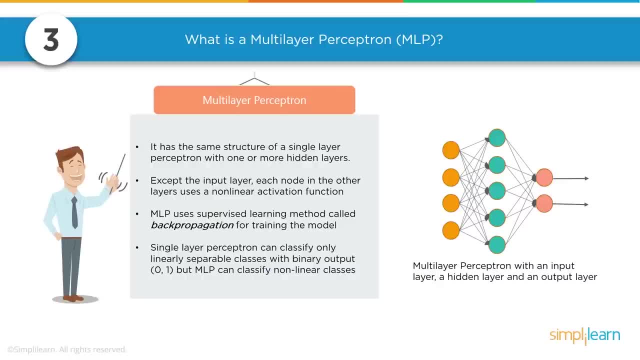 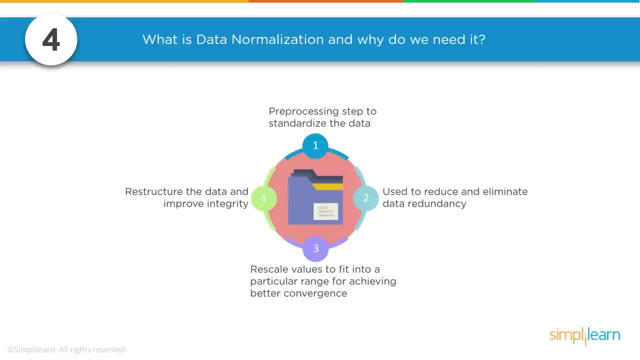 perceptron, MLP, put that down as your vocabulary word- and, of course, back propagation. what is data normalization and why do we need it? this is so important. we spend so much time in normalizing our data and getting our data clean and setting it up. so we talked about data. there's a pre-processing. 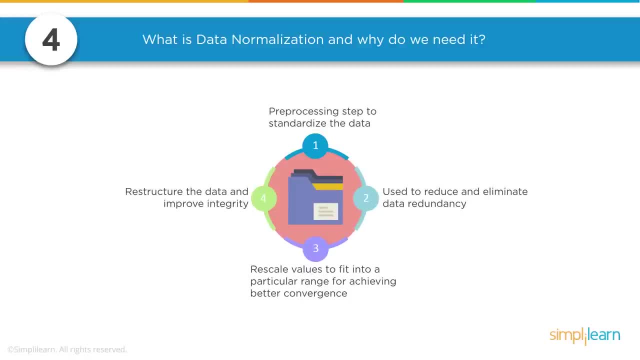 step to standardize the data. so whatever we have coming in, we don't want it to be a, you know, one gigabyte file here, a two gigabyte picture here and a three kilobyte text there. even as a human I can't process those all the same group. I have to reformat them in some way that. 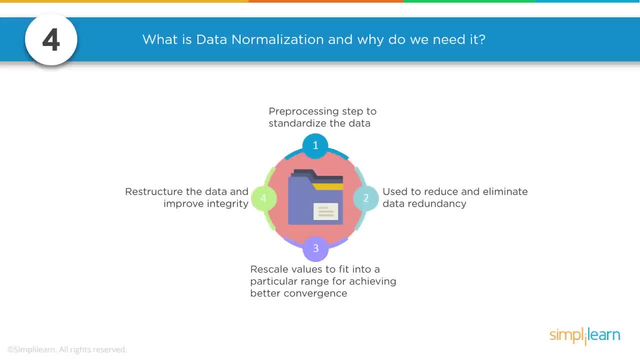 loops them together so they standardize format. we use this data normalization and in pre-processing to reduce and eliminate data redundancy. a lot of times the data comes in and you end up with two of the same images or the same information in different formats. then we want to rescale values. 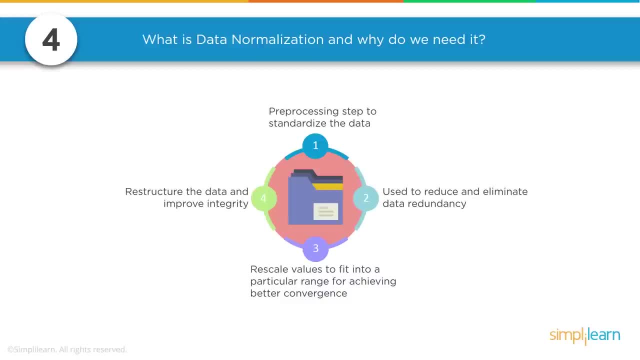 to fit into a particular range for achieving better convergence. what this means is, with most neural network production, that we're going to start with the actual data data and the actual data they're going to be, and we're going to look at the information that we want to see in the data. 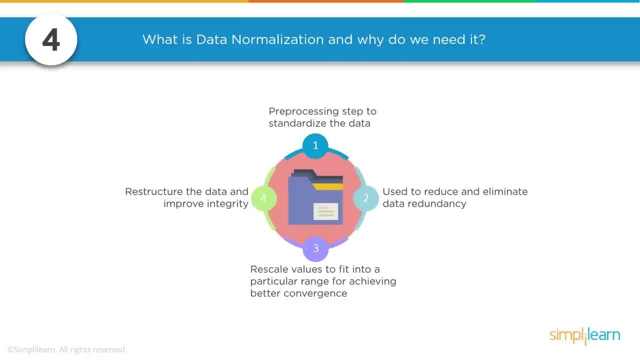 on the data and we're going to need to do a search and we're going to want to see if it's possible to do this. networks, They form a bias. We've seen this recently in attacks on neural networks, where they light up one pixel or one piece of the view and it skews the whole answer. So suddenly. 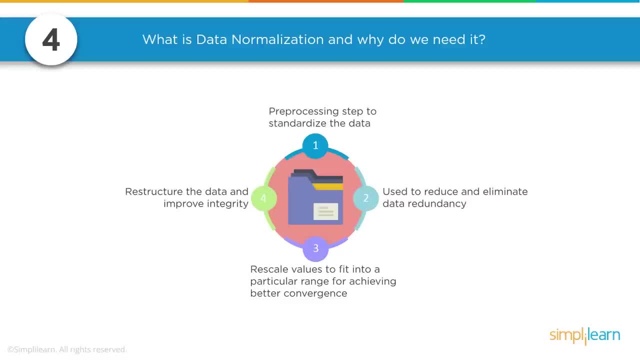 because one pixel is really bright, it doesn't know what to do. Well, when we start rescaling it, we put all the values between, say, minus one and one and we change them and refit them to those values. it helps get rid of that bias. It helps fix for some of those. 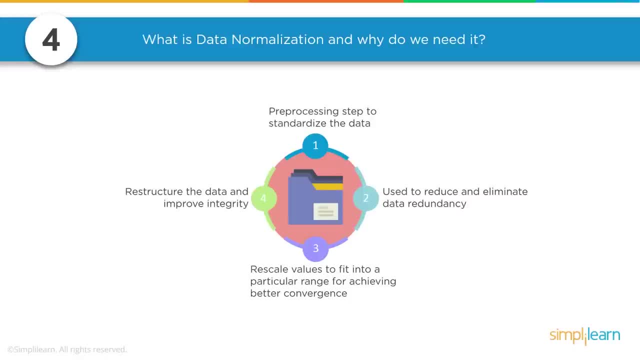 problems And then, finally, we restructure the data and improve the integrity. We want to make sure that we're not missing values or we don't have partial data coming in. One way to look at this is: bad data in, bad data out. So you want clean data in and you want 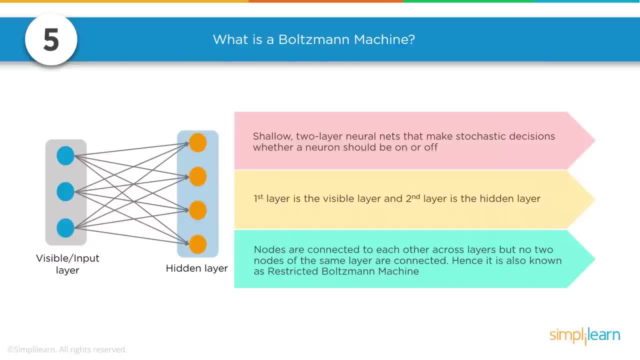 good answers coming out. One of the most basic models used is a Boltzmann machine. So let's address what is a Boltzmann machine And, if you know, we just did the MLP multi-layer Perceptron. So now we're going to come into almost a simplified version of that And in 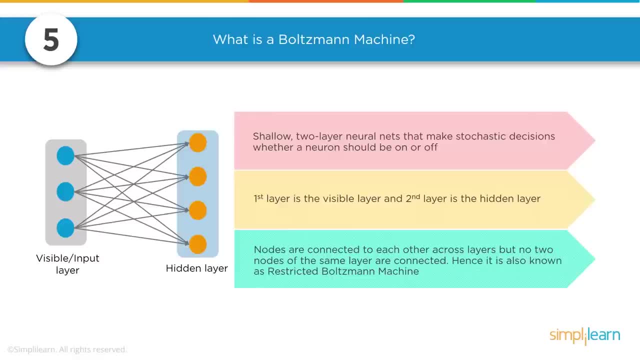 this: we have our visible input layer and we have our hidden layer. The Boltzmann machines are almost always shallow. They're usually just two-layer neural nets that make stochastic decisions: whether a neuron should be on or off. True, false, Yes, no. First, 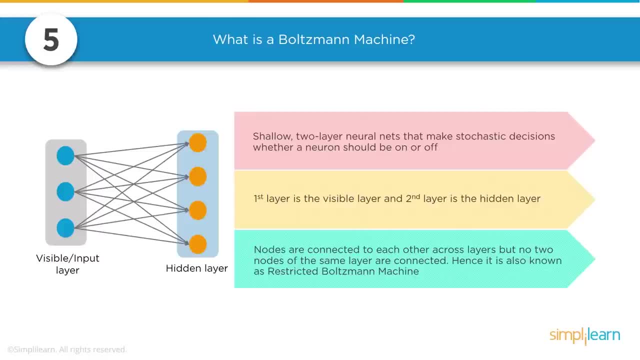 layer is the visible layer and second layer is the hidden layer. Nodes are connected to each other across layers, but no two nodes of the same layer are connected. Hence it is also known as restricted Boltzmann machine. Now that we've covered a basic MLP or multi-layer- 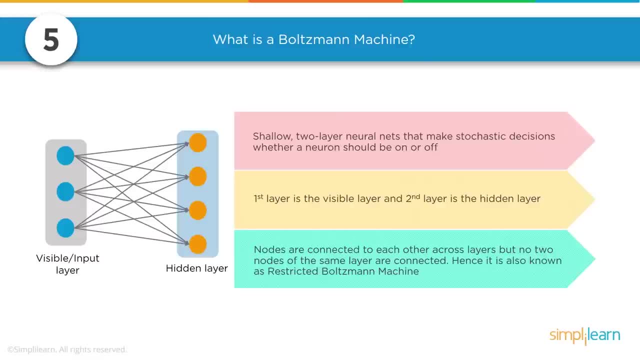 Perceptron and we've gone over the Boltzmann machine, also known as the restricted Boltzmann machine. Let's talk a little bit about activation formulas, And this is a huge topic that can get really complicated, but it also is automated, So it's very simple. So you have both a complicated 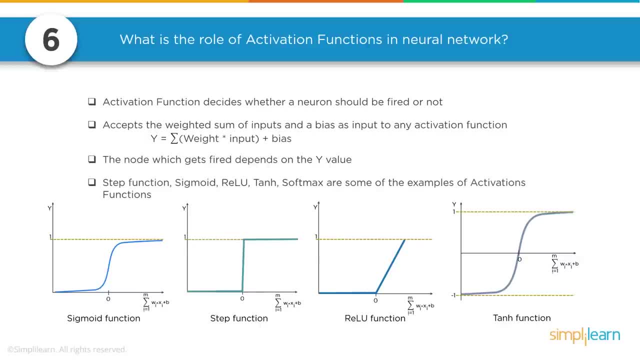 and a simple at the same time. So what is the role of activation functions in a neural network? Activation function decides whether a neuron should be fired or not. That's the most basic one, And that actually changes a little bit, because it's either whether it's 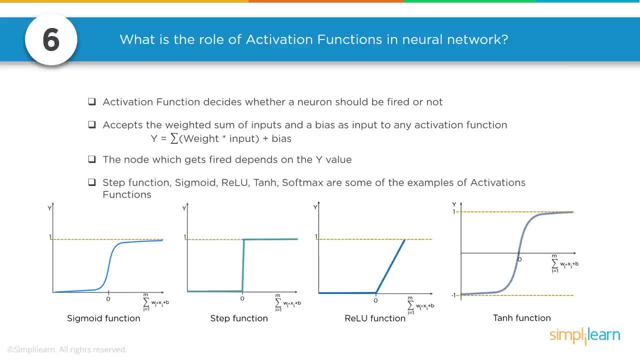 fired or not- in this case activation function, or what value should come out when it's fired. But in these models you're looking at just the Boltzmann restricted layers. So this is what causes them to fire. Either they don't or they do. It's a yes or no, true, false. 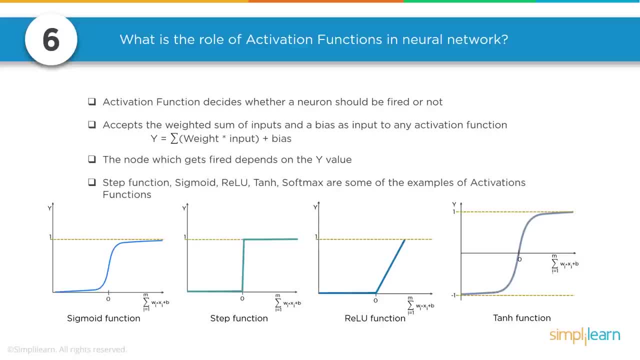 All or nothing. It accepts the weighted sum of the inputs, the bias, as an input to any activation function. So whatever activation function is, it needs to have the sum of the weights times the input. So each input, if you remember, on the model And let's 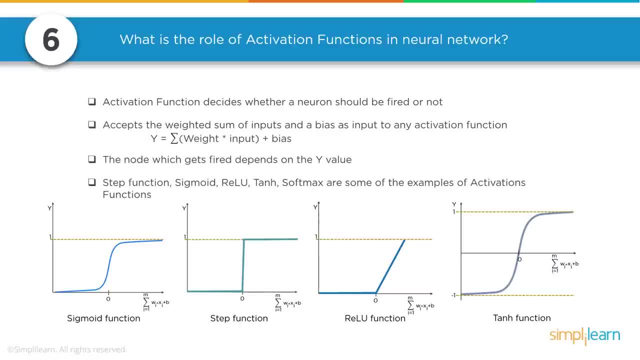 just go back to that model real quick And then you always have to add a bias and you can look at the bias, if you remember, from your Euclidean table. you can add a lot of debates above that you've got here. If you're using trans Breadajo model, if you use Euclidean. 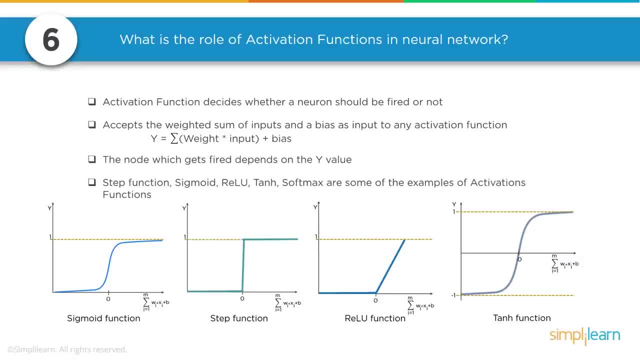 models. if you want to recognize any of both. that's another benefit you don't want from your Euclidean geometry. You draw a straight line. The formula for that line has a y-coordinate. at the end It's always cx plus m, or something like that, where m is where it crosses the y. 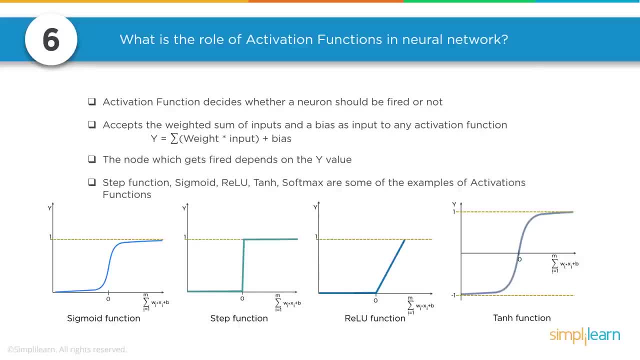 coordinates if you're doing a straight line With these weights. it's very similar, but a lot of times we just add it in as its own weight. We take it as a node of a one value coming in and then we compute its new weight, and that's how we compute that bias, just like we compute all the other. 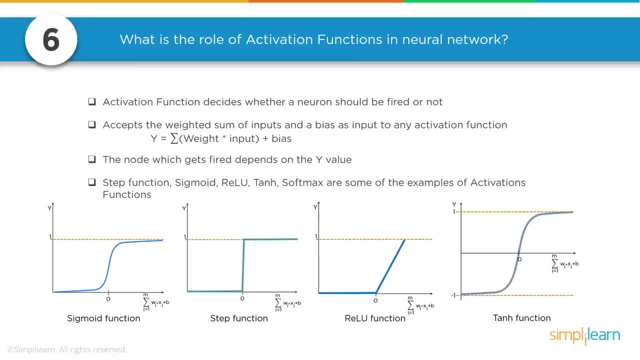 weights coming in The node which gets fired depends on the y value, and then we have a step function. In the step function- this is where, remember, I said it's going to get complicated and simple all at the same time- We have a lot of different step functions. We have the 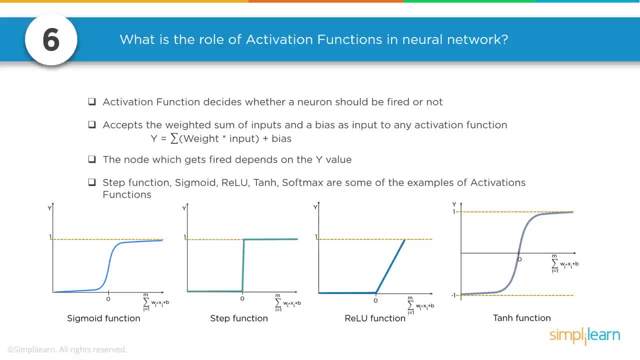 sigmoid function. We have just a standard step function. We have the ReLU. It's pronounced like Re, the Re from the sun and Lu like a name, so ReLU function. and we have the tangent h function and if you look at these they all have something similar. They all either force it to be. 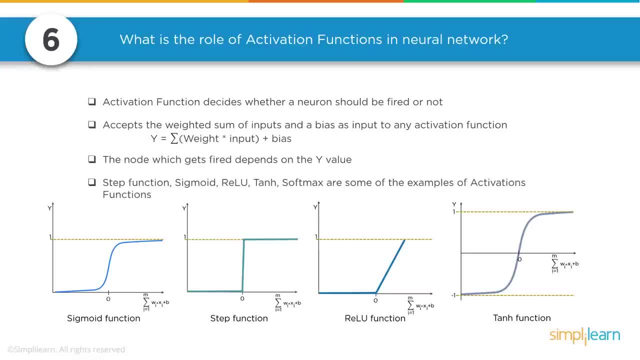 more or less the same, or they all have something similar. They all either force it to be more or less one value or the other. They force it to be, in the case of the first three, a zero or a one, and in the last one it's either a minus one or a one, and you can easily convert that to a zero. 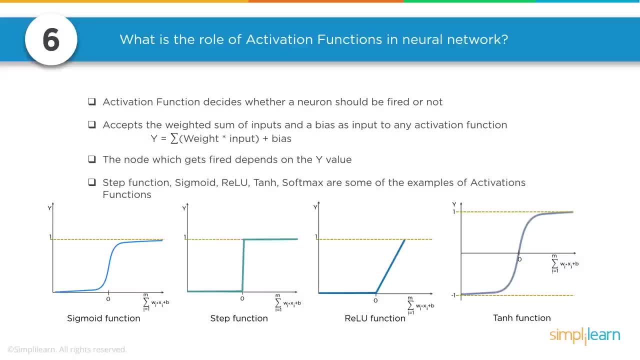 one, yes, no, true, false. and on this, one of the most common ones is the step function itself, because there is no middle value, There is no discrepancy that says well, I'm not quite sure, but as you get into different models, probably the most commonly used used to be the sigmoid. 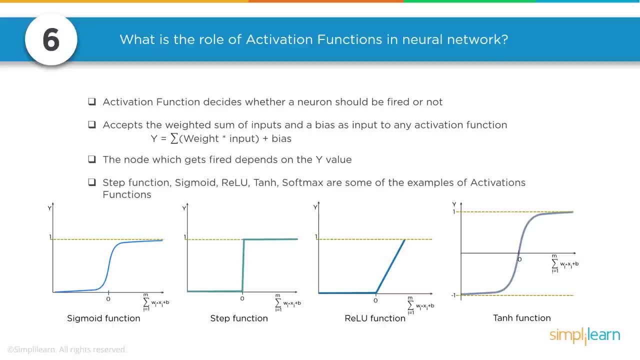 was the most commonly used, but I see the ReLU used more often. Really, depending on what you're doing, you just have to play with these and find out which one works best, depending on the data and your output. The reason to have a non-zero-one answer or something kind of in the middle is when 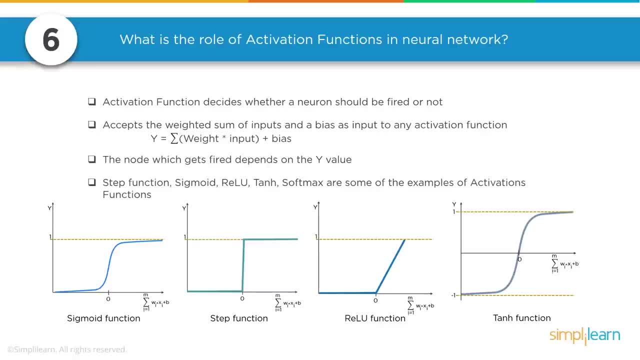 you're looking at this and it's coming out. you can actually process that middle ground as part of the answer into another neural network. so it might be that the ReLU function says, hey, this is only a 0.6, not a one, and even though the one is what's going into the next neural network? 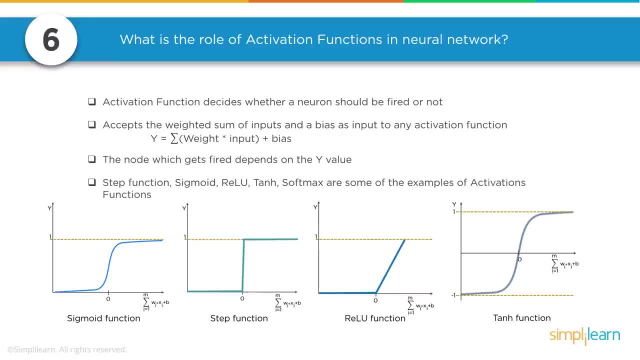 or the next hidden layer as an input. the 0.6 value might also be going in there to let you know. hey, this is not a straight-up one or a straight-up zero, It's someplace in the middle. This is a little. 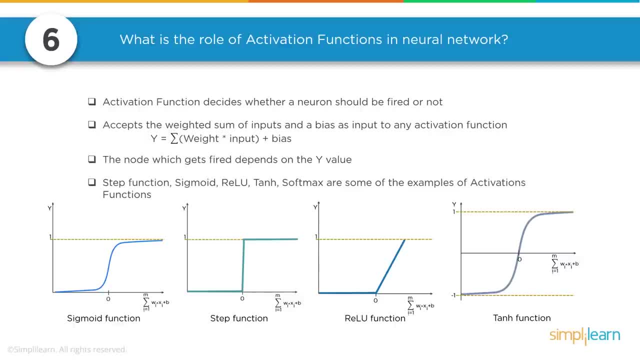 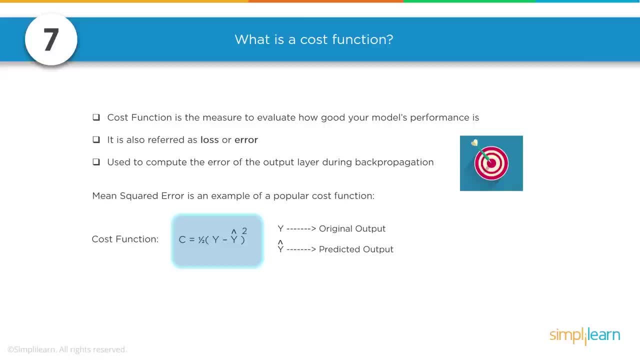 uncertain what's coming out here. so it's a very powerful tool, but in the basic neural network you usually just use the step function. It's yes or no. Let's take a big step back and take a kind of an overview. The next function is: what is a cost function that we're going to cover? 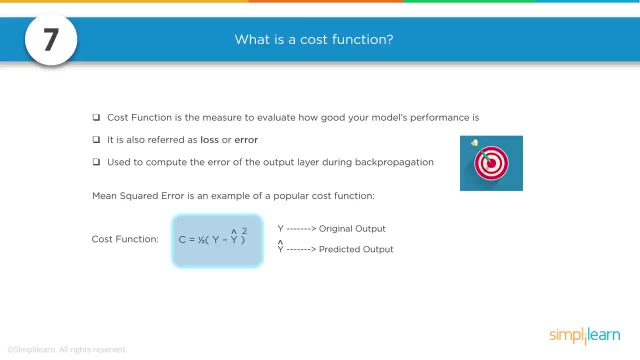 This is so important because this is your end result That you're going to do over and over again and use to decide whether the model is working or not, whether you need to try a different step function, whether you need to try a different activation. 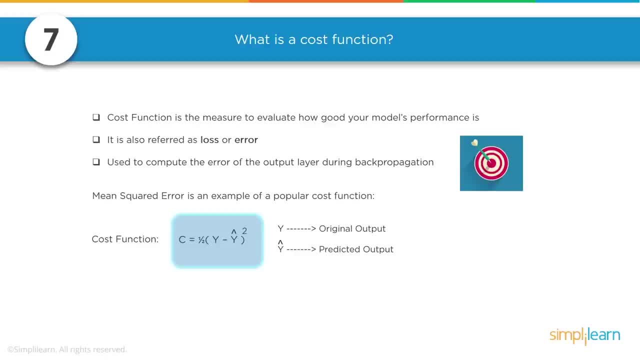 whether you need to try a fully different model used. So what is the cost function? Cost function is a measure to evaluate how good your model's performance is. It is also referred as loss or error, used to compute the error of the output layer during back propagation. There's our back. 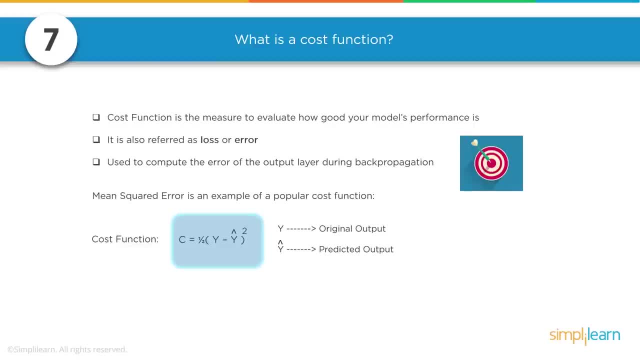 propagation, where we're training our model. That's one of our key words. Mean squared error is an example of a popular cost function. and so here we have the cost function: c equals half of y minus y predicted, and then you square that. So the first thing is: you know real quick if you haven't. 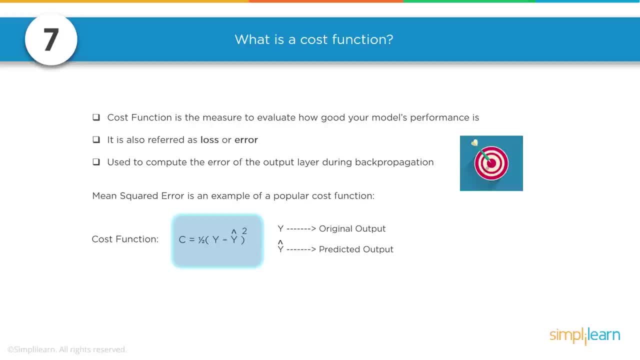 done statistics. this is not a percentage. It's not a percentage of how accurate it is. It's just a measurement of the error and we take that error for training it and we push that error backwards through the neural network and we use that through the different training functions. 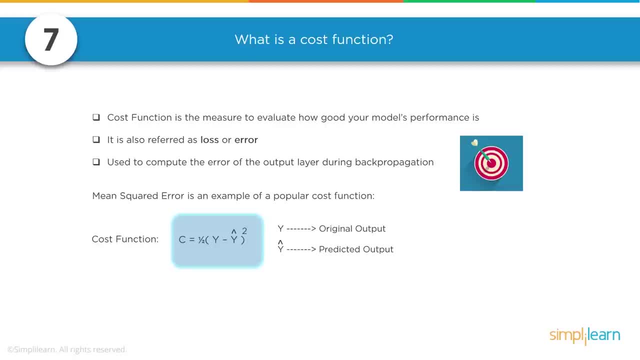 depending on what model you're using to train the neural network. So when you deploy the network, you're usually done training it, because it takes a lot of computational force to train it. This is a very simple model, and so you deploy the trained one. 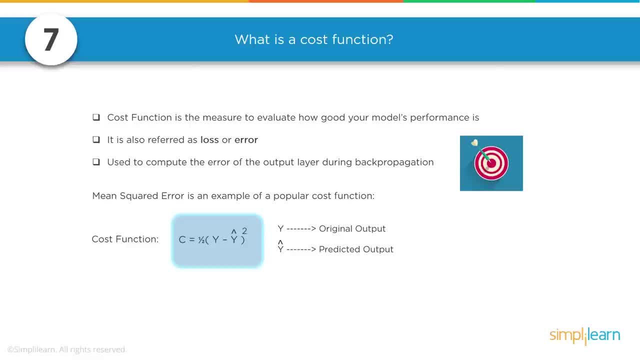 but we want to know how your error is, and so how do we do that? Well, you split your data. Part of your data is for training and part of your data is for testing, and then we can also test the error on there. So that's very important, and then we're going to go one more step on this. 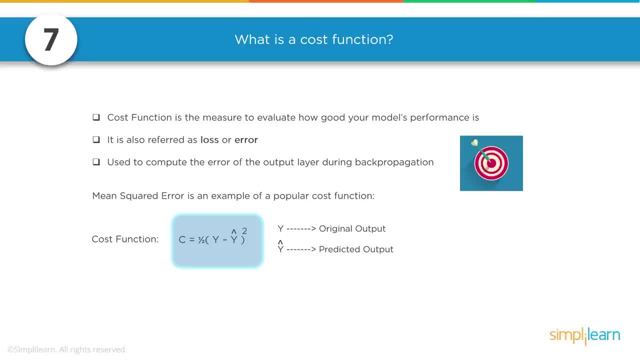 We got to look at both the local and the global setup. It might work great to test your data on what you have on your computer, But that's different than in the field. So when we're talking about all these different tests and the error test, as far as your loss, you want to make sure that you're in a closed 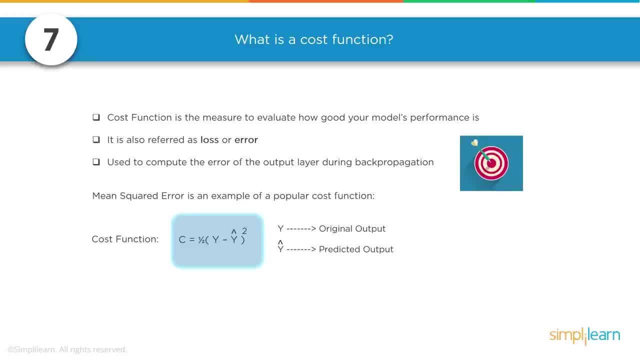 environment when you do your initial testing. but you also want to open that up and make sure you follow up with the testing on the larger scale of data because it will change. It might not fit the larger scale. There might be something in there in the way you brought the data in. 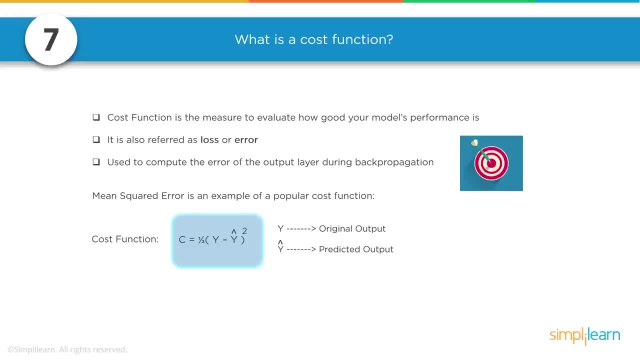 specifically, or the data group you used, or any of those could cause an error. So it's very important to remember that we're looking at both the local and the global context of our error. And just to wrap up, if you have any questions, please feel free to ask them in the Q&A section. 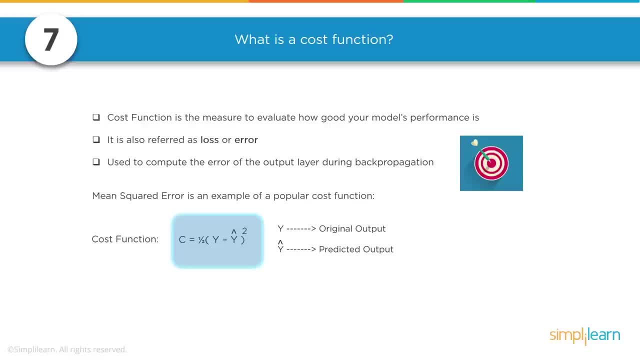 And just to wrap up, if you have any questions, please feel free to ask them in the Q&A section. And just one other side note on a lot of the newer models of neural networks: by comparing the error we get on the data, our training data, with a portion of the test data, we can actually 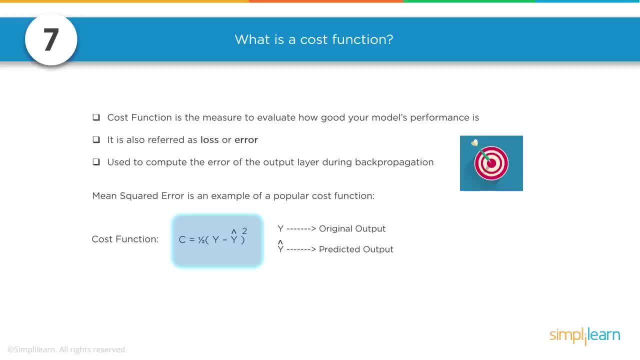 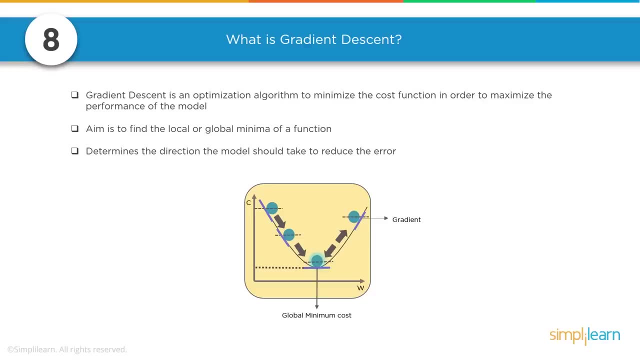 figure out how good the model is, whether it's overfitted or not. We'll go into that a little bit more as we go into some of the different models. So we have our output. We're able to figure out the error on it based on the square means usually, although there's other. 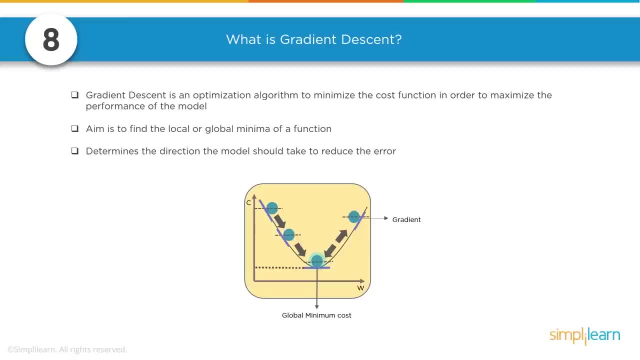 functions used. So we want to talk about what is gradient descent, another vocabulary word, Gradient descent is an optimization algorithm to minimize the cost function or to minimize the error. Aim is to find the local or global minima of a function, Determine the direction the model should take to reduce the error. So, as we're looking at this, 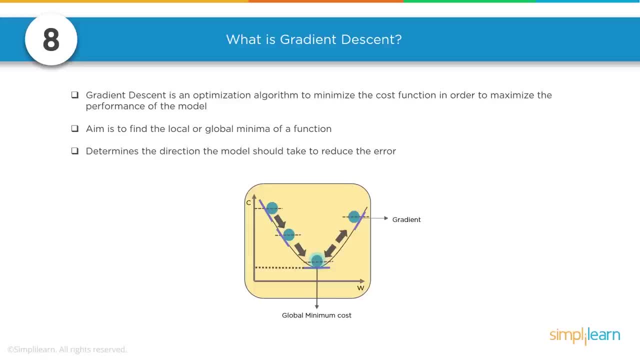 we have our squared error that we just figured out based on the cost function, It says: how bad is my model fitting the data I just put through it, And then we want to reduce that error. So how do you figure out what direction to do that in? Well, it could be that you're looking at just that. 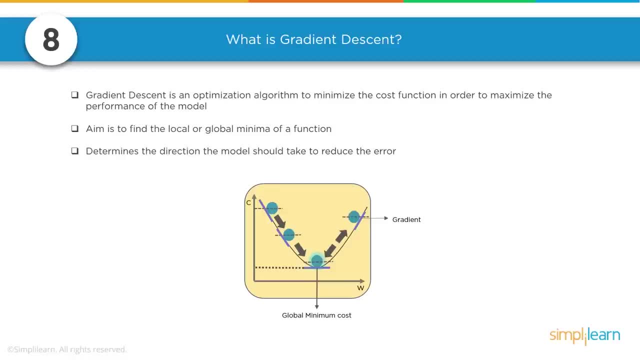 line of data coming in, So that would be a local minima. We want to know the error of that particular setup coming in And then you have your global, your global minima. We want to minimize it based on the overall data we're putting through it And with this we can figure out the global. 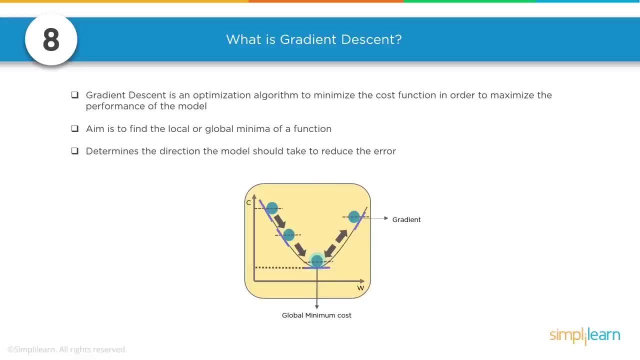 minimum cost. We want to take all those local minimum costs of each piece of data coming in and figure out the global one. How are we going to adjust this model to fit all the data? We don't want it to be biased just on three or four lines of data coming in. We want it to 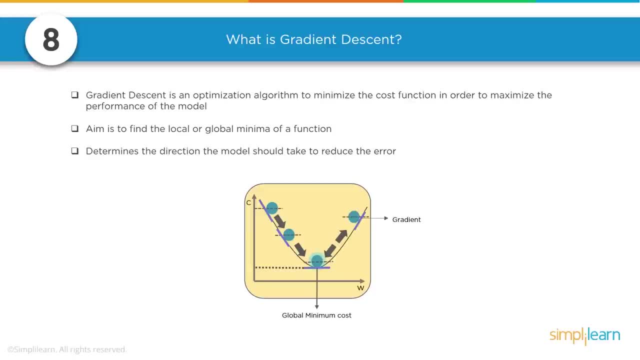 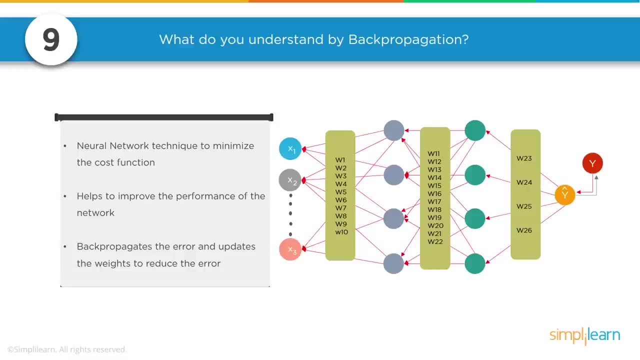 kind of extrapolate a general answer for all the data coming in This. of course we mentioned it briefly about back propagation. This is where it really comes in handy. is training our model Neural network technique to minimize the cost. function Helps to improve the performance of. 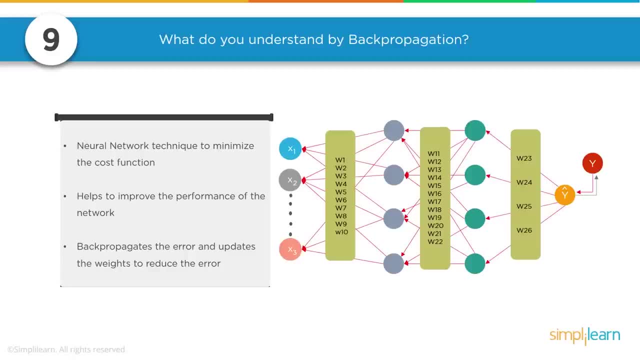 the network Back propagates the error and updates the weights to reduce the error. So, as you can see, here is a very nice depiction of a back propagation. We have our predicted Y coming out And then we have- since it's a training set, we already know the. 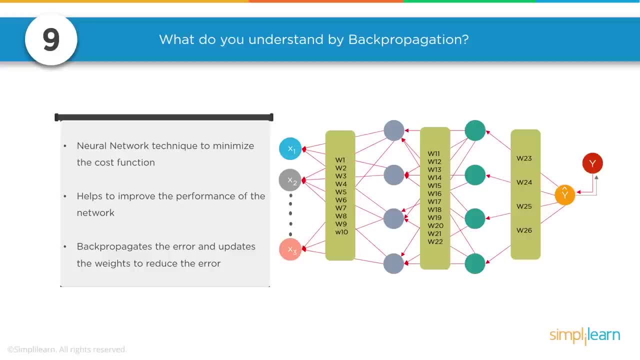 answer, And the answer comes back And based on case of the square means, was one of the functions we looked at, One of the activation functions based on cost function. That cost function, then, depending on what you choose for your back propagation method, and there's a number of them. 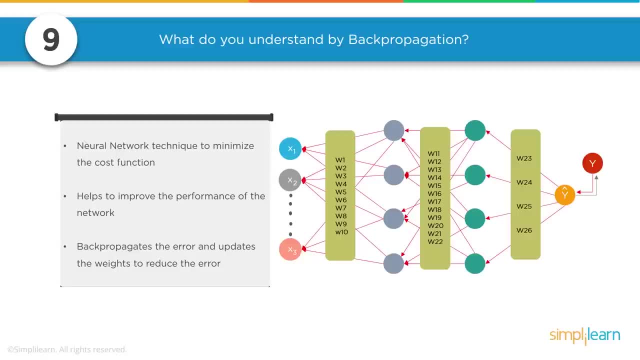 will change the weights. It will change the weight going to each of the one of those nodes in the hidden layer And then, based upon the error that's still being carried back, it'll change the weights going to the next hidden layer And then it computes an error level on that and sends that. 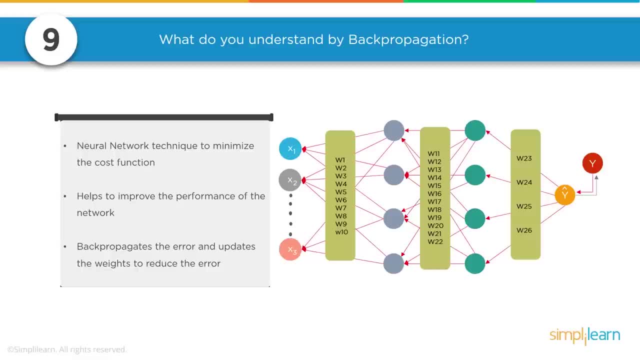 back up And you're going to see that the error level is going to go up. And you're going to see, well, if it computes the error into the first hidden layer and fixes it, why would it stop there? Well, remember, we don't want to create a biased neural network, So we only make small. 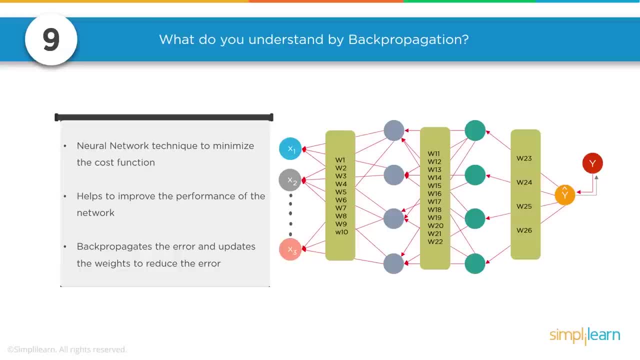 adjustments on these weights. We don't make a big adjustment. that changes everything right off the bat. So no matter how far back you go, you're always going to have a small amount of error, And that's still going to continue to go all the way back up the hidden layers. For right now, 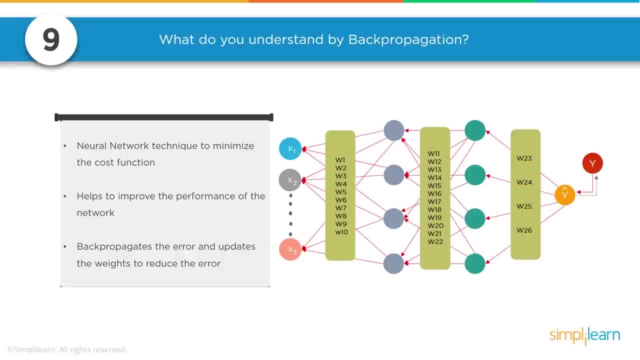 focus on the back propagation is taking that error and moving it backwards on the neural network to change the weights and help program it so that it'll have the correct answers. So far we've been talking about forward propagation, neural networks. Everything goes forward, goes left to right. 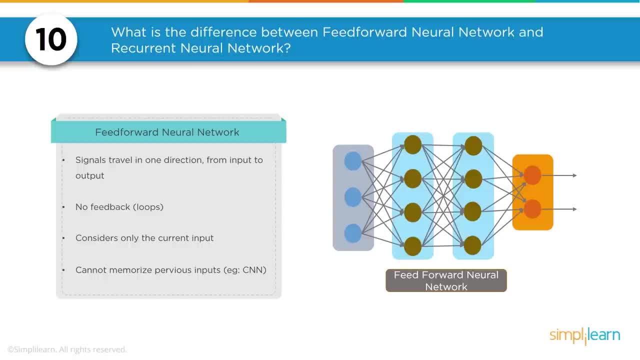 But let's take a little detour And let's see what is the difference between a feed forward neural network and a recurrent neural network. Now, this is in the function, not when we're training it using the back propagation. So you've got new information. 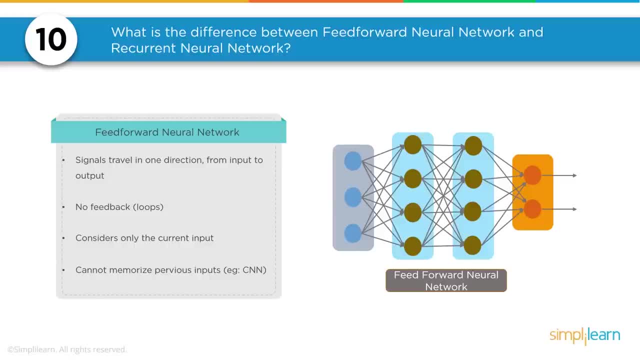 coming in. You want to get the answer And there's a couple of different networks out there And we want to know. we have a feed forward neural network and we have a new term, recurrent neural network. a feed forward neural network, signals travel in. 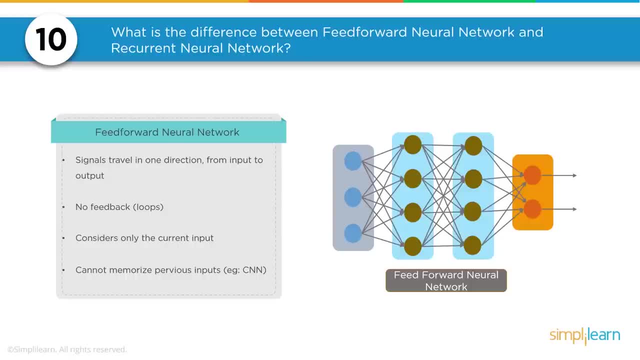 one direction, from input to output. no feedback loops. considers only the current input. cannot memorize previous inputs. one example of one of these feed forward neural networks, and we've covered a number of them, but one of the ones that has a big highlight nowadays is the CNN. a convolutional neural 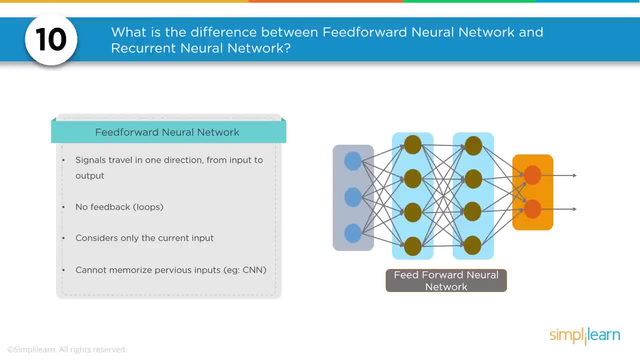 network tensorflow- the one put out by Google is probably most known for their CNN- where the information goes forward. it first takes a picture, splits it apart, goes through the individual pixels on the picture so it picks up a different reading, then calculates based on that, goes into a regular feed forward- neural. 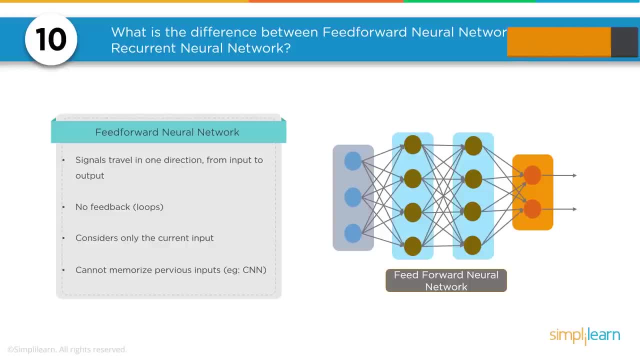 network and then gives your categorization on there. now we're not covering the CNN today, but we do have a video out that you can look up on YouTube, put out by: simply: learn the convolutional neural network. wonderful tutorial. check that out and learn a lot more about the convolutional neural. 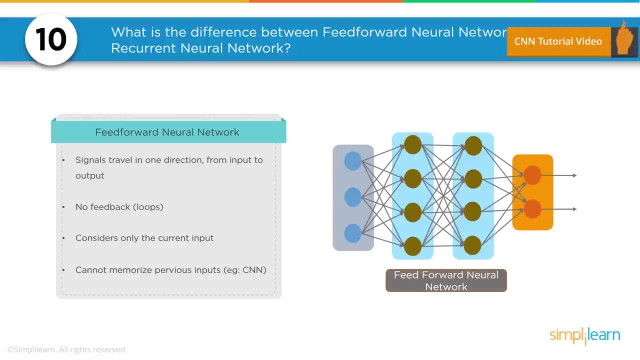 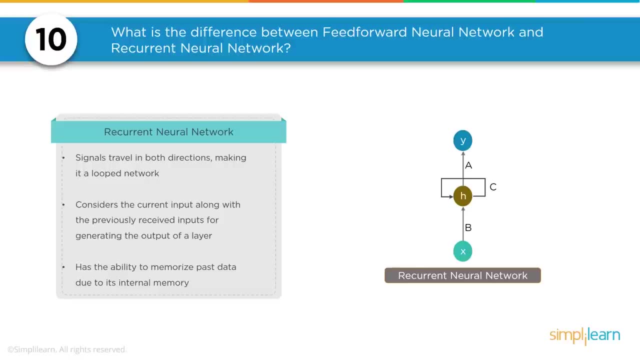 network. but you do need to know that the CNN is a forward propagation neural network only, so it's only moving in one direction. so we will look at a recurrent neural network. signals travel in both directions, making it a looped network. considers the current input, along with 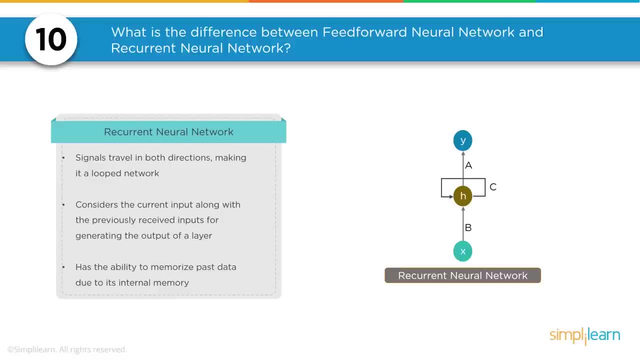 the previous received inputs for generating the output of a layer has ability to memorize past data due to its internal memory and you can see they have a nice image. here we have our input and for some reason they always do the recurrent neural network in reverse from bottom up. 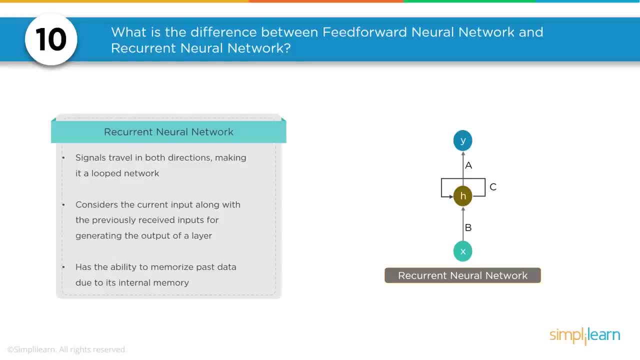 the images, kind of a standard, although I'm not sure why your ex goes into your hidden layer and your hidden layer- the answer for part of the answer from that it generates feeds back into the hidden layer. so now you have an input of both X and part of the hidden layer and then that feeds into your output. now, if we go, 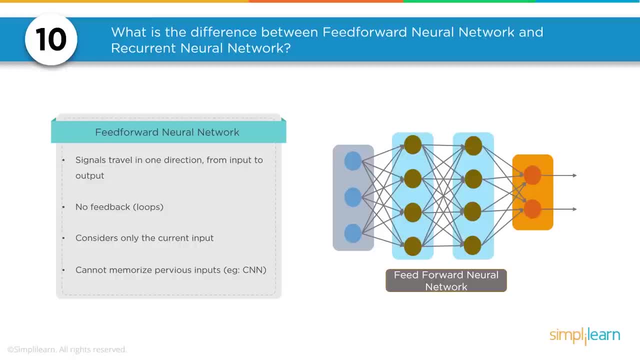 back to the forward. let me just go back a slide and we're looking at our forward propagation network. one of the tricks you can do to use just a forward propagation network is if you're in a what they call a time sequence- that's a good term to remember- or a time series, meaning that a sequential data. 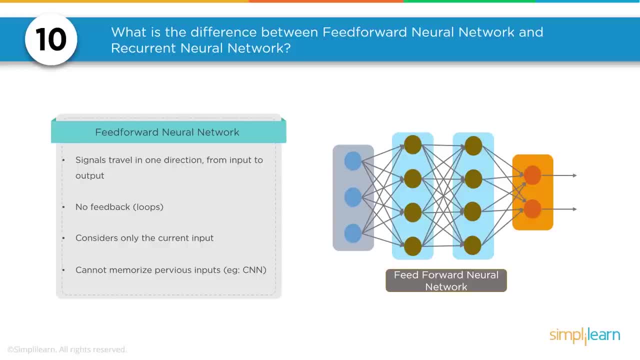 each term comes after the other. you can trick this by creating your input nodes, as with the history. so if you know that you have values 1, 5 & 7 going in and you know what the output is from one but those outputs are, you can expand the. 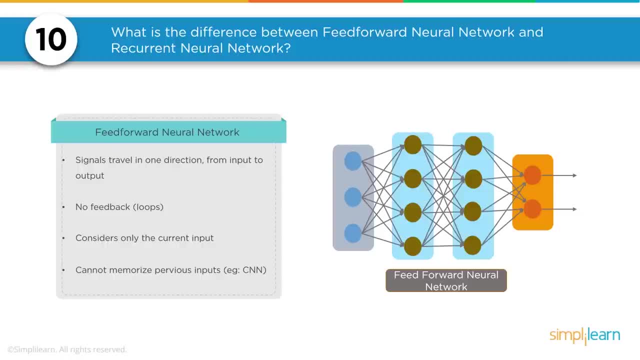 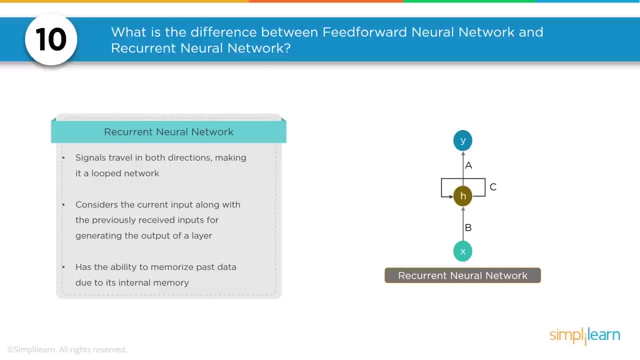 input to include the history input. that's one of the ways to trick a forward propagation network into looking at that. but when you do with a recurrent neural network, you let the hidden layer do the that for you. it sends that data and reprocesses it back into itself. what are? 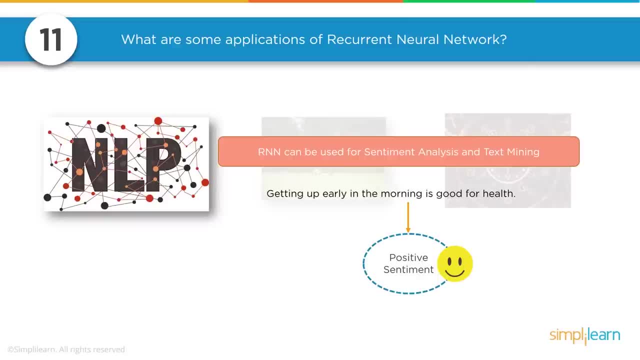 some of the applications of recurrent neural network. the RNN can be used for sentiment analysis and text mining. getting up early in the morning is good for health. it's a positive sentiment. one of the catches- you really want to look at this when you're looking at the language- is that I could switch this. 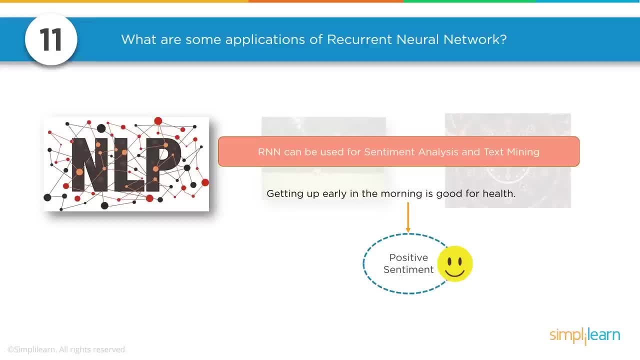 around and totally negate the meaning of what I'm doing, so it no longer be positive. so when you're looking at a sentence, knowing the order of the words is as important as the meaning of the words, can't just count how many good words there are versus bad words to get. 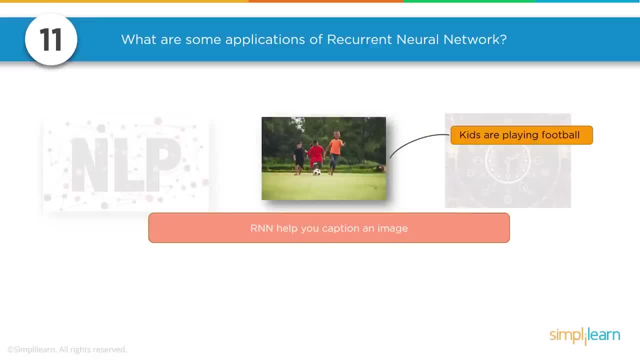 some positive sentiment. you now have to know what they're addressing, and there's lots of other different uses. kids are playing football or soccer, as we call it in the US. RNN can help you caption an image. so, based on previous information coming in, it refeeds that back in and you have a image setter and then time. 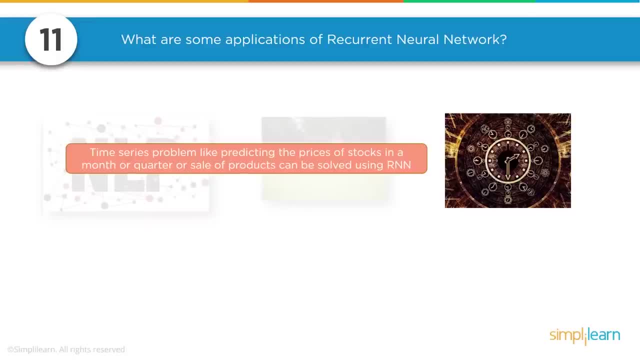 series. problems like predicting the prices of stocks in a month or quarter or sell of products can be solved using an RNN, and this is a really good example you have. whatever your stocks were doing earlier this month will have a huge effect on what they're doing today if you're investing. so having an RNN- 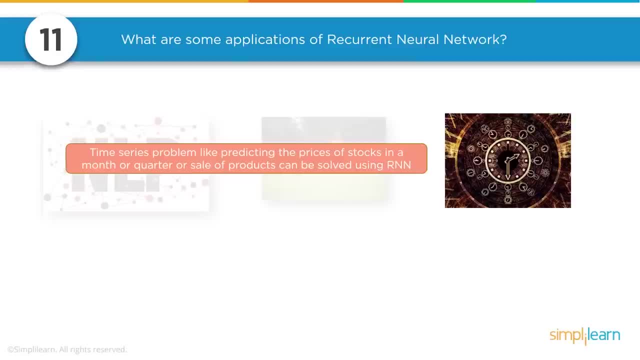 model, a recurrent neural network feeding into itself what's happening previously, allows it to take that model and program in that whole series without having to put in the whole month at a time. of data you only put in one day at a time but if you keep them in order it will look back and say: oh this, because what happened? 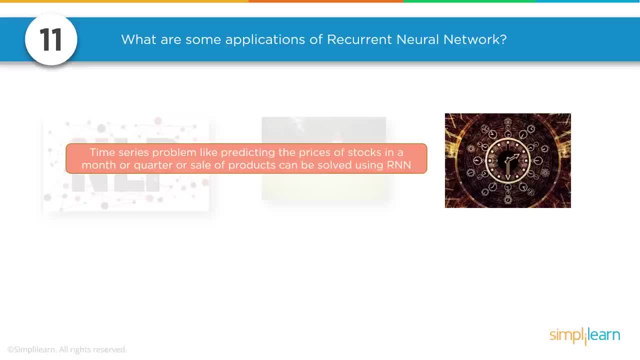 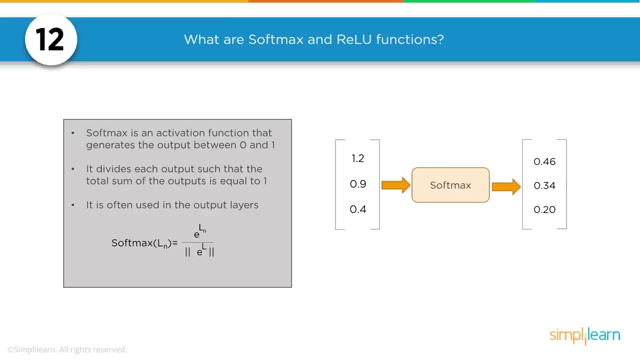 yesterday. I need some information from that and I'm gonna use that to help predict today's and so on and so on. we're gonna go back to our activation functions. remember I told you ReLU was one of the most common functions used, so let's talk a little bit more about ReLU and also softmax. 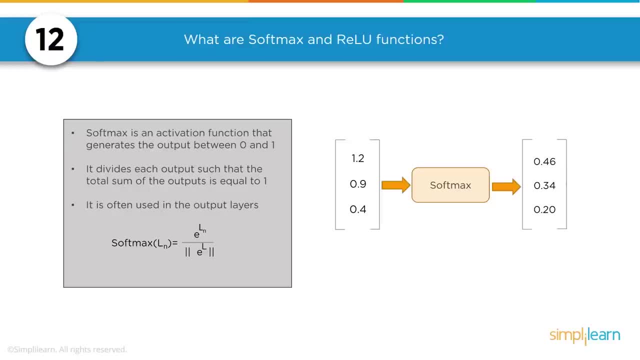 softmax is an activation function that generates the output between 0 and 1. it divides each output such that the total sum of the outputs is equal to 1. it is often used in the output layers. softmax L of the N equals e to L on the N over. 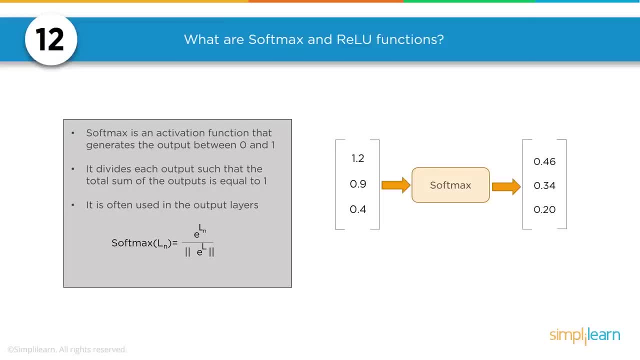 the absolute value of e to the L. so what does this function mean? I mean what is actually going on here? so we have our output notes and our output nodes are giving us- let's say, they give us 1.2, 0.9 and 0.4. as a human being, I look at that and I say, well, the. 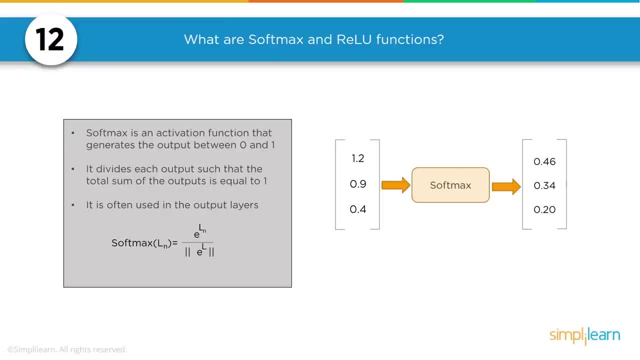 greatest value is 1.2. so whatever category that is, if you have three different categories, maybe you're not just doing if it's a cat or it's a dog, or oh, let's say it's a cow. we had cats and dogs earlier. why the cats and dogs? 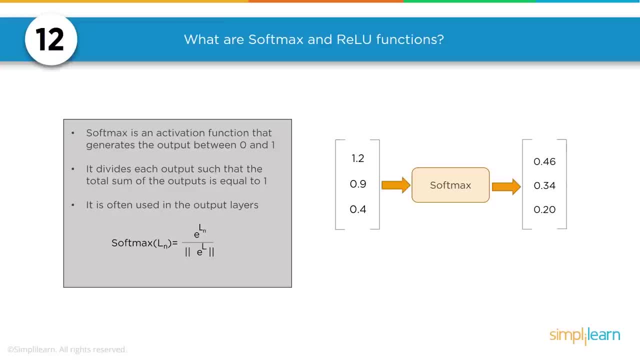 are hanging out with a cow. I don't know, but we have a value and it might say: 1.2 is a cat, 0.9 is the dog and 0.4 is a cow. for some reason it thinks that there's a chance of being any one of these three. 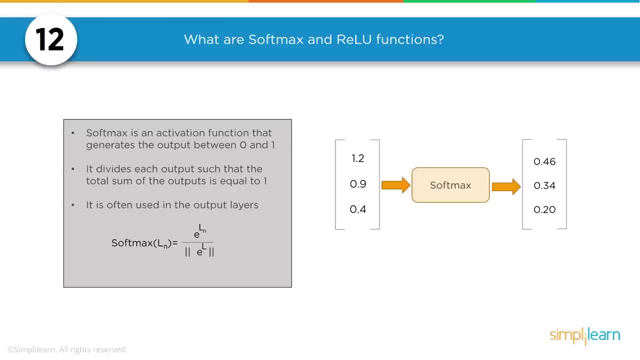 items and that's how it comes out of the output layer. well, as a human, I can look at one point two and say this is definitely what it is, definitely a cat or whatever it is. maybe looking at different kinds of cars might be a better, whether it's a car, truck or motorcycle, maybe that'd be a better. 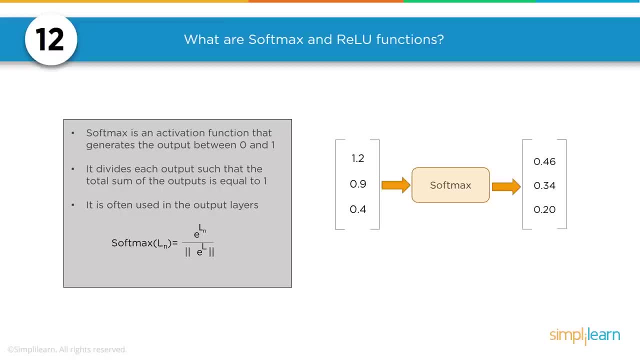 example. well, from a computer standpoint that may be a little confusing, because they're just numbers waving at us, and so with the softmax we want all those numbers to always add up to one. so when I add three numbers together, I want the final output to be one on there, and so it goes through. this formula changes each of these numbers, in this case, 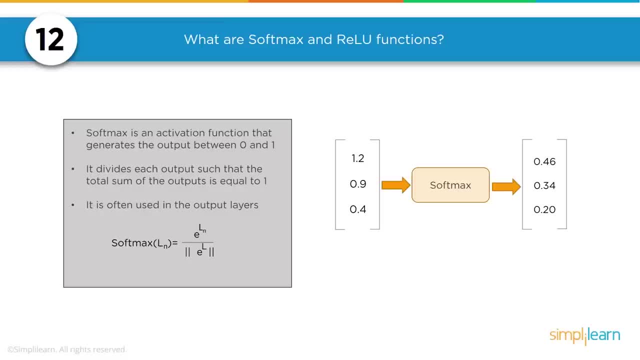 It changes them to point four, six, point three, four and point two. Oh, they all add up to one, and that's a lot easier to register because it's very set. It's a set output, It's never going to be more than one, It's never gonna be less than zero, and so you can see here that there's probably a pretty high chance. 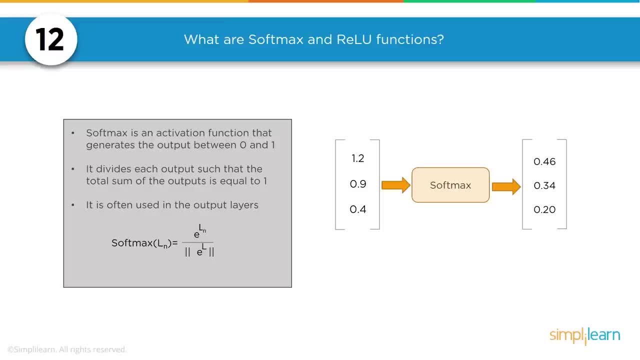 That it's the first one, so you're a human being. we have no problem knowing that. but this output can then also go into, say, Another input, so it might be an automated car That's picking up images and it says that image in front of us is probably a big truck. 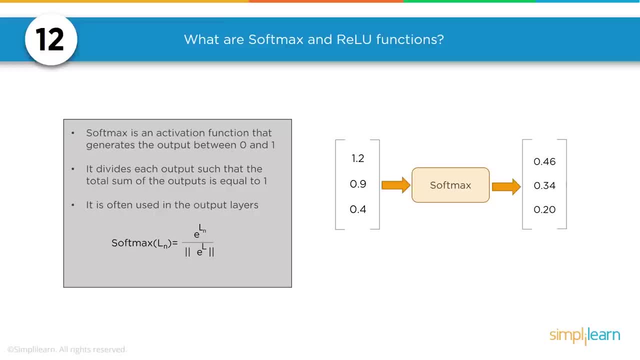 We should deal with it like it's a big truck. It's probably not a motorcycle or whatever those categories are. That's the softmax part of it. but now we have the ReLU. Well, what's where's the ReLU coming from? 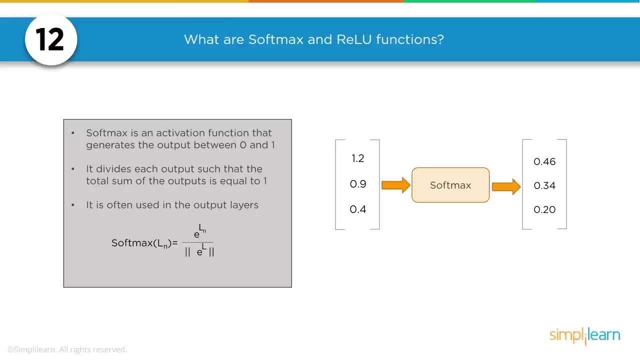 Well, the ReLU is what's generating the 1.2 and the 0.9 and the 0.4, And so, if you remember, our ReLU stands for rectified linear unit and is the most widely used Activation function. We looked at a 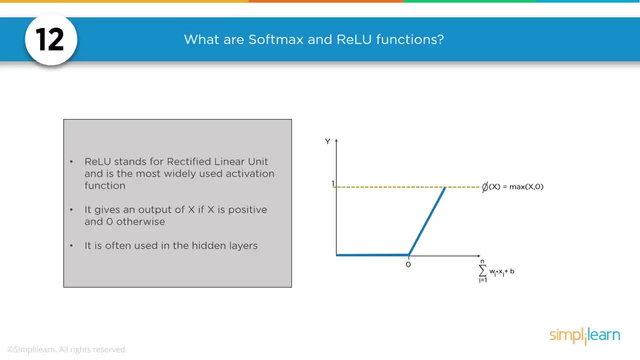 Number of different activation functions, including tangent age. the step function. I remember I said the step function is really used if that's what your actual output is, because then you know it's a zero or one, But the ReLU, if you have that as your output, you know have a discrepancy in there. 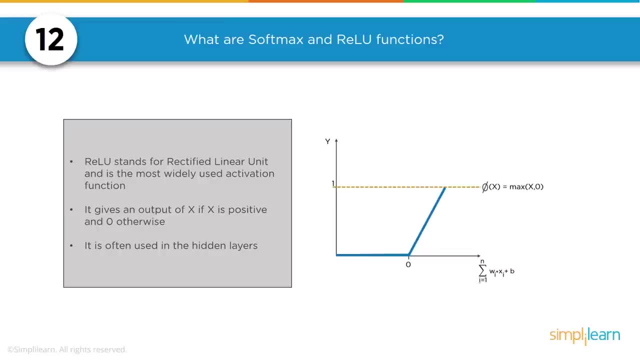 And if that's going into another neural network or another process. Having that discrepancy is really important. and it gives an output of X if X is positive and zero otherwise. so it says my X value is going to be somewhere between 0 or 1, and then the usually. 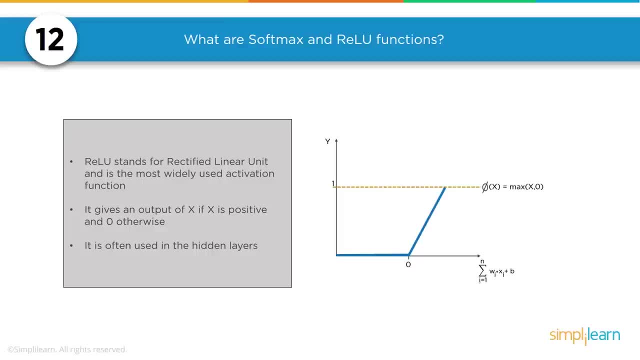 unless it's really uncertain, the output is usually a 1 or 0. then you have that little piece of uncertainty there that you can send forward to another network or you can look at to know that There's uncertainty involved and is often used in the hidden layers. 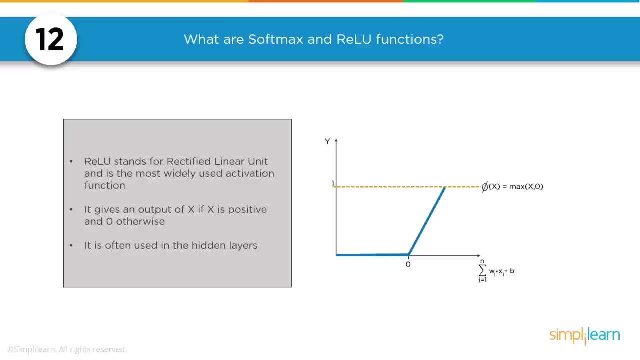 this is what's coming out of the hidden layers into the output layer. usually, or as we reference the convolutional neural network, the CNN- You'd have to go to another video to review the ReLU- is the most common used for convolutional part of that network. 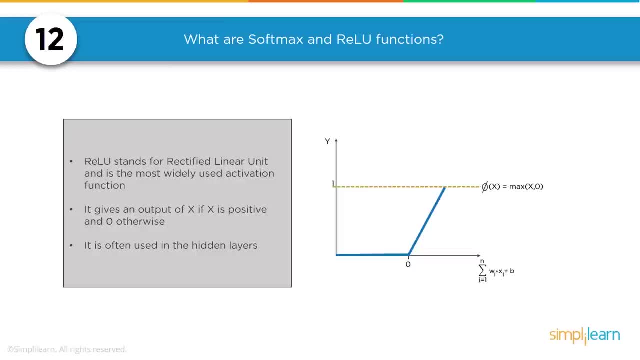 It has a bunch of layers- DNA, for instance, bunch of little pieces that are very simplified. looking at all the different images or different sections of the map, and the ReLU works really good for that. Like I said, there's other formulas used, but that this is the most common. 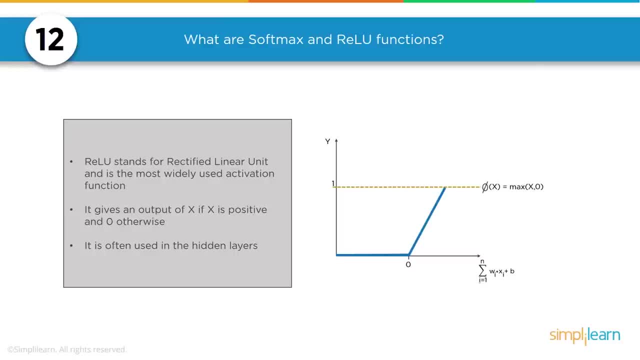 one, and you'll see that in the hidden layers, going maybe between one layer and the next layer. So just a quick recap: we have our soft max, which means that if you have numerous categories, only one of them is going to be picked, but you also want to have some value attached to it. how well it picked it and you put that. 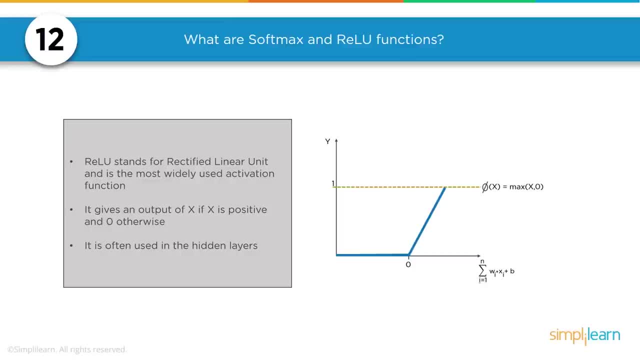 between 0- 1, so it's very standardized. So we have our soft max. we looked at that, let's go back one- we looked at that here- where it transforms in numbers. and then we have our ReLU function, which takes the information and the summation and 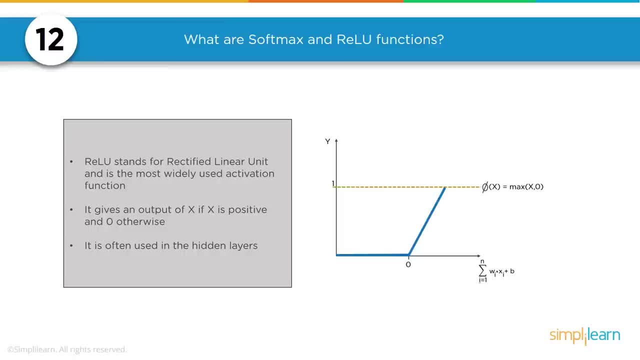 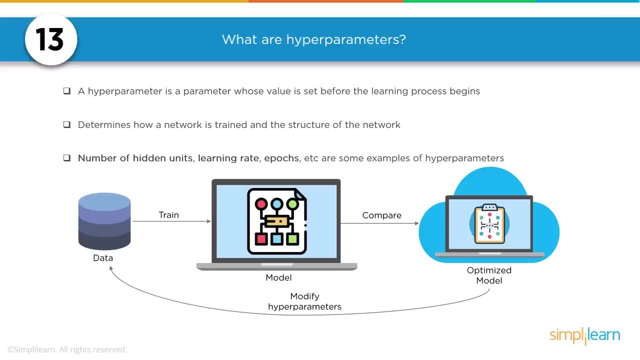 puts it between a 0 and a 1, where it's either clearly a 0 or, depending on how confident our model is, it'll go between the 0 and 1 value. What are hyper parameters? Well, this is a great interview question: Hyper parameters when? 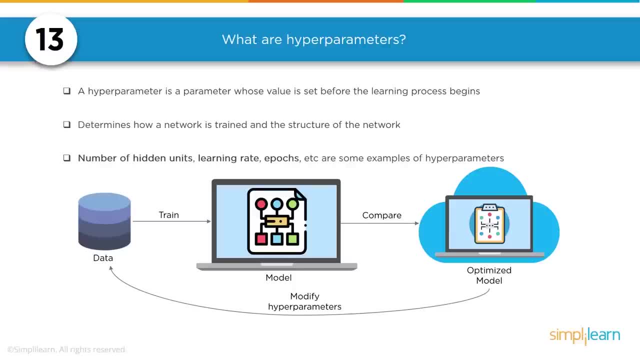 you are doing neural networks. this is what you're playing with most of time, once you've gotten the data formatted correctly. A hyper parameter is a parameter whose value is set before the learning process begins, determines how a network is trained and the structure of the network. This 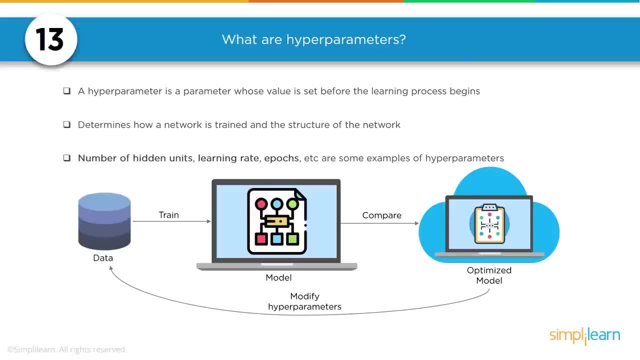 includes things like the number of hidden units, how many hidden layers are you going to have and how many nodes in each layer. Learning rate- Learning rate is usually multiplied once you've figured out the error and how much you want to change the weights We talked about- or I mentioned it early, just 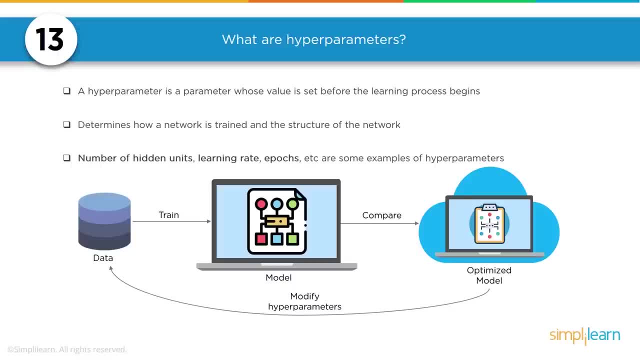 briefly, you don't want to just make a huge change, otherwise you're going to have a biased model. so you only take some little incremental changes and that's what the learning rate is. is a small incremental changes Epics. How many times are you going to go through all the data in your training set? So one. 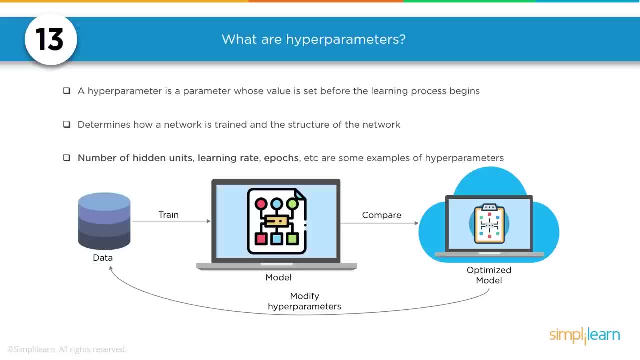 epic is one trip through all the data and there's a lot of other things depending on which model you're working with and which programming script you're working with, Like the Python sklearn package will have a slightly different than, say, Google's tensorflow package, which will be a little bit different. 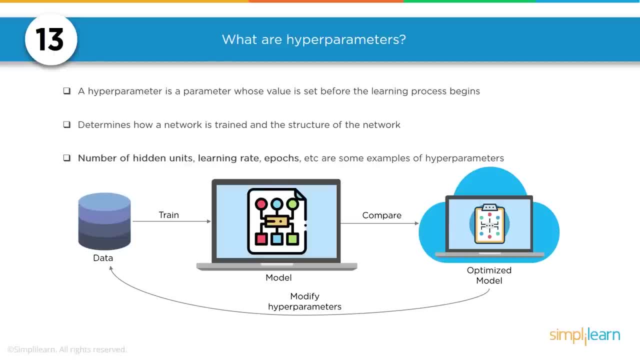 than the spark machine learning package. So some examples are just some examples of the hyperparameters, and so you see, in here we have a nice image of our data coming in and we train our model. then we do a comparison to see how good our model is. Then we go back and we say, hey, 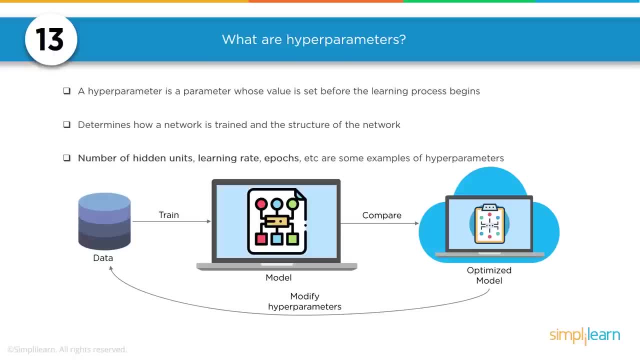 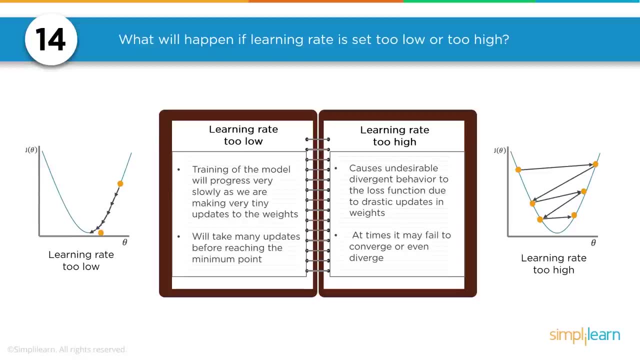 this. this model is pretty good but its biased so and we send it back and we change our hyperparameters to see if we can get it unbiased model or we can have a better prediction on it and it matches our data closer. What will happen if learning rate is set too low or too high? We have a nice couple graphs here. we have one over here says a learning rate set too low At first it's a few. 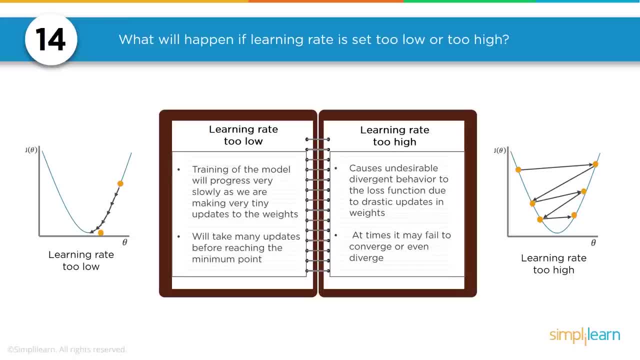 see that it slowly works its way down the curve and on the right you can see a learning rate set too high. it's just bouncing back and forth when your learning rate is too low. that's what we studied in two slides over this: what the learning rate was. training of the model will progress very slowly, as we are. 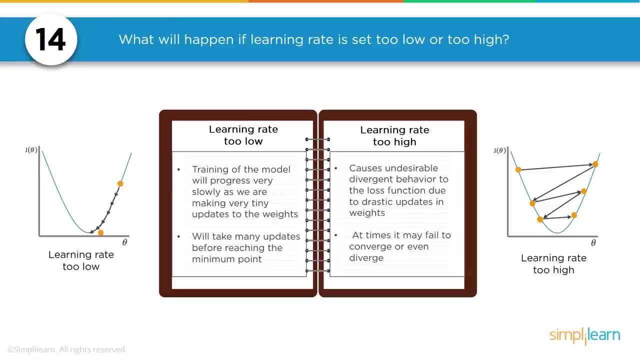 making very tiny updates to the weights. we'll take many updates before reaching the minimum point. so I just mentioned epic going through all the data might have to go through all the data thousand times instead of 500 times for it to train. learning rate too high causes undesirable divergent behavior to the 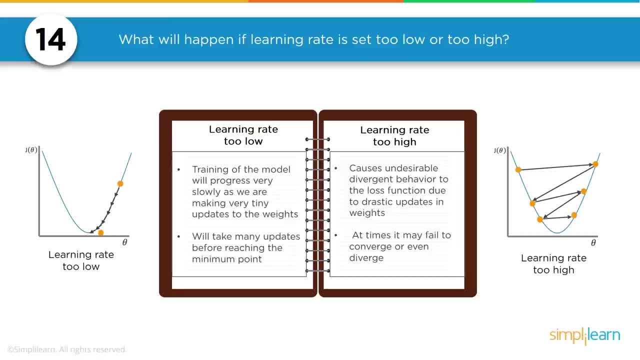 loss function due to drastic updates and weights, at times it may fail to converge or even diverge. so if you have your learning rate set too high and it's training too quickly, maybe you'll get lucky and it trains after one epic run, but a lot of times it might never be able to train because the weights are. 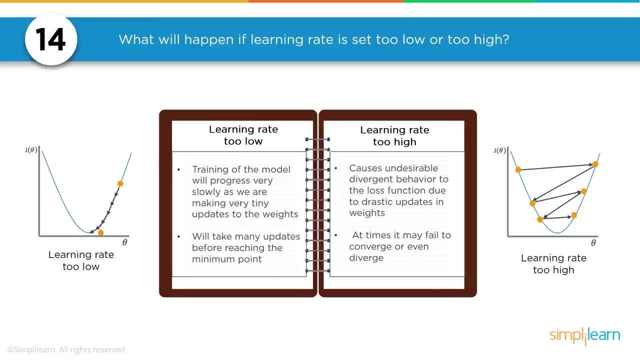 changing too fast, they flip back and forth too easy and you see, down here we've introduced two new terms: converge and diverge. a converge means that our model has reached a point where it's able to give a fairly good answer for all the data we put in. all those weights have adjusted and it's minimized. the 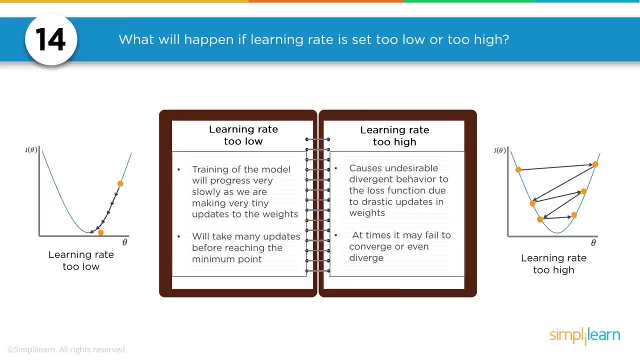 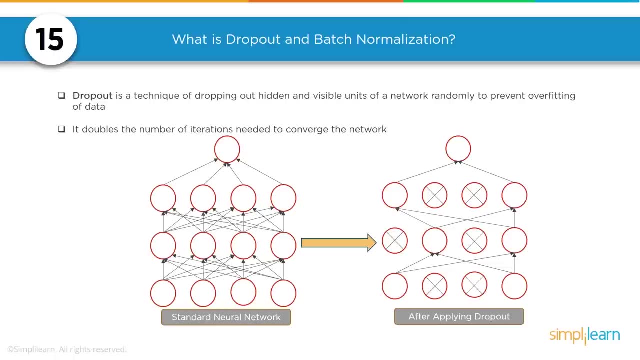 error. diverge means that the data is so chaotic that it can never manage to to train to that data. the data is just too chaotic for it to train. so we have two new words there. converge and diverge are important to know. also, what is dropout and batch normalization? dropout is a technique of dropping out hidden and 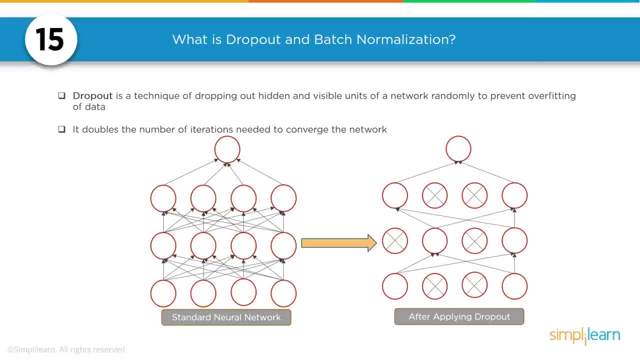 visible units of a network randomly to prevent overfitting of data. it doubles the number of iterations needed to converge the network. so here we have our standard neural network and then after applying dropout- now it doesn't mean we actually delete the node, the node is still there. 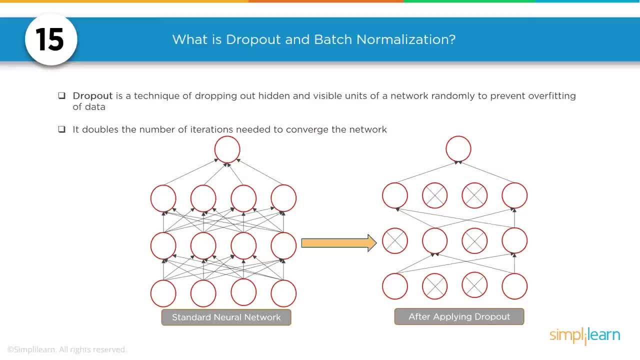 and we're still going to use that node. what it means is that we're only going to work with a few of the nodes a lot of times. I think the most common one right now used is 20%, so you'll drop out 20% of the nodes when you do your training. 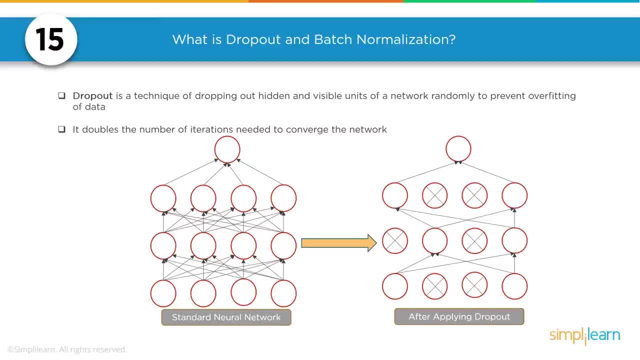 you reverse, propagate your data and then you'll randomly pick another 20 nodes the next time you go through an epic data training. so each time you go through one epic, you will randomly pick 20 of those nodes not to not to mess with, and this allows for less overfitting of the data. 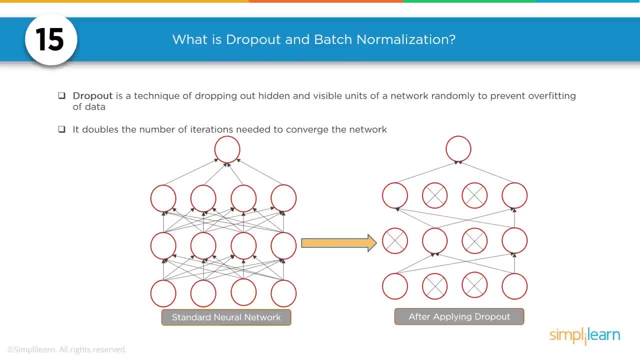 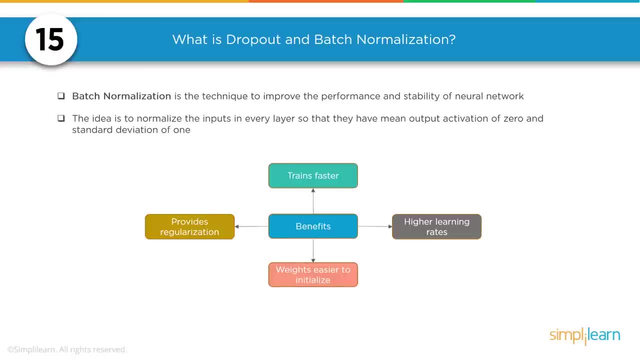 so by randomly doing this you create some. I guess it just kind of pulls some nodes off to the side. it says we're gonna handle the data later on, so we don't over fit. batch normalization is a technique to improve the performance and stability of neural network. the idea is to normalize the inputs in every layer. 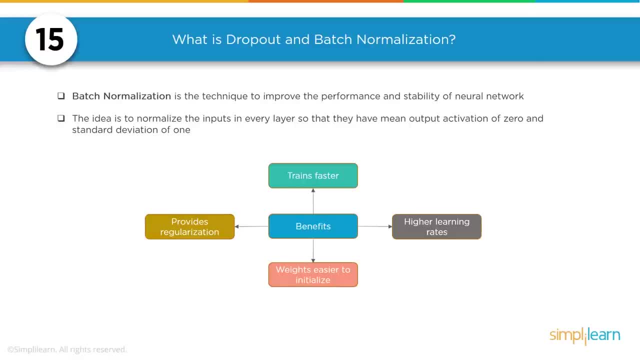 so that they have mean output and activation of zero in standard deviation of one. this question covers a lot of different things, which is great. it's a great interview question because it pulls in that you have to understand what the mean value is. so a mean output, activation of zero, that means our average activation is zero. so when you 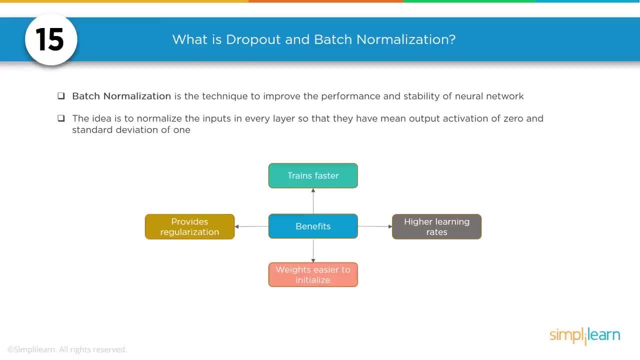 normalize it. remember, usually we're going between minus one and one on a lot of these. it's a very standard setup, so you have to be very aware that this is your mean output activation of zero, and then we have our standard deviation of one. so we want to keep our error down to a. 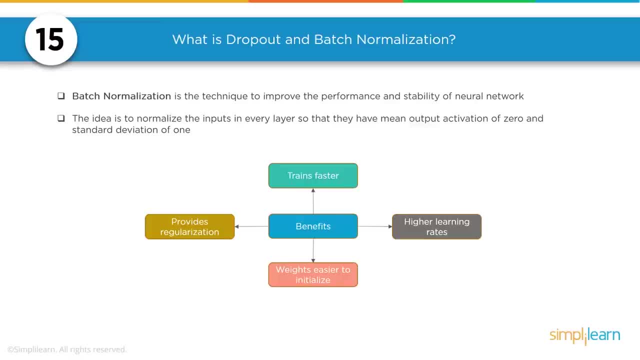 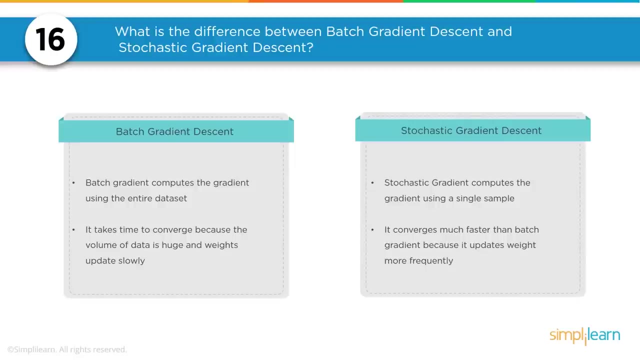 just a one value. The benefits of this doing a batch normalization is it provides regularization. it trains faster, higher learning rates and weights are easier to initialize. What is the difference between batch gradient- descent and stochastic gradient? descent- Batch gradient- descent- Batch gradient computes the gradient using the entire data set. It takes time to. 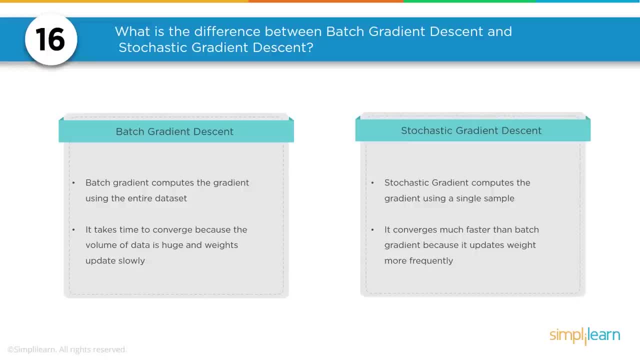 converge because the volume of data is huge and weights update slowly. So you can look at the batches A lot of times. if you're using big data, batch the data in, but you still go through a full epic, You still go through all the data on there. So batch gradient descent means you're going to 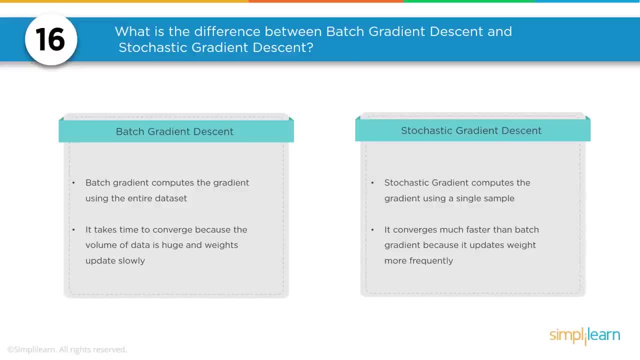 use it to fit all the data and look for convergence there. Stochastic gradient- descent Stochastic gradient computes the gradient using a single sample. It converges much faster than batch gradient because it updates weight more frequently. Explain overfitting and underfitting and how to. 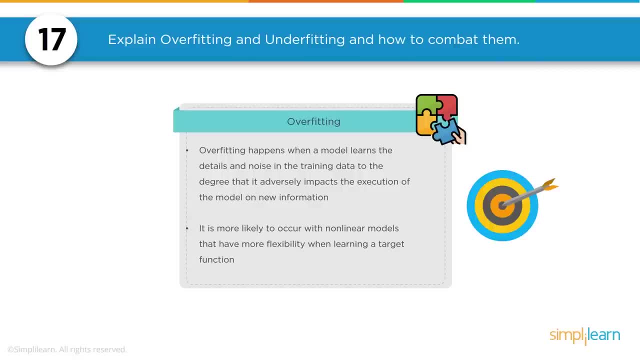 combat them. Overfitting happens when a model learns the details and noise in the training data To the degree that it adversely impacts the execution of the model. on the new information, it is more likely to occur with nonlinear models that have more flexibility when learning a target. 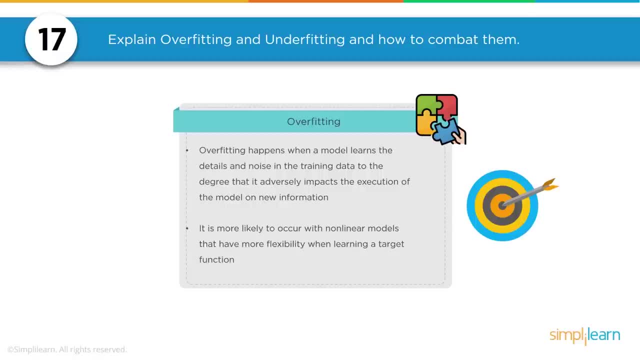 function. An example of this would be: if you're looking at, say, cars and trucks and motorcycles, it might only recognize trucks that have a certain box-like shape. It might not be able to notice a flatbed truck, unless it's only a specific kind of flatbed truck or only Ford trucks, because that's 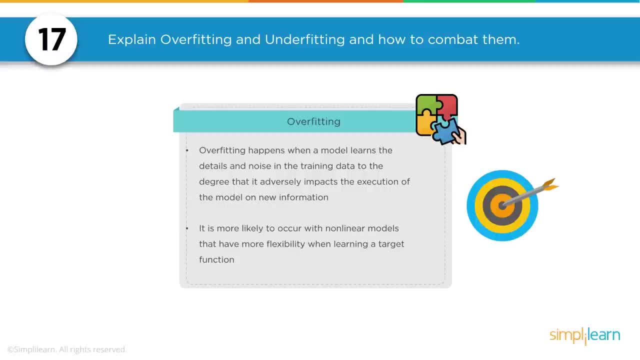 what it saw on the training set. Overfitting performs great on your trained data and great on maybe a small test amount of data, but when you go to use it in the real world it leaves out a lot and is not very functional outside of your small area, your small laboratory data coming in. 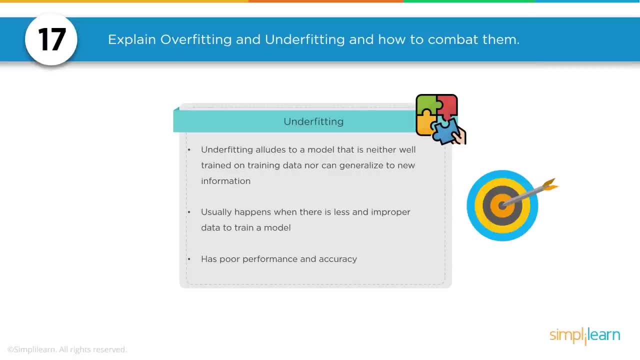 Underfitting, doing the opposite when you underfit your data. underfitting alludes to a model that is neither well trained on training data nor can generalize to new information. Usually happens when there is less and improper data to train a model has a poor performance. 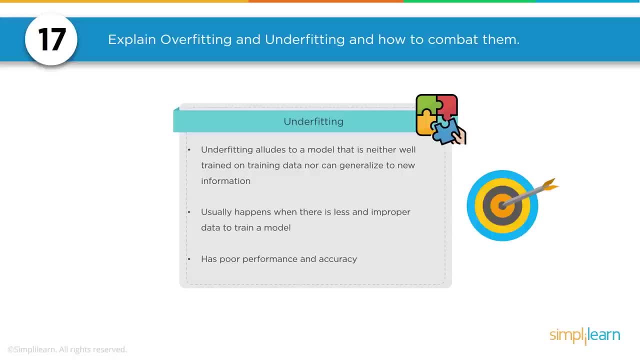 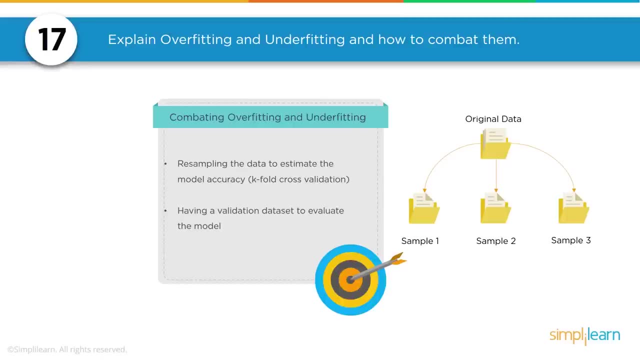 and accuracy. So if you're using underfitted data and you generate a model and you distribute that in a commercial zone, you'll have a lot of people unhappy with you because it's not going to give them very good answers. So we've explained overfitting and underfitting, so now we want to ask how to combat them. 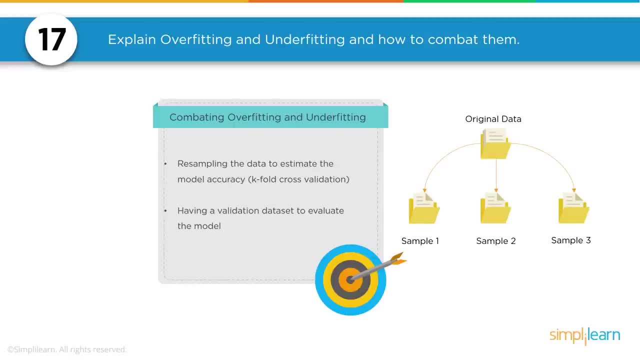 Combating overfitting and underfitting, resampling the data to estimate the model accuracy, k-fold cross-validation, having a validation data set to evaluate the model. So when we do the resampling, we're randomly going to be picking out data and we'll run it a few. 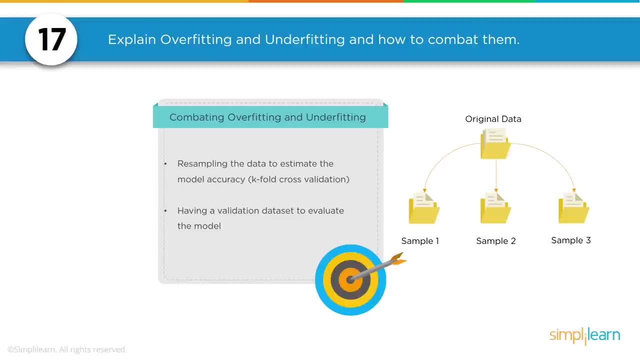 times to see how that works, Depending on our random data and how we sample the data to generate our model. and then we want to go ahead and validate the data set by having our training data and then keeping some data on the side, testing data, to validate it. 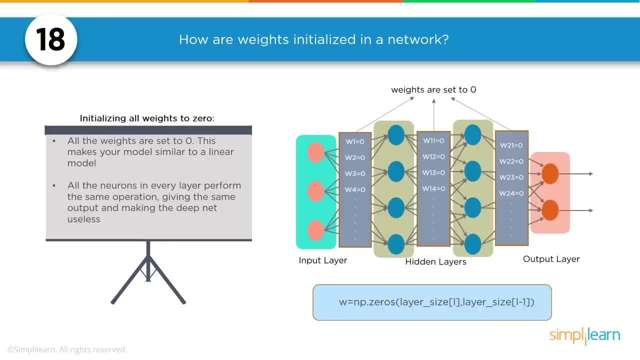 How are weights initialized in a network? Initializing all weights to zero. All the weights are set to zero. This makes your model similar to a linear model. So if you have linear data coming in, doing a basic setup like that might work. All the neurons in every layer perform the same operation, given the same output. 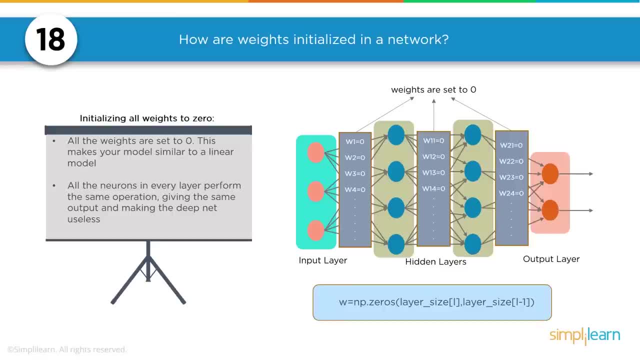 And making the deep net useless. Right there is a key word: It's going to be useless if you initialize everything to zero. At that point, be looking into some other machine learning tools Initializing all weights randomly. Here the weights are assigned randomly by initializing them very close to zero. 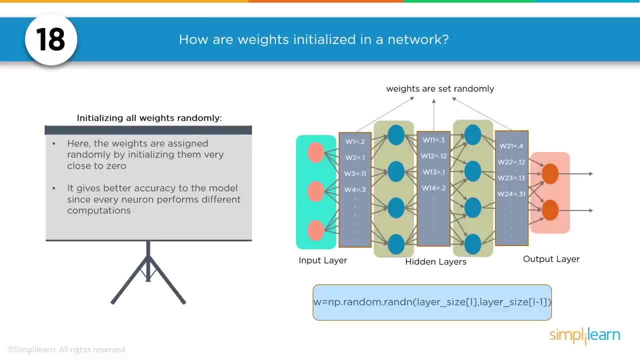 It gives better accuracy to the model, since every neuron performs different computations. And here we have the weights are set randomly. We have our input layer, the hidden layers and the output layer, And W equals NP, random, random in Layer size, L. 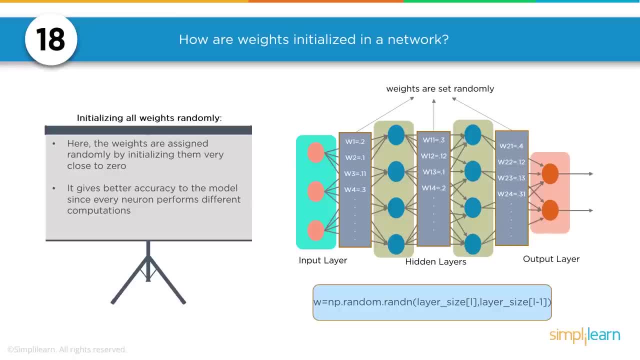 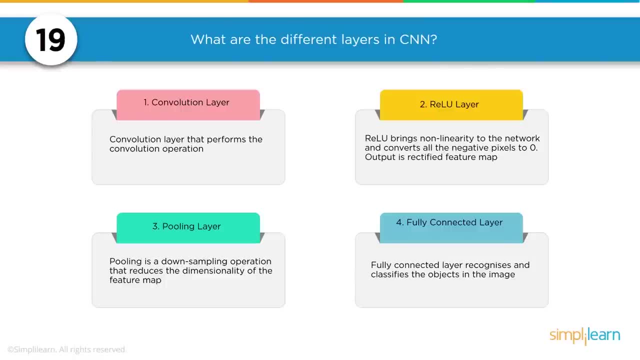 Layer size L minus one- This is the most commonly used- is to randomly generate your weights. What are the different layers in CNN Convolutional Neural Network? First is the convolutional layer that performs a convolutional operation. We have our other video out if you want to explore that more so you can go into detail. 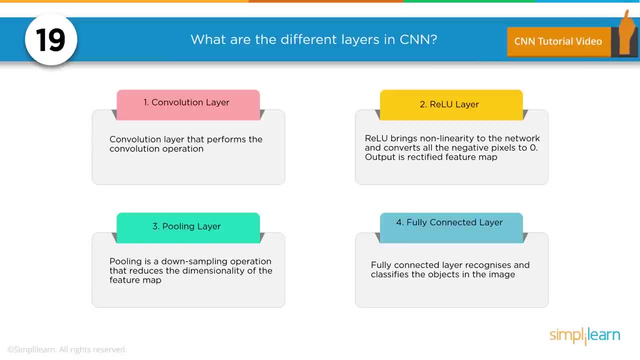 exactly how the convolutional layer works in the CNN as far as creating a number of smaller picture windows that go over the data. The second step is as a ReLU layer. ReLU brings non-linearity to the network. It converts all the negative pixels to zero. 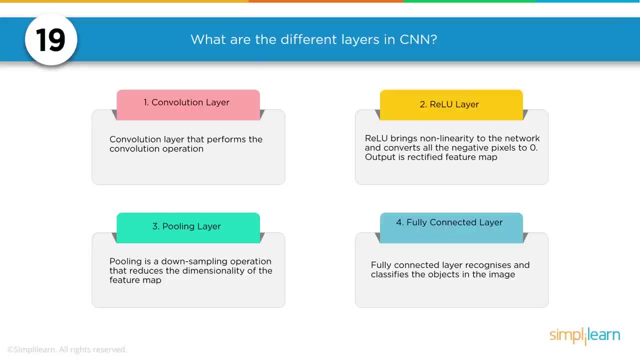 Output is rectified: Feature map. So it goes into a mapping feature there, Pooling layer. Pooling is a downsampling operation that reduces the dimensionality of the feature map. So we have all our ReLU layer, which is pulling all these little maps out of our convolutional 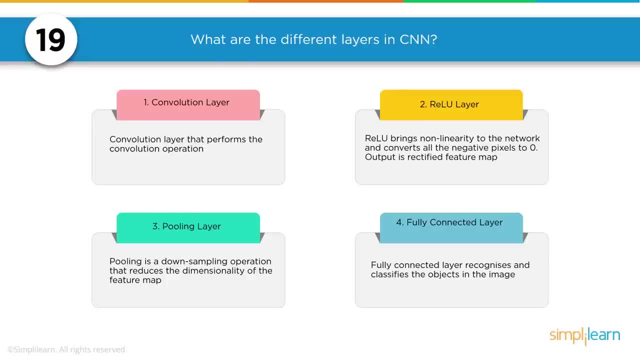 layer. It's taking that picture and creating little tiny neural networks to look at different parts of the picture. Then we need to pool it together And then finally the fully connected layer. So we flatten our pooling layer out And we have a convolutional layer. 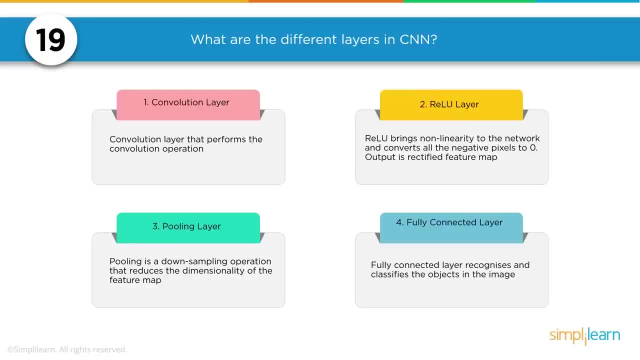 The fully connected layer recognizes and classifies the objects in the image, And that's actually your forward propagation, reverse propagation, training model Usually. I mean there's a number of different models out there, of course. What is pooling in CNN and how does it work? 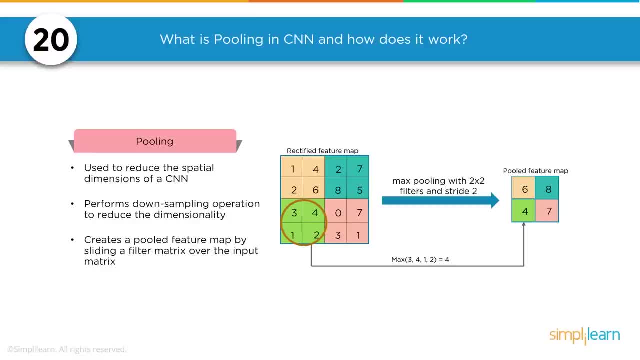 Pooling used to reduce the spatial dimensions of a CNN. performs downsampling operation to reduce the dimensionality. creates a pooled feature map by sliding a filter matrix over the input matrix. I mentioned that briefly on the previous slide. Um, You know that you have. 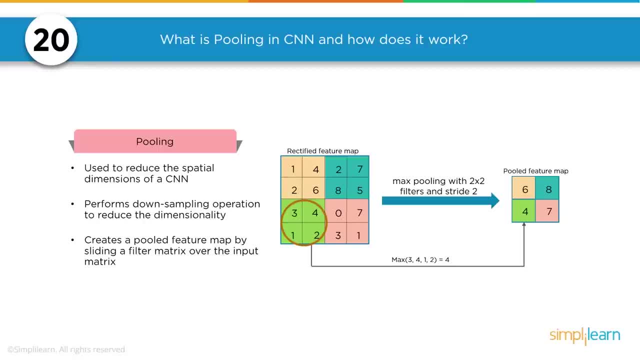 If you can see, here they have a rectified feature map And so each one of those colors- like the yellow color That might be one of the smaller little neural network- using the ReLU You'll look at. You'll just kind of go over the main picture and look at all the different areas on the 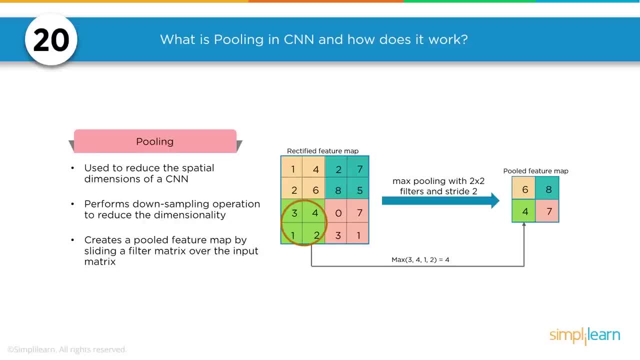 main picture. So you might step one, two, three, four spaces, And then you have another one that's also looking at features And it has a two, seven, eight, five. Each one of those is a map. So it might be the first one might be a map looking for cat ears. 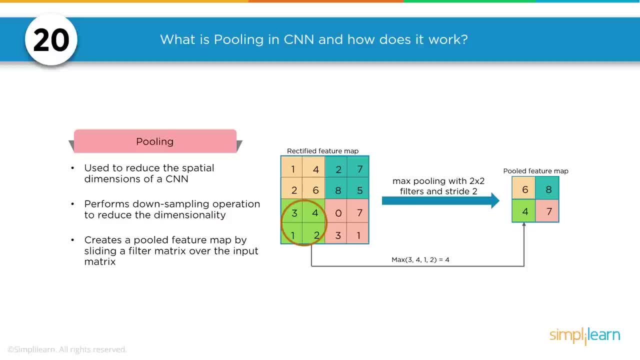 The second one, looking for human eyes. When it does this. you then have this rectified feature map looking at these different features And the max pooling with a two by two filters and a stride of two. Stride means, instead of skipping every pixel, you're going to go every two pixels. 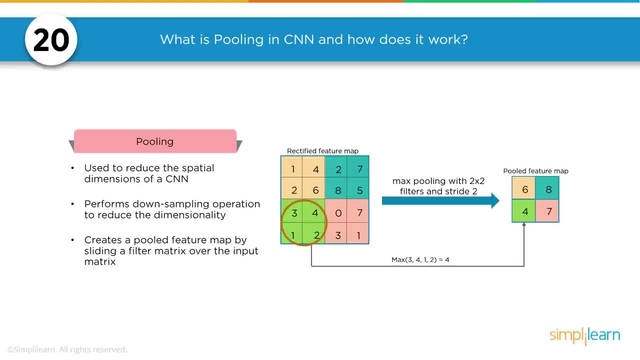 You take the maximum values And you can see. over here we look at a pooled feature map. One of the features says: hey, I had a max value of eight. So somewhere in here we saw a human eye labeled as eight. Pretty high label. 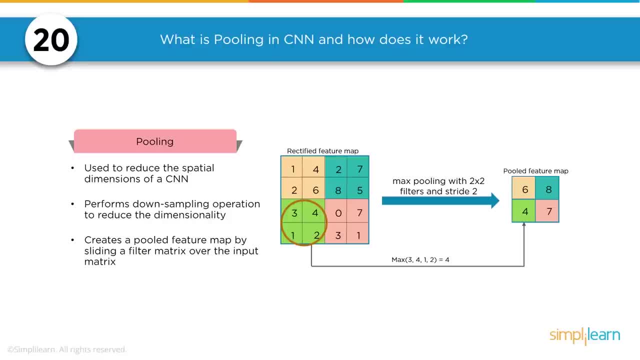 And maybe seven was a human hand And maybe four was cat whiskers Or something that we thought might be cat whiskers. Four is kind of a low number in this particular case compared to the other ones. So you have your full pooled feature map.